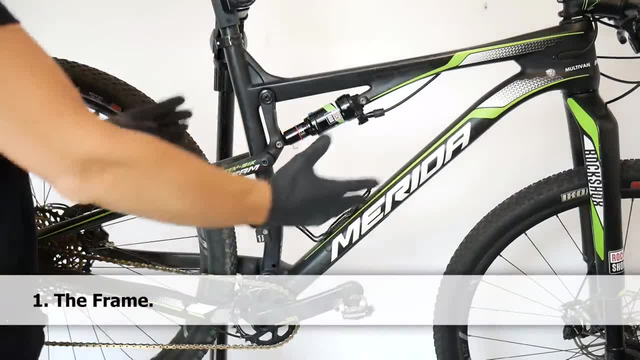 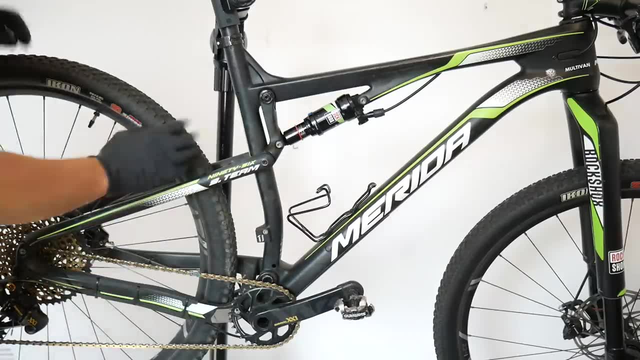 We'll start maintaining our bike from the frame, because this is the sole of our bike. We attach anything else to the frame, like the components, the wheels, the seat post and our handlebars, So we can replace the wheels, we can replace the groups that we are using. 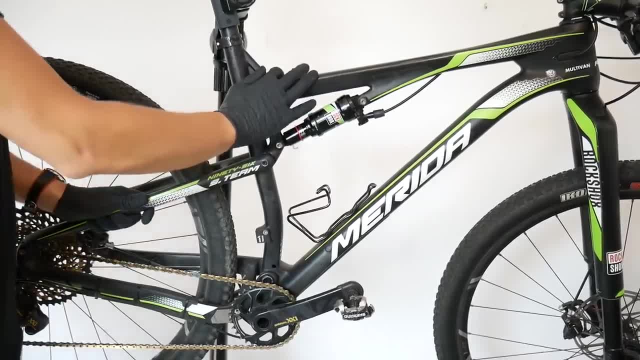 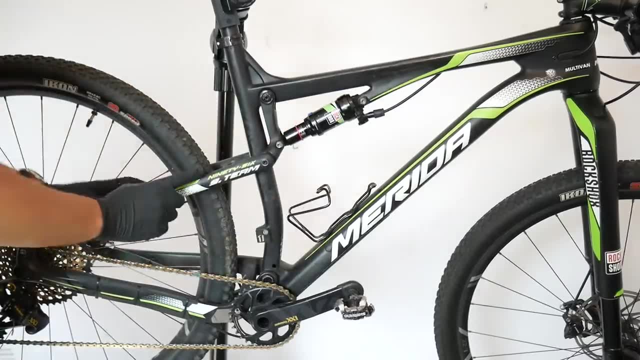 but the frame will stay with us and this is the sole of the bike. That's why it is really important to take good care of this chassis, of our whole machine. So we'll start the inspection By looking at any damages of the frame. 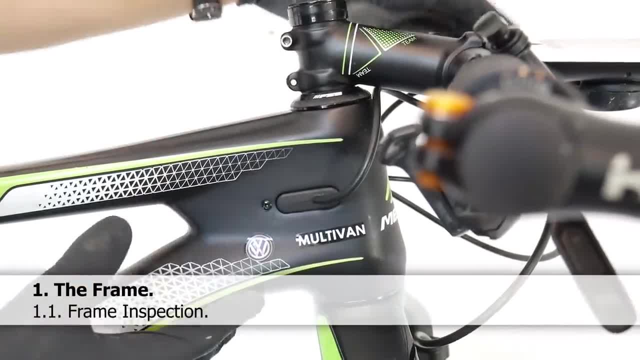 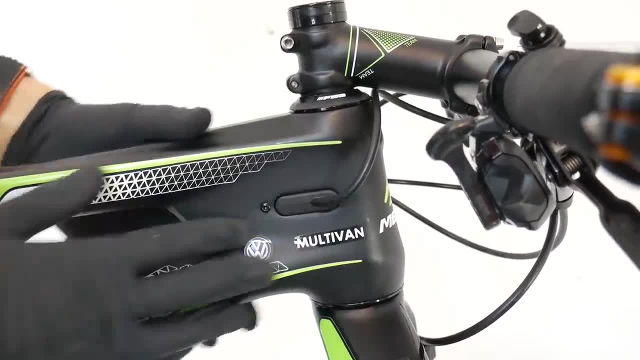 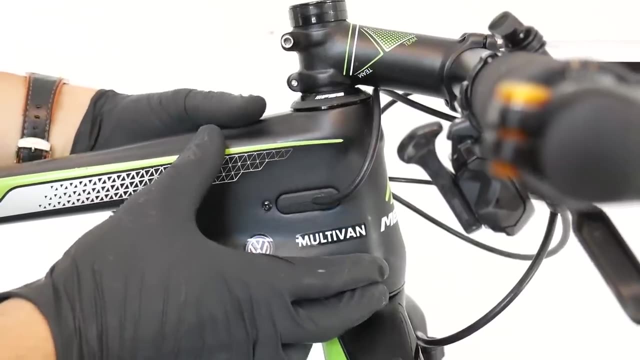 Great opportunity to check and inspect the frame is the bike wash. So while we are washing the bike, always looking for some new scratches or imperfections on the paint, We can find some places which could be damaged. One of the areas of our frame which we should inspect regularly is the head tube, or now, on the modern bikes. 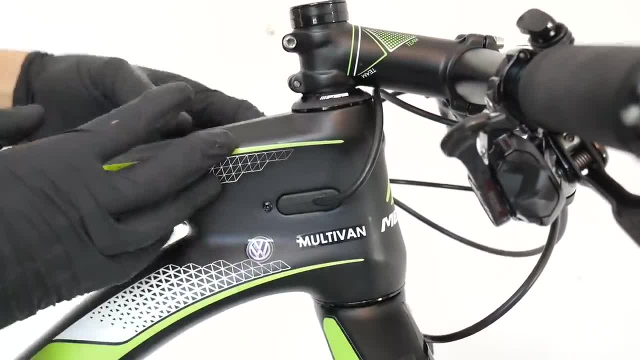 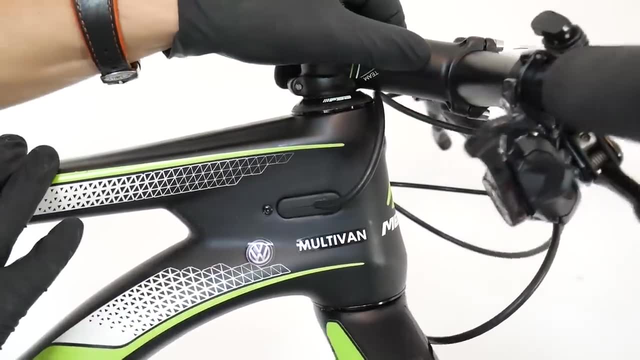 this huge head box because it transfers a lot of forces from the bike, From the fork, from the wheel, from the fork to the other parts, like the top tube and the main tube of the frame. One place where a crack may occur, for example, is right here: the bottom surface of the head tube. 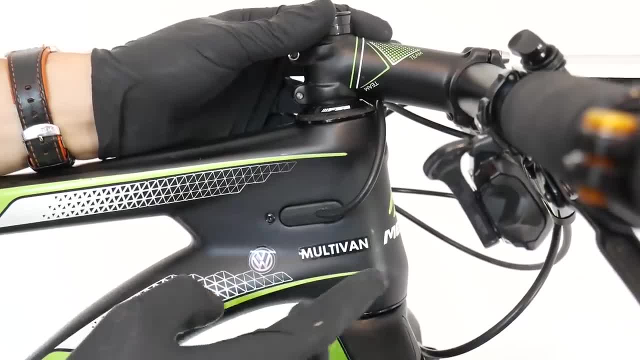 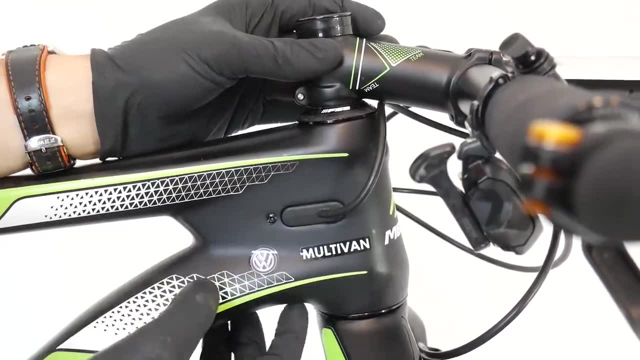 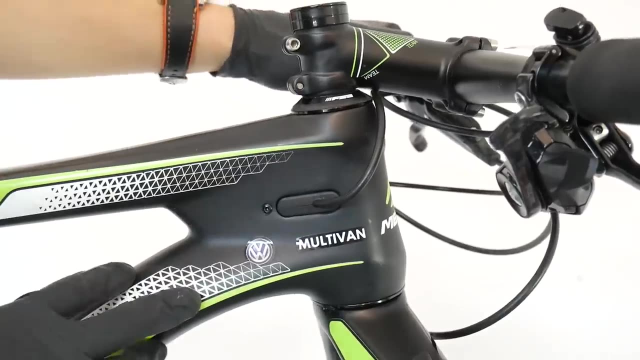 So look for any damages there. If you react pretty quickly to some small cracks- if this is the carbon bike- you sometimes may be able to repair the frame, which would be awesome instead of simply buying a new one. Another thing that we should take care of is the housing rubbing against the frame. 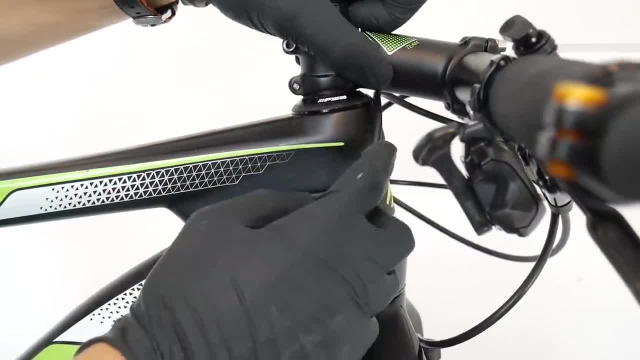 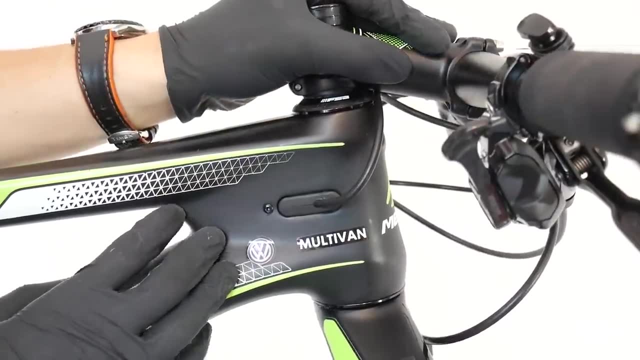 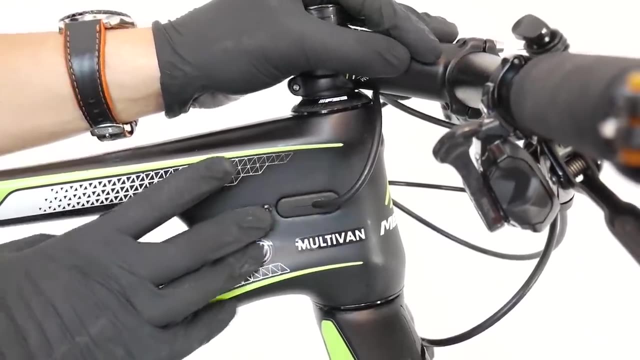 As you can see, on many bikes, like on this one, the housing will not actually touch the frame, so that we don't have to put any additional protection just to protect the paint of the frame. But as you will see in a second, there was some place, one place on the fork- which I did have to protect. 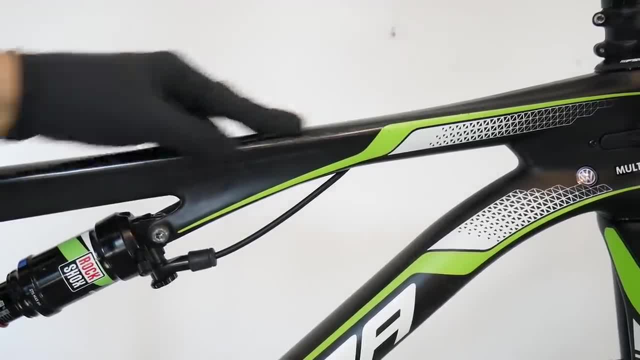 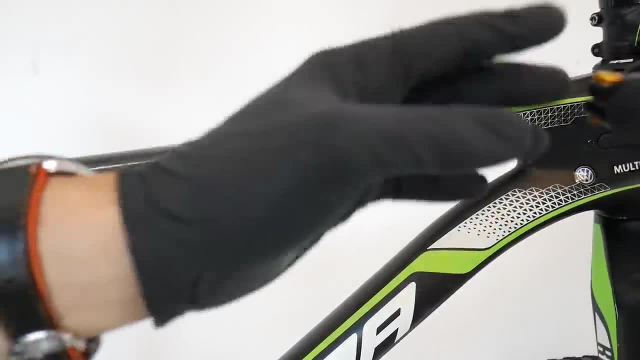 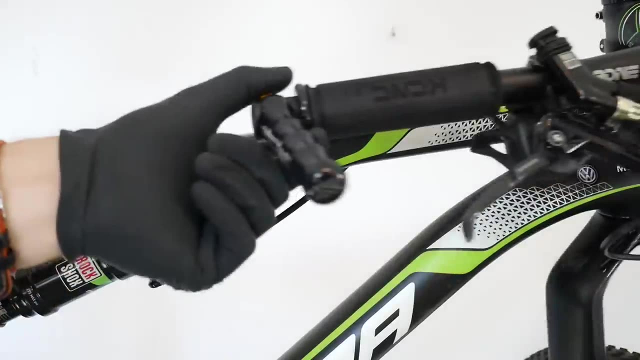 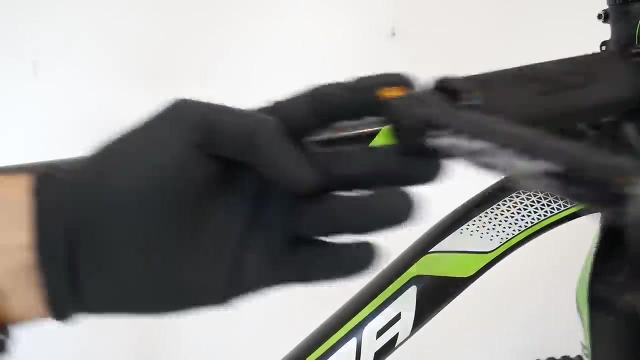 The next area we want to inspect is the top tube, especially where the handlebar can touch it or can actually damage it. On my bike, there is the shifter that touches the top tube, not the handlebar. but especially when we crash, which really happens quite often for us. 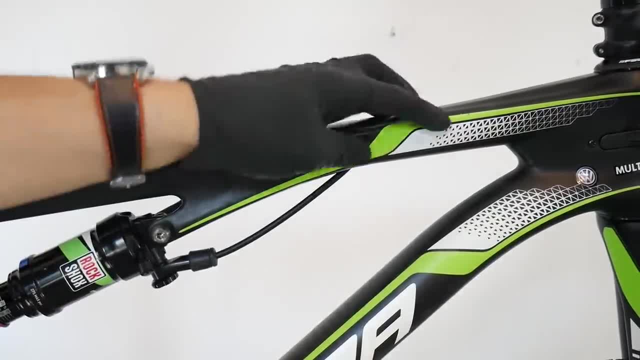 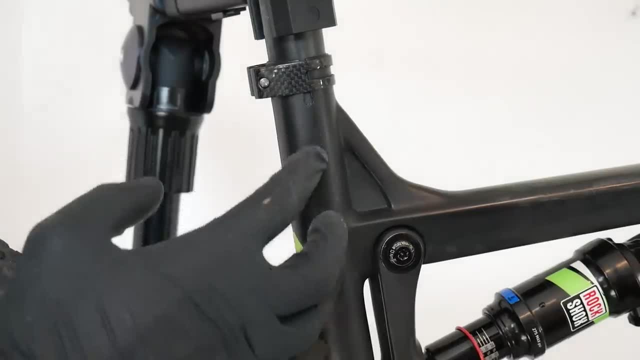 the handlebar can damage the top tube, so inspect this area regularly. Here's the next area, that's the joint between the top tube and the seat tube, because in the seat tube we have our seat post. on the seat post there is our saddle. 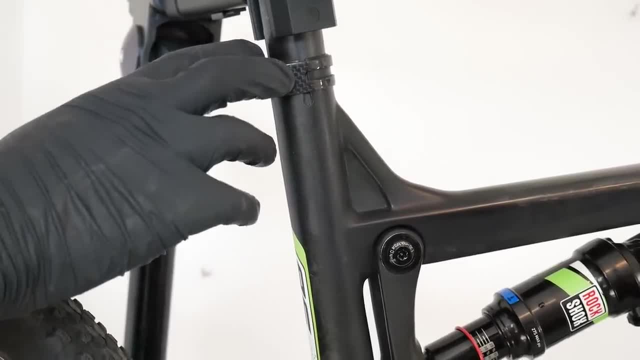 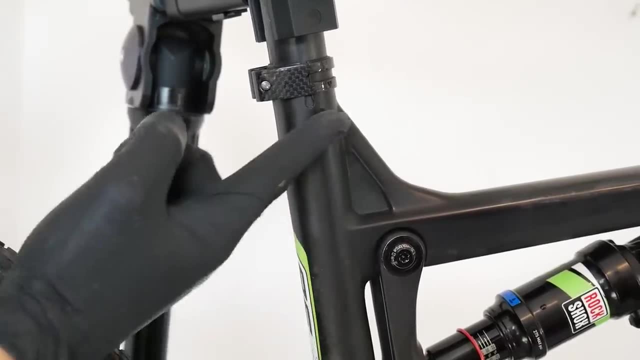 and sometimes we just jump on the bike with the whole weight of our body. sometimes we go through some bumps in the terrain sitting on the saddle and some cracks may occur right here. So on the carbon frame, just inspect the whole area. 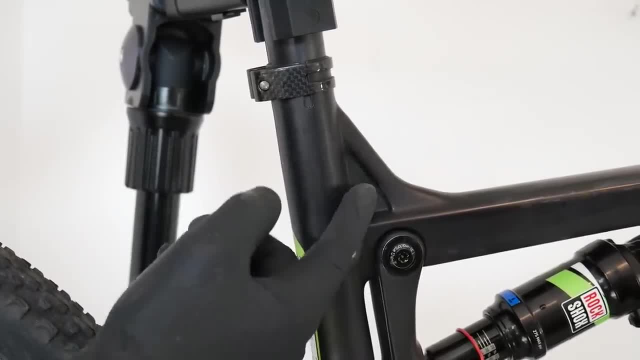 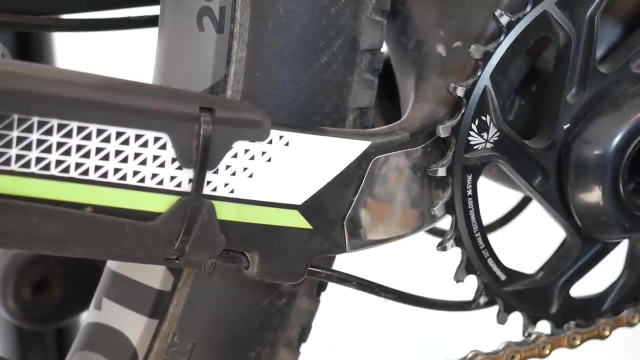 on the alloy or steel frame you should inspect, especially all the welds. Here's the next area we should inspect. that's the area of the chainrings on our crankset. it happens to be here. Here's the next area we should inspect. that's the area of the chainrings on our crankset. 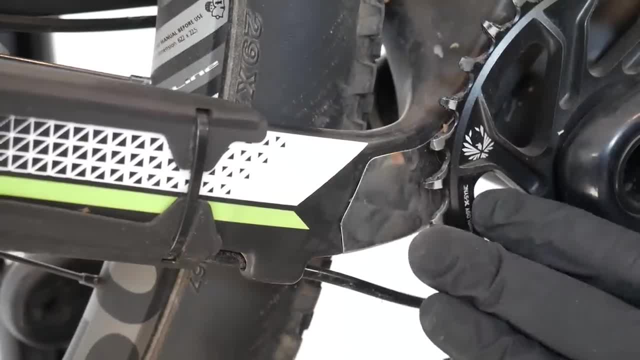 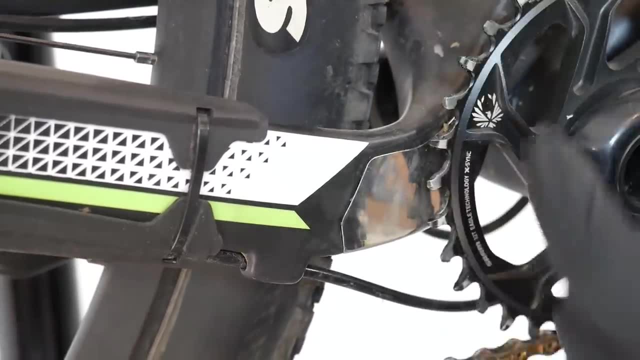 it happens to be here. Here's the next area we should inspect, that's the area of the chainrings on our crankset, especially in the muddy terrain somewhere on the trails, even on the new drivetrains that we have our chain dropped between the chainring and the frame. 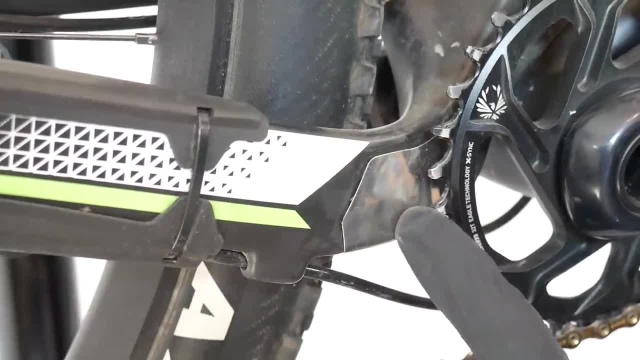 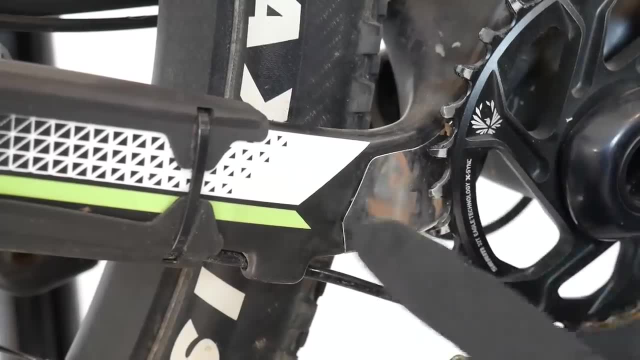 or it will be sucked in between right here. Then some serious damage can occur. make sure there is no damages here and also make sure that there is some really good protection on the surface of this area, on the frame, even if it's. 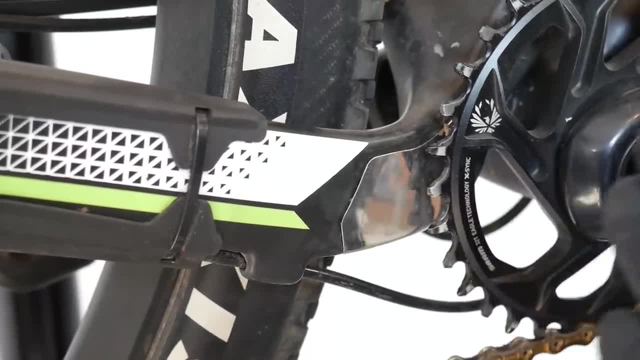 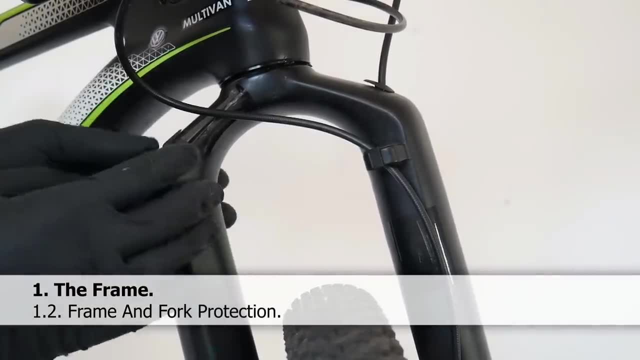 an alloy. it's not only for carbon alloy frames, steel even frames. it's good to have this kind of protection here. What areas of the frame should we protect? I would say protect anything that will have any contact with the housings or with the chain of your bike. 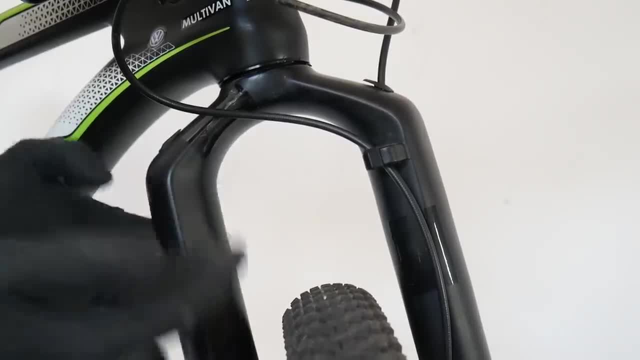 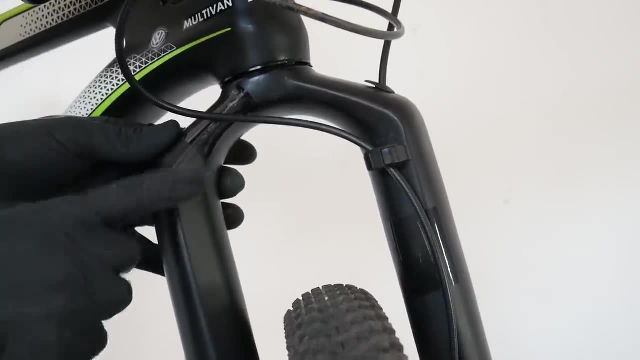 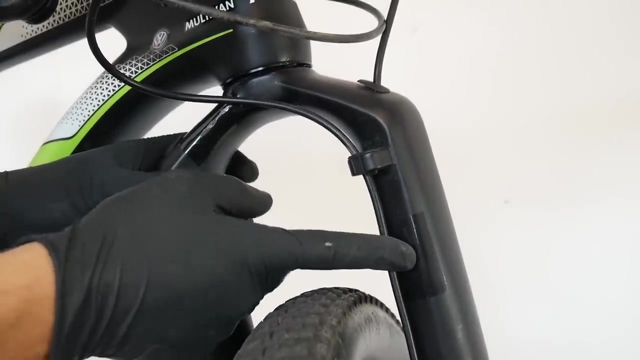 so the chain stays on the drive side, that's for sure. The only place or area where I found some rubbing the housing, rubbing against the bike, was the fork. that's the crown here and that's some area on the left side of the fork. 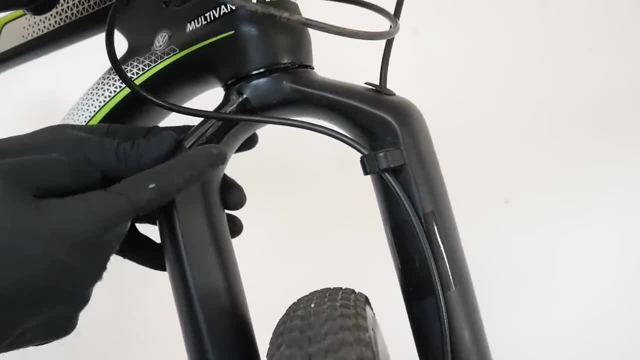 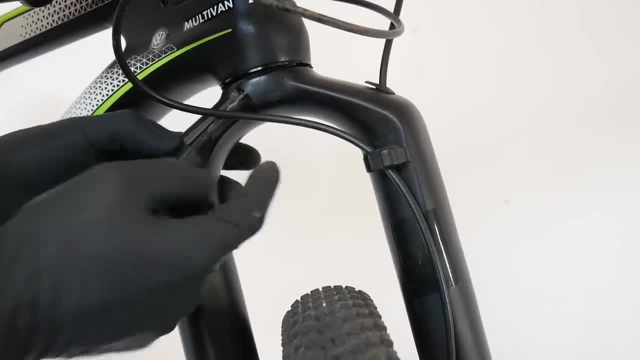 I just used some regular tape for this which is not specifically designed for it. If you buy some special protection for the frame, it will be thicker, it will last longer. but also at the edges of those thicker stickers there may be some dirt. 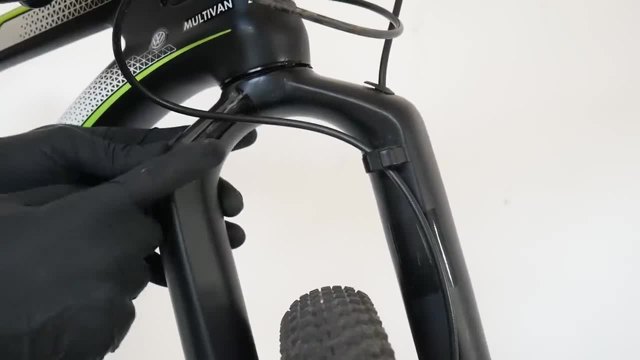 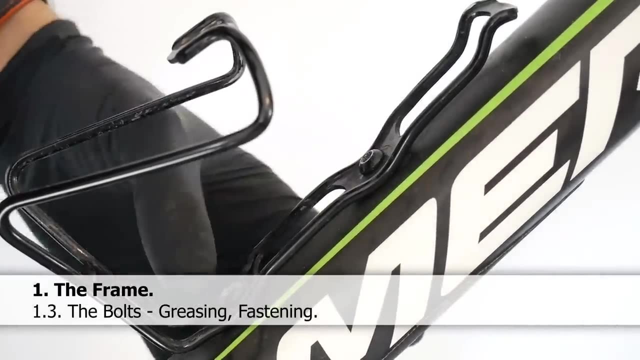 just looking not very nice, so I'm using just the thin one and I'm replacing it regularly. These are the bolts that assemble the bottle catch to the frame. We also have such a small bolts assembling, for example, fender and racks. 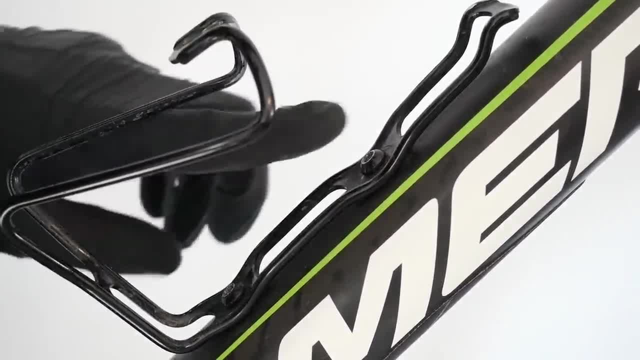 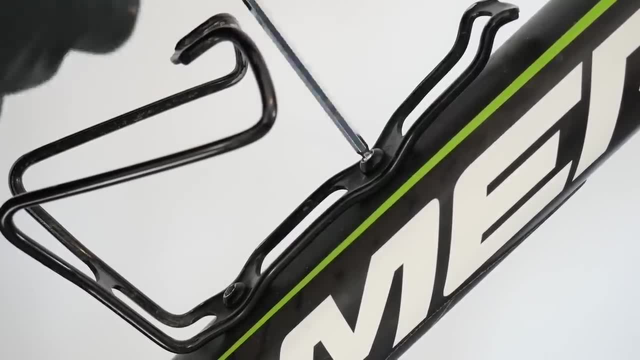 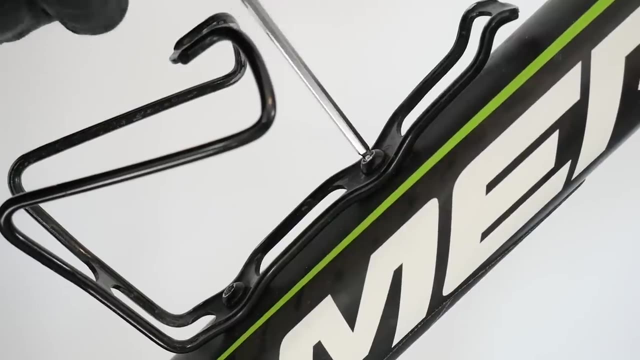 and also the derailleur hanger to the frame, and these are not the ones we would use very often. that's why, at least once in a year, I would just check those out, clean the threads, put some grease and make sure those will be just fastened as they should be. 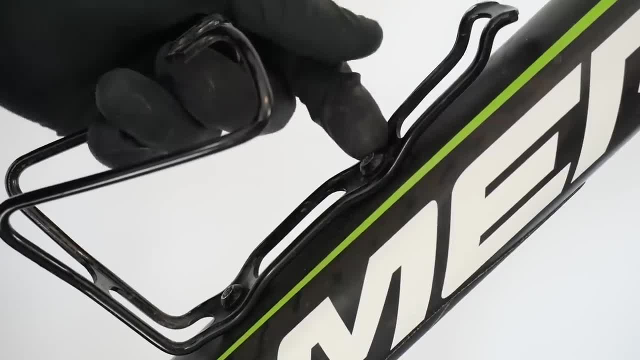 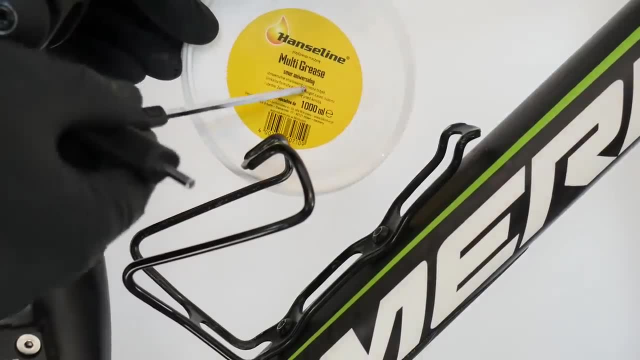 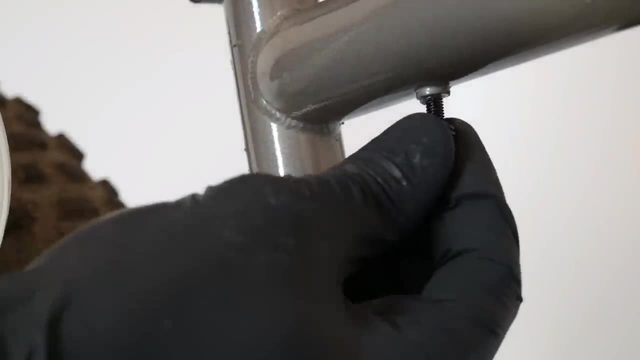 so that we don't lose it and we also don't damage them when we try to unthread the bolt, which has been there for years and it's really rusty. some multi-purpose grease will be just fine. for that reason, we just put a little bit of the grease on the clean thread of the bolts and then we can. 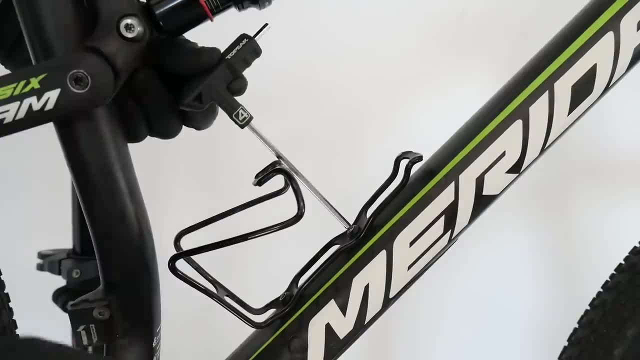 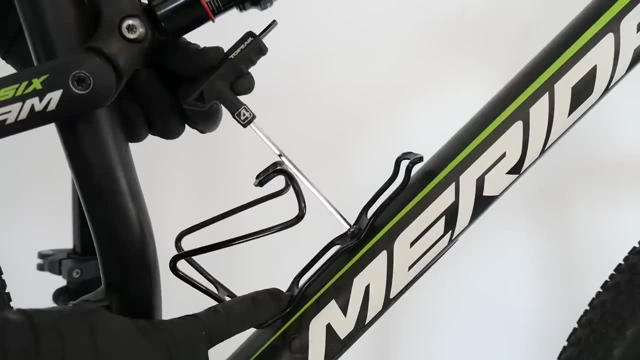 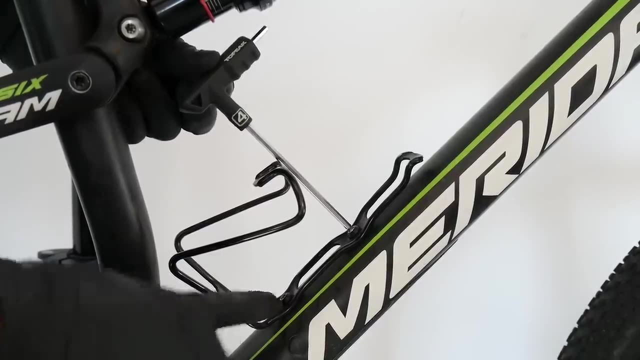 thread those in. the other thing we should remember about is not to over tighten those balls. normally you should have those info on the manual of your bike. but these little balls, like for the bottle cage, should need just about two or three newton meters of your force. so if you do not use the 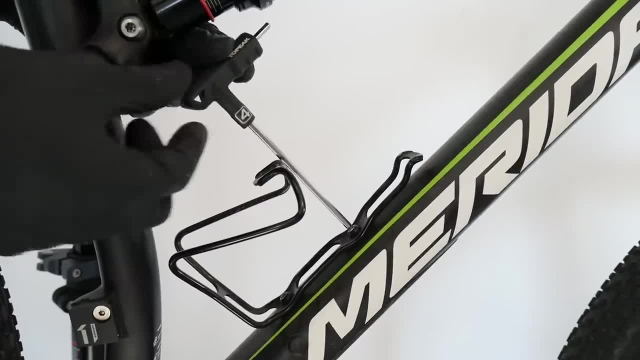 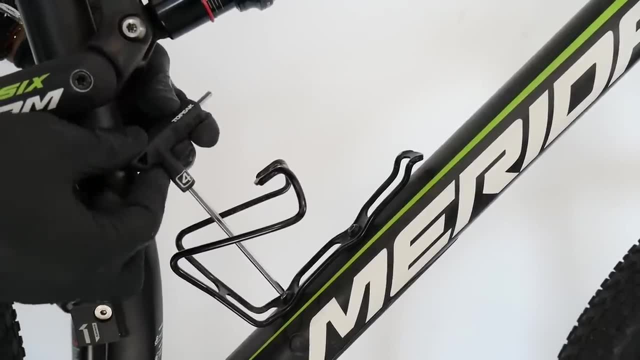 torque wrench, i would hold the alan key by the shorter arm and then you can be sure you're you're not gonna use too much force while threading those in. after some months or years of using your bike you can find out how much force you need to thread in your bike and then you can find out how much. 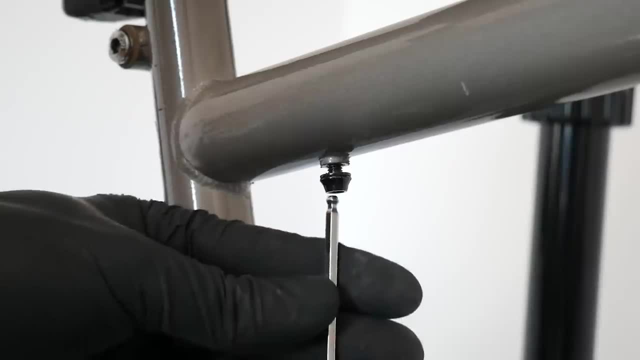 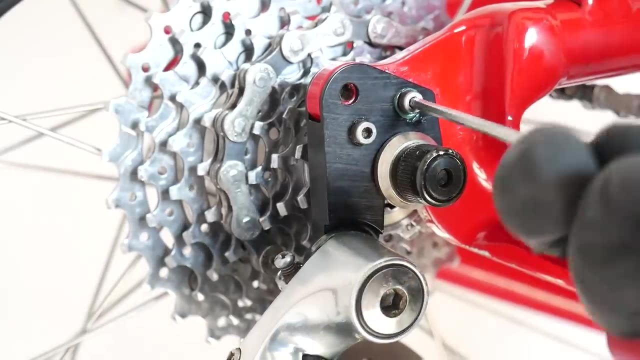 force you need to thread in your bike, and then you can find out that you're just about to lose some of those bolts. so make sure you pay attention to those at least once a year. if these two little bolts that will assemble the durella hanger to the frame are loosened, the hanger can move around. 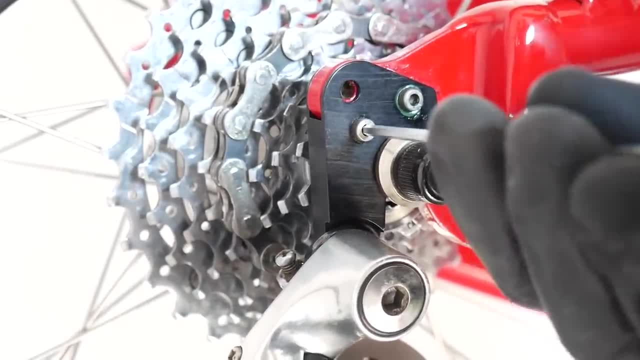 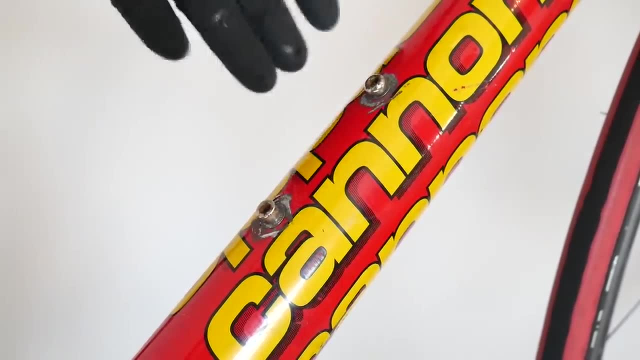 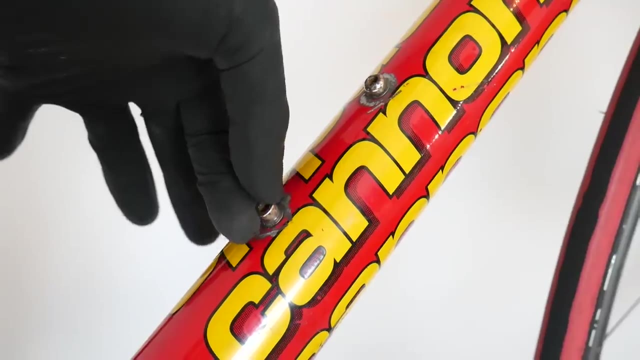 a little bit and also the shifting performance will be not as good as it should be. if you don't clean and grease your your bolts from time to time, maybe once a year, you can cause a very serious problem like this one. here the thread on the frame is loosened because 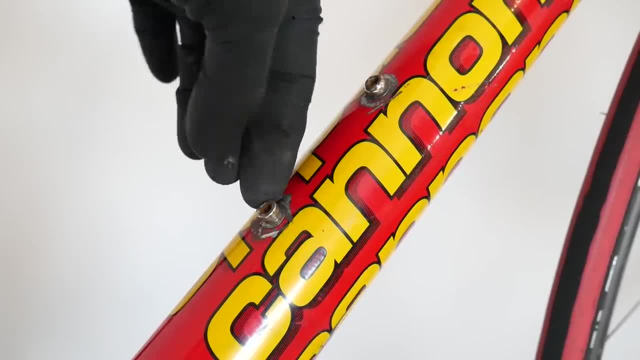 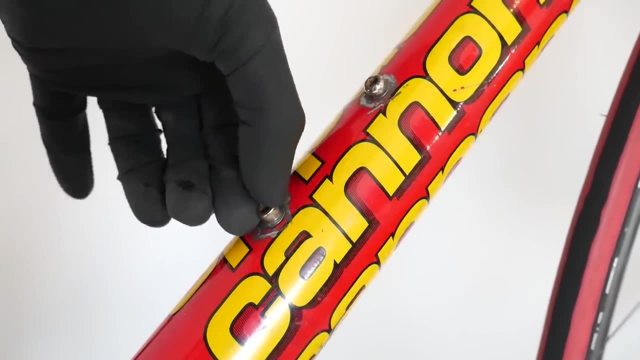 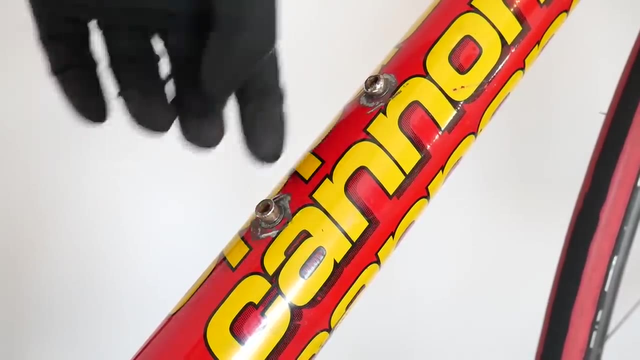 this bolt was rusty and somebody had to use a lot of force in on in order to unthread the bolt, and so the thread in the frame wasn't able to to withstand that force and it's losing now. so now we have to fix the frame. another important area of our frame is the seat post clamp. 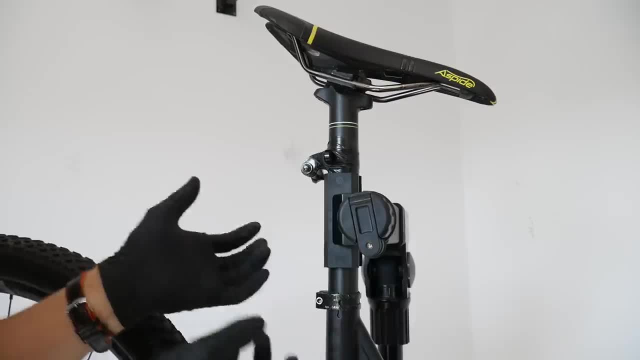 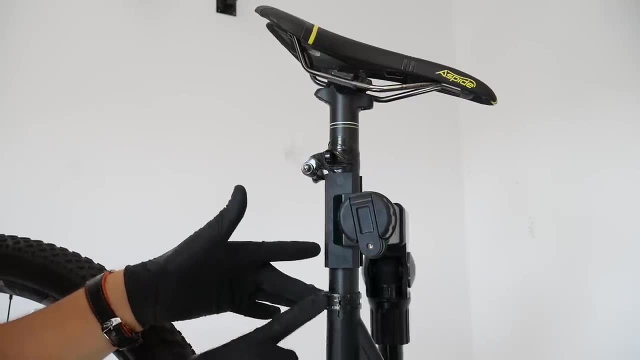 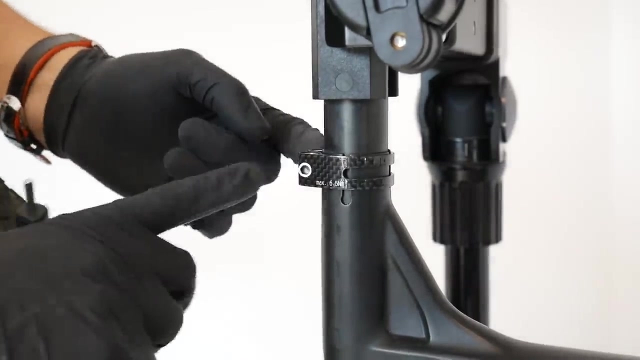 if the seat post clamp will not be fastened strong enough, well enough, the saddle will be just slipping down during our ride. if we over tighten this bolt, we can damage the frame or the seat post. it is very good idea to check from time to time whether the bolt is pretty clean and also clean. 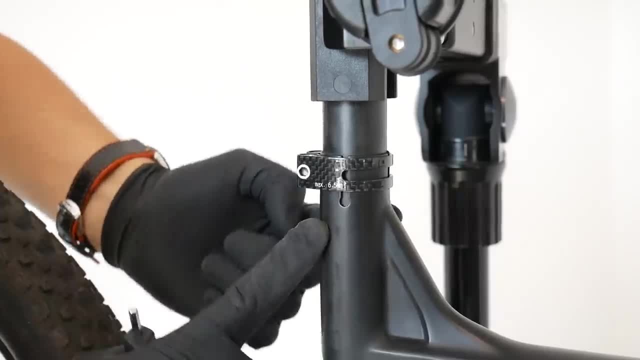 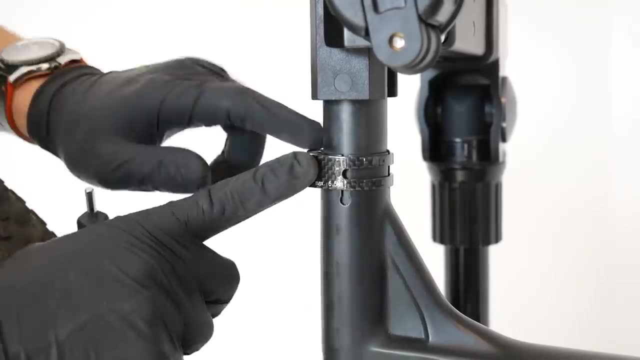 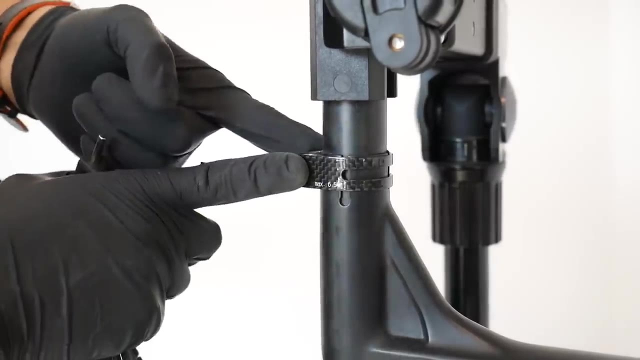 the surface between the seat post clamp and the frame. if it was not the carbon frame, i would also use a little bit of a grease just in between the seat post clamp and the frame. it will make for the seat post clamp easier to fasten just around the frame. now we should tighten the bolt. how do we do? 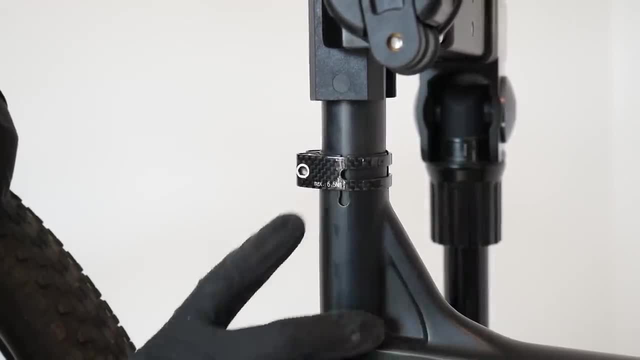 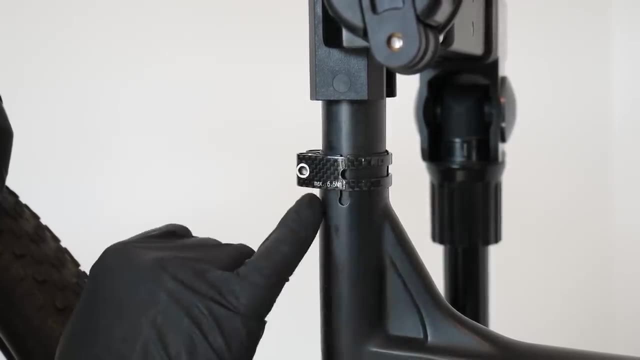 it. on almost each of of those seat post clamps on your bikes there will be some torque um just written by the manufacturer. here we have the maximum torque- six and a half newton meters, since i've used some special paste for the seat post clamp, and now this is the maximum torque- six and a half newton meters, since i've used some special paste. 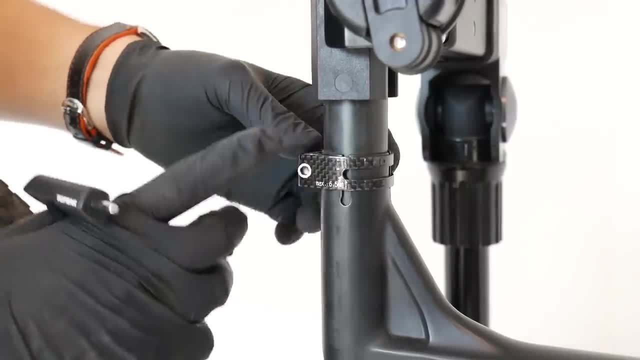 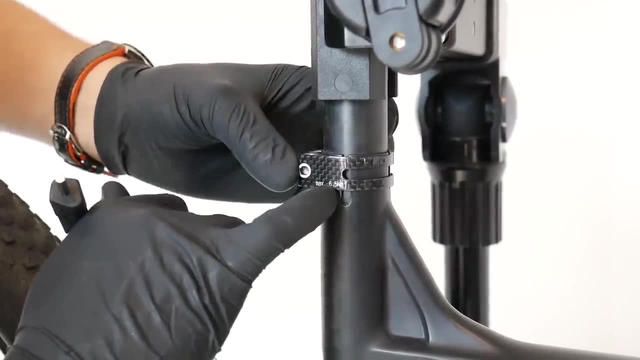 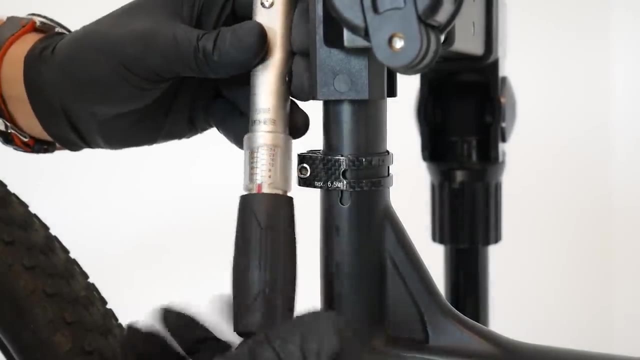 Just on the seat post. that will increase the friction between the seat post and the frame. I can use some lower force, So I'm gonna use, let's say, just below six Newton meters. I'm using a Torque wrench for this reason, So let's just set. 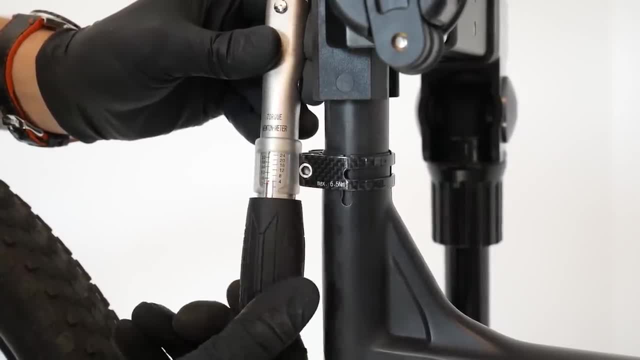 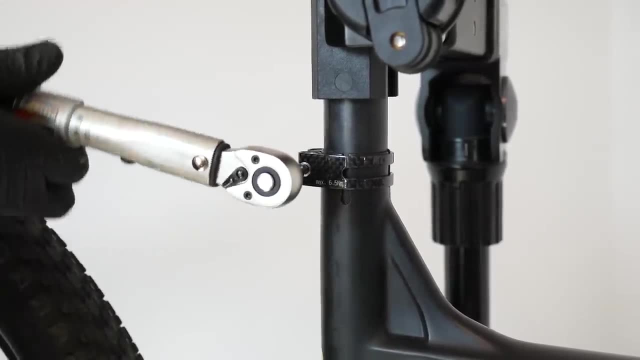 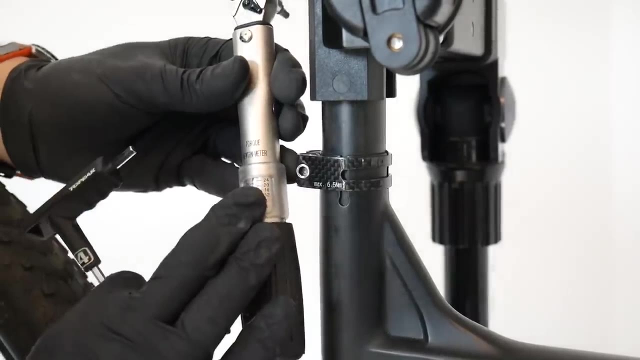 just below six Newton meters, It's still pretty much. I would say. That's it, it's done. If you don't have a torque wrench, it is really good idea to go to your local store and ask them to do it for you If you have to do it by hand. 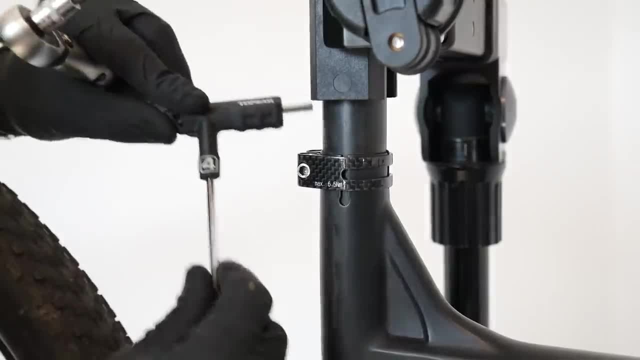 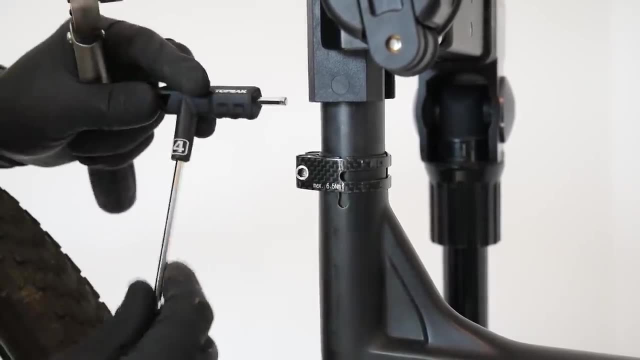 really try to feel well that you are not over tightening the bolt, which can be a difficult thing. Six Newton meters, Well it's, It's pretty much, I would say. But if you over tighten the bolt it's gonna be a little bit more difficult. 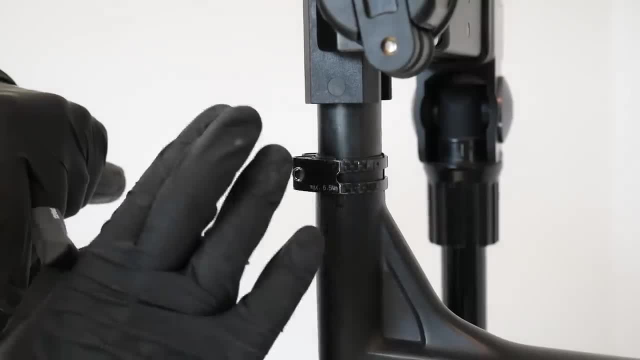 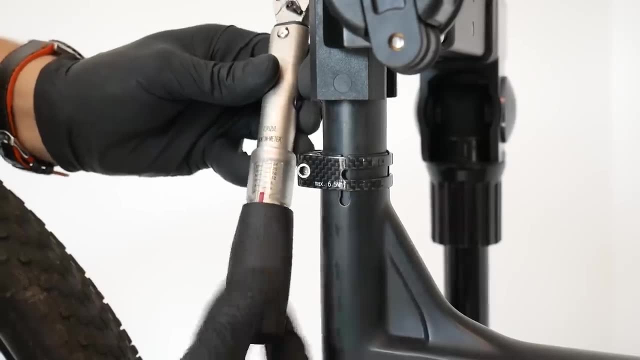 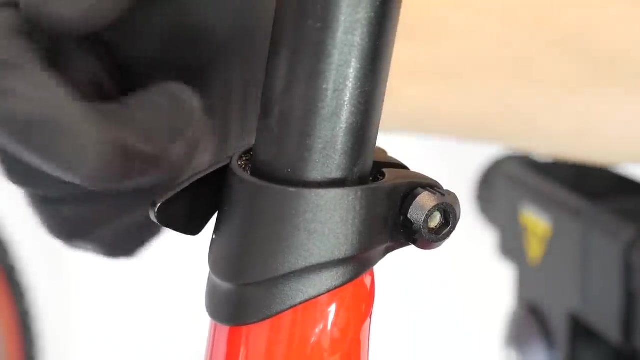 But if you over tighten the bolt, If you over tighten this, it can really cause some damage. if you use the torque wrench, Remember about setting it just back to the zero Position so that you don't have to calibrate it. Some seat clamps have really smart design with the quick release. 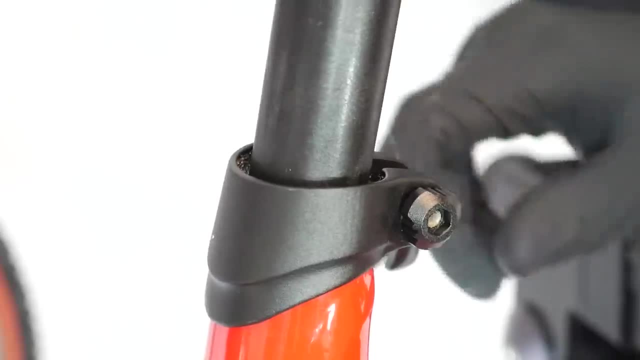 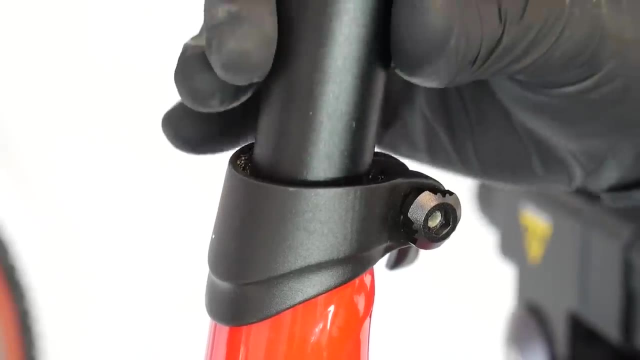 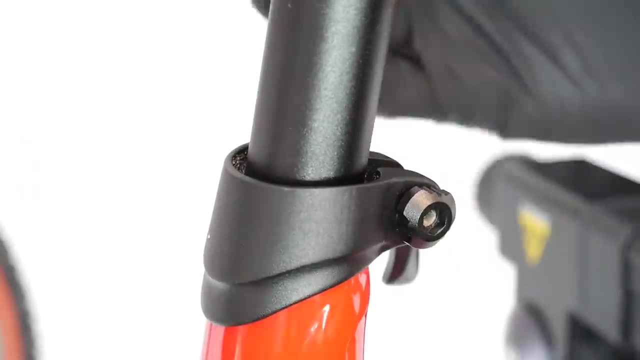 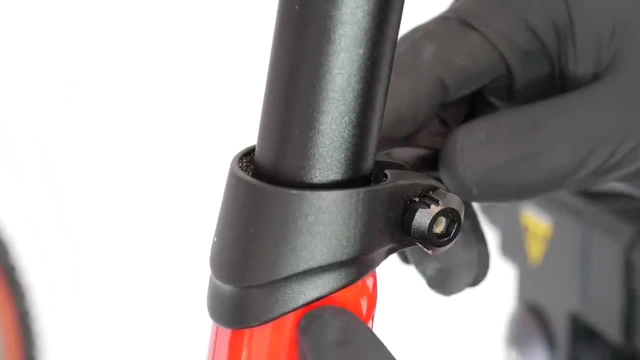 That means we can open our Seat post somewhere on the trails if we want to go on some steep descents And lower our seat. that's possible without using Any tools. in this case, we should remember the same things: having our screws clean and Greased, having grease between the seat clamp and the frame, if it's not a carbon frame. 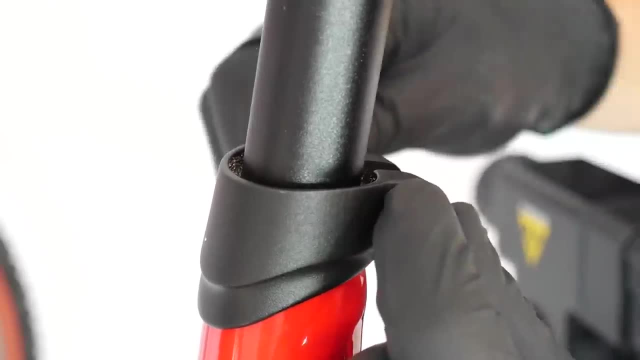 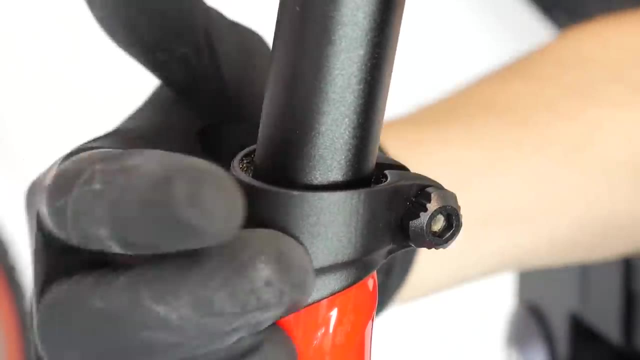 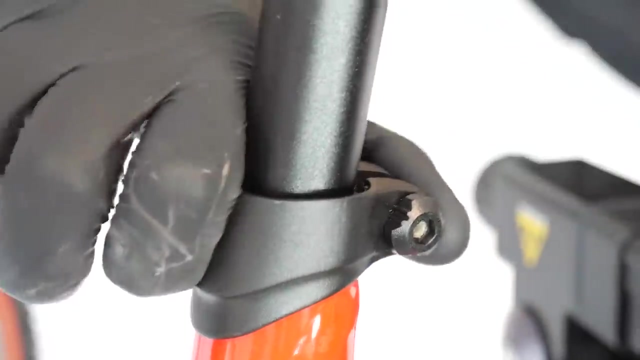 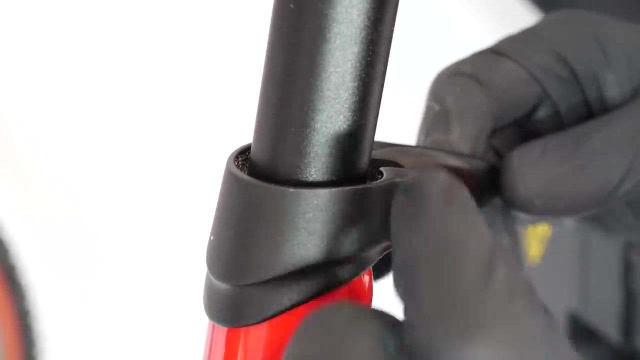 We do not put the grease on the carbon frame and also The the surface where the lever is Rubbing or pushing against the seat clamp. There should be some grease as well. It will make Closing it and opening it much easier. Another thing we should remember about in this case is this little micro adjustment. if this bar adjustments, if you will- is. 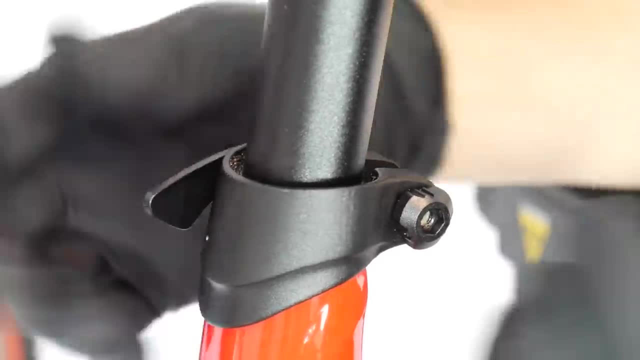 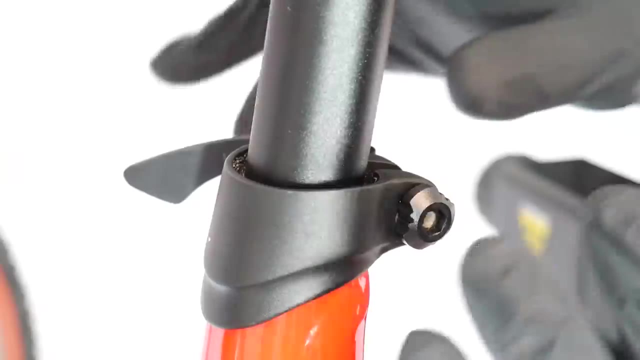 Opened too much. the quick release won't clamp our seat post Just strong enough, So we should find the right spot for it. for it, The rule of thumb is to Set this bar adjuster so that, so that we will start to feel some resistance. 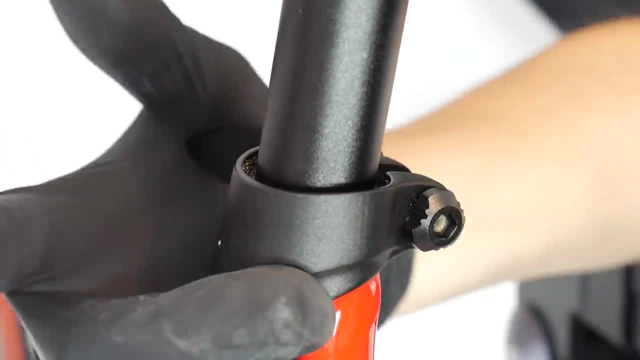 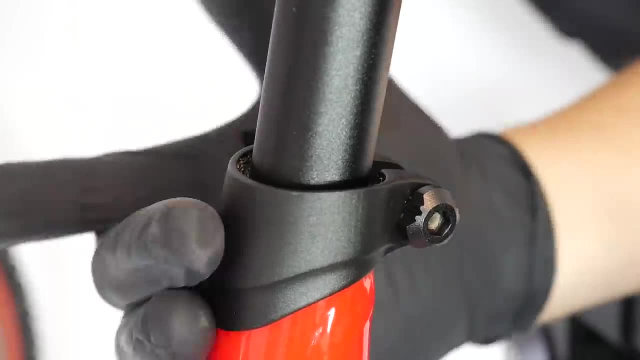 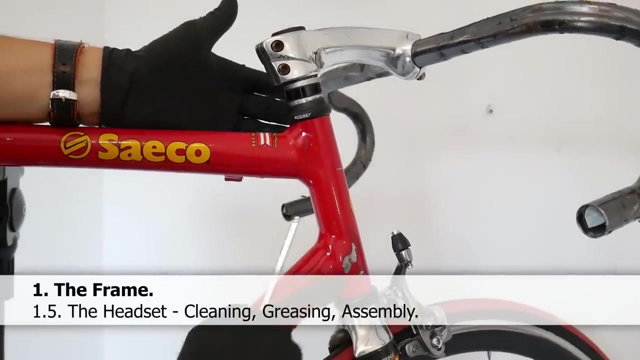 on the lever 90 degrees before it's Clamped and fastened. so that would be something. it's loose. now I feel the resistance. now It's fastened and this it post won't go down the headset. That's the part of our bike which 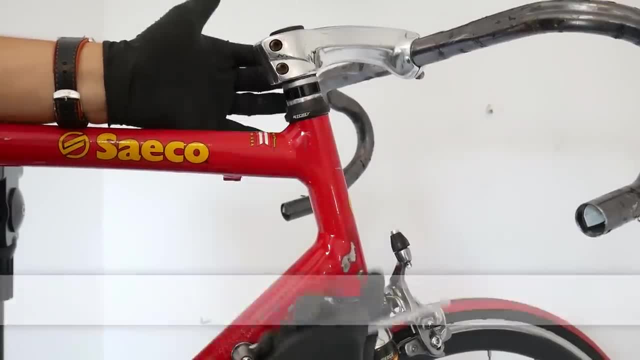 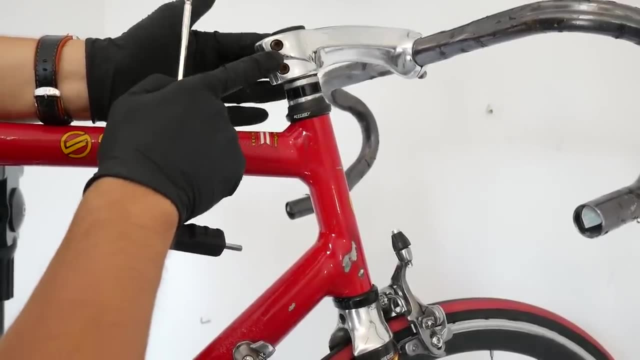 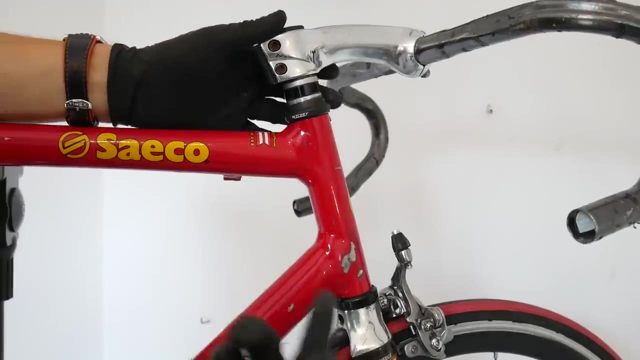 Joins the frame with the fork. the steering tube of the fork is here inside the head tube. this part, which just stands out, allows us to assemble The stem and the handlebar to it so that we can turn the bars. It doesn't matter whether you have the modern bike with fully integrated 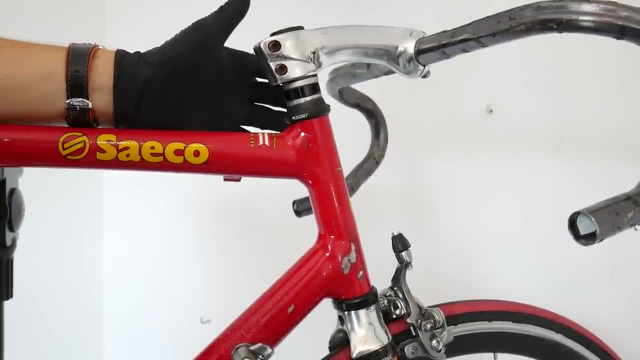 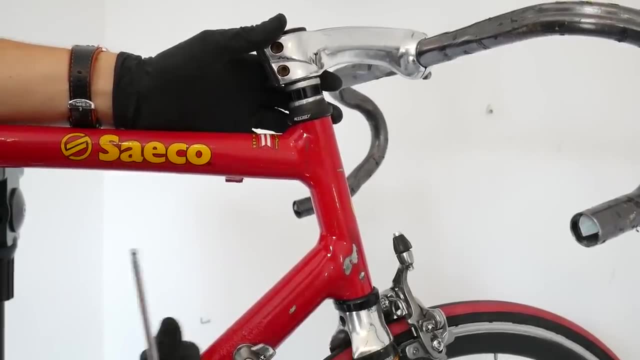 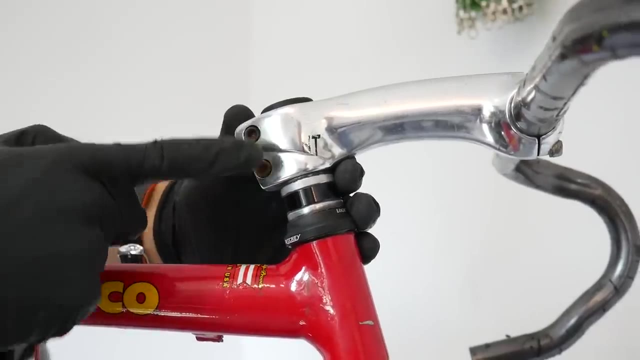 Bearings or the older type. the basic rule is the same. We have two bearings, the upper one And the one at the bottom, and those two bearings allow us to handle the bike. We've got three bolts here. these two bolts assemble the stem to the steering tube. Some stems will have just one bolt and 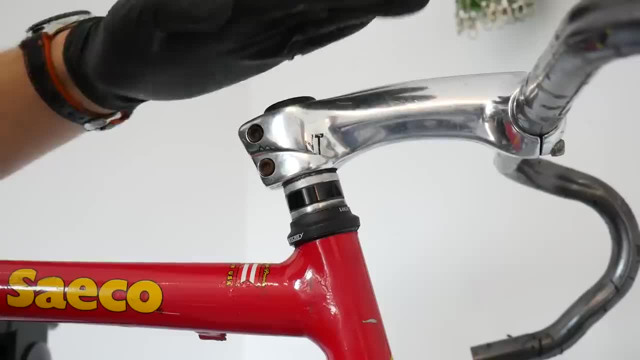 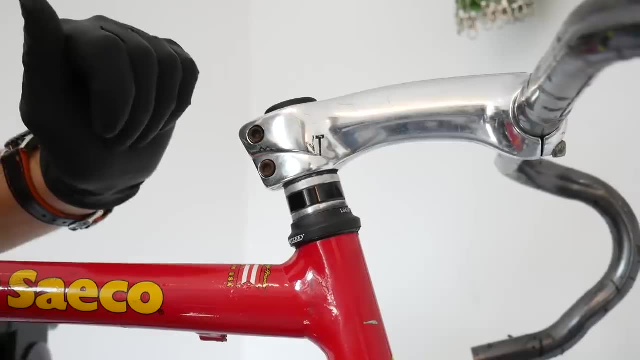 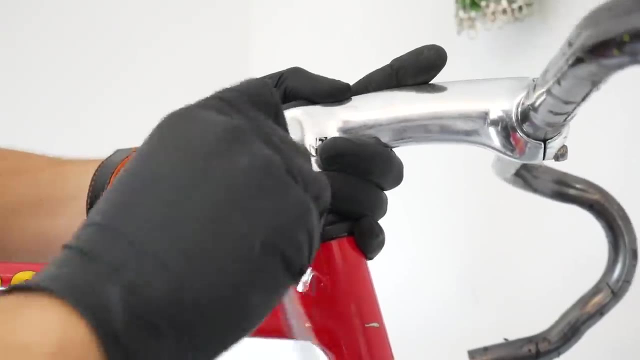 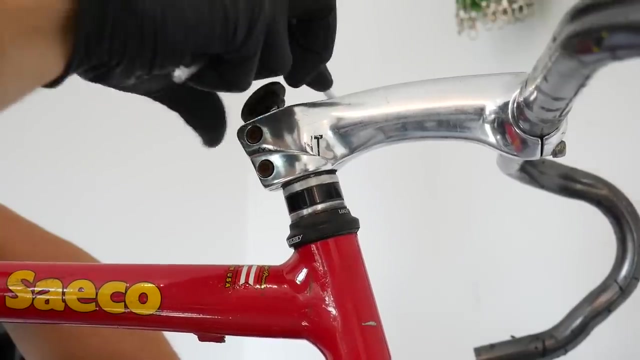 the third one here compresses the whole system, compresses the bearings and allows us to get rid of any play in the headset. Now we're gonna unthread these two and then the third one. Before I unthread these two completely, I'm removing the wheel and holding to. 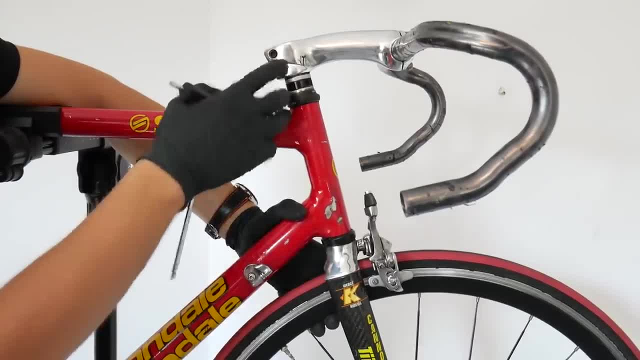 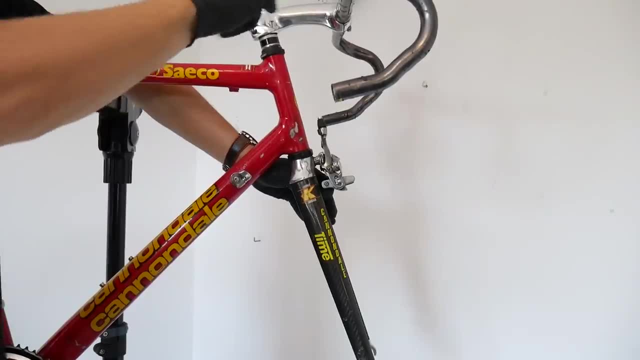 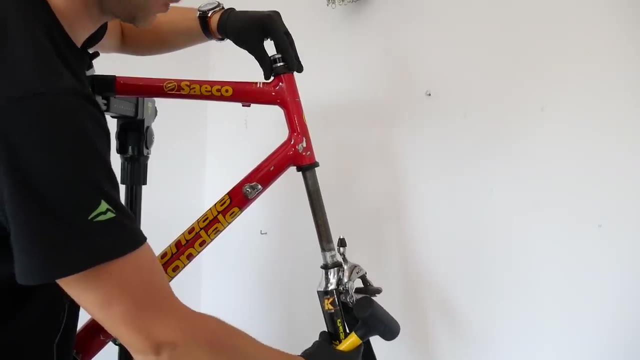 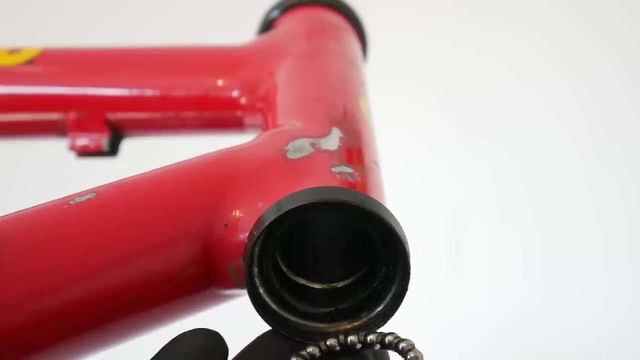 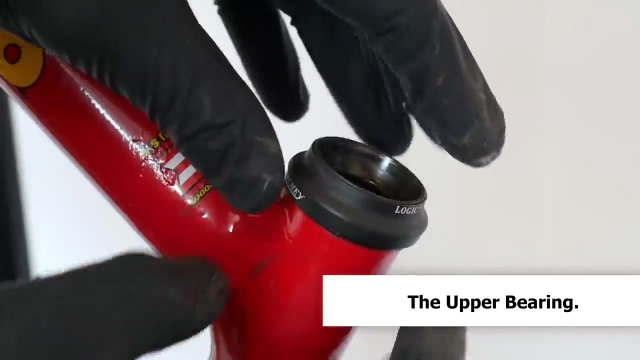 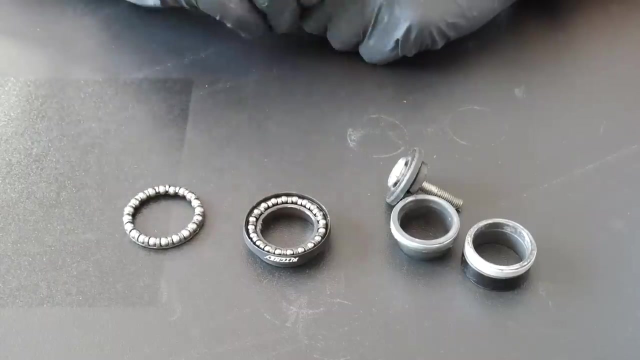 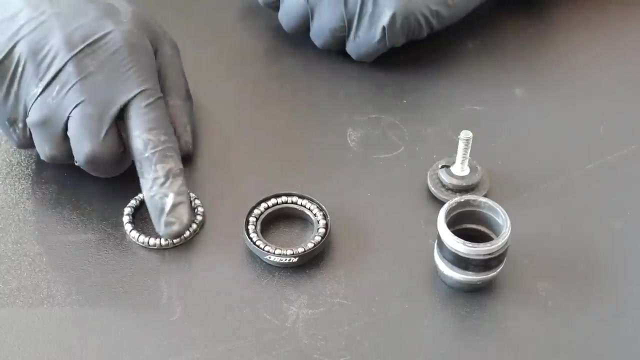 the fork, because then the steering tube of the fork will be loose and it all will just come off. This is the lower bearing on our headset. This is our lower bearing, the upper bearing, some spacers and the top cap with the bolt here. Now we're going to clean these bearings, We're gonna take off this. 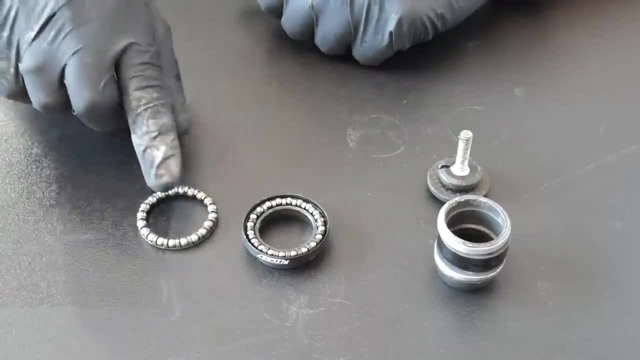 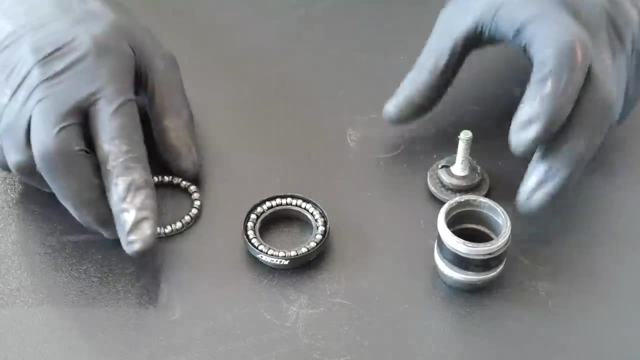 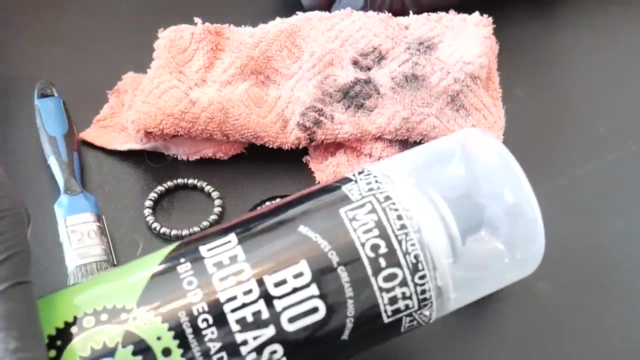 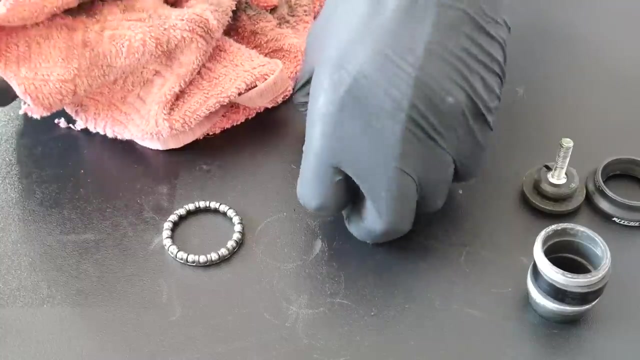 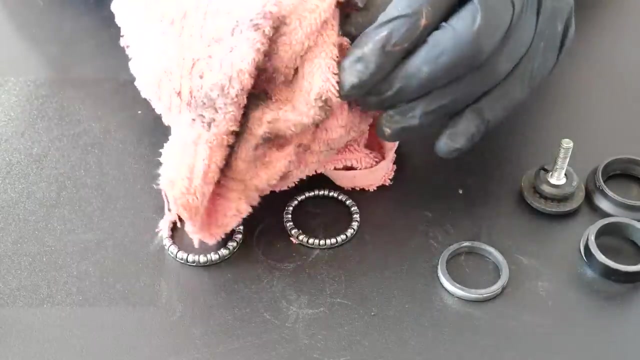 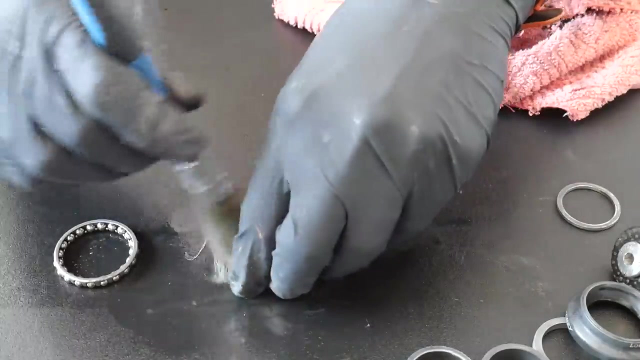 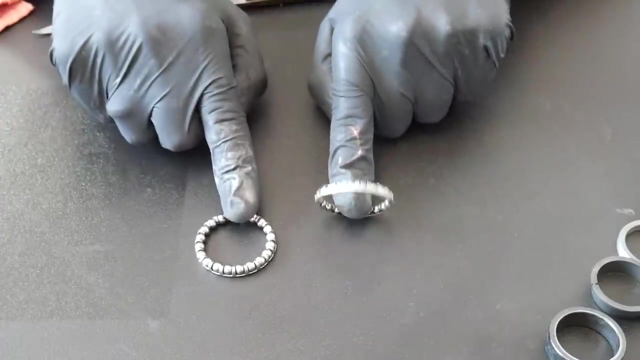 old grease, some grime, some sand, some some dirt which can come into the bearing, especially the lower one. In order to do that, I'm gonna use my brush, some rug, and you can also use a degreaser. These are the bearings we've taken off, we removed from our old, vintage road bike. 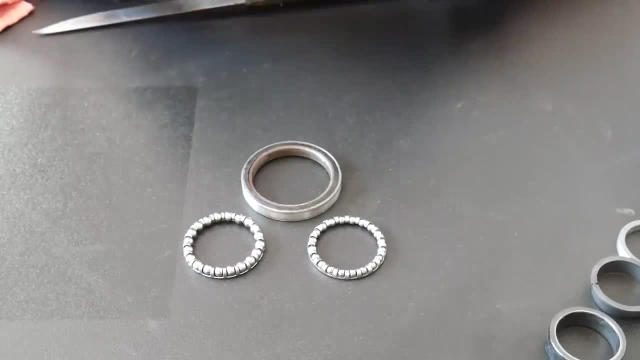 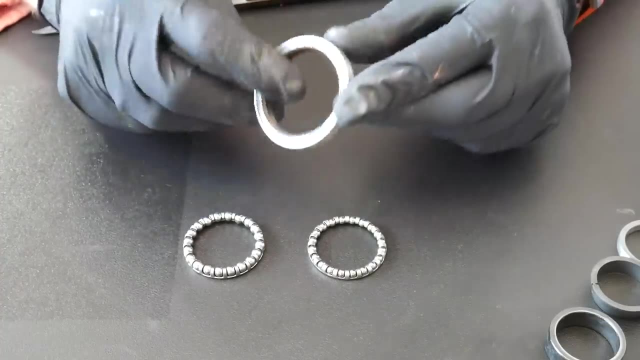 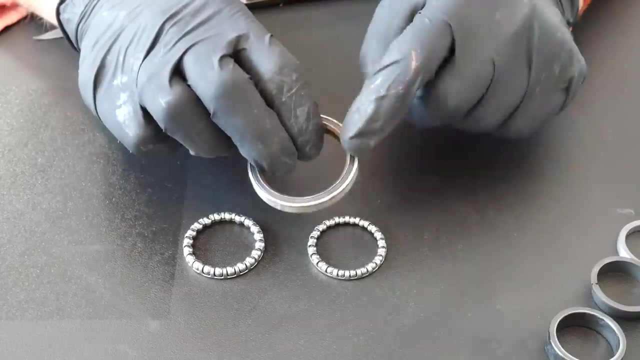 You may find such a kind of bearing in your bike, which is the cartridge bearing. Well, some will say that these bearings we should only replace, but I will tell you that if you feel that there is some grime or dirt inside or you are sure that there was some water which came into the 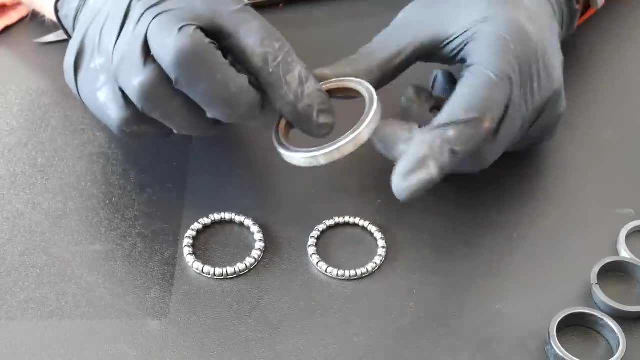 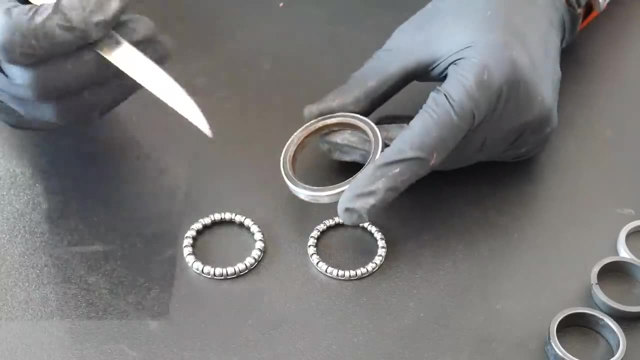 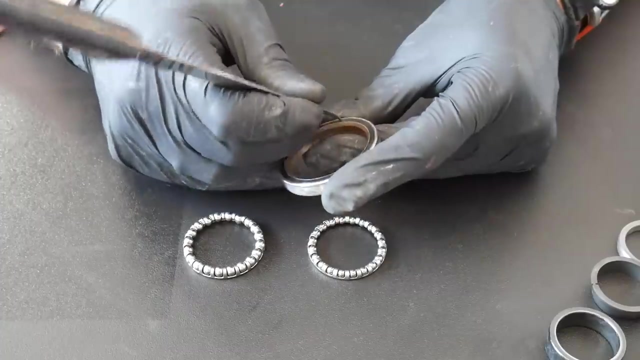 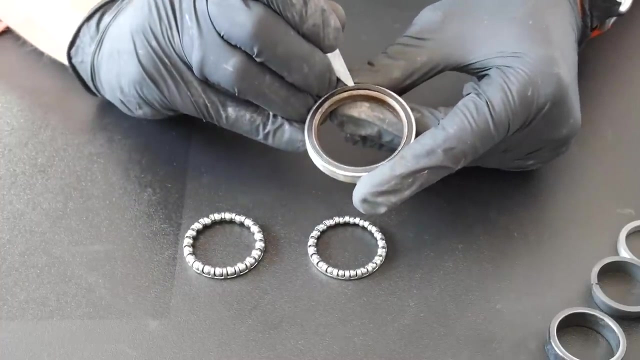 bearing and there is still no play on the bearing. you can open it up and clean it. I'm using my old knife, which is so handy in many maintenance situations. I will just very gently try to open this little seal, because these are sealed bearings. We want to do it gently so that we can. 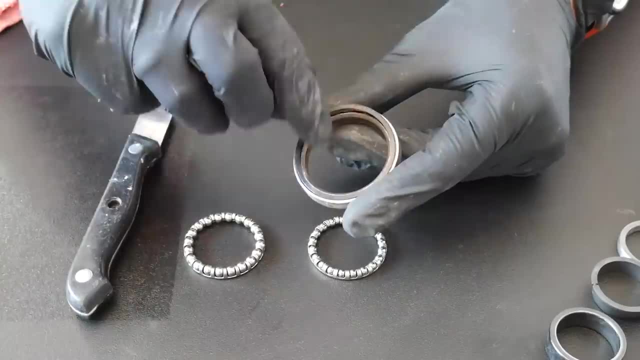 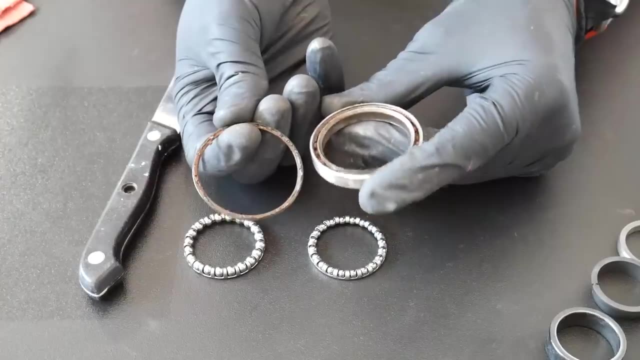 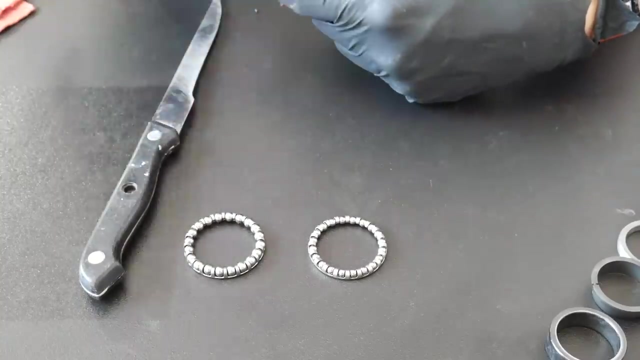 reuse the seal. That's how I did it- and we can see grime, dirt and rust here inside. Now we can just proceed to degrease, clean and re-grease this bearing, just as we would do with these bearings. Clean and shiny lower upper. 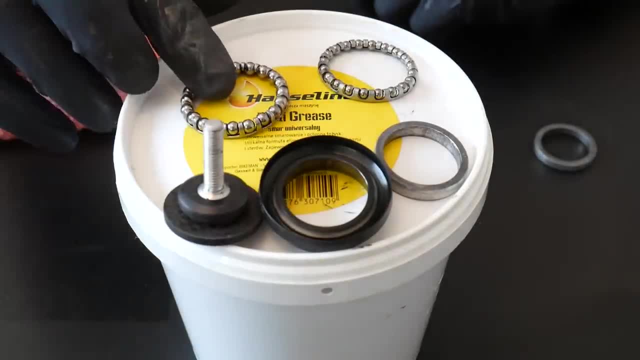 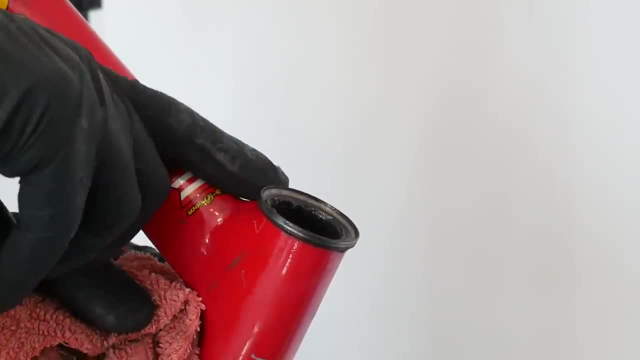 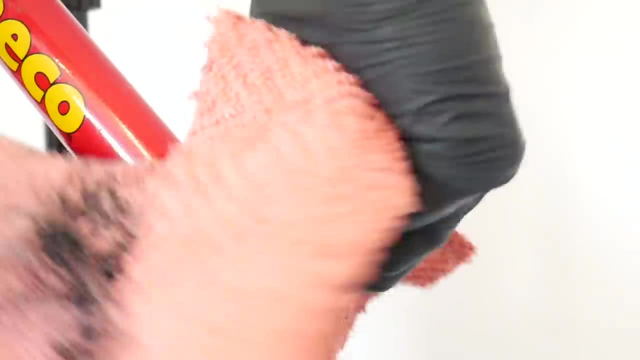 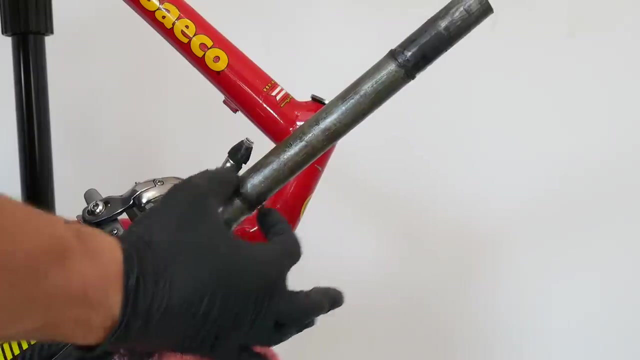 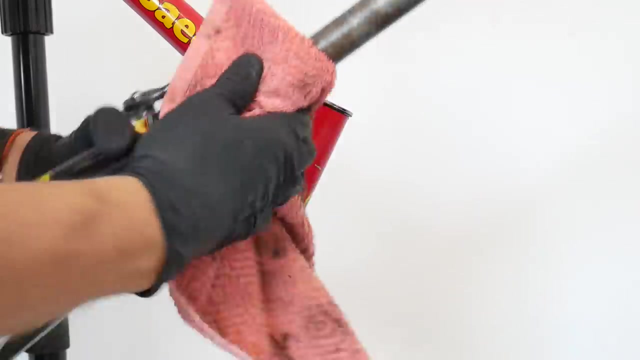 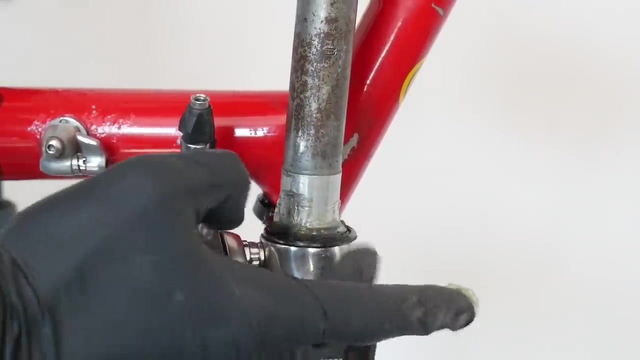 bearings, spacers, races- all the parts are ready for greasing now and being put together. It's time to clean these races so that they will be ready To get some new grease and our bearings, which are already shiny and clean. It's good to bear in mind that the grease is not only making the bearings. 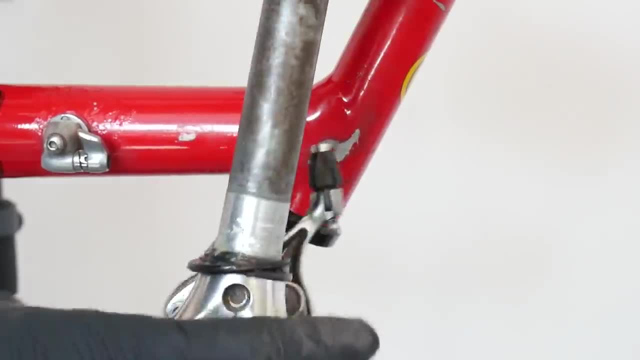 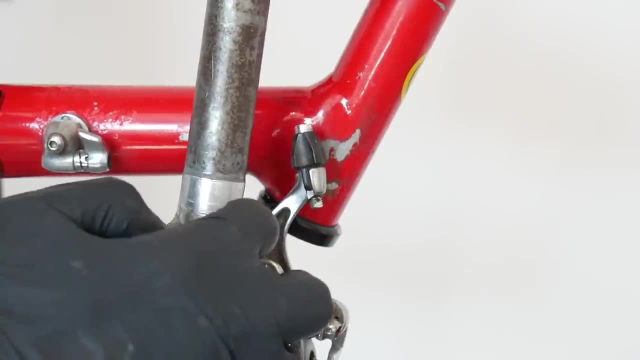 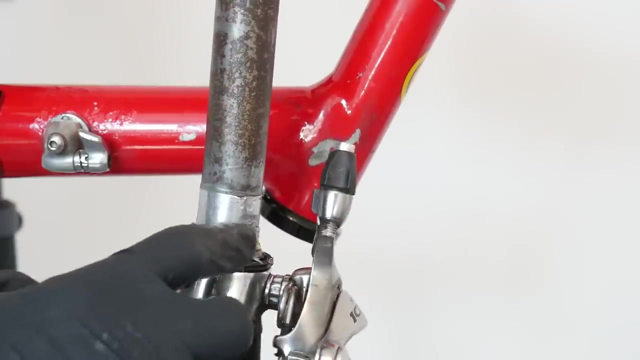 work so well, but it's also making the bearings work so well that they will be smoother, because it decreases the friction, but also it protects the whole system against the water and dirt. So I'm using quite a lot, and then all the excess I will be just wiping off with the cloth after the headset is all put together. 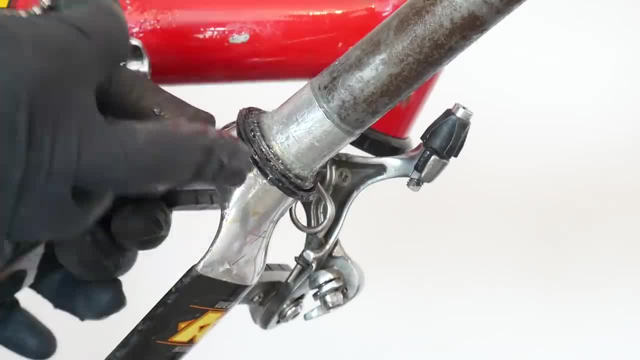 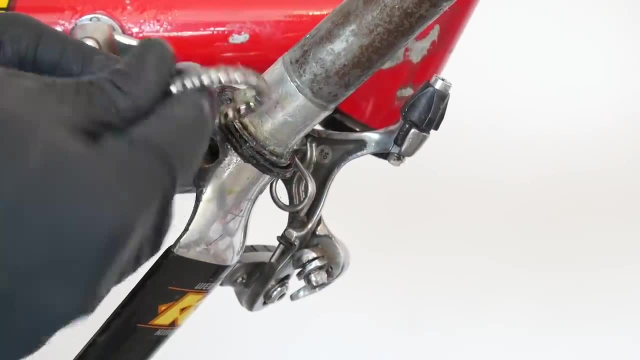 When assembling all parts back together, we should try to keep the bearings good and clean. When assembling all parts back together, we should try to keep the bearings good and clean. remember the order in which we were disassembling all these spacers and seals. and also, how should the bearing sit here on the races, in this case those. 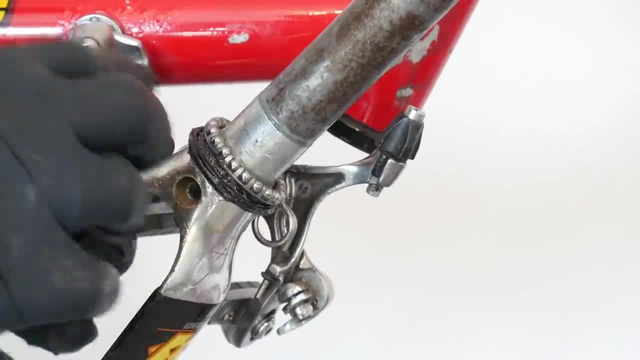 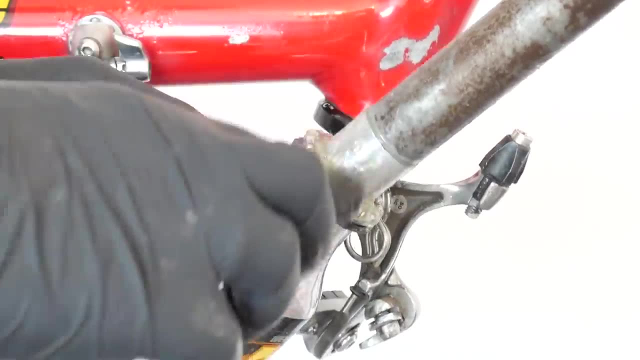 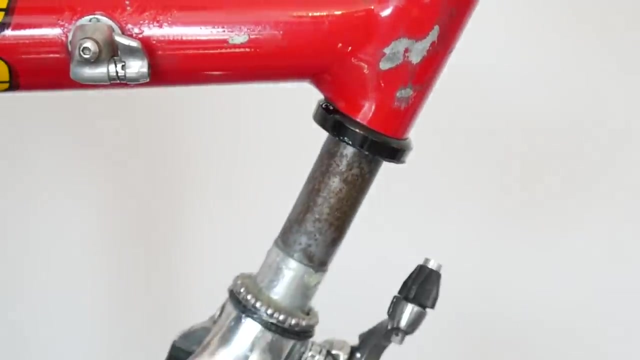 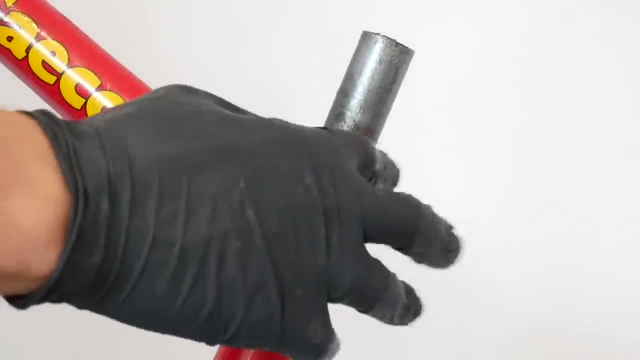 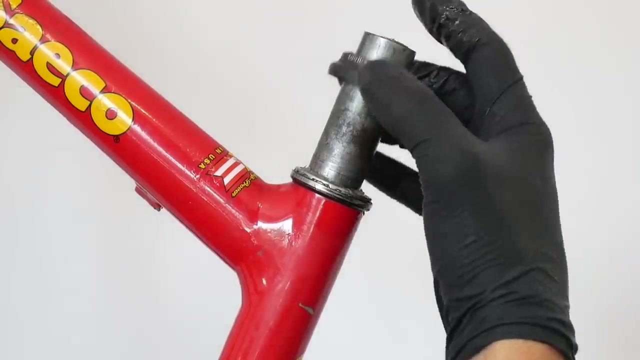 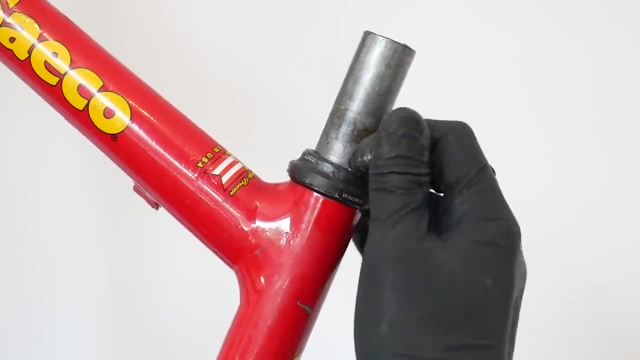 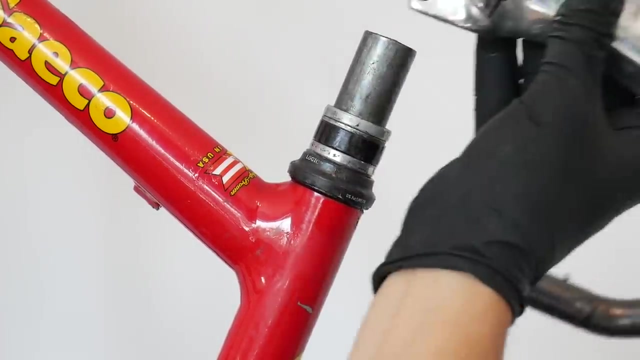 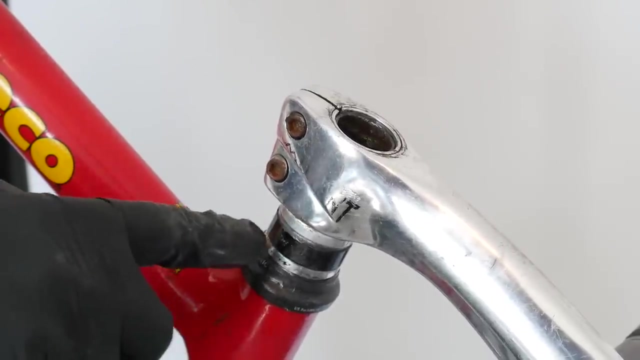 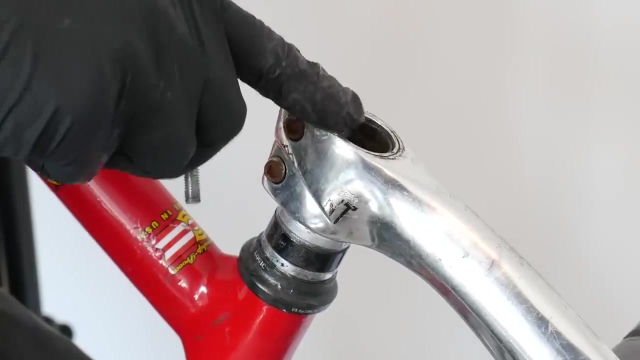 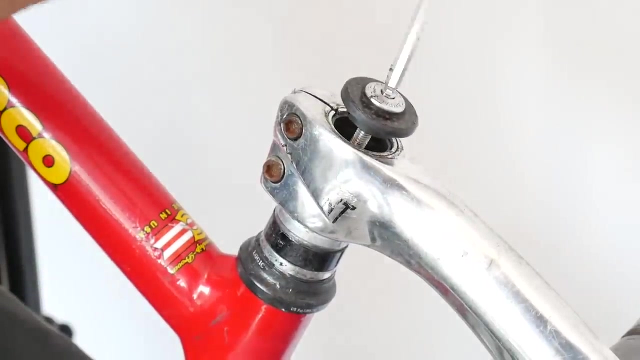 balls should be upwards here so that if the bearing will fit to the races right there, all right, we've put the stem on the steering tube, making sure we have all the spacers needed so that the stem will stand out at least a little bit above the steering tube edge, and now we can put the cup. that will make. 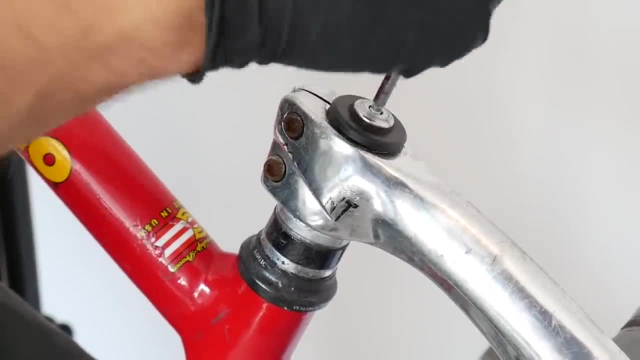 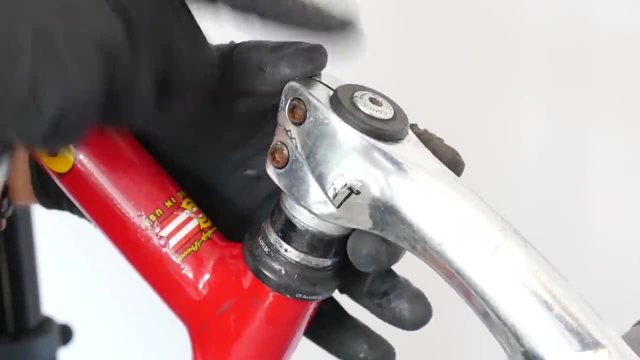 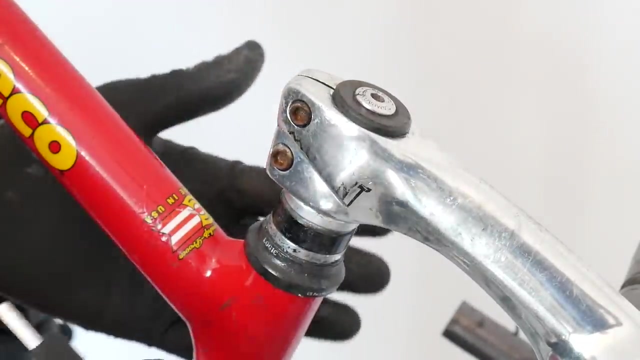 a possible to put the preload on those bearings. now we are not ready to assemble the stem, the fasten, the stem on the steering tube. we are starting with this nut here, with this cup, because we are putting some preload on all those bearings. the best way to do it is to put 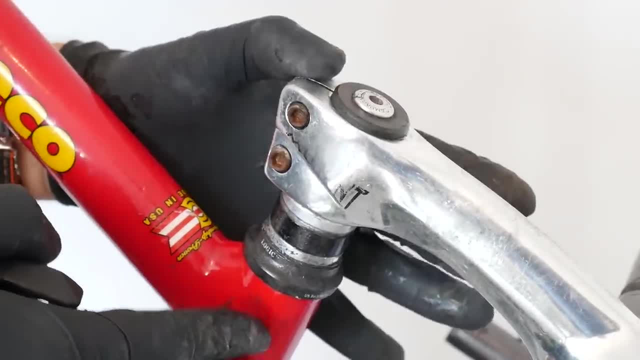 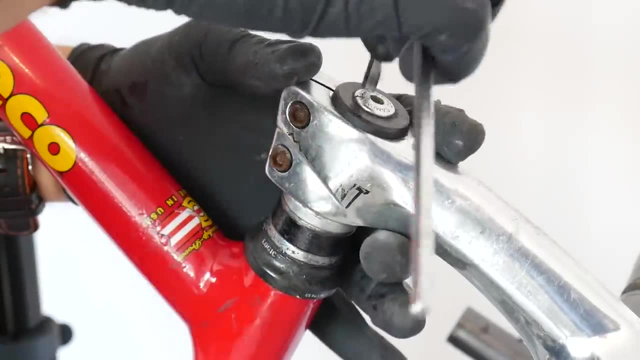 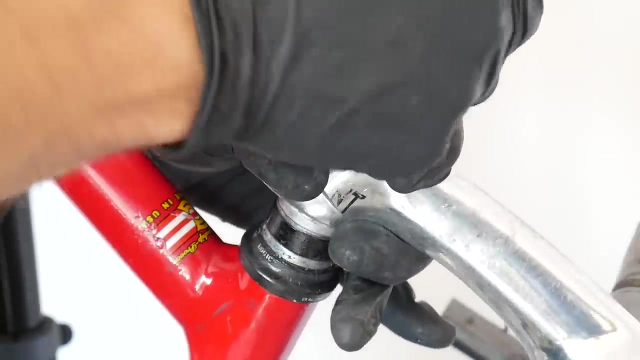 the wheel back on the on the bike and put the bike on the floor, break the front brake, rock the bike back and forth and see whether there's some play or not. but just make sure you are first fastening this bolt here and then, when there is enough preload, on the. 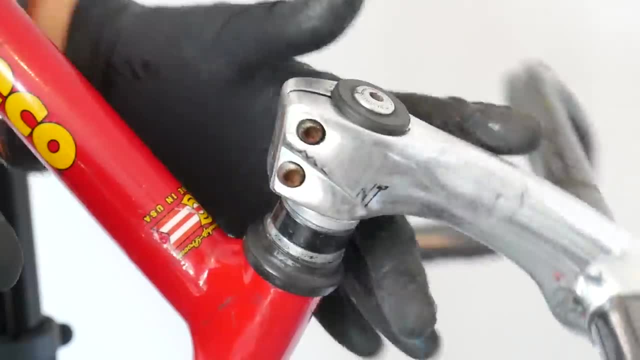 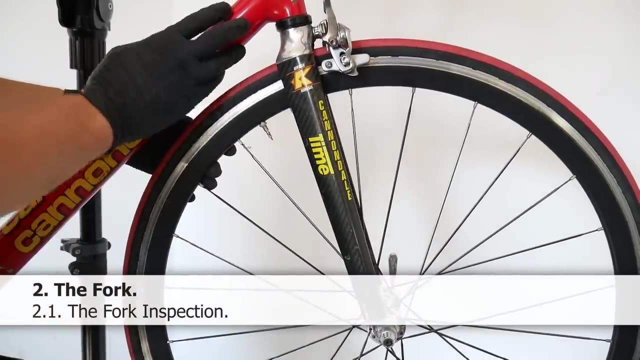 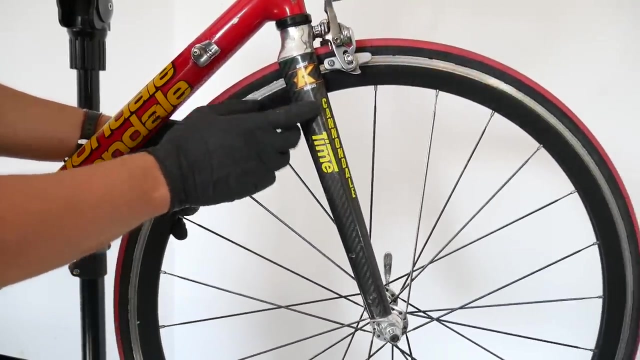 bearings. and still the bearings are working really smooth. we are fastening the stem on the steering tube. The fork inspection will be pretty much the same as with the frame. We want to look for any cracks, damages of the surface of the fork being rubbed by the housings. This one is pretty okay. 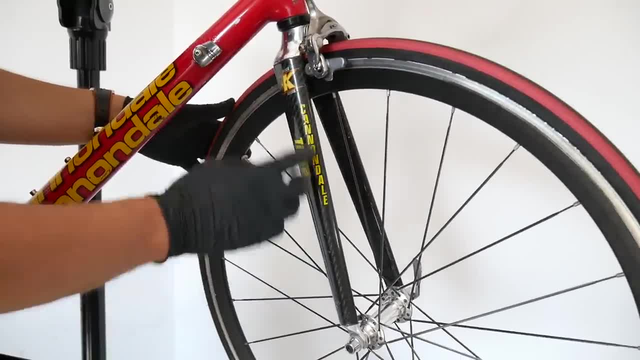 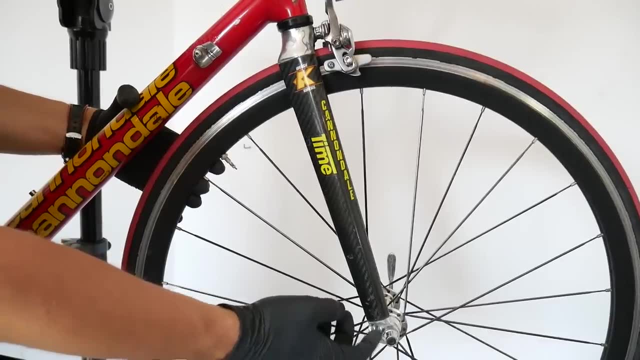 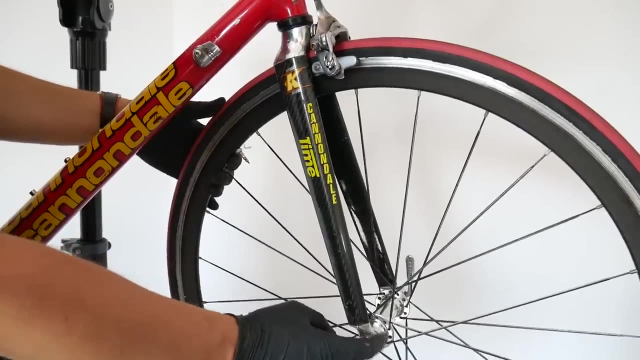 There is lots of scratches. This is an old one, but it looks good. Dropouts- Especially if we have carbon dropouts and we buy a used bike, make sure that somebody- the previous owner- did not squeeze those too much, because then they can just be damaged. There can be some cracks, so always look. 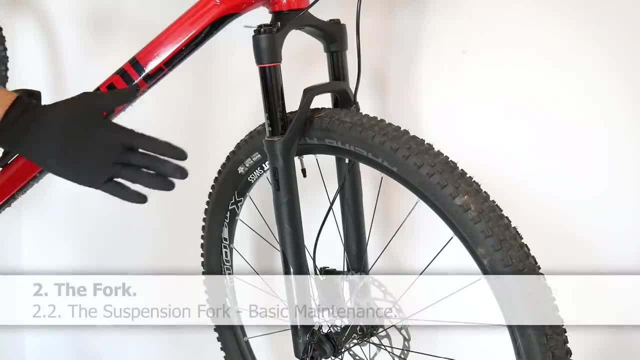 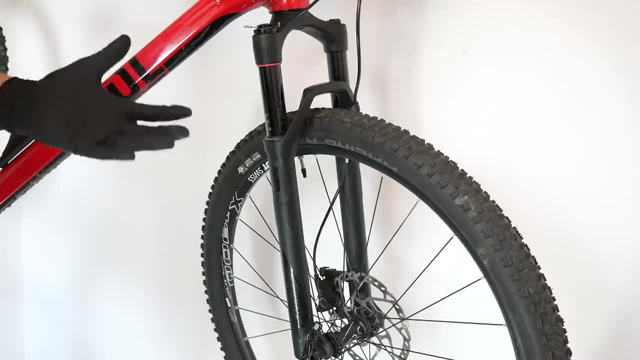 for the cracks on, especially carbon dropouts. The front suspension fork makes our ride fun and safe And, even though you are probably not a professional mechanic, you don't have to take your fork apart. The thing that you can really do for your fork is to keep the good stuff inside and the 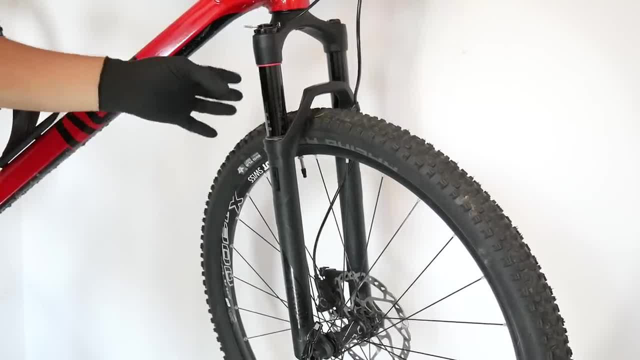 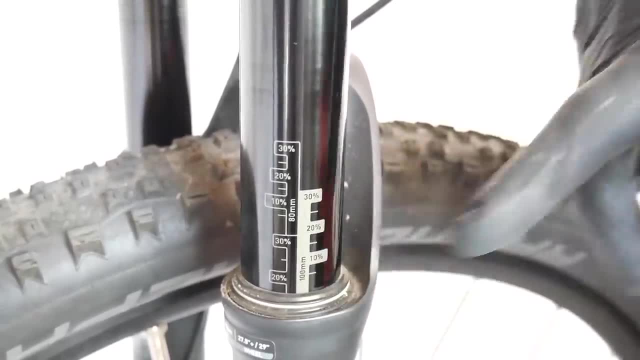 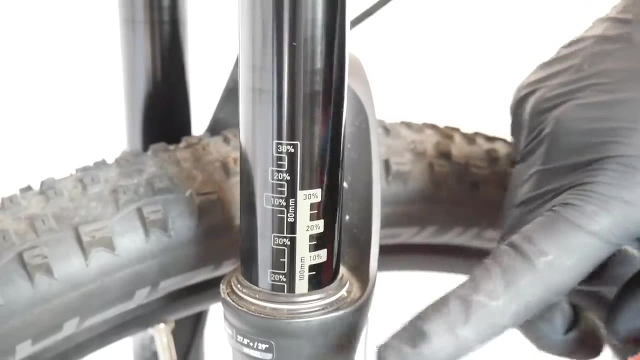 bad stuff outside, and that means cleaning your fork. This is the part of our fork that we all can and should be taking care of. That's the dust seal. The dust seal- that's something we can see from the outside, but there are also some seals inside the fork, inside those outer legs. We should keep. 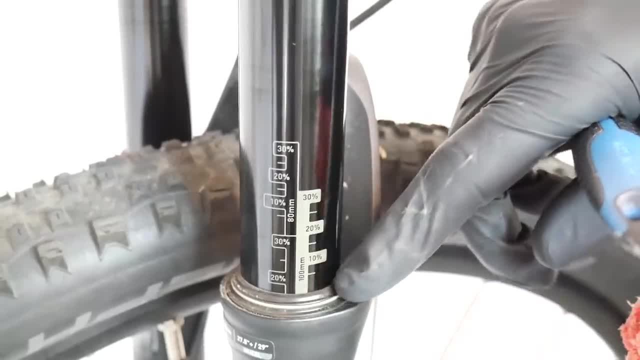 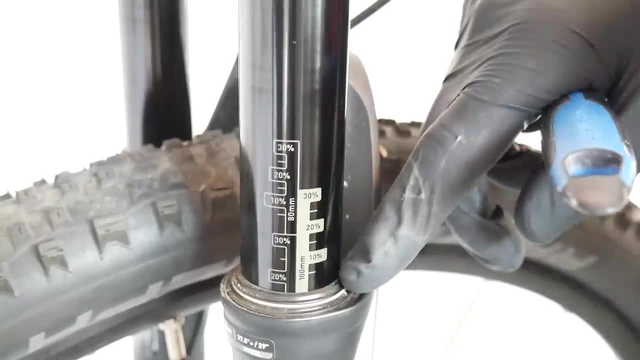 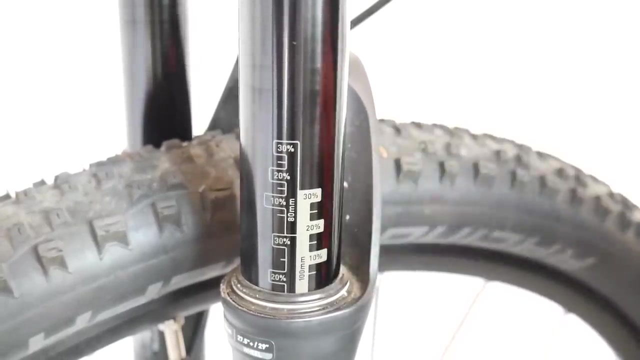 this area clean. While we are cleaning the bike, washing the bike, we should always take a look closer, look at this part. We don't have, we don't want to have here any sand, any grime or anything. but I would also clean this part more often than I wash the bike and I use just a cloth. 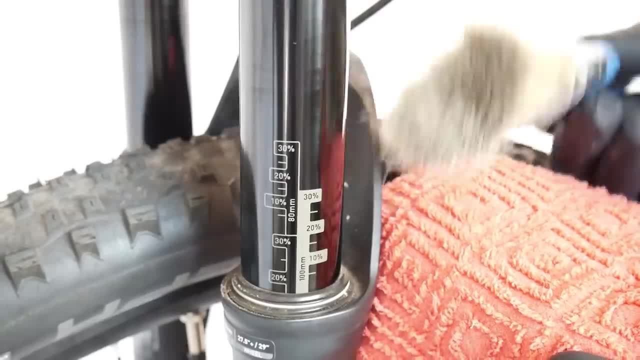 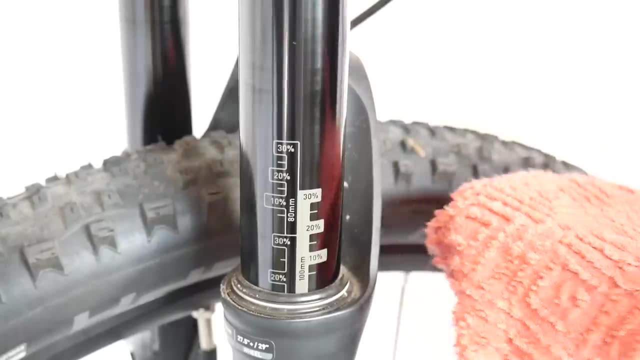 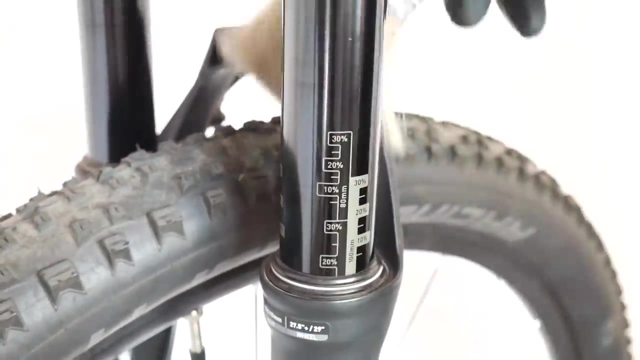 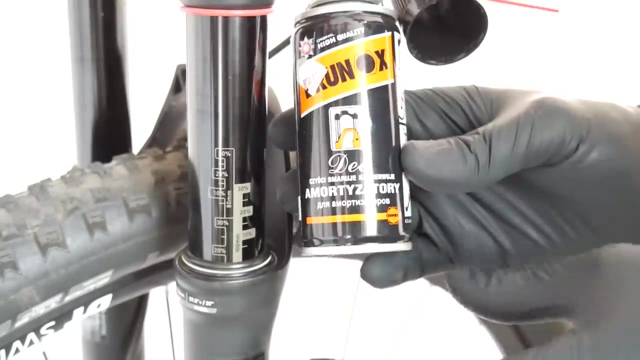 with a little bit of water on it and such a tool, which is super helpful, heel here, I'm trying to keep my brush clean by just rubbing it against the cloth, the rack, and then cleaning my seal. The next step we want to do is to use some kind of a lubricant, but not just some kind of a lubricant. 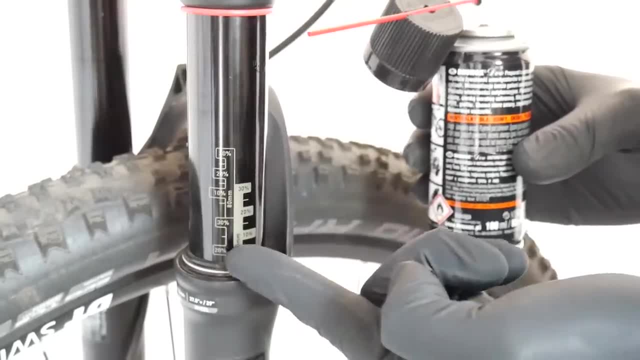 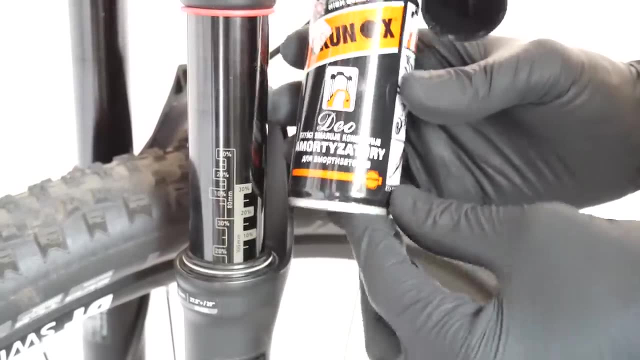 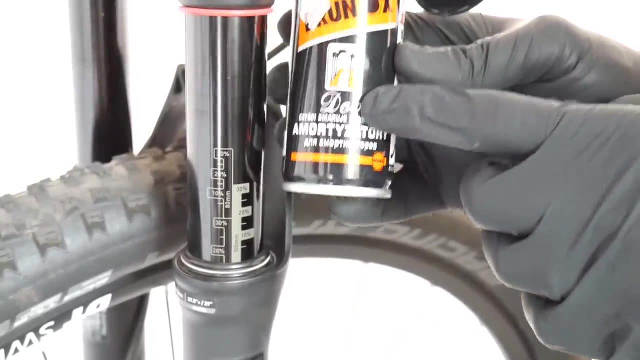 We don't want to spray on the upper legs and on our seat seal any stuff, any spray that would damage the rubber, So it has to be rubber friendly. This Brunox DIO that I'm using is really good. It will really. 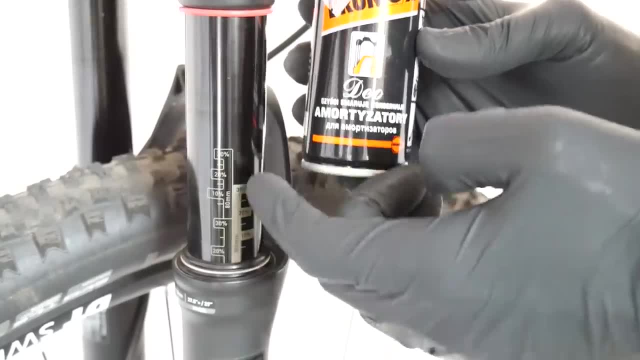 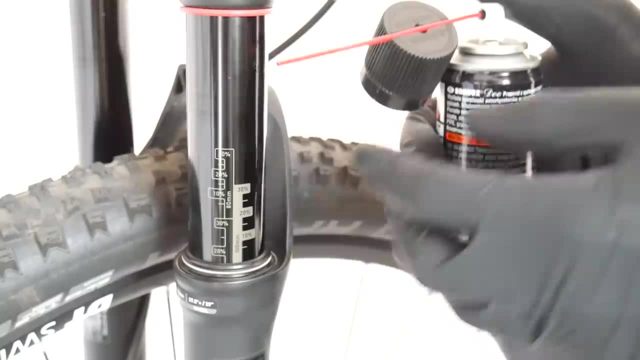 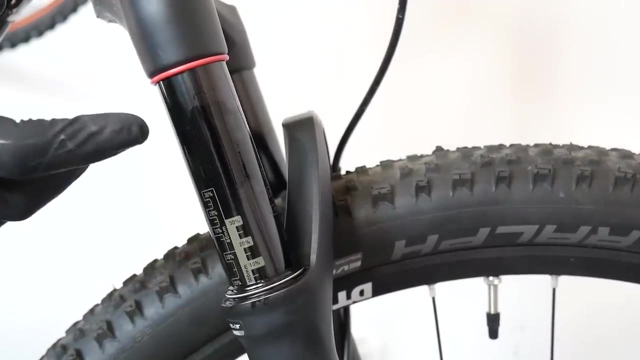 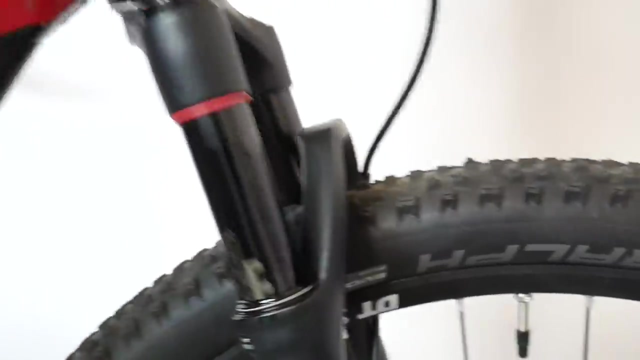 prolong the lifetime of your seals and it will also make your fork working smoother. So what we're gonna do is to put just a little bit on the upper leg here Now we take our bike off the bike stand because we want to spread our lubricant all over the seal and the upper legs simply by working the fork. 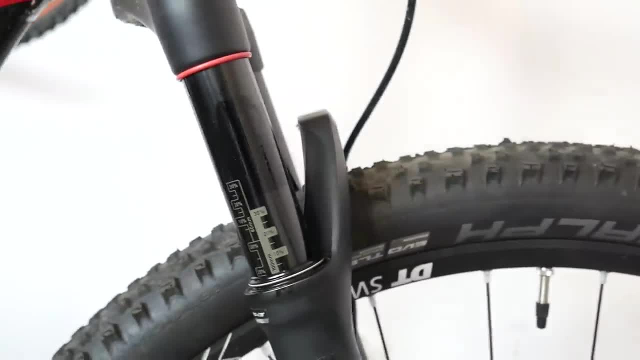 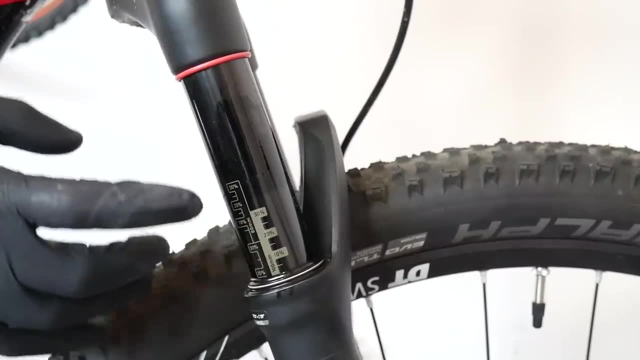 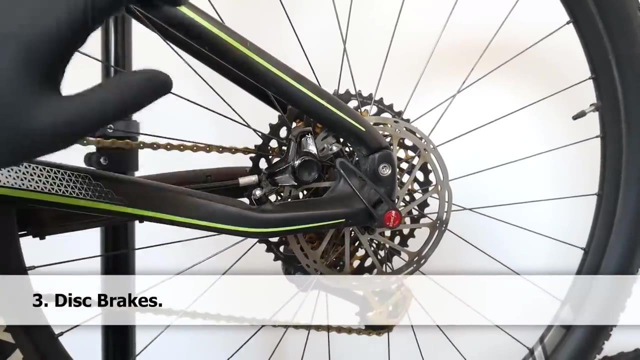 And then the last step will be simply using some dry cloth in order to clean everything. I would sometimes let it stay like that overnight and then clean the whole thing the next morning. This is the disc brake. It is powerful, pretty good in terms of the 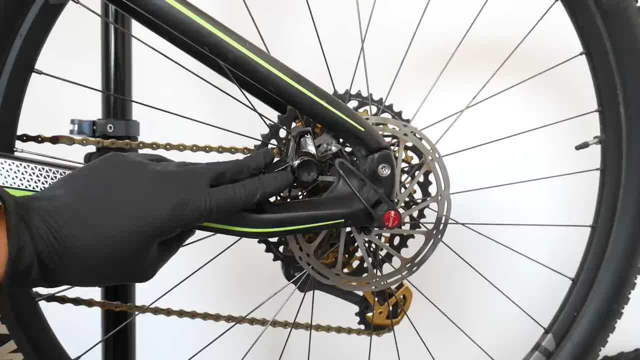 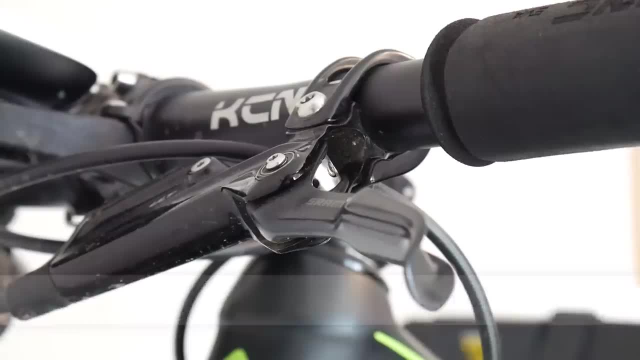 modulation, and this type of the brake is becoming more and more popular, not only on the mountain bikes, but also on the road bikes. So let's see how to maintain and adjust these. The first thing we can adjust on our disc brakes according to our preferences is the position of the lever meaning. 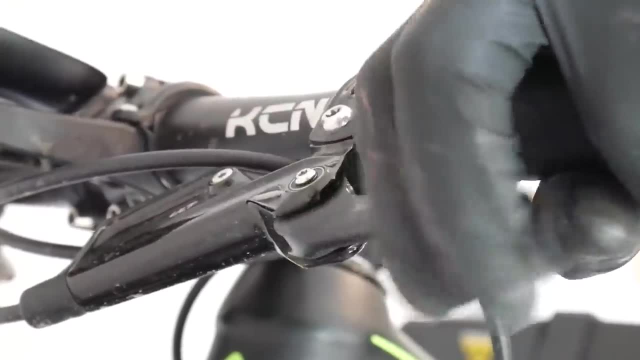 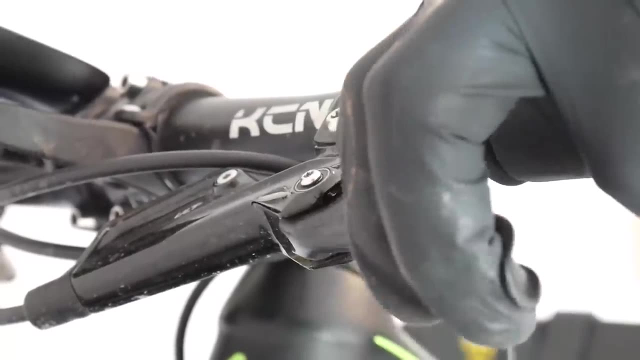 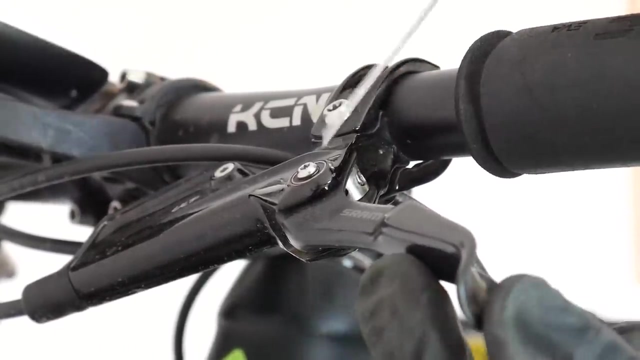 how far the lever will be from the handlebar in the starting position. People with smaller hands would like to have it closer. with larger or longer fingers would like to have it further away from the bars. Most of the manufacturers will give us this option Here on my SRAM level. 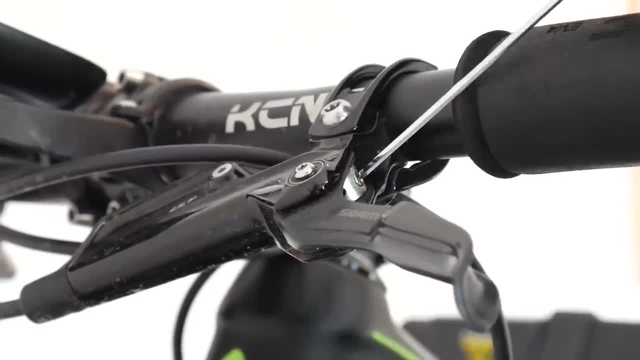 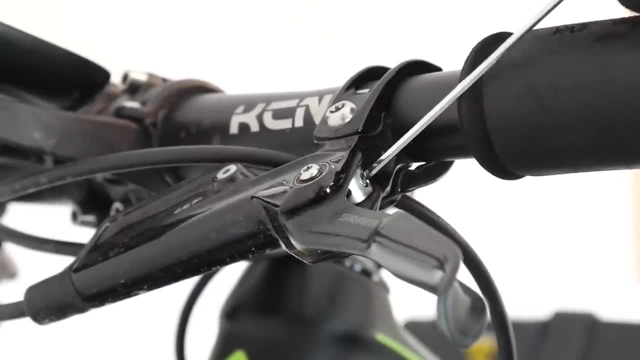 brakes. I have this small two millimeters allen key or the bolt there. When I'm threading it in, as you can see, the distance between the lever and the handlebar increases. That means if I have larger hands I can adjust the distance between the lever and the handlebar. If I have larger hands. 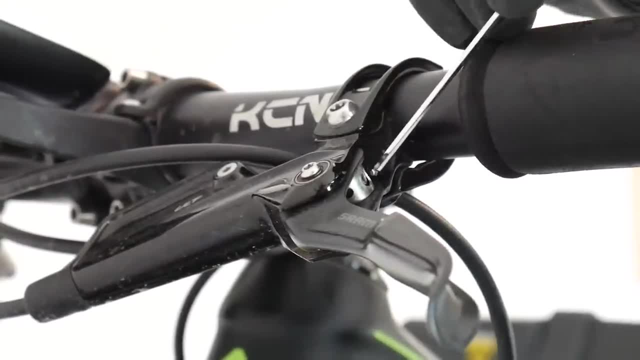 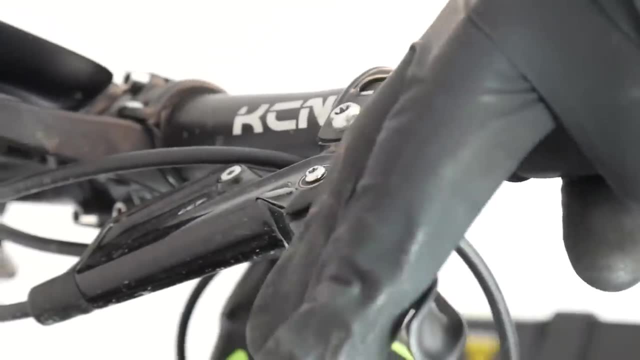 I can adjust the distance between the lever and the handlebar If I have larger hands. I can adjust the distance between the lever and the handlebar If I have larger hands. it will suit me better. I'd like to have it really in the furthest possible position. This fits me well, So you should be. 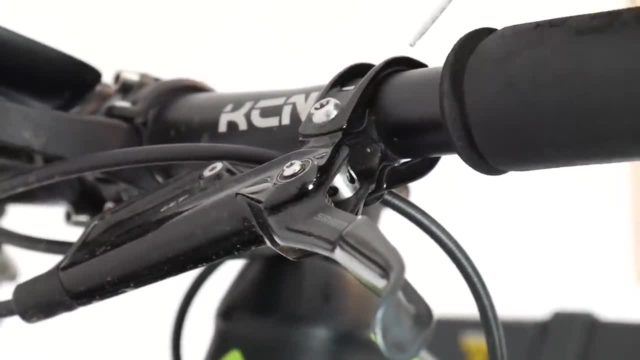 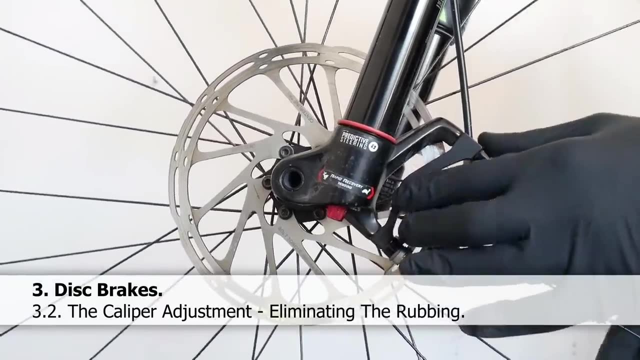 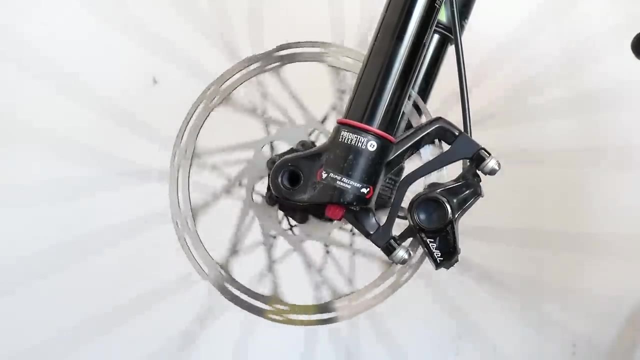 searching for some small adjustment bolts somewhere on your braking lever. One of the main problems that a disc brake user can come across is this: It is the disc rotor rubbing against the brake lever. It is not only annoying because it makes some noise, but also it will wear down our 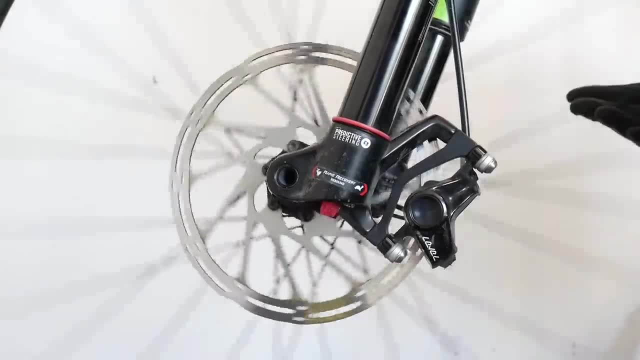 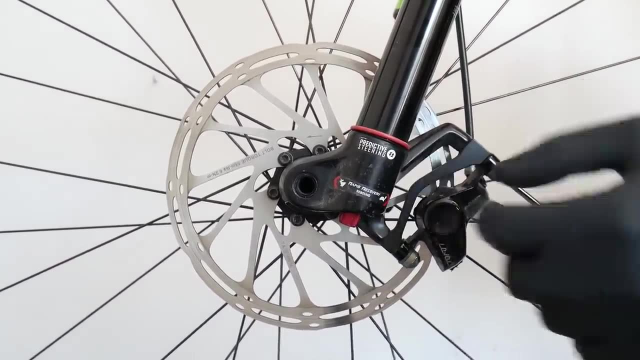 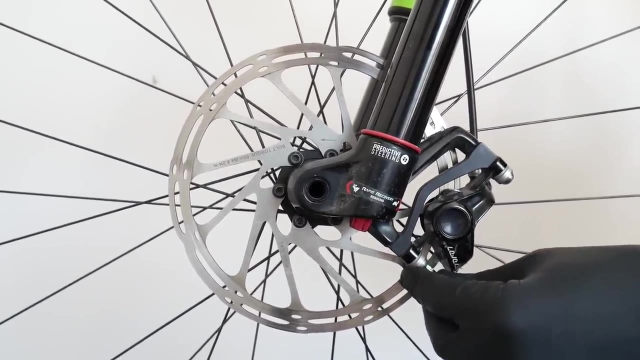 disc brake rotor and the braking pads faster. And the solution of this problem is pretty easy. These two bolts assemble our caliper brake to the fork, So we want to unthread these just a little bit. We don't want to have this caliper completely loose, Just having the chance to move it. 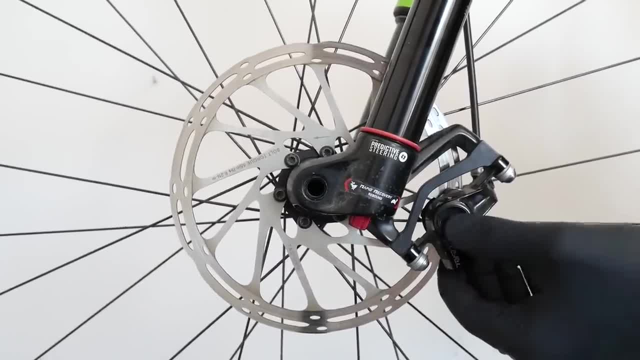 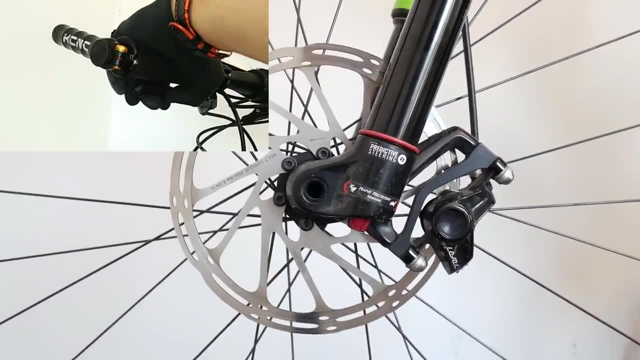 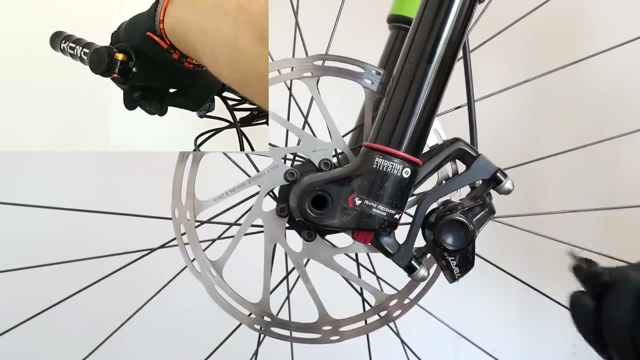 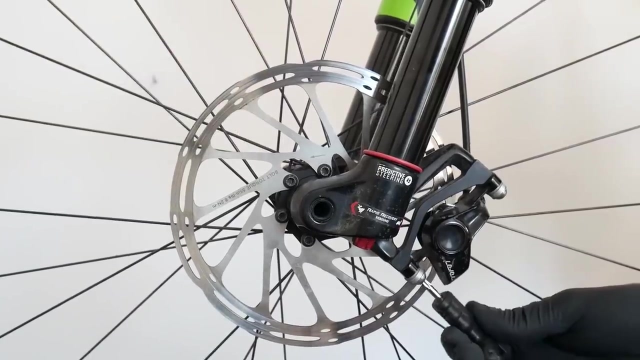 around. a little bit is enough. This is just enough. What we do next is that we squeeze the braking lever. Now the pads are squeezing against this brake rotor and the caliper brake is being centered, And now we thread those in, fastening the whole caliper brake to the fork. Let's see how it. 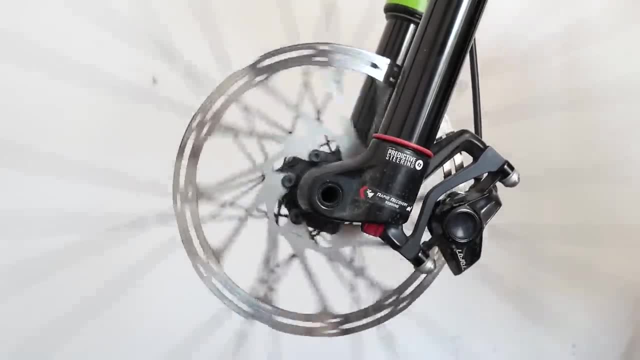 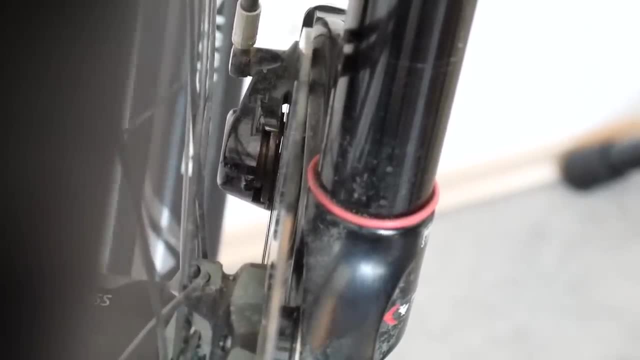 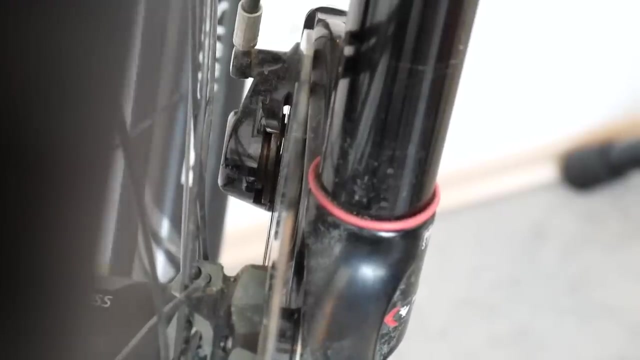 worked. It worked very well. The problem is solved. This method works pretty well. but if you are going to adjust your rear caliper brake, it may be difficult for yourself, if you're just alone, to squeeze the braking lever and also to reach to the caliper to the rear. So adjusting 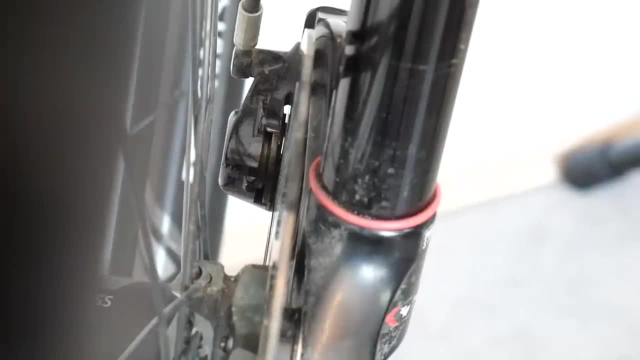 this just manually can be a good thing. A white piece of paper can help you to see exactly what's the position of the caliper brake. If you want to adjust the caliper brake to the rear, you can do it with a white piece of paper. 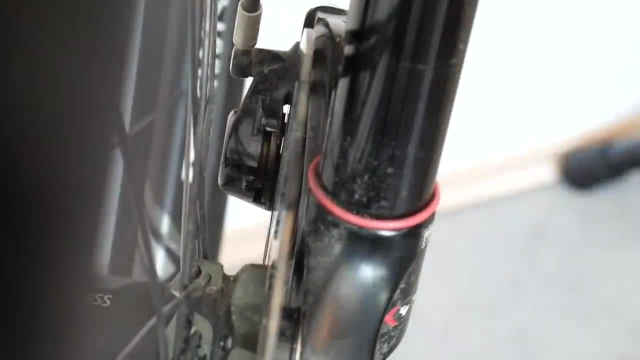 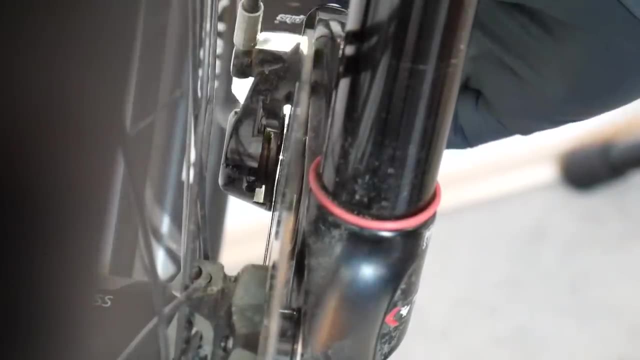 This is the disc brake rotor against the braking pads, And also using a flashlight, just like bicycle light, you can see exactly what's happening in between the disc brake rotor and disc brake pads. Remember also to spin the wheel, because the rotor is almost never perfectly true, So it will. 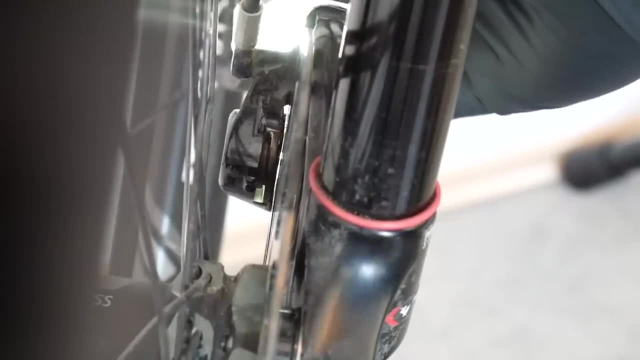 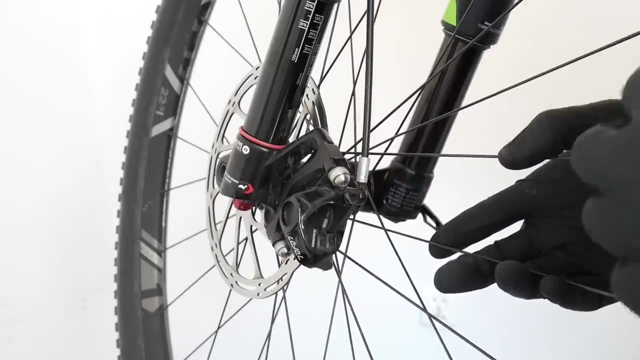 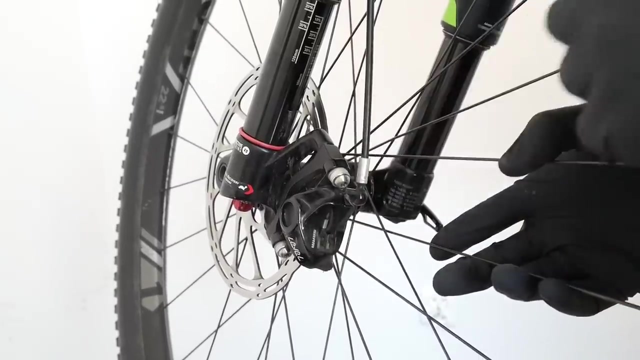 just move a bit, and when you adjust it by hand manually, it may help you to find the right spot. There are also two other reasons for the disc brake rotor rubbing against our braking pads: It's the rotor being out of true, and if it's really out of true, we won't be able to adjust the caliper. so 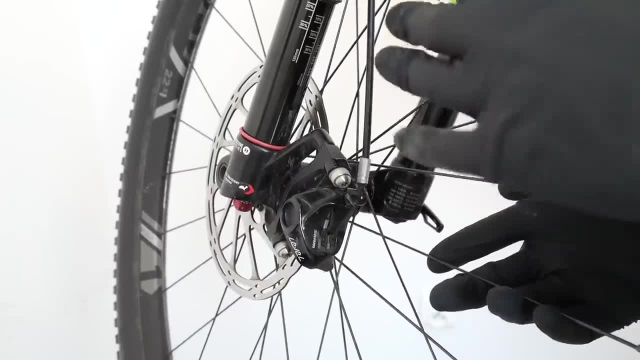 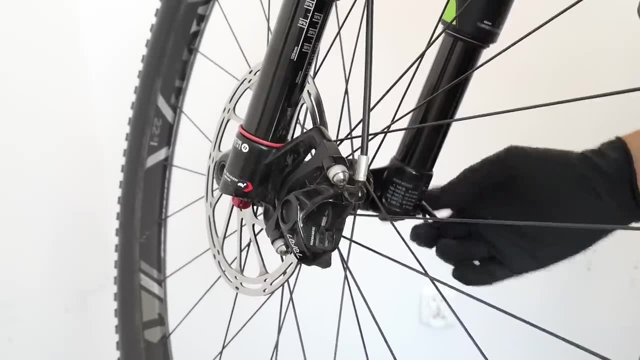 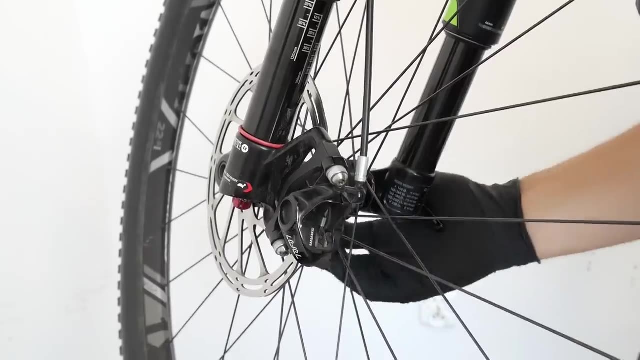 that it won't be rubbing at all, Then we just need to true the rotor, and that's we're gonna do in the second. And the second reason for this rubbing is also our quick release or the through axle. We should try to squeeze the whole system with the same force each time we remove the wheel and put it back together. 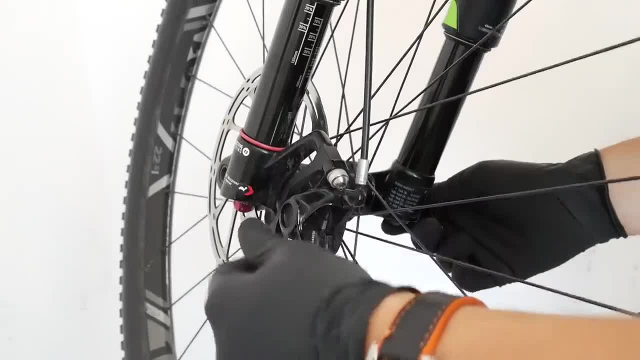 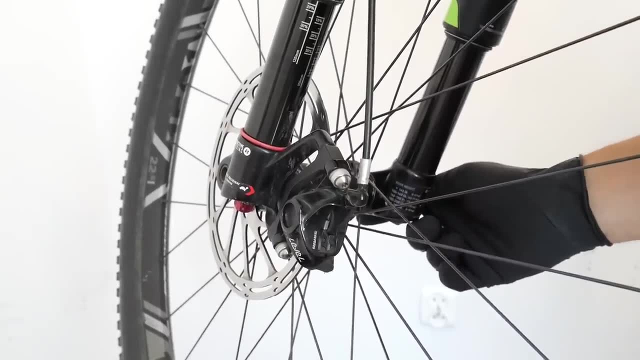 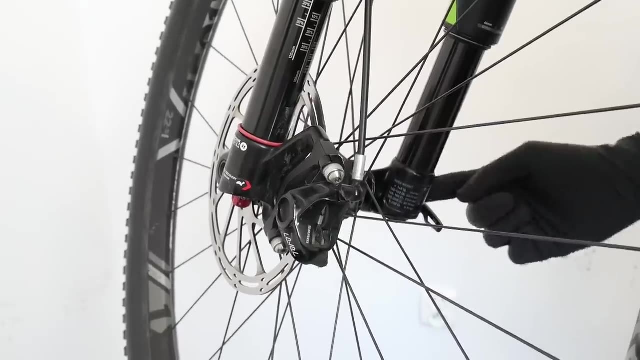 So if we have a quick release, we should know how many turns we use in order to remove the wheel on the nut And then, when we put the wheel back together, we just count the same number of turns on the nut. And if it's a through axle, we want to have this lever always in the same position. 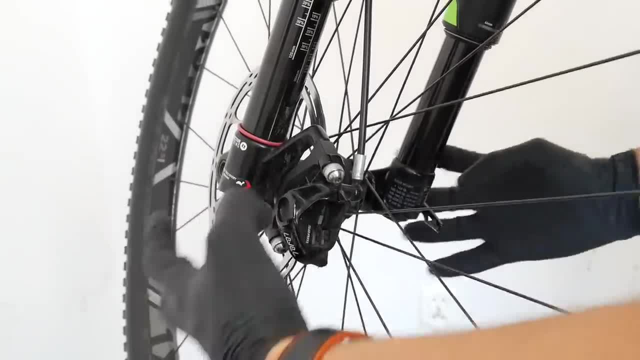 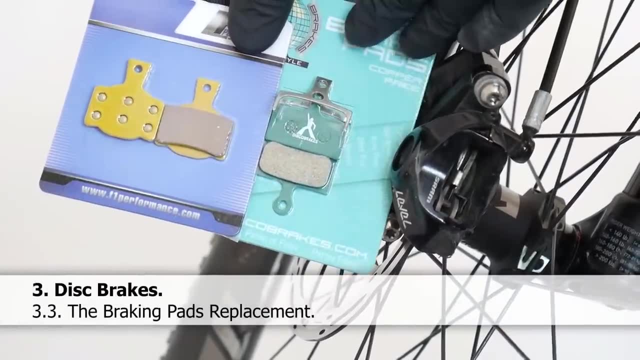 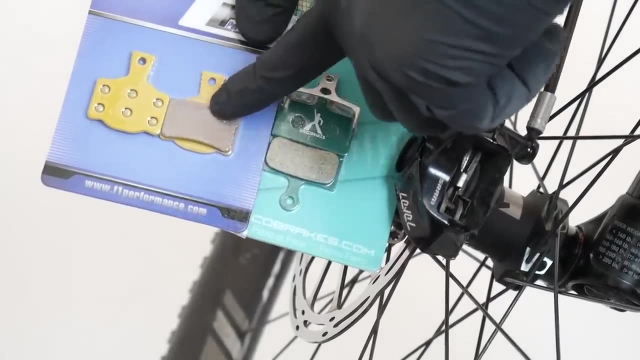 when the wheel is fastened, And then we have same force squeezing the whole system and no rubbing. These are the braking pads for our bicycle. When you buy one, you should find the right type that will fit the model of your brakes, and also the right compound that will fit your riding style. 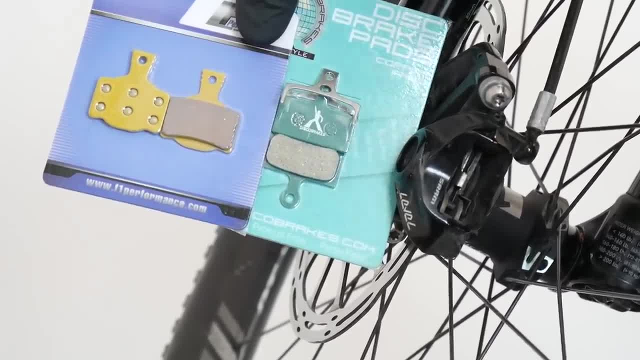 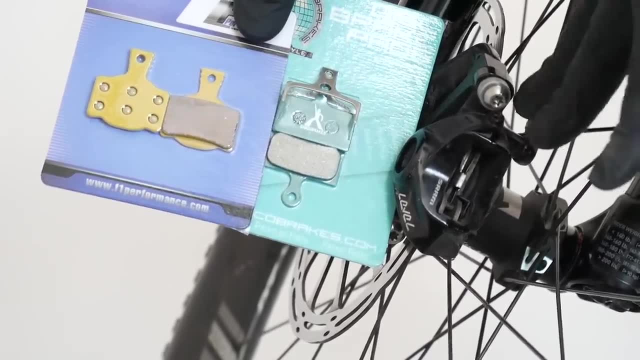 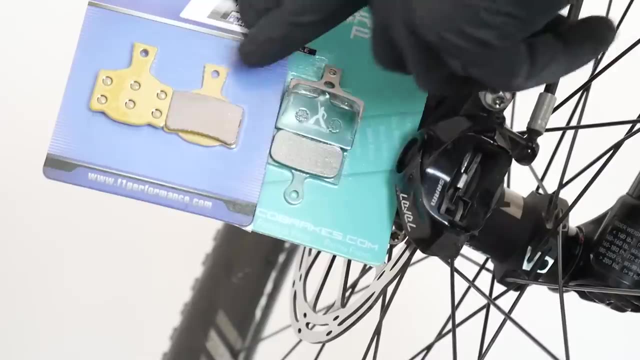 and the weather conditions that you are going to be riding in. As you will see, replacing the braking pads, it's pretty easy job for different models and pretty similar for the bike, And we replace these when this compound not the plate itself, but the compound on the plate. 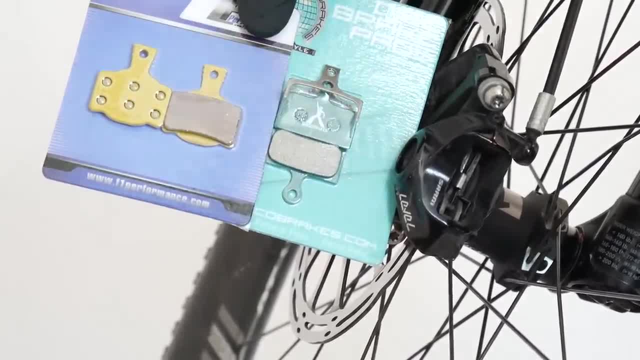 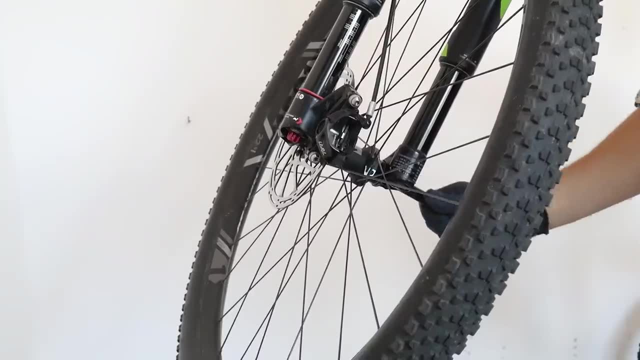 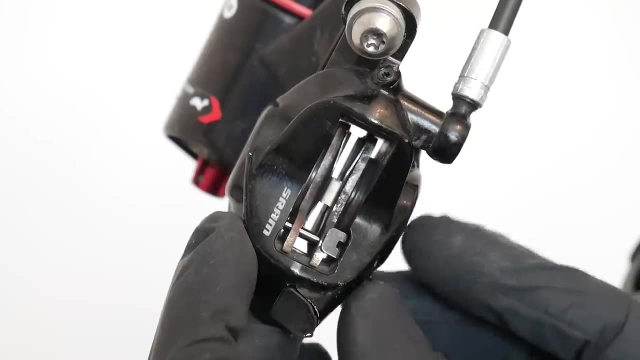 is getting thinner than around one and a half millimeter. Before we replace our pads, it's really good idea to remove the wheel. Replacing the braking pads is pretty easy job. You can find some pins on, for example, Shimano calipers. 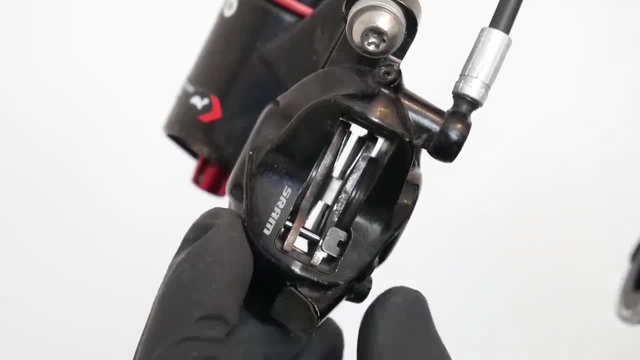 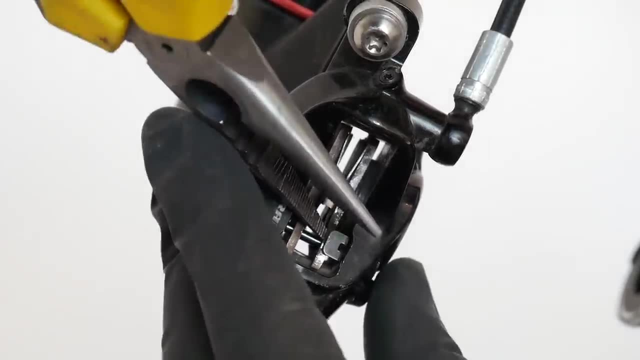 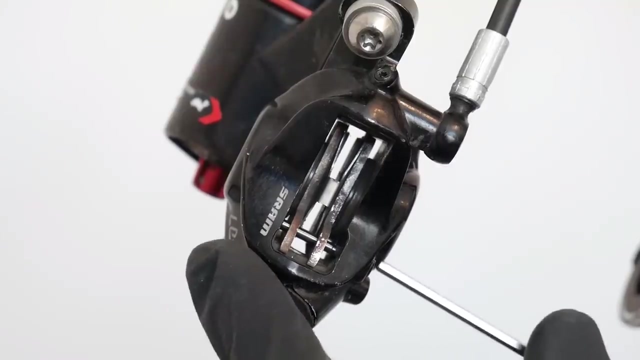 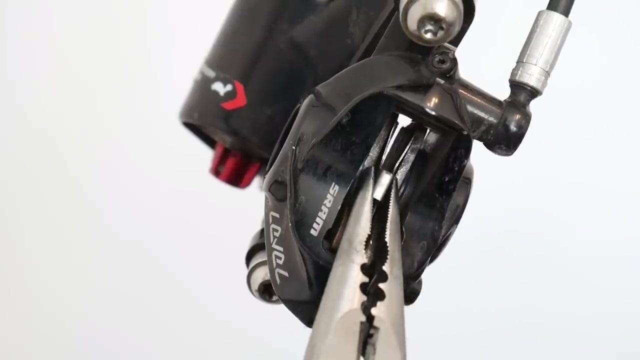 or some bolts on this SRAM level, for example. Also, my Magura brakes would have the bolt Here. there is some additional protection that I have to remove. first It looks just like this, And then I can unthread the bolt and now remove the braking pads. 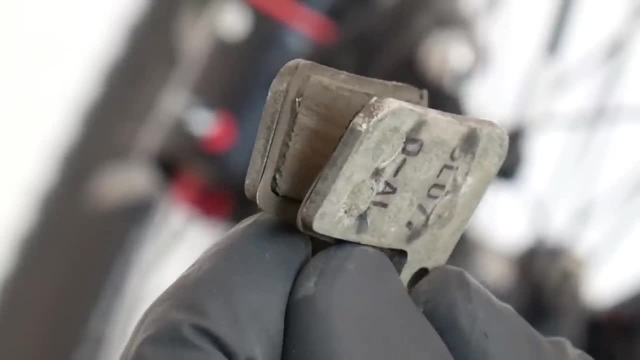 This is how my braking pads look like. These are still in good condition. These are still in good condition. These are still in good condition. These are still thicker than one and a half millimeters, so they can stay here. Before we do that, this is a very good opportunity to clean and degrease. 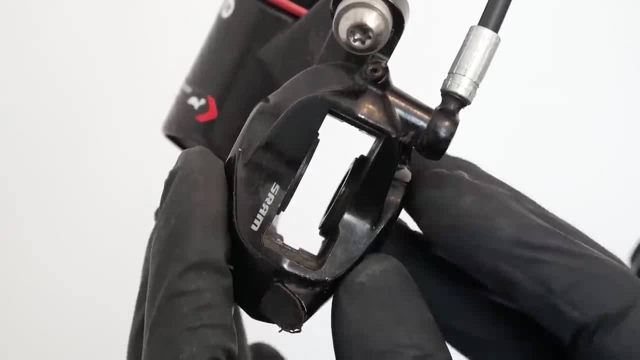 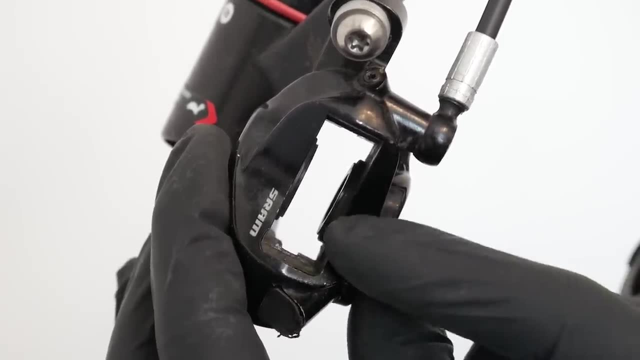 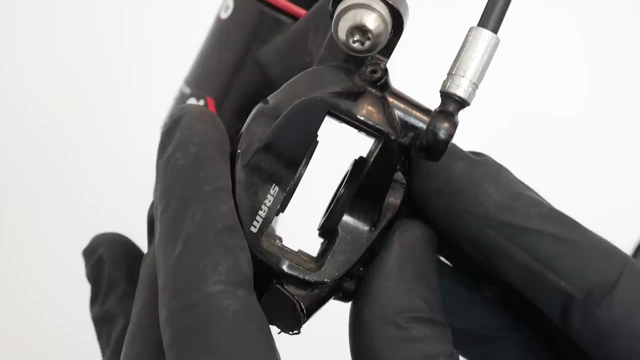 our caliper. And one very important thing: we should never squeeze the braking lever when the braking pads are removed, or the braking pads are there but the wheel is removed, because we can cause some oil leak and really severe problems. So never pull the braking lever. 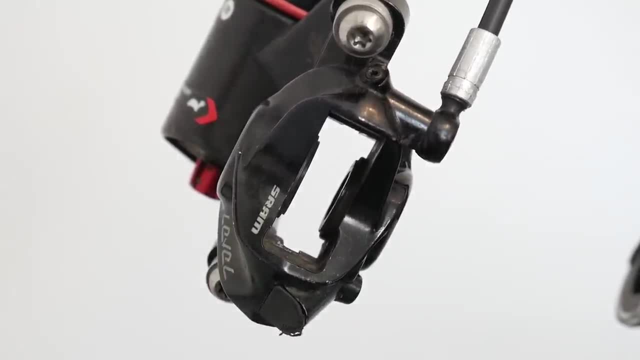 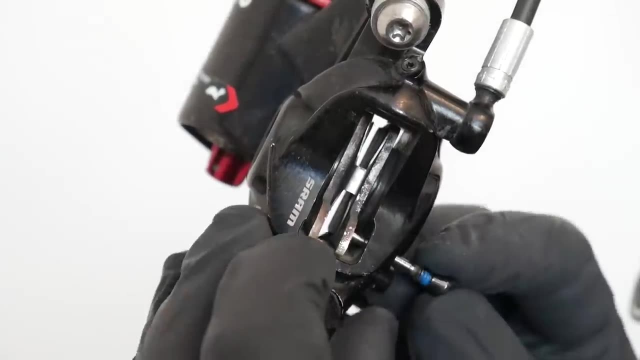 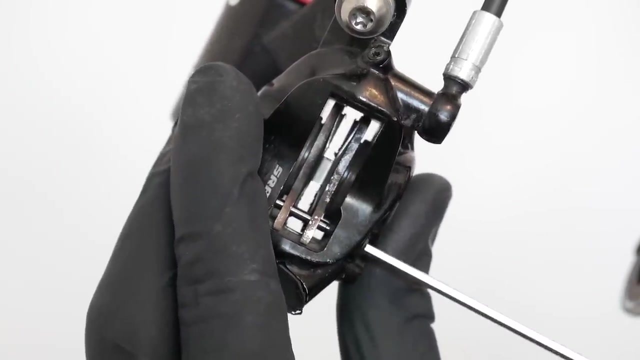 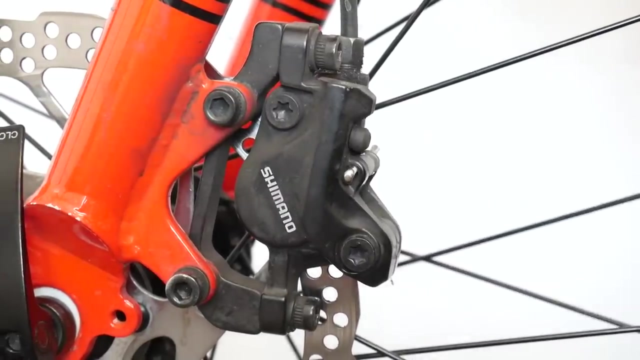 when there is nothing in between the braking pads. Now let's just put it all back together, which is pretty simple, And here we have the Shimano system with a special pin. so there is no bolt, nothing that we would unthread. I just have to remove the pin. 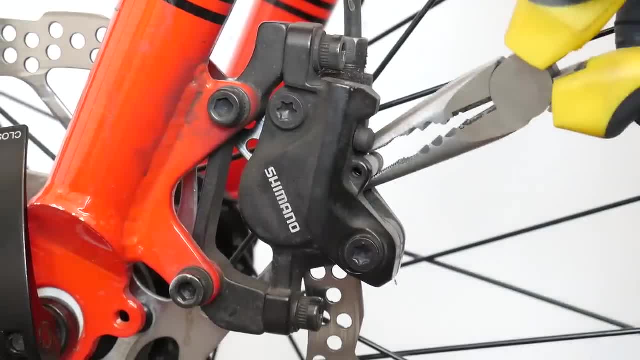 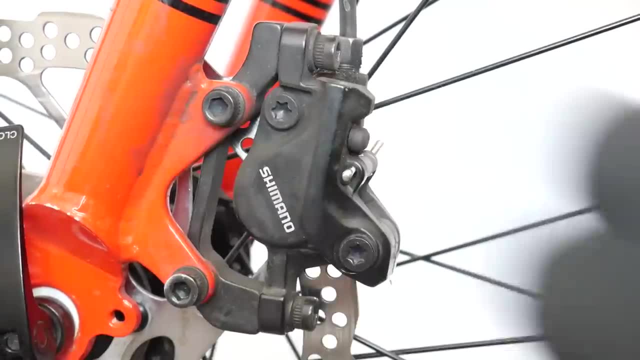 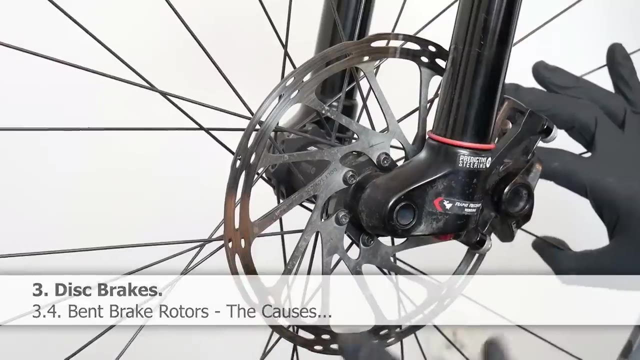 and, once removed, I will be able to remove my braking pads. All right, so what happens when our disc brake rotor is out of true, and what's the reason for that? There are mainly three reasons for this problem. It can be caused by overheating, So 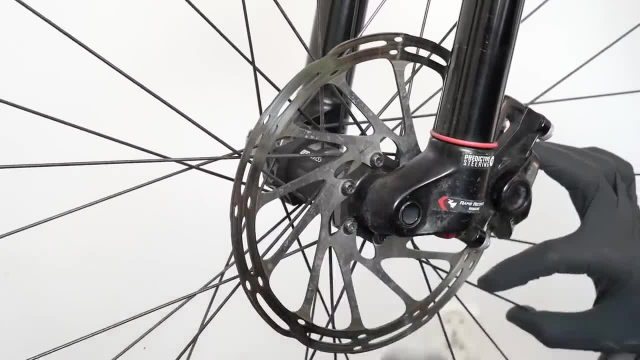 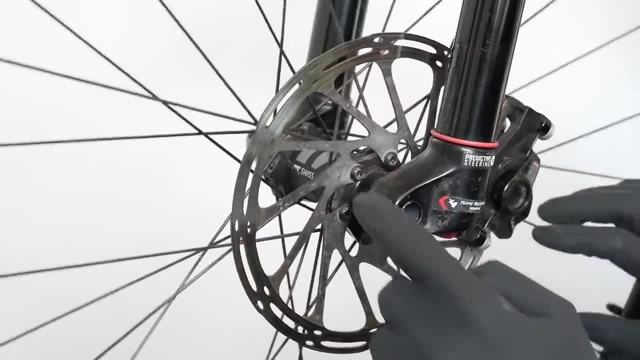 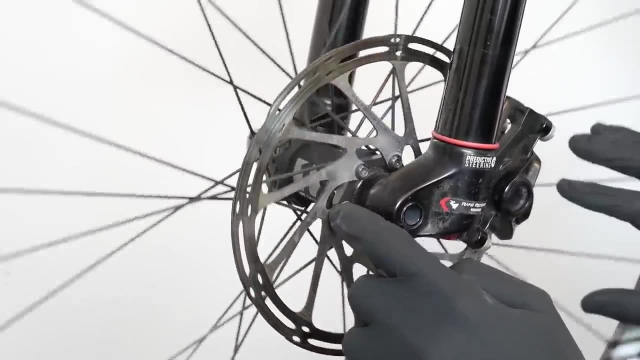 when we really abuse our bicycle on the descents- long descents- and we overheat the disc brake rotor, it can get a bit out of true. The second reason is not using these mounting bolts properly. These should be fastened with the even force and also while you are assembling the disc brake rotor. 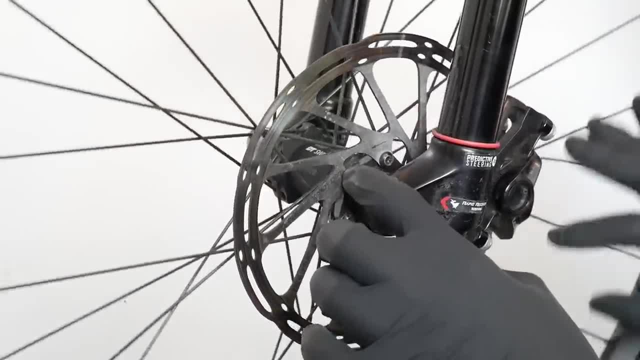 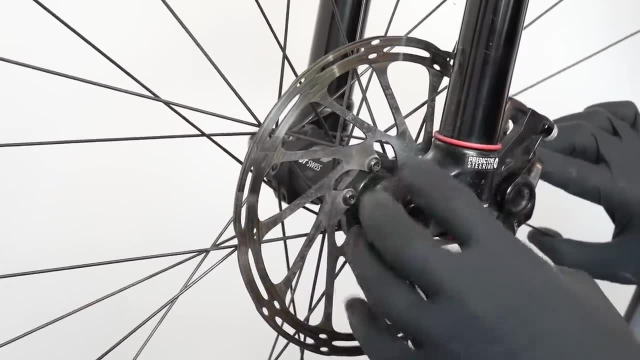 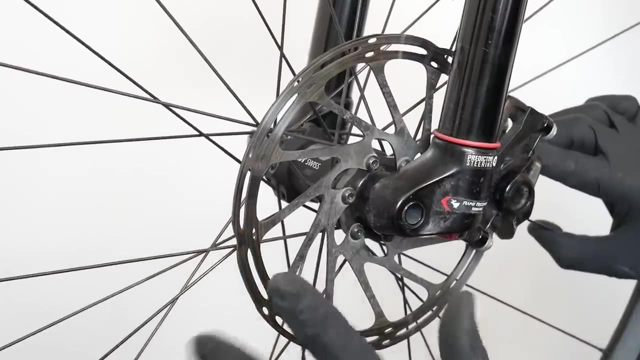 to your hub. don't just fasten those in a row, but like every other bolt, so that all the forces working on the disc brake rotor will be even, Even, and then the rotor will be really true. The third reason is just the mechanical. If you 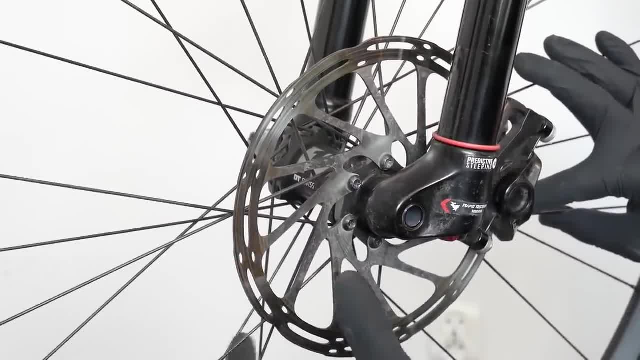 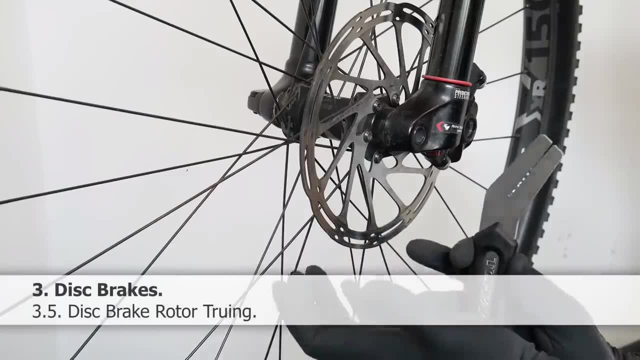 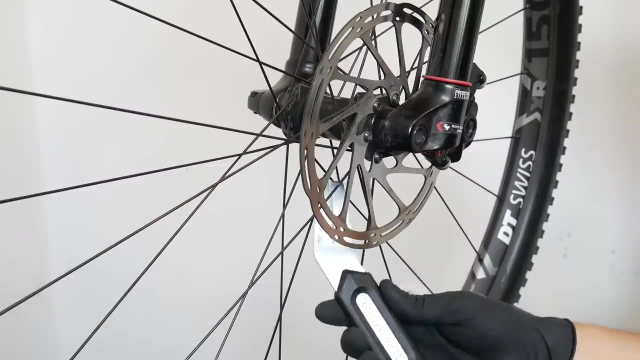 just lean the bike against itself during the transportation. it is pretty easy to damage our disc brake rotor, so make sure you avoid that. Trueing our disc brake rotor isn't really complicated, but it's a very good idea to purchase a special tool for that. It will make our job so much easier. First off, 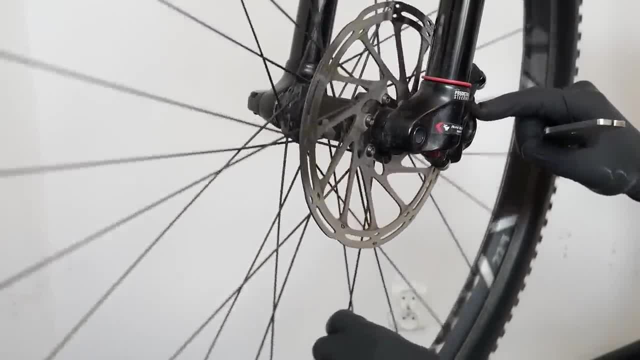 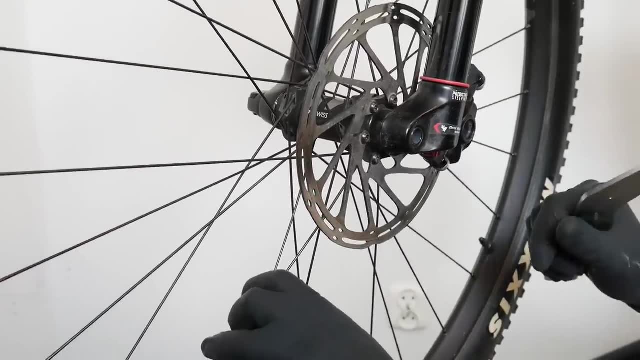 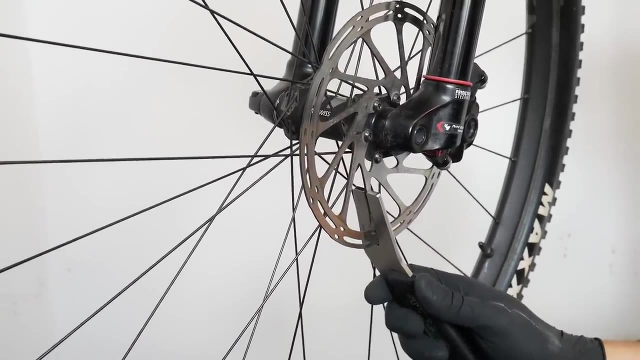 we need to find the place where the rotor gets out of true. Once we find it, we can use the paper or the bicycle light, as we showed you. Once we find the place, we will try to true it. Now, how not to do it? I would not use the tool. 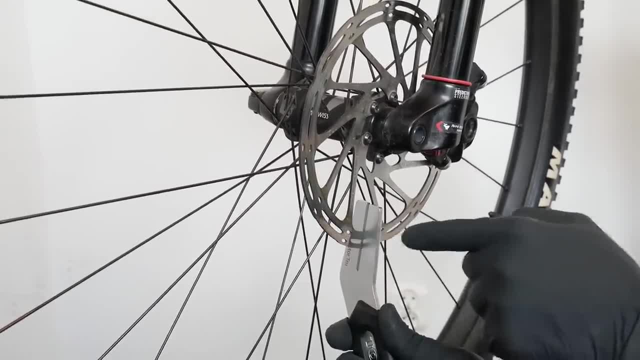 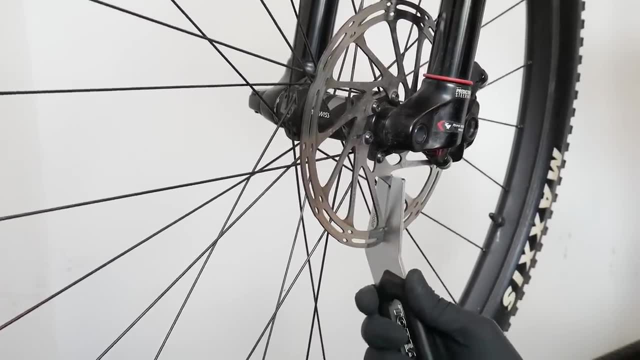 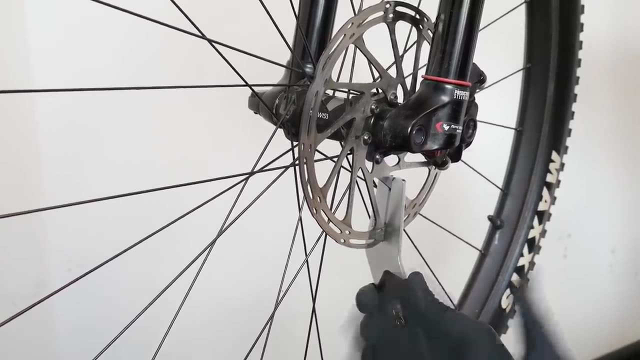 just like this right here, because I will just mess up with the surface of my rotor. I would rather use it with the arms or like that. So holding by the arms, holding them with my arm of of my rotor. it would be much better for the whole shape of the whole thing. 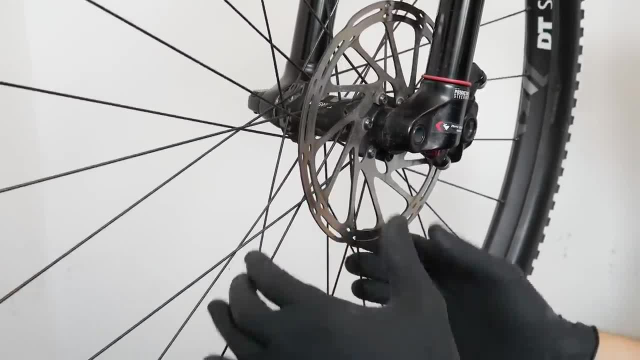 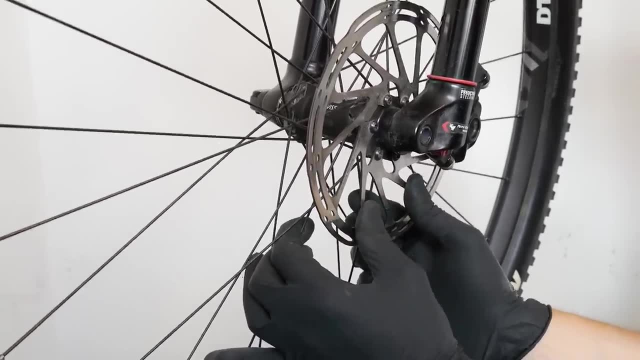 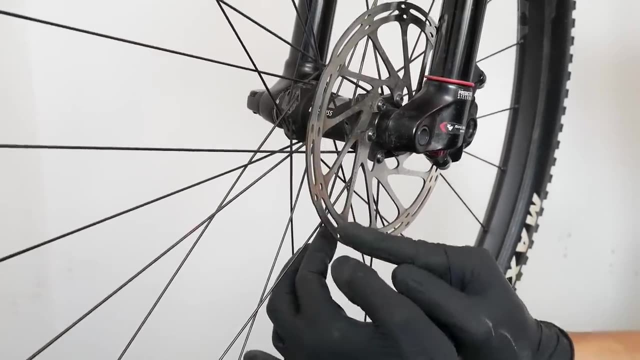 you can also do it somewhere on the trails. when something happens, crash or anything occurs and you want to just get home or to the finish line, you can push it with your fingers or pull it outwards. just make sure you try not to touch the braking surface with your fingers, because then you would have to decrease. 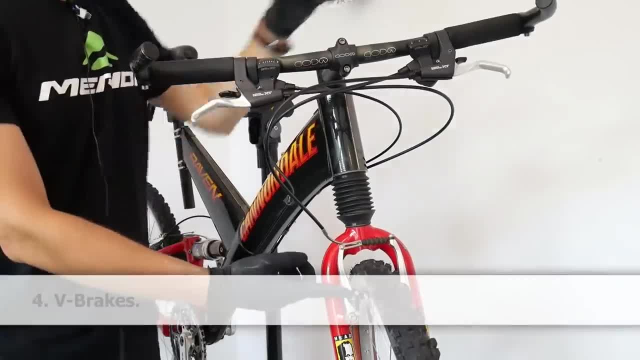 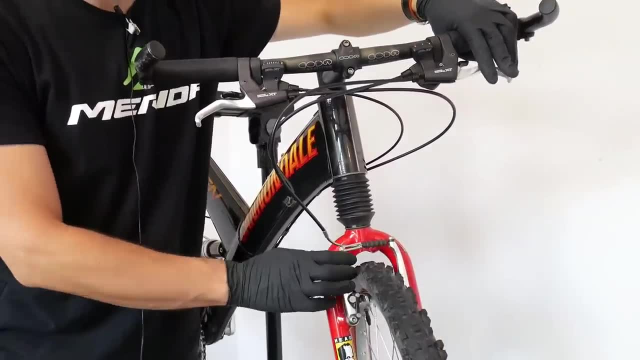 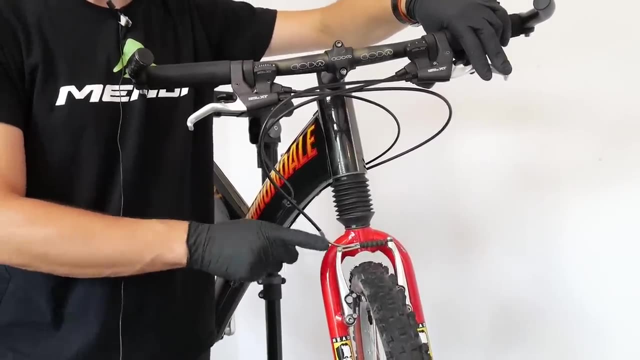 it, which will not be possible somewhere on the trail. these are the V brakes: very simple, efficient and good brakes. they were used on the professional mountain bikes in the past. now you can find this type of a brake on some entry-level mountain bikes, but also, especially as a mini V brake version on the cyclocross. 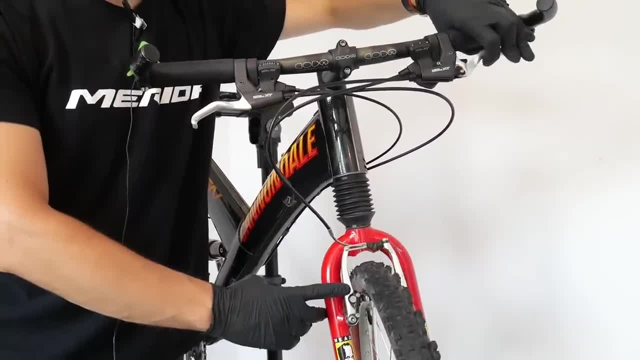 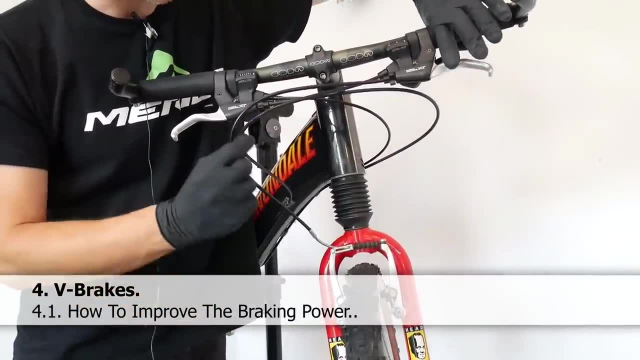 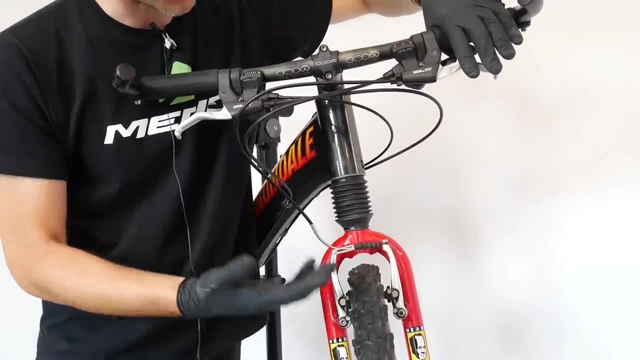 bikes and some road bikes. let's see now how to maintain and adjust these. V brakes are the mechanical brakes. that means these are optimal brakes for mountain biking. they are operated by a cable which is here inside the housing. it's good to know that, because the power of these brakes will depend largely on how clean. 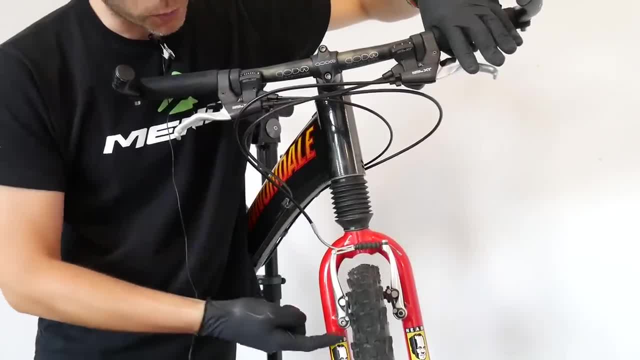 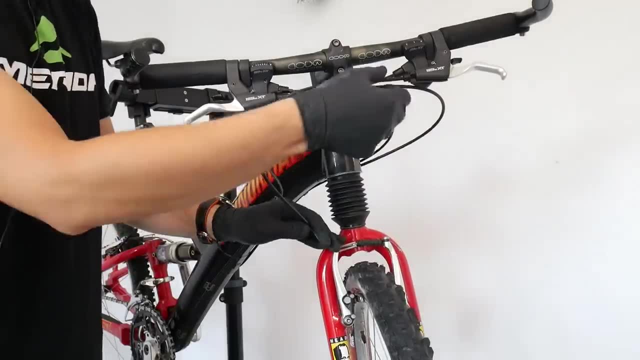 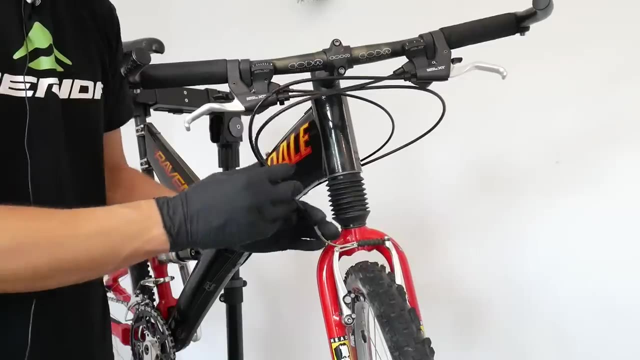 the housing and the cable is. and also we should take care of the pivots here. those should be also clean and greased regularly. let's start with the inspection of the cable. if the cable will be still in good condition, I'm gonna just clean it and put some lube on it and still use it. if it's in bad condition, 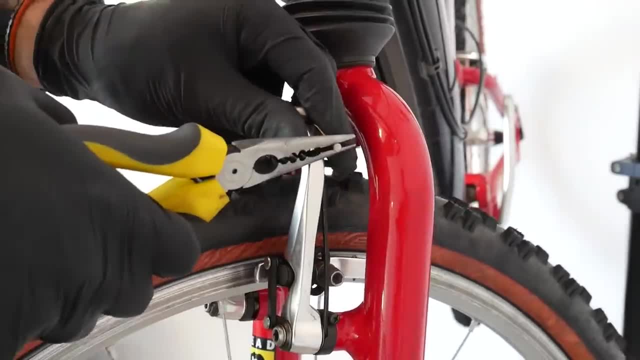 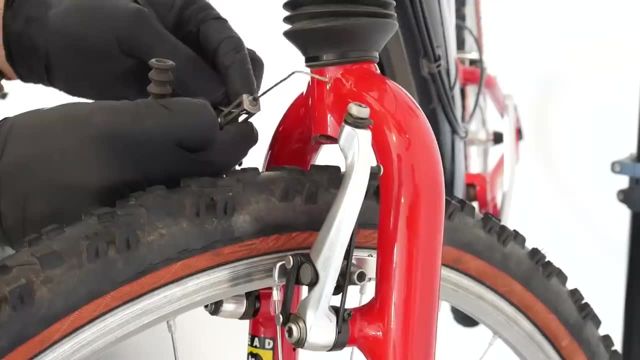 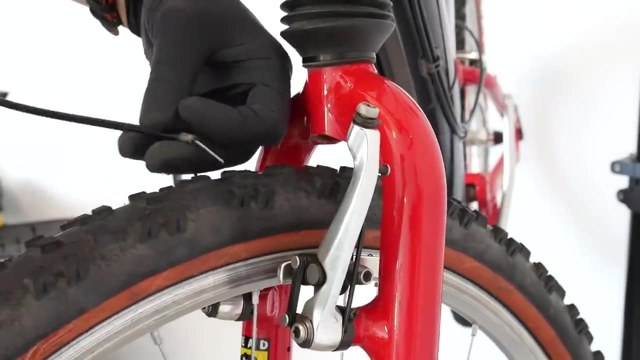 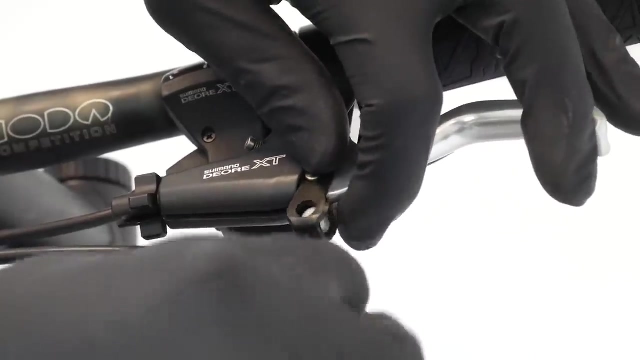 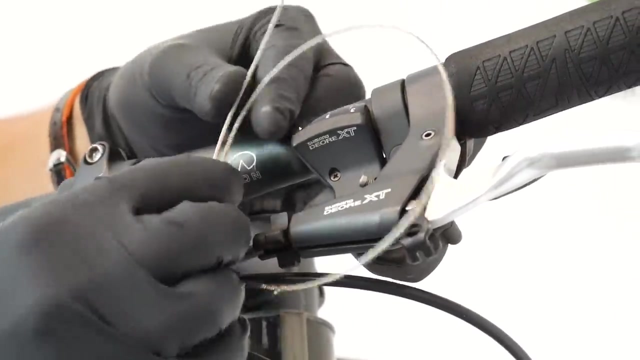 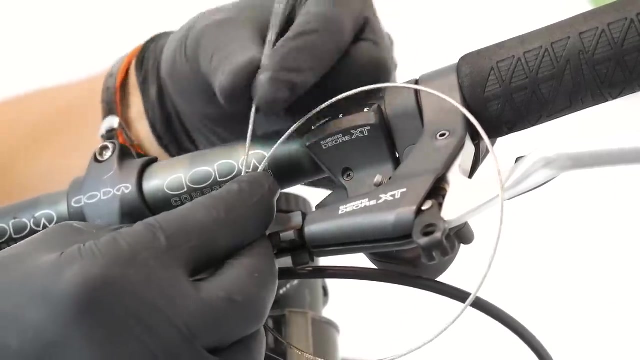 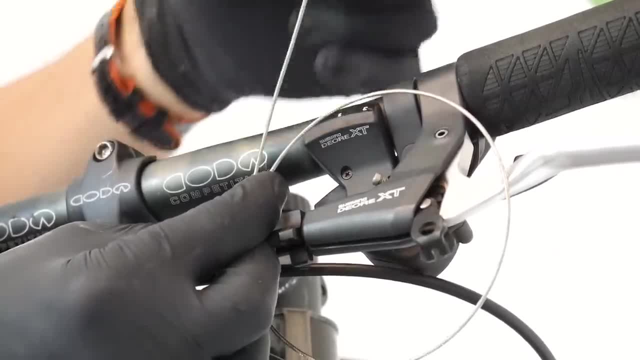 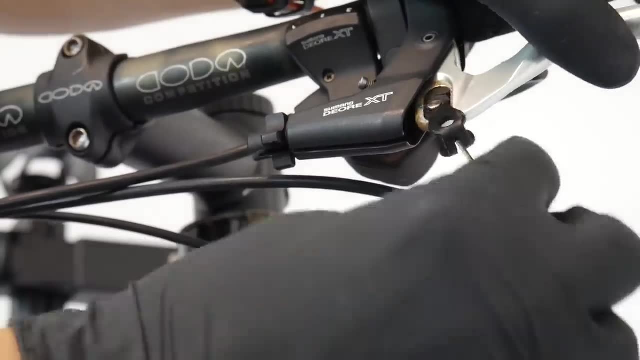 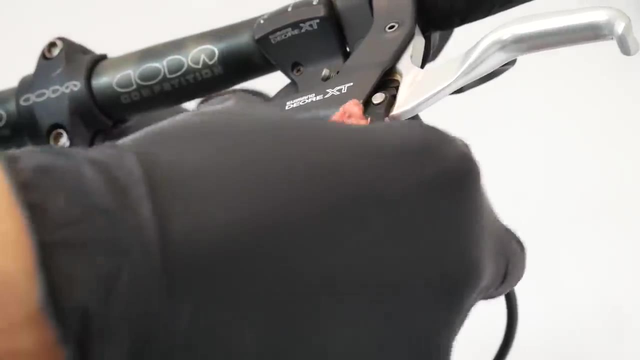 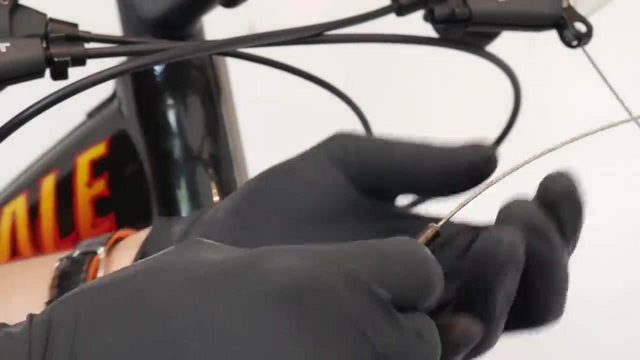 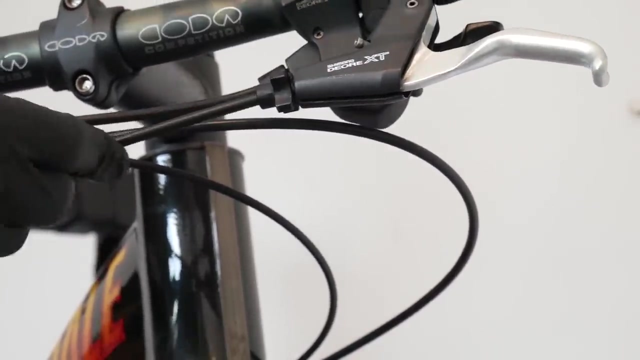 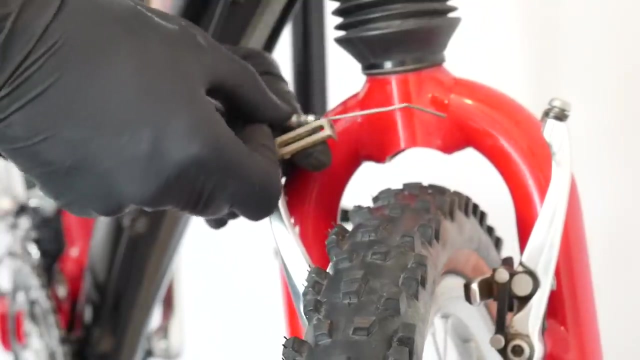 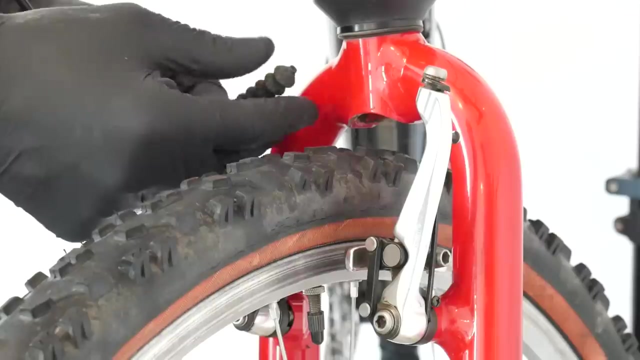 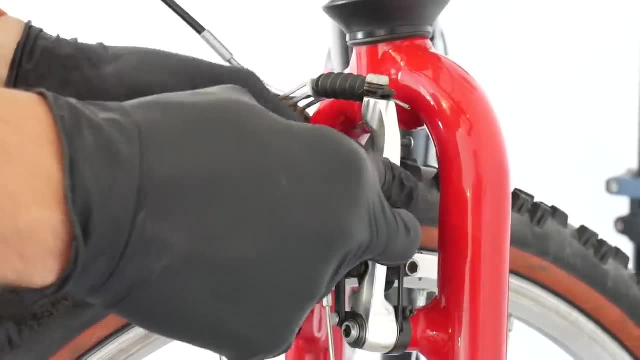 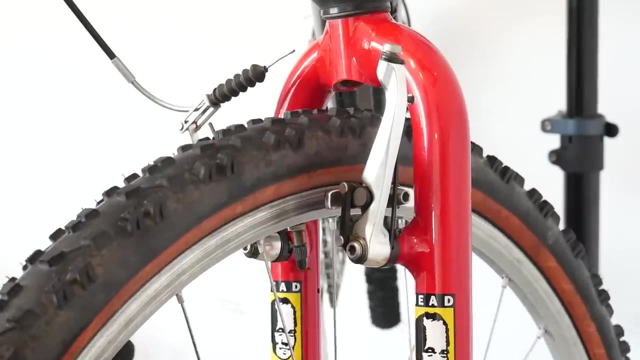 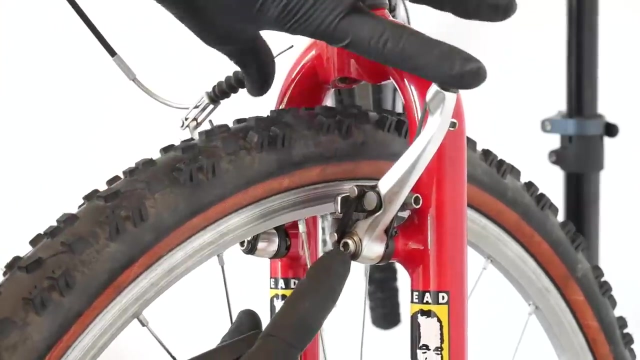 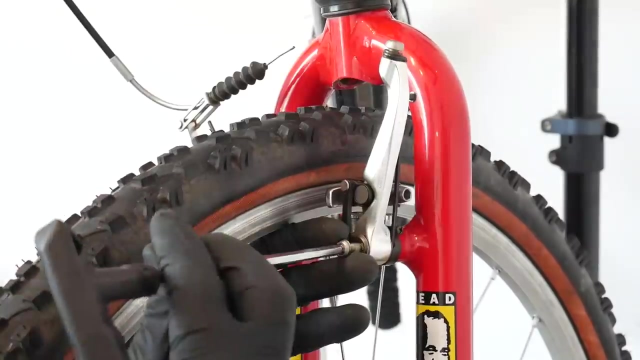 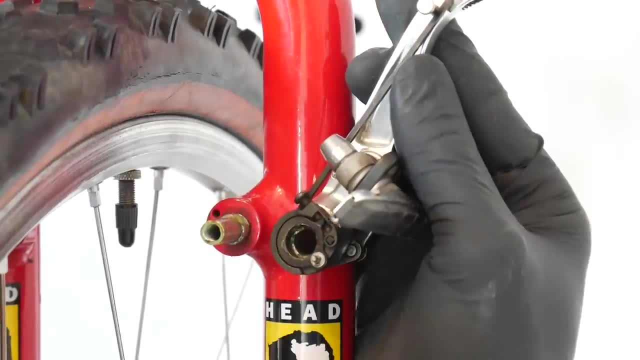 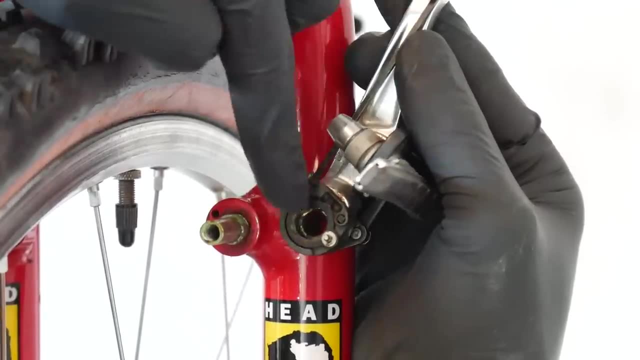 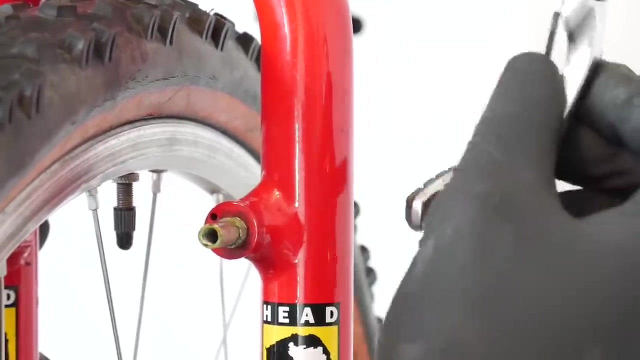 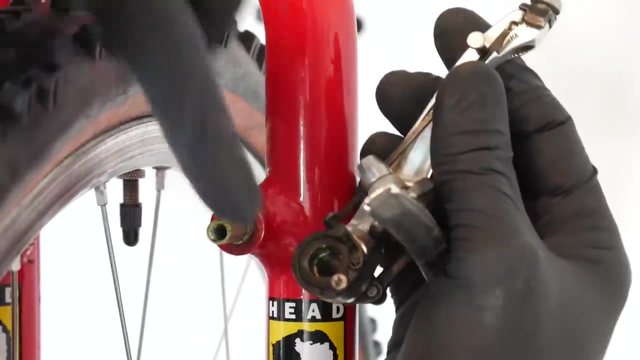 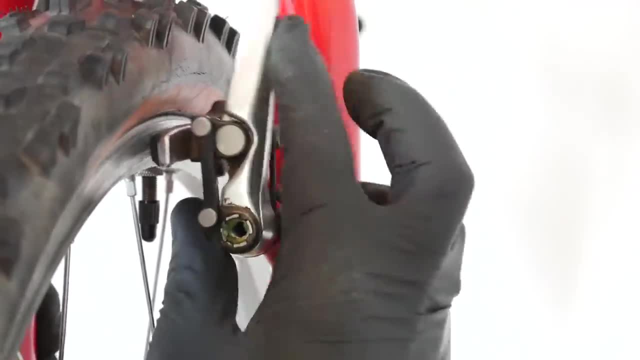 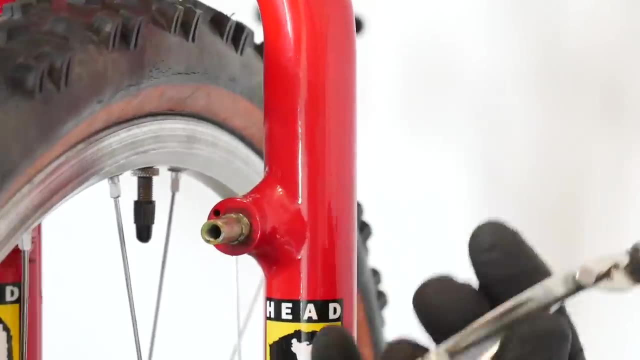 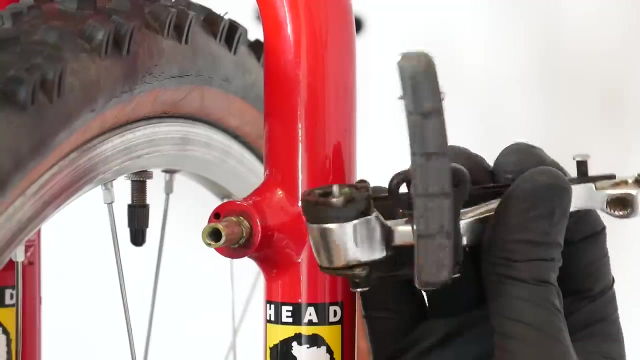 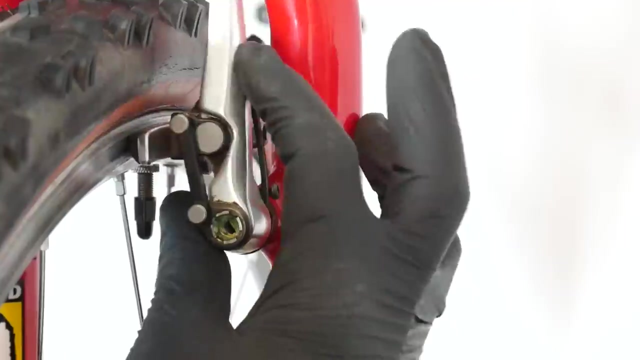 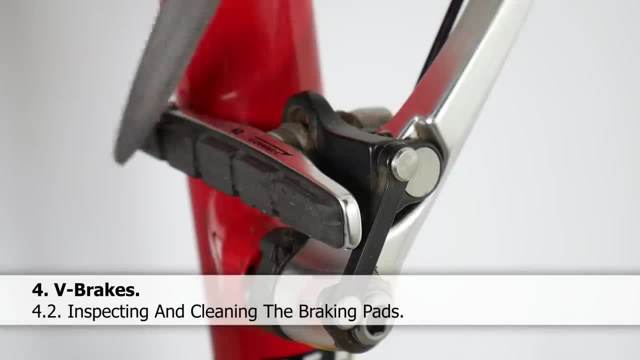 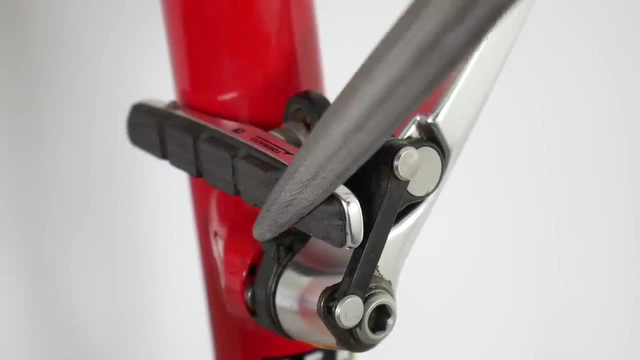 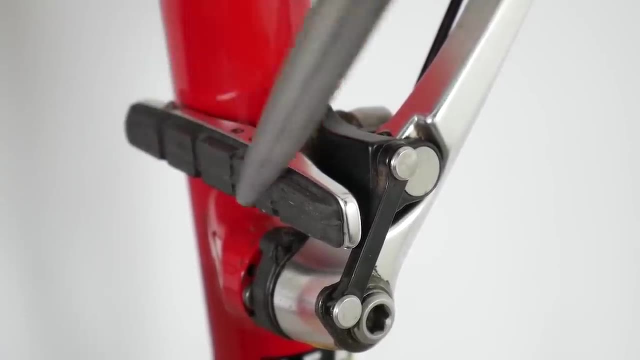 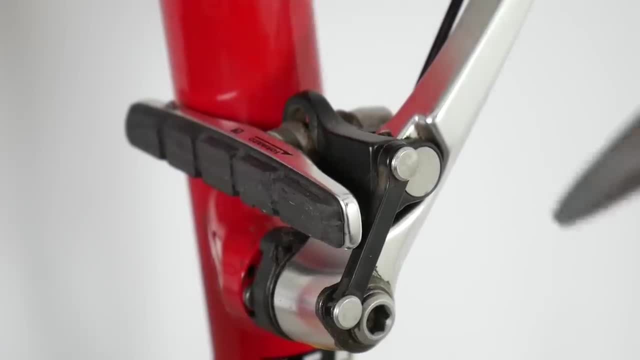 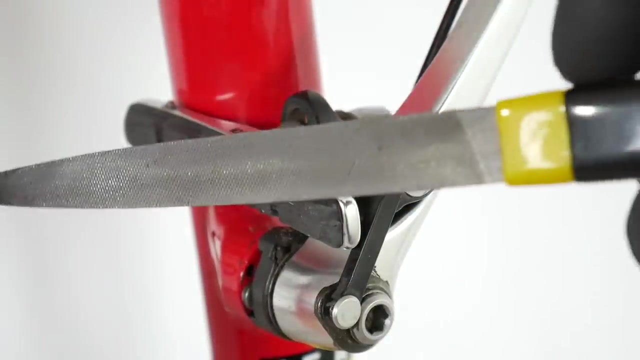 but if you take a closer look at the pad you're gonna see some particles in it, some pieces of sand, some dirt, some metal parts, and all these will wear down our rim pretty quickly. so we want to have our braking pads a pretty clean. that's why I'm using a special file from topic, but you can just use any type of a file. 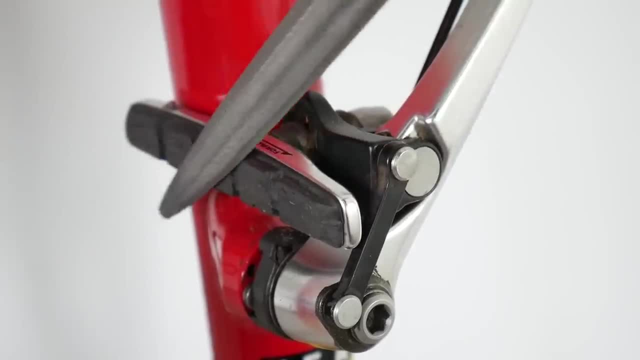 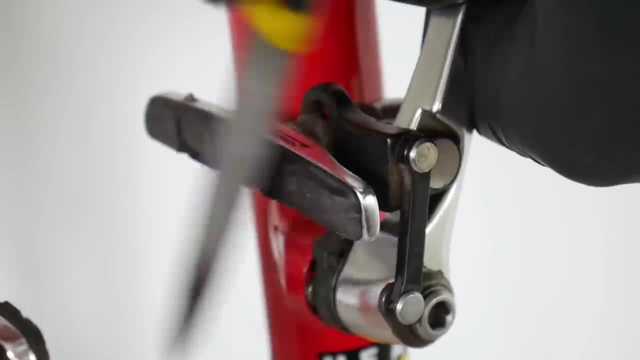 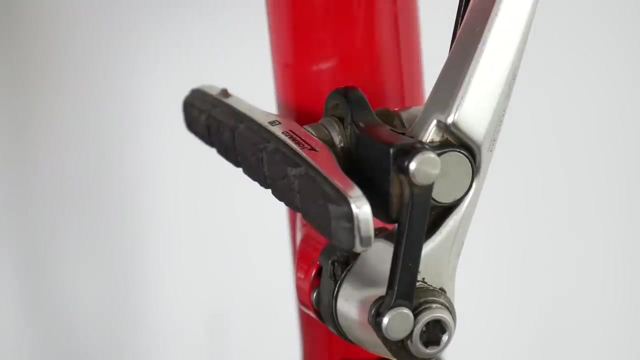 which will not wrap too much of a rubber. you just want to take off all this dirt. of course we are wearing down the braking pad by doing it, but we will prolong the lifetime of our wheels a lot. now the braking pad looks much better. there is no particles in it. it will also break better and you will not hear that. 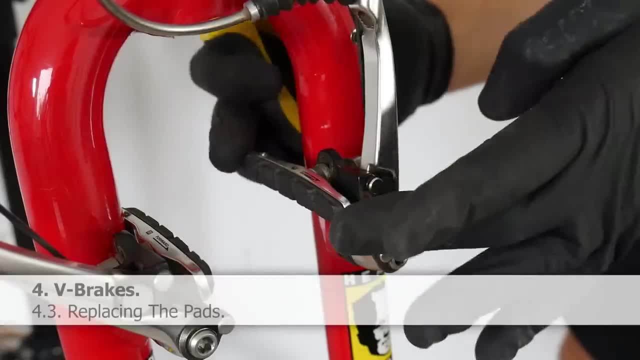 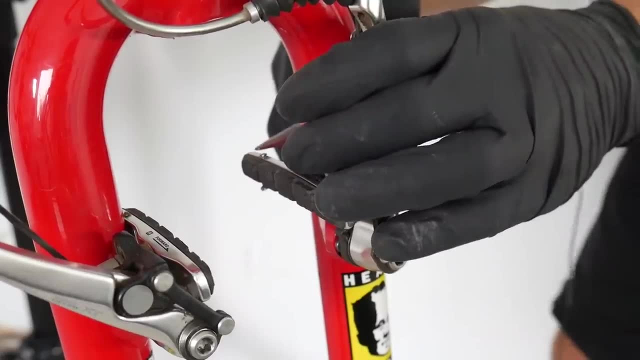 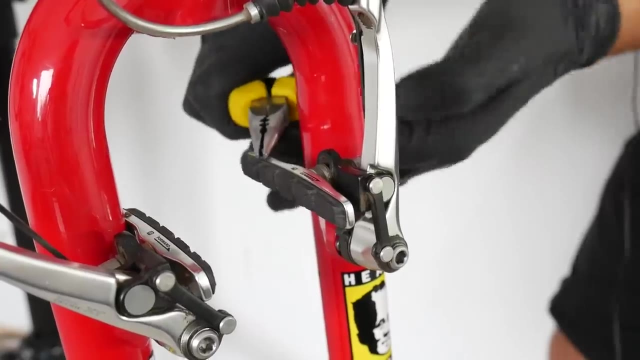 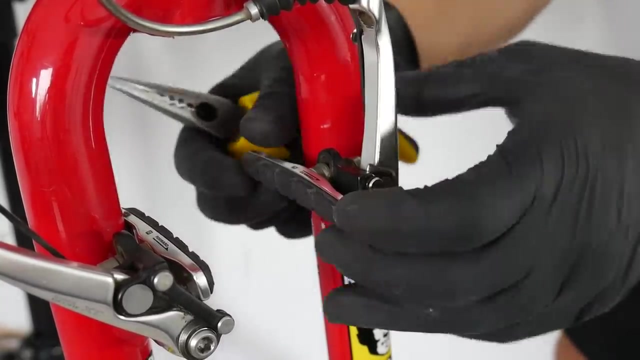 metallic sound while braking. replacing the pads is very easy if you have a cartridge like this- I do. you've got here some kind of a pin. I'm just pushing it from the, from the bottom first, and then I can pull it off with my, with my pliers, and now it's very 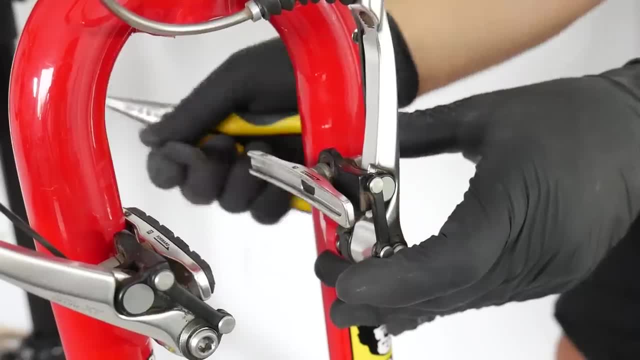 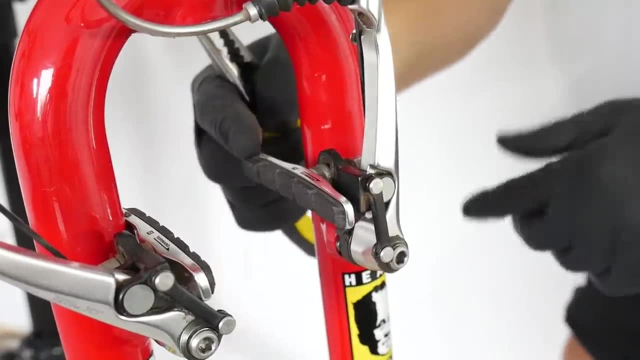 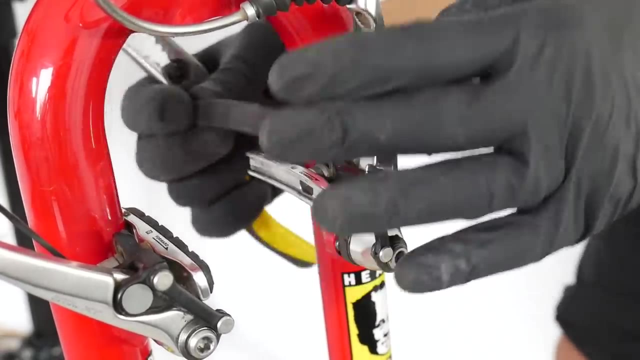 easy: simply slide it to the back and then we can put a new one and put the pin back. if you don't have a cartridge system, I recommend that you buy one, because then we are only replacing the compound and it takes very little time and you don't. 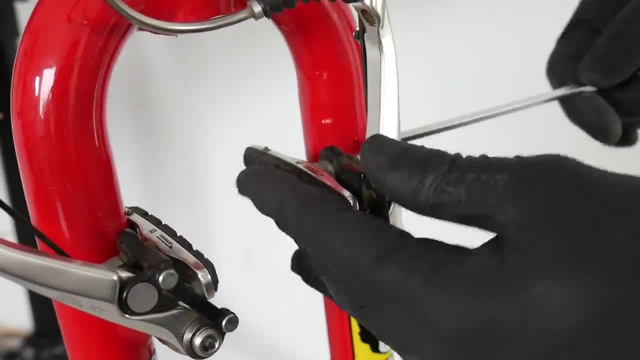 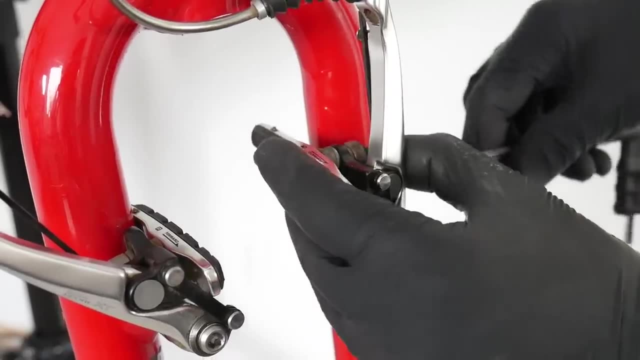 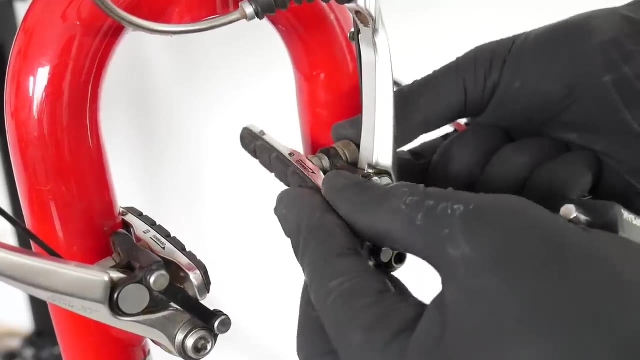 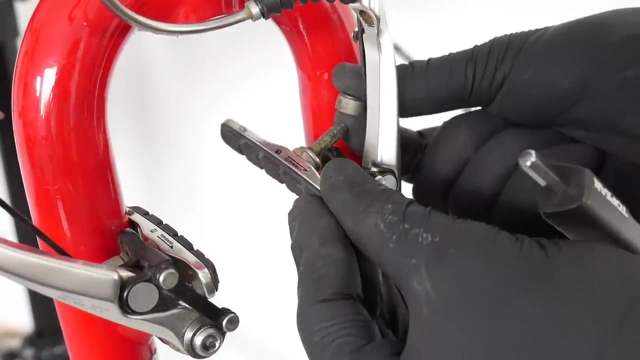 have to readjust the brakes. if you don't have a cartridge system, you just have to replace the whole thing, which is also easy, but you're gonna have to readjust your brakes. now, very important thing here is when you are removing the braking pads. just pay attention to all the spacers which can fall to the to the floor. 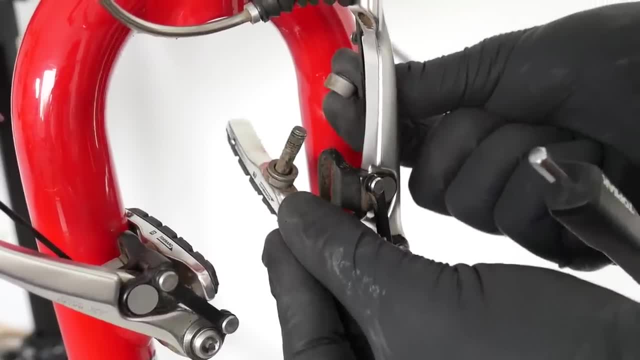 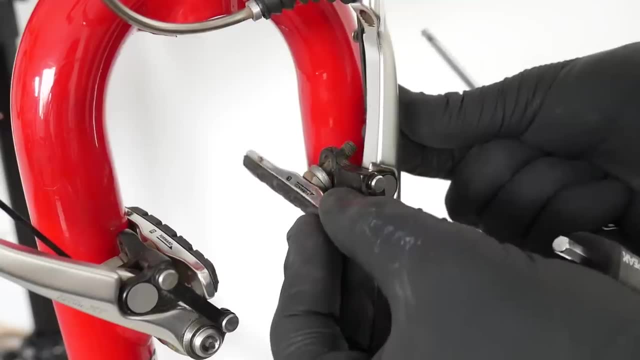 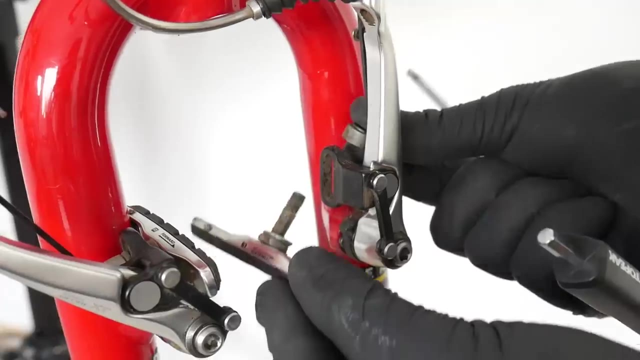 because we need to put those in the same order. if we don't do it correctly, we're not going to be able to adjust the brakes as they should be aligned. so remember to pay attention to all these spacers and then put the new braking pad and make the whole job easier. 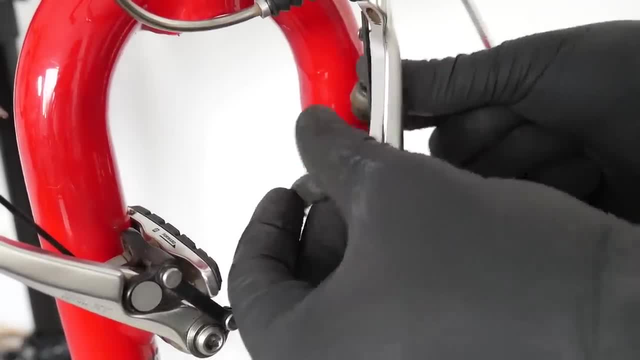 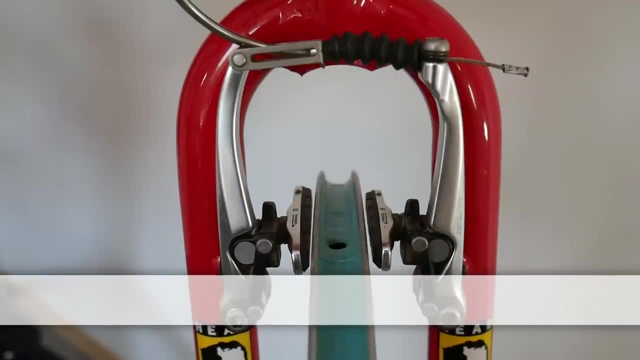 Thank you for watching. If you liked this video, please subscribe to our channel. See you in the next one. Bye, bye with the alignment just as shown in the video, and now we will learn in just a few steps, how to adjust our V brake so that they will be pretty powerful. first, 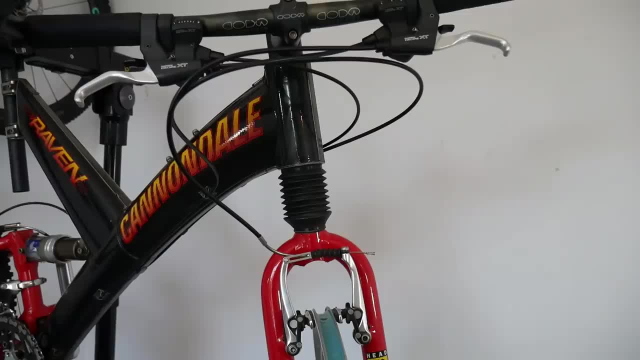 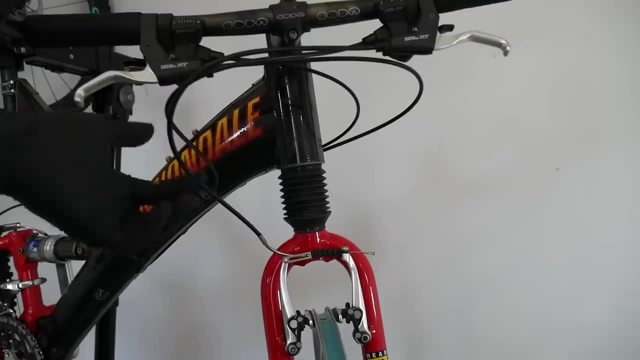 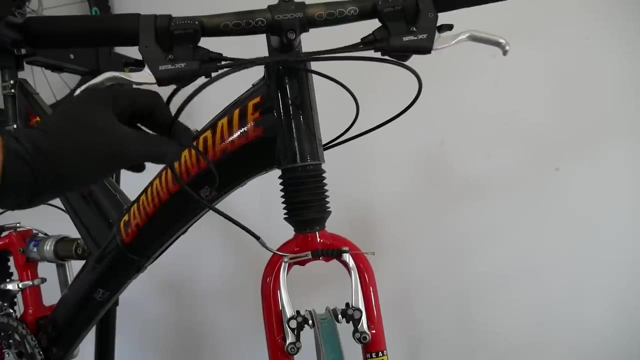 off. let's just see what kind of adjustments we've got. the first adjustment we've got- and many people would really not notice it- is the length of the housing. by manipulating with the length of the housing, we can make our V brakes working smoother and also we can avoid spongy brakes. 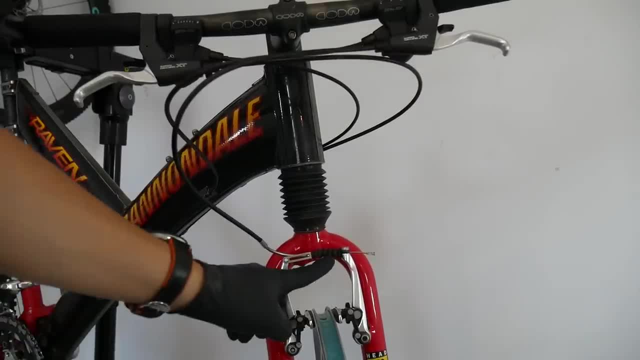 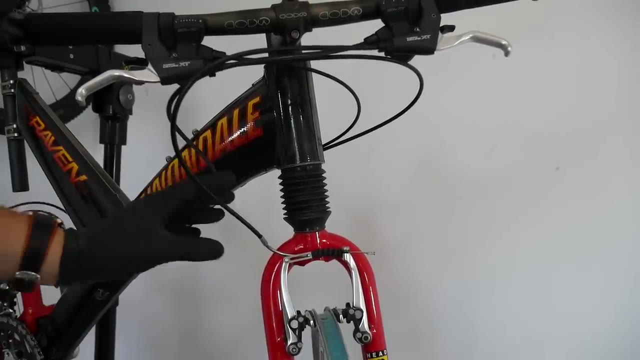 first thing that I'm noticing here is that this part of the cable is being pushed upwards. can you see that we would like to have, we want to have a really straight line between those two arms of the V brakes. that means this housing is too long and it pushes this aluminum part or steel part upwards, just like. 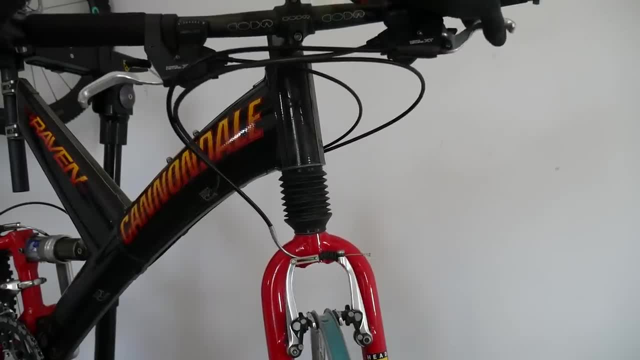 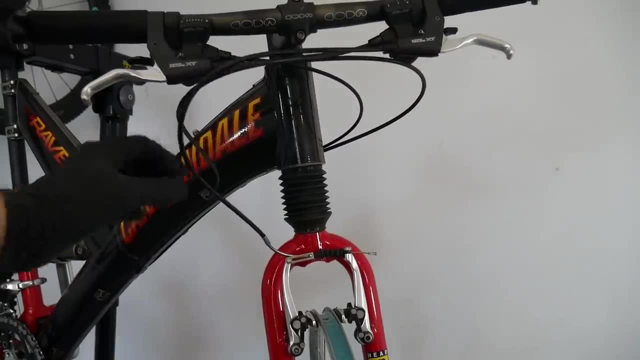 that, so that we are getting just a little bit of a sponginess right here. can you see that? Can you see how the whole housing is moving? So we need to cut this a little bit and we're gonna do some cutting later. Now let's just move on to different adjustments of those V-brakes. 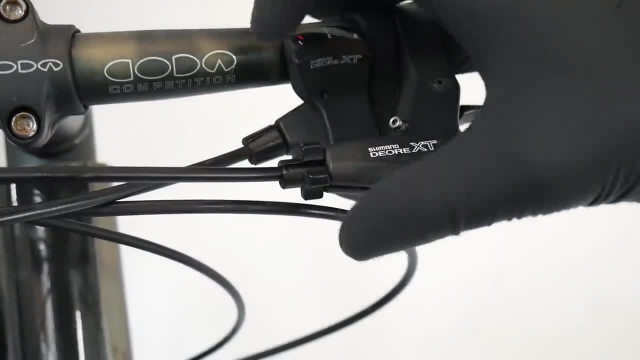 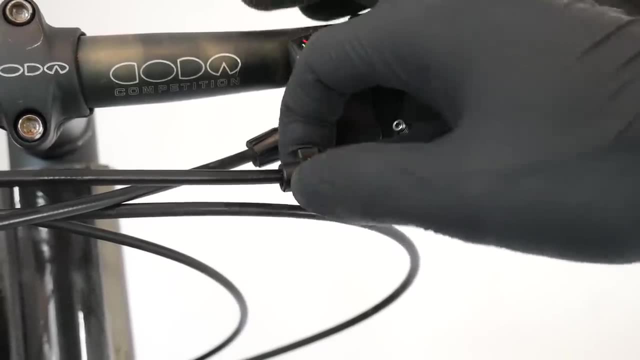 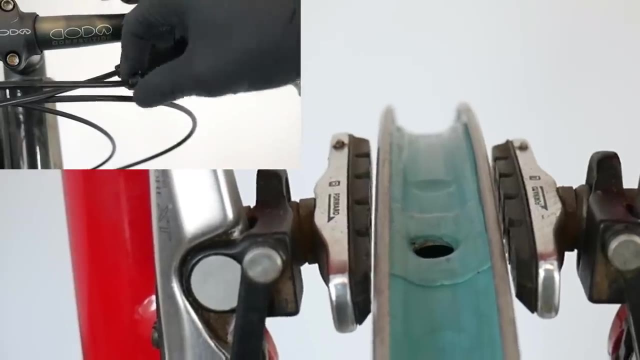 One of the basic adjustments we can do on our brakes is the cable tension, and for that we can use the barrel adjuster. So I'm unthreading it right now and, as you can see, those braking pads come closer to the rim. When I'm threading it back, I'm getting more distance between the braking pads and 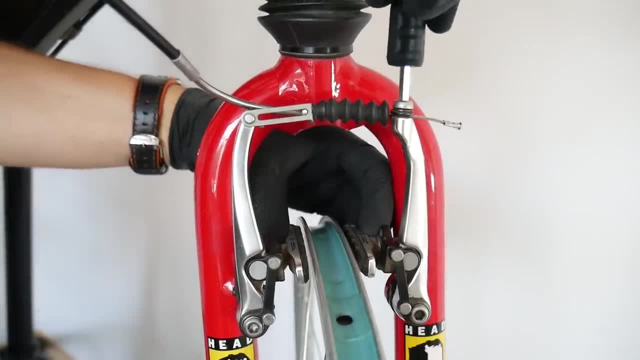 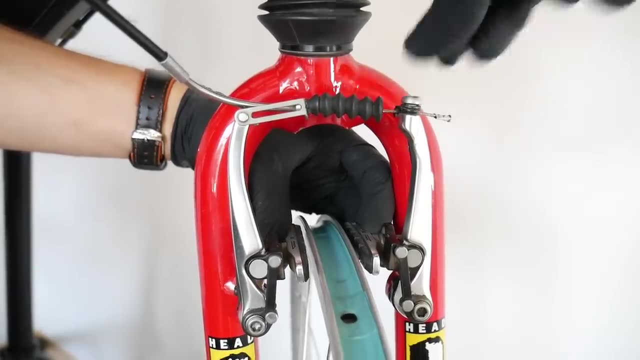 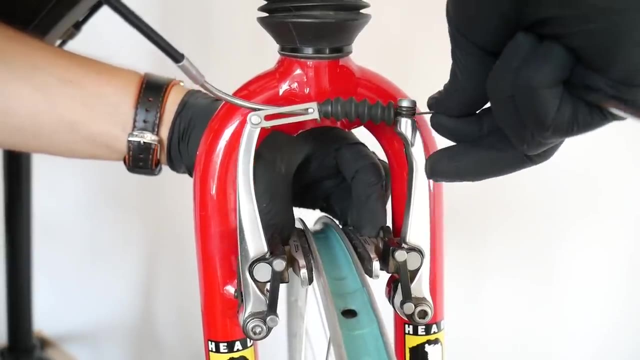 the braking surface, which is the rim. Of course, if you want to make some larger changes on the cable tension, we use this mounting bolt which is assembling, fastening the braking cable. Now we can either make this gap between braking pads and the rim larger or smaller. 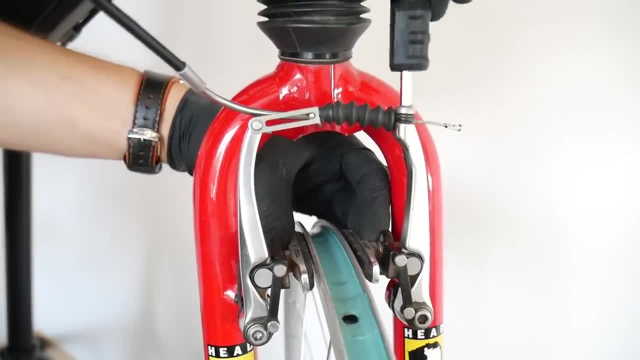 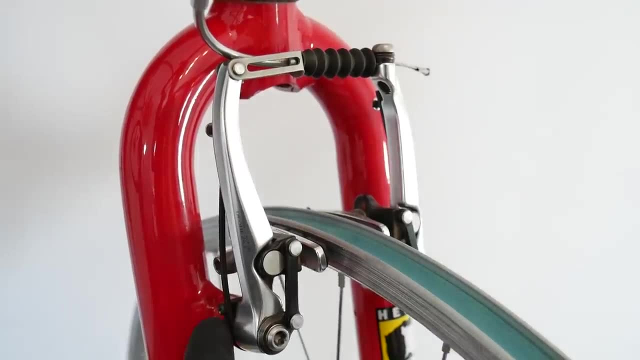 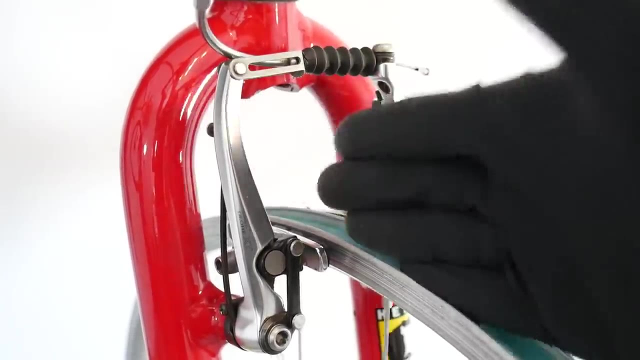 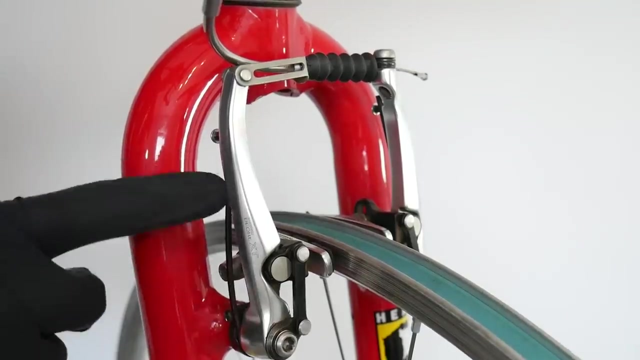 And then we use the barrel adjuster for the micro adjustments In order to center the position of our brakes against the rim. we're gonna use these little screws, but first off we wanna make sure that our wheel is in line with the frame or with the fork, and now we can proceed to the adjustment. these little screws will regulate the tension. 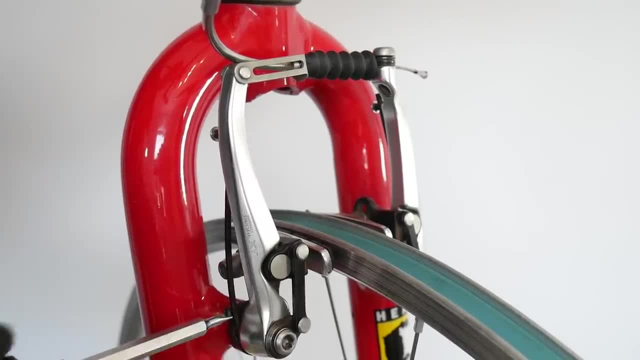 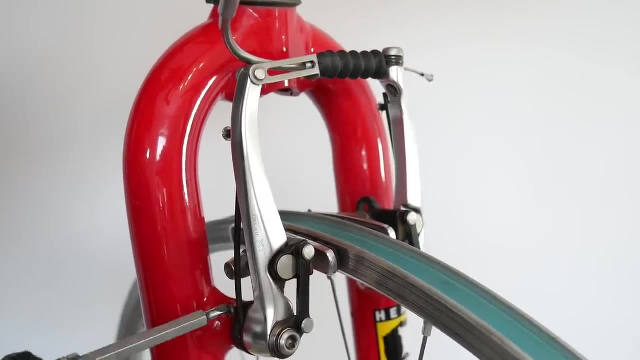 on this spring. so if I'm unthreading this one, I am lowering, decreasing the tension of this spring. So if I'm unthreading this one, I am lowering, decreasing the tension of this spring. so if, as you can see, the opposite arm is just pulling the whole brake towards the left, 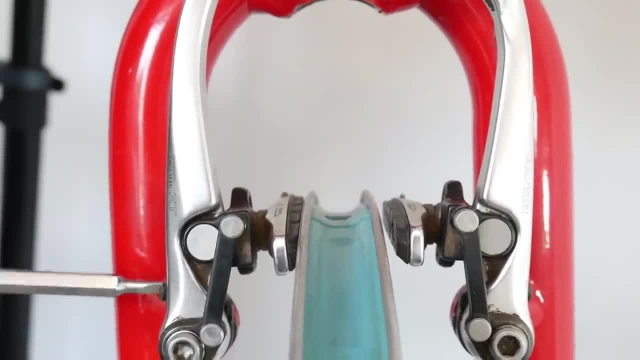 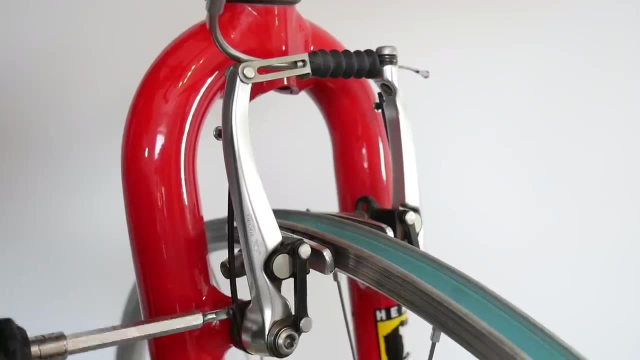 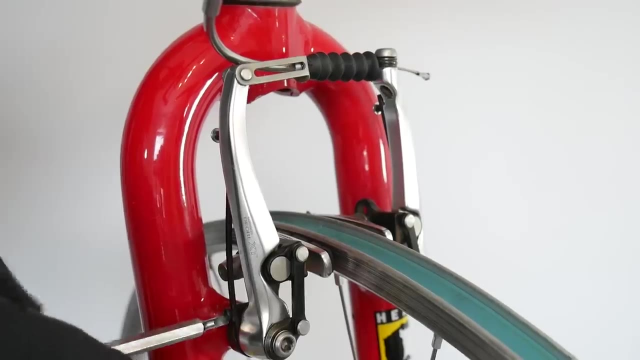 side. and now when I'm increasing the tension of the spring, I'm just pulling the brake to my side, to the side of the brake which will have more tension on the spring. of course we want to have those brakes centered, so the distance between the braking pads and the rim should be even on both sides. I'm always 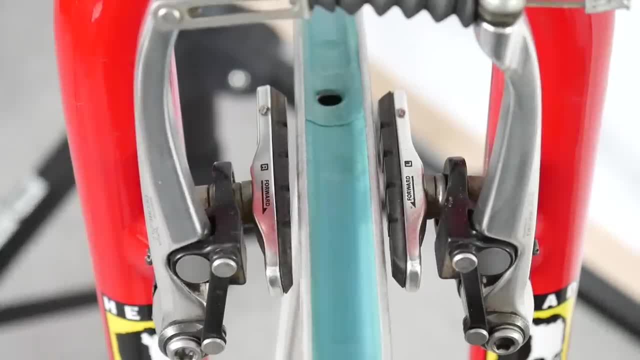 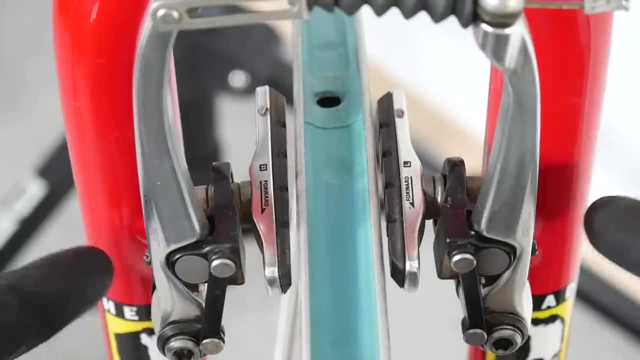 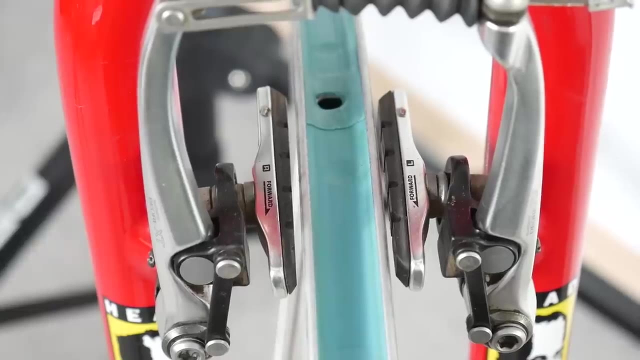 trying to have the minimal possible tension. that will make my brake working smooth, because as we increase the tension on both sides we'll still still have balance between left and right side, but we will feel more resistance while braking. so minimum tension here that that will allow for the brake to work. 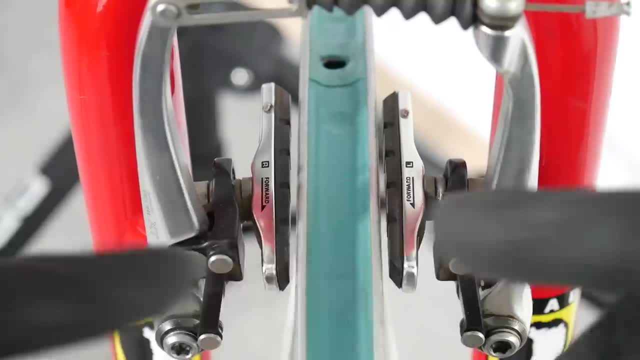 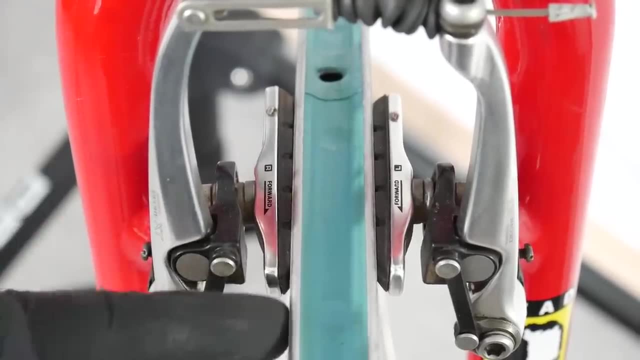 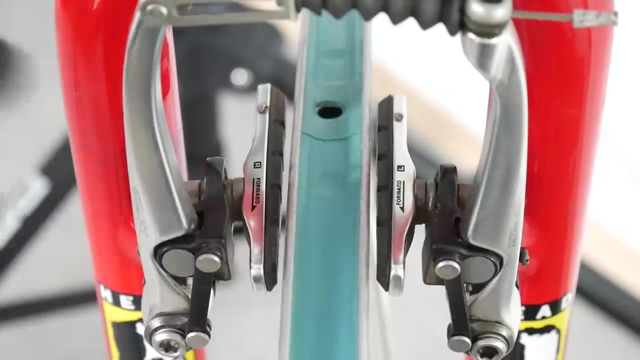 smoothly. now we can start adjusting our braking pads. it's pretty easy. what we want to have here is the whole surface of a pad touching against the rim. that means not being too low, not too high, because then the braking pad would rub against the tire and damage it, and we want to see those braking pads being we're down. 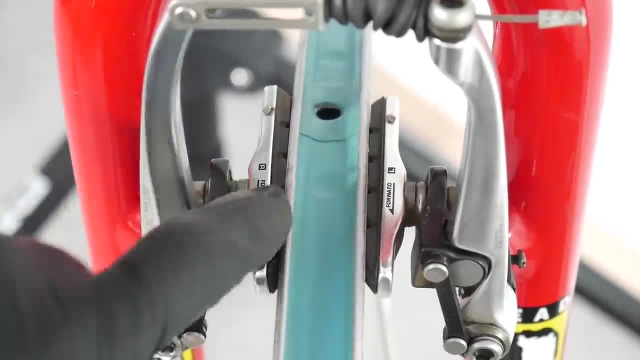 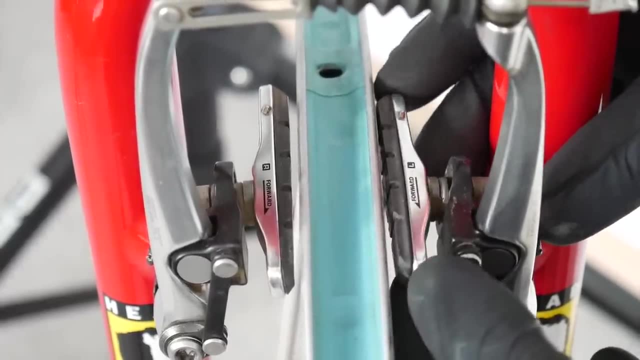 evenly on this side, on this side and also left and right. this is why we want to look at our braking pads and we want to look at our braking pads and we want to look at our braking pads at this level and set it at this level, just like this. 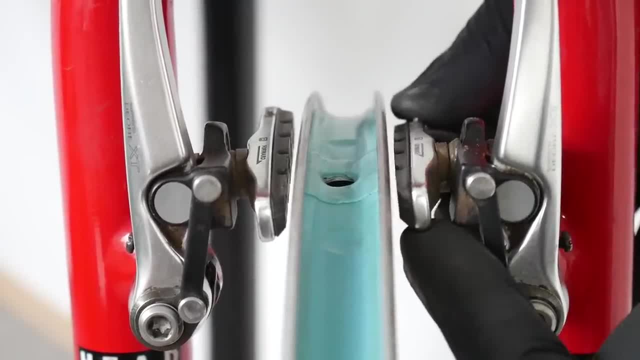 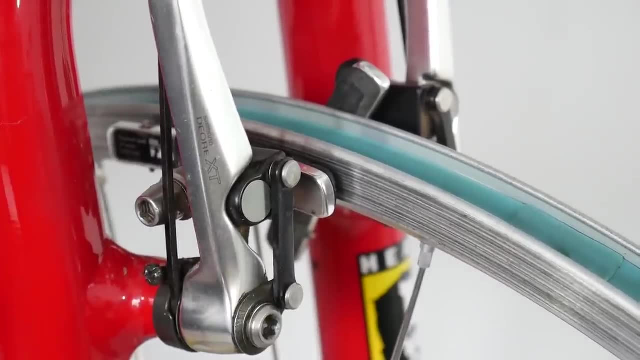 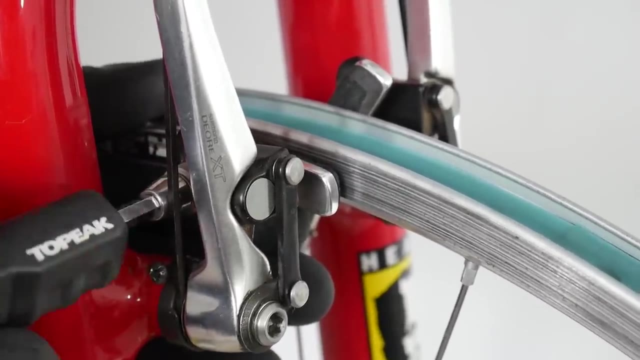 and we also want to pay attention at this position of each of those braking pads. this bolt is fastening our braking pads. this bolt is fastening our braking pads. in this case, this is a 5 millimeter allen key. when unthreading this one, we now have access to a hole adjustment so we can move those up down. at theате, at each of those breaking paths. this bolt will help. If I move all these braking pads, as you can see, all equipment realise when I first start這裡 that we also strengthen in the阅 это flexible braking pads affair. when I start Lindseyelin we can move those up. 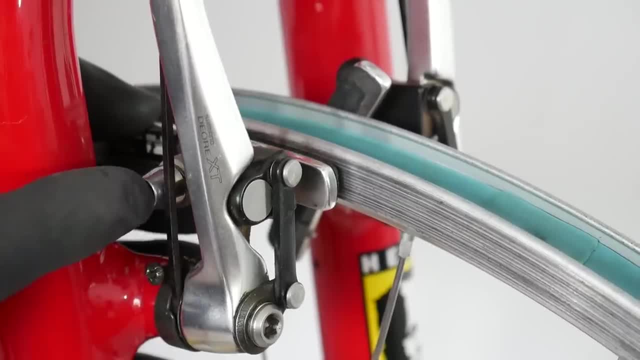 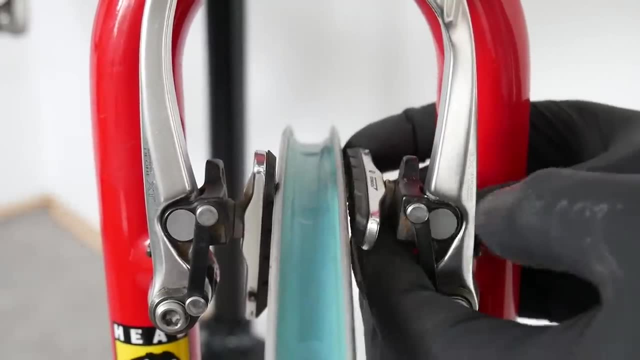 to use the Sevilla one, this petty bry sectors if there is no кли Glasøng, and in different directions. So we're gonna use this one bolt in order to adjust the braking pad. Both braking pads are loose now so that we can proceed with the adjustment. Some bike mechanics would recommend not adjusting those. 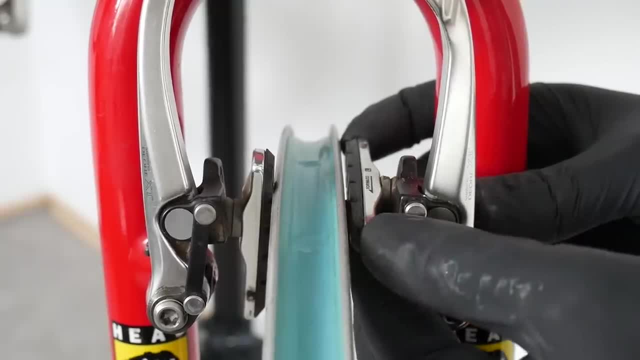 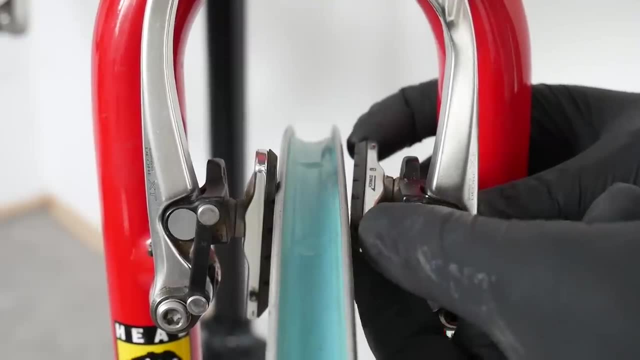 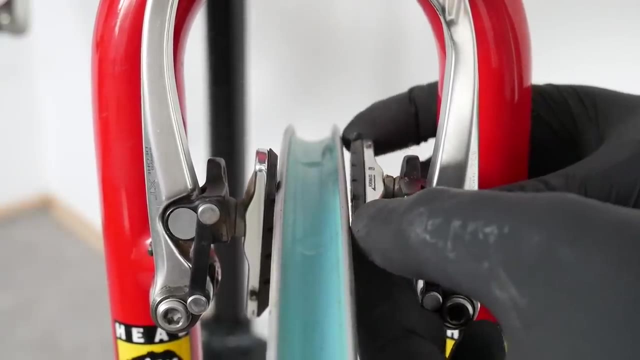 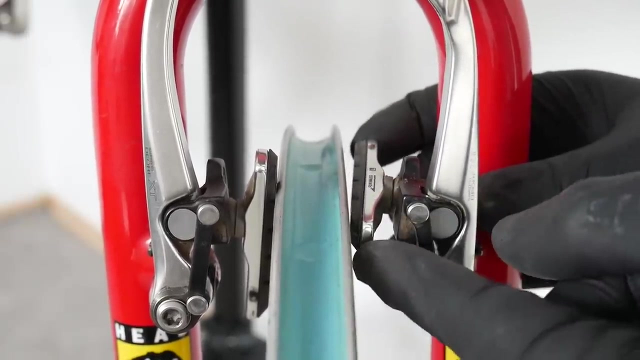 exactly parallel to the rim, but having slightly more distance in the rear than in the front. I'm just exaggerating it right now. It probably helps with the squeaking noise and also some say that the brakes are flexing while we brake, so it will help with the even wear of the on the compound when it's set like that. 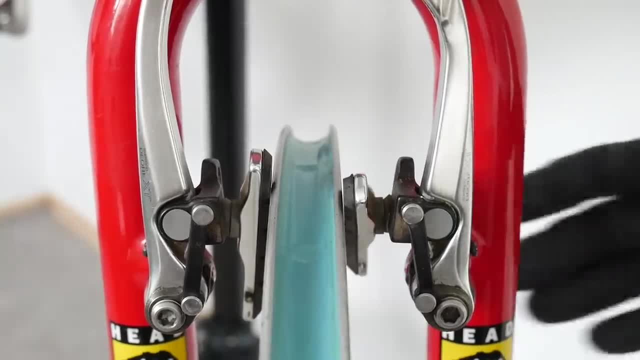 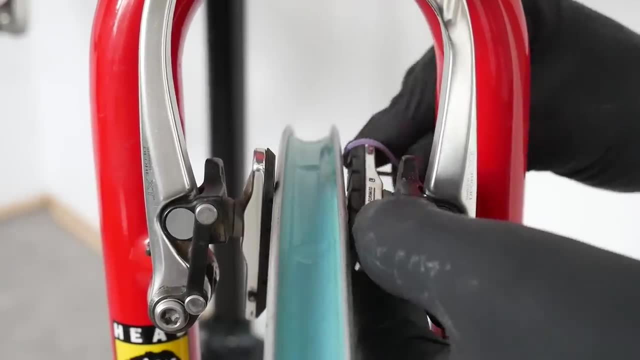 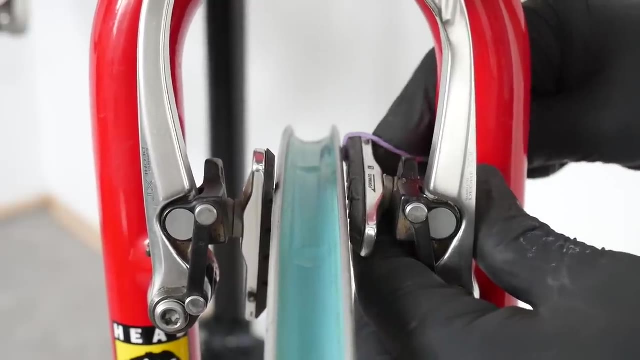 and not parallel. If you want to use this method, which I'm not a great fan of, you can also take some piece of a rubber, put it at the back of the braking pad on both sides, so that you will have this- the same exact distance on both sides, and now you can proceed with the 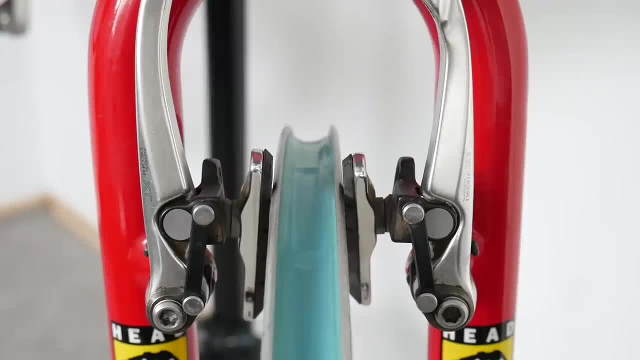 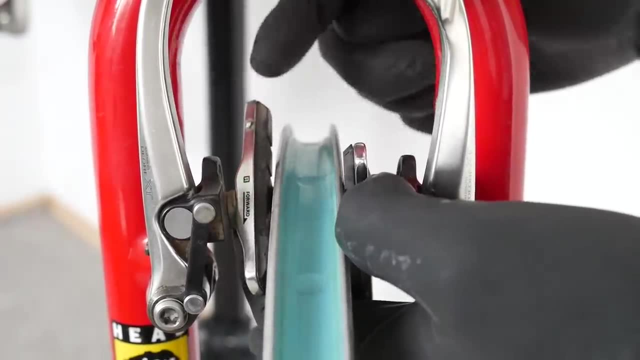 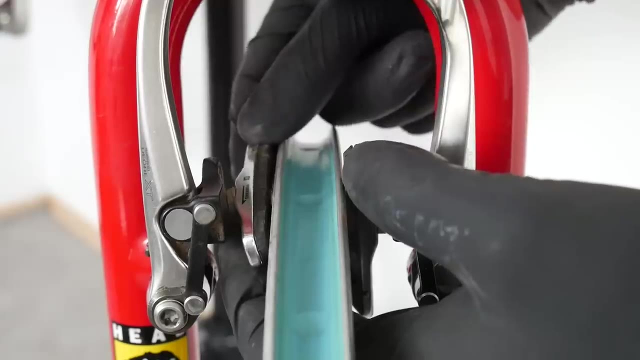 alignment. I'm not doing it with any of my bike and also my observation is that on this bike somebody did use this method and you can see there is more compound at the back of the braking pad than in the front because somebody did set it like this. So I'm not using this method. My method is much more simple. I 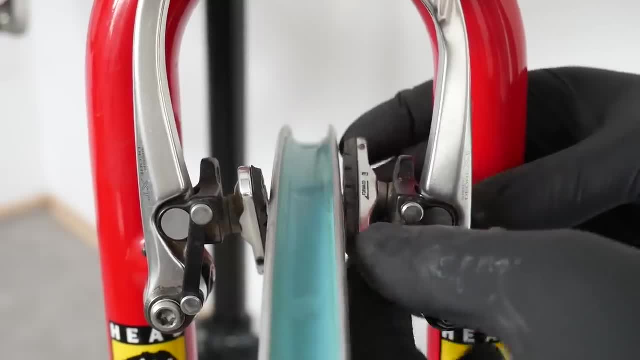 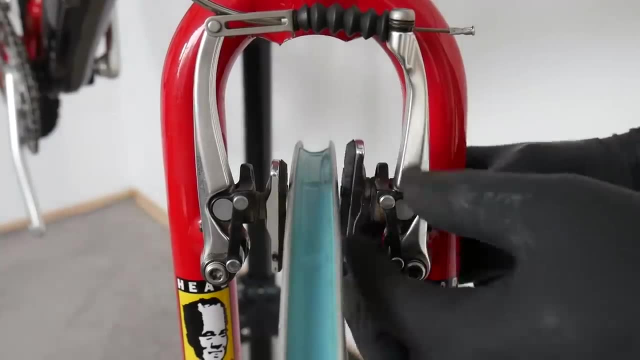 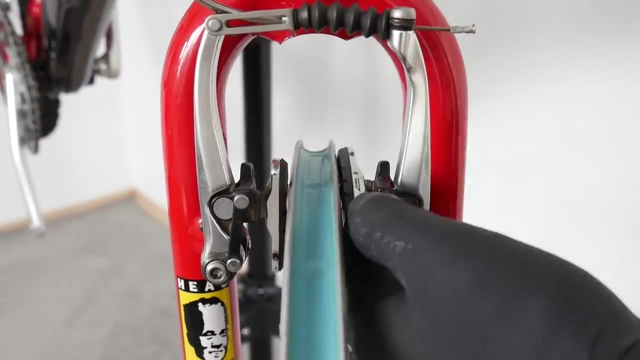 don't have problems with the squeaking noise, And the compound on those pads is being wear down very evenly. This is how I do it. Operating with these pads. having just two hands isn't that easy, because we want to hold to the braking pad with one hand. The other one we're gonna use for 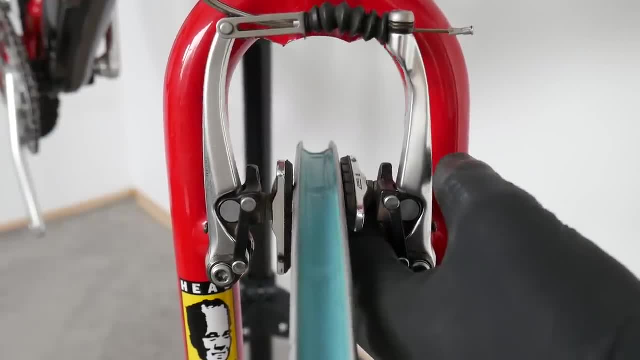 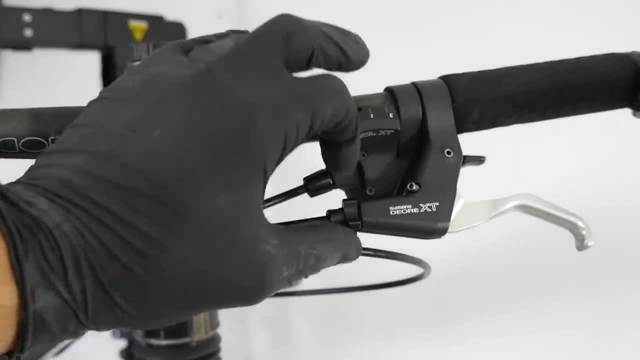 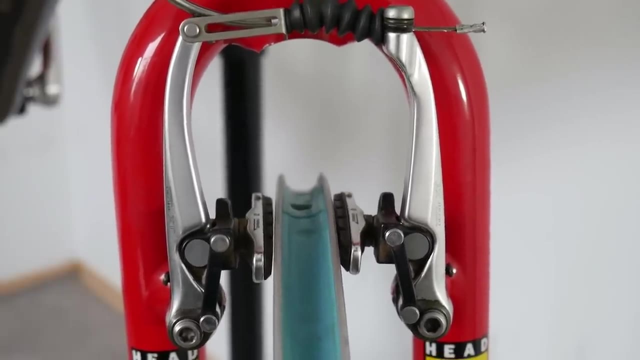 fastening. and also the third one would be really helpful for braking. So this is what I do: Instead of using one of my hands for braking, I'm simply using the barrel adjuster. So now my braking pads will just brake and it will be extremely easy to align. 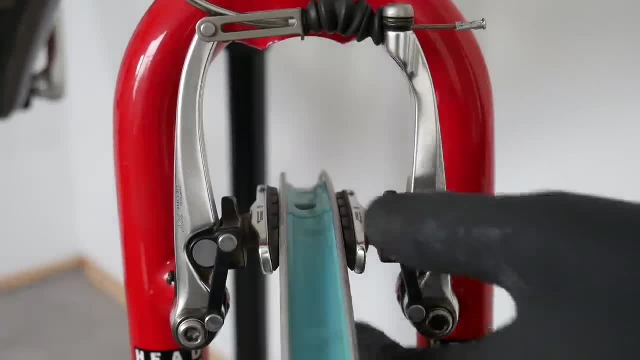 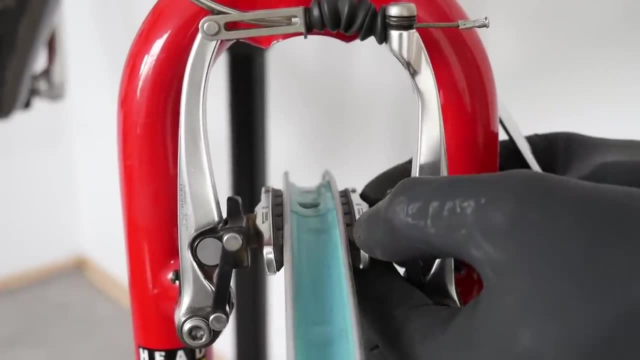 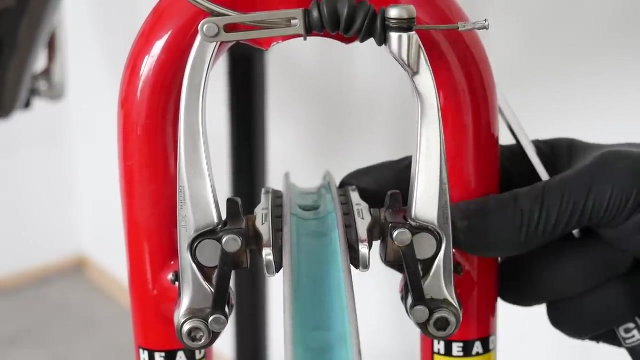 those and fasten the bolts. Now I have my both hands available, so I'm focusing now on aligning the braking pads, So not too high, not too low, the right angle and hundred percent parallel to the rim. This is going to be very good. 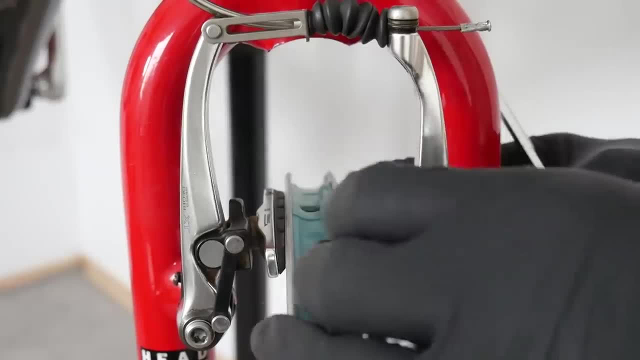 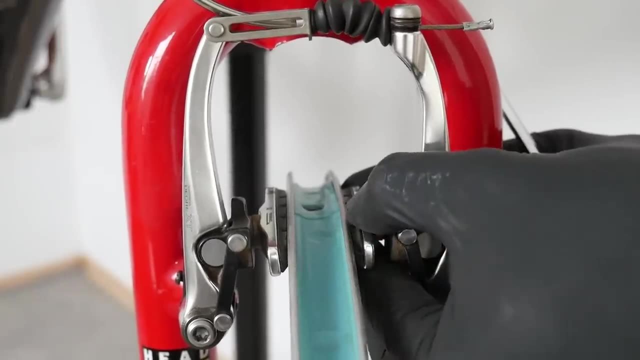 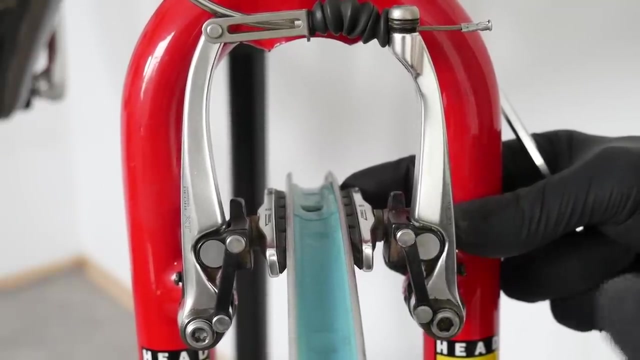 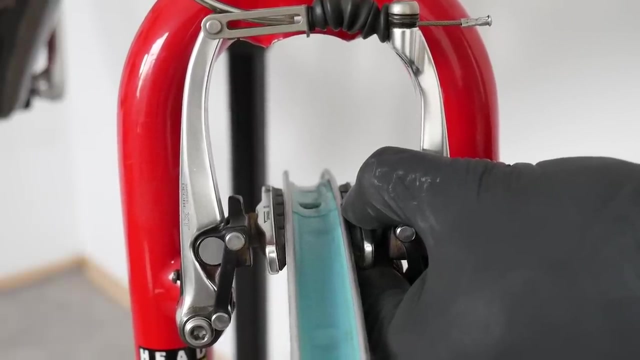 When you have your tire on the rim, that's even better, because then you will see whether it touches or will wrap against the tire or not. But this should be just fine. The braking pad is exactly in the middle of the braking surface on the rim, And so now I can fasten the bolt holding to my braking pad and the job. 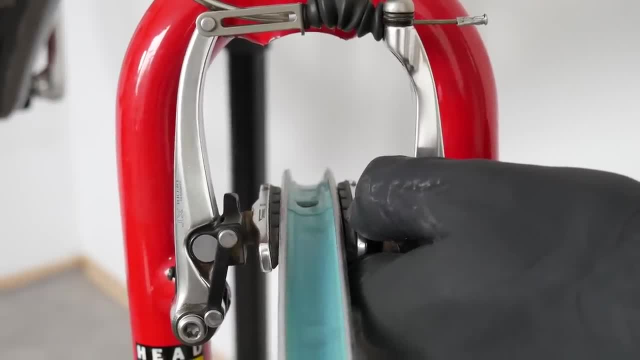 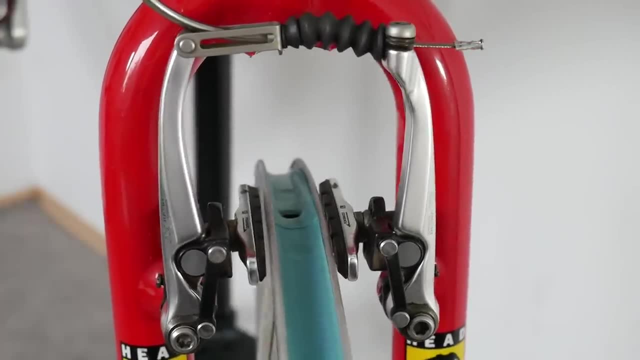 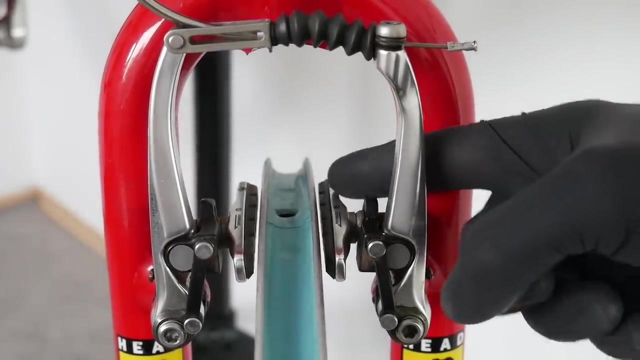 will be done once. I do it On both sides. After threading the barrel adjuster back to its position and releasing the cable, we can see how the brake is working. This is nearly perfect. You can see that these braking pads weren't being used evenly on this side and this side, and also here back. 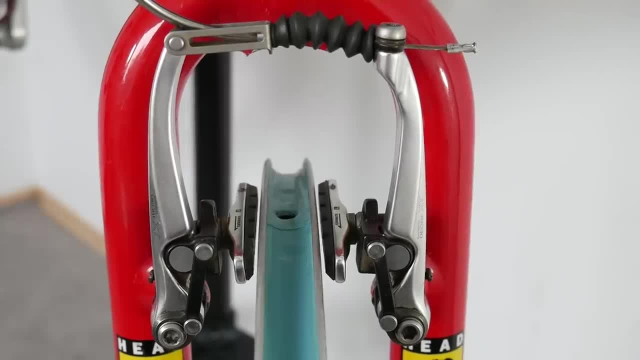 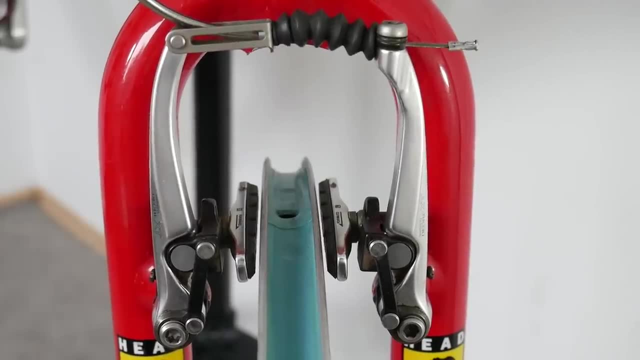 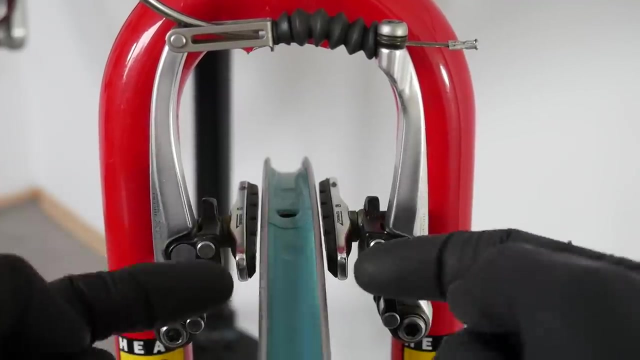 at the back and the front. That's because that system of alignment- In my opinion the parallel alignment- is just better and it works perfect. There will be no squeaking noises. If you've noticed that these V brakes have the parallel system, that makes those, those braking pads, work and move just parallel to the rim, Don't? 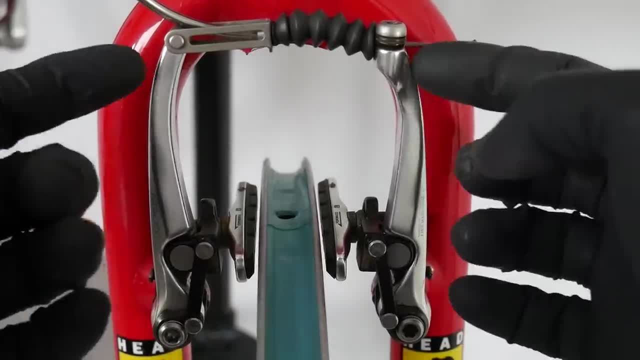 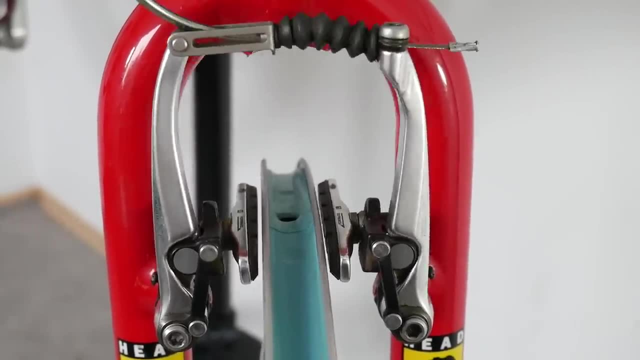 worry, you're gonna be aligning, adjusting your brakes on the standard normal V brakes just in the same manner. So this is almost perfect. Adjusting the caliper brakes on the road bike isn't that much different from what we've done with the. 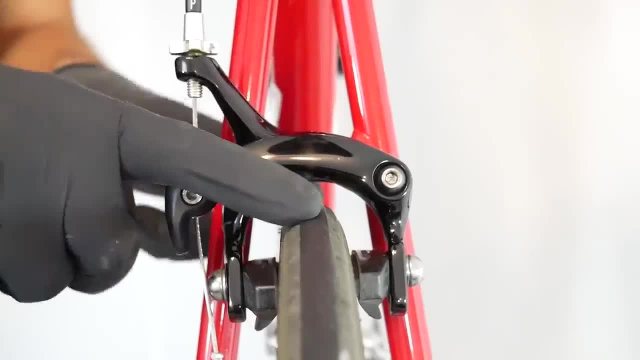 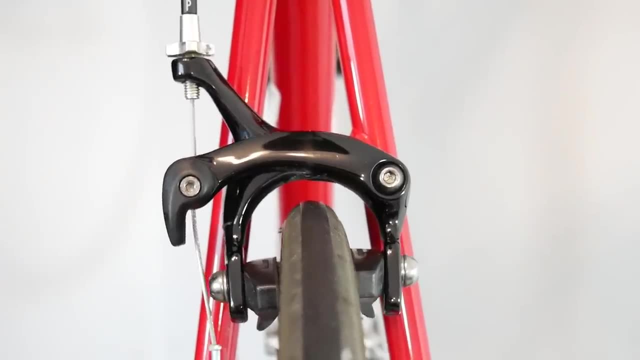 V brakes. In this case, we also want to adjust the caliper brakes on the road bike. In this case, we also want to have our wheel being centrally located between those two braking pads. As you can see, on this bike, one of these pads is already touching the rim and the 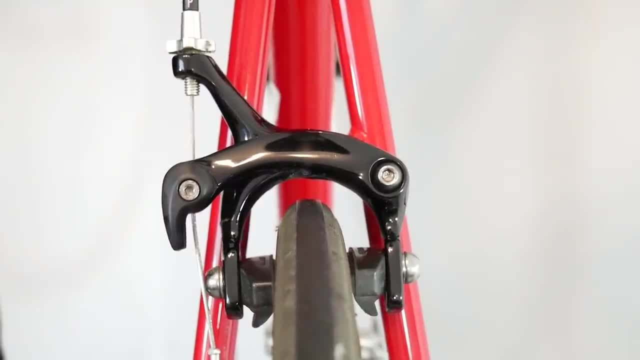 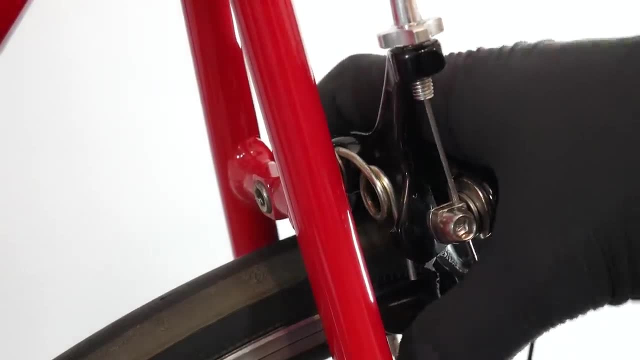 other one has still three or four millimeters of a distance. That means we have to readjust the position of a whole caliper brake. In order to readjust the position of the whole caliper against the wheel, we need to unthread this bolt. 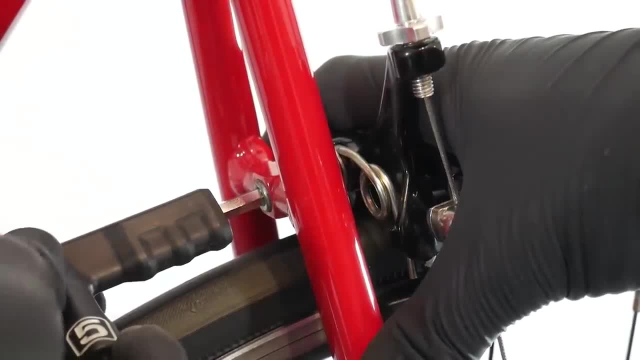 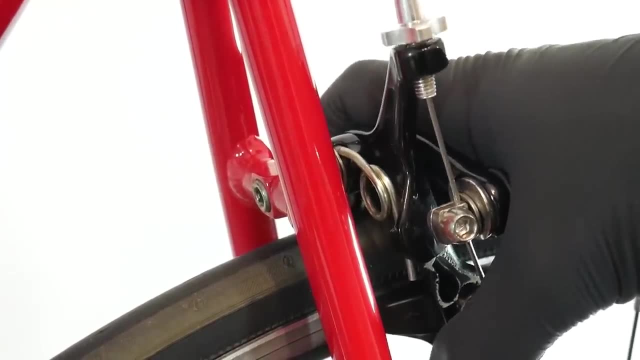 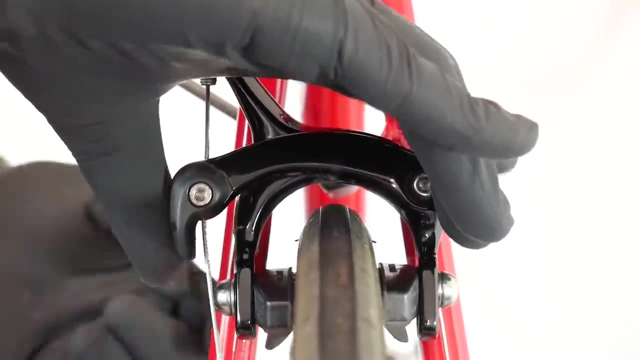 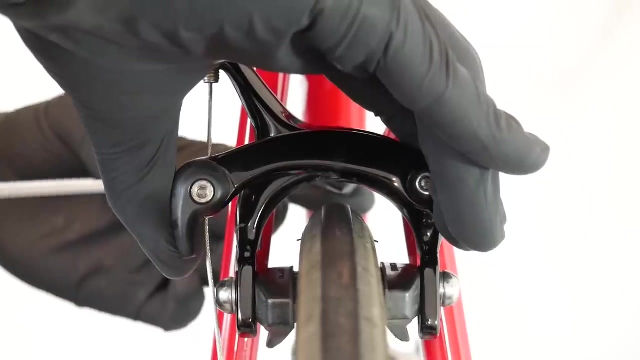 which is fastening our brake to the wheel. Now I can feel we can proceed to the readjustment. Now we can move the caliper brake, finding the perfect position of our braking pads against the the rim on both sides, and once it's centered, I'm fastening the bolt here After fastening. 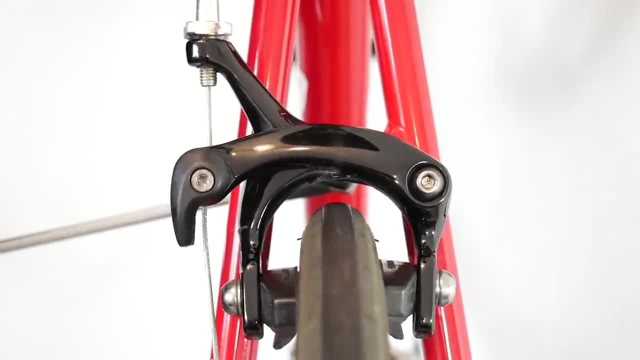 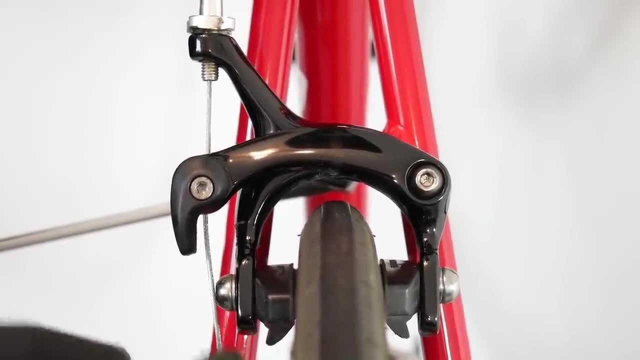 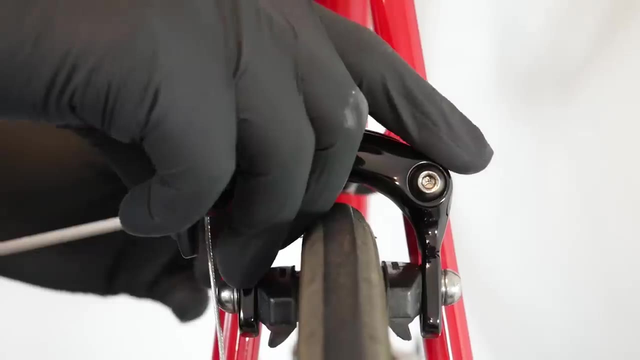 just a little bit. I'm gonna check whether the braking pads are working perfectly. Yeah, this is exactly same distance on both sides between the braking pads and the rim on the left and the right side. so now I can fasten it, holding to my caliper brake, making sure it will not move. Now it's working. 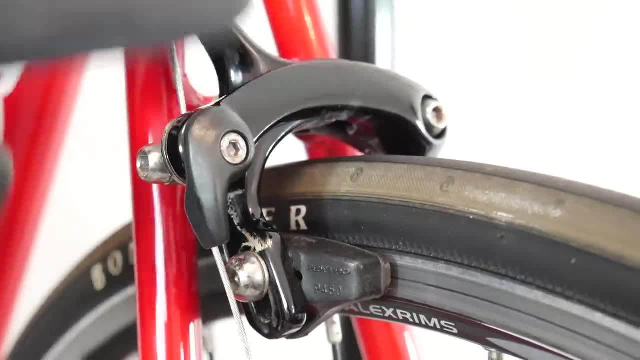 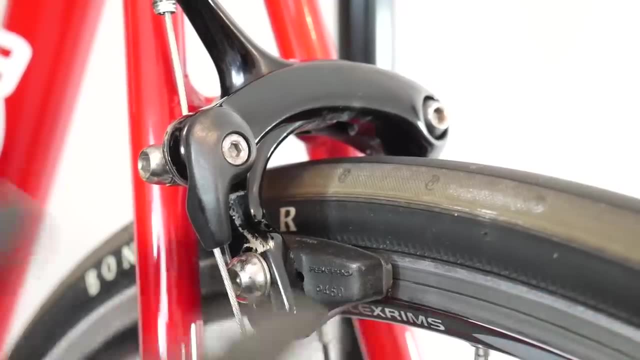 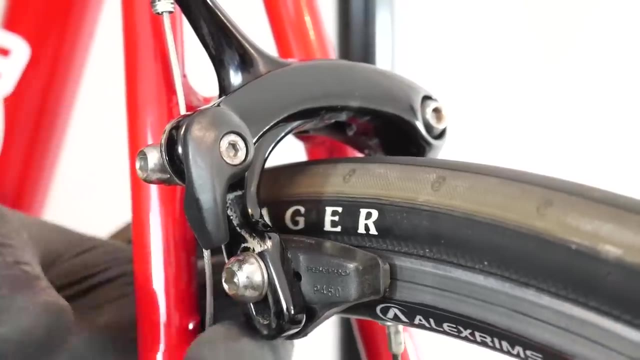 perfectly. Our caliper brake is now set correctly and fastened so that we can proceed with the adjustment on our braking pads. In order to do that, we need to find the bolt which is fastening the braking pad to the caliper brake. that's the one here. 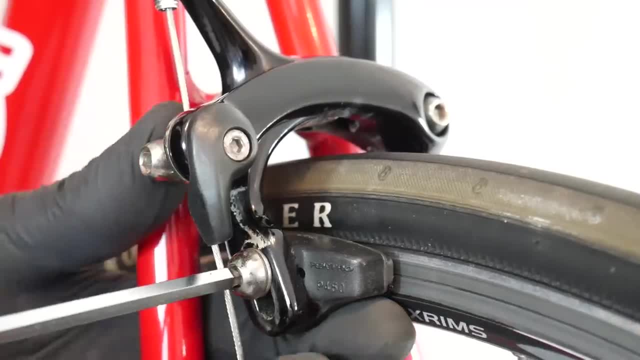 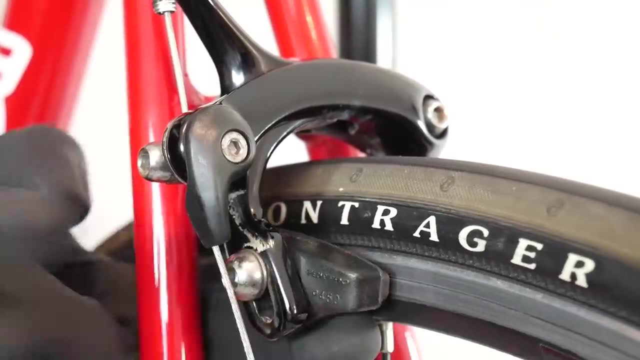 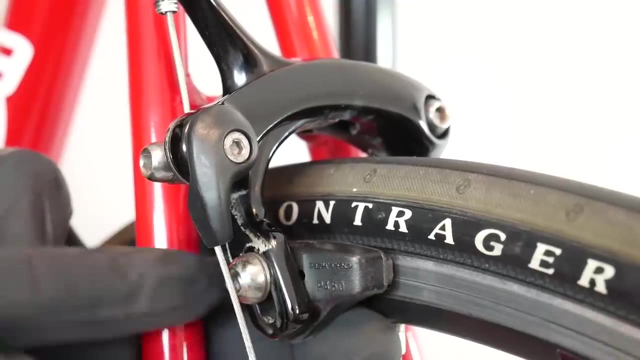 it looks exactly the same as on the V brakes. after releasing it, I can now move the braking pad around once more. some bike mechanics would like to set larger distance between the braking pad and the rim at the back of the pad, comparing to the front. I don't do it. I would always set the braking pad exactly parallel to. 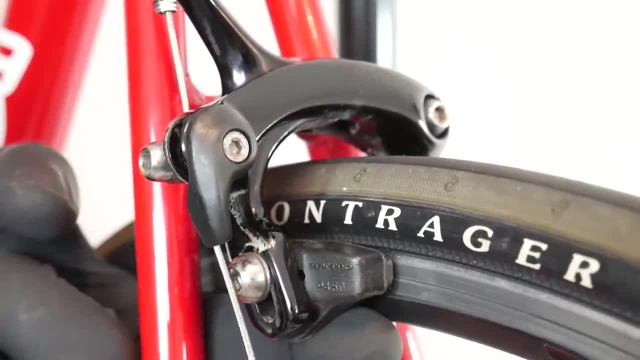 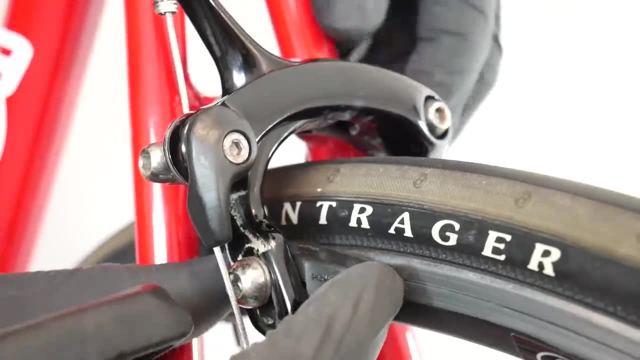 the rim, and that seems to work very good for me. on all the brakes I've been using so far- and there have been many- in order to set the right position of the braking pad, you can use one hand in order to squeeze the whole brake. and now 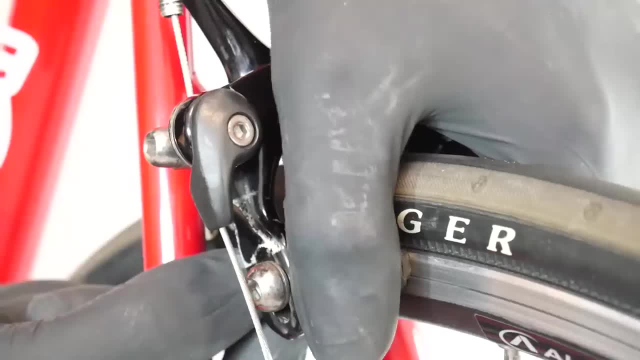 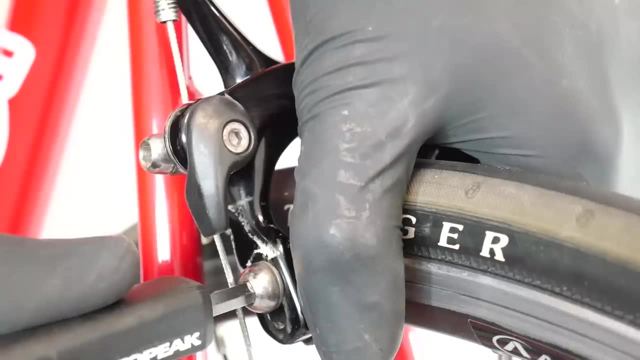 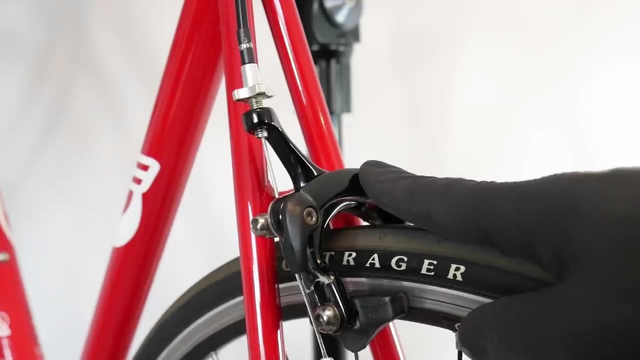 you can just move this braking pad around and after you find the right position, you just fasten the bolt. but there is another way to do it easily. I will show you an easier one which I'm using almost always. just as I did that with the V brakes, I'm using the barrel adjuster to make my both braking pads. 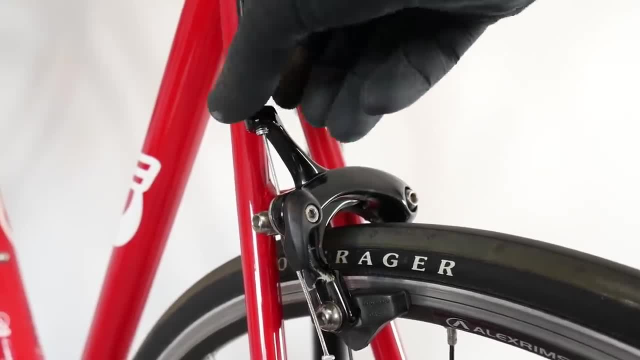 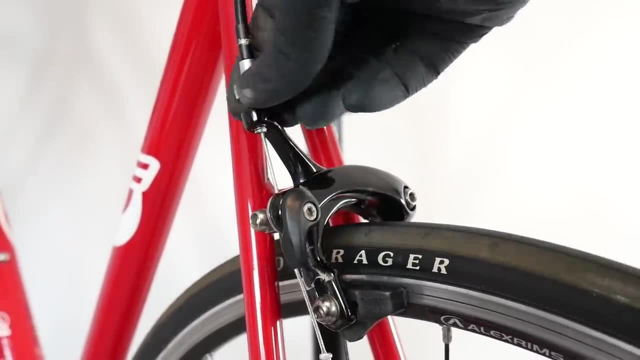 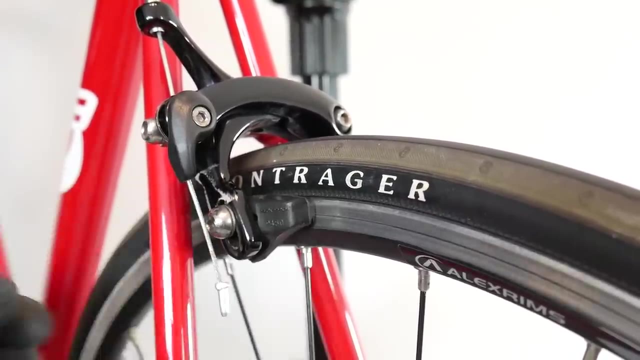 touch the rim, just as it would be during the braking, and then setting the position of those braking pads will be very easy. after I'm threading my barrel adjuster, I can see both of my braking pads touching the rim, which makes the whole adjustment so much easier. 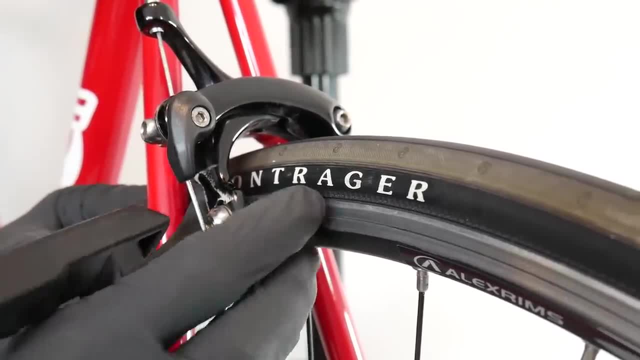 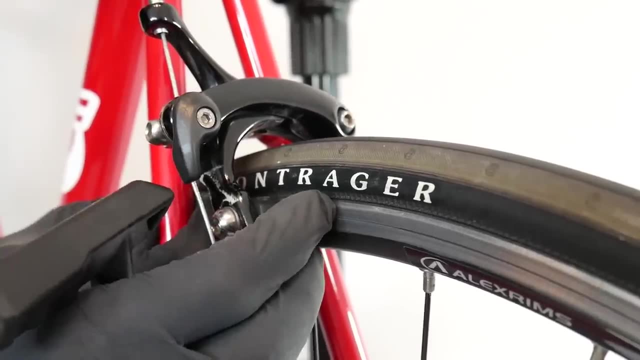 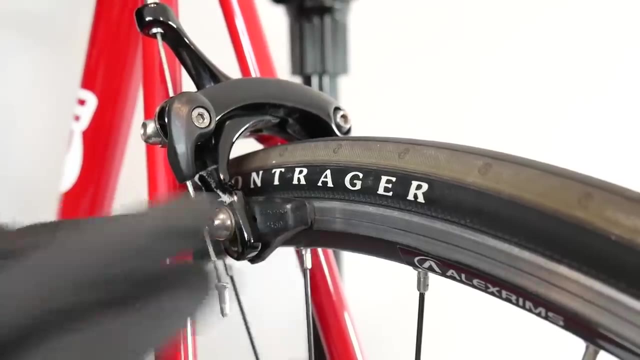 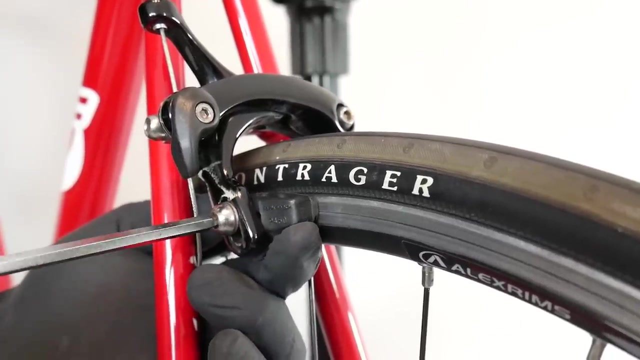 Now, I don't want my braking pad to be too low or too high- it should not rub against the tire, obviously- and I want to see the whole surface of the braking pad touching the braking surface of the rim. this position seems to be perfect and now, holding to my braking pad with one hand, I will gently and slowly fasten. 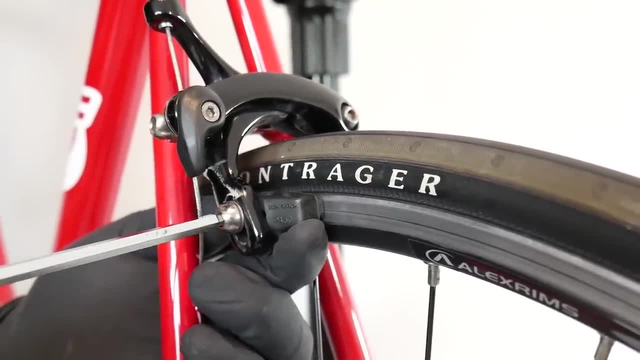 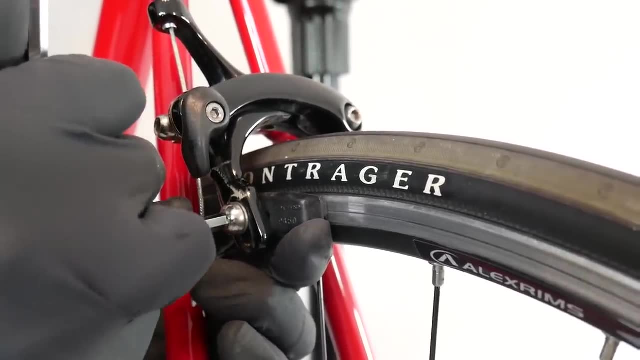 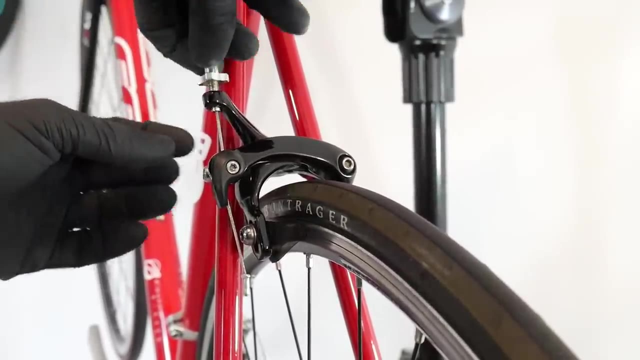 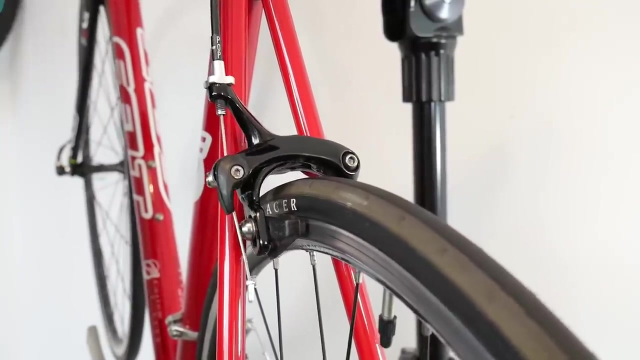 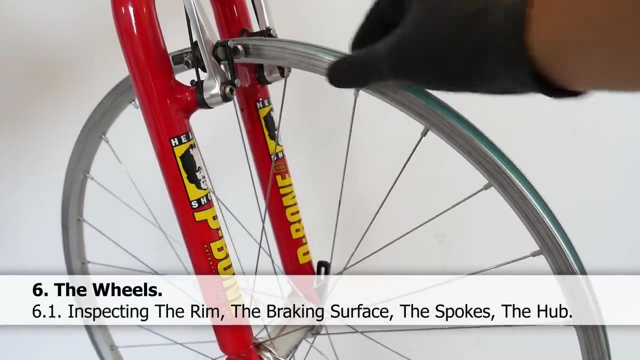 the this bolt, Making sure that the braking pad is not moving while I'm threading it in. after adjusting the braking pads on both sides, I will now thread the barrel adjuster back in, releasing the cable. now the brakes are ready for some high speed. During the wheel inspection, we want to take a closer look at the rim. meaning is: 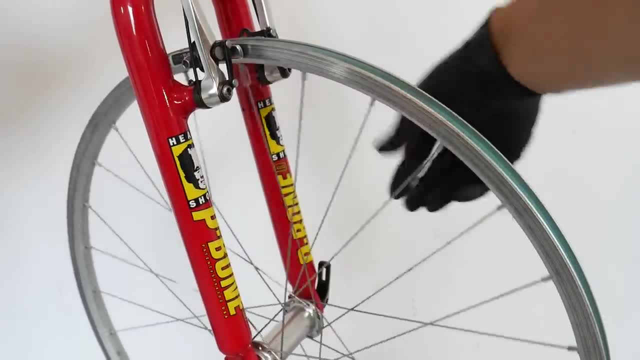 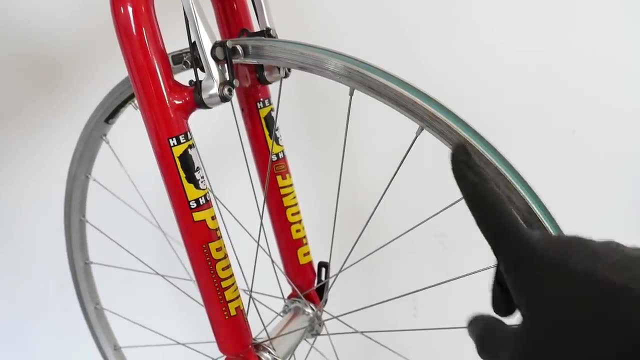 the rim. true, What is the tension of different spokes? Is it very even, or some spokes are pretty loose and other very tight? How does the braking surface look like if we don't have the disc brakes? And finally, what's the condition of the bearings in the hub? 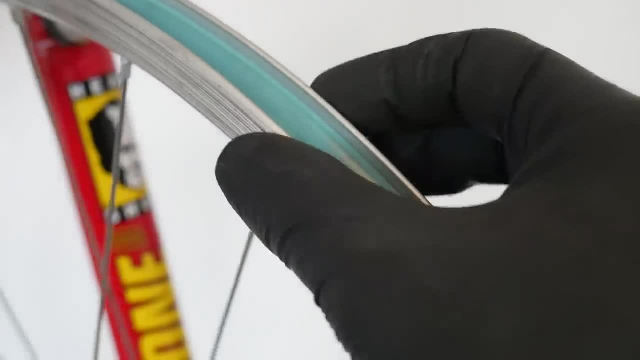 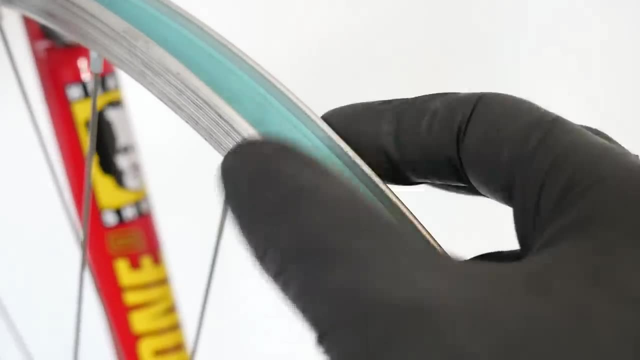 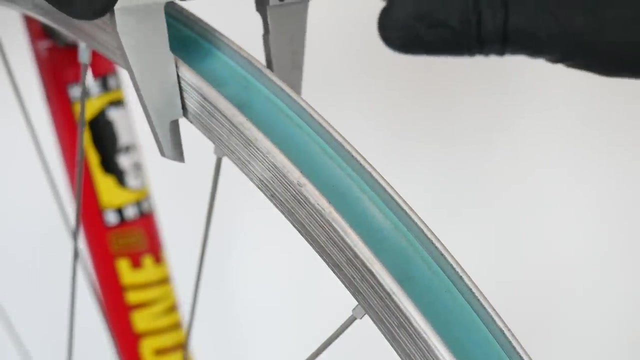 Let's look into the details now. Let's start with the braking surface. we can try to feel under our fingers. how does the braking surface look like? Is it being wear down evenly on both sides, and also whether it doesn't have some larger holes? I do like to use the caliper for this reason. I'm not measuring anything. 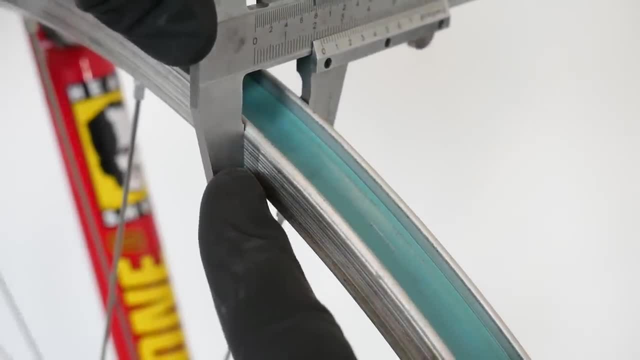 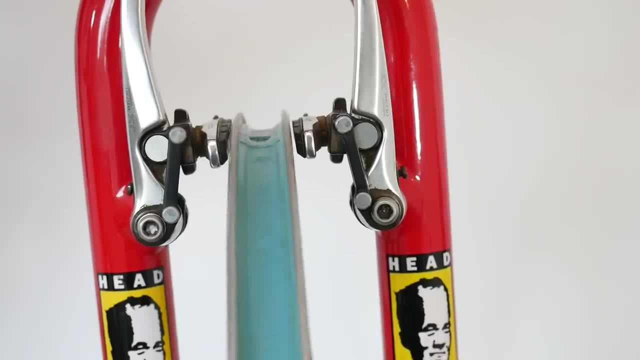 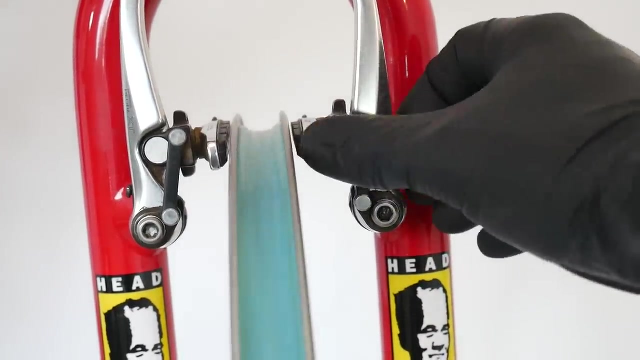 anything here and now I can see that the surface of my rim is very even straight. so this rim is in very good condition. let's see now whether the wheel is true. having caliper brakes or v brakes is very helpful here, because we have here the reference point. but if you have the 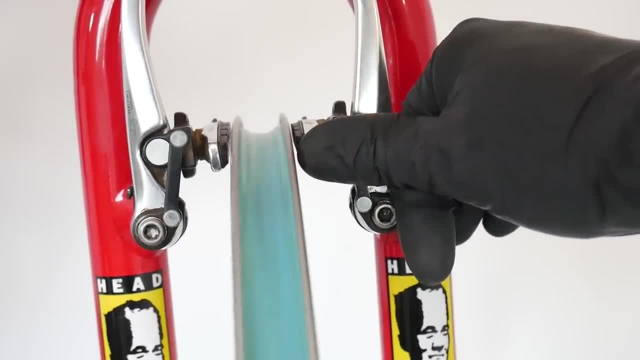 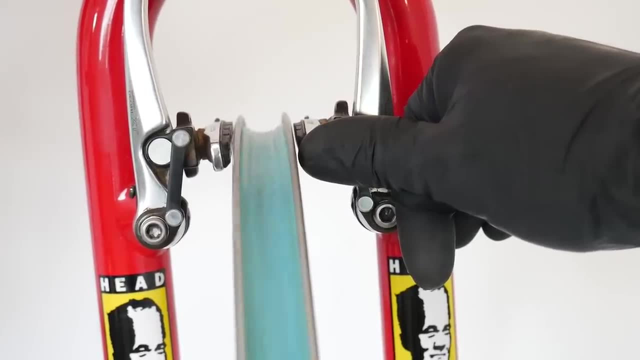 disc brakes. you can just use your palm And a thumb, just like this. as you can see, this wheel is in pretty good shape. there is just a slight movement from side to side, maybe about one millimeter or so. we can, we can try to true this. 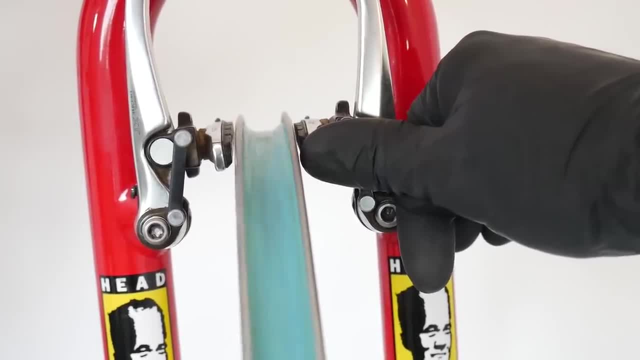 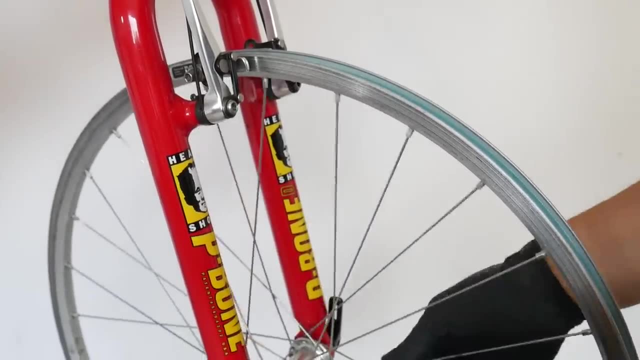 wheel, but this one is still in very good shape, and we also want to look at the up and down movement of the rim. after spinning the wheel and looking at the rim, we also want to check the tension of these spokes. of course, doing it by hand doesn't give you a good feeling, but it's still a good. 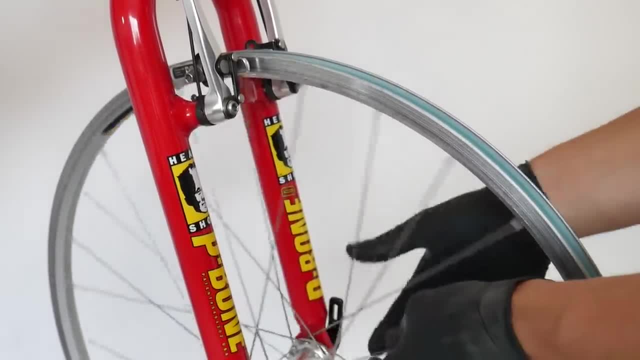 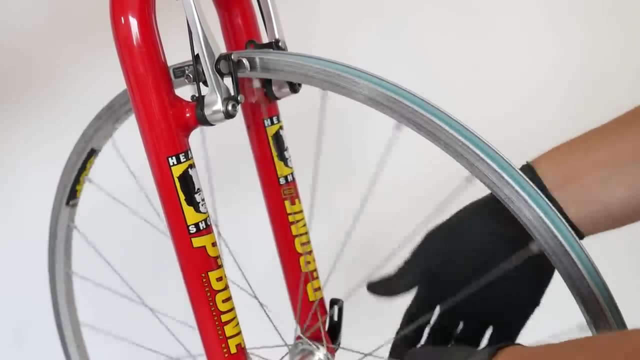 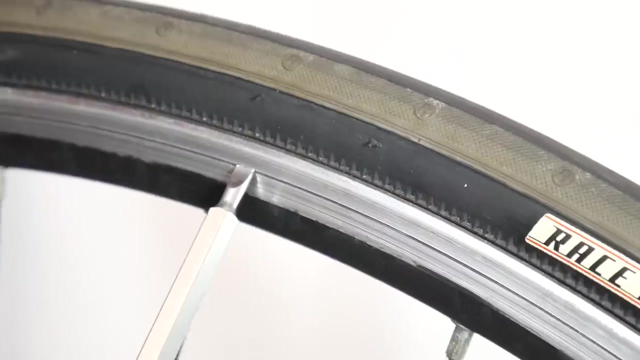 feeling to do very, very exact measurement. but if you don't feel any very tight spokes and very loose spokes, that's good for the wheel. this one is very good. this is the example of a rim with a special wear indicator. this groove, which goes around a whole rim, will show us how much of the 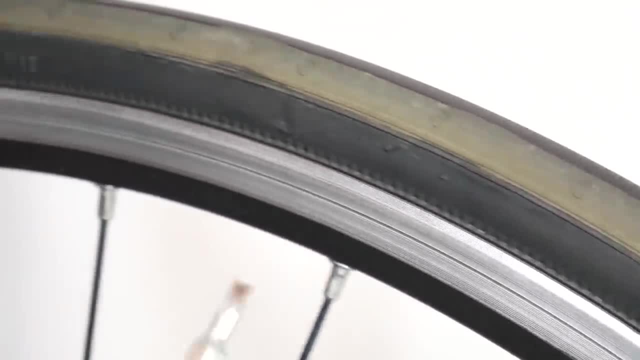 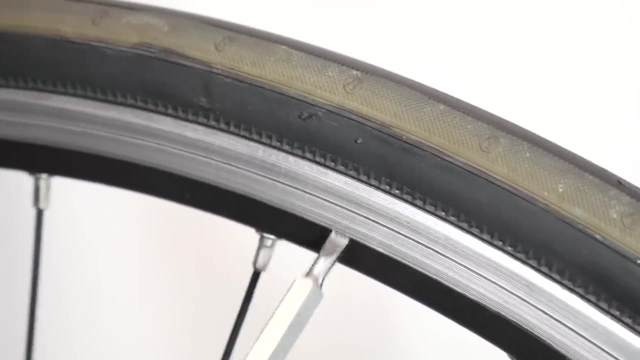 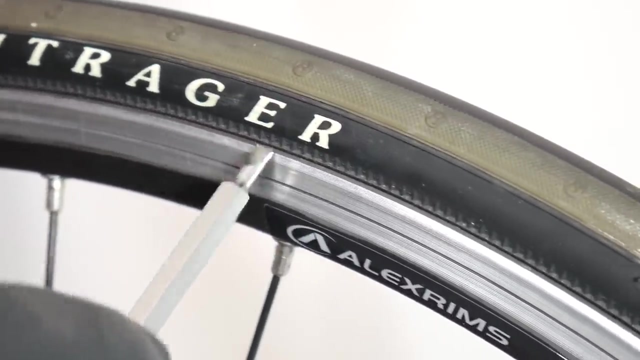 braking surface. we've already taken off with our braking pads by braking. this one is still pretty deep. it shows that this wheel, this rim, doesn't have many miles on it. we need to replace the the rim once this indicator will disappear completely. now we can check out the bearings. 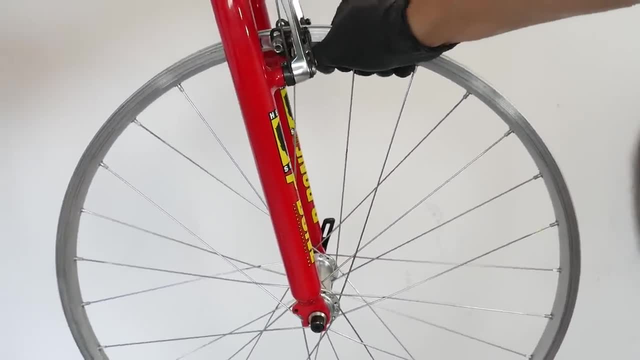 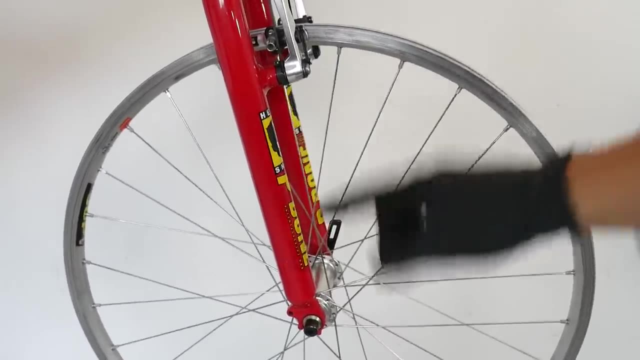 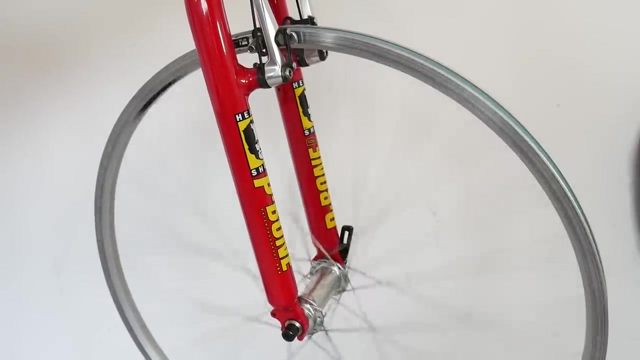 first off, we want to hold the bike and rock the wheel from side to side, searching for any movement. there is no movement here, so there is no play on the bearings. then we of course spin the wheel and we'll see how, how long it will spin. this one spins pretty long, so the bearings are clean at least. and also we want to listen for any 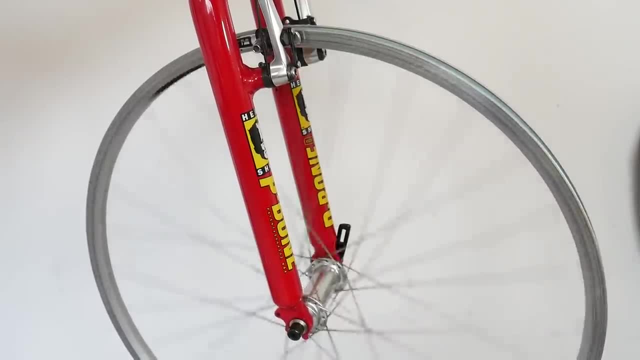 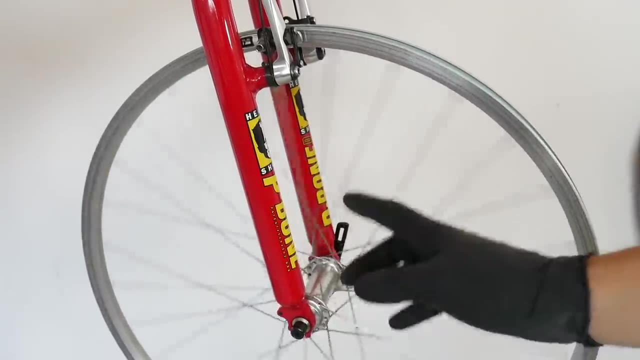 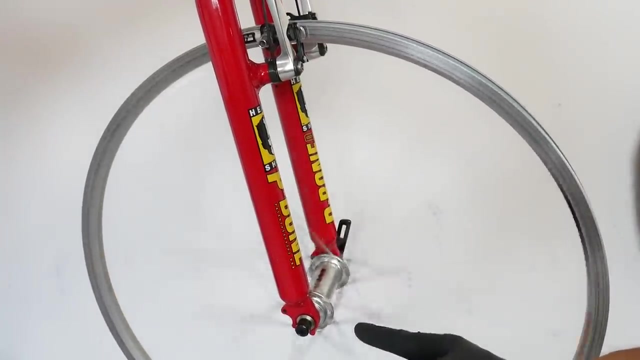 type of of noise coming from the bearings. it can be noise that comes from the dirt being in between the balls in the bearings, or if the bearing is clean but dry, you will also hear some noise. this one here: no noise. so very good condition of the bearings. now how to remove the wheel from our bike. 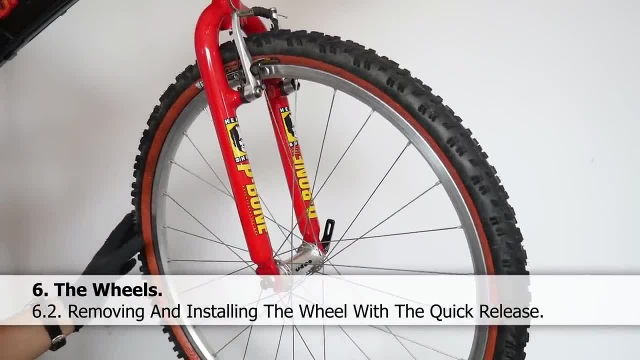 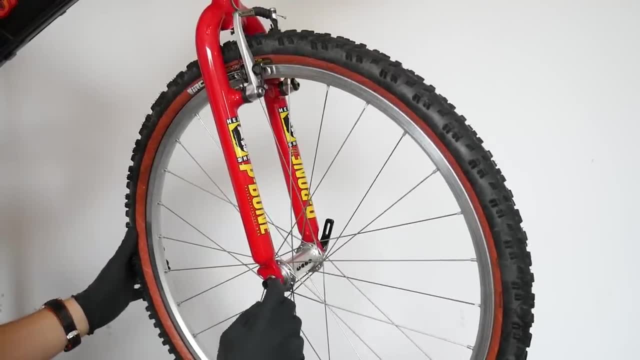 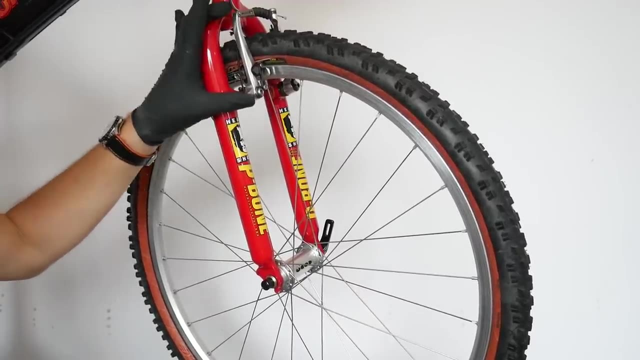 from the fork or from the frame. first off, we need to consider what type of brakes we have. if we have a disc brakes, it's no problem. we can start by simply unthreading the bolts at the axle or just opening the quick release. but if we have v brakes or any other type of caliper brakes which are braking on the rim, 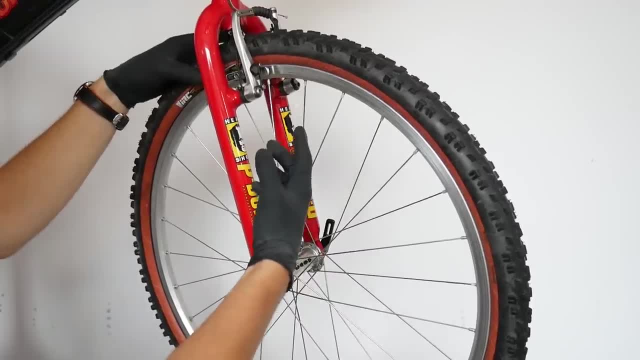 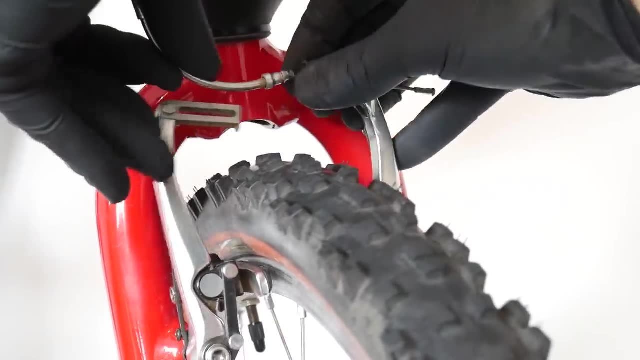 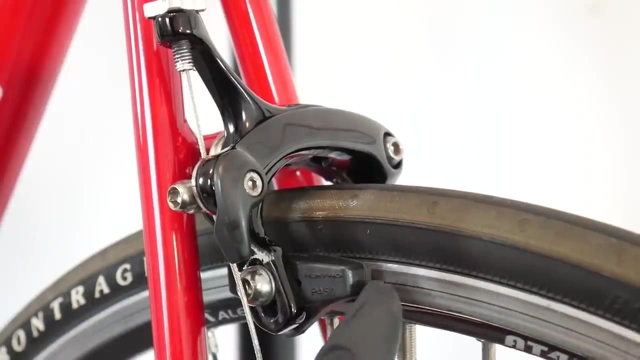 that means we need to open those so that the tire will be free to be removed. in order to remove the wheel from a road bike, we also need to open up the space between the braking pads and the rim. on most of the road bikes, caliper brakes- we have some kind of a lever. 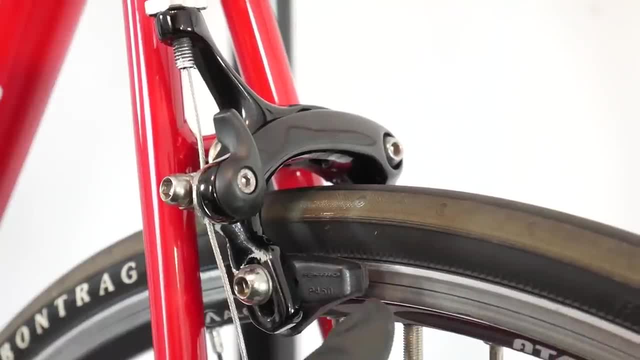 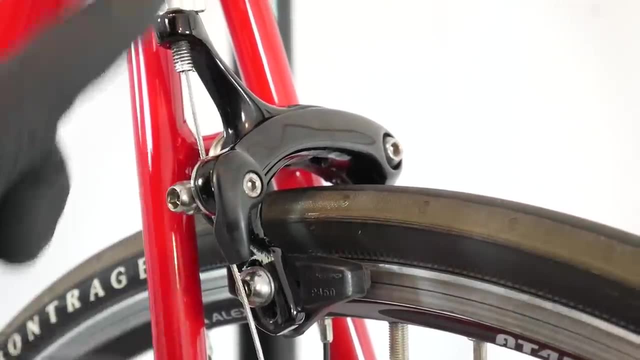 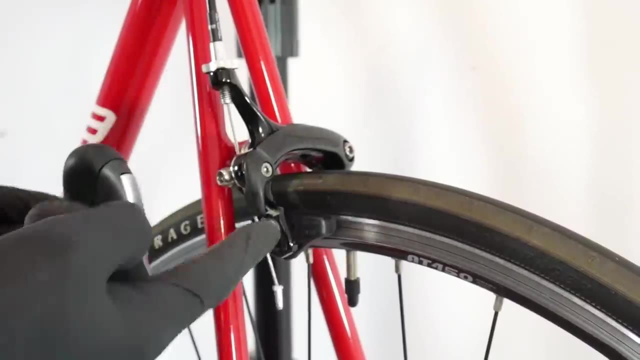 this is the open position. now the space is larger, larger and the tire will go through, and now it's in the locked or closed position. remember to close the brake after putting the wheel back on the bike on the campagnolo systems. we won't find such a lever on the caliper brakes, but we will find a. 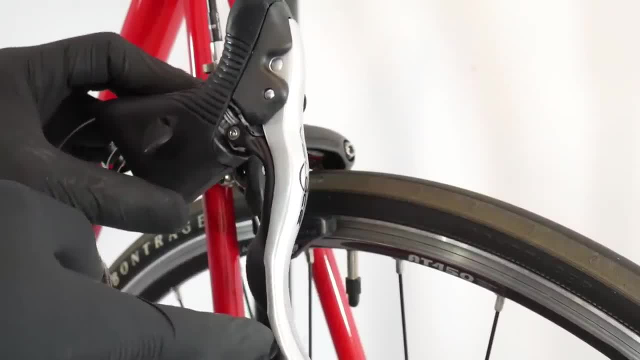 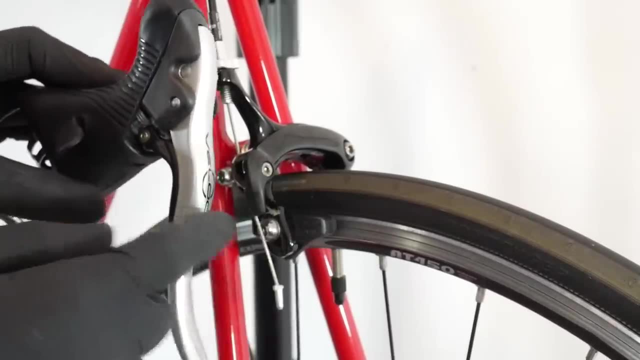 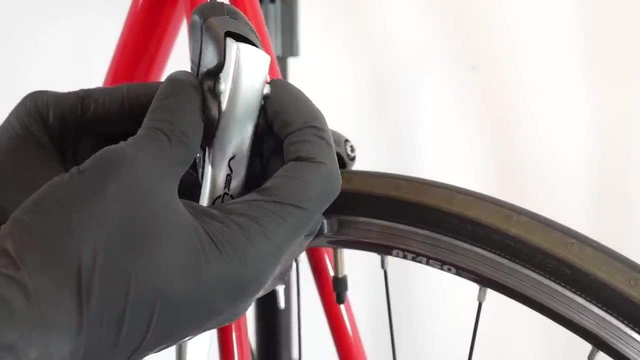 special pin on the shifter. i'm pressing this one in and now you will see that the braking lever will release more cable. that means the distance between the braking pads and the rim will be larger and will remove the wheel after putting the wheel back on the bike. we are pushing this one back to its 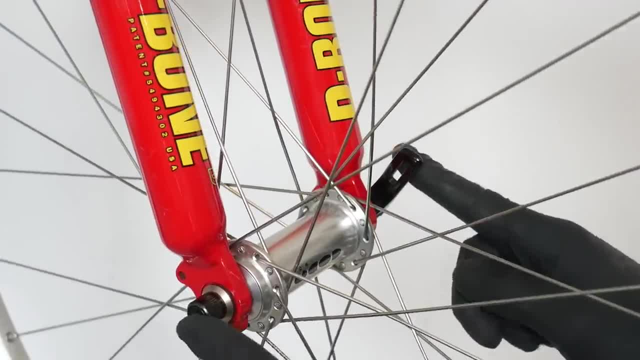 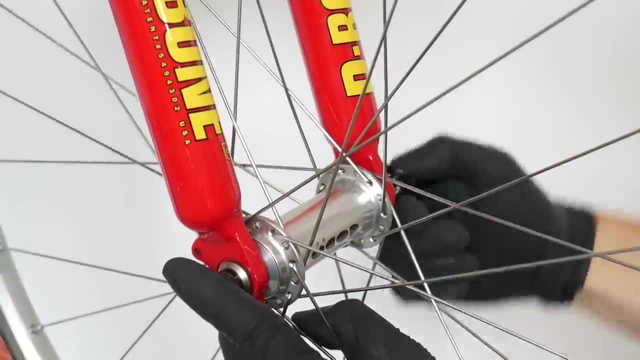 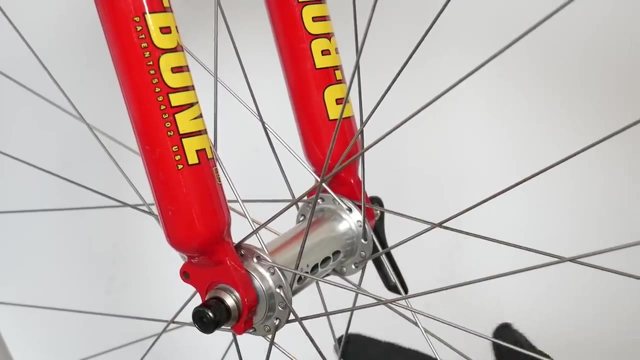 position. now we can remove the wheel in case of having quick release. on one side we'll have a small lever, on the other side a nut. by opening the lever we are loosening the wheel. on some bikes, on some folks, we will be already able to remove the wheel, especially in the front, as you can see. here we have additional. 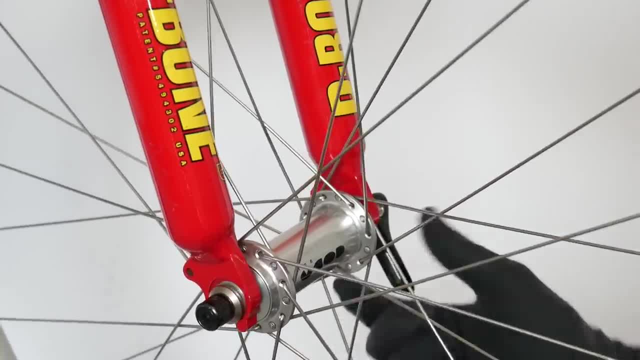 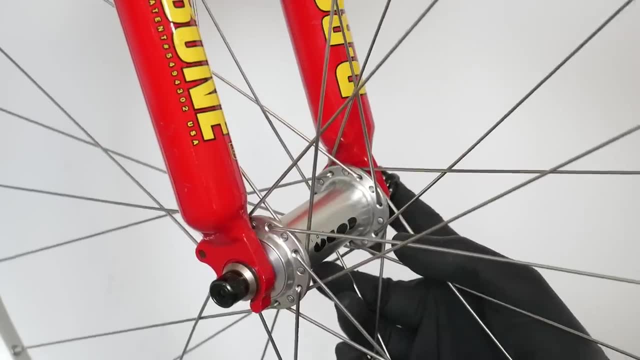 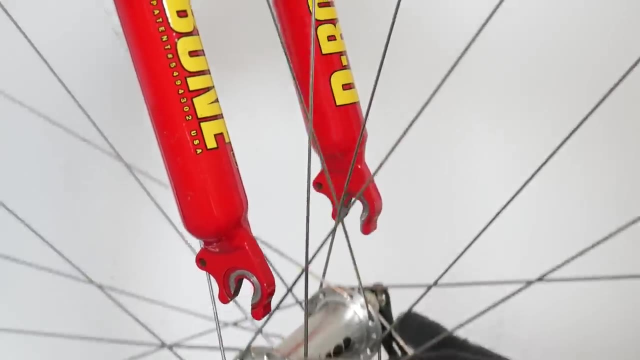 protection. there is some groove so that we don't lose the wheel. if the quick release is opened so that we need to use the the nut in order to remove the wheel, maybe one or two turns and and a half and then the wheel is removed. putting the wheel back on our machine means doing all the things in the opposite. 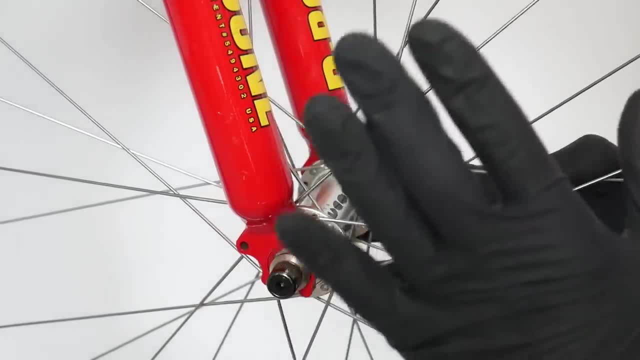 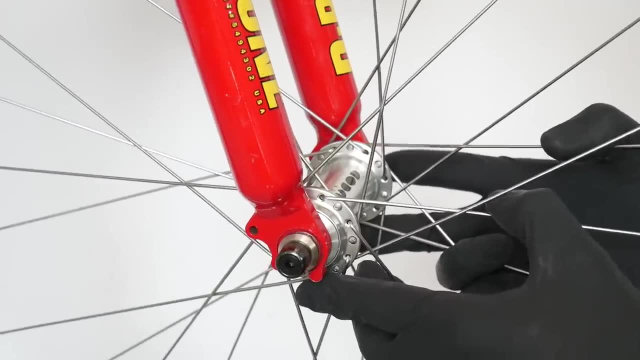 order, with one difference. I would recommend to have the bike put on the floor so that the weight of the bike will stay on the floor and it will not damage the bike during this process. center our wheel in the fork and in the rear in our frame. Now we are using the nut here in order. 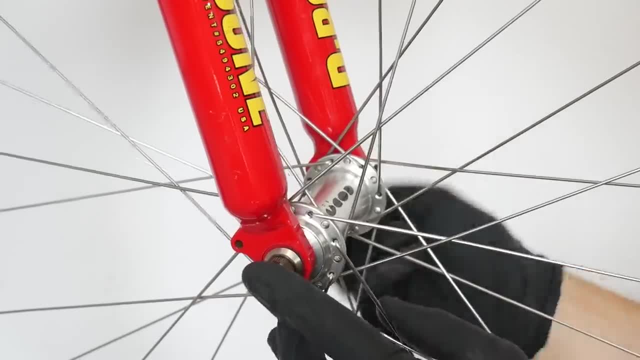 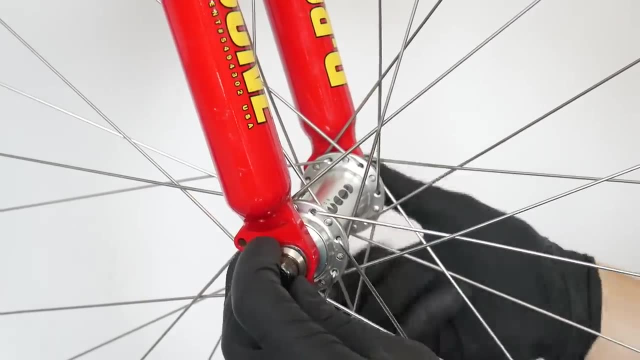 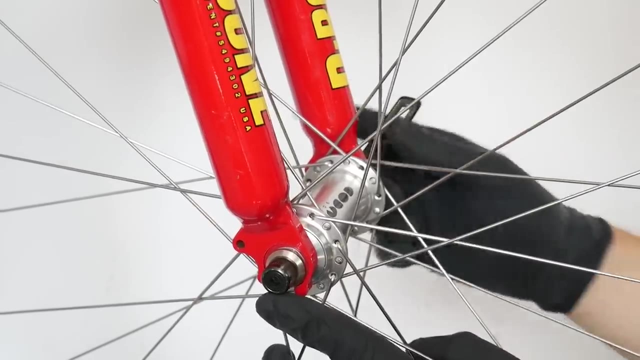 to find the right resistance for our lever, How strong, how much force we need to use in order to lock the wheel securely and tightly. The rule of thumb is that we should start to feel resistance on the lever at about 90 degrees before it's locked. So this is the final position. Now I'm 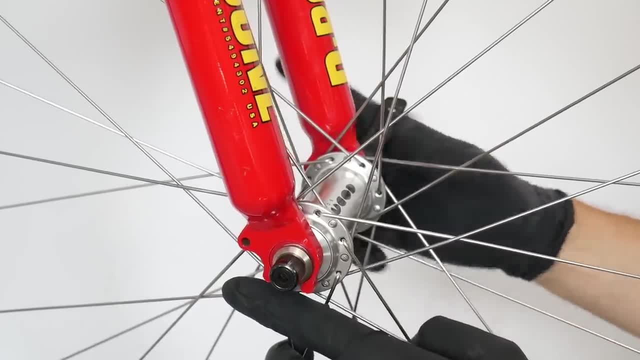 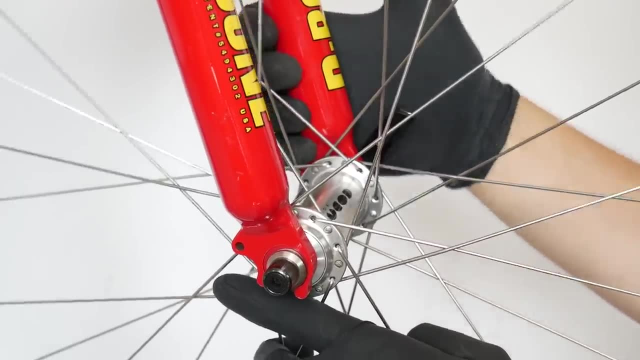 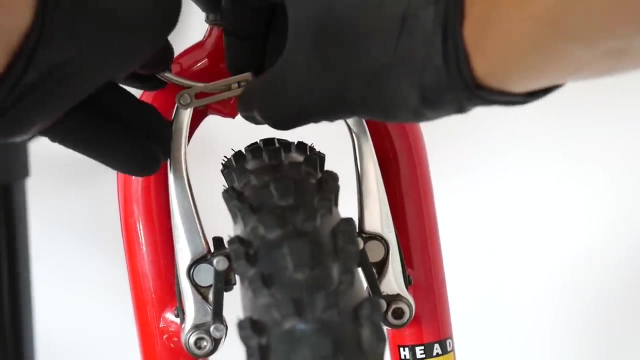 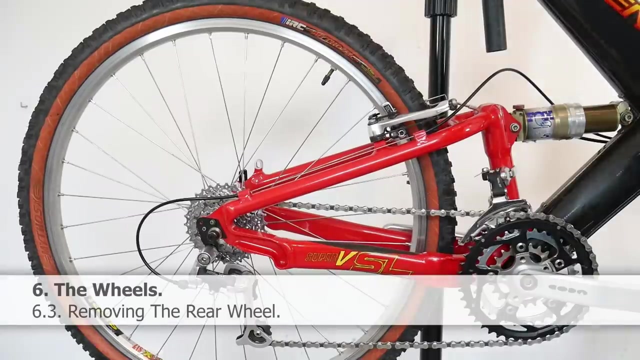 starting to feel the resistance somewhere here, which is pretty good, and now I'm locking it. I feel some resistance when locking it, so I'm sure it's secured In order to remove the rear wheel from the bike after releasing the rear brake. we also want to 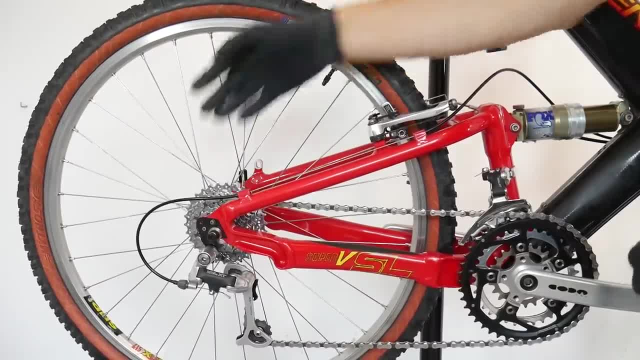 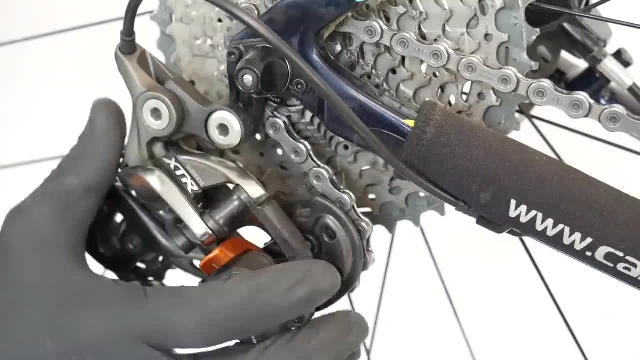 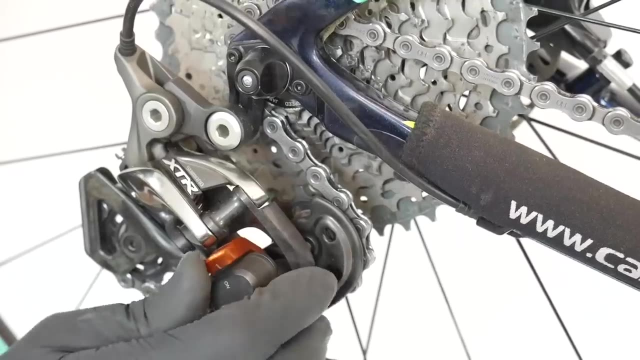 shift the chain to the smallest sprockets, both in the rear and in the front, so that there will be no tension on the chain. If you've got on your bike one of these modern Shimano Durellas with a special clutch, remember to switch this lever from on to off position. that will help you to lock the chain. Now we are going to remove the rear wheel from the bike After releasing the rear brake. we also want to shift the chain to the smallest sprockets, both in the front, so that there will be no tension on the chain If you've got on your bike one of these modern Shimano Durellas. 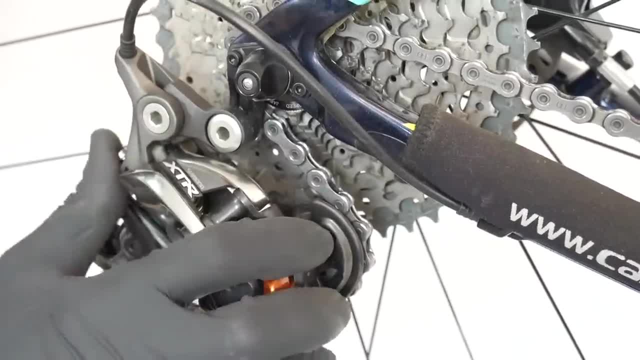 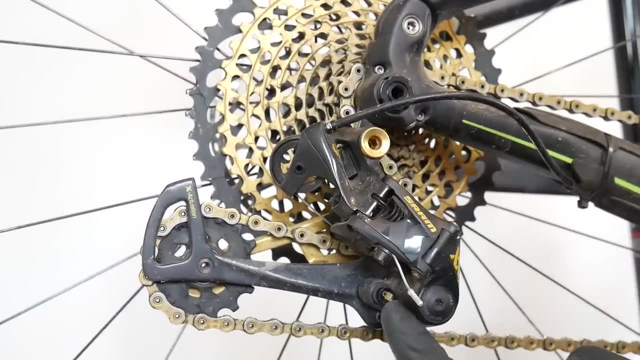 will help you to lock the chain. If you've got on your bike one of these modern Shimano Durellas, make removing the wheel much more simple. after putting the wheel back on your bike, switching back to the on mode, These Ramry Durellas will have yet another system. There is a button. 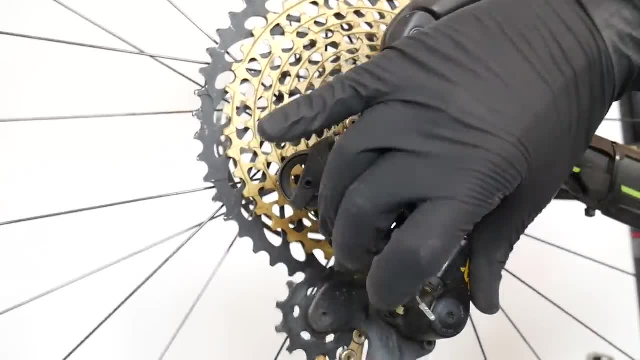 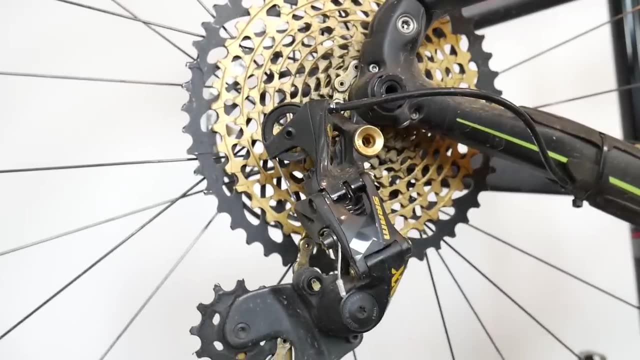 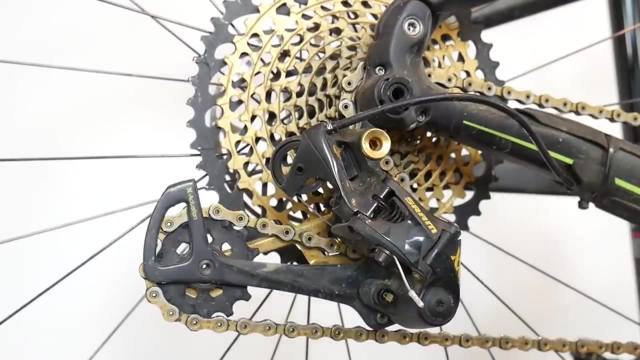 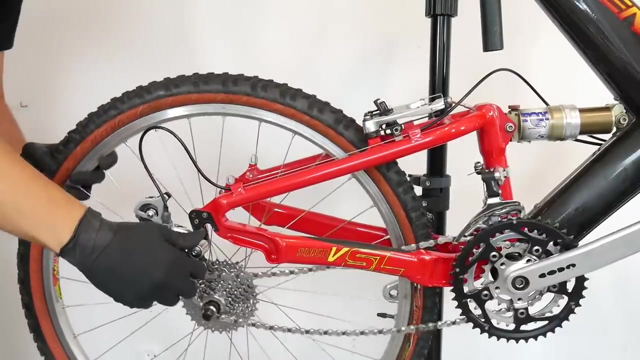 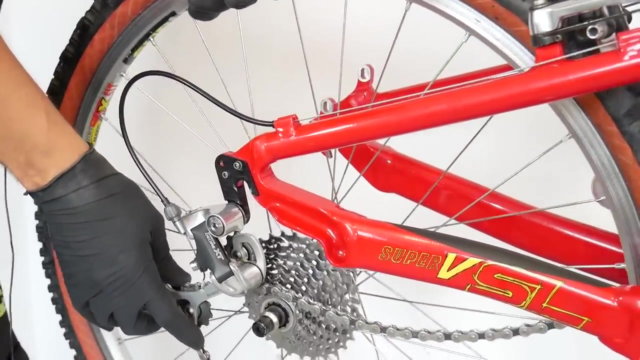 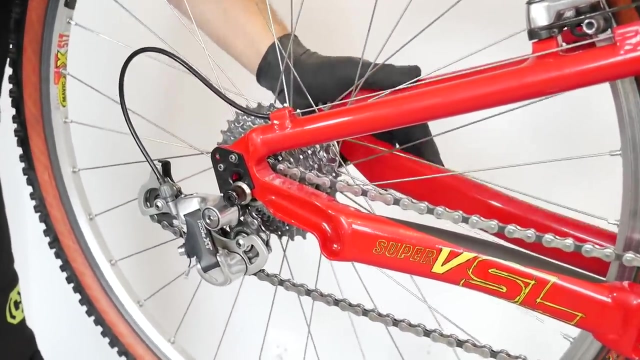 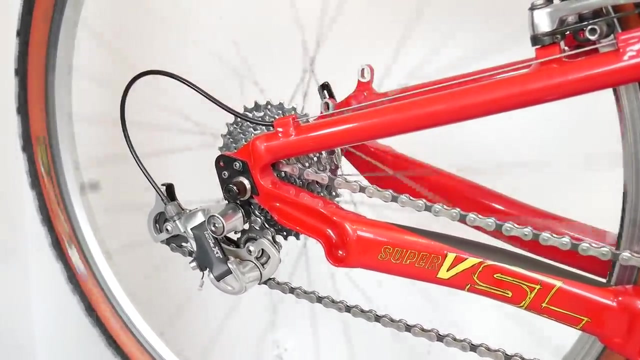 here I will first open up my derailleur, then push the button and lock my cage like this: Now I can remove the wheel from the bike, put it back and then unlock it and it's ready to go. go. And now we're going to remove and assemble the wheel with two main types of the thru-axles. 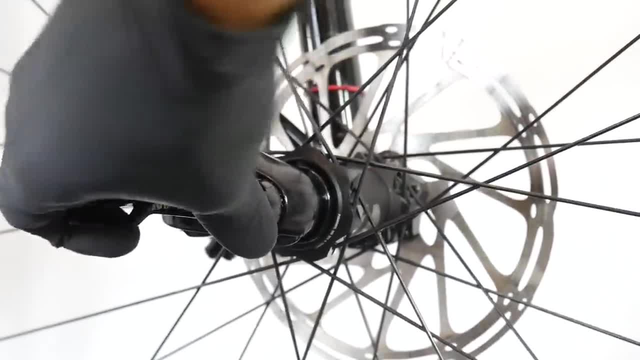 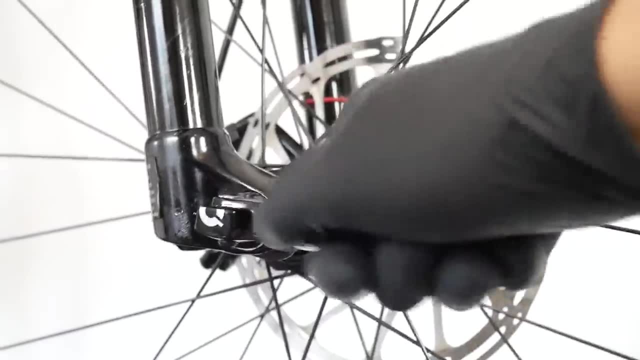 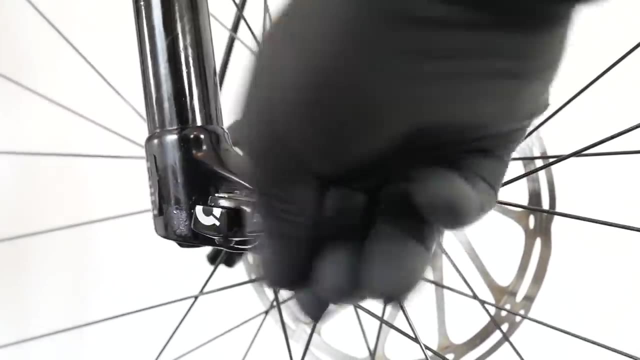 This is the thru-axle with the lever that we need to open, and now we can unthread the whole axle. Now, some thru-axles will also have a special groove somewhere here, and in order to unthread the axle, we need to fit the lever into the groove in the open position. 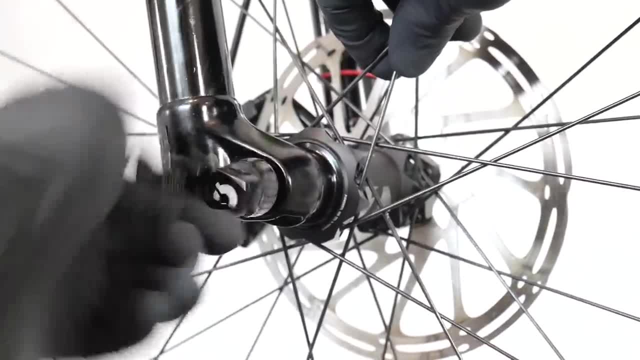 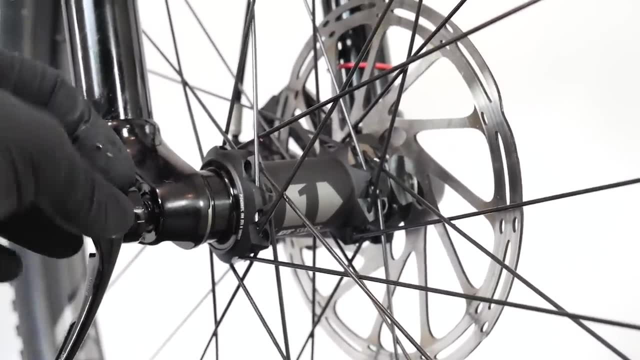 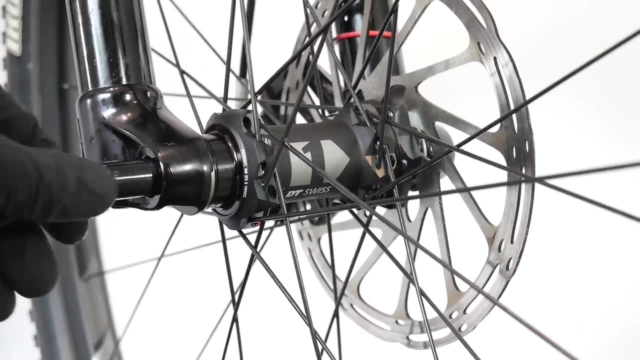 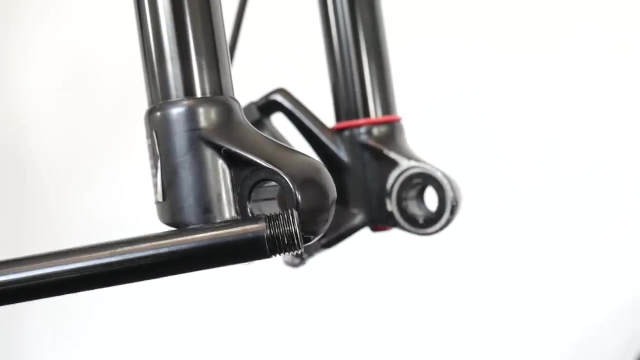 Now we can unthread the whole thing. Now we can remove the thru-axle. This is why it's called thru-axle, because it goes through the fork or through the dropouts of the frame. Now we can see exactly how the system looks like. 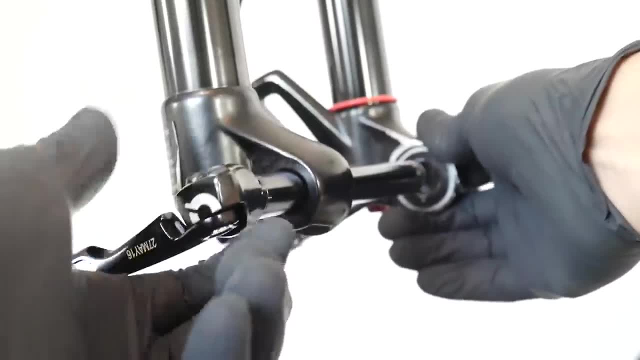 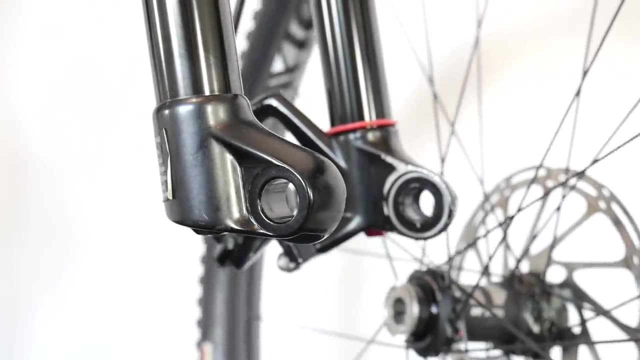 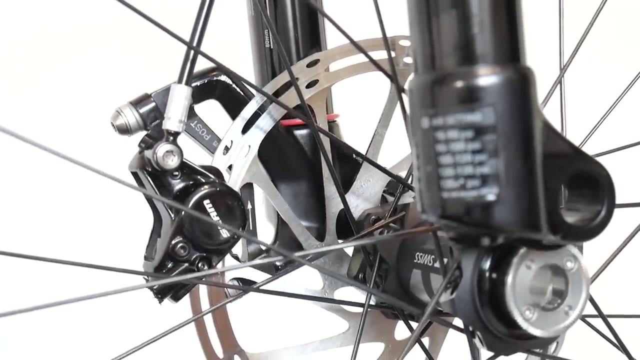 Okay, Now we're going to put the wheel back on the bicycle and fasten it with the right force, So let's just put it back on the fork or on the frame, knowing that the disc brake rotor must go exactly in between the braking pads. 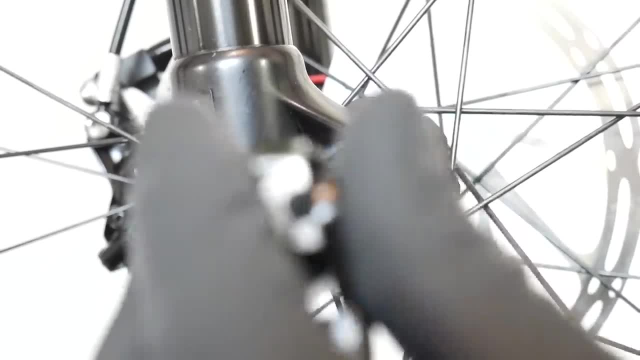 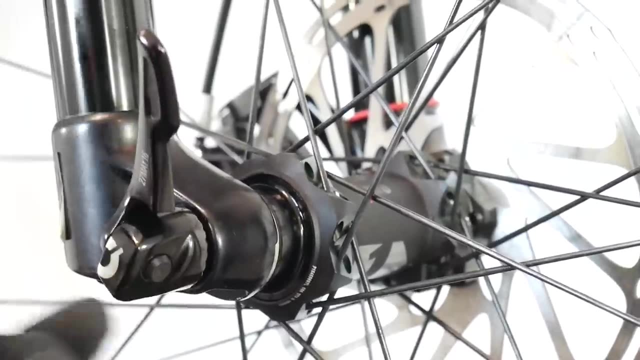 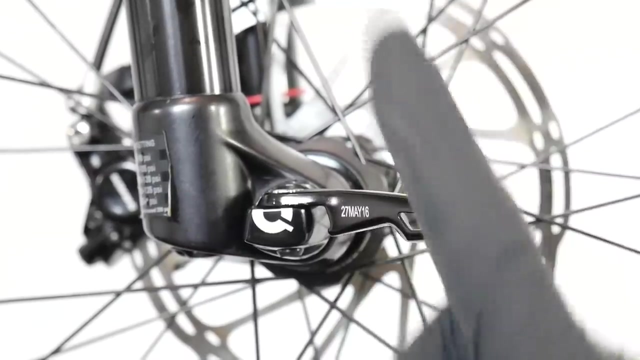 Now the wheel is on its place. If the thru-axle is already fitted on the both sides, we are threading it in In order to fasten our wheel with the right, and always the same amount of force. we should pay attention to the position of the lever. 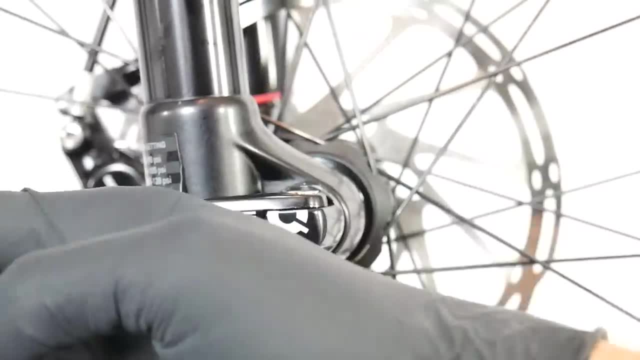 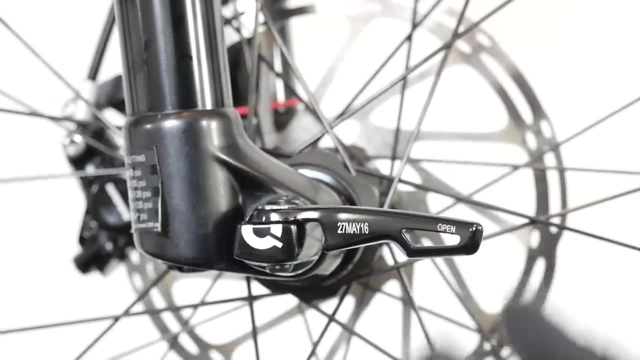 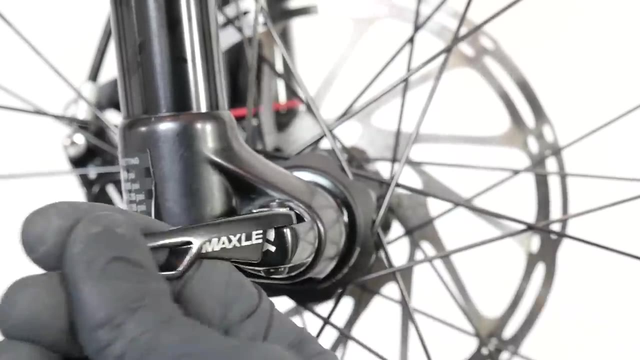 On my bike it is always directed to the back of the bike and parallel to the ground. If you're not sure whether it's the right amount of torque, you should start feeling some resistance on the lever, just about 90 degrees before it's fastened. 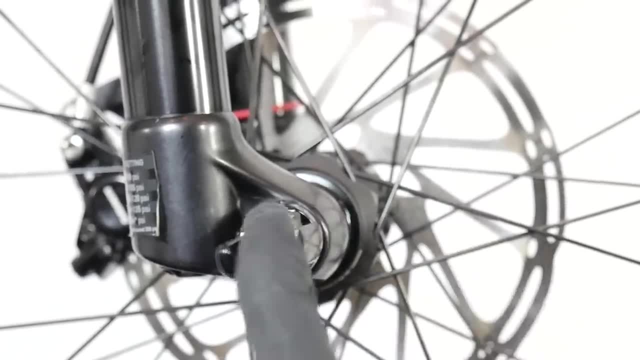 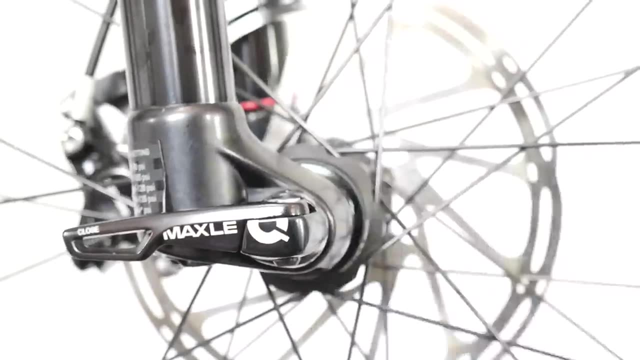 So this is loosened right now. So I don't feel any resistance. I'm just starting to begin to feel the resistance. Now I'm locking it and it's fastened. very well, Doing it in this way, you won't have any problems with the disc brake pads rubbing against the 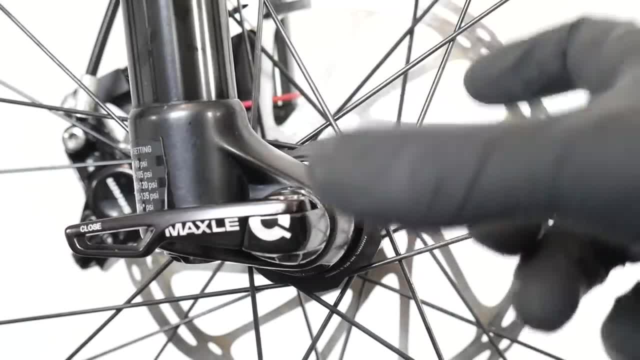 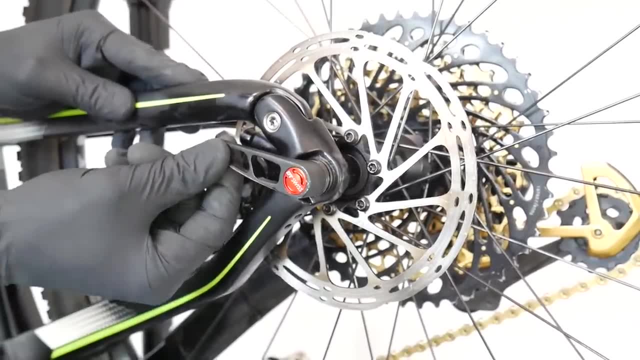 rotor, because you will always have the same amount of force on your axle. And this is the second, very similar type of the thru-axle. In this case we don't have any lever which would open and close like a quick release, We simply pull. 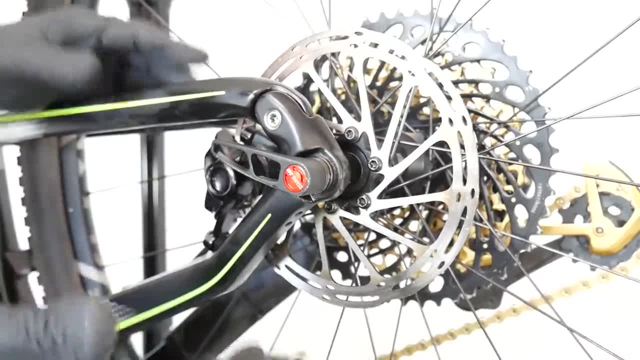 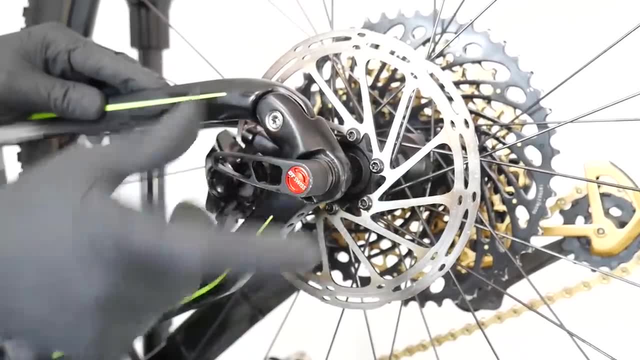 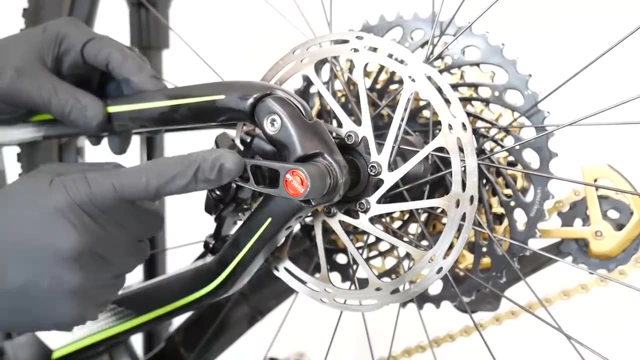 Unthread the thru-axle in order to remove the wheel and then thread it back in. So the whole procedure of removing the wheel or replacing the wheel is pretty much the same. We only need to find the right position for the lever and have it always the same before. 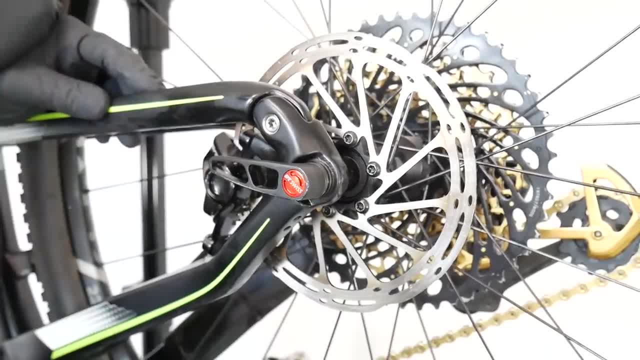 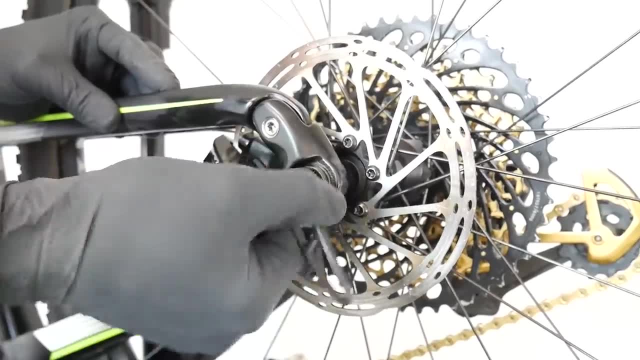 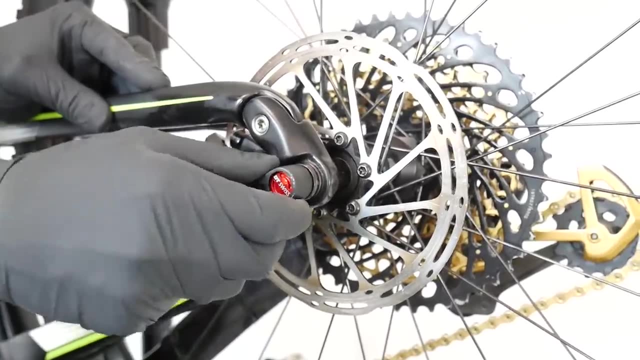 removing the wheel and after putting it back on the bicycle. If you do it for the first time, it may occur that your lever will be in some awkward position. That's why these systems will allow you to change the position of the lever. In this case, we need to pull the lever and then we can find the best position for it. 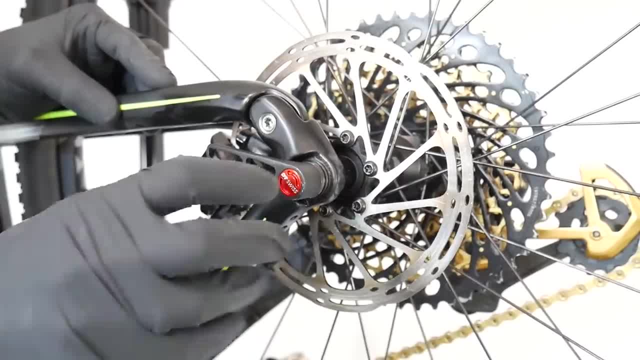 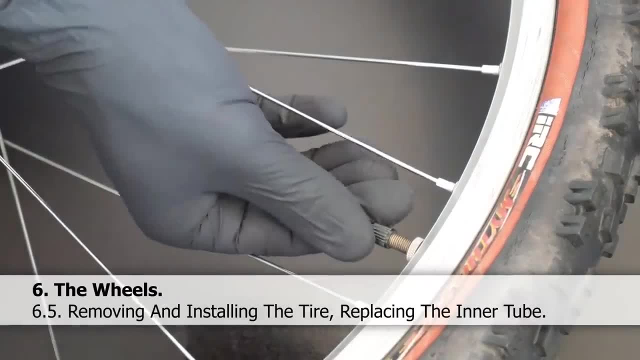 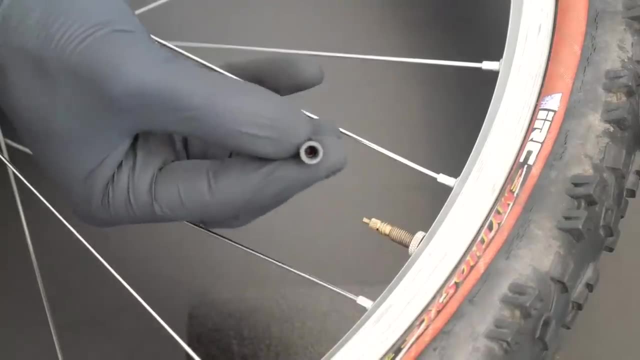 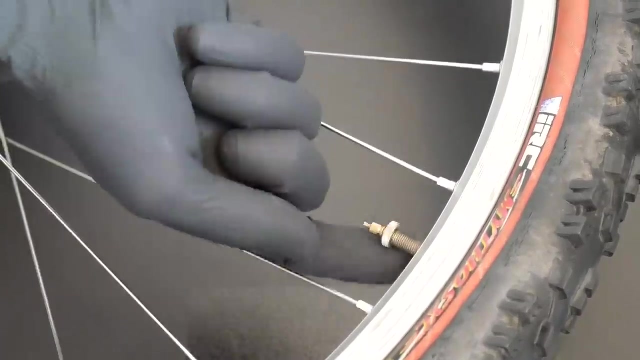 On some other quick releases or thru-axles, we would need to push the lever and then change its position Very easy. After removing the wheel from the bike, we are now removing also the valve cap which is protecting the valve against any dirt, And then also the nut which is securing the valve against the rim. 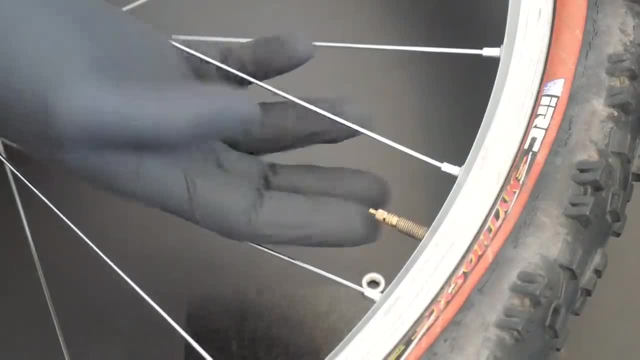 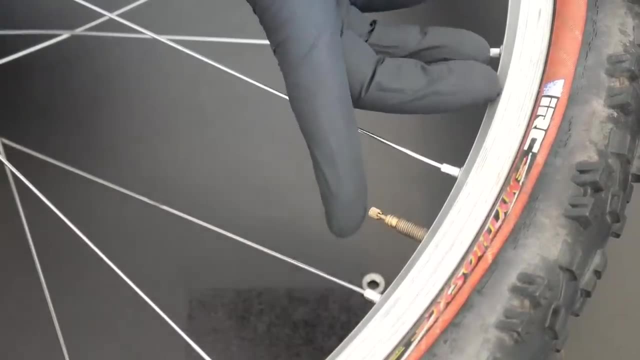 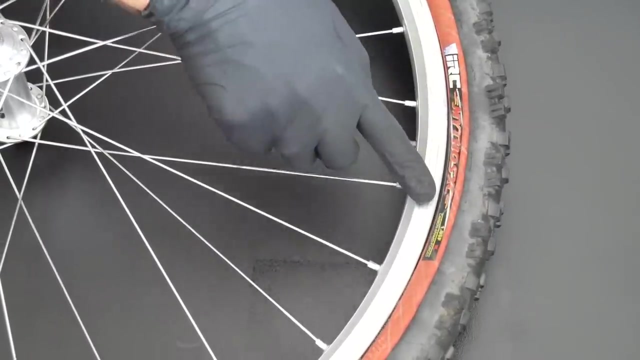 Don't lose somewhere these two little things. In order to let the air out thru the Presta valve, we need to unthread the additional protection here and now. the air is going out. Now we just need to remove the bead of the tire, at least from one side out of the rim. 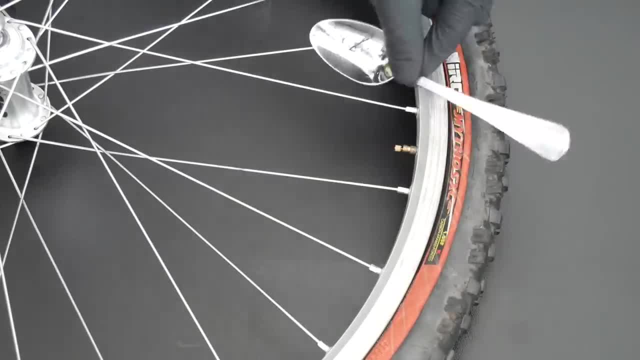 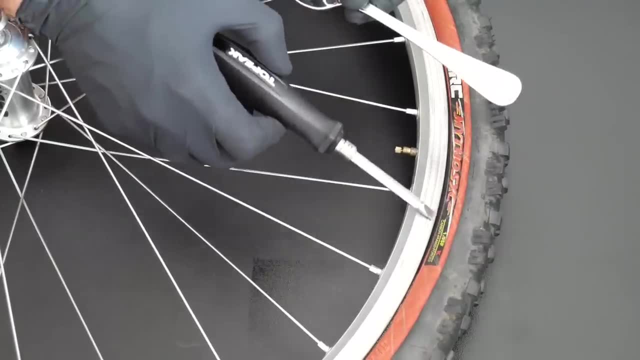 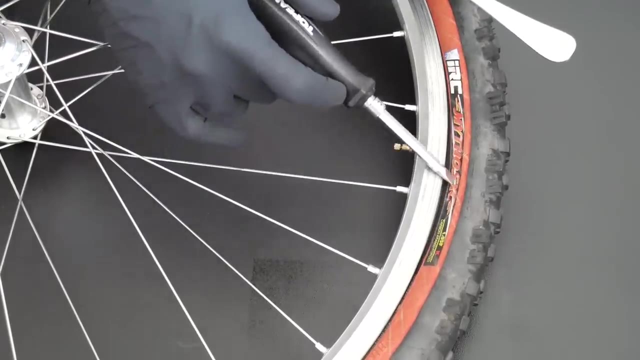 so that we have the access to our inner tube. We do not use for this purpose A spoon or a metal screwdriver or any other object that could scratch the surface of the alloy rim or damage the carbon one, or even more so it could cut thru the tire or thru. 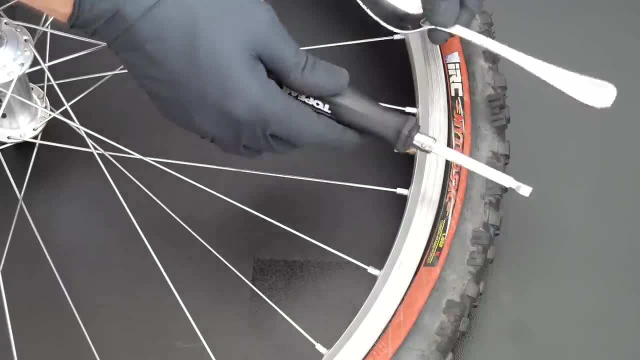 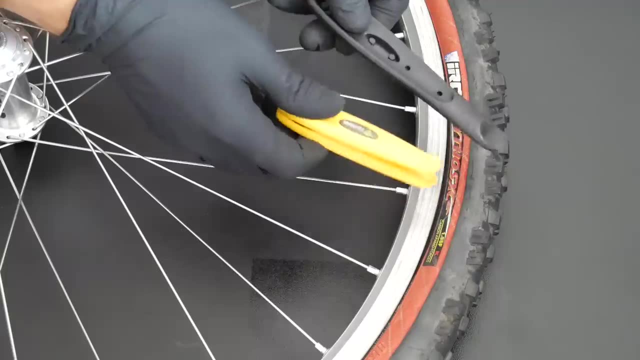 the inner tube. So keep these away from your inner tube. The original tire levers are not so expensive and this help a lot, not threatening your inner tube. The longer one might be helpful if the tire is too heavy. The longer one might be helpful if the tire is too heavy. 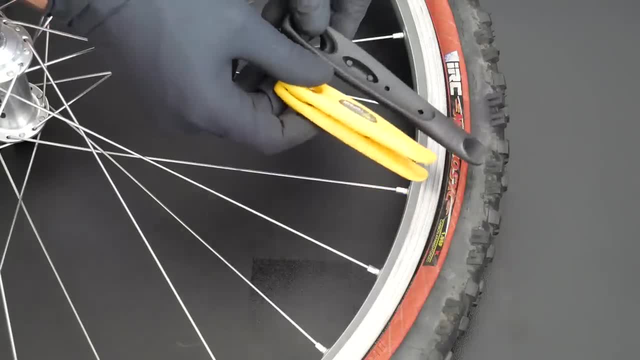 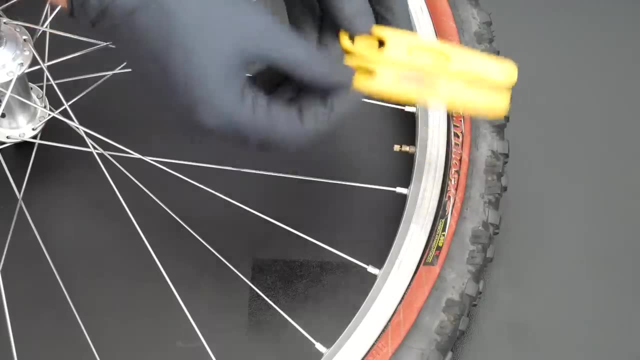 The longer one might be helpful. if the tire is too heavy, The longer one might be helpful if the tire is to tight approached and difficult to remove. but it does not happen so often, so normally I would use just 2 smaller levers. So one side of the tire lever so that it will scoop up the bead of the tire and the other 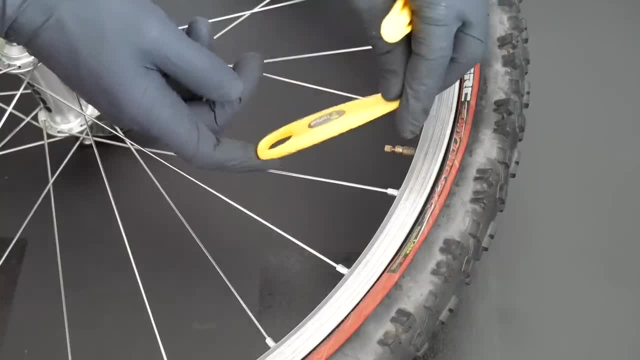 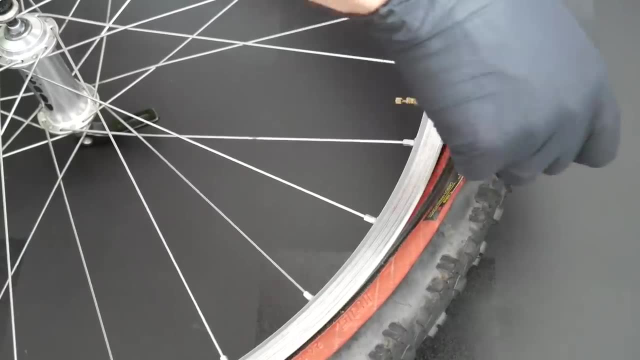 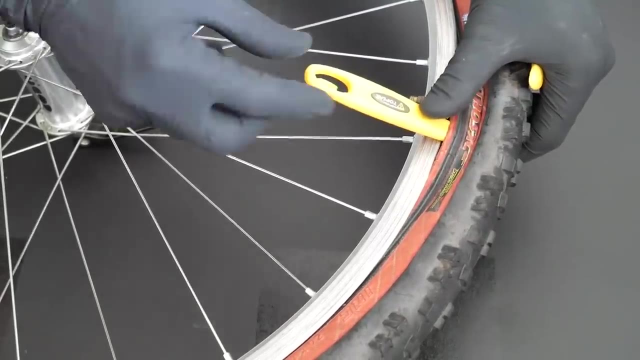 has some of kind of a hook for the spokes for their Bend function, and it works like that. I am scooping up the bead of the tire and making sure that I only catch the tire and not the inner tube, Which is there also. I could also damage it, and now I'm using this hook and fastening my tire lever like that. 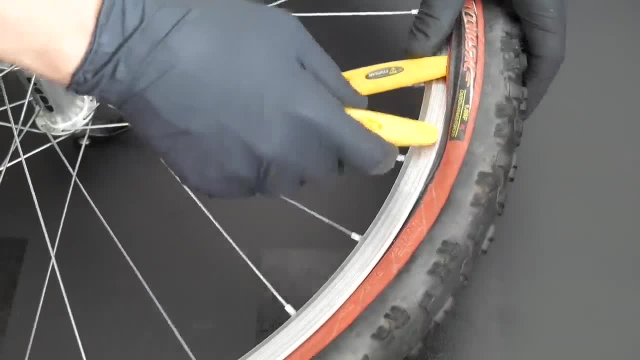 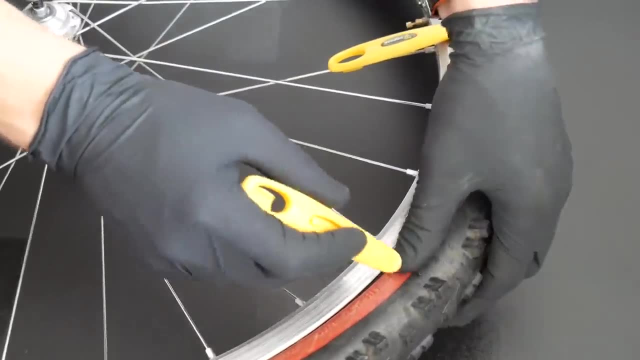 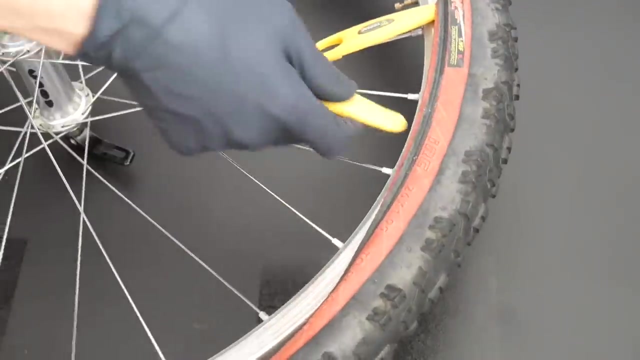 now I have both- both hands free so that I can continue removing the bead just very gently. the tire is still pretty tight, so I'm just gonna do it for the third time and now it will be very easy to remove the whole tire. it just goes like that. 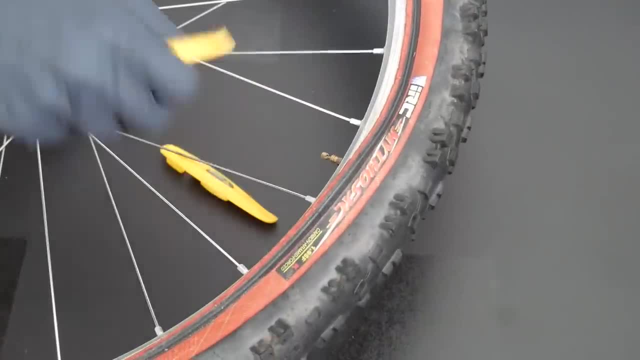 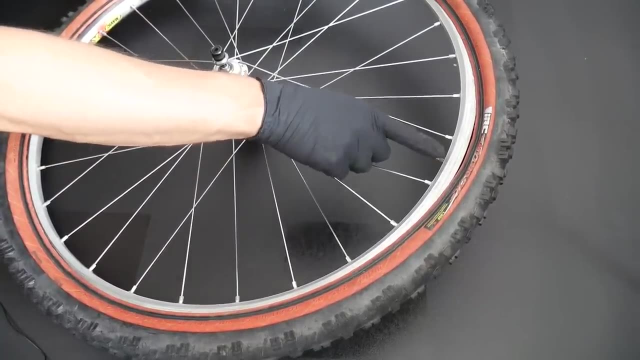 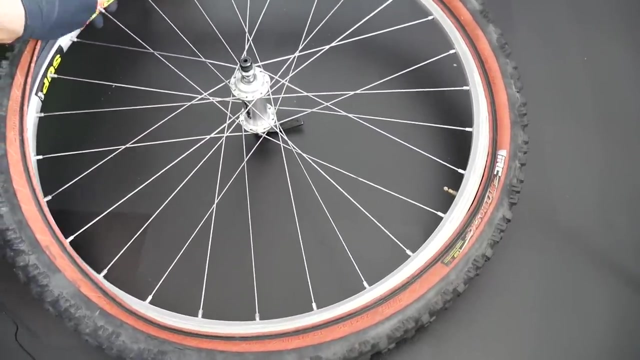 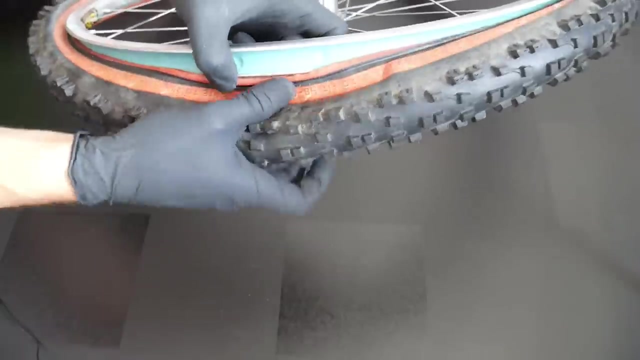 and the bead is off. you may have noticed that I started and finished opening the bead of the tire just around the valve area and now, in order to remove the inner tube, I'm just beginning at the opposite side. it is very simple right now. if you wish, you can also remove the other bead of the tire in order to inspect the tire or the rim. 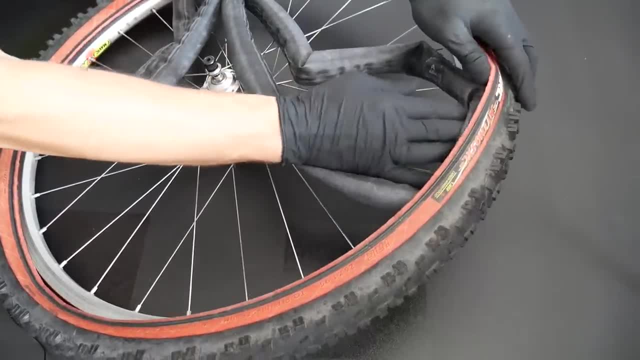 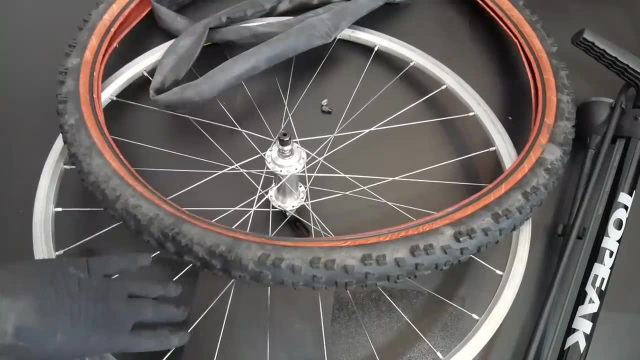 now I'm just pushing the valve back through and my inner tube can be replaced. putting the tire with the inner tube back on the wheel is a fairly easy job, but we need to remember about a couple of things, because if we do some mistakes, it can cost you as a flat tire or a very 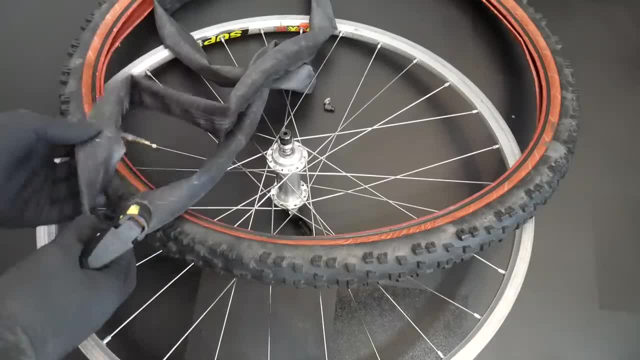 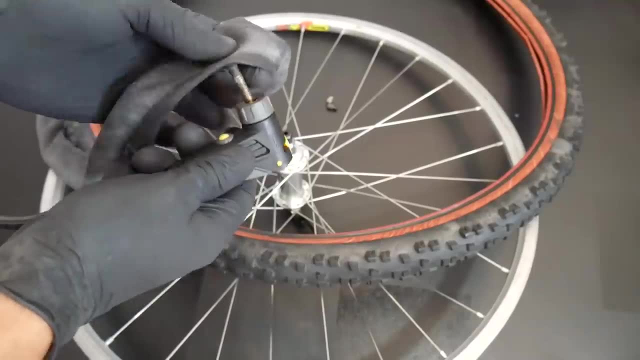 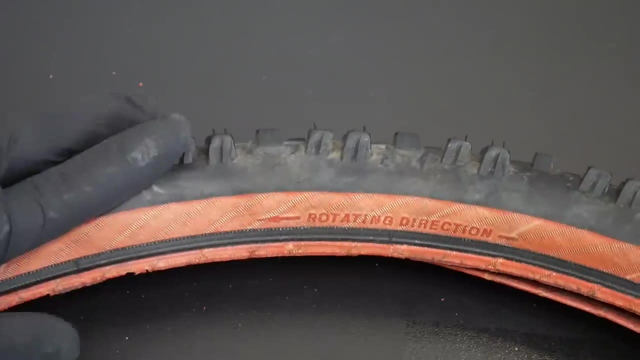 unbalanced rack. alright, here is the first step we want to make, and it's inflating our inner tube just a little bit so that it will get into its shape. now don't forget about the second step, which is deciding in what direction your tire or whole wheel. 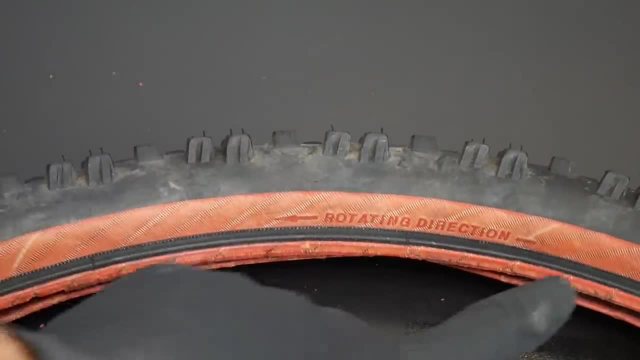 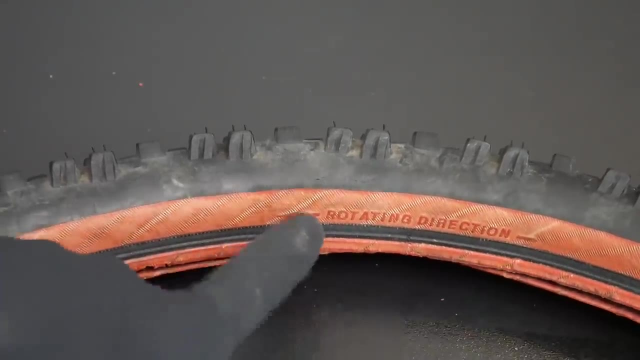 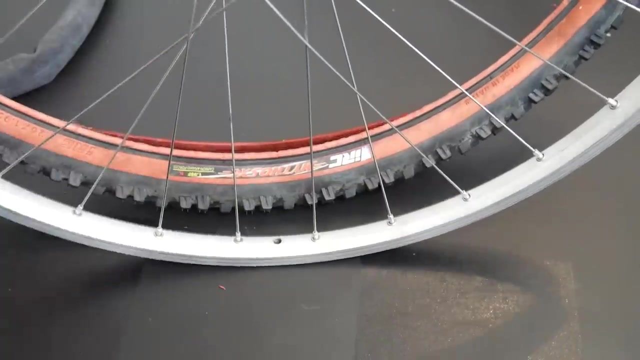 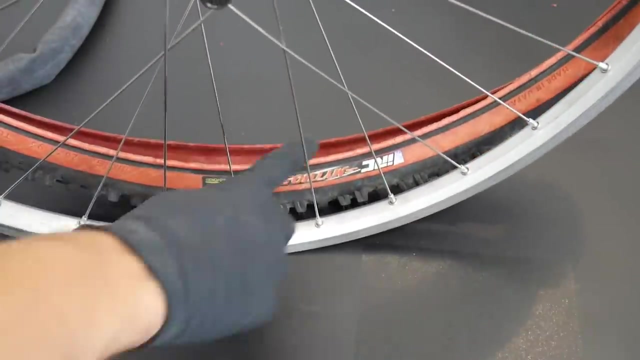 should spin if you have the directional tires, like in this case, usually we would adhere to the recommendation of the manufacturer. so in this case this tire should spin to the left, so counterclockwise. in the third step, once we know in what direction our tire should go, we can put one bit of the tire. 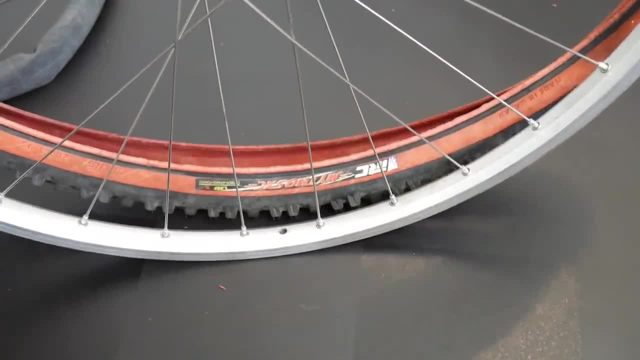 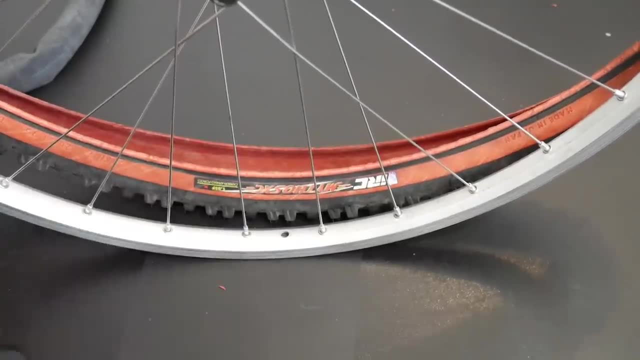 into the rim. it is also a good idea to align some graphics on the tire with the valve so that it will be always easier for us to find the right tooth. validated some graphics on the tire with the valve, so that it will be always easier for us. 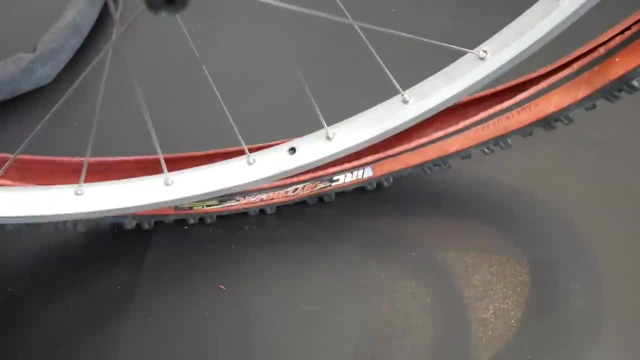 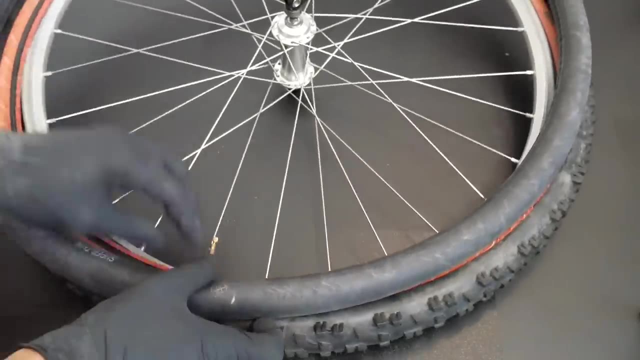 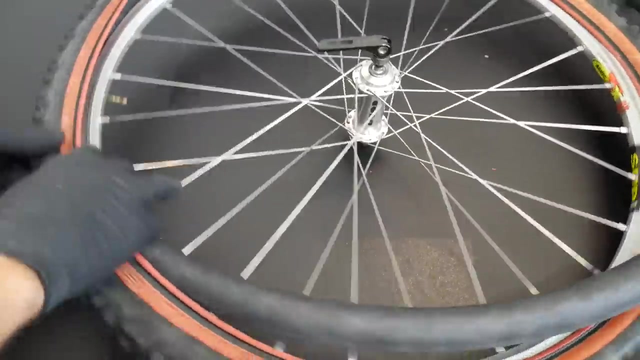 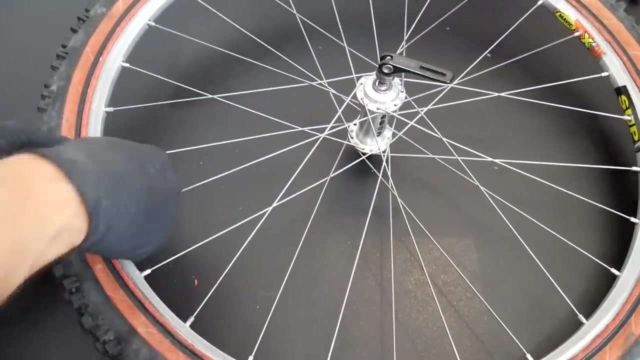 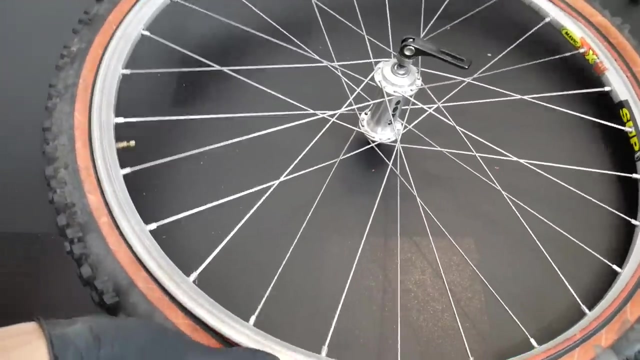 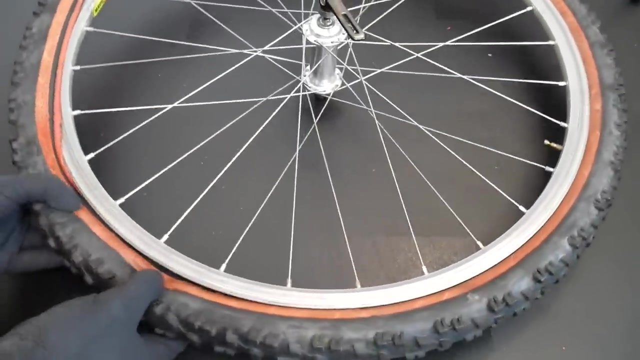 to find the valve on our wheel. it's time for the inner tube. at this point we want to make sure that the valve is absolutely perfectly straight. if the bit of the tire seems to be very tight, make sure you just push it deep into the inner tube, so that it will be always easier for us to find the valve on our wheel. 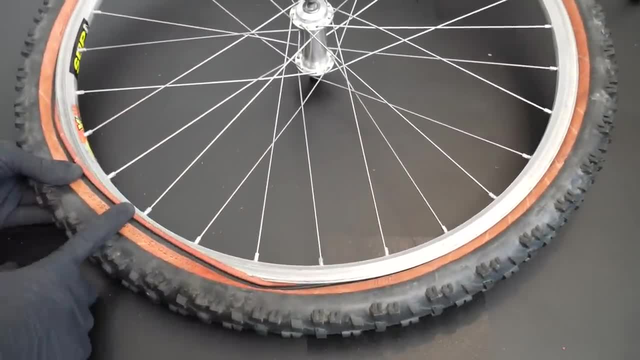 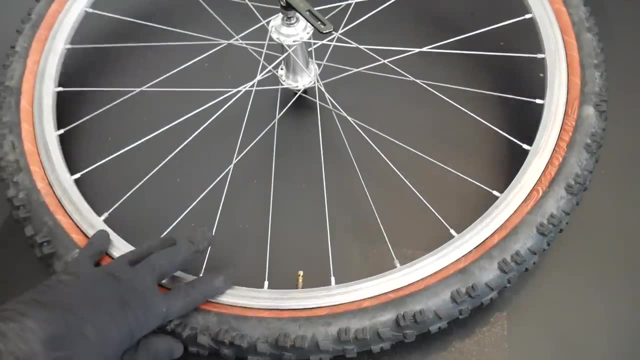 if the bit of the tire seems to be very tight, make sure you just push it deep into the inner tube, the rim, and you can also have help yourself with the tire levers. and so we've made the fourth step, which was putting the inner tube into the tire and 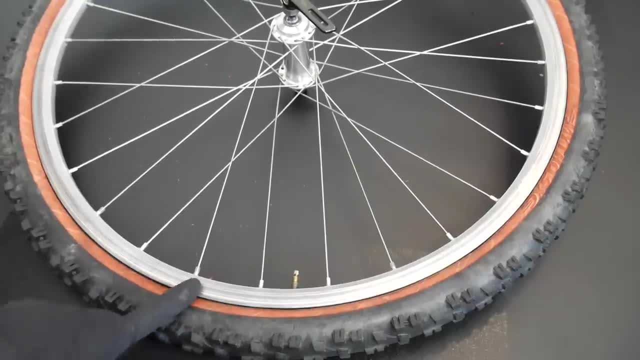 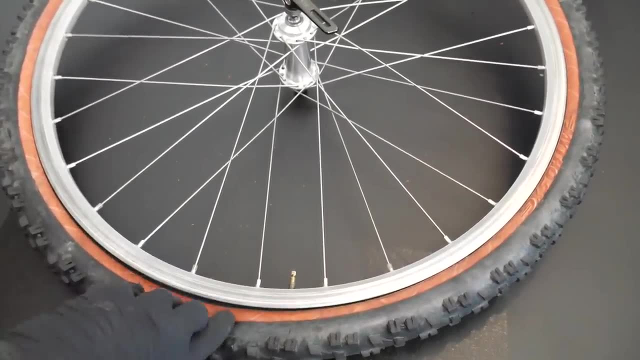 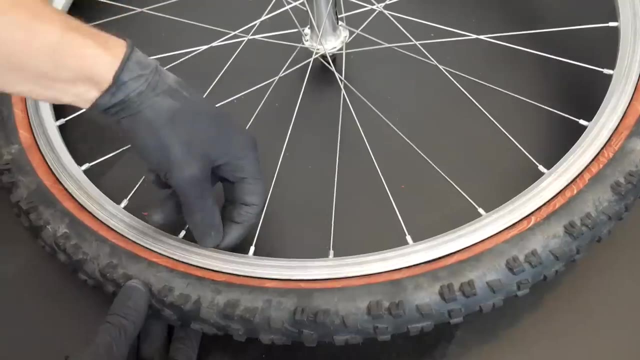 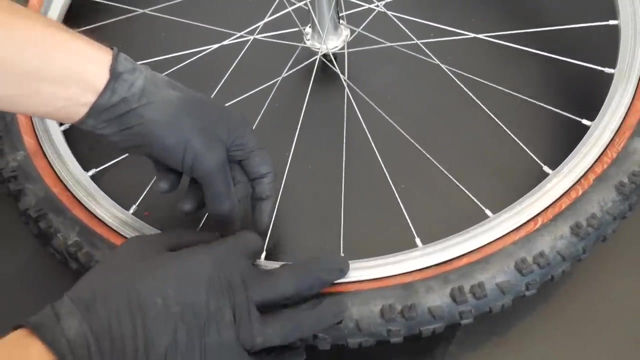 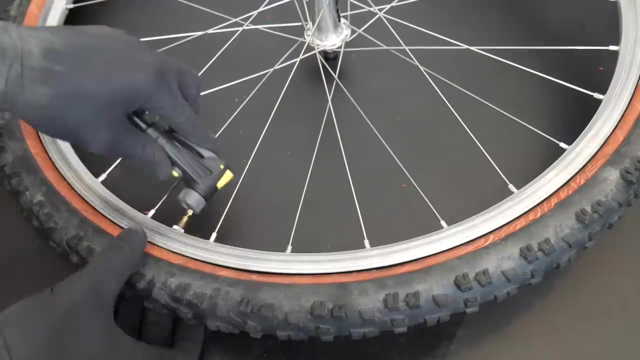 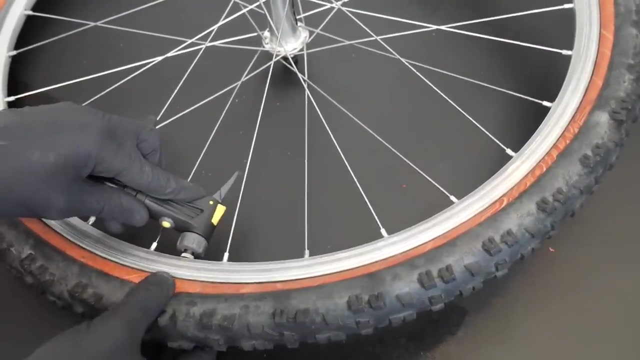 also putting the other bit of the tire into the rim. in the fifth step we are fastening the valve, putting just a little bit more pressure or the air into the tire and we will align the tire throughout the whole length of the bead. beat easy underneath piece. 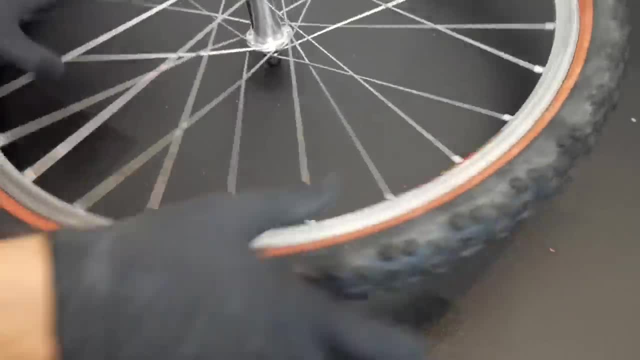 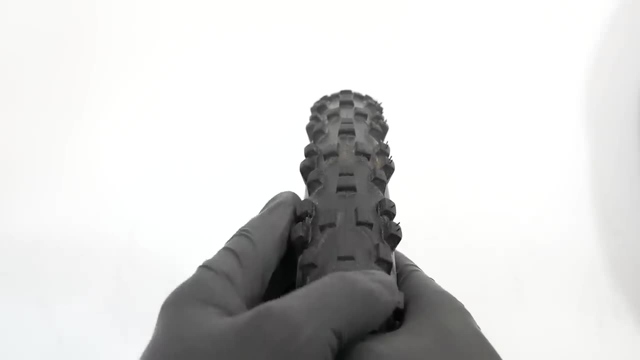 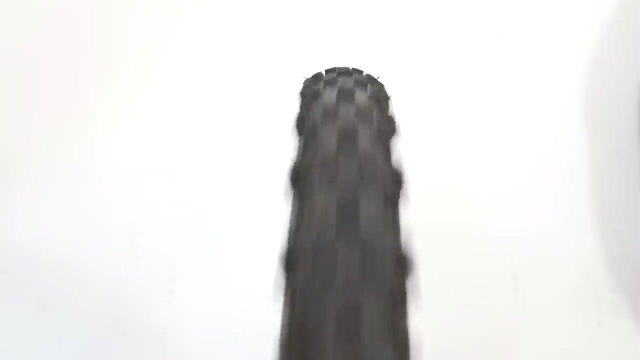 you not comfortable with the pieces? we're going to check the alignment of our tire. Does it move up and down or to the sides? Is it really well aligned with the rim? Let's just see. This tire looks pretty good. It is time for the. 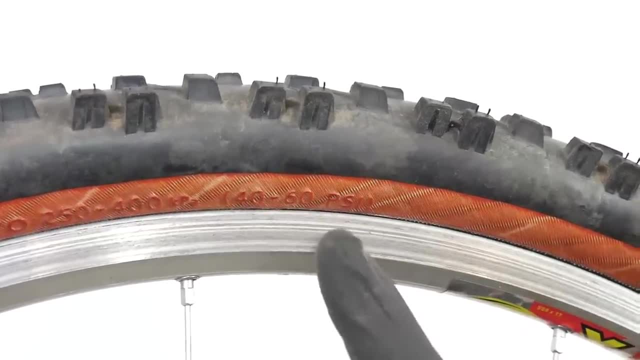 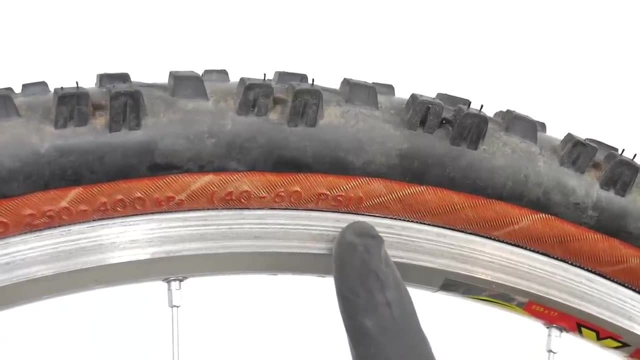 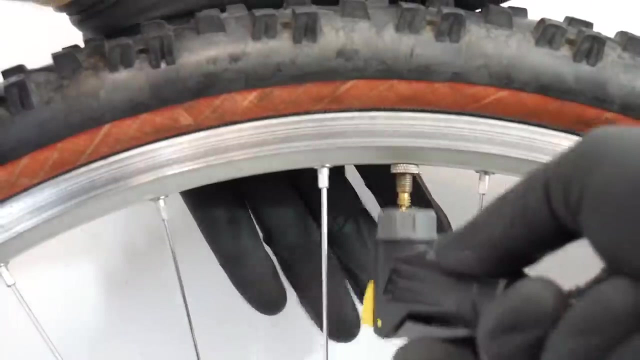 sixth and the last step, We need to find the air pressure recommendation for our tire. For this model it is between 40 and 60 psi. Now, according to our preferences, we're gonna inflate the tire somewhere between these two numbers, 40 and 60.. 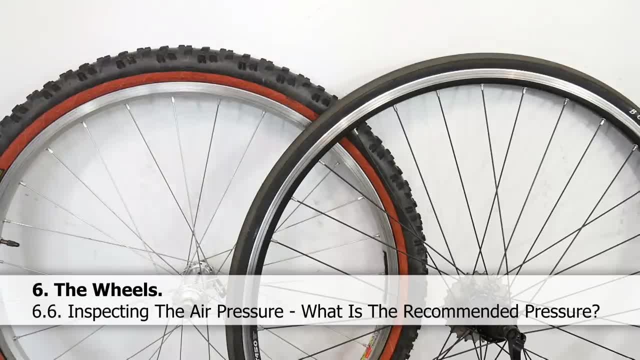 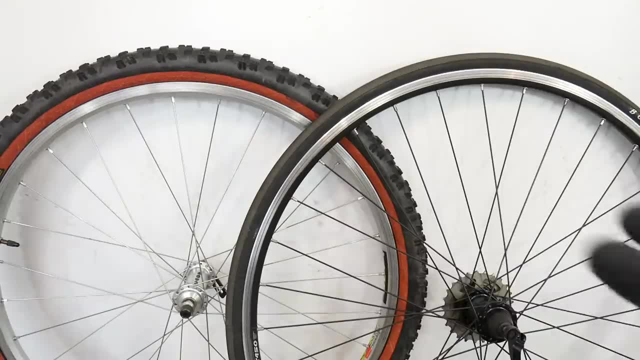 Why should we regularly monitor the tire air pressure on our road bikes and mountain bikes? Because it will affect our safety, traction, speed and efficiency, and also puncture resistance and comfort. So what is the best air pressure for my mountain bike and a road bike? Well, it will. 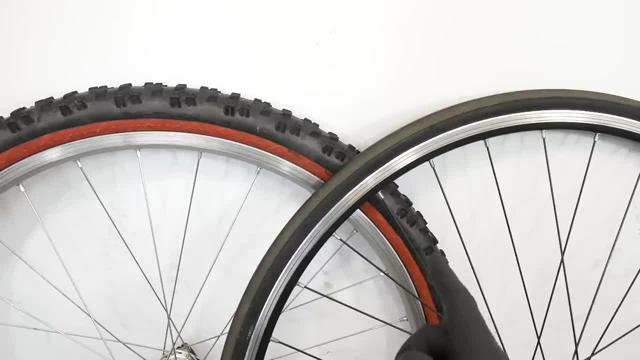 depend on your weight, the size of the tire, the size of the wheel and, of course, the terrain you choose to ride through. But the general rule of thumb is that on the mountain bikes and the system it would be around 2 bars. Mountain bikes with the inner tube that would be more, around 3. 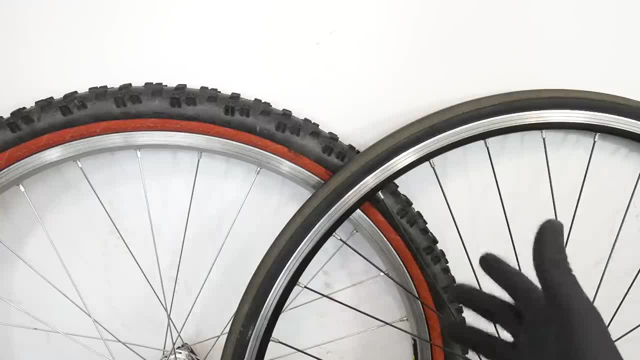 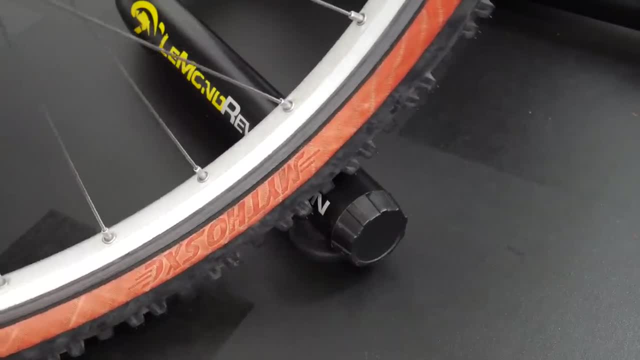 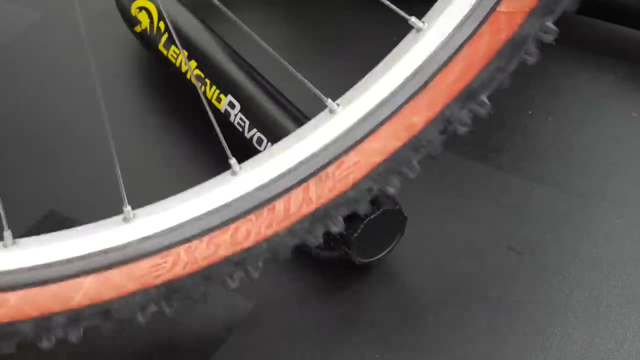 bars and road bikes with the inner tube, that would be just around 7 bars. If you don't have the pump with the air pressure gauge, here's the test you can do to at least find out whether the air pressure on your bike isn't too low. Find yourself some kind of an obstacle just like this one. 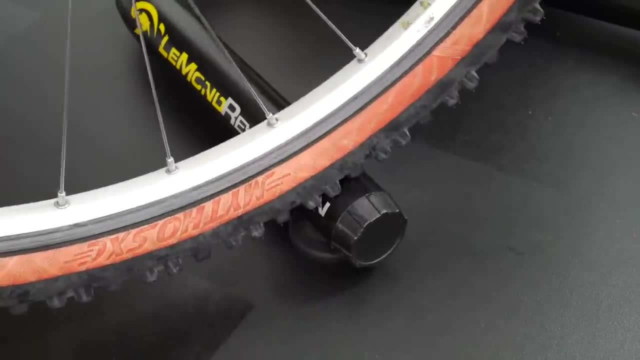 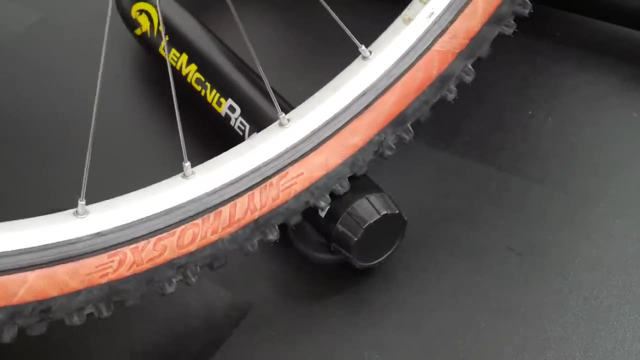 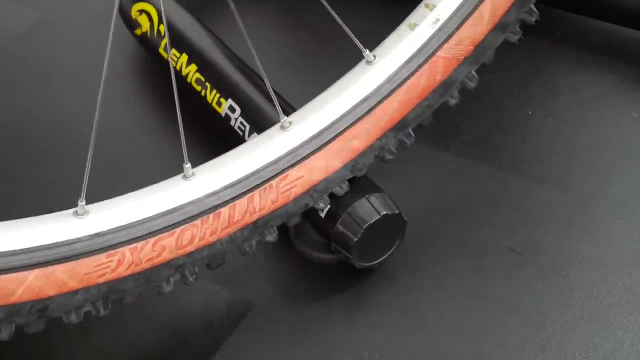 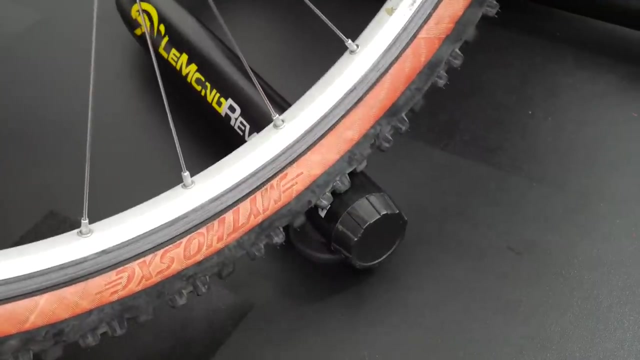 and then push the wheel of your bike, the weight of your body, against this obstacle. As you can see, if you can easily push it the whole way through, feeling that it's the edge of the rim that stops on the obstacle, the air pressure in this tire is too low for you. It will be very easy for you to get a pinch flat or even damage. 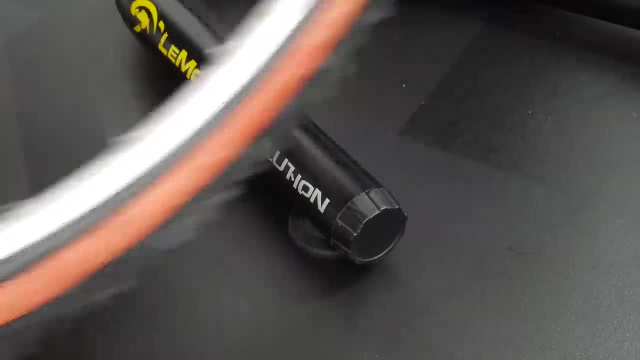 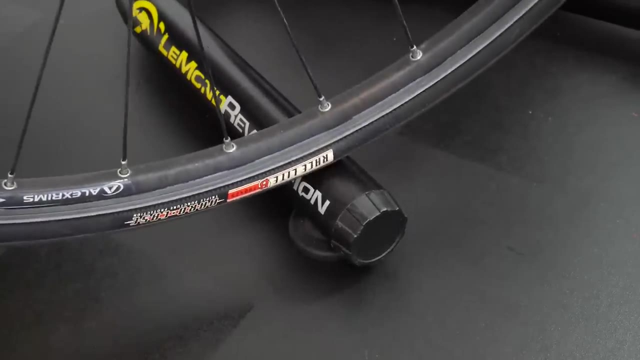 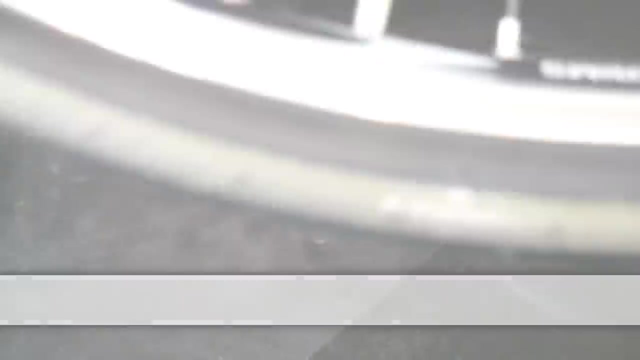 the tire, the inner tube or the rim, And it will look the same for the road bike. This is too low. Now we're going to clean and re-grease the angular bearings of the rear wheel, because we have to remember to start the whole process from the non-drive or the left side of. 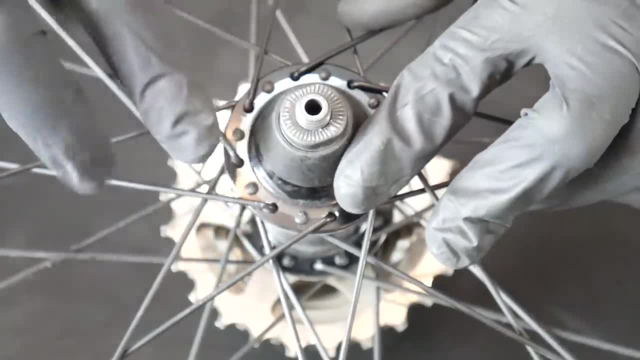 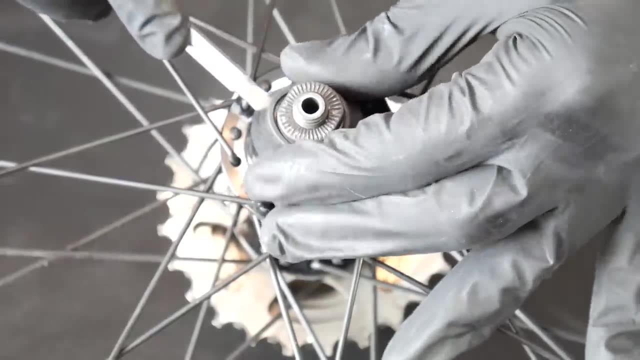 the bike. Now we can see the nut here, but we need the access to both nuts, so the other one must be hidden under the seal. Just be careful with all kinds of seals and rubber parts of your bike. I'm trying to gently remove it from the axle. 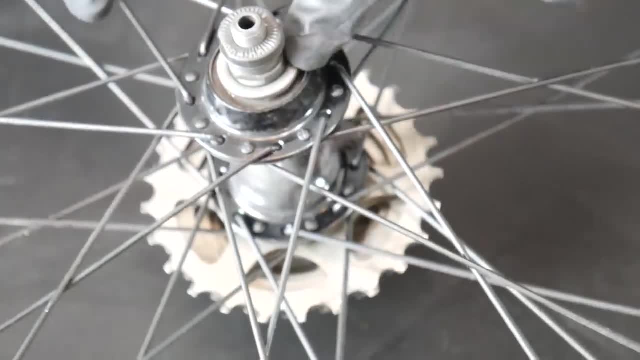 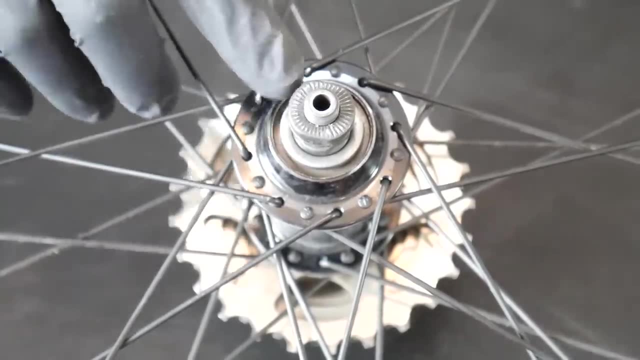 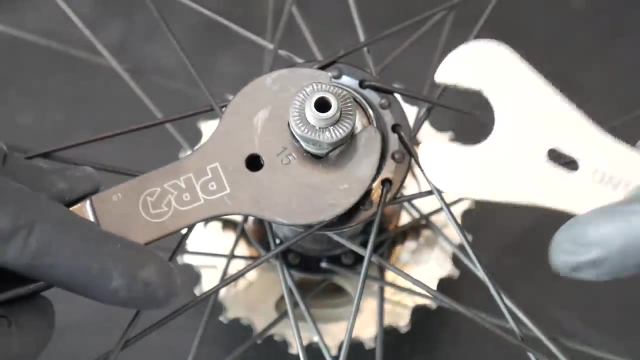 Just like that. Now we have access to both nuts. Now we just need to find out what kind of wrench we're gonna use for both nuts. In this case, on this bike, the external one is the 17 millimeters and the internal one, the one here, is 15 millimeters. Now we know what to do. 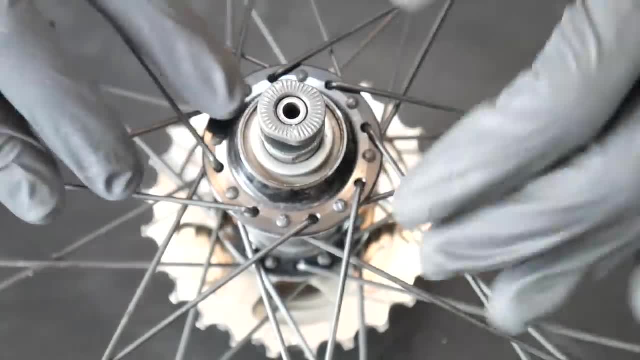 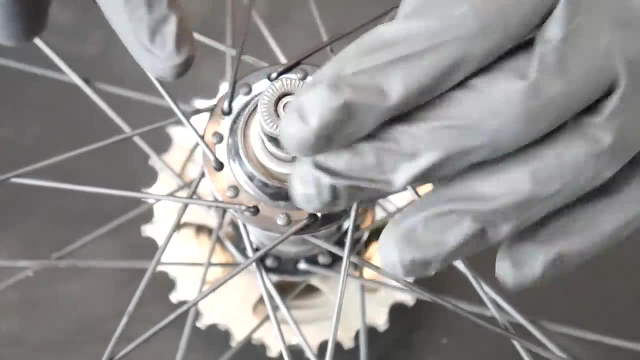 Now very important principle: before removing anything from the bike, We need to make sure that we will remember the order of all the nuts and spacers and shims. So put those aside just one by one, knowing in what order you will be putting them back. 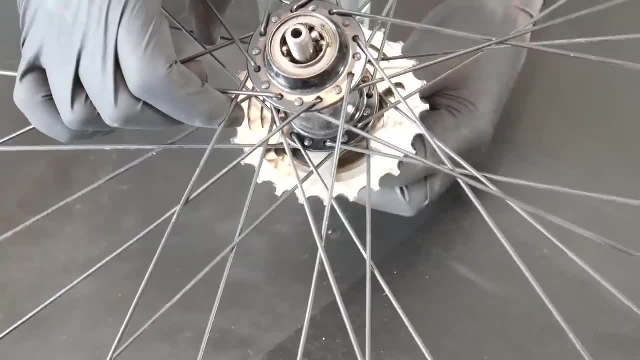 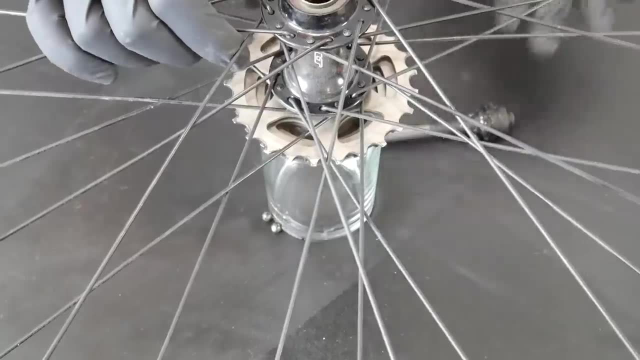 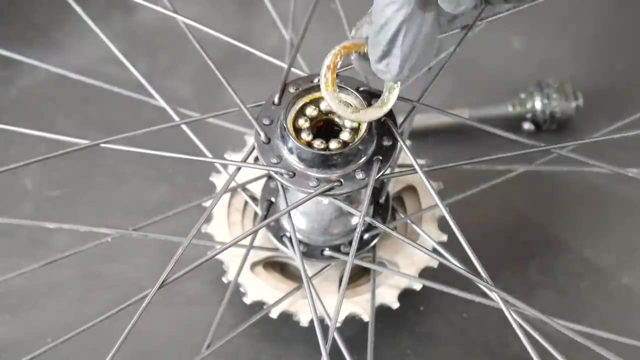 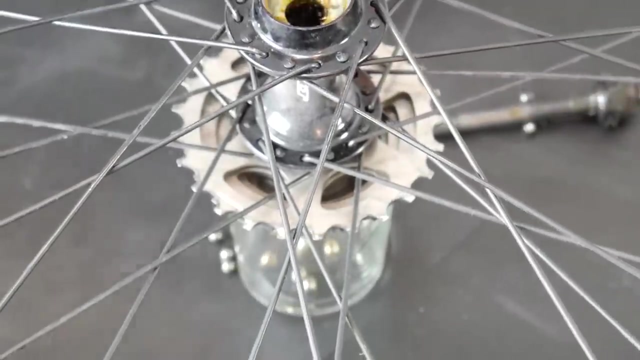 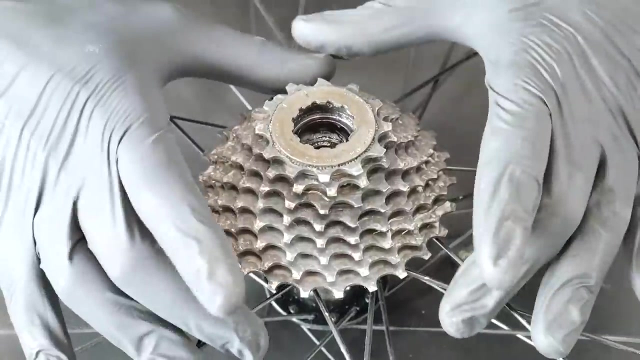 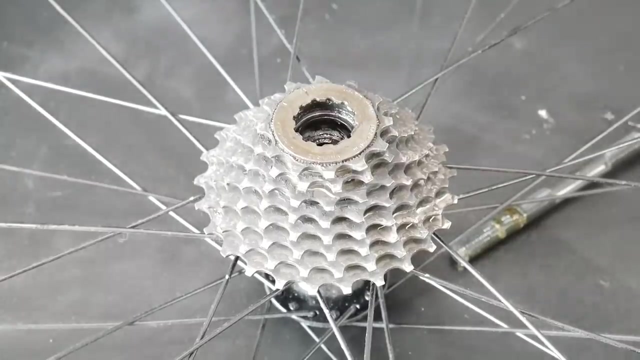 Great. we can already see the balls of our bearings. Let's take a look at the assembly. After removing all the balls and gathering those in one safe place, we have now the access to the. In order to make the job even easier, I do recommend removing the cassette. 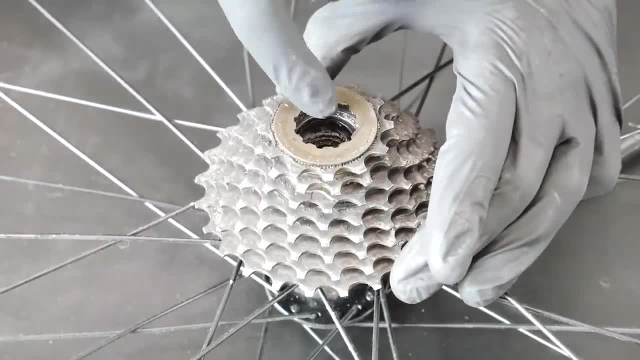 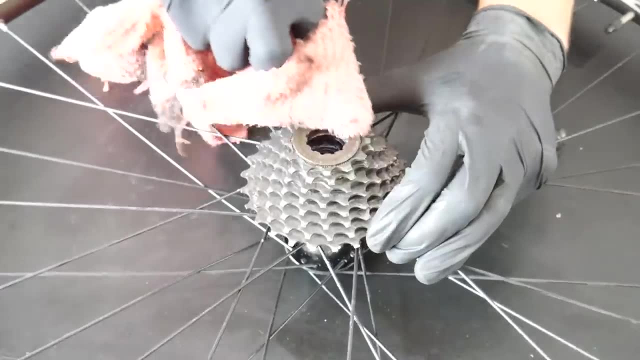 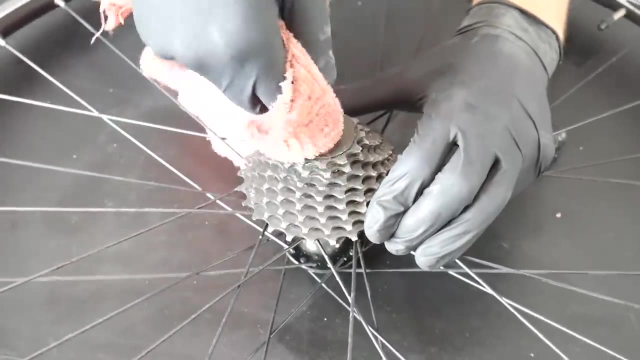 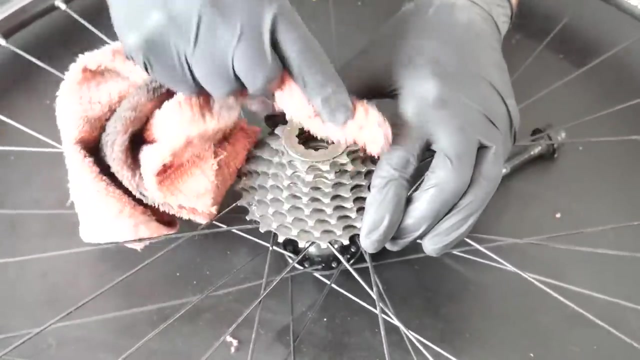 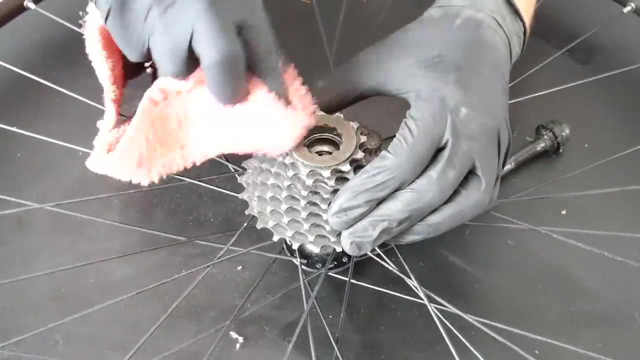 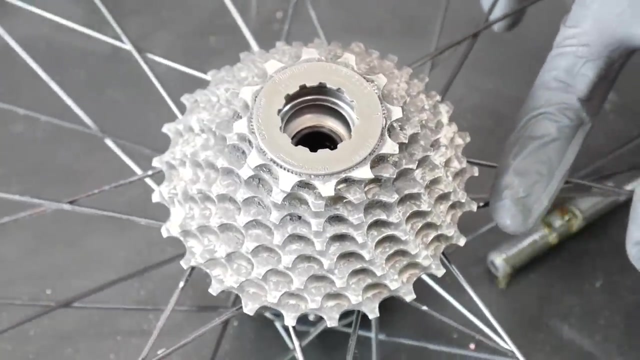 On some hub models it will be also possible for you to remove some seals and clean those. Here the access is very easy, so we start cleaning. The bearing races are clean and degreased on the drive side. You don't have to use degreaser here. 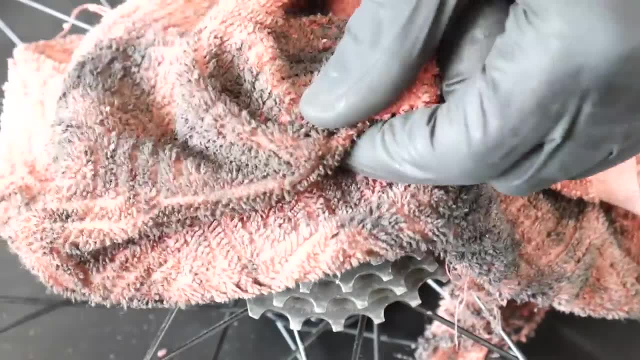 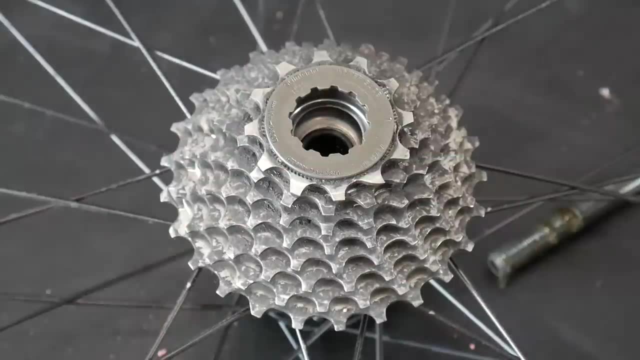 What I would recommend to do is to use two cloths at least: The one which will be the first, one more dirty, and then the second one very clean, so that you make sure there is no, even not even one piece of sand in there. 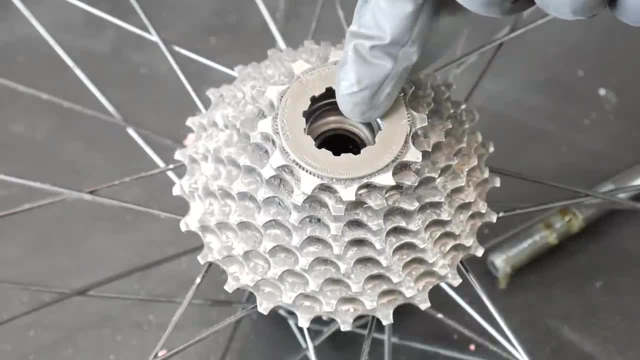 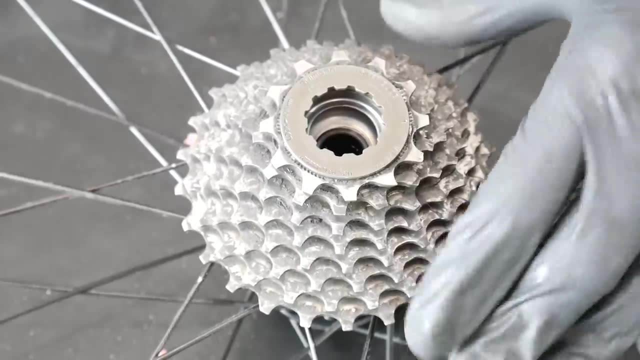 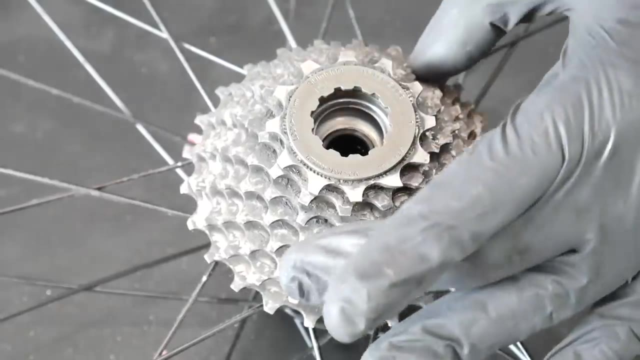 This is also a good opportunity now to inspect the bearing races. You can perhaps see that these are not perfect, Even though this wheel doesn't have a lot of miles on it. this would maybe indicate that someone hasn't been servicing the wheel or that the hub isn't really of high quality. 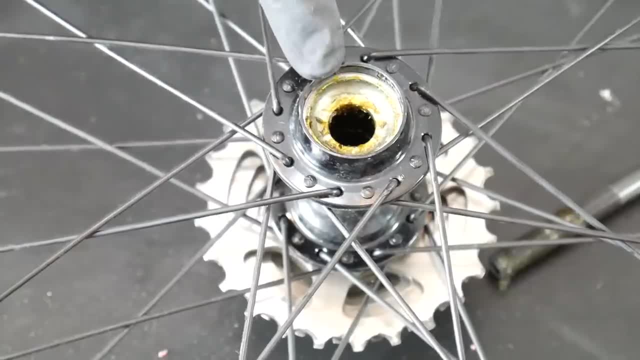 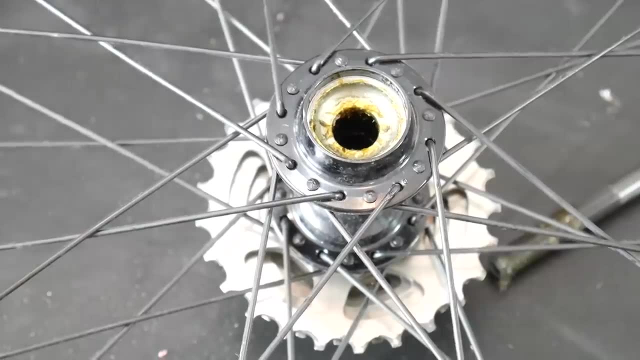 Now we proceed to do the same thing on the other side. This is how easy access I would have to the other side drive side If I removed the cassette. but the cleaning didn't take much time anyway, so I did not do it. It's good to do it. 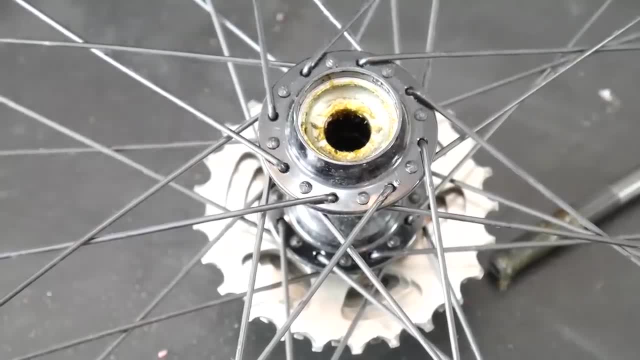 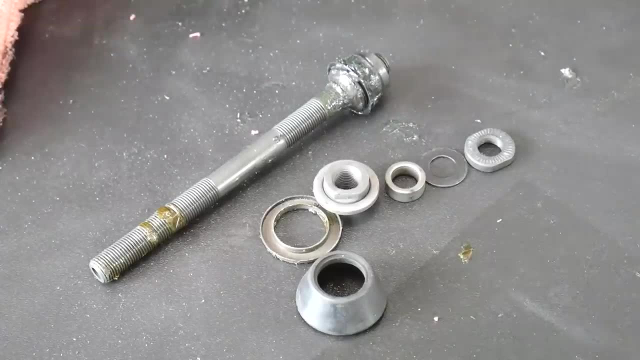 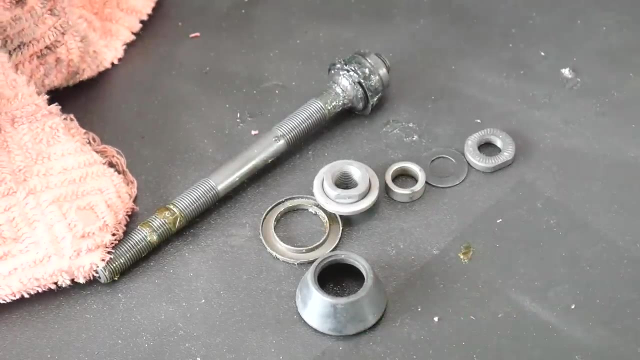 Now I'm cleaning this side and then the axle, the nuts and the bolts. In this case, I'm going to do the same, using first the cloth which is already dirty and then the clean one After that. I'm not putting these clean parts back on my table, which can be dirty. 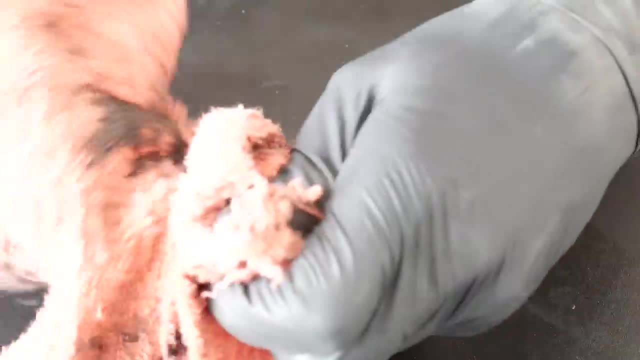 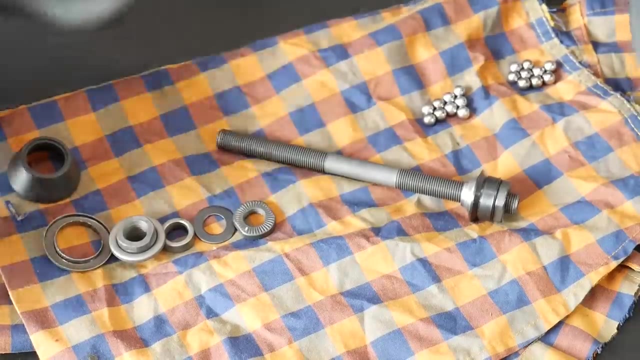 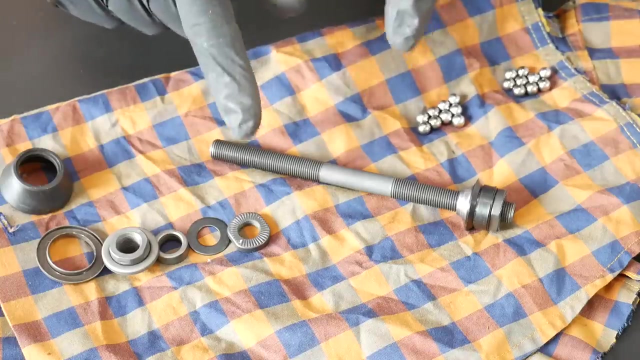 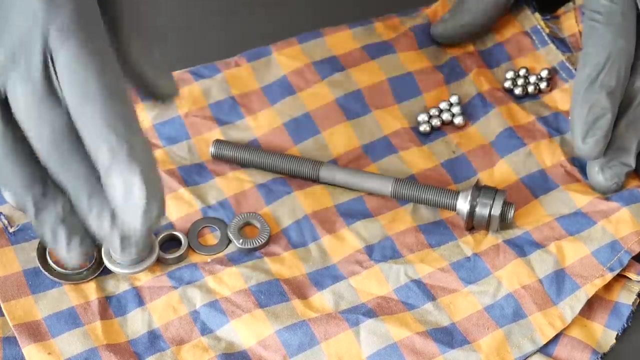 My table is clean, this cloth is clean and, believe me, this is not exaggerating. Just one piece of sand and you're gonna have to disassemble your whole hub again because you will hear that one piece of sand or dirt. So here are all the clean parts. 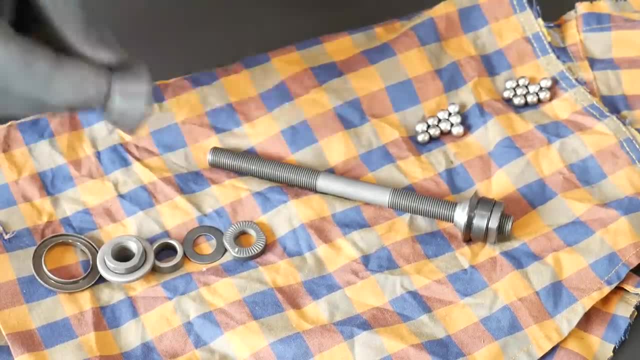 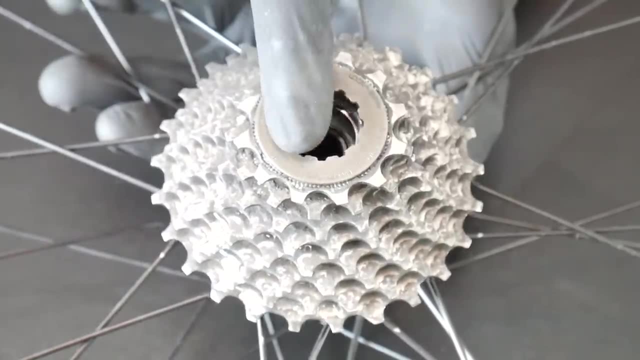 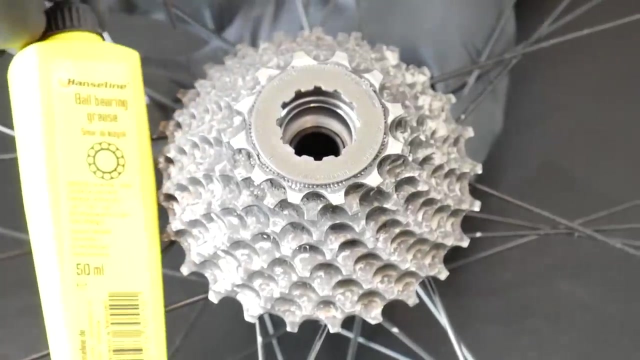 The axle, All the nuts, The seal and then the bolts for both sides of my hub. Now we're going to put all back together. We will start with greasing the bearing on the drive side. What should we use? We can use a grease which is specifically designed for the bearings. 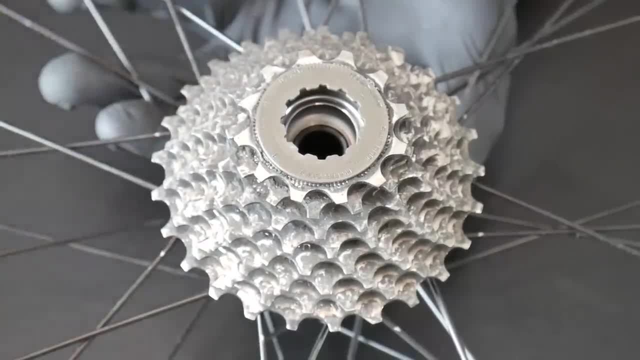 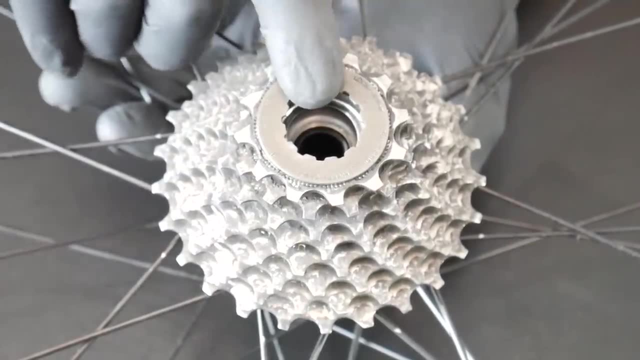 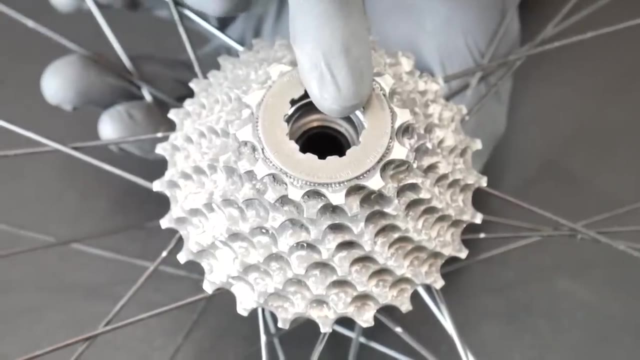 We can use some just general grease for the bicycle. Some advanced racing cyclists would not even use grease- but some oil, some lubricant, which will save them maybe one or two. It will not protect the bearings as good against the water as the grease and it will make them. 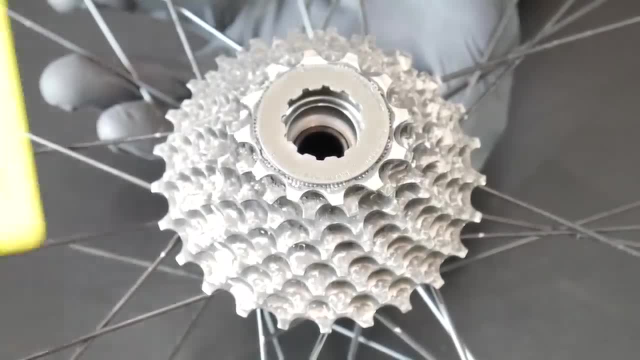 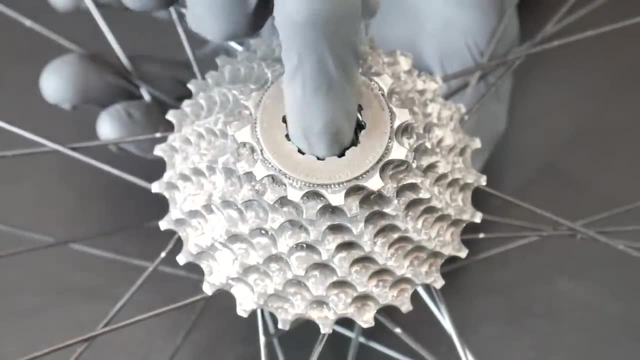 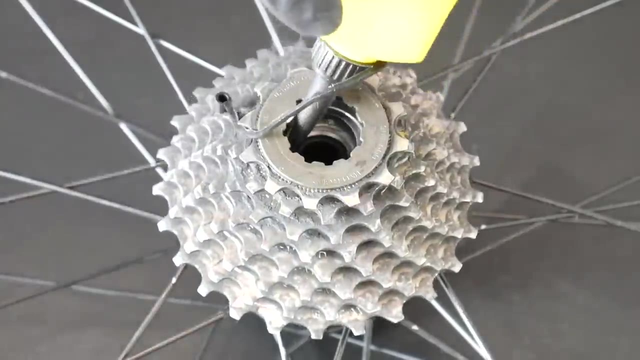 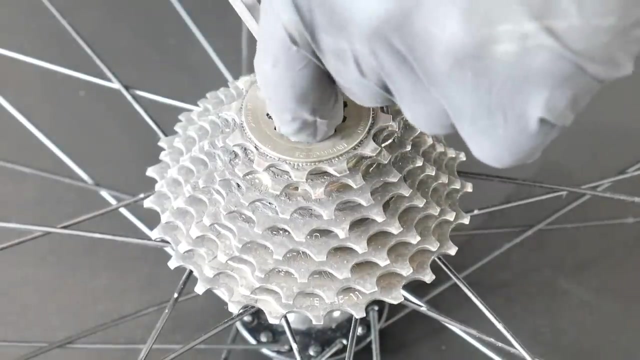 servicing those bearings more often. So we are just using the grease and we use just the amount that will be enough for all the bolts to just stick into it so that we can put the axle. Make sure you have the right amount of the bolts in the bearing. 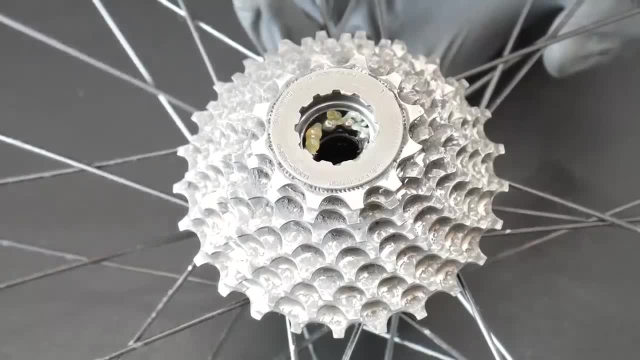 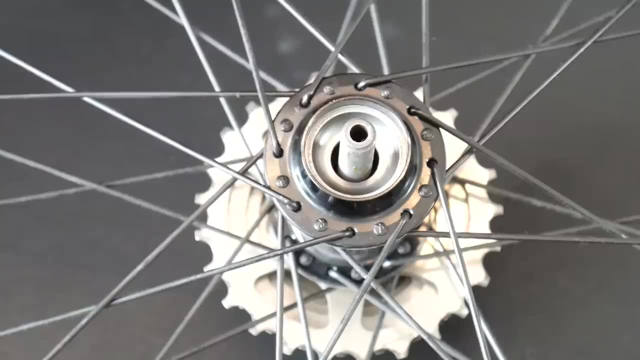 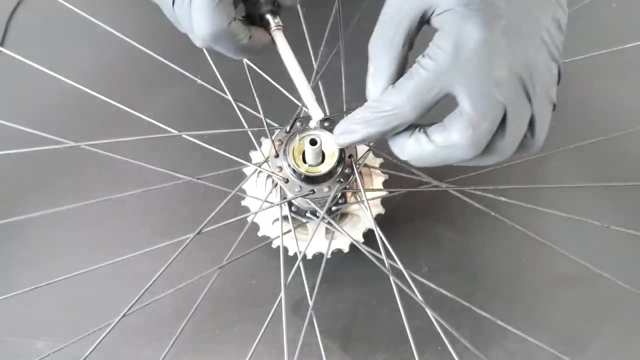 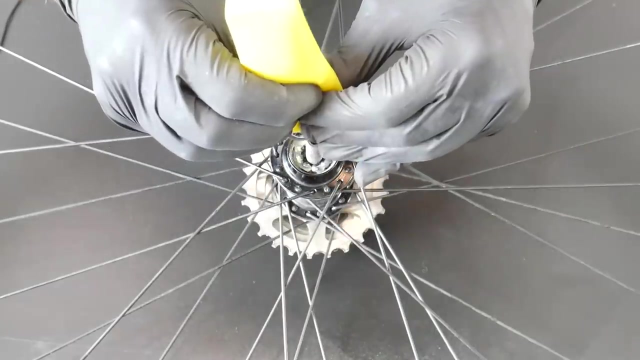 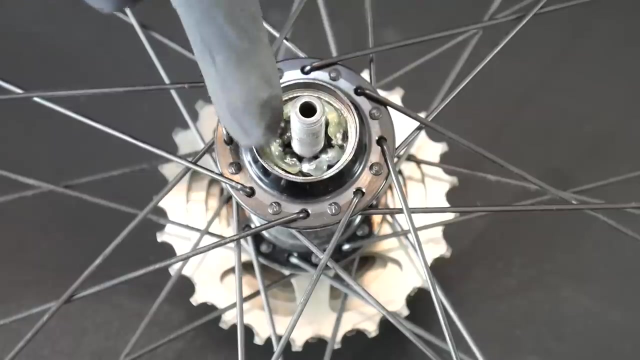 Should be nine. there is nine. Now we can proceed to install the axle. The same thing on the other side, OK, Perfect. Having the axle already assembled secures the bolts on both sides. That makes it very easy for me to put the ones on the left side and put the grease on. 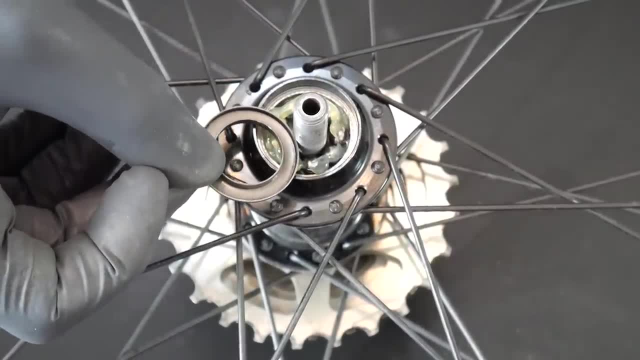 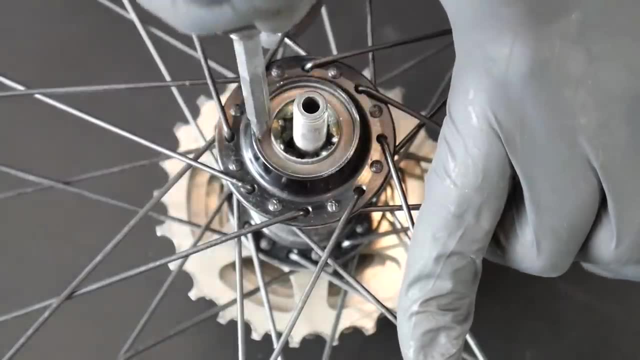 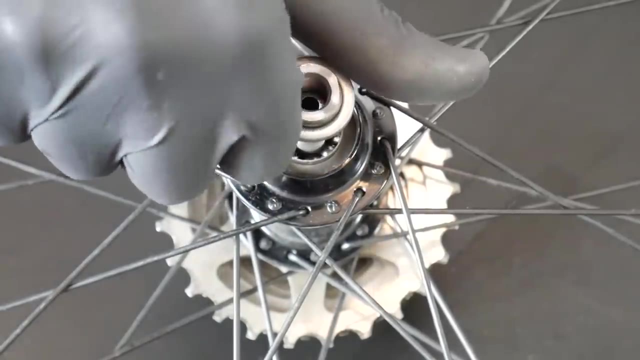 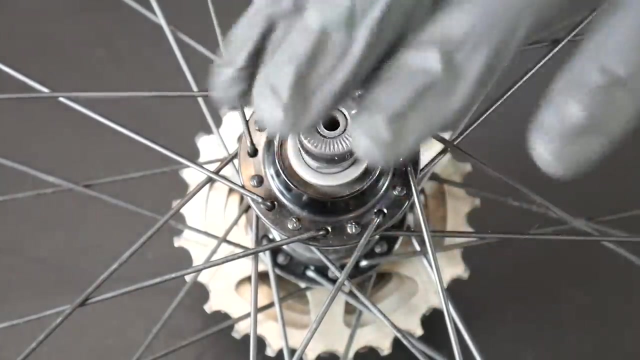 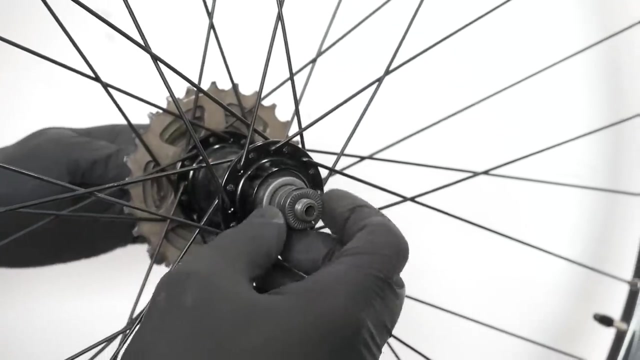 them. Now. it's time for all the parts- spacers and shims- in the right order. Now we can assemble the whole thing. We don't want to have any play on the hub like right now, and also we don't want to squeeze. 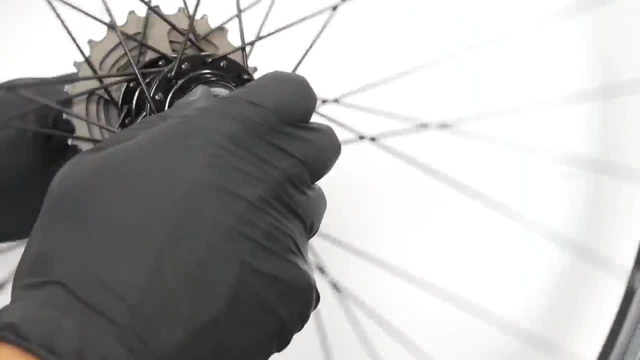 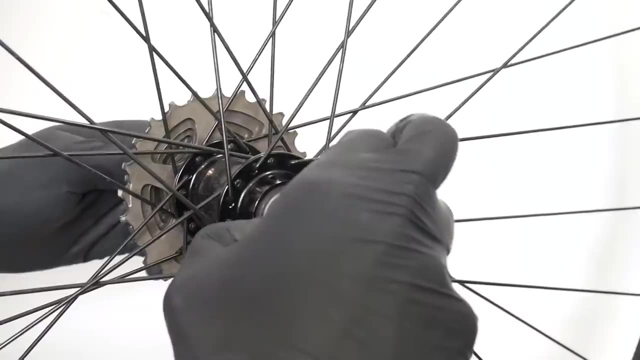 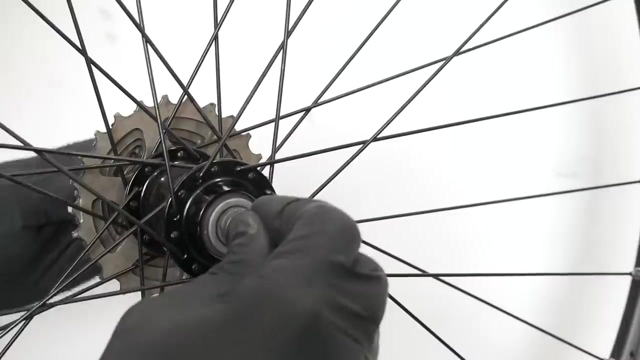 those bearings too much, so that there will be too much friction on the wheel. Right now I feel a lot of resistance here, So once more going back having some play threading this one in. Ok, no play on the hub, Very smooth operation. 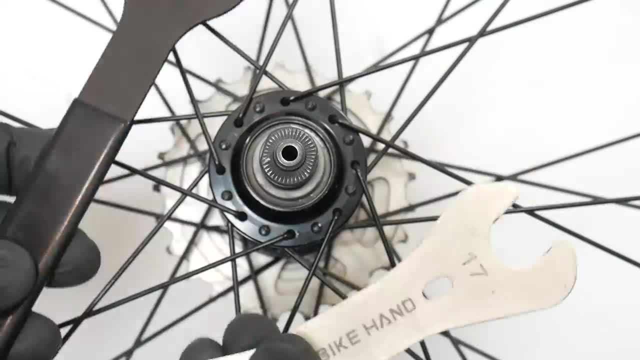 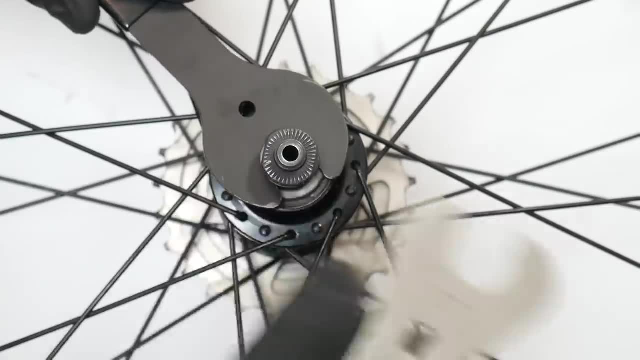 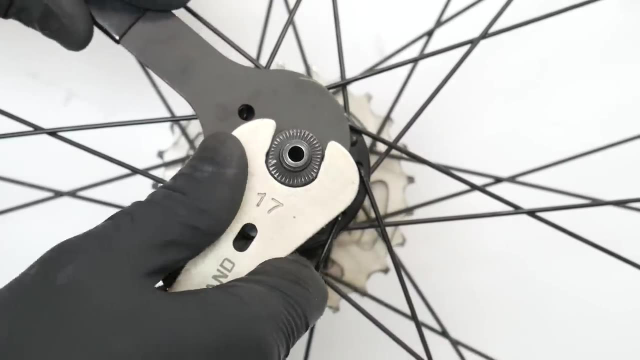 Ready to be assembled. It's time to use our wrenches once more. So 15 on the inside here and 17 on the outside. Sometimes, while threading this nut in, you will see that the axle is moving with it. That means after threading it in, you will probably have once more some play on the hub. 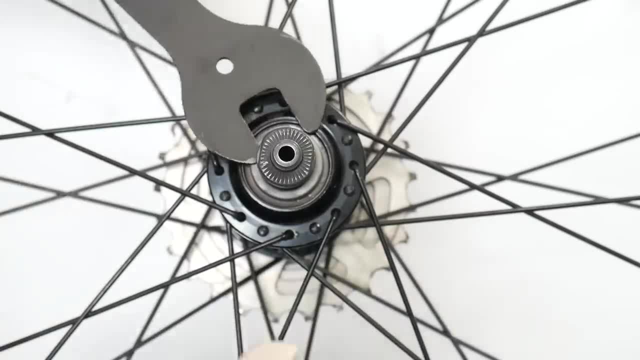 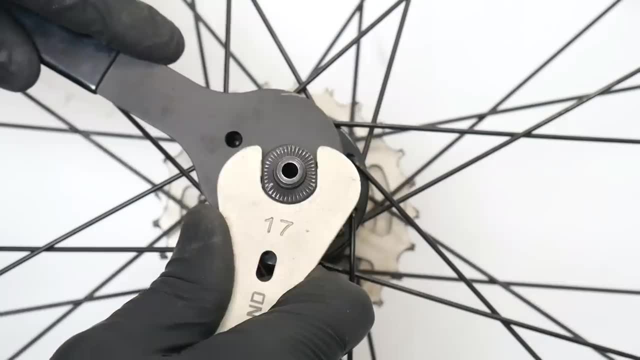 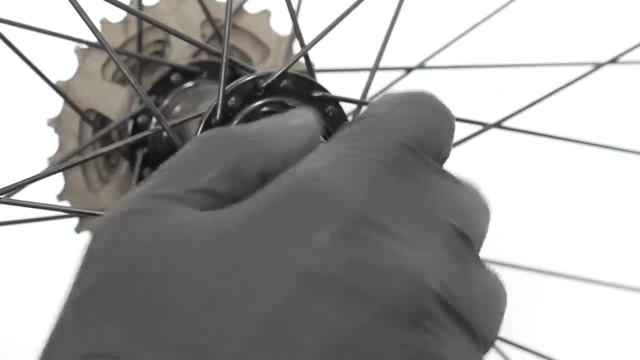 So you just need to be patient and try it just a couple of more times. Maybe you should thread the internal one a bit more And then, after threading the external one, you will have the exact amount of preload on the bearing. Very smooth operation and also no play on the bearings. 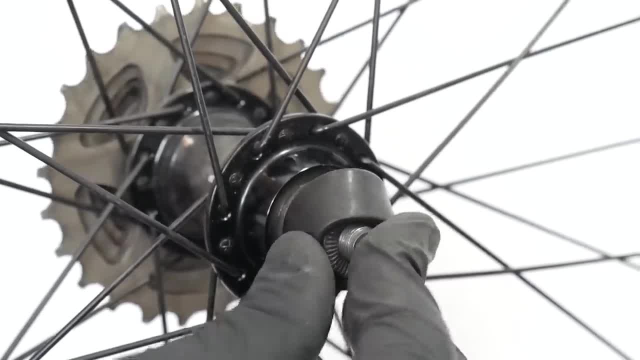 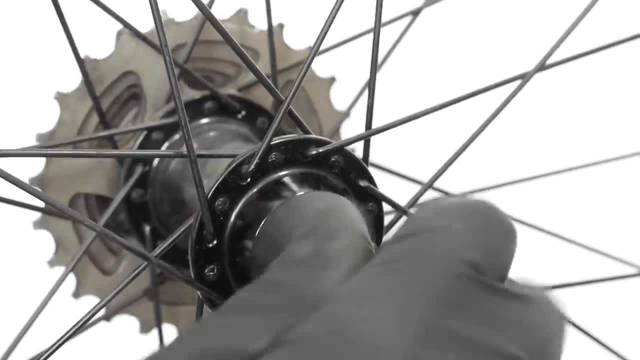 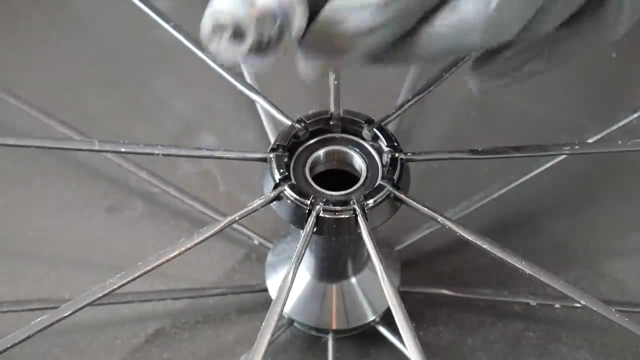 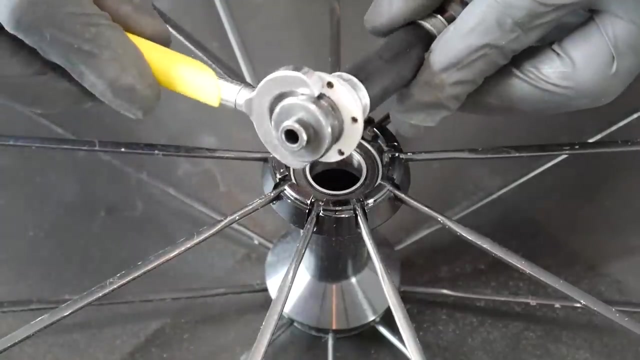 Well done. Of course, the hubs on your bikes can have different systems and different axles. For example, this one, Mavic Crossmax, will need the use of the Allen key on one side and a dedicated key on the other side. So make sure you check out what type of the hub you have before you try to remove anything. 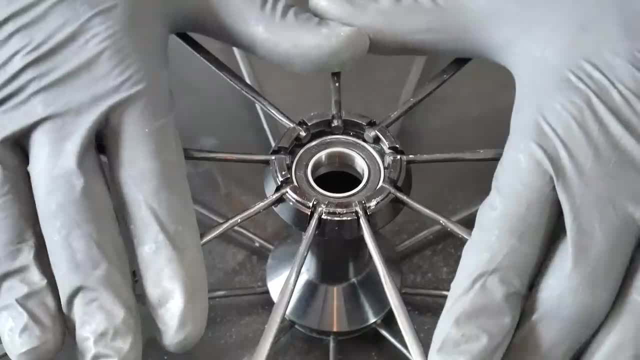 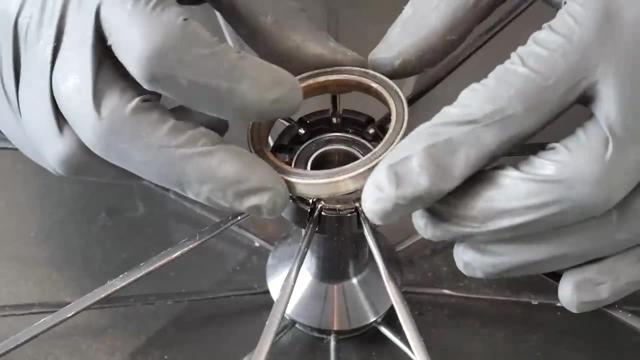 because you might need some special tools for it. You might also have the cartridge bearings on your hubs. How to go about this? You may remove those from the hub, but you will need a special tool for that. And then how to open those and service we are showing in the video. 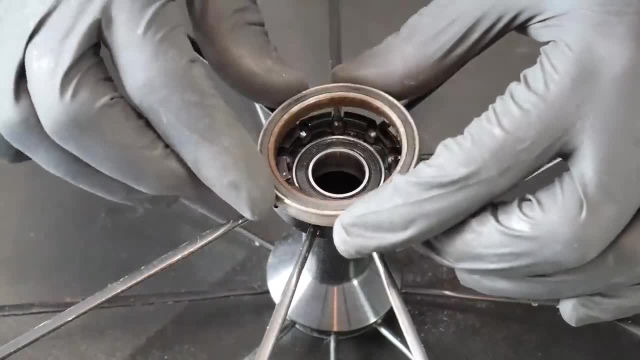 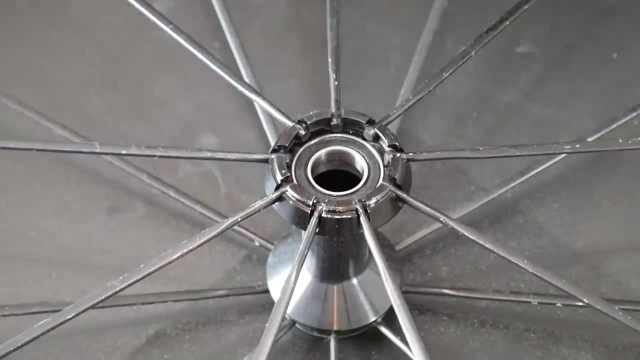 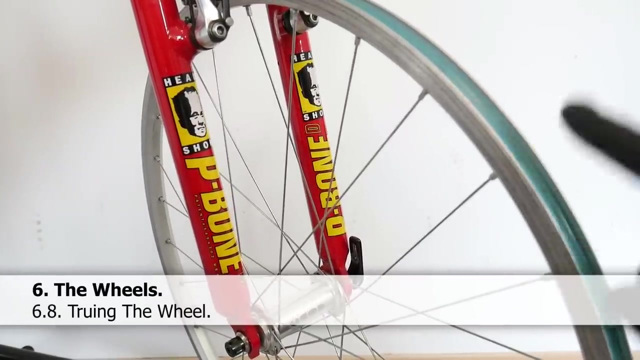 Now some will say you should only replace these bearings. but I do service my cartridge bearings and their lifetime is like thousands or tens of thousands of kilometers- True- in the wheel If we are not fully satisfied with the shape of our rim. I'm gonna give you some basic. 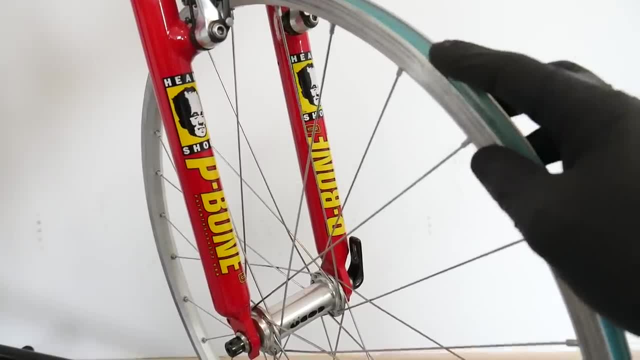 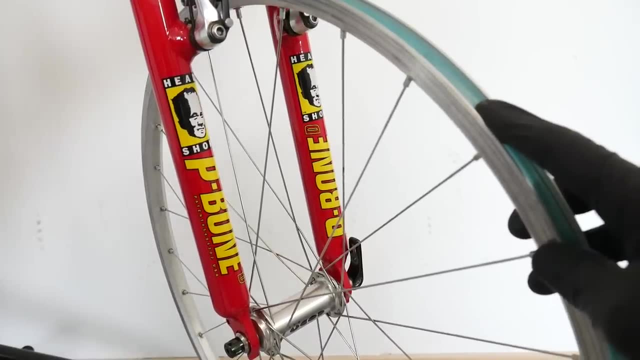 principles which will help most of you to fix the wheel. If you've got some deeper problem with the wheel which is bent, maybe it was hit, there's a link in the description to a whole tutorial about it, So let's see what are the basics. 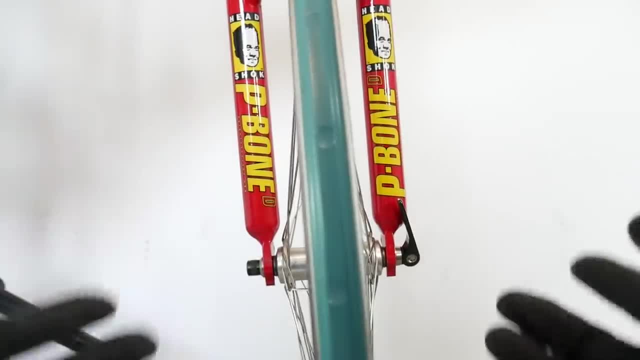 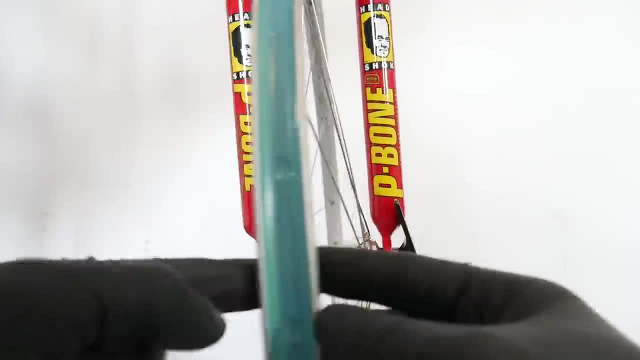 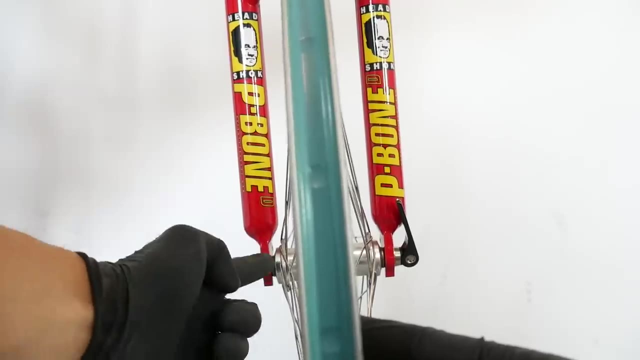 The wheel. truing can be really enjoyable if you know these simple principles. The rim of the wheel is connected with the hub by the spokes. Now some of the spokes, usually the half in their number, will go from the rim to the right flange of the hub, and some will go from the rim to the left flange of the hub. 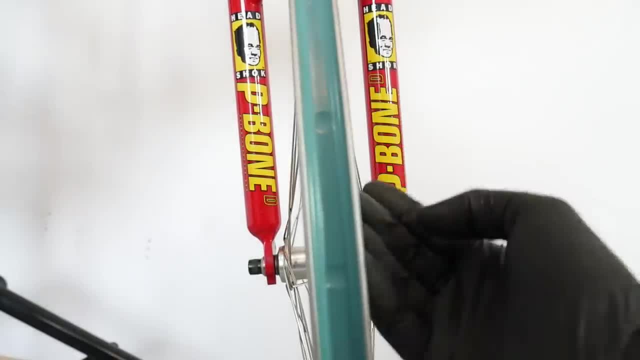 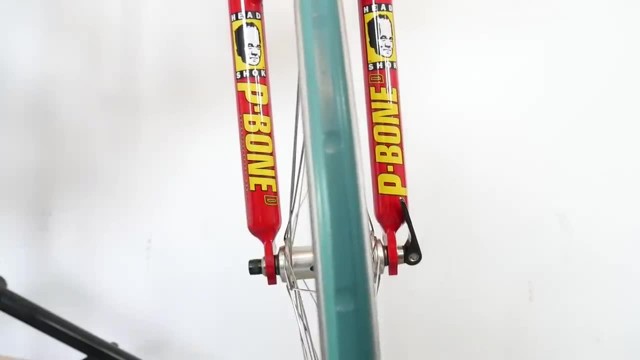 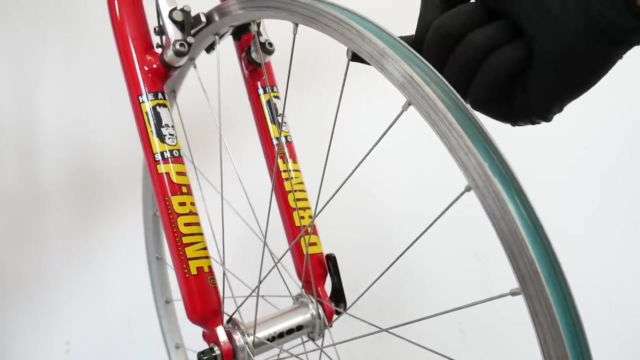 So let's say that the spokes from the left side will pull the rim to the left side and the spokes from the right side will pull the rim to the right side. Now, in order to change the tension on different spokes, we need to use the nipples. 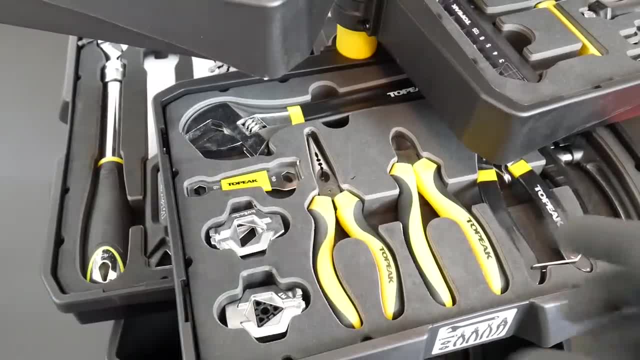 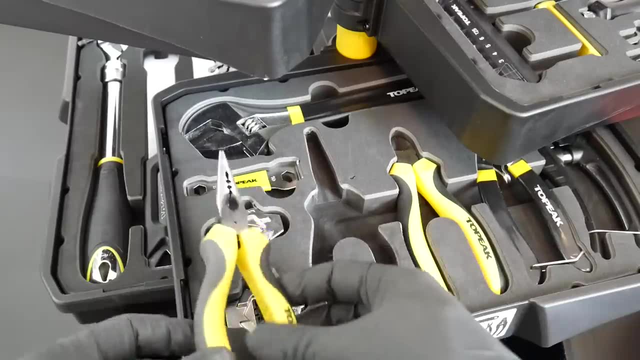 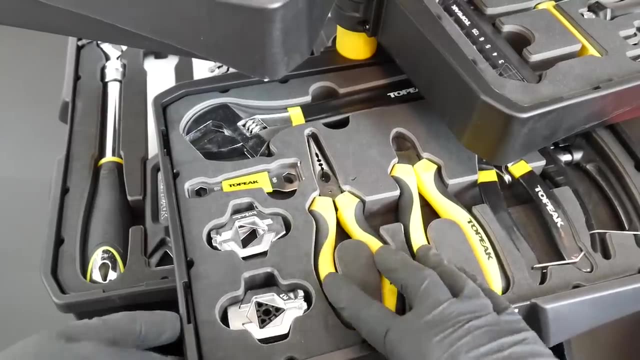 Now we just need a special tool for the nipples In order to true the wheel. we never use any kinds of pliers because we can be almost sure that they will damage the nipples, and then the nipples should be replaced, which can be pretty costly on some fancy wheels. 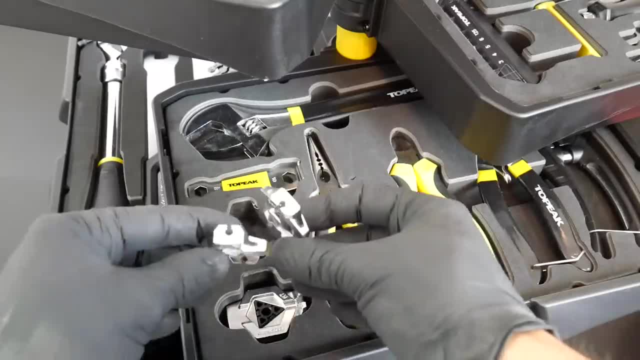 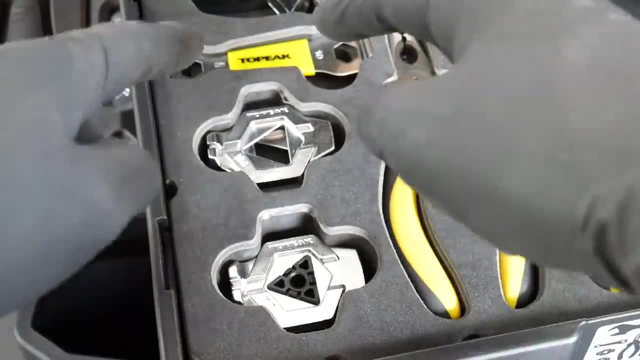 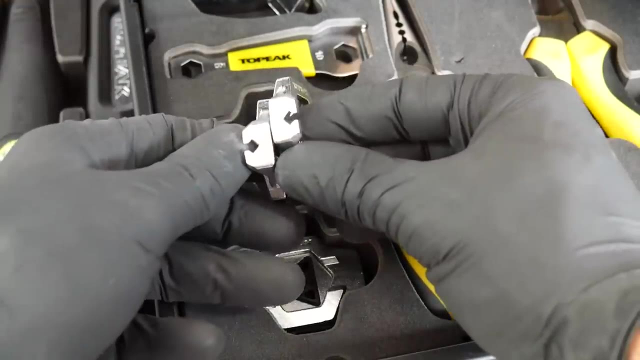 So this kind of tool should fit the type of the nipples we have on our wheels and also the size of it. Here we have different types and different sizes of the nipple tools. For example, here you can see the standard nipples in four different sizes and this one. 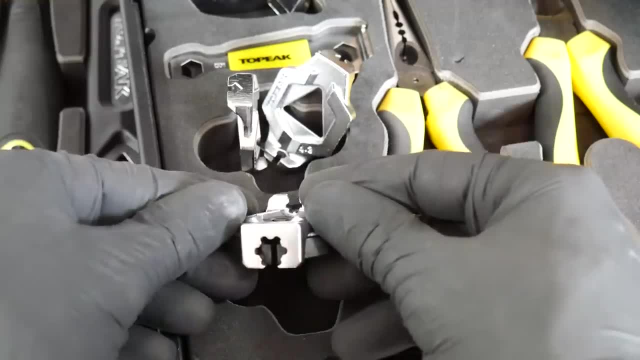 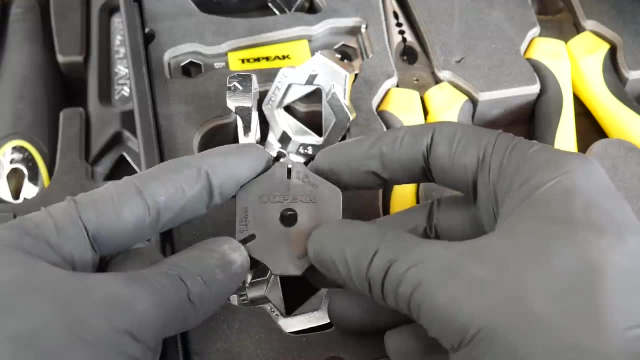 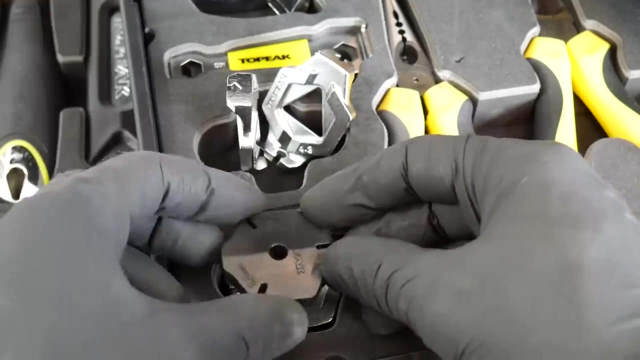 is specifically designed for some of the Mavic wheels. You can also use, in addition to that, a tool for holding the spokes. If we have bladed aero spokes in different sizes, you can use this one to hold it while you manipulate with the nipples. 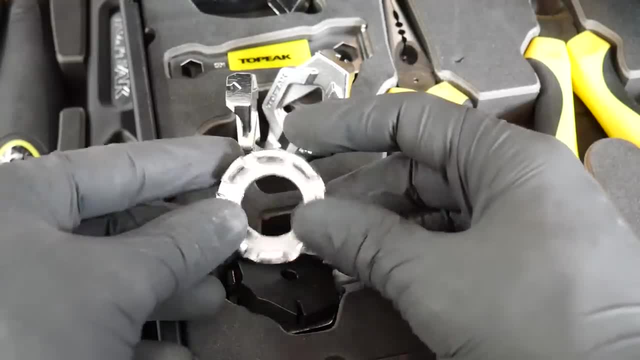 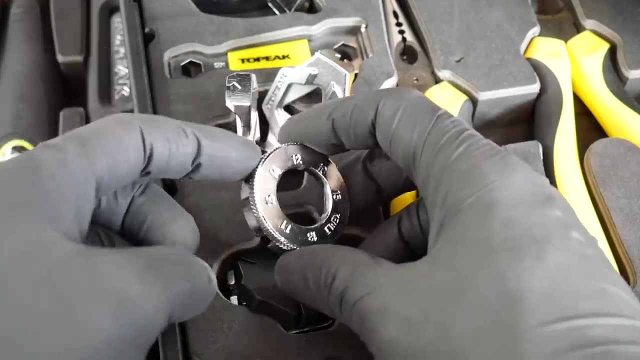 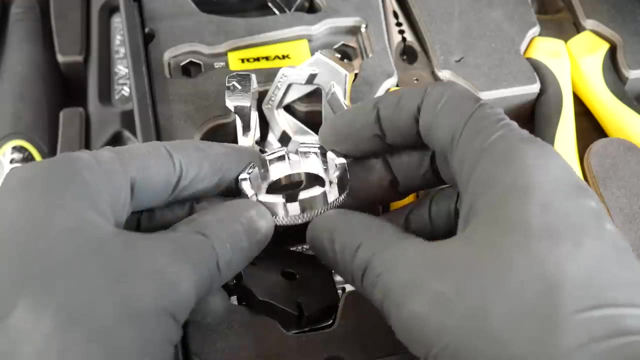 You can also buy such a kind of tool which has many different sizes. I would not maybe buy the cheapest ones, because those cannot be that accurate and can also damage the nipples, But something just interesting In the mid range of the price would be very good choice. 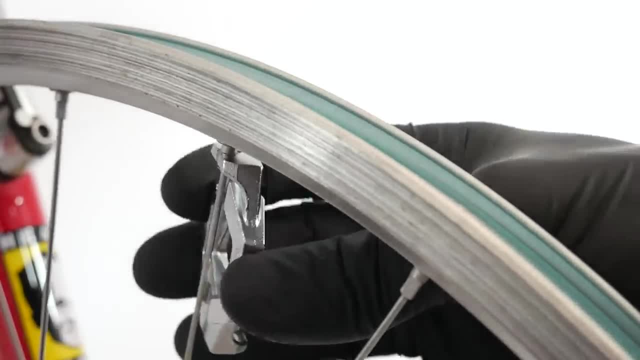 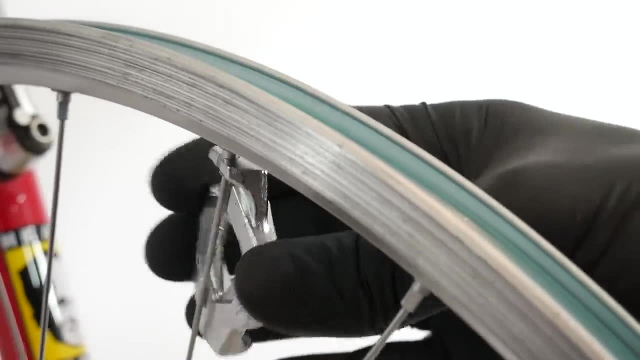 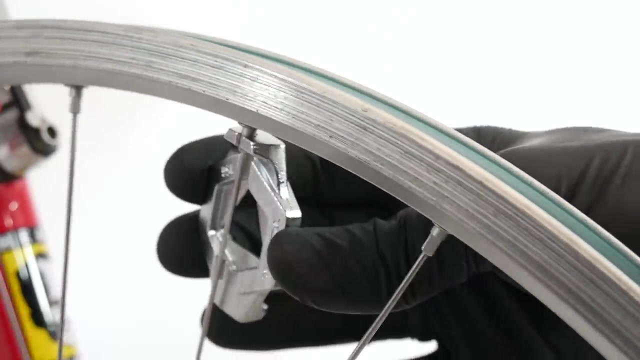 Let's find the right tool for our nipples. This one doesn't fit. This one doesn't fit at all. We've got two left. This one still not the best for the nipples. This one fits and we're gonna use this one for withdrawing. 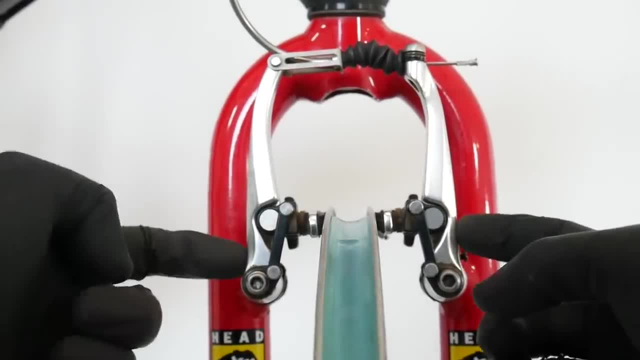 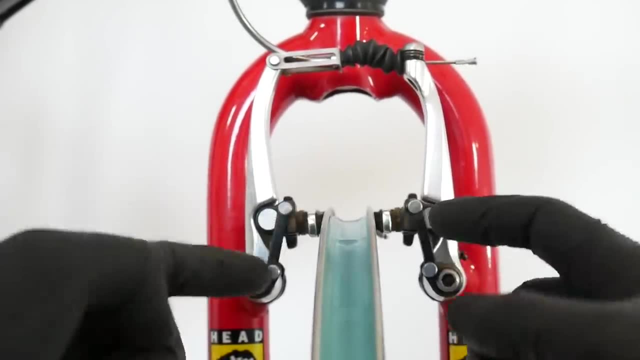 We can finally move on to the truing On the caliper brakes. On the caliper brakes, we can use the barrel adjuster in order to decrease the distance between the braking pads and the rim, so that we will hear when the rim is moving in any. 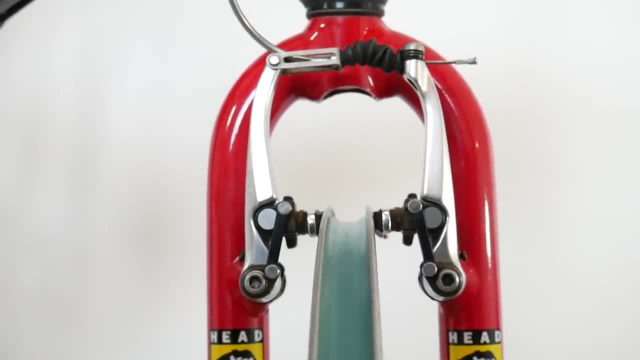 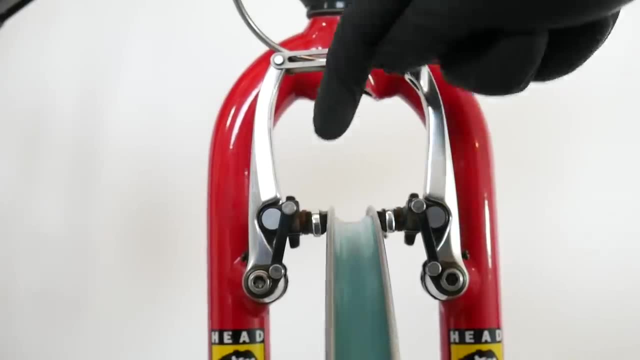 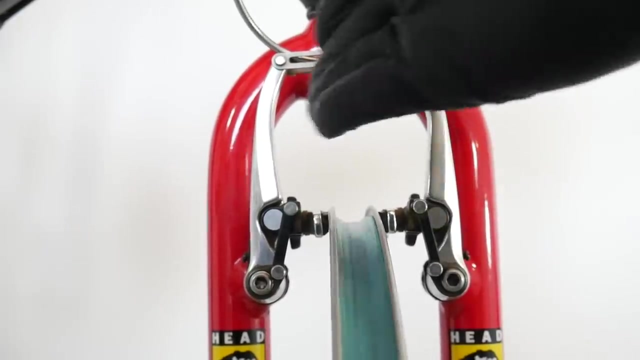 direction. Let's try it. I'm unthreading the barrel adjuster. We start to hear it. That's it The right one. the right braking pad is rubbing against the rim, so the rim goes a little bit to the right. 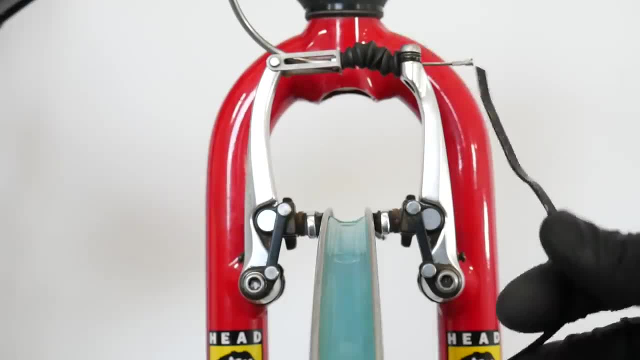 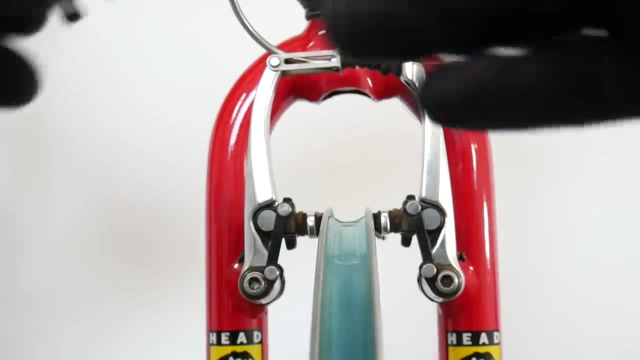 If your bike is spec'd with the disc brakes, you can simply use the zip ties. by assembling those to the blades of the fork, One can indicate the side to side movement and the other one, if you set it just above the edge of the rim, will indicate the up and down movement. 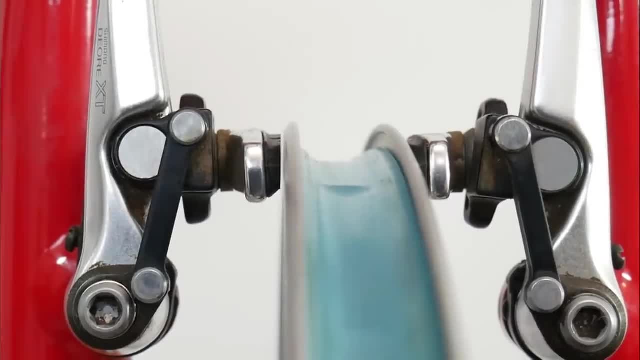 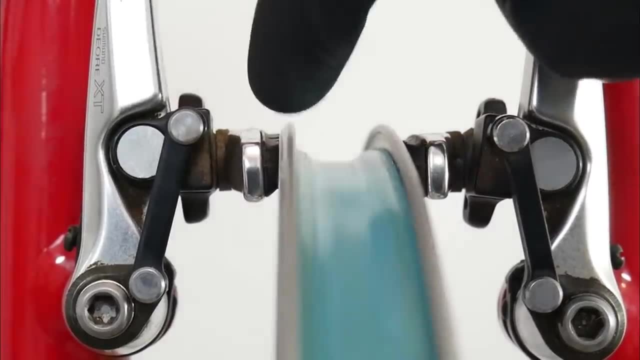 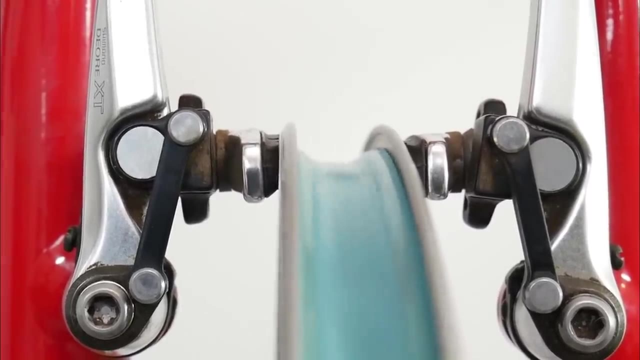 Pretty clever. All right, first off, we need to find out what part of the wheel we want to fix. Okay, the camera is set so that you can see this little distance between the braking pad and the rim, And you can see the wheel moving right here. 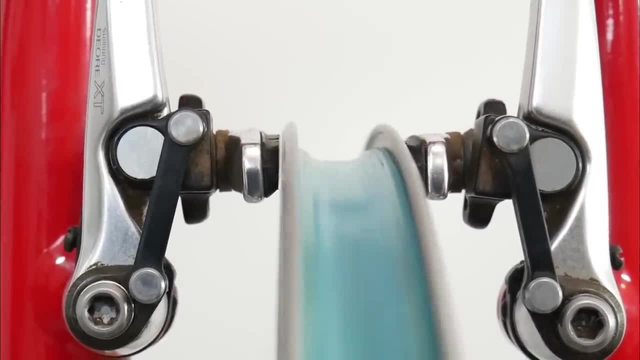 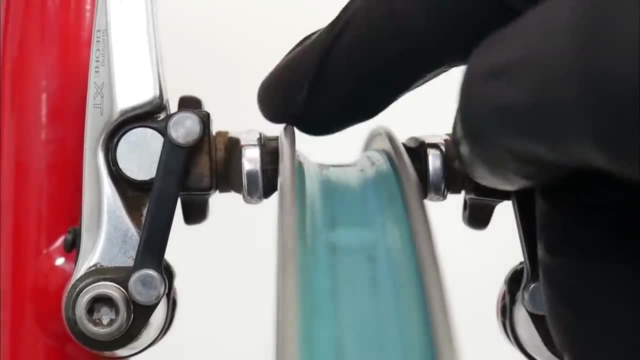 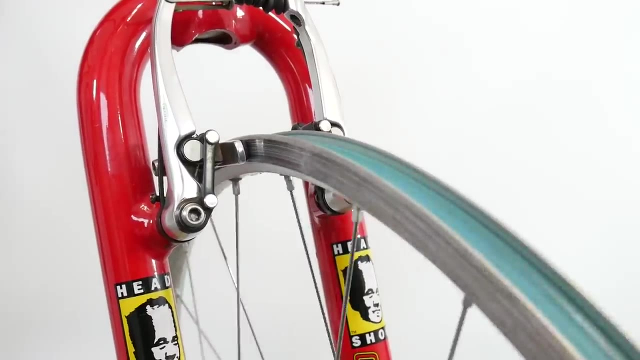 No distance. Yeah, so that's where the rim is rubbing against the braking pad. That's exactly here. So that's the place we want to fix. Let's look at the wheel from another perspective. That's exactly where the rim is touching the braking pad. 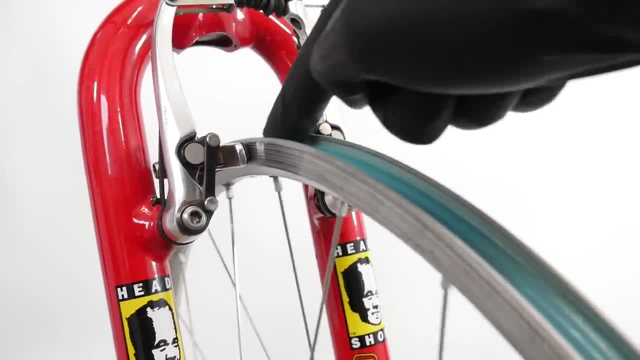 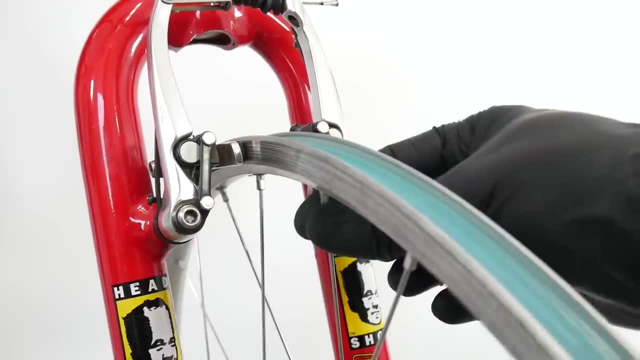 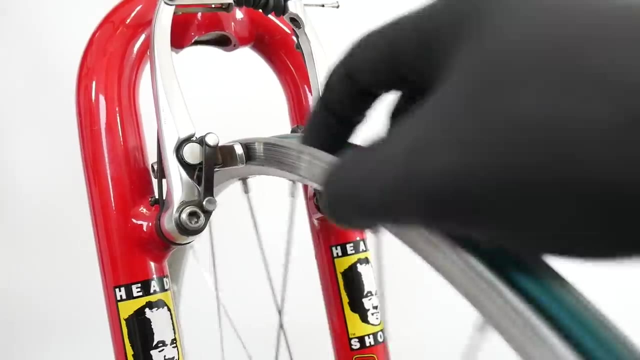 On our left side, And so we want to increase the tension on the spokes on our right side- It's the bicycle's non-drive side- and decrease the tension on, perhaps, these two spokes. We're going to see how it goes. It's not a huge one, so we're going to do it very, very gently. 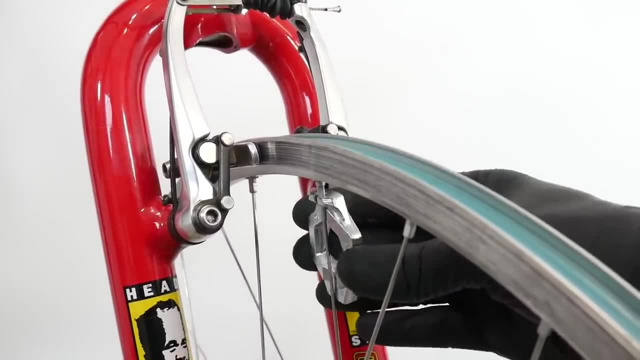 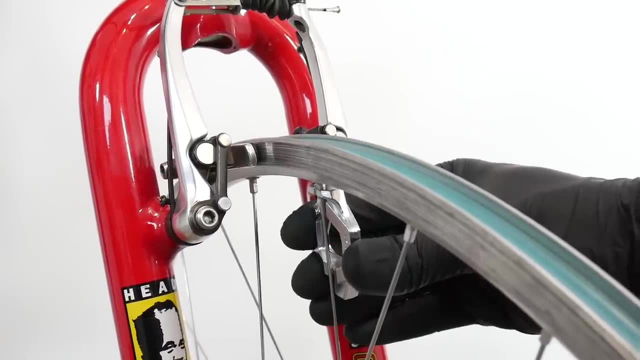 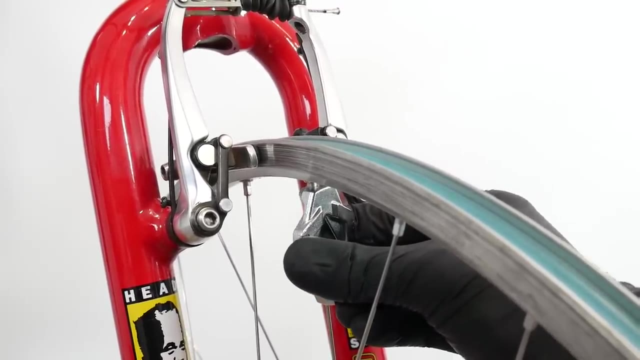 What I'm going to do right now is to use my tool, and now I'm going to thread the nipple on the spoke, Increasing the tension of the spoke just by, let's say, not more than 90 degrees, maybe 70 or 80 degrees, like this: 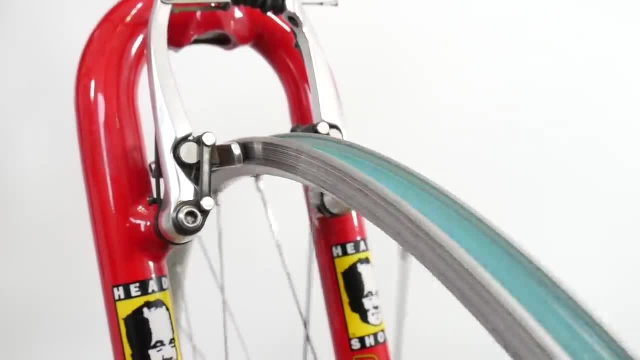 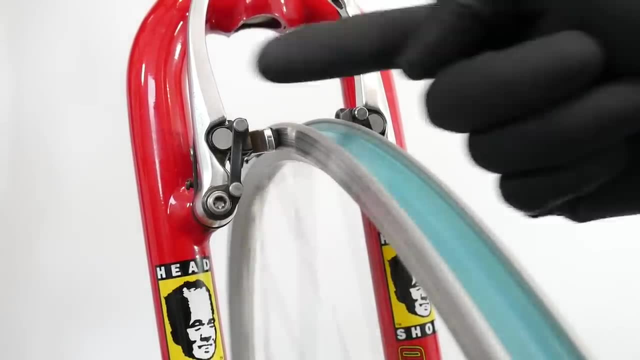 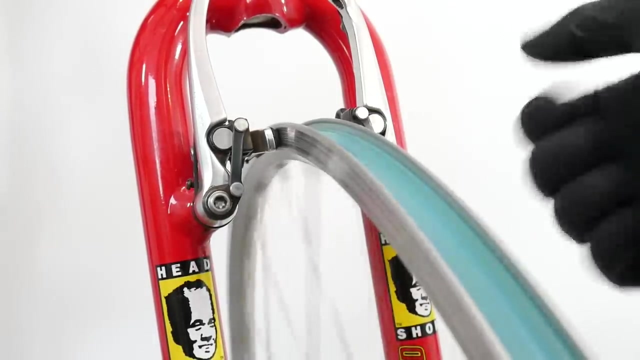 And see the reaction. Okay, no rubbing here. These are the basic principles of wheel-throwing. You know now that when the rim is escaping into one side, you want to increase the tension on the spoke on the other side so that they will just pull the rim into their side. 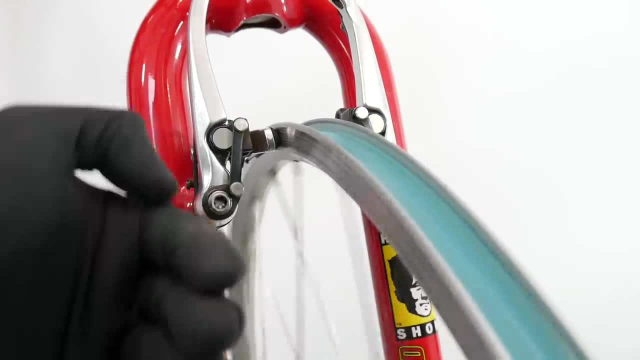 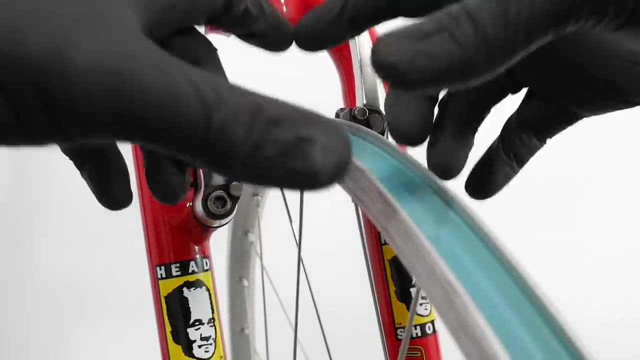 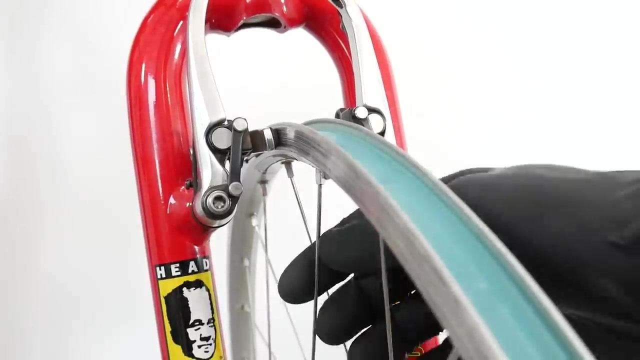 Or also decrease the tension on the same side into the rim is escaping. We were working on some small problem. You should also know that while we are working on some area of the rim, the other area can also change its shape. So make sure you always look at the whole wheel, check out the tension of those spokes. 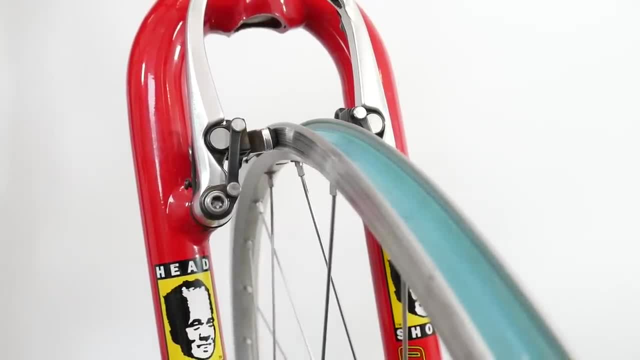 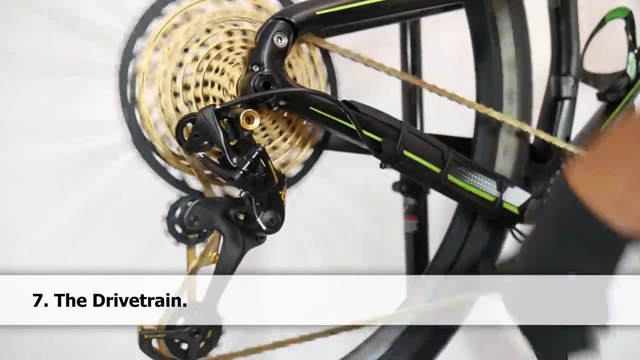 And if you need some further help, you can just watch our whole episode about wheel-throwing. Duralers on our bike have to provide a smooth and nice gear change. If they don't do their job properly, this will be very annoying for us. 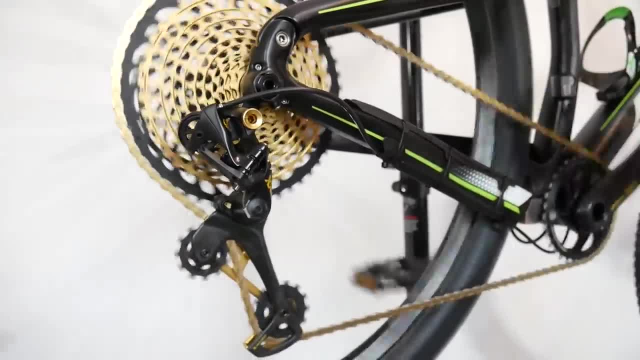 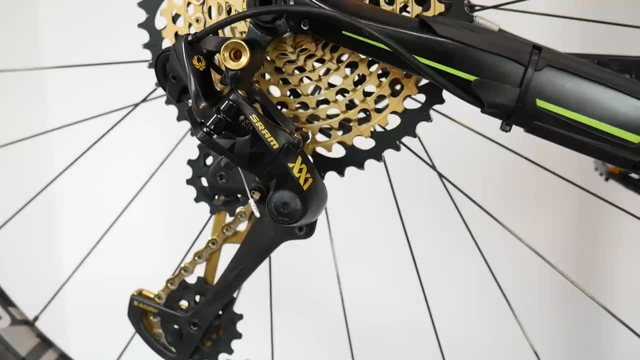 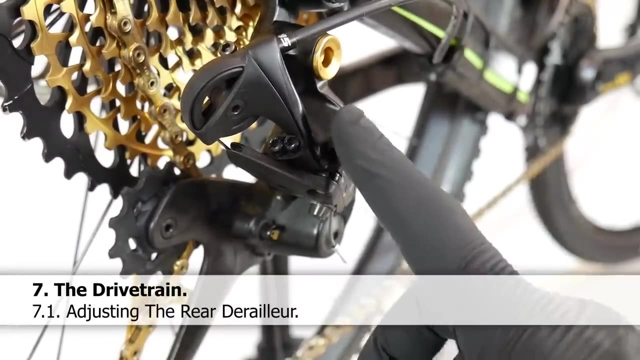 It will make our ride much more difficult, especially off-road, And also it can cause a chain snap. Let's see first what kind of adjustments are available on most models of the rear duralers. The first adjustment we want to make after replacing the duraler or the cable are the. 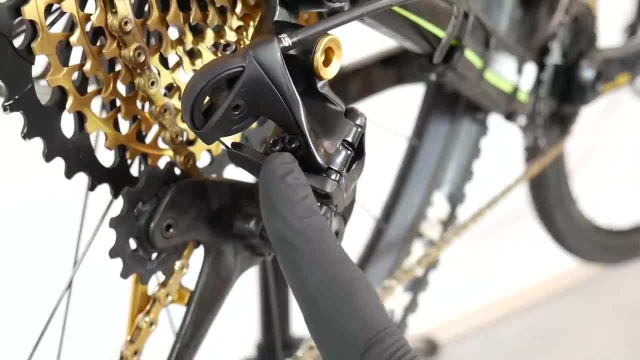 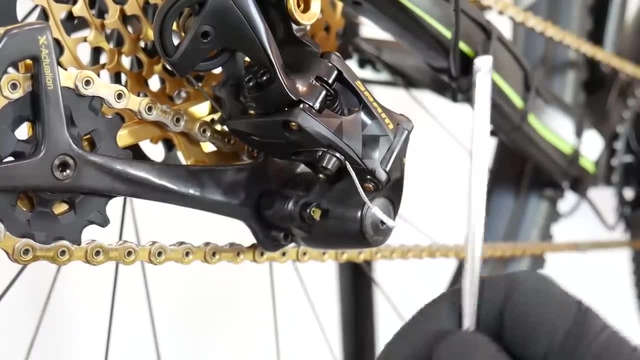 limiting screws. One is for the highest gear and the other one is for the lowest gear. In order to correctly adjust these two, I'm going to release the cable In this way also. I'll be sure that on the highest gear it will be the limiting screw. 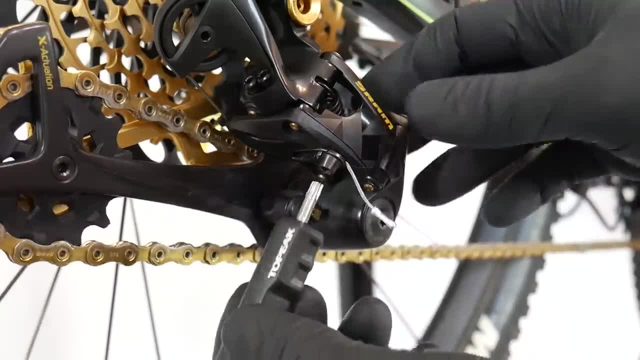 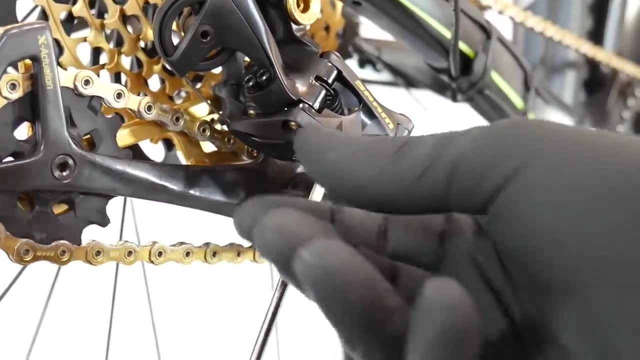 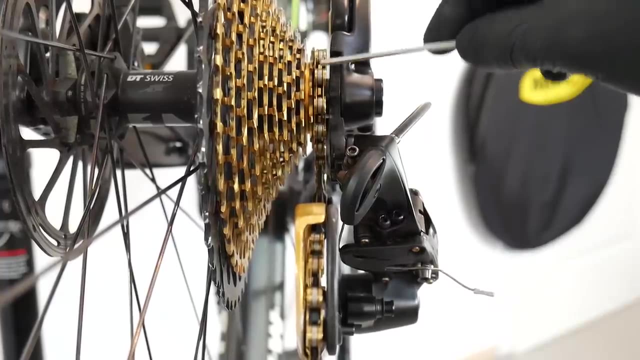 and not the cable tension that will stop the duraler. Let's adjust the limiting screw for the highest gear right now. This screw will allow the chain to come out, And this screw will allow the chain to come out. And this screw will allow the chain to go to the highest gear, but not further meaning. 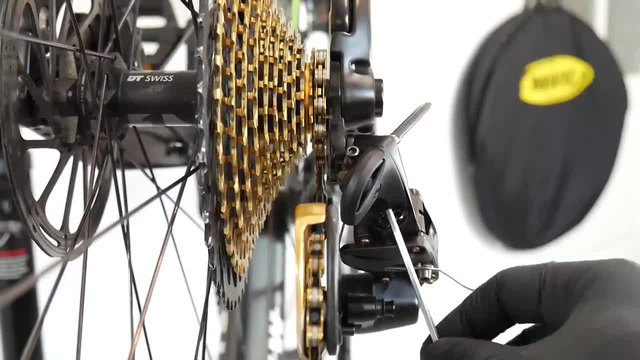 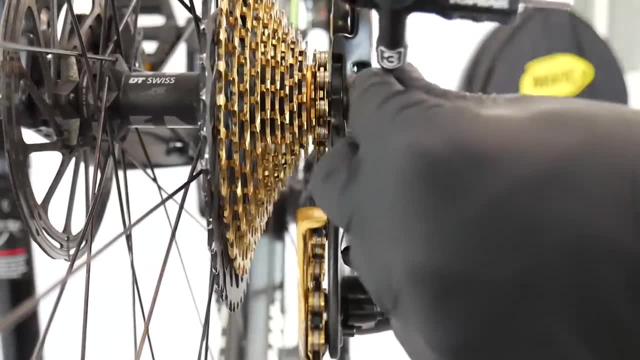 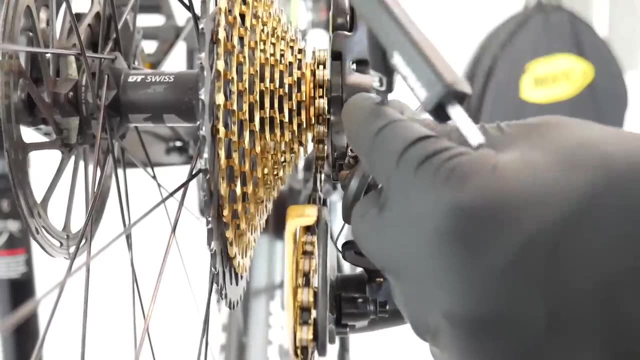 between the frame and the cassette. On some duralers it will have the symbol H, which means high, highest gear. Let's see what happens when I'm threading this one in. As you can see, the cage of the duraler goes inwards, so to the lower gear. 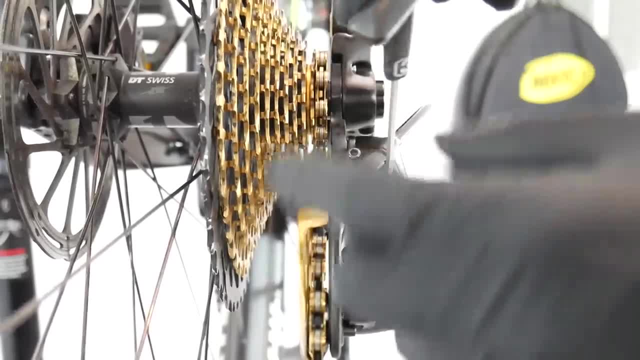 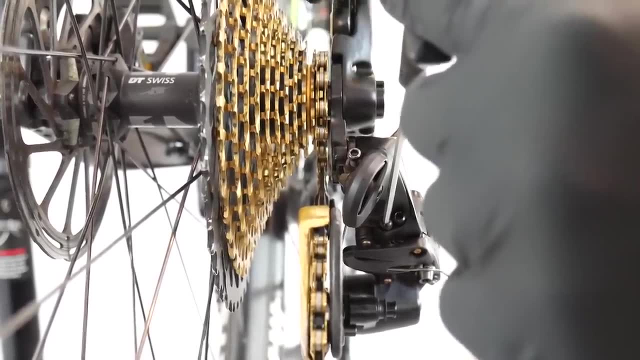 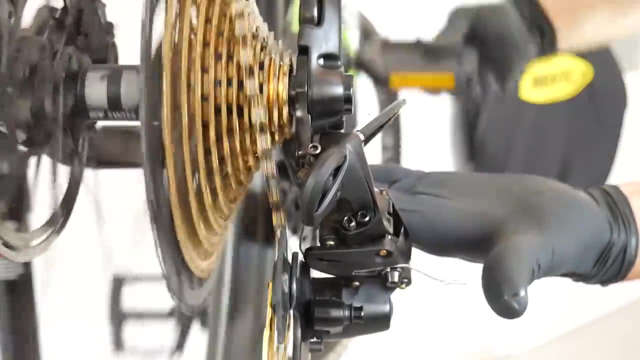 And how should this one be set? It has to allow the duraler for the easy gear change to the highest gear, But not further. so not further, not between the frame and the cassette. Let's check it out. Seems to be perfect. 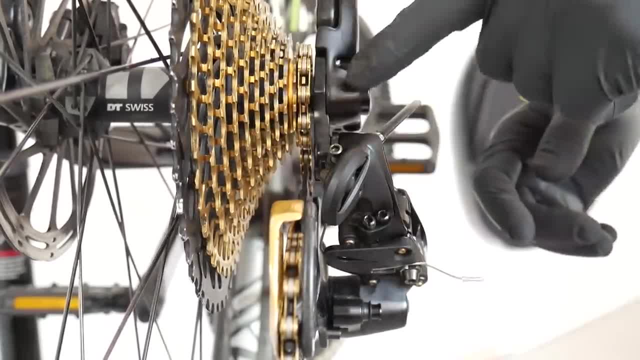 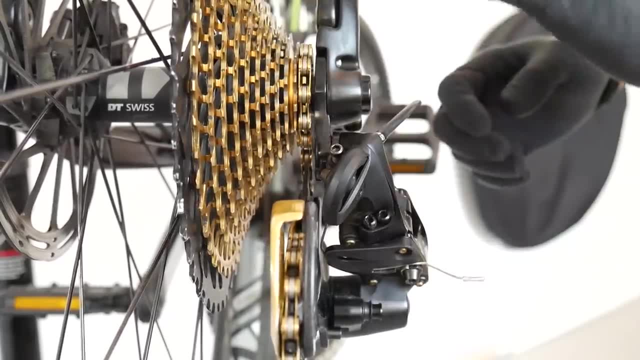 Many bike mechanics will try to set the upper pulley of the duraler not in line with the highest gear, but a little bit further, just a little bit. That means that the duraler will jump from here from the 11th to the 12th gear easily. 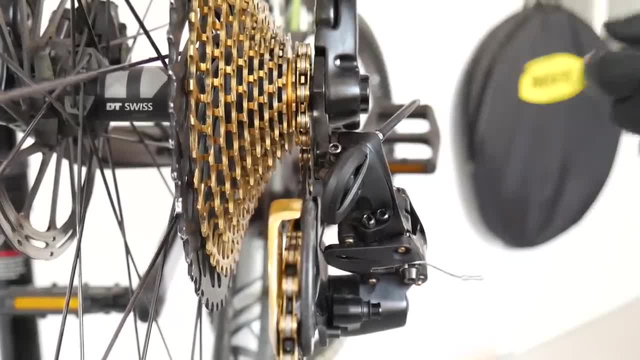 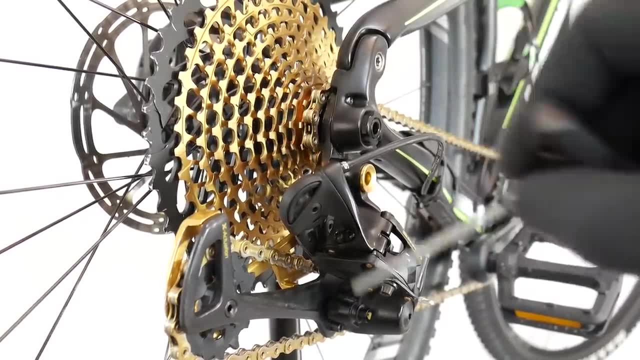 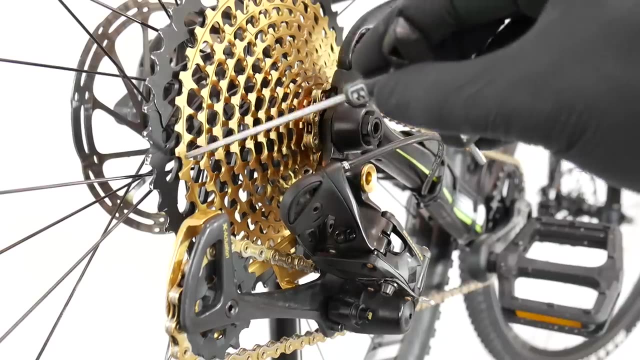 but still, the chain will not go any further. Now it's time to adjust the low gear limiting screw. so might have the symbol L. The principle is exactly the same and pretty easy. If the duraler has hard time shifting from the second to the first gear, we will be unthreading. 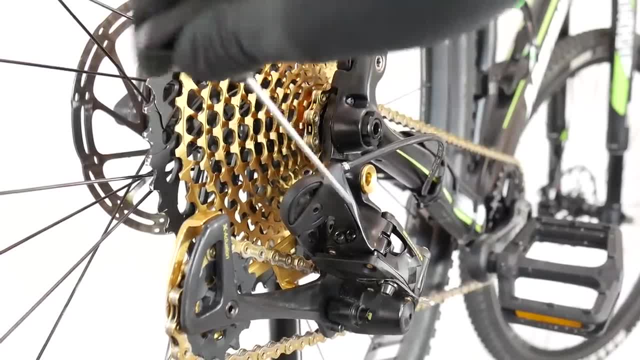 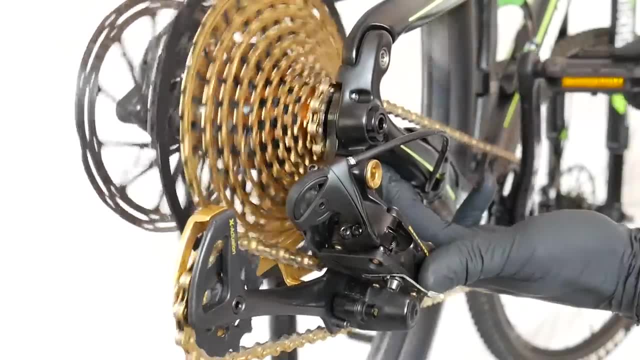 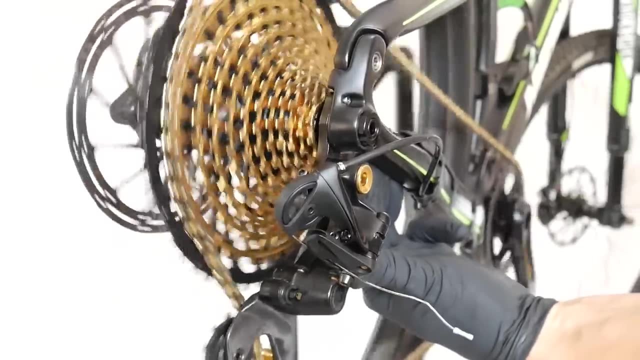 this one so counterclockwise, And if the chain will be able to go in between the cassette and the spokes, we will be threading this one in. Now we're checking out the lowest gear And, as you can see, the duraler doesn't want to shift into it. 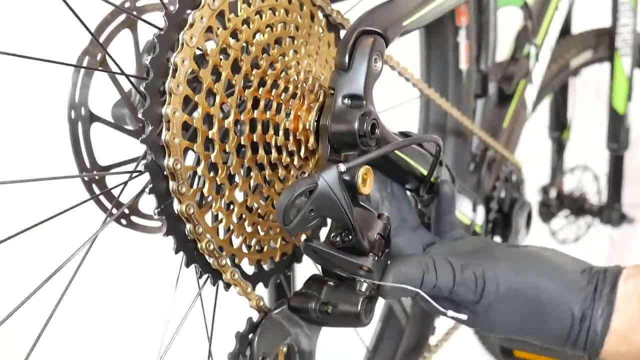 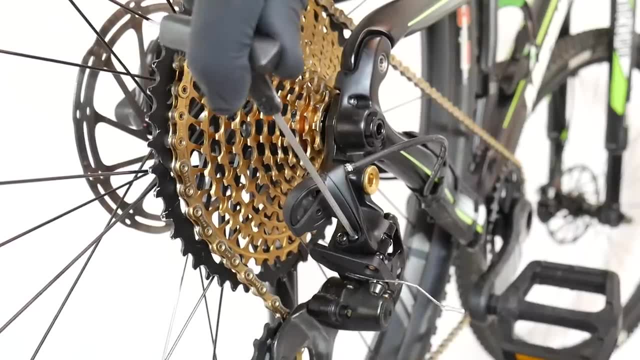 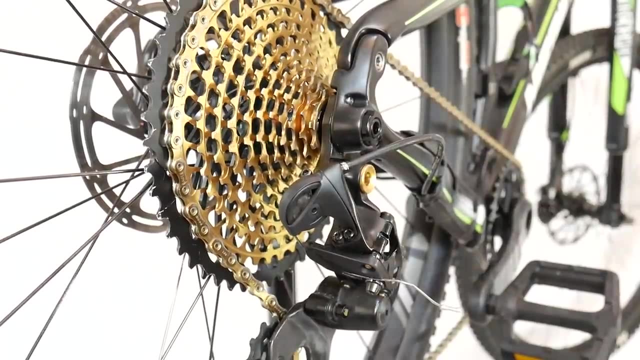 Hardly. no, it won't do it. That means we need to unthread this bolt, And normally this adjustment means maybe unthreading by 15 degrees or so, but I've really made it bad so that you see how it works. 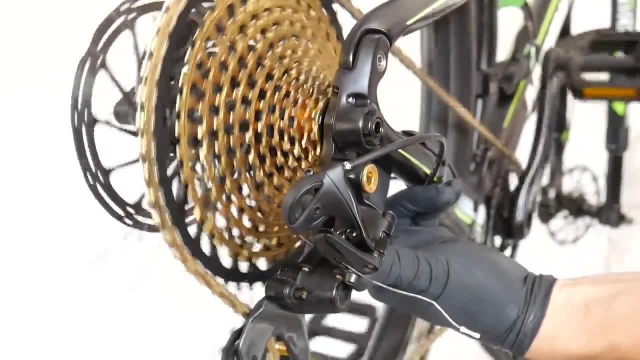 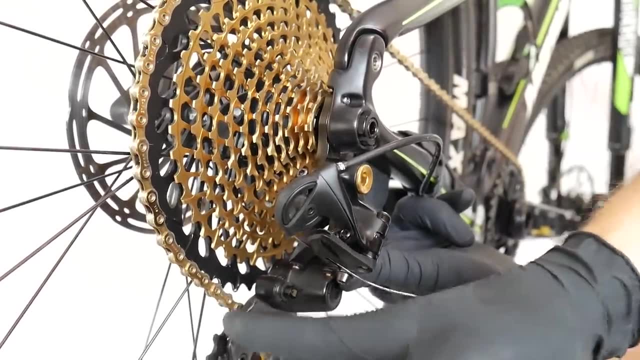 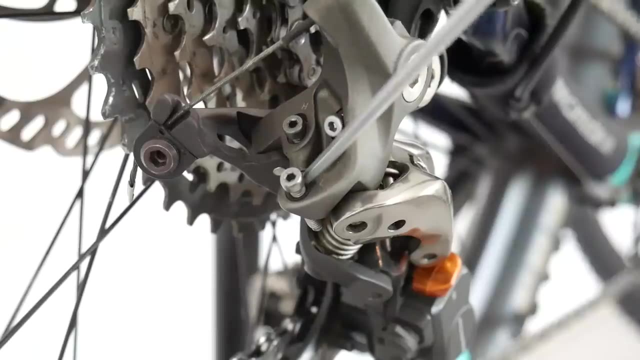 Okay, It seems to work just fine, So I'm unable to push the chain further, but I have the lowest gear, the first gear, so it's okay. This is how these limiting screws can look like on other duralers like this one, Shimano. 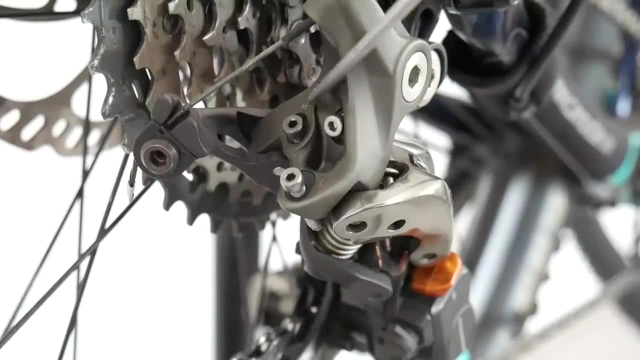 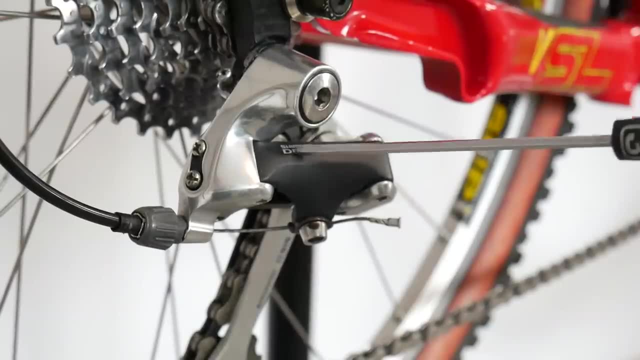 XTR M9000.. In this case, we do have these symbols: H for high and L for low. Here is the 20 years old Shimano Dura XT M9000.. Okay, And we have the same exact two limiting screws with the H and L symbol. 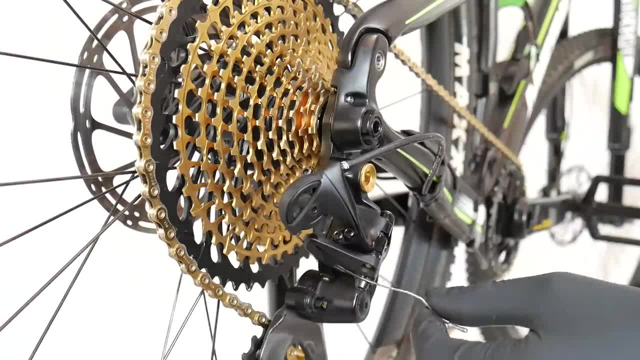 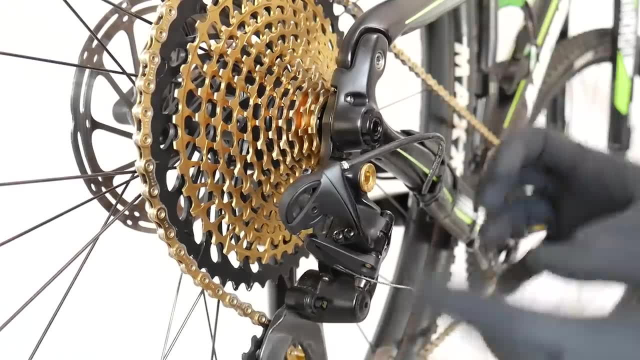 Just one additional piece of advice. After you are done with everything like mounting the cable and adjusting the tension of the cable, you might need to tweak these two just a little bit so that you are really sure that changing the gear to the lowest and to the highest is really smooth. but the chain will. 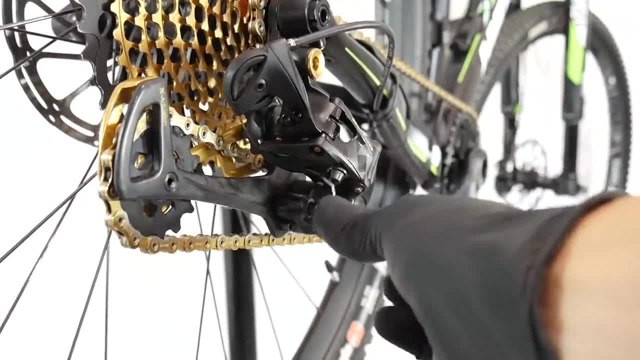 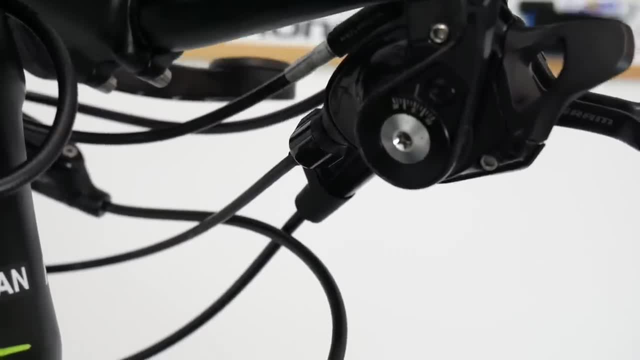 not go any further. Now we're going to fasten the cable of the duraler and adjust its tension. Before we fasten the cable, though, it is good to look at our barrel adjusters. Those could be just at the shifter or at the rear duraler, or both. 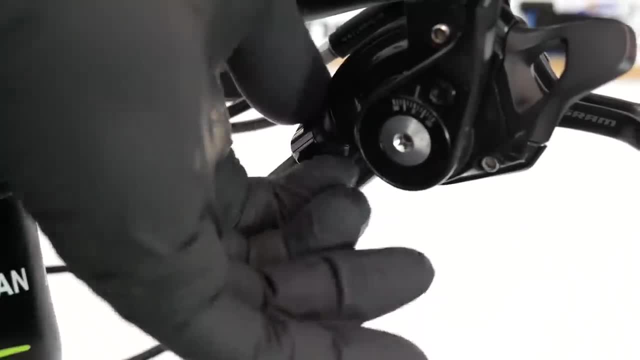 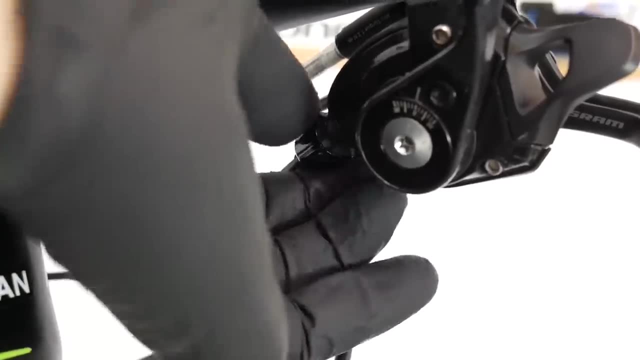 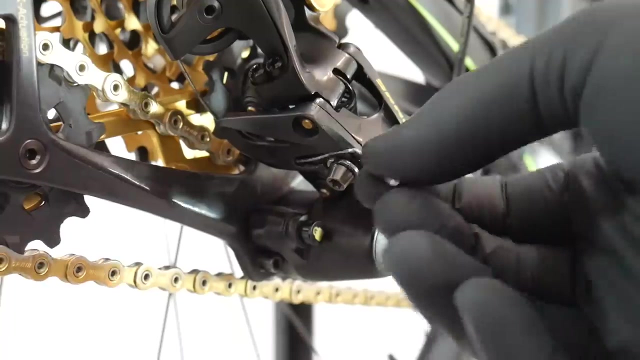 I would set those to the zero position like this, and then maybe unthread those by two turns so that we'll be able to change the cable tension both sides, increasing it and decreasing it. First off, I need to find out how the cable should be fastened. 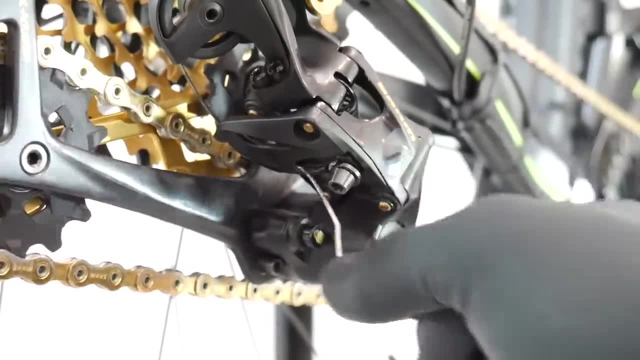 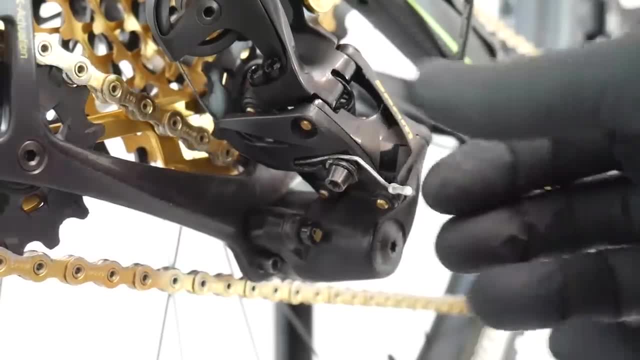 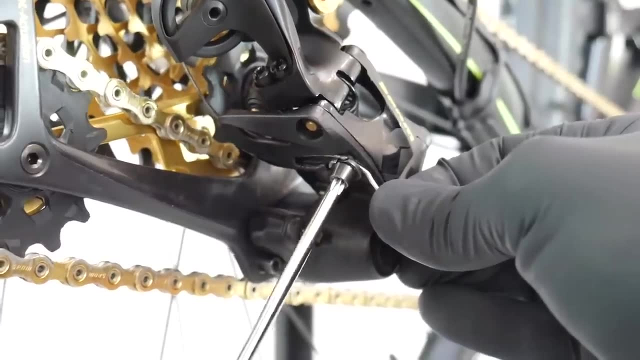 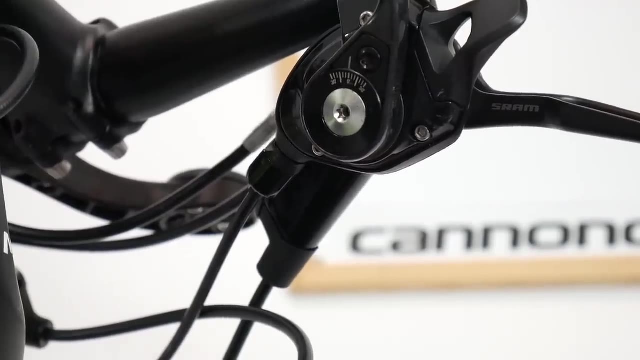 Then we want to make sure that all the housings are in place, and now I'm just pulling the cable a little bit and fastening the bolt. Now we need to learn how to operate this barrel adjuster, and it's also very easy. When unthreading it, we are increasing the tension on the cable. 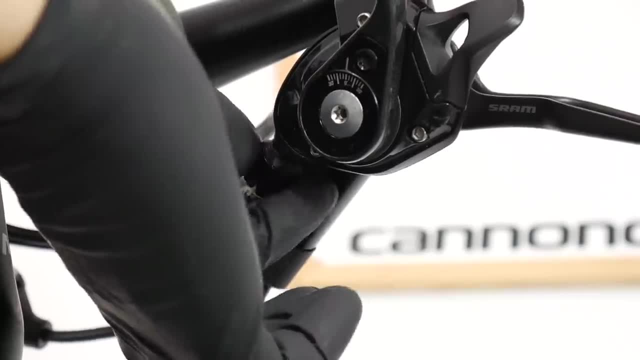 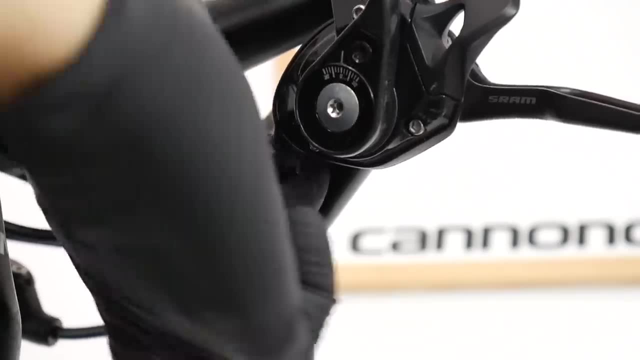 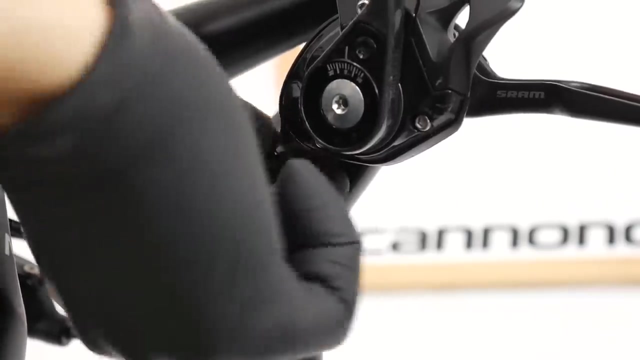 so the derailleur will be easier going up the cassette from the highest to the lowest gears. And when I'm threading this one in I'm decreasing the tension of the cable so that the derailleur will be more willing to go down the cassette from the lower to the higher gears. 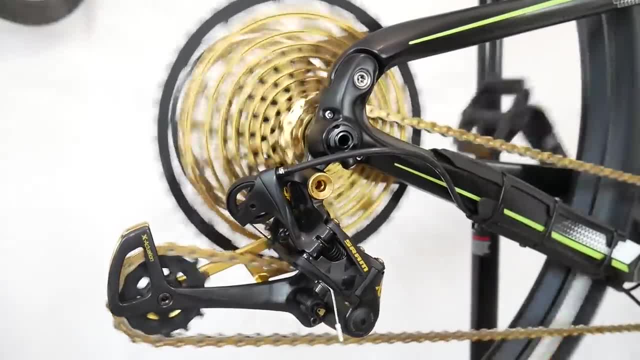 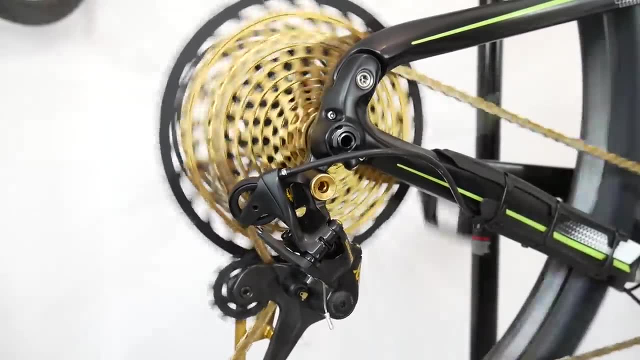 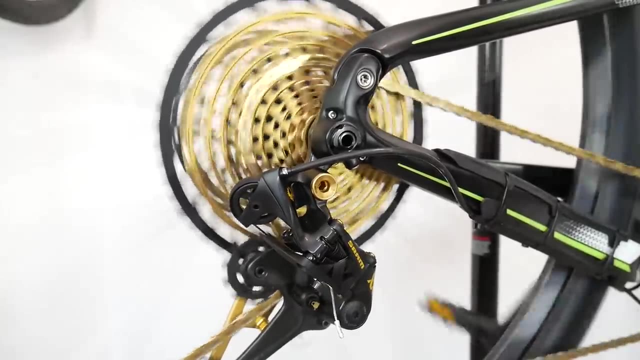 And let's just make one short exercise. We are trying to shift both ways on the cassette. Shifting up the cassette goes very easily, even a bit too fast, and down the cassette, so shifting to the higher gears doesn't work properly, It doesn't work at all here. 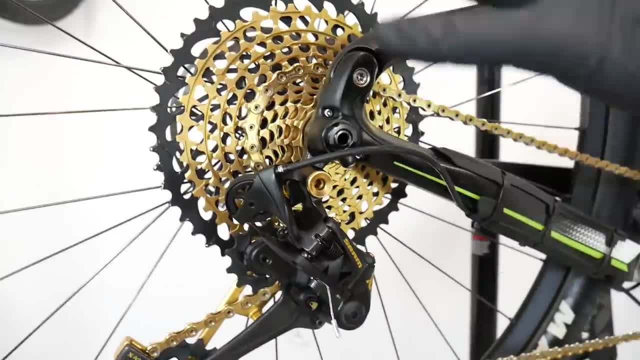 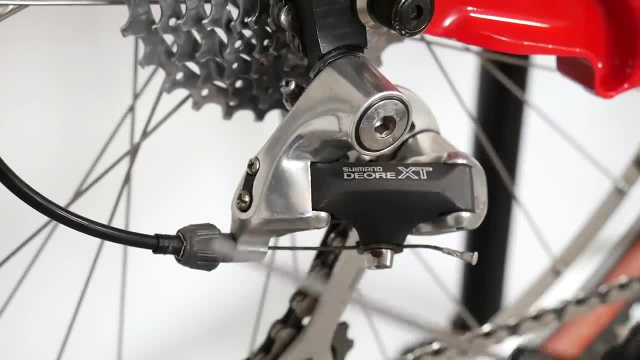 What it means. It means that the cable tension is too high and we need to thread the barrel adjuster in. Here is the barrel adjuster situated just by the rear derailleur on the old Shimano Diora XT. Let's see how it worked. 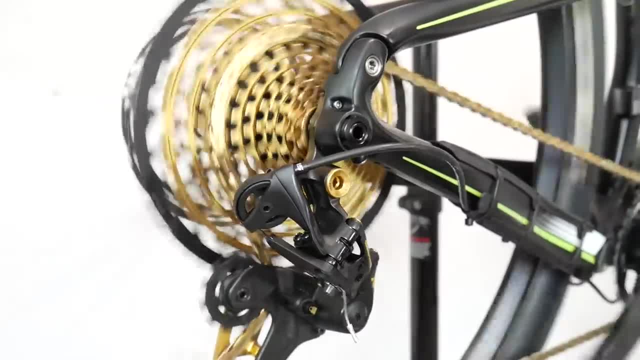 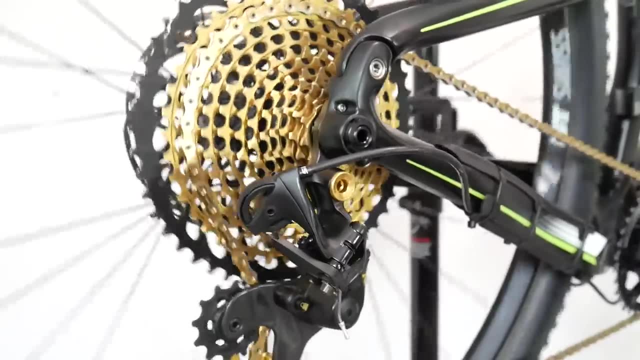 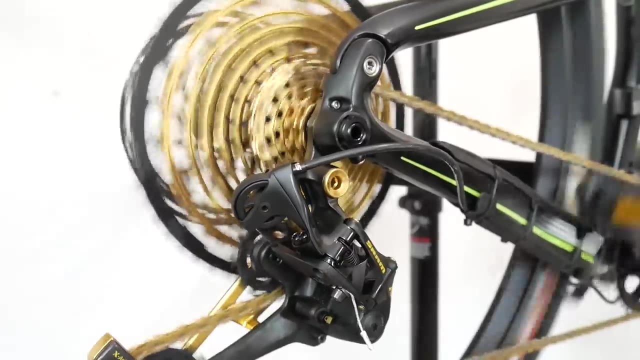 Shifting up the cassette called downshifting because we are going to the lower gears very smooth And also silent. we don't hear any clicking noises. Okay, upshifting to the higher gears very smooth. I'm happy with this, very, very good. 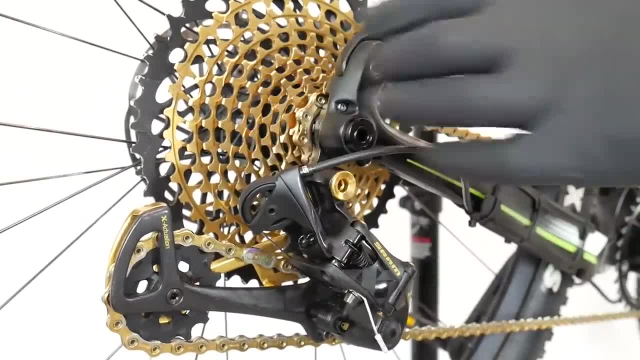 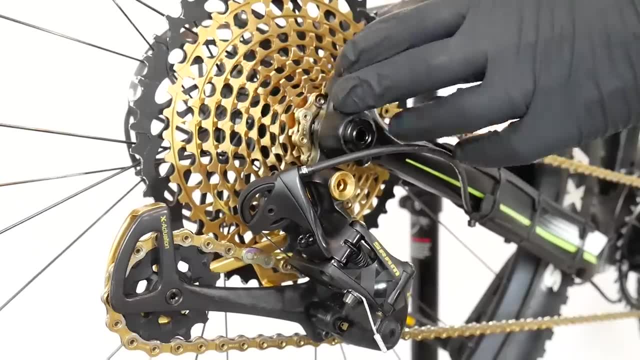 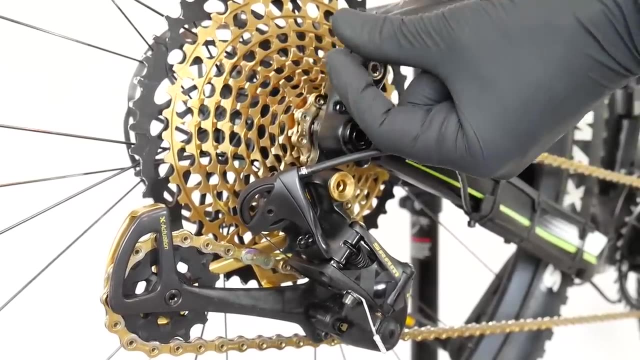 Of course adjusting the gears on the new drivetrain with the new chain and super clean cables is very easy, But it should be done in different phases. So with each phase we're gonna turn this barrel adjuster by really maybe 10 or even five degrees. 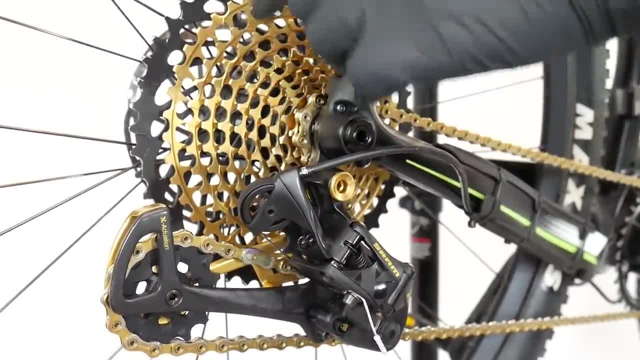 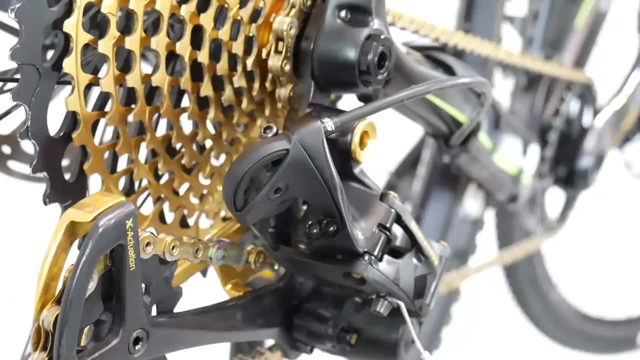 so that we find the right spot on each gear for the derailleur. And now there's just one little bolt left. Let's see it. We already know these two. These are the limiting screws: the H and L high gear and the lowest gear. 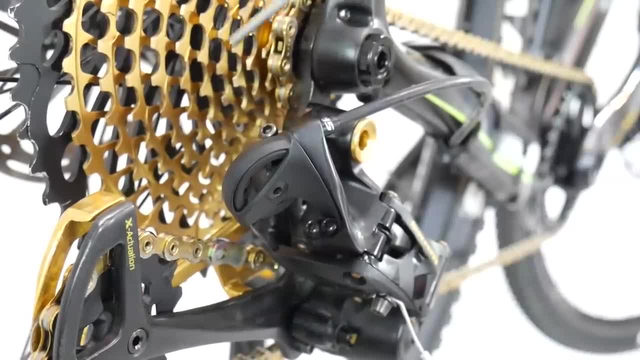 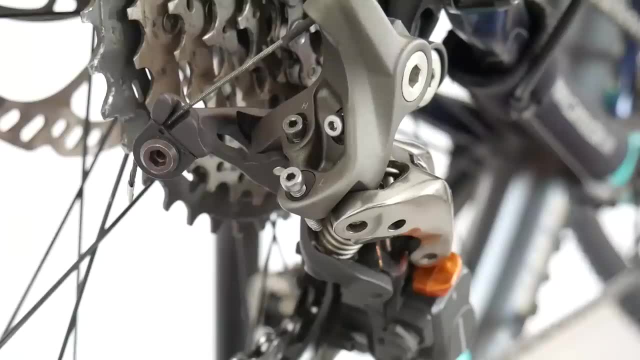 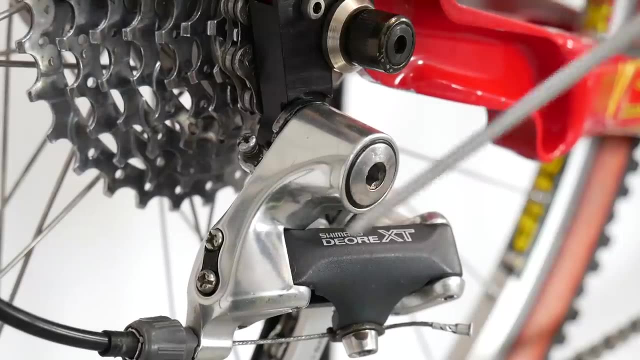 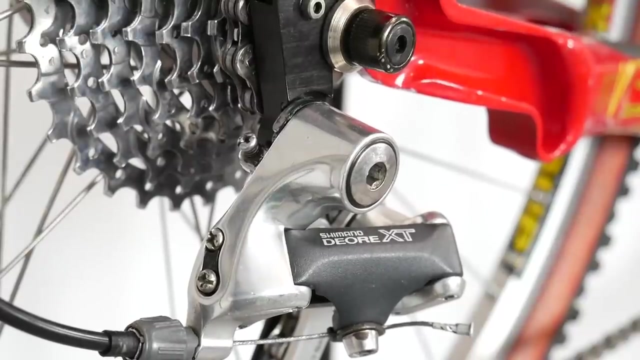 But this one here. that's the little screw which will adjust the distance between the upper pulley of the rear derailleur and the cassette. Here is how this little screw is situated on the Shimano XTR-M9000 derailleur And once more we've got the 20 years old rear derailleur and there is also this kind of adjustment almost in the exact same place. 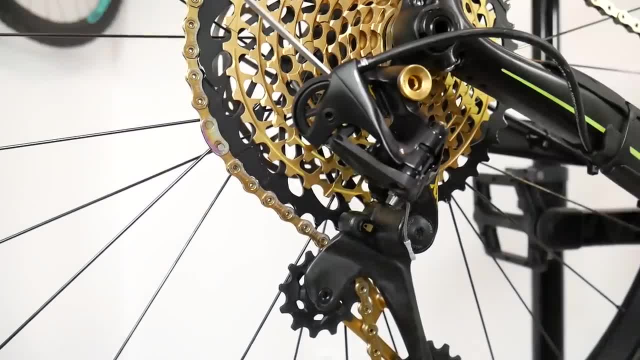 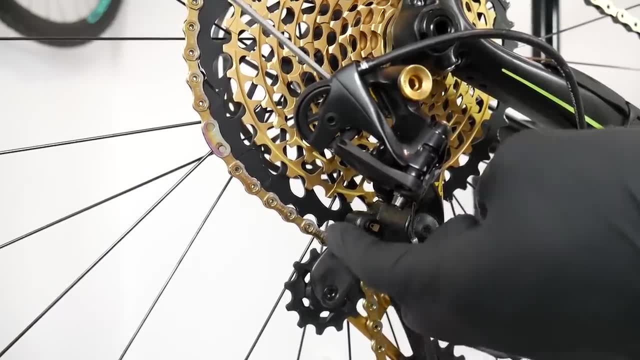 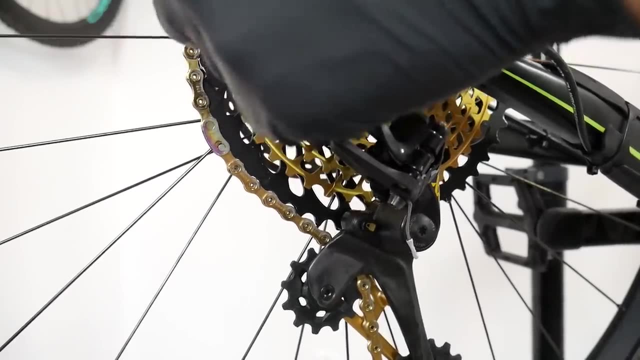 Let's see how this one works. I am unthreading the bolt. Pay attention to the upper pulley, to the guide pulley. The distance between the guide pulley and the cassette is lower now. Now I'm threading this bolt in and the upper pulley goes away from the cassette. 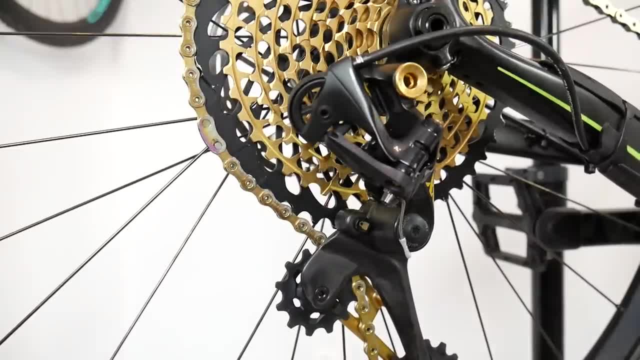 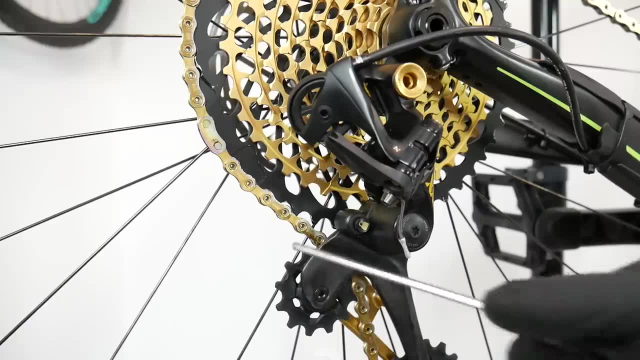 The question is how to adjust it and what should be the distance between the pulley and the cassette. You should be paying attention to the manual because the different models of the derailleurs will require different distances here. but I would say it also depends a lot on how long cage you have of the derailleur and what's the range of your cassette, how many teeth it has. 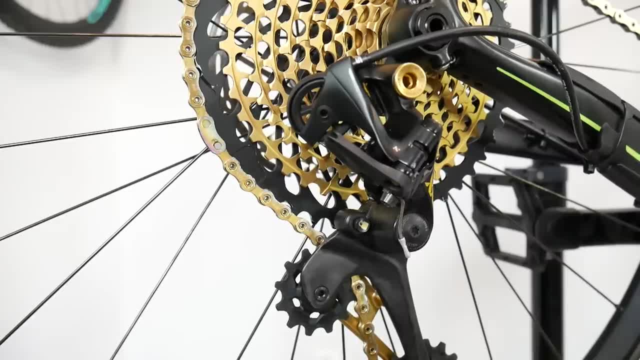 So my principle here is to check out whether the gear change from the second to the first gear, so to the lowest gear, doesn't feel stiff, and I try to set this distance as small as possible. If it's too small, then you will feel stiff. 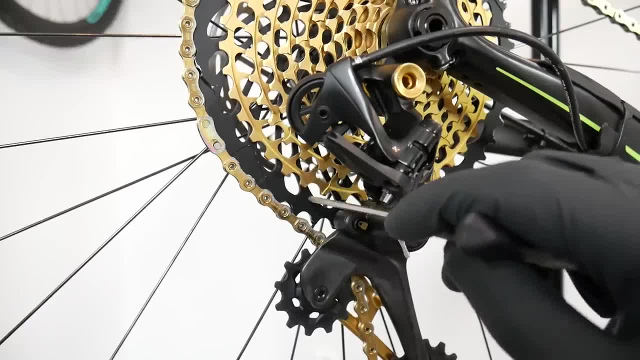 If it's too small, then you will feel stiff. You will also feel stiff gearchange from the second to the first gear, Maybe even from the third to the second. But as long as it doesn't feel stiff, it's smooth. 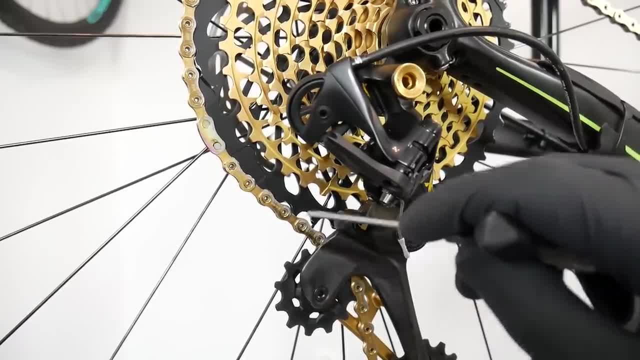 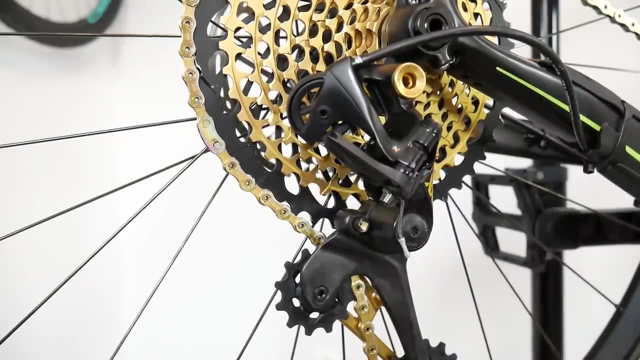 I will be trying to keep my upper pulley as close to the cassette as possible, because then the gearchange on other sprockets will feel just faster. If you already know how to adjust the reed derailleur, the front one shouldn't be a problem. 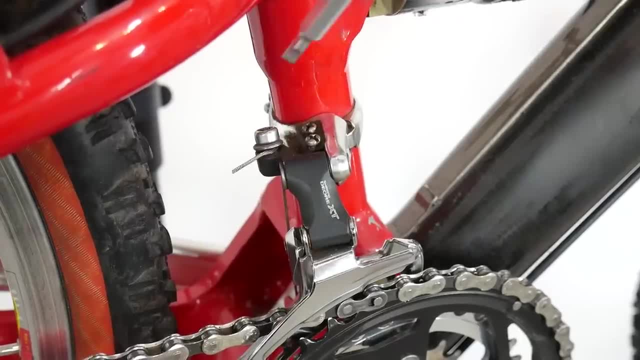 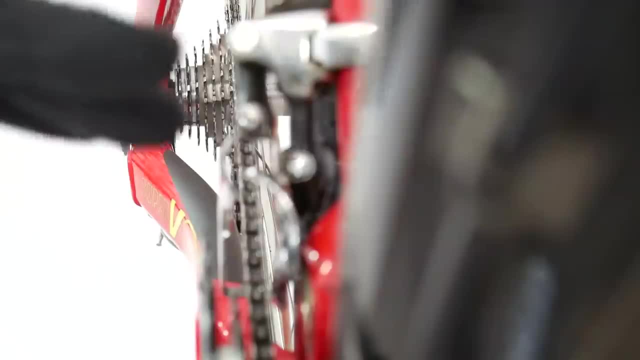 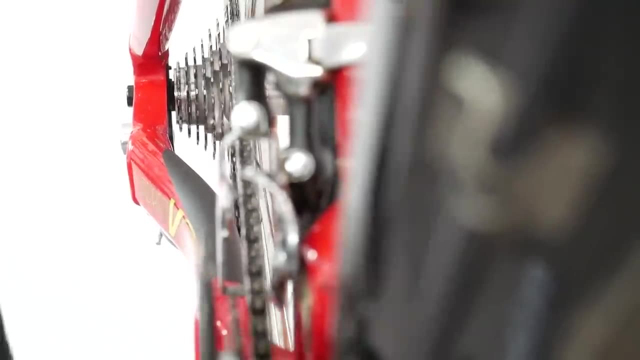 screws for the highest gear and for the lowest gear. First we are going to look at the cassette. We are now on the lowest gear, both on the crankset and in the rear. I'm going to shift down the cassette, maybe three or four gears just. 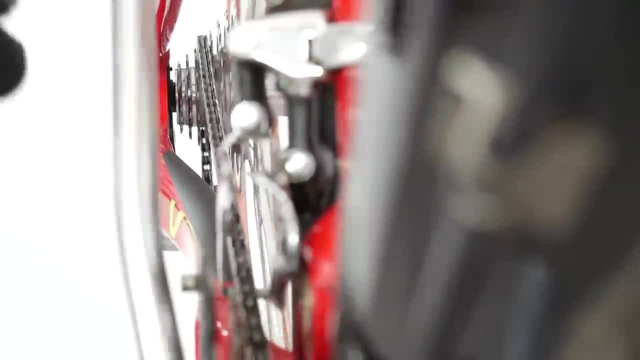 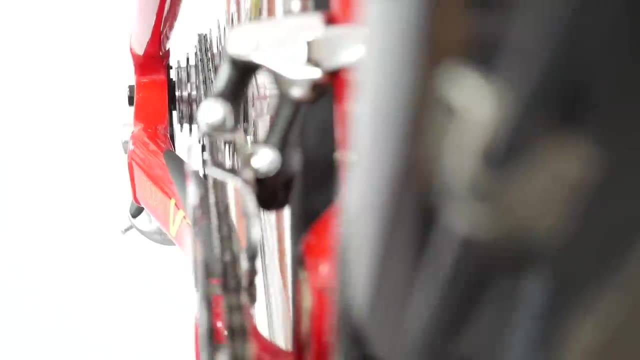 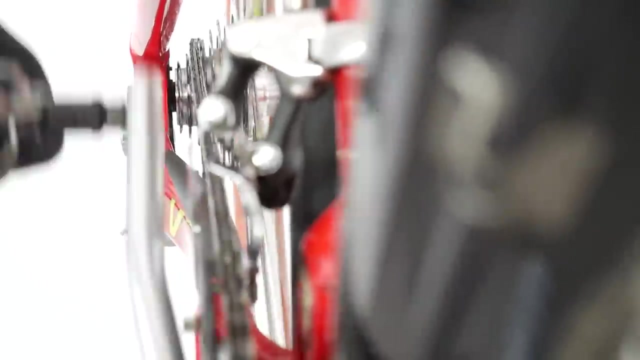 like that- There is no rubbing between the chain and the front derailleur. Then I'm shifting to the second gear in the front and then we can operate some gears in the rear just freely. As you can see, my front derailleur cage is exactly in. 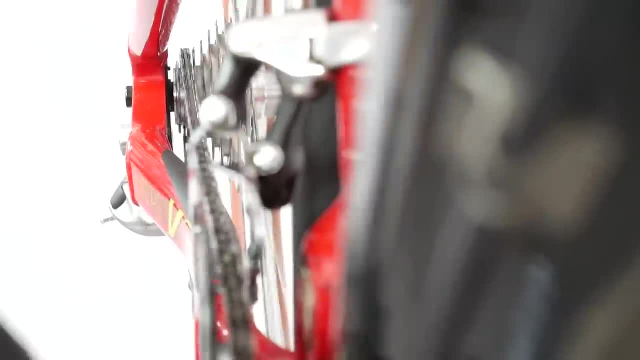 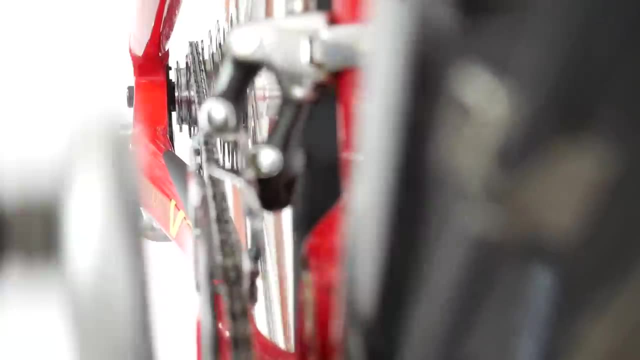 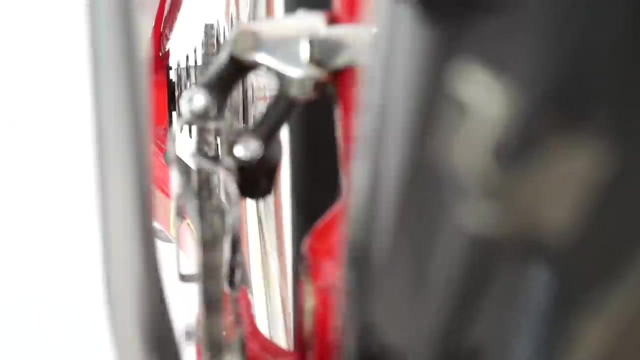 the middle so that I can shift all those gears with no noise between the chain and the front derailleur. Now we're gonna shift into the highest gear and use the highest gears in the rear- No rubbing, Everything, just fine. and now we're gonna look at the front derailleur. Now we're 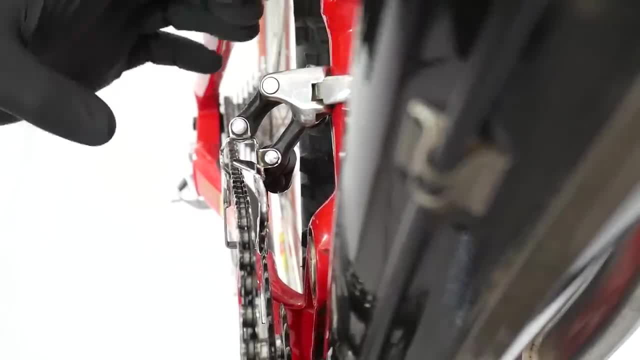 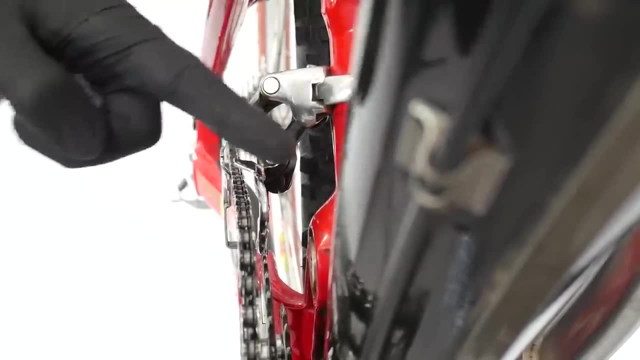 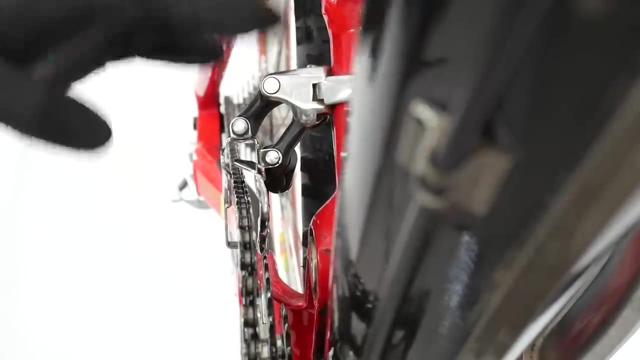 looking at our beautiful front mech Principles. all the same, The limiting screws will not allow the chain to come off the crankset, either outwards or in between the frame and the crankset. That would be really damaging for our frame, for our bike, especially the carbon one. And then, if the front derailleur doesn't, 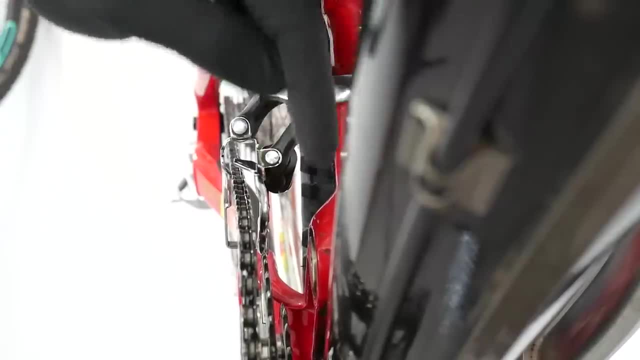 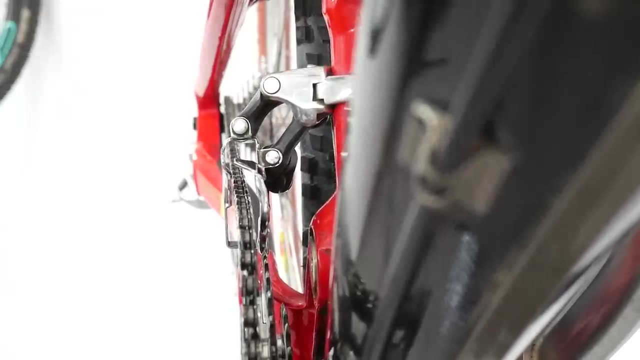 want to shift from the third to second, from second to first, we need to thread in the back of the chain. I'm using a bar adjuster so that the tension of the cable will be lowered and if it doesn't want to go up the crankset from the first to the second, from the second. 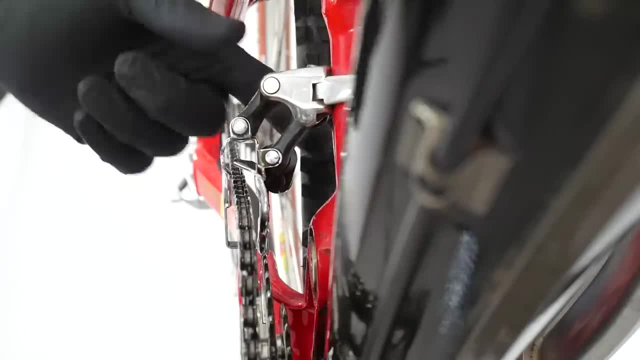 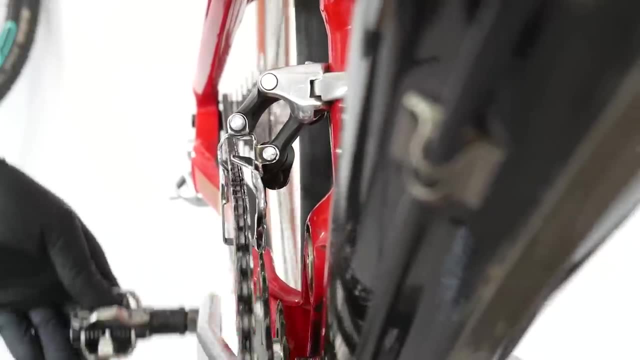 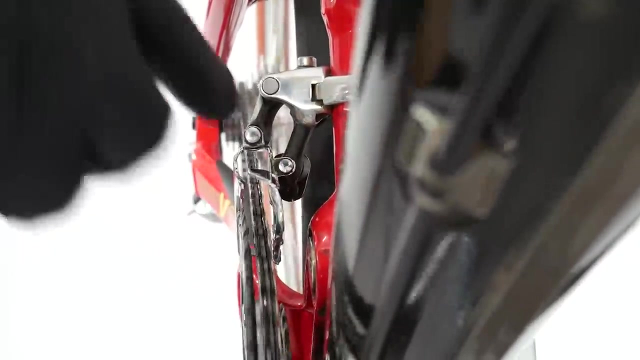 to the third. then we need to increase the tension of the cable by unthreading the bar adjuster. Let's just see how it works right now. So I'm going up the cassette. now to the lower gears. Now here in the middle, no rubbing. 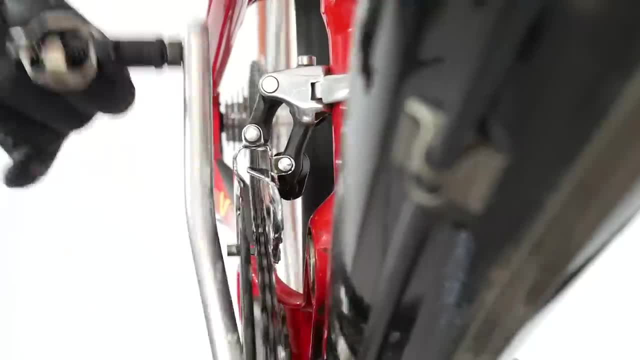 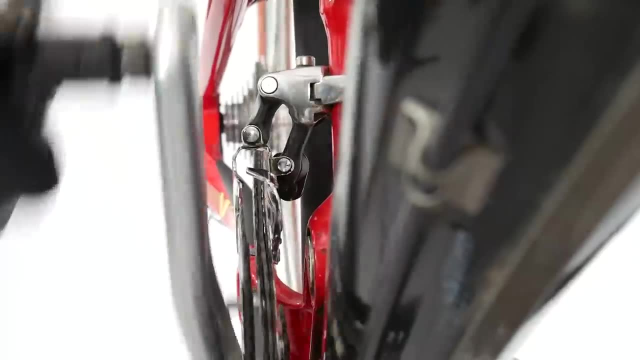 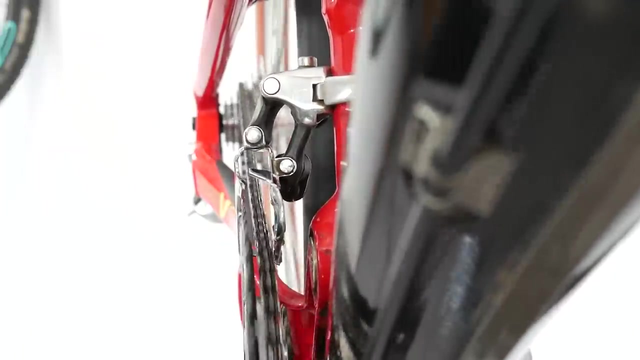 here It works just perfectly. Now you can operate many gears, You can operate a whole cassette, which is not recommended because of extended use of our chain, but it's possible and it's no problem for the derailleur. And then we are going up the cassette to the lower. 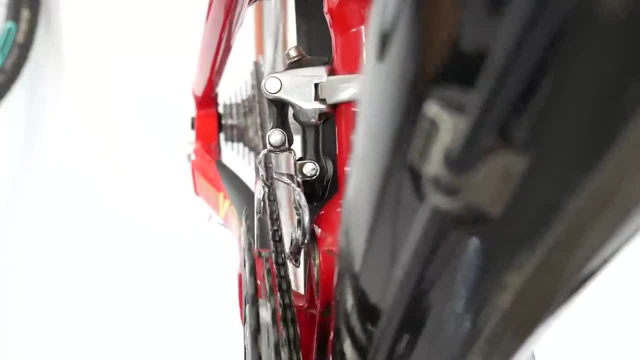 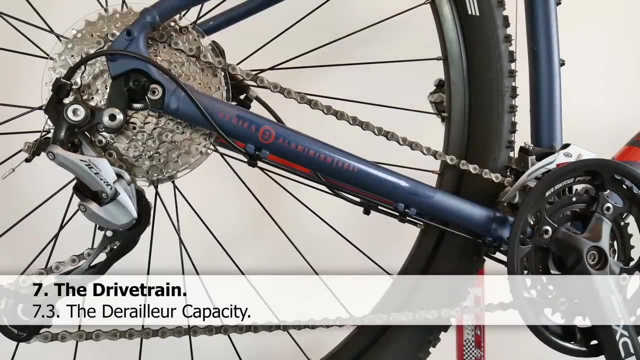 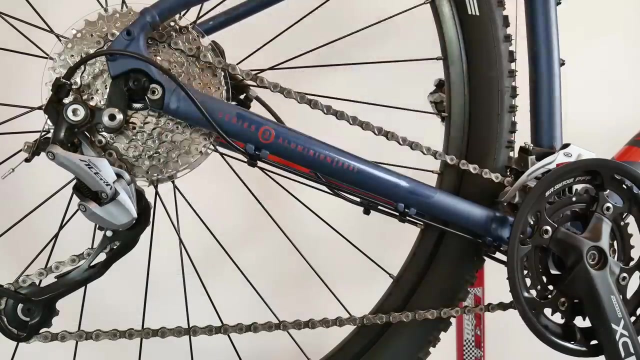 gears, the lowest gear in the front, and it's all perfect. The capacity of our rear derailleur and front derailleur isn't a complicated matter If we only understand roughly how our drivetrain works. So let's talk about what the capacity is, what happens if the derailleur has either too high or too low capacity and finally, how. 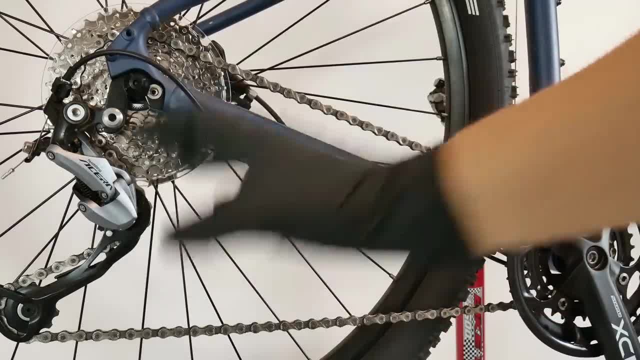 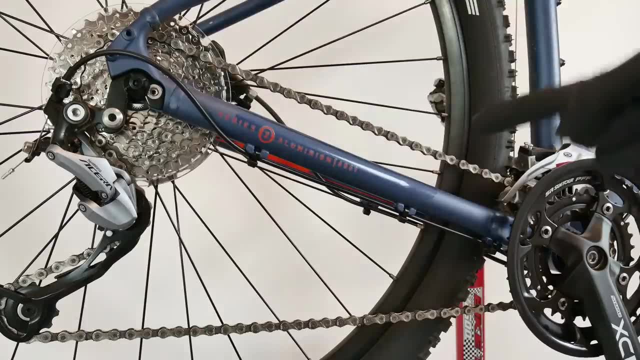 can we find out what kind of capacity derailleur we need for our drivetrain, and we're going to do that in three steps for the rear derailleur and in just one simple step for the front derailleur. The capacity of the rear derailleur basically tells us what is the distance between these. 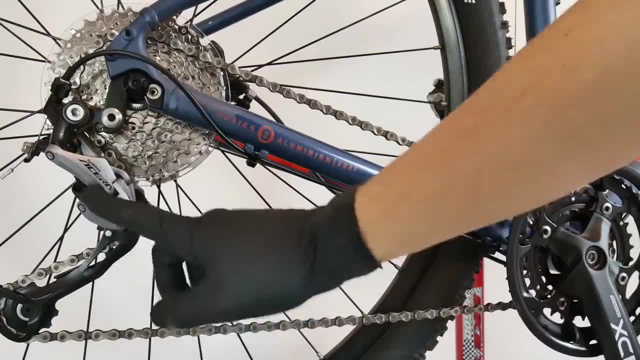 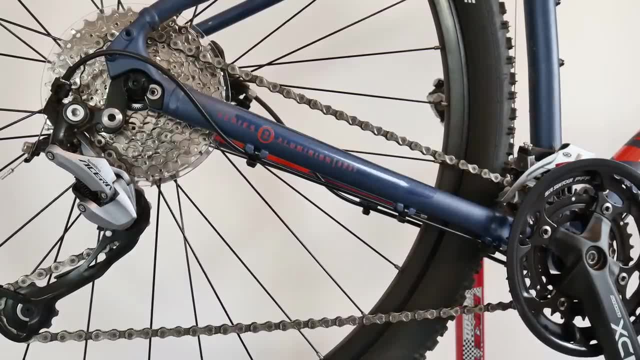 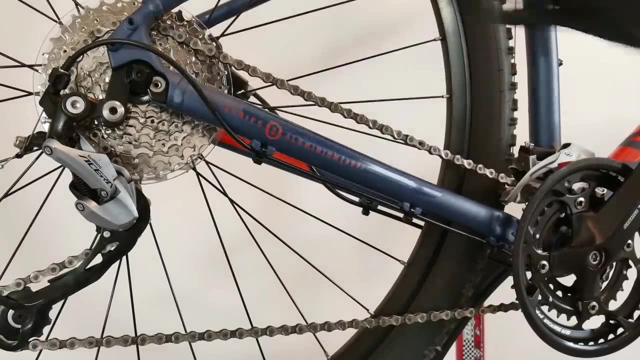 two pulleys. In other words, what is the length of the derailleur's cage? It can be either short, medium or long, And in case of the front derailleur, the capacity is all about shaping of its plates. Now, why do we need different capacities of our derailleurs for different drivetrains? 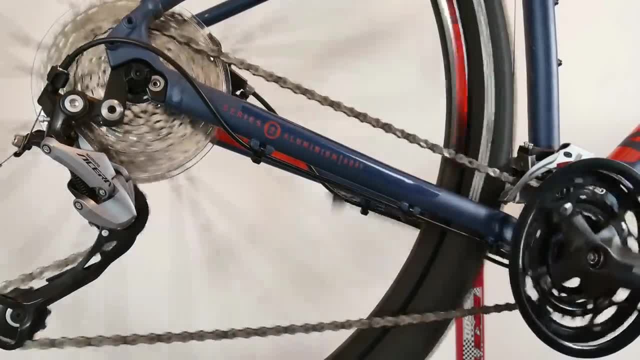 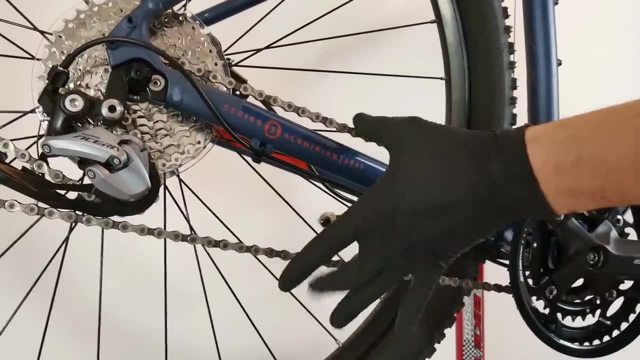 Please look at the cage of the rear derailleur and see what happens while we change the gears. The cage of the derailleur will try to keep the tension on our chain, because we don't want our chain to be too tight, We want it to be just like that. 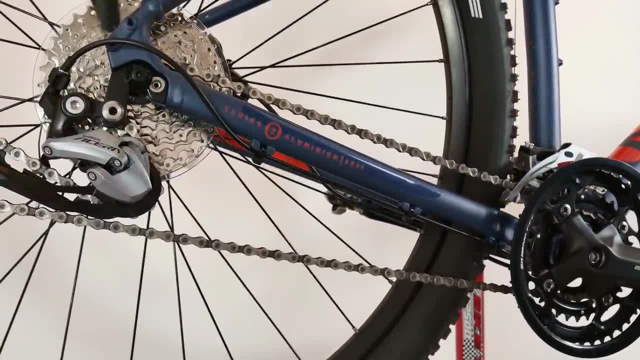 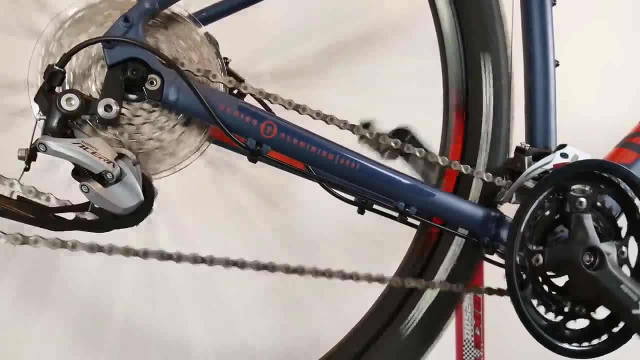 It would cause many problems And while the chain goes through the smaller sprockets it will travel shorter way. so the cage has to adjust accordingly And when we shift to those bigger chainrings like in the front and sprockets in the rear, 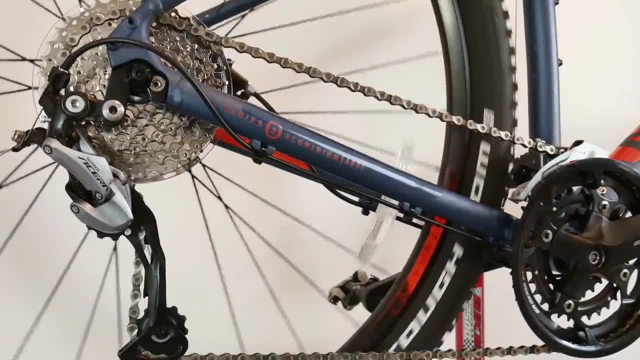 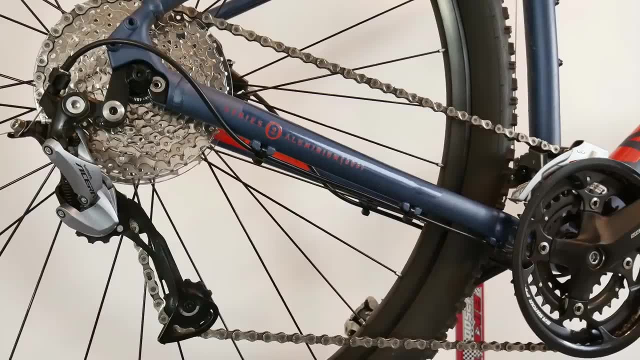 as you can see, the chain will travel a longer way, so that the cage has to adjust accordingly. once more, What would happen? The capacity of our rear derailleur was too low. In this case, that would mean installing short cage rear derailleur instead of long cage, as 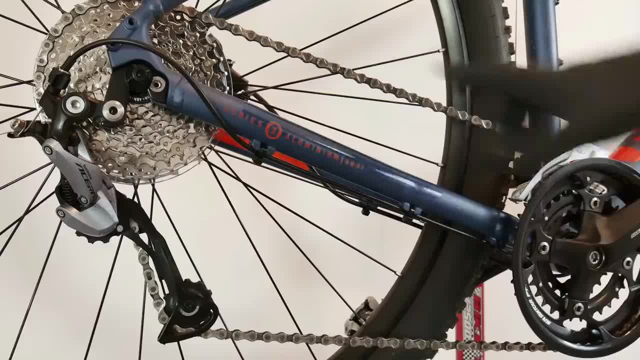 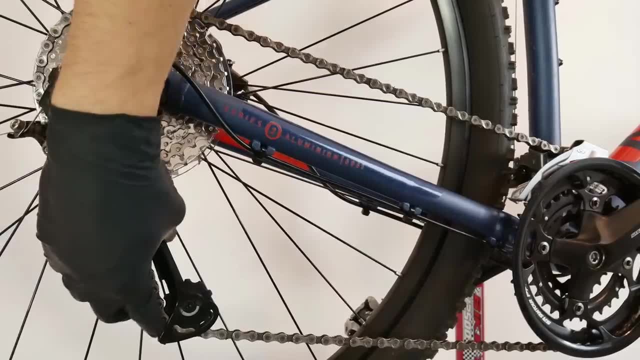 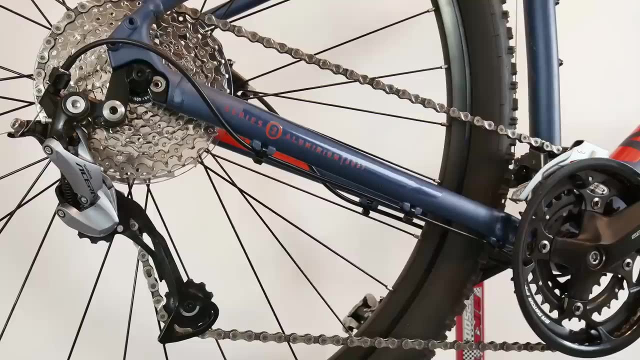 we can see on this video, And that would mean also having shorter chain. So this is the extreme position, but in that position the cage of the rear derailleur would be extremely tight and also sometimes the rear derailleur would be able to get stuck on the largest sprocket. 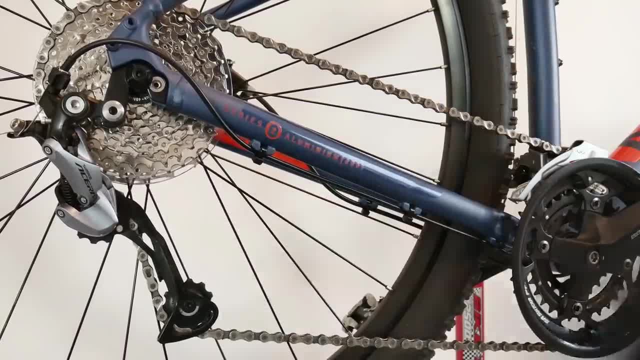 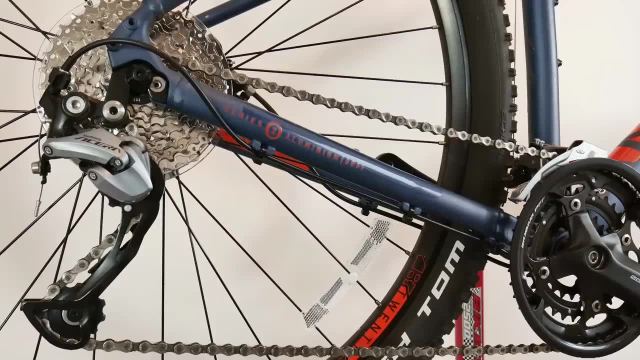 So this cage cannot be too short, So the capacity has to match a whole range of the gears on our drivetrain. What would happen, though, if the capacity of the rear derailleur was too high? Basically, nothing would happen. We would just have the chain longer than needed and the rear derailleur heavier than needed. 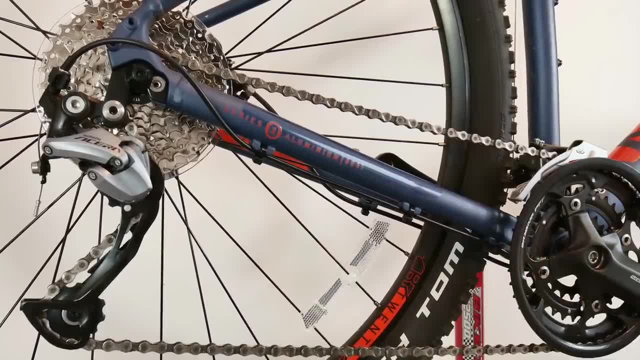 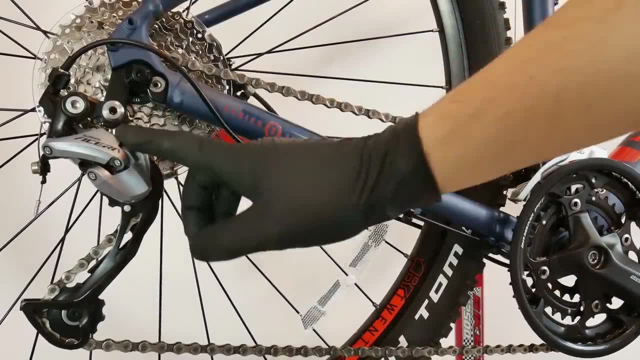 It would still be able to put the tension on the chain. so having the capacity of the rear derailleur too low is the problem, is bigger problem than having the capacity too high. In case of the front derailleur it's all much more simple because the front mag's capacity 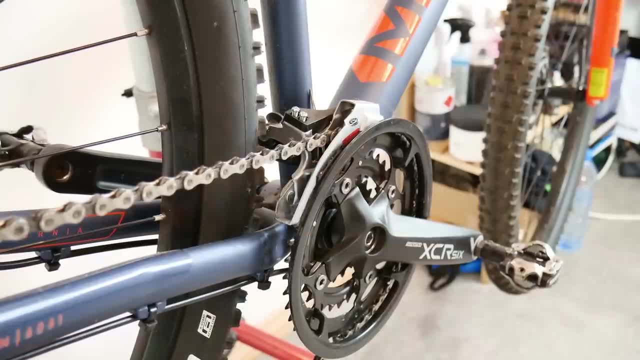 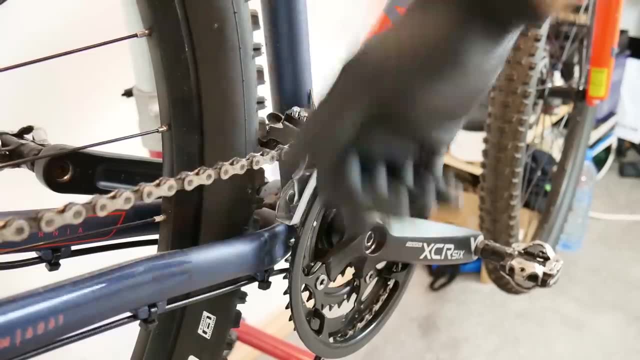 has nothing to do with the chain length or tension. It's just all about the shaping of those plates so that the derailleur will be able to, let's say, scoop up as low as possible in case of the double chainrings or triple chainrings. 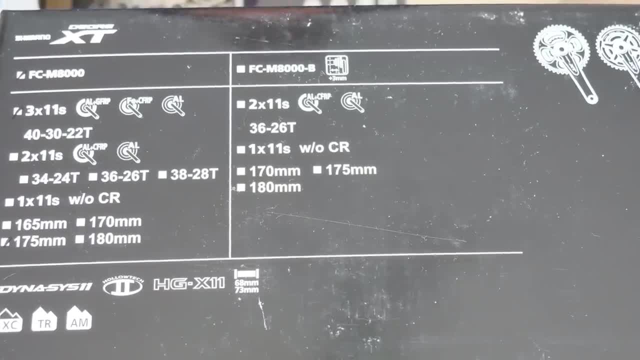 on the crankset. And now we're ready to find out What capacity of the derailleurs we need for the drivetrain which is bought for our project. So let's say we've got 3 by 11,, 40,, 30, 22 teeth chainrings on our crankset. 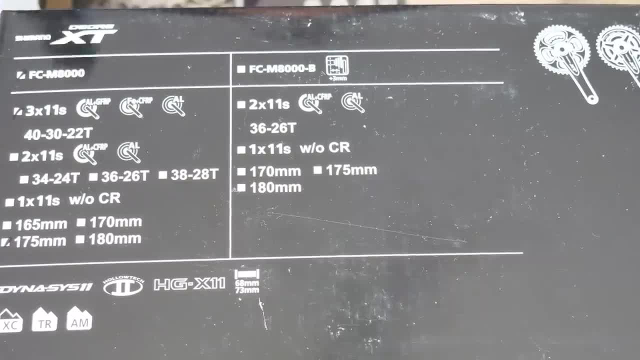 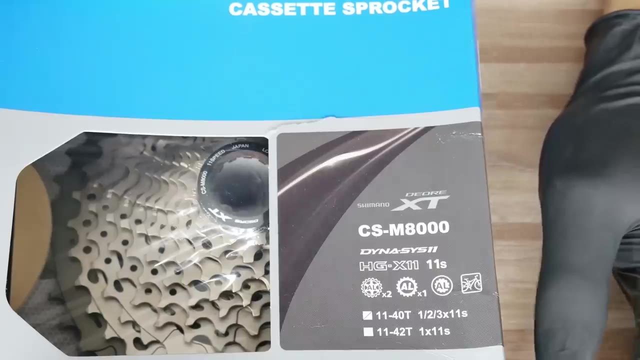 This is the XT1.. The first step is to find out the difference in the range of those teeth between the largest and the smallest. So 40 minus 22, that gives us 18.. Write it down 18.. In the second step we need to find out what is the gearing range on our cassette. 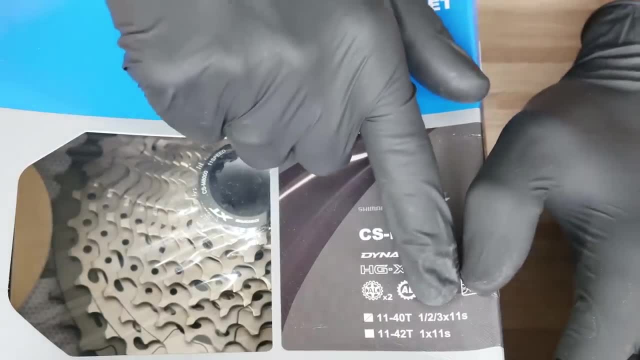 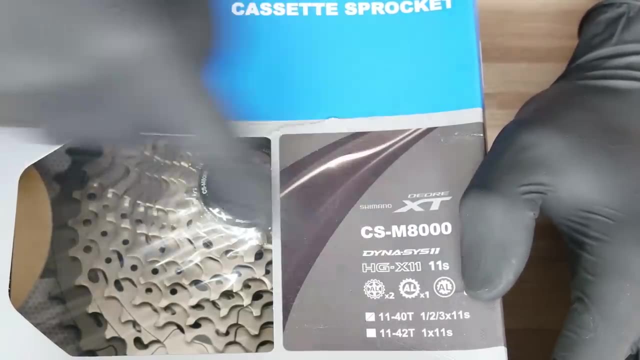 We've got here the XT1 for single, double and triple chainrings. That's good, because we have triple chainrings on the crankset, And the teeth are 11 through 40. So once more, 40 minus 11, that gives us 29.. 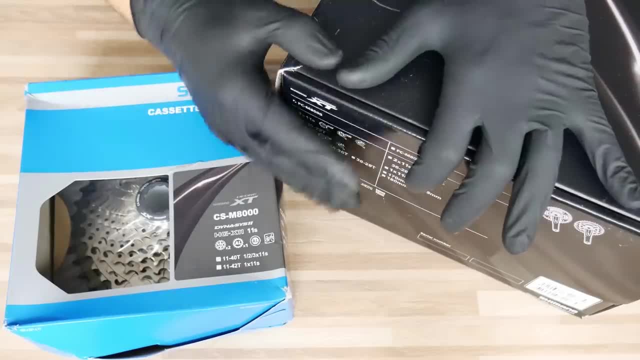 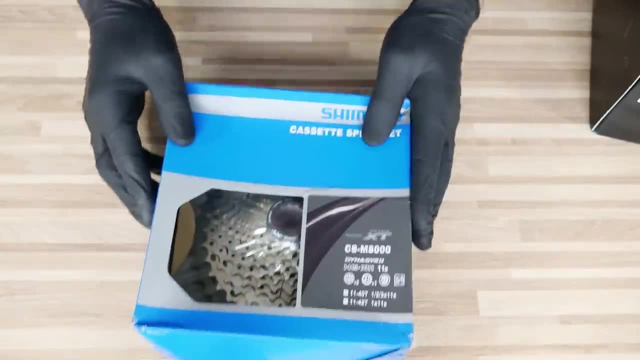 In case of 1 by drivetrain, because we've got here the triple chainrings on the crankset. If it was only 1, we don't need to even bother about the crankset. We only need then the gearing range on the cassette. 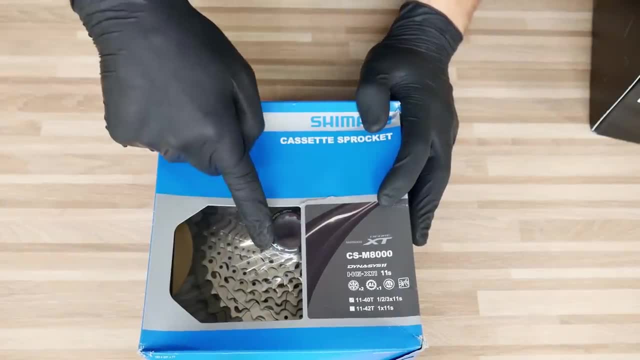 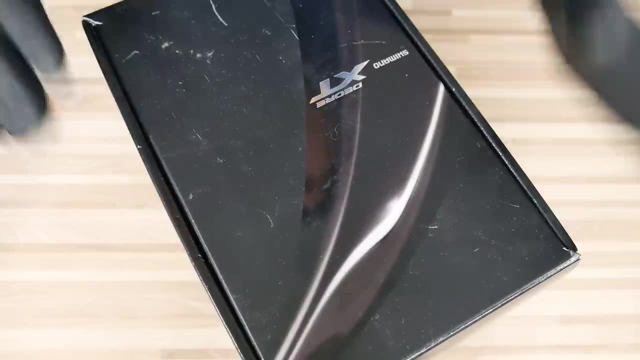 So that would be 40 minus 11, and that's 29.. In case of the front mech capacity, we are only interested in the gearing range of our crankset. In this case, 40 minus 22 and that's 18.. We are almost done. 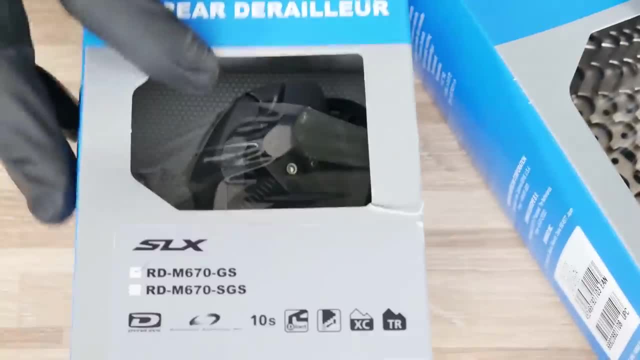 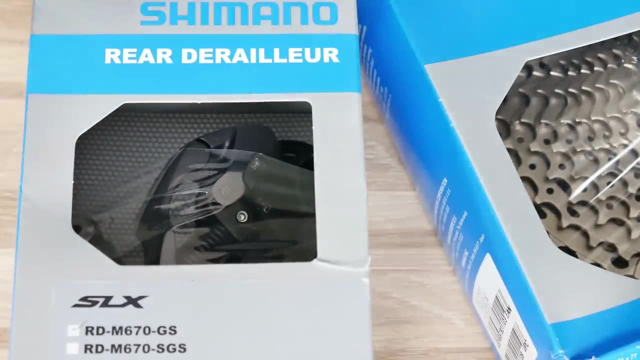 We need just one more parameter of the rear-directing The rear derailleur, and that's the largest sprocket on the cassette that our rear derailleur will be compatible with. So once we know the capacity, we only need to check out for this largest sprocket on the 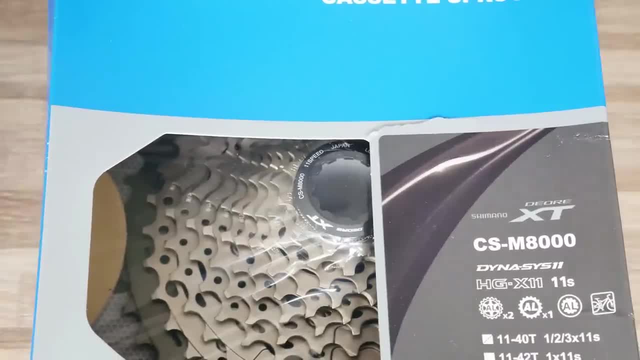 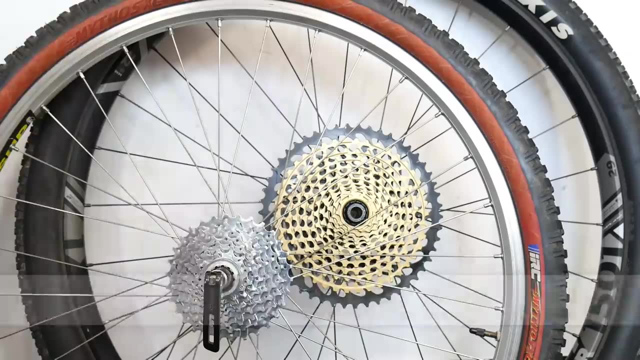 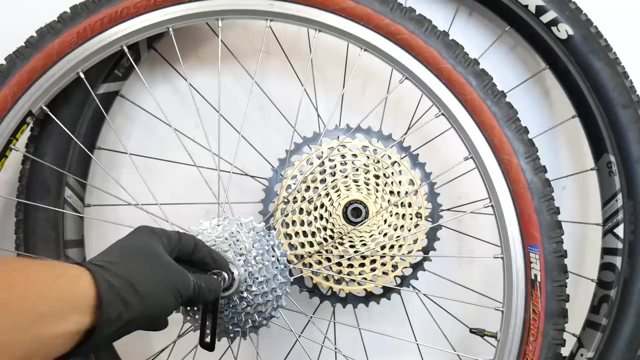 cassette that our rear mech will work with. So, knowing the capacity and this number, we are ready to purchase the right derailleurs for our projects. Removing and installation of the cassette is pretty easy. We need to remove the wheel from the bike, Then we remove the release, or quick release, from the axle of the hub. 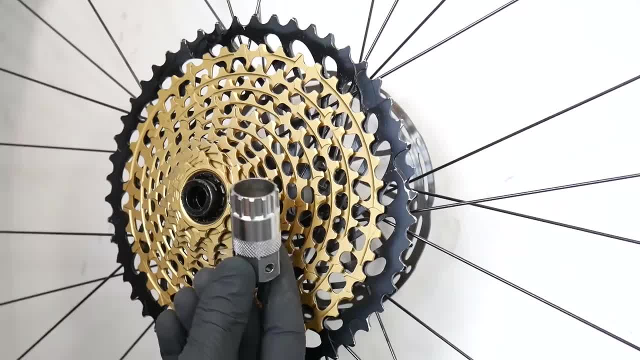 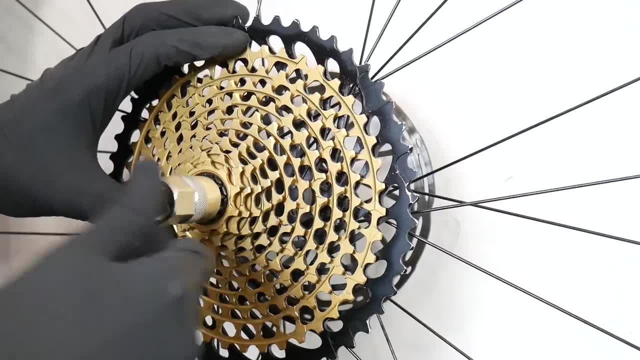 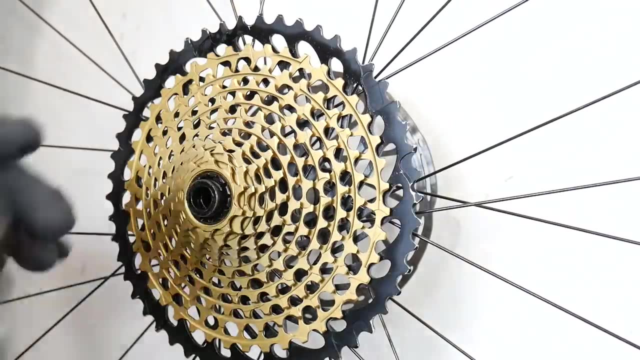 And then we need some tools. First off, we need a special tool that will fit the lock ring on our cassette. This is how it looks like It will go right into this space here, And then we can use another wrench for it, or we can buy a dedicated tool with the centering. 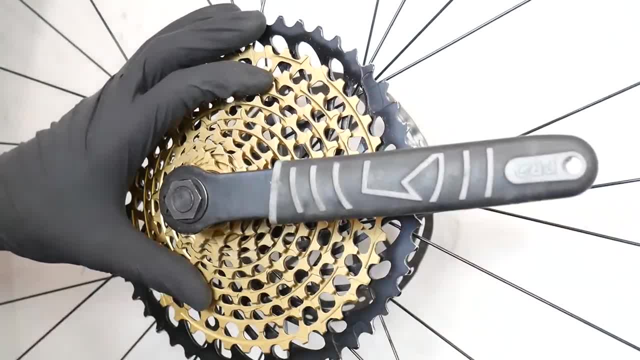 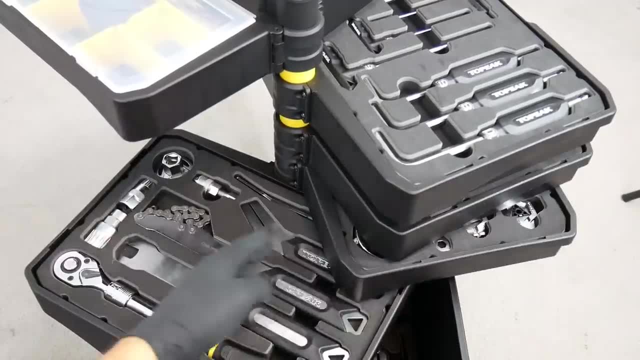 pin. This will allow us to unthread the lock ring. The problem is that, while unthreading the lock ring, the cassette will turn as well, and so we need yet another tool. This is called a chain whip, and this will allow us to do it in the safe way. 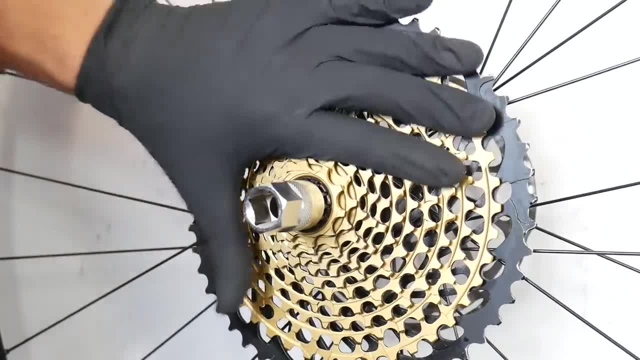 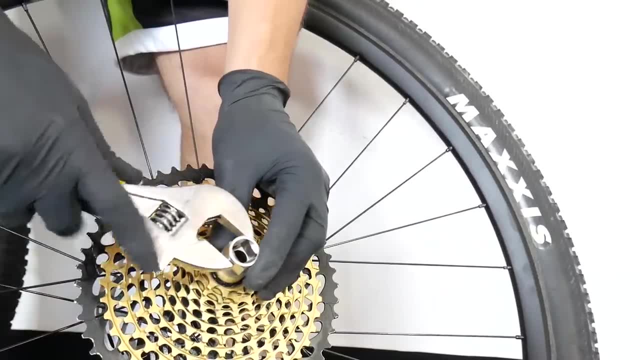 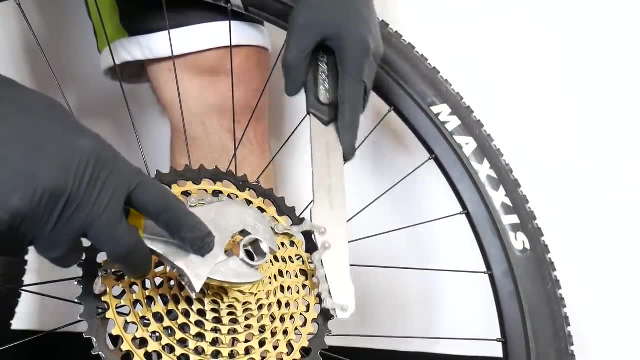 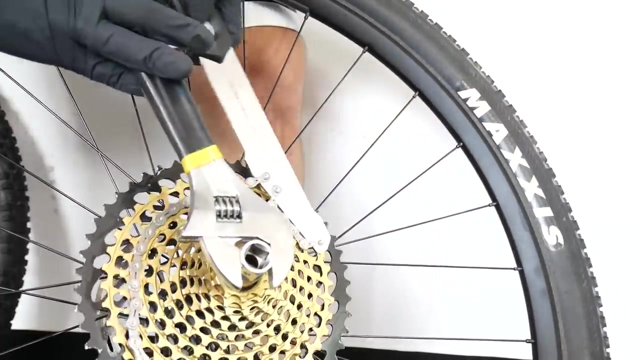 So do not try to hold the cassette with your hands, even through some rack, because these teeth are pretty sharp. So this is how it looks like when we unthread the lock ring. You can see how the lock ring is going to be used when we are going to be installing the. 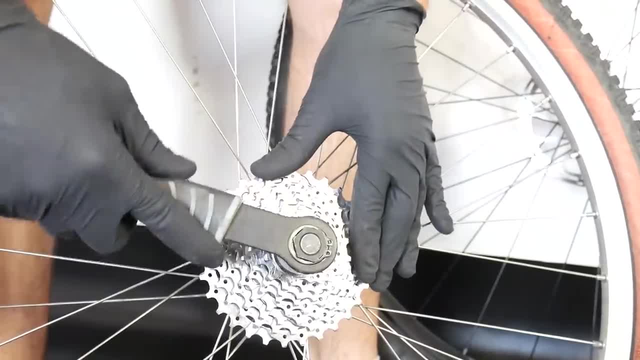 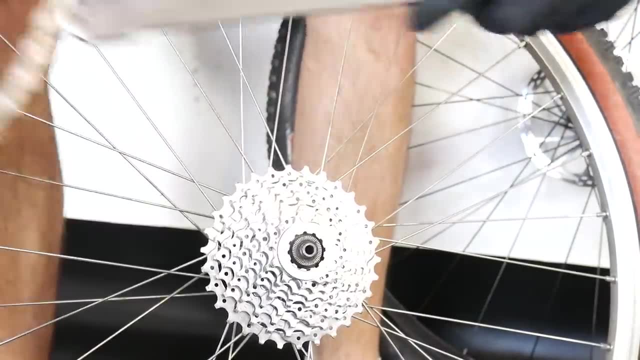 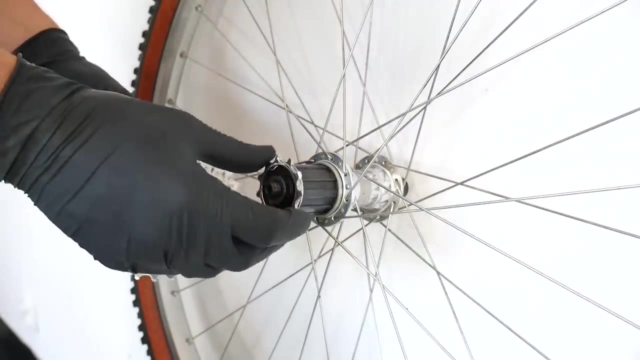 cassette. Let me show you how to do this. So we are going to take our chain whip Unthread, Unthread, Unthread. good news for the beginners: when assembling the cassette on the freehub body- this part- you don't have to be worrying that you will put something. the 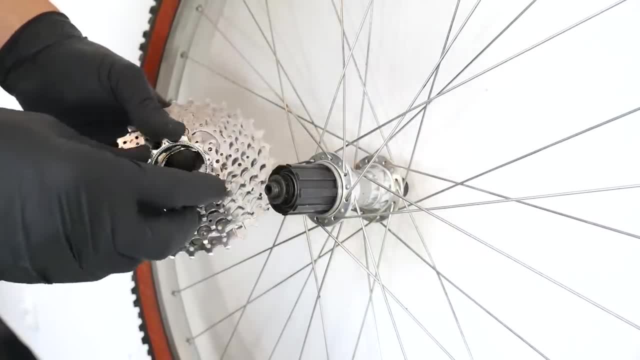 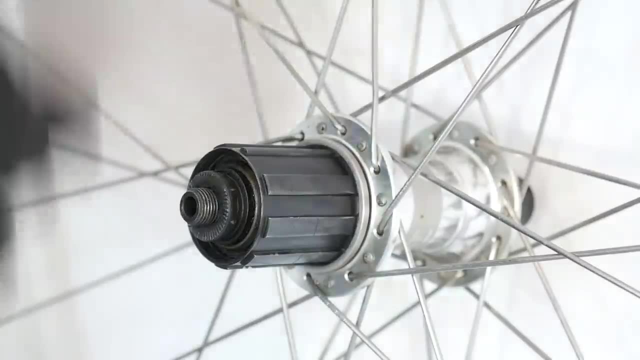 other way around, or you would twist some sprockets against the others, because the special grooves on the freehub body will not allow you to do anything wrong. how to assemble the cassette on the freehub body. if you take a closer look at it, you. 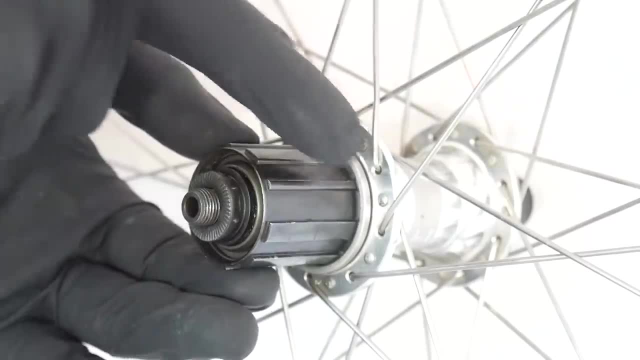 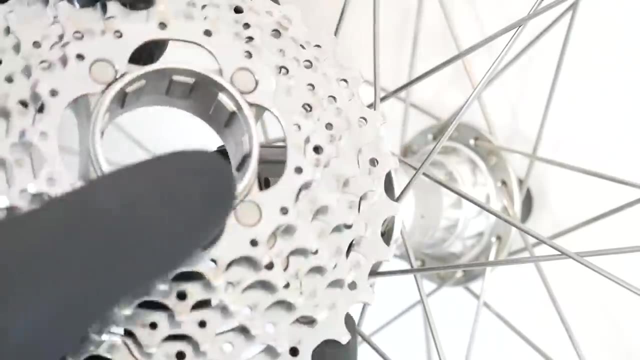 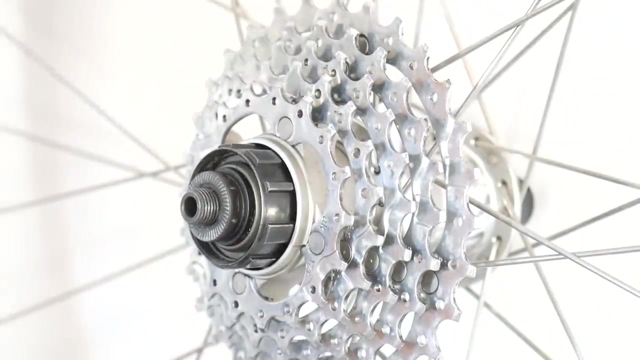 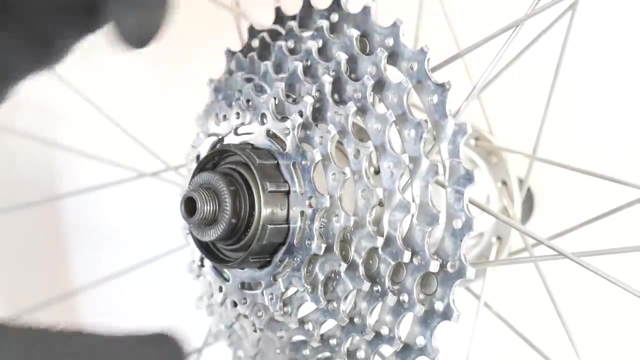 will see that one of these grooves, if you will, is smaller, and so there is a larger space between these two. now we can find the corresponding grooves on the cassette, and then we'll be able to assemble it in the right way. I will proceed in the same manner with all the other sprockets. so this fits okay, and so. 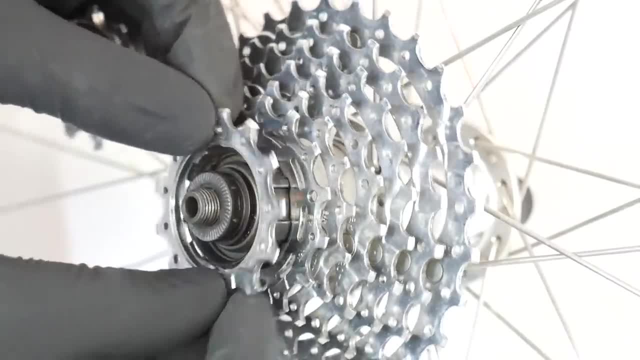 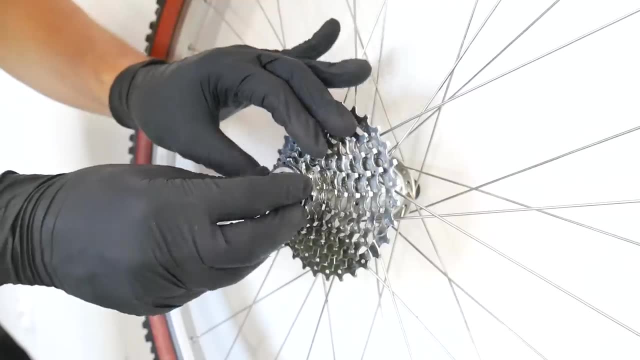 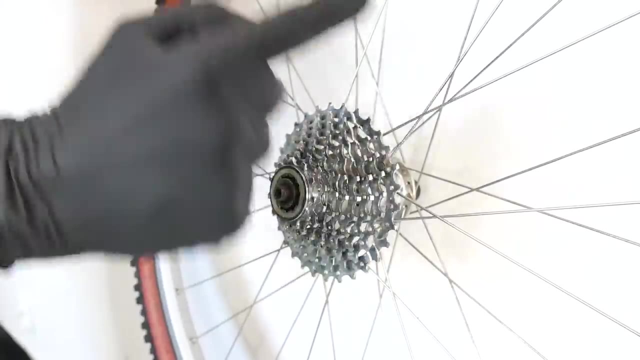 you won't be able to do anything wrong here. we just do it like this: after putting here all the sprockets, we are using the lock ring, and in this case we won't need the chain whip, because the cassette will not turn clockwise, so that we can only use our 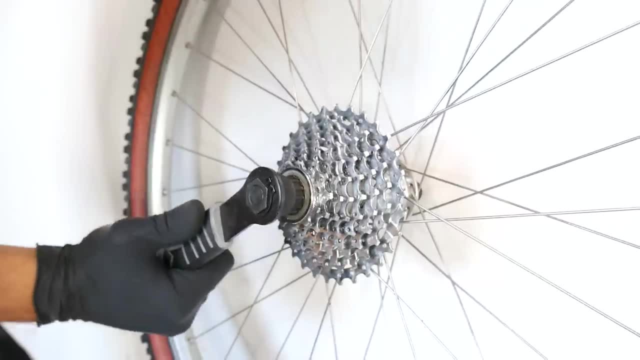 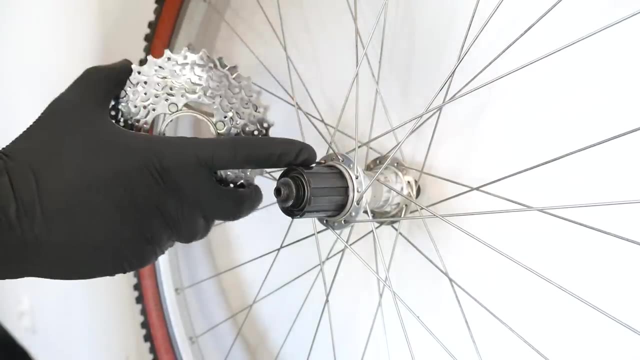 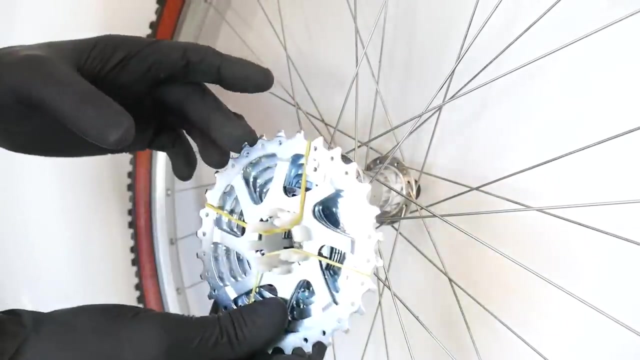 tool and the job is done. let's just remember that on the Shimano and SRAM freehub bodies we will be able to put Shimano or SRAM cassettes- so these are interchangeable- but we won't be able to put the Campagnolo. 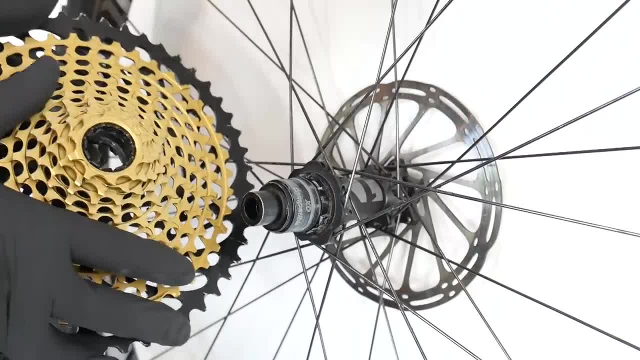 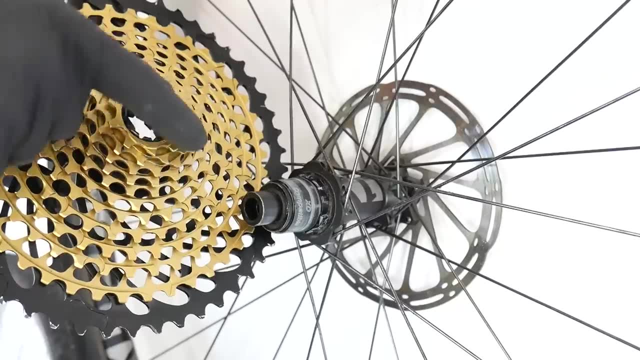 which is also in the same size. so that is not an issue only for Shimano or SRAM, but you can also put any other type of cassette which has different pattern. the exception for the Shimano and SRAM cassettes compatibility is the SRAM. 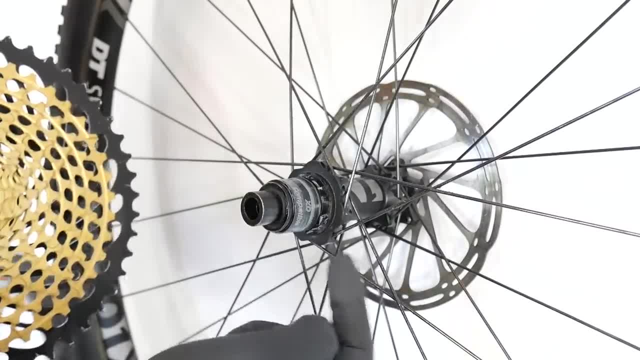 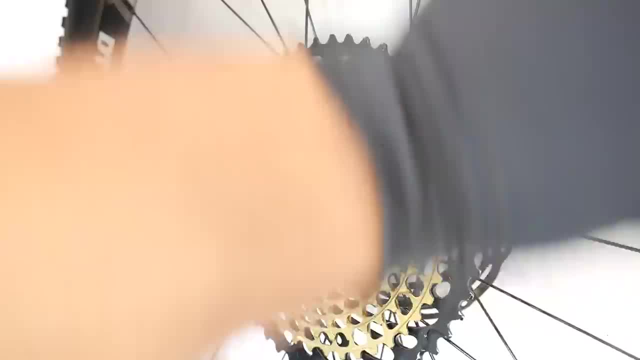 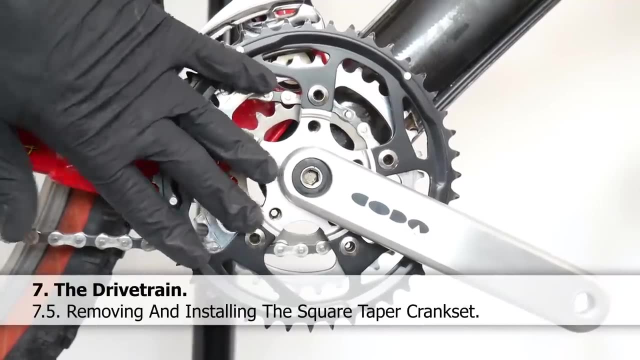 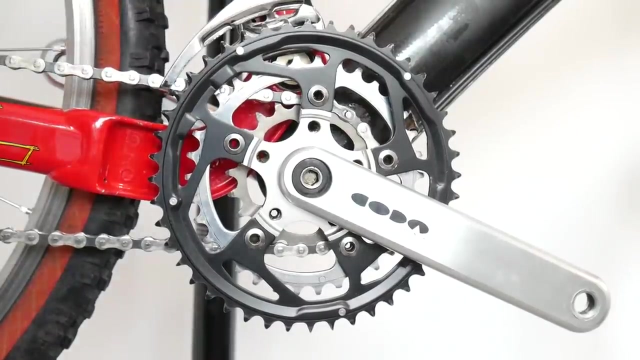 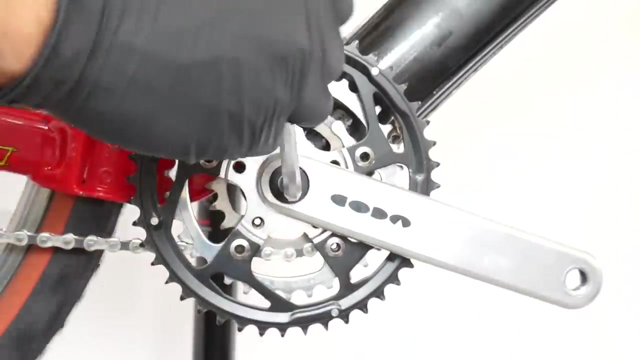 cassette which will have only ten teeth on the smallest sprocket. this type of cassette will need a special freehub body which is called XD. you Removing the crankset on the square tapered system, we will begin by removing the small dust cap. in this case it's a bolt, so we're going to unthread it. 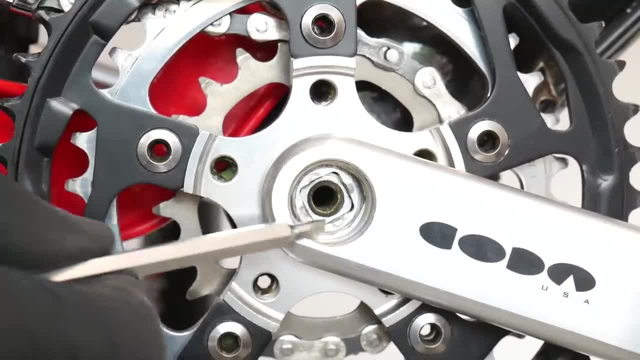 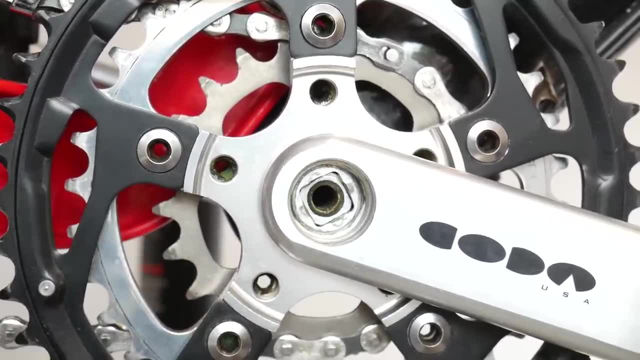 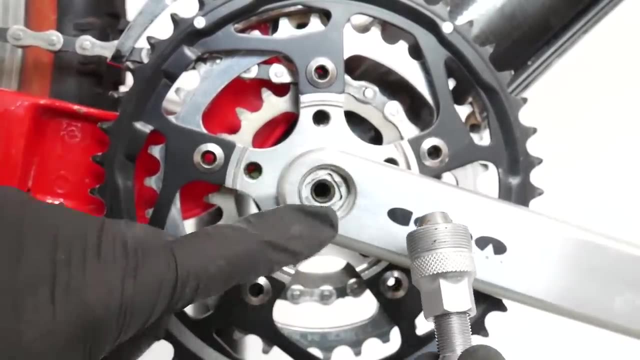 Now we can see our square tapered axle and the bolt that we just removed. that was the one which assembled the crankset on that axle. Now we need a removing tool, and this is the tool we are going to use. This thread will be threaded into the crankset's arm. so the arm of the crankset and then this. 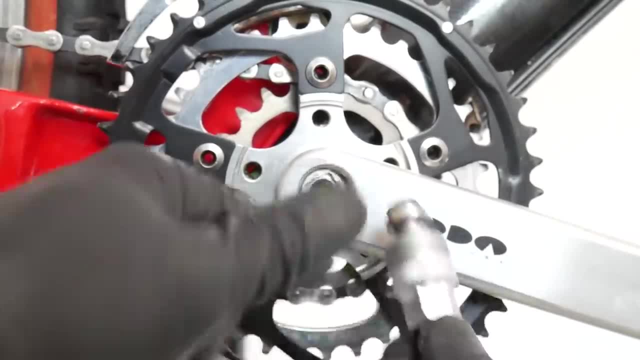 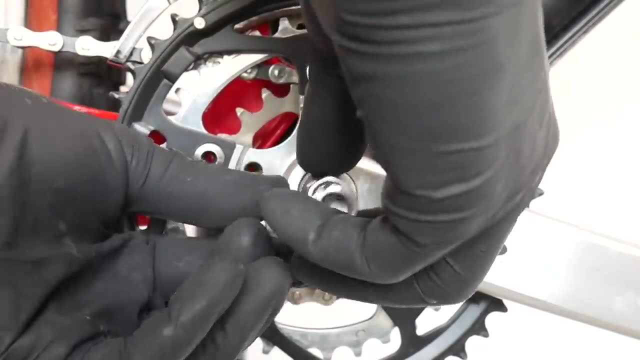 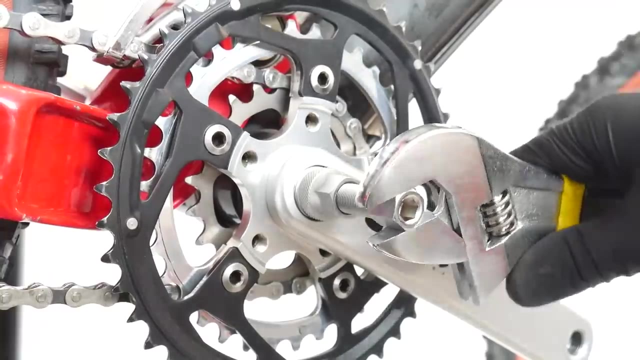 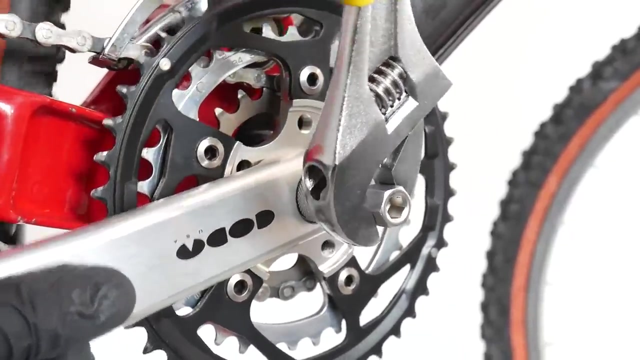 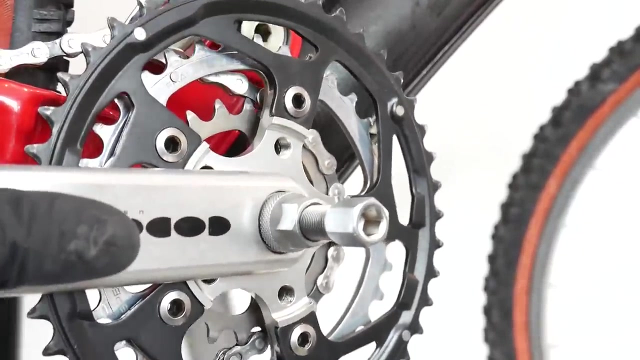 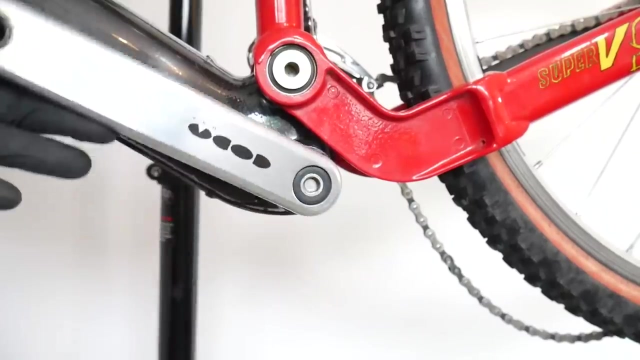 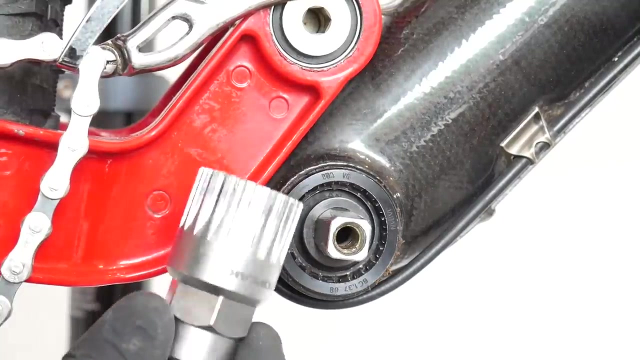 pin will be pushing against the axle of the bottom bracket, removing a whole thing. And now, just slowly, Okay, And now we'll do the same exact thing on the left side with the left crank arm. Both crank arms removed. now we can use the special tool for the square tapered bottom. 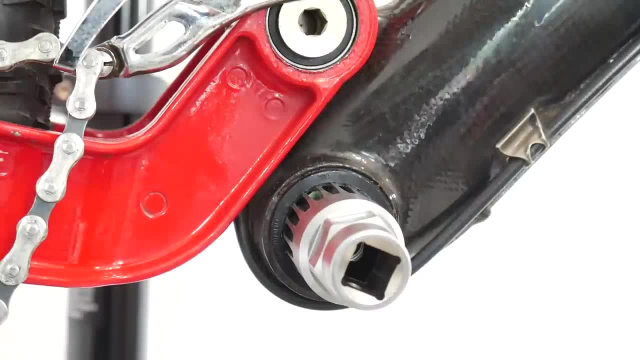 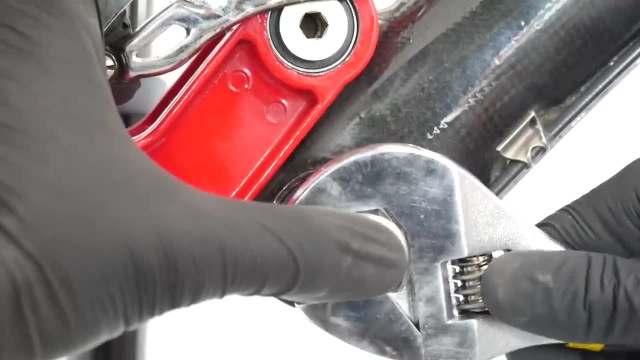 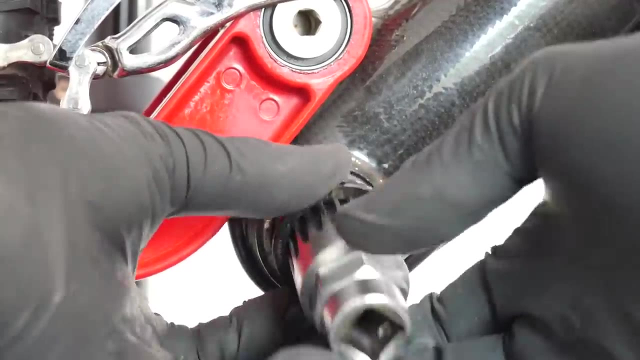 bracket removal. Now, please pay attention to this- we are on the drive side on the bike, so this is the front derailleur and we are going to unthread the bottom bracket, moving the tool clockwise. The drive side is already removed, but the axle is still there. 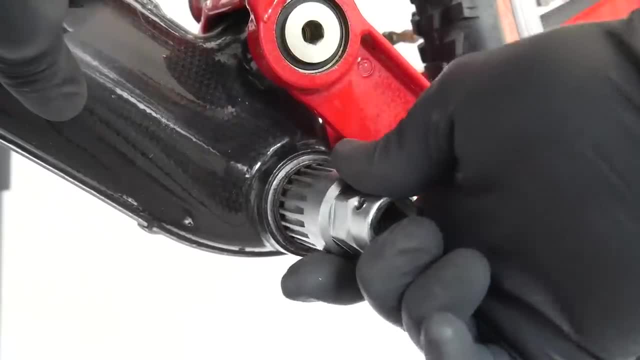 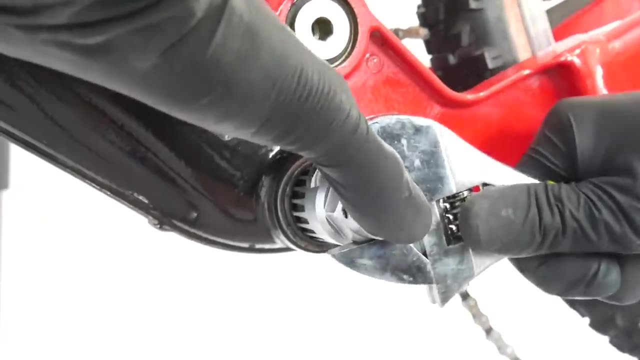 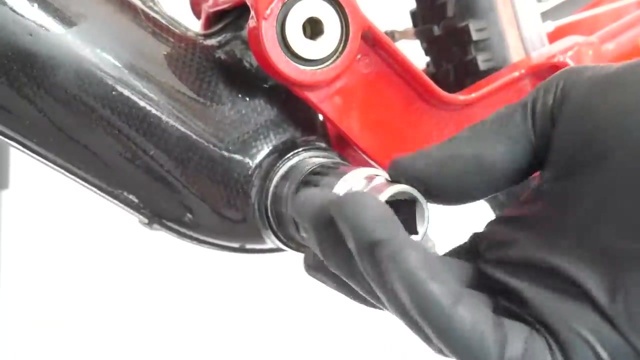 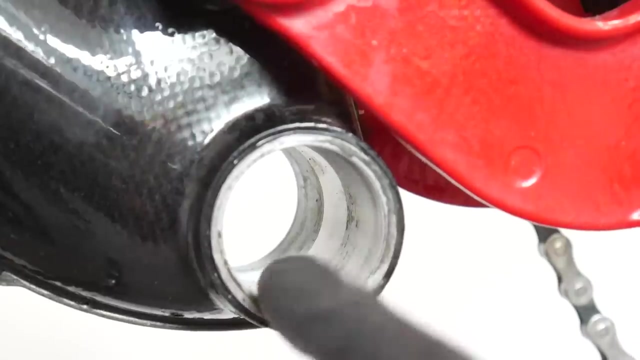 We are now on the left side, the non-drive side of the bike, and we are going to unthread the bottom bracket. We are turning our tool counter-clockwise. The cartridge is removed, so now we can take a closer look at the shell of the bottom bracket. 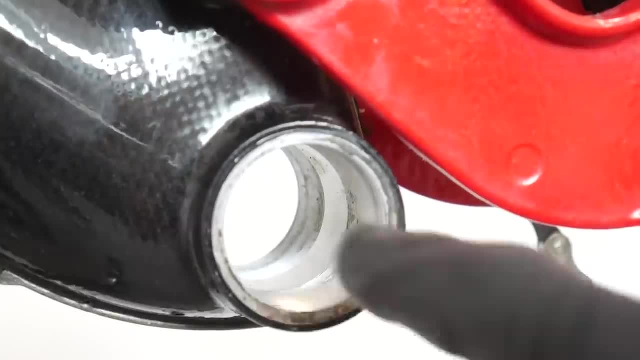 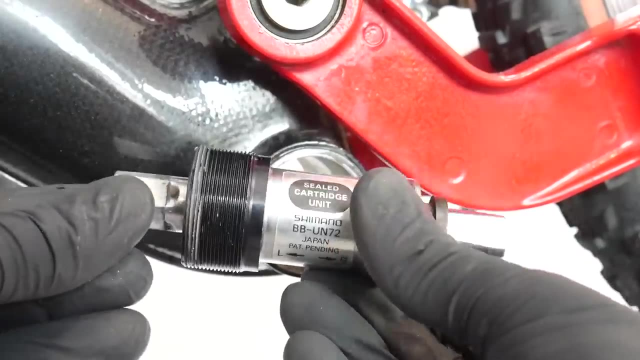 inside the frame. The threads are in perfect condition. I'm going to just clean it, put some grease and also take a look at the bottom bracket cartridge. And this is our removed bottom bracket. As you can see on the square tapered system, the axle is integrated with the whole cartridge. 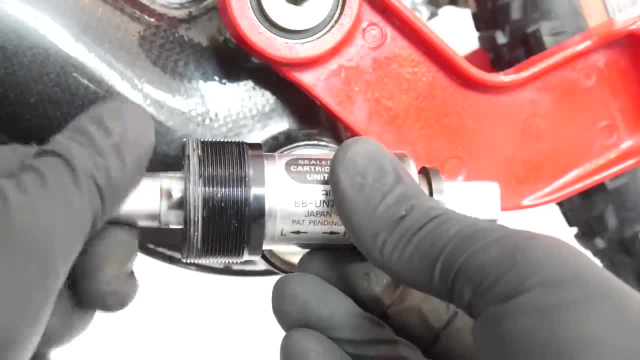 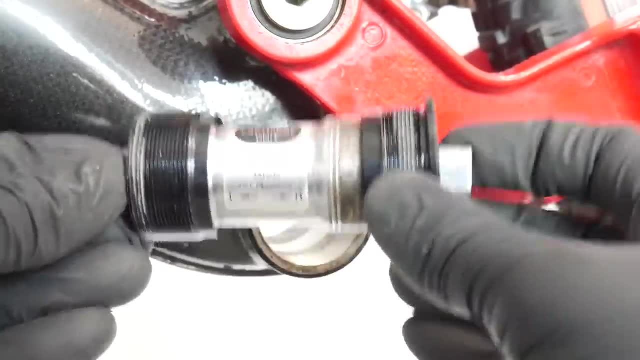 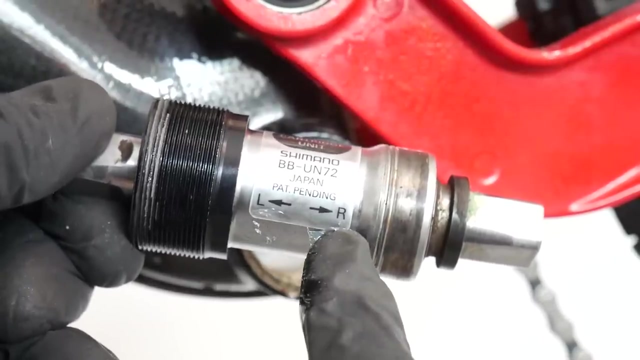 The threads are in very good condition. it's working super smooth and also the nut has the threads and everything in a perfect condition. This cartridge will make another thousands of miles. Left side, so non-drive side. Right side, the drive side. 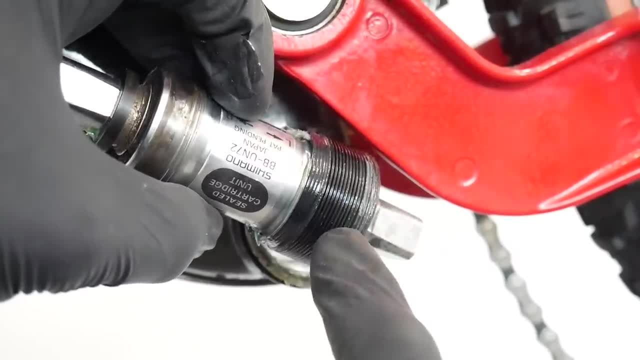 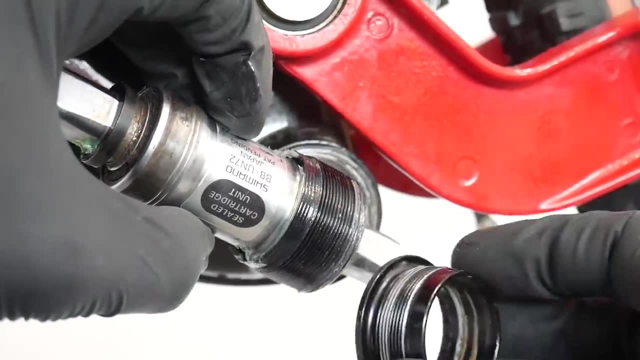 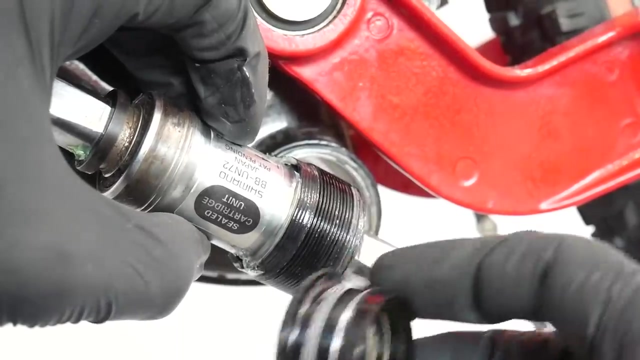 Very important observation here: This thread on the left side, the non-drive side, on this particular cartridge bottom bracket, doesn't have any edge comparing to this nut here which has the edge. That means that we could be threading this one in just endlessly. That's why we need to start the assembly with the drive side, with this edge. 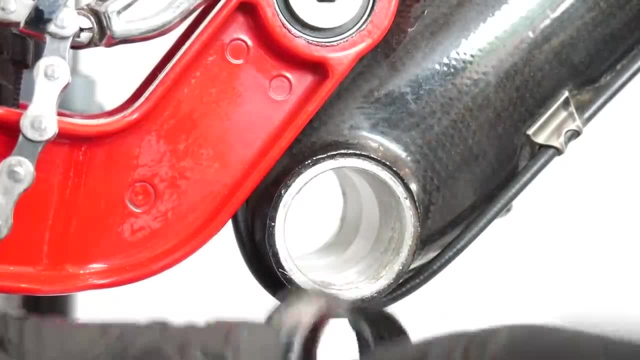 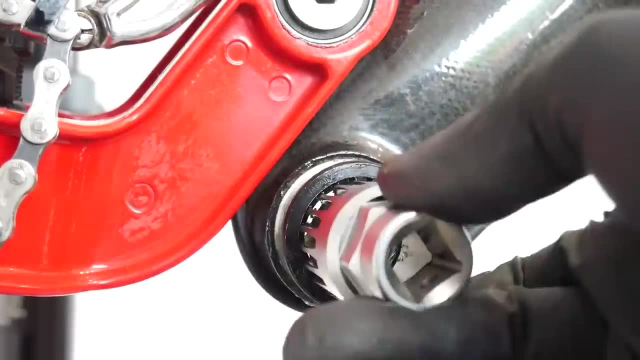 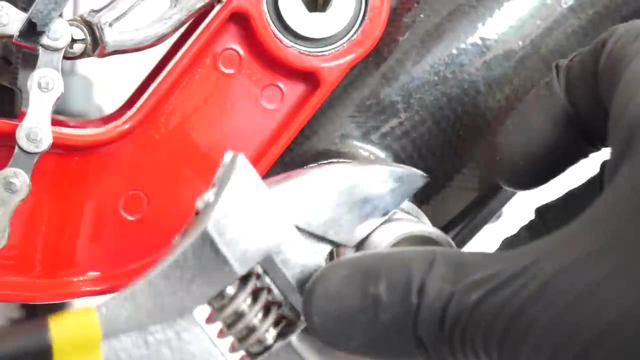 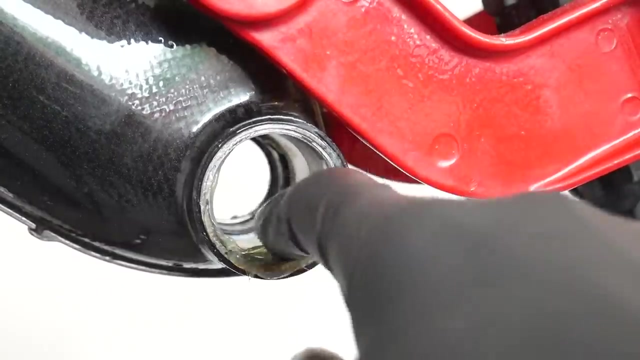 So we're just going to take one side here. And we're just going to take one side. Okay, We're just going to take, or the other side. As you can see, it is in perfect condition, So we're just going to take one side. 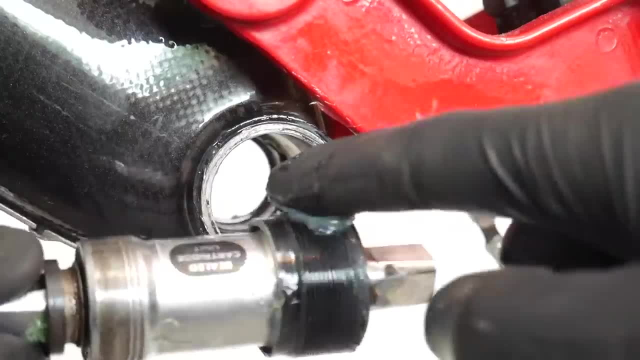 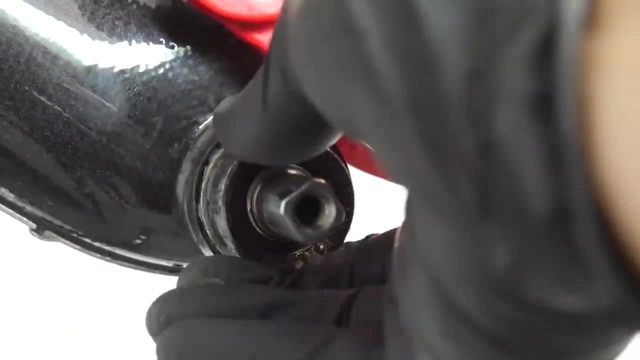 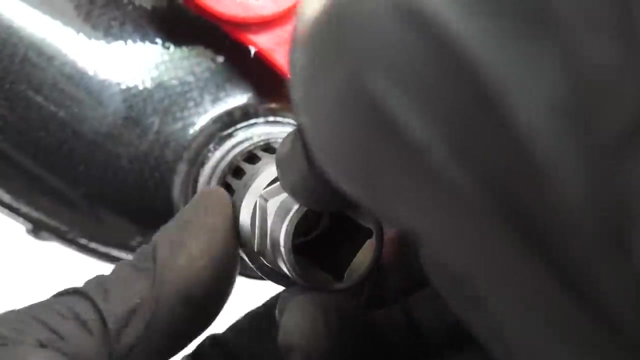 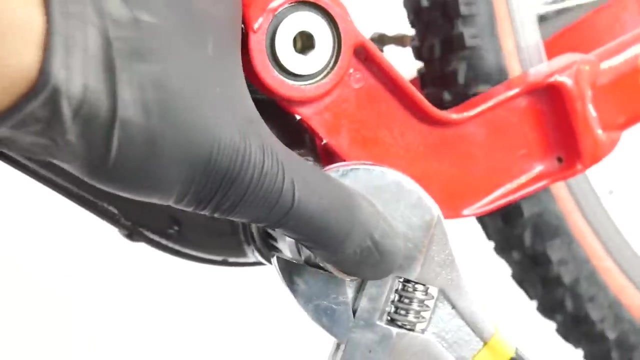 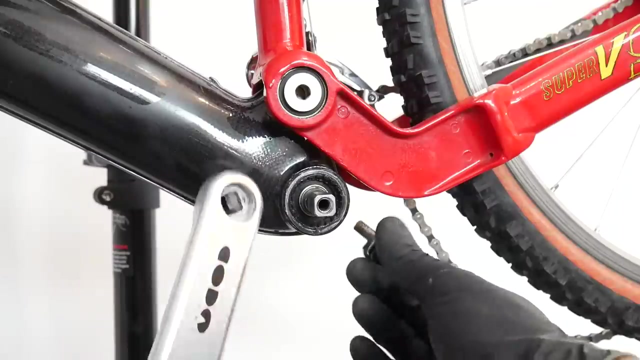 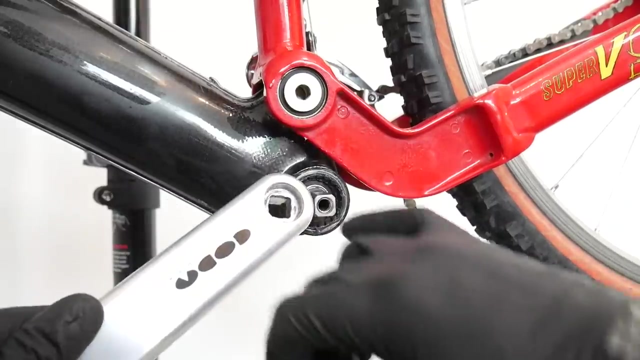 We're just going to take the other side. Alright, Let's do this. Okay, It is time now to install our crank arms. We want to minimize the friction between the axle and the crank arm, and also between the crank arm and the fastening bolt. 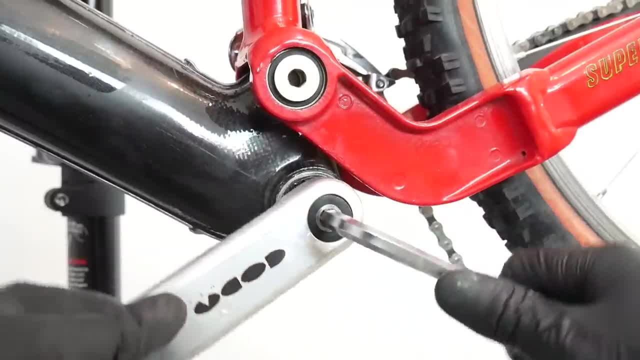 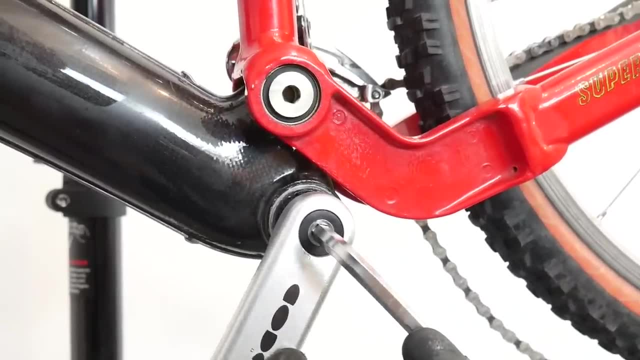 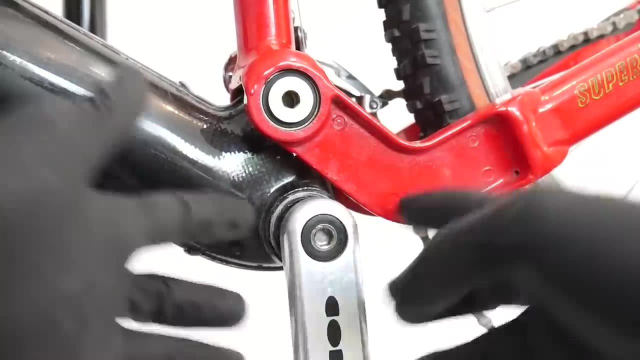 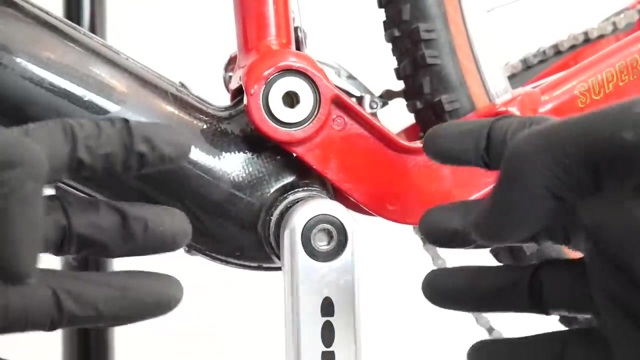 The left side is ready, I'm going to assemble the right one. It is also a good idea, after maybe a couple of minutes, to fasten these bolts a little bit more, because we are pushing the crank arm through the axle which is tapered. When assembling the right crank arm, just remember to align. 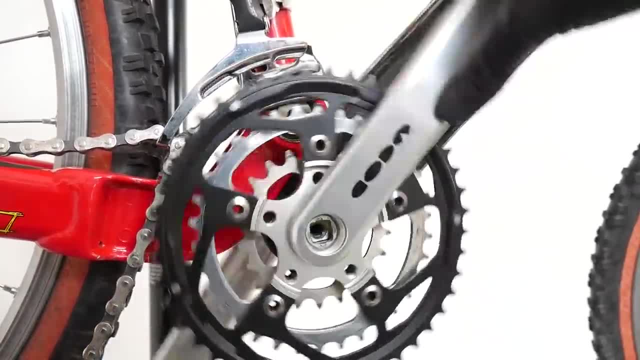 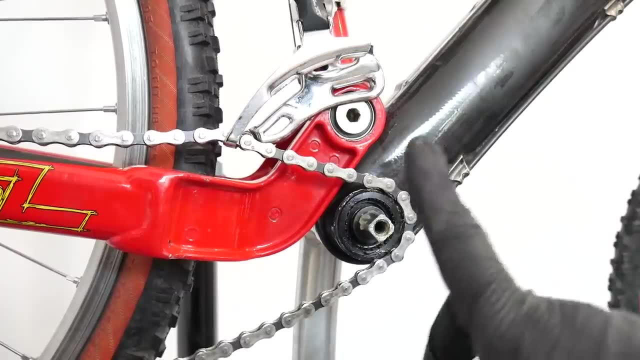 both arms to each other correctly. It is also a good idea to set the chain like that. It will make our job easier when the crank arm is already on the axle. When fastening the right crank arm, just be careful not to hurt yourself against the chain. 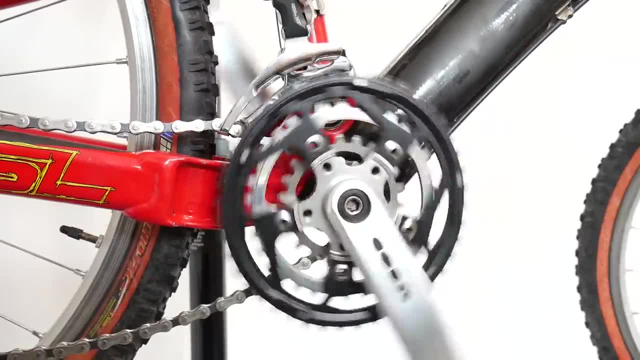 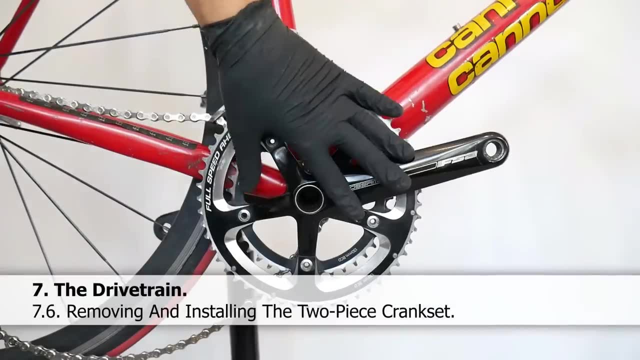 rings. otherwise it is pretty easy job. The job is done. we can now set the chain on the chain rings. How to remove the two-piece crank set and its bottom bracket. The two-piece crank set means one arm of the crank set will be integrated with the. 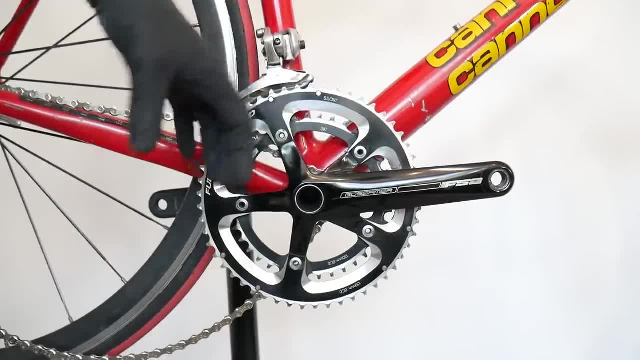 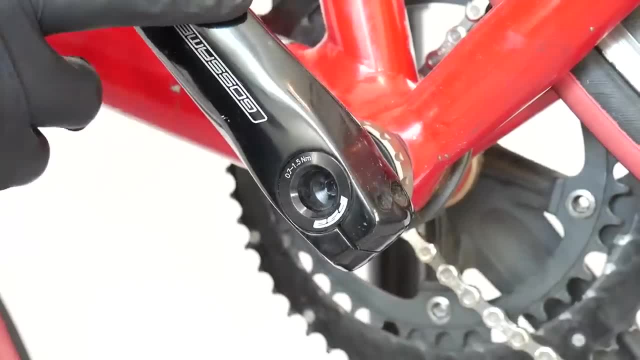 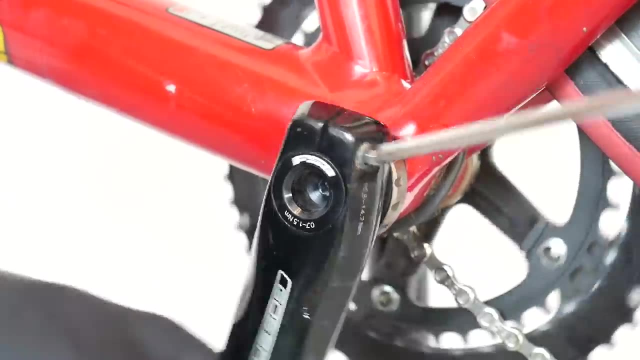 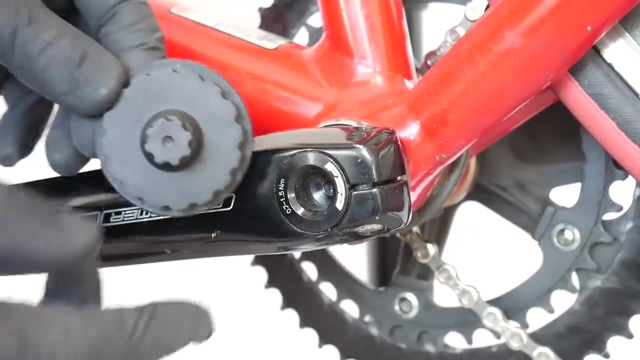 axle with the spindle and then the other arm will be assembled onto it. This operation we are going to start by unthreading the bolts which are fastening the other arm to the spindle. Then we are unthreading this preload nut In case of Shimano crank sets. 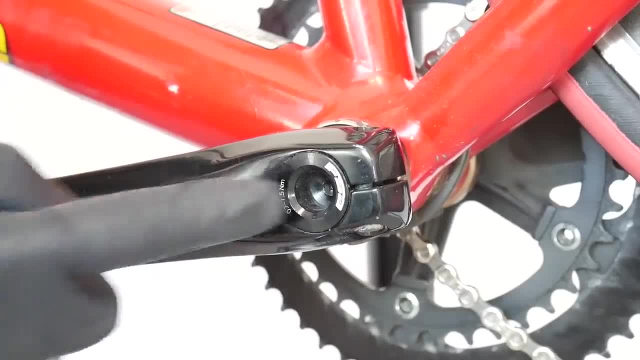 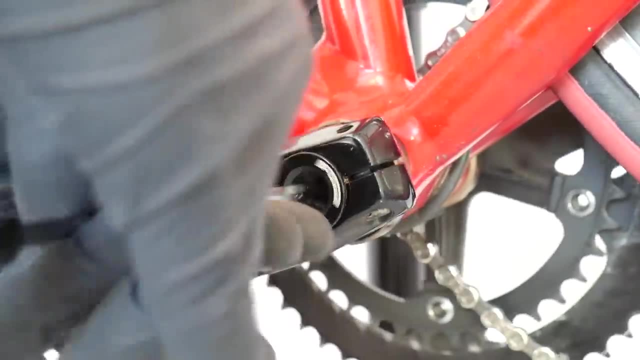 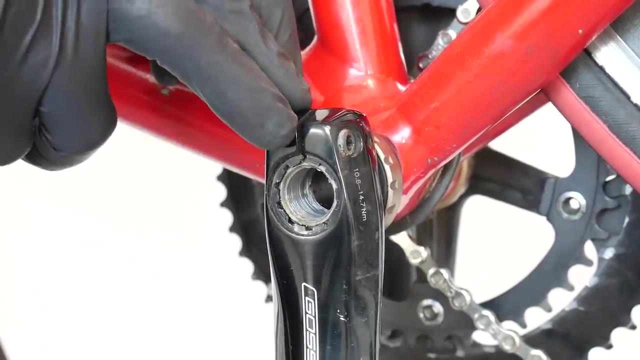 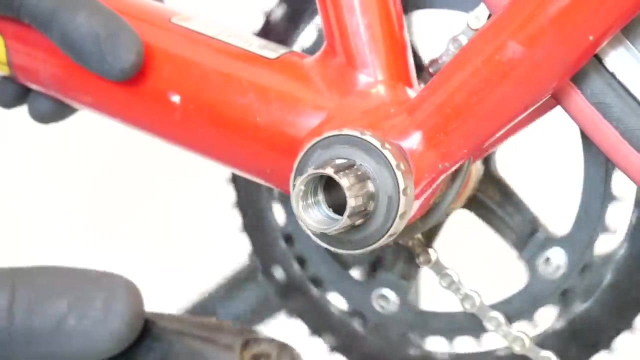 We might need some special tool On this, for example FSA Ghost Summer crank set. we are using the same 5mm allen key On some Shimano crank sets. we are going to have to open a special safety lock right here On this crank set, though we can already remove the crank arm. 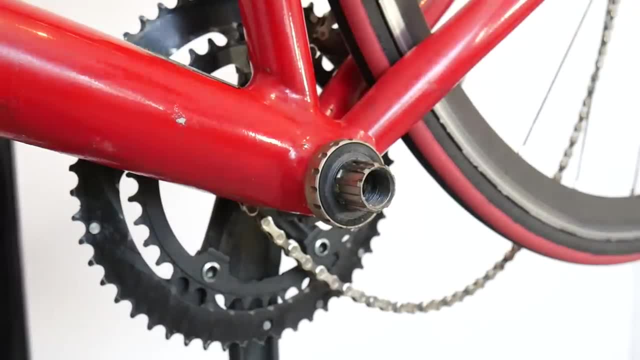 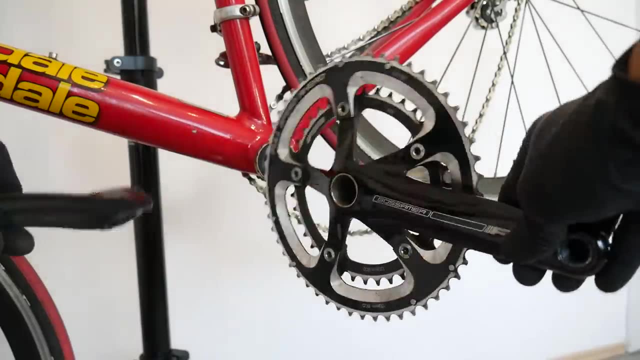 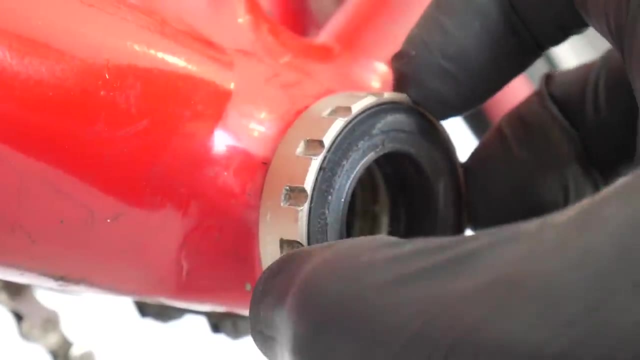 To remove the other side. we don't need any additional tool, maybe just the mullet. Now we clearly see why is this system called a two-piece crank set. We are now on the non-drive side of the bike, so the left side, and we can see this arrow. 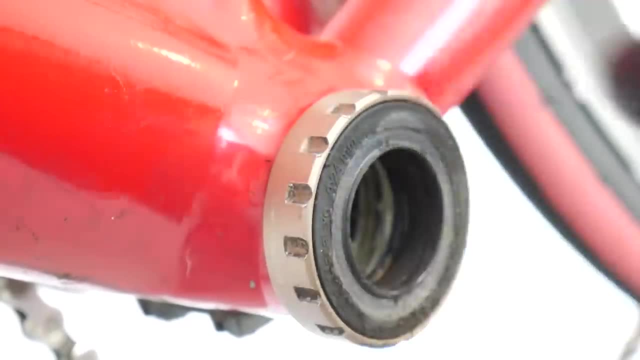 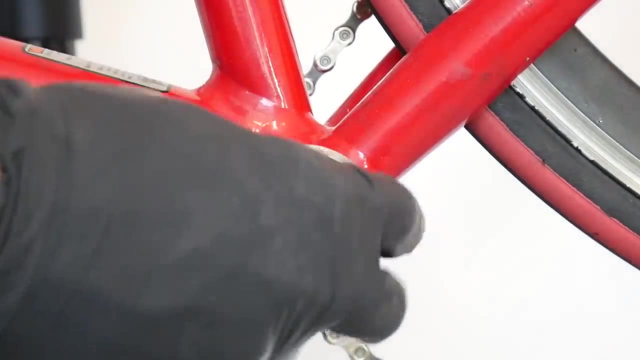 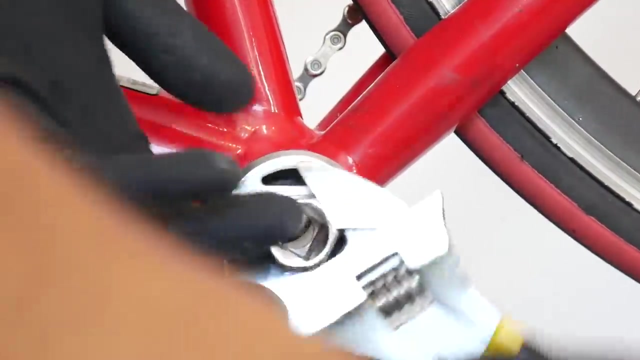 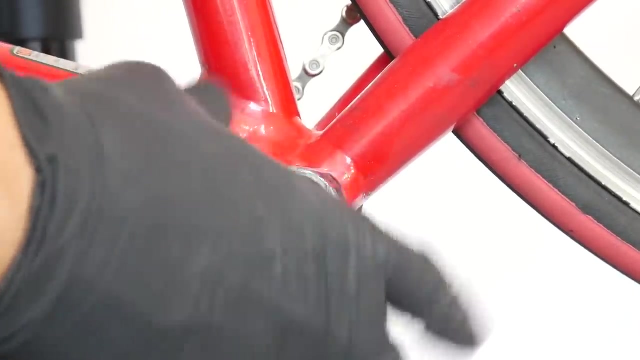 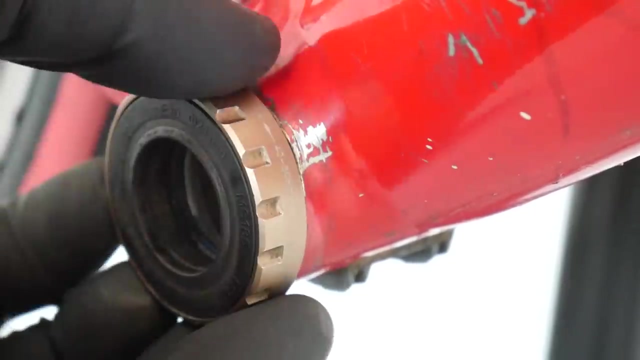 which is indicating the tightening direction. So we are going to unthread this counterclockwise. Now we are on the drive side of the bike and we can see the arrow which indicates tightening direction. So we are going to unthread it clockwise. 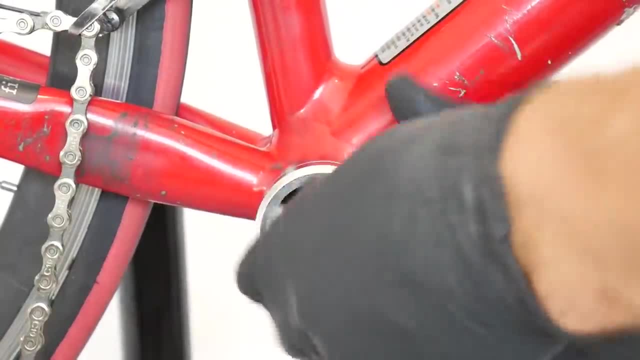 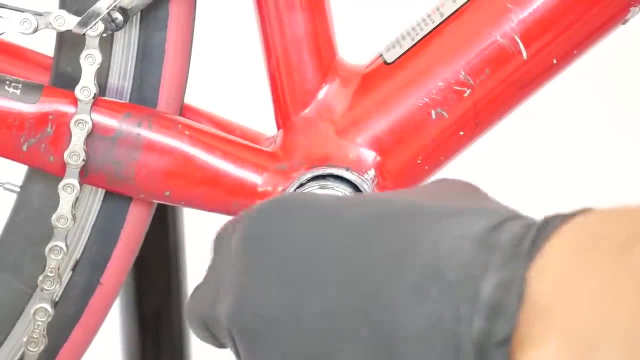 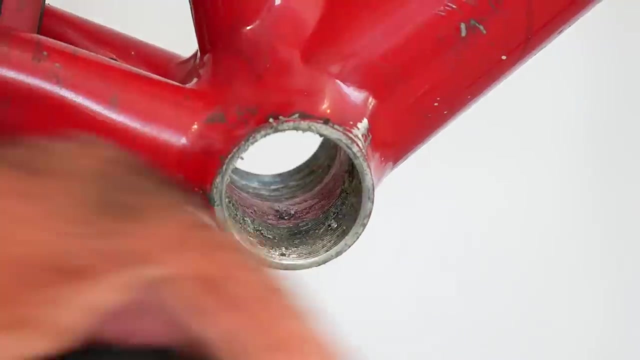 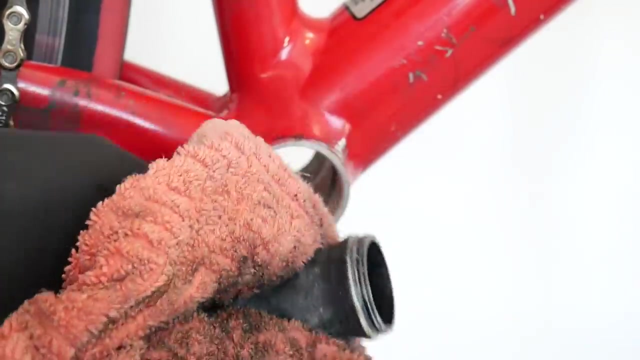 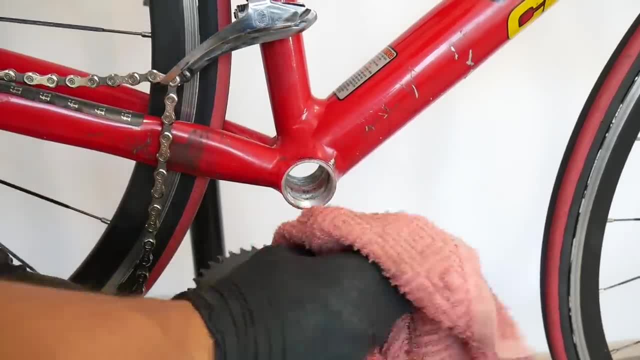 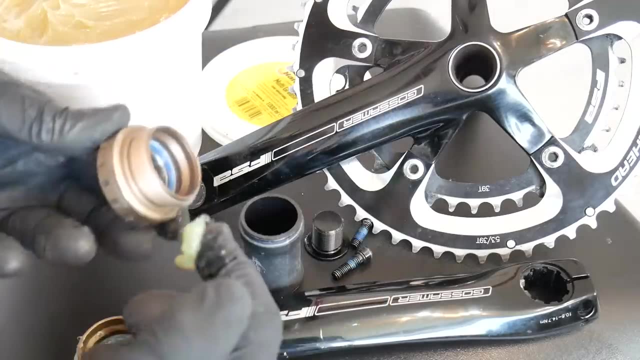 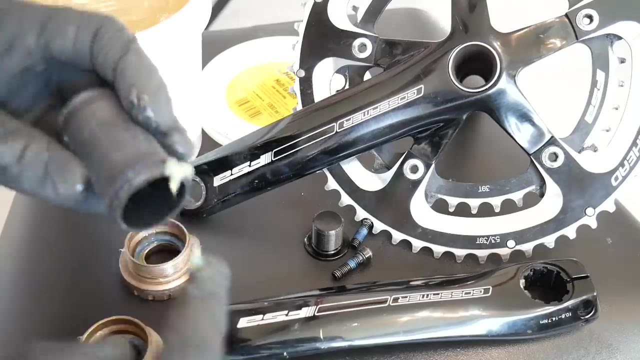 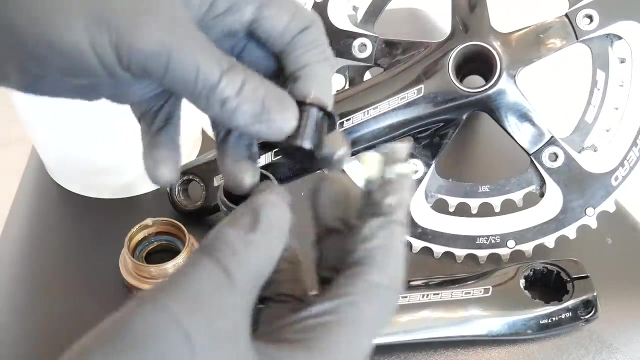 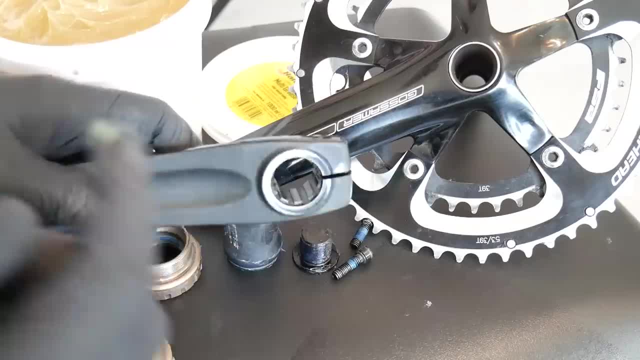 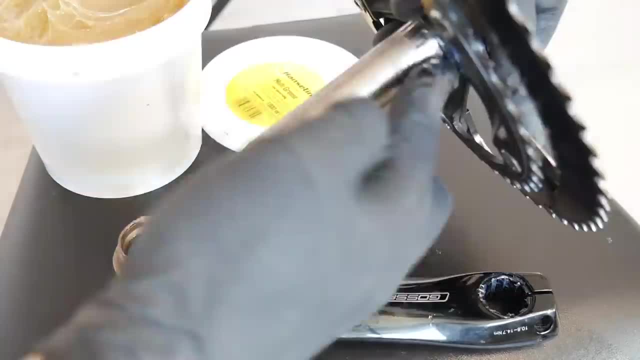 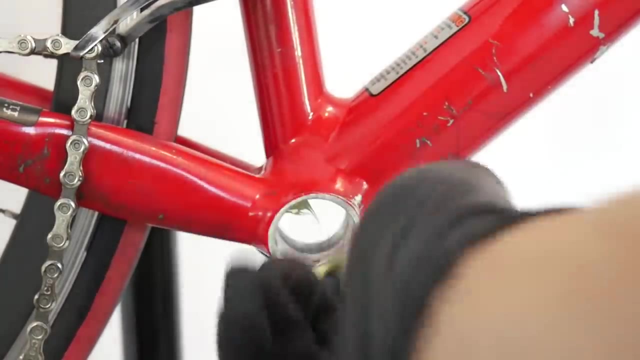 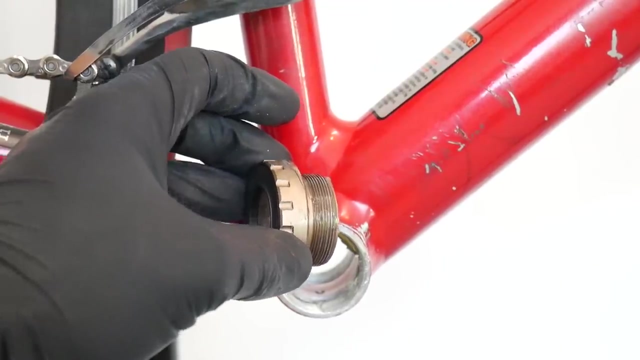 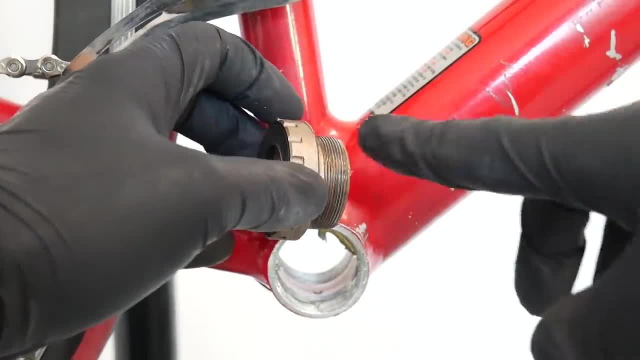 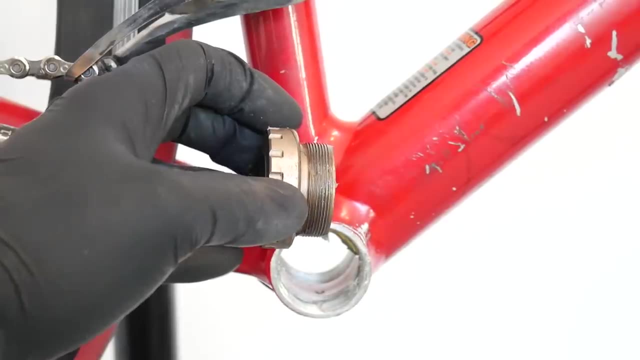 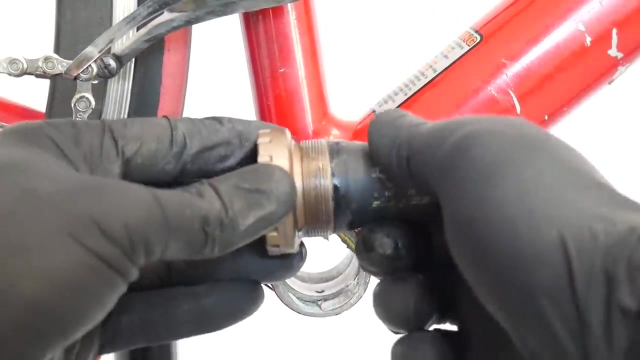 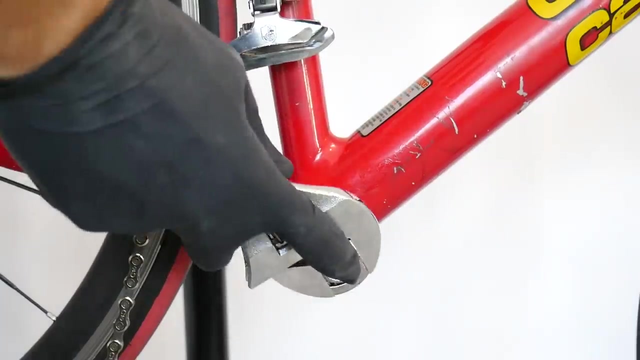 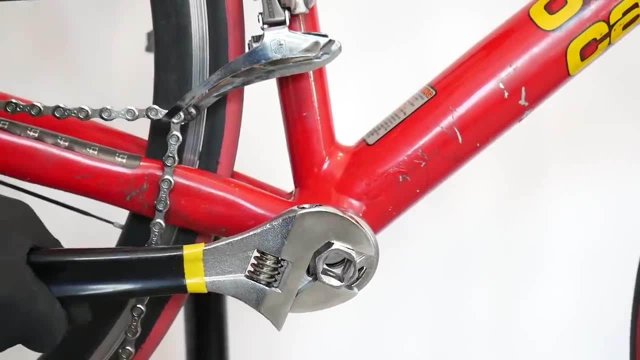 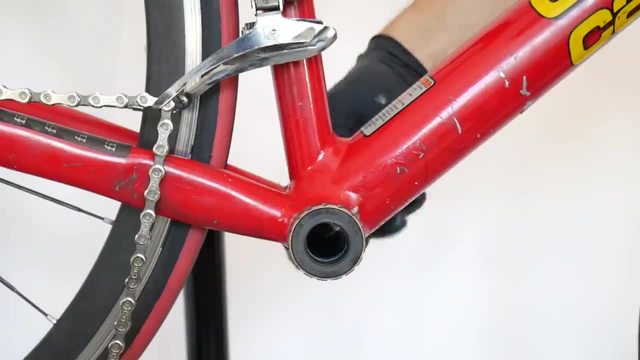 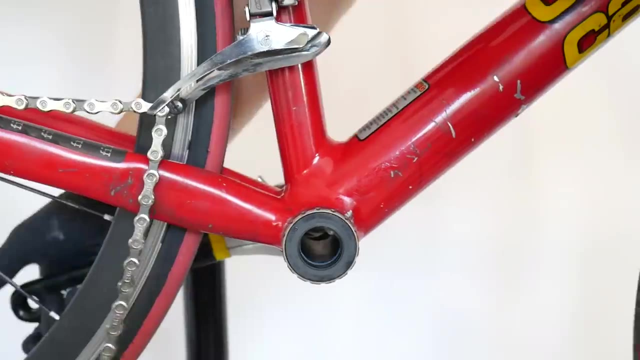 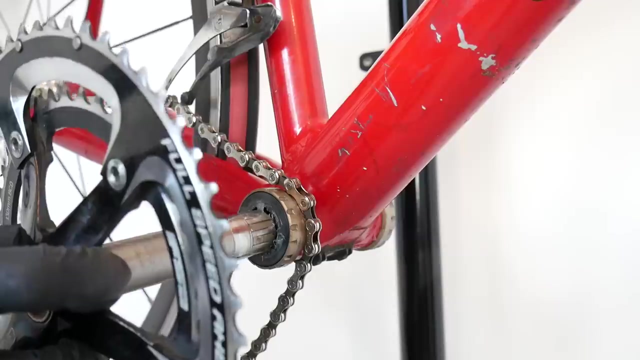 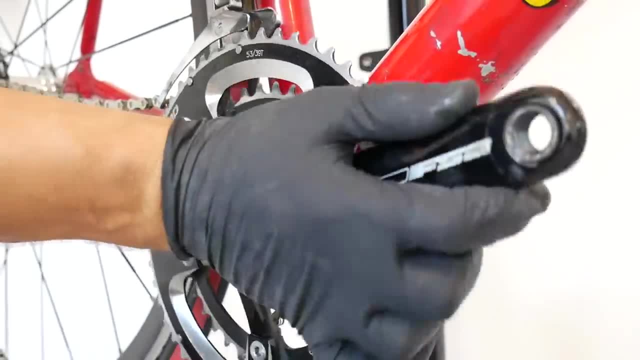 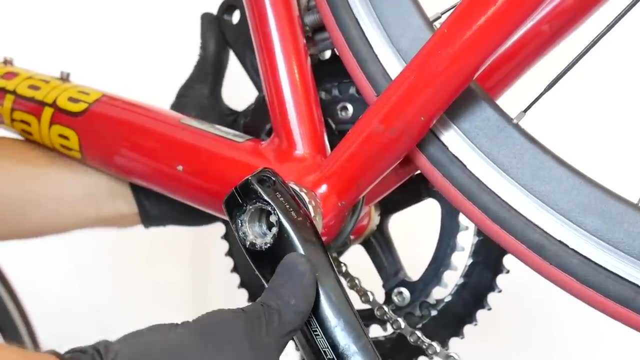 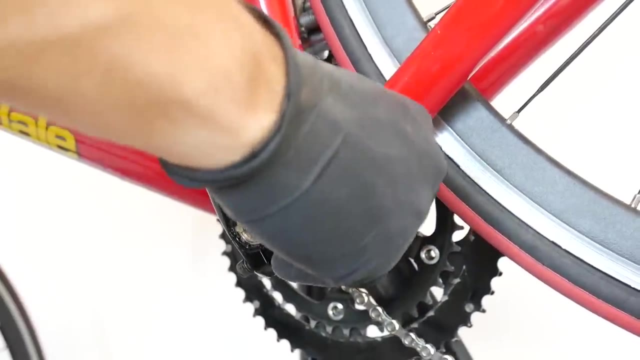 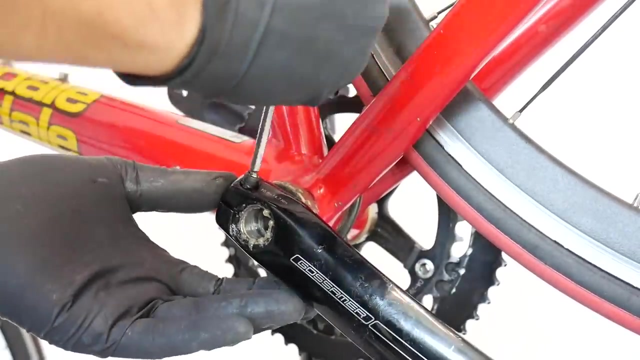 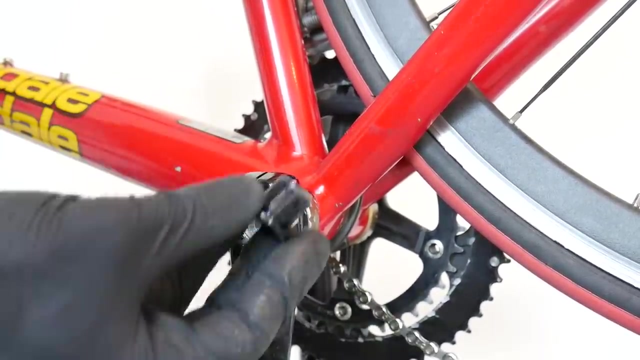 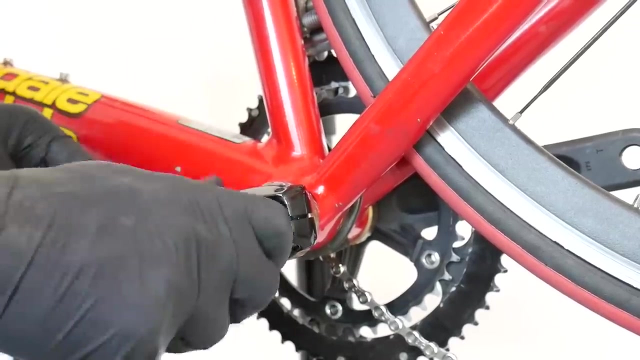 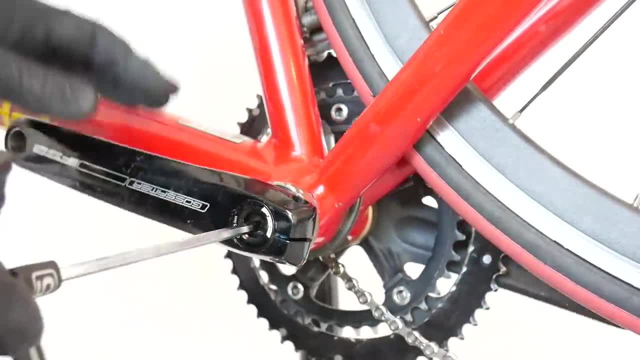 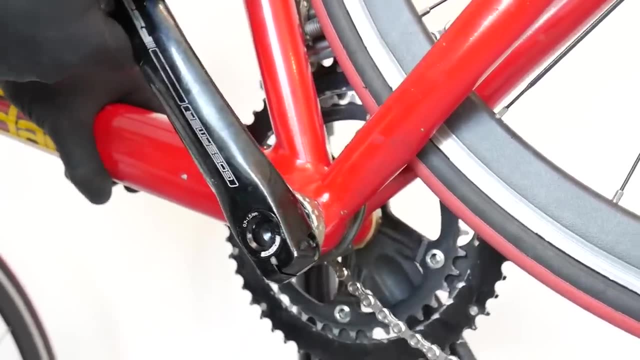 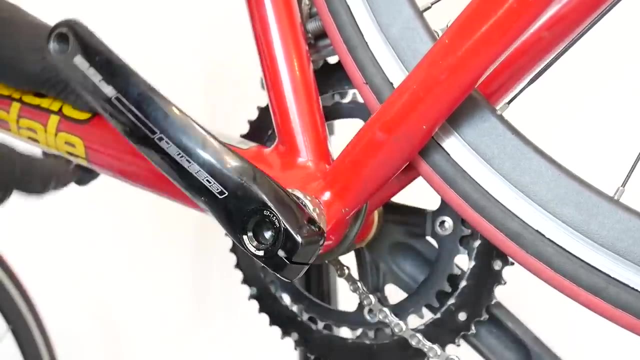 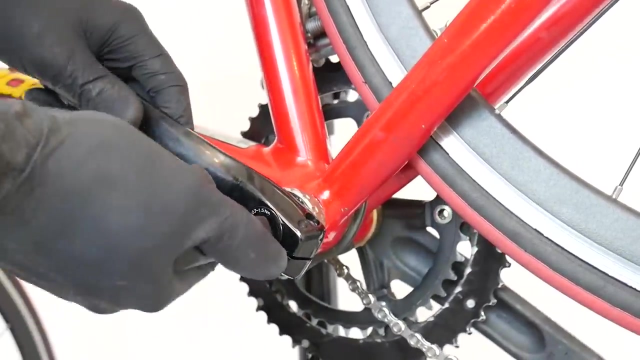 If we don't fasten this nut well enough, there will be some play on the crank arm, on the bottom bracket bearings. If we over-tighten this one, then the crank will not spin freely, So we should find the right spot. As long as we don't have any play on the bearings, then we don't need to tighten it up. 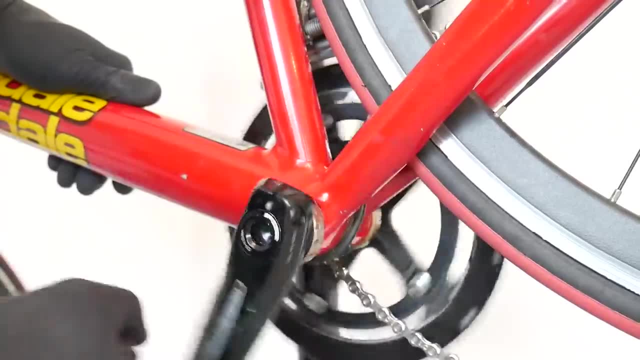 So we should find the right spot. As long as we don't have any play on the bearings, then we don't need to tighten it up. Let's crank it even more. Just no play And a pretty smooth operation. That's good. 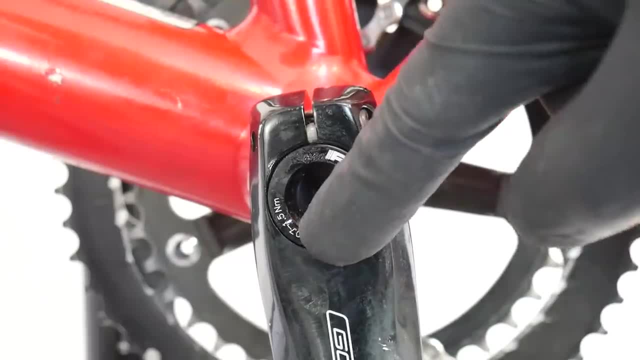 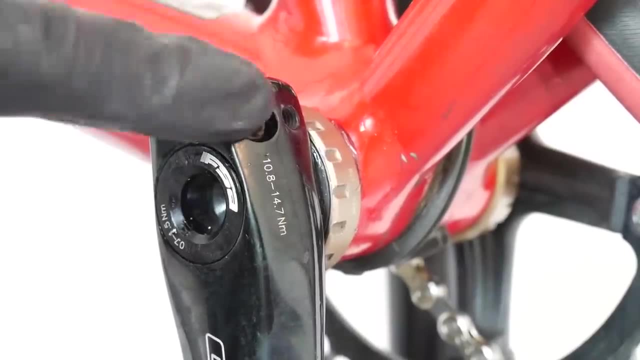 Let's crank it even more. Just no play And a pretty smooth operation. That's good. This nut is fastening somewhere in between 0.7 and 1.5 Nm. This is recommended torque for fastening bolts. This is NOT a lot of torque: 10.8 Nm. maximum is 14.7 Nm. 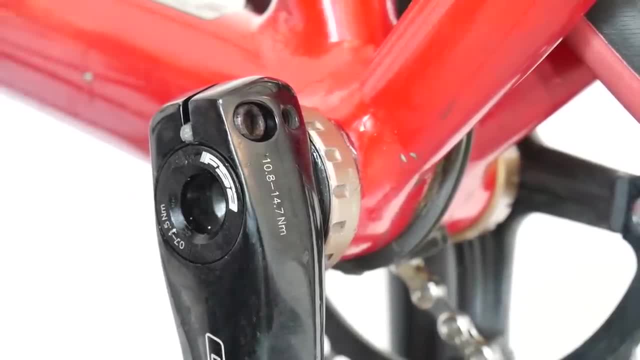 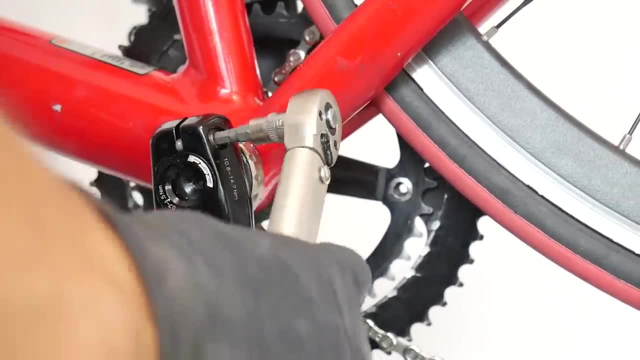 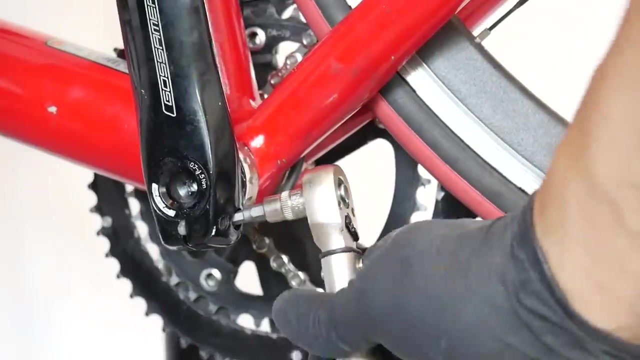 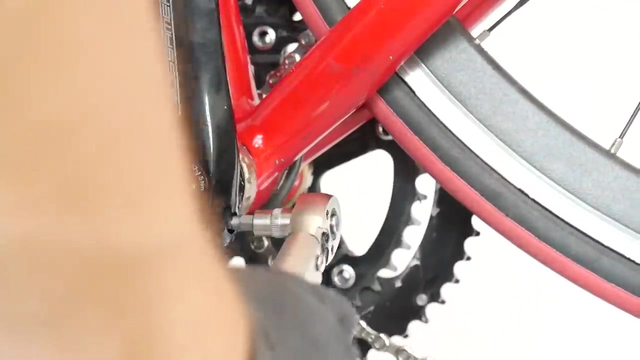 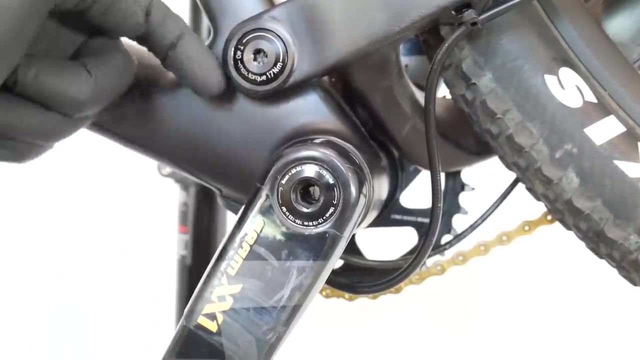 This is recommended torque for fastening bolts. This is NOT a lot of torque: 10.8 Nm. maximum is 14.7 Nm. this is also the two-piece crankset, so one crank arm is integrated with the spindle inside, but this one has the self-extracting system. here we have the 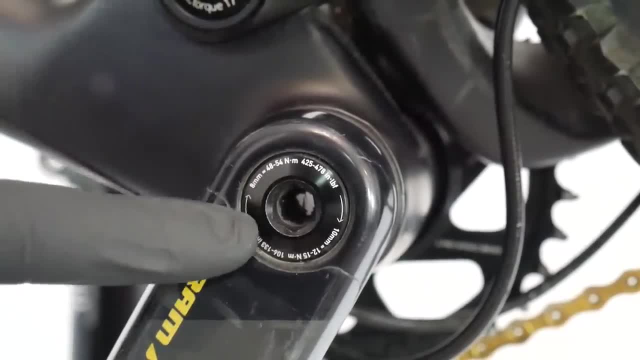 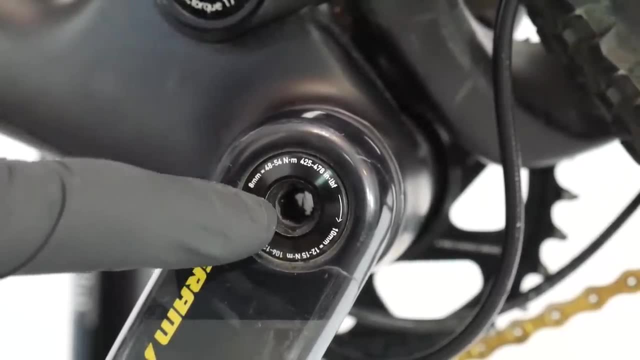 cap which will fit the 10 millimeters allen key, but we are not unthreading this one and then inside you can see a smaller one. this is a bolt: 8 millimeters allen key. when unthreading the bolt will be pushing against the cap and the cap. 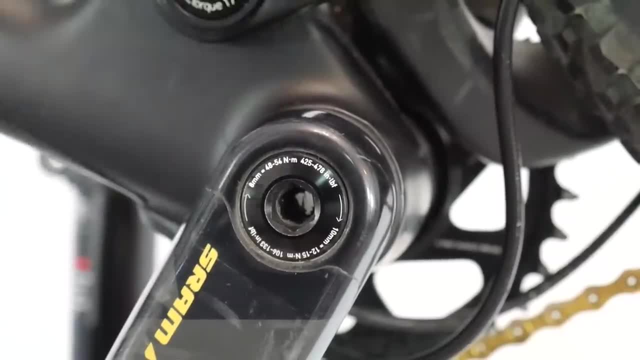 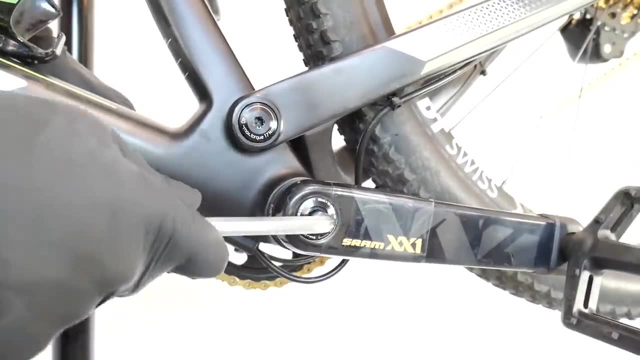 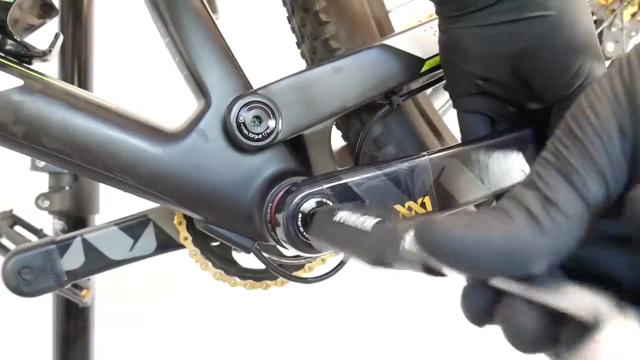 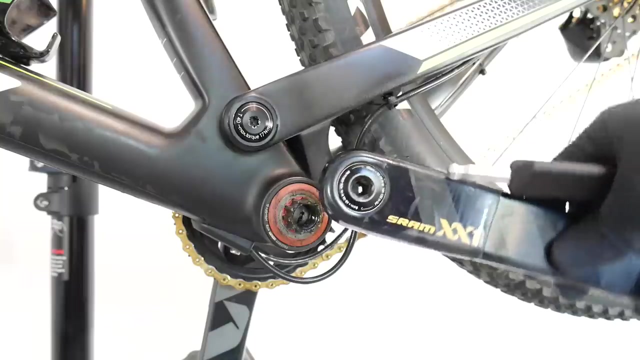 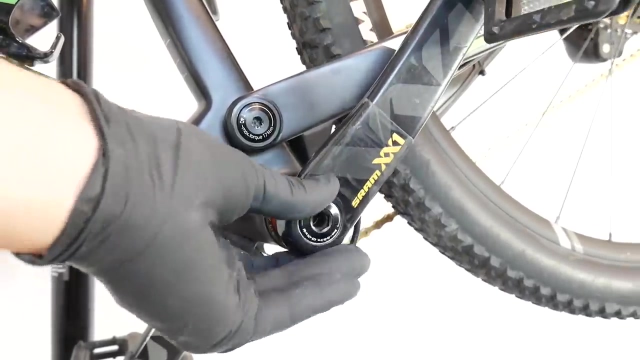 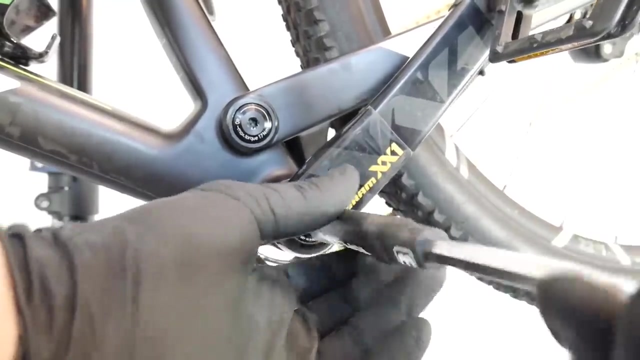 is assembled to the crank arm, and so we're gonna remove the crank arm. in this way, the assembly is as easy as the removal. we're gonna use the same exact bolt to push the crank arm onto the spindle. it says here that for the 8 millimeter bolt we should use the torque between 48. 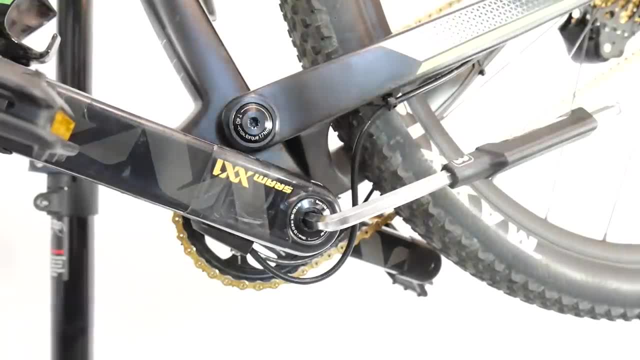 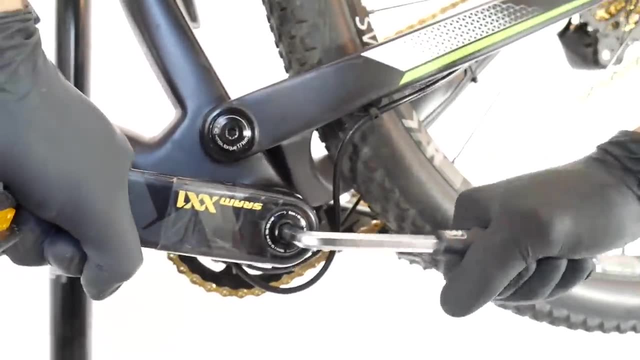 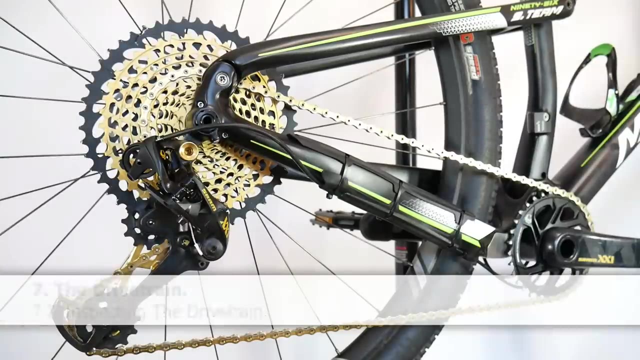 and 54 newton meters, which is pretty much brighten up for our bike. we are gonna use the torque between 42 and 53 newton meters and that's gonna be set to the percent you want to, and after chỉing the cam it's gonna be a little bit more Clear. 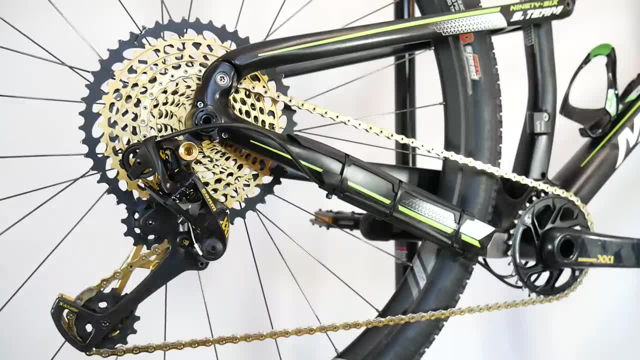 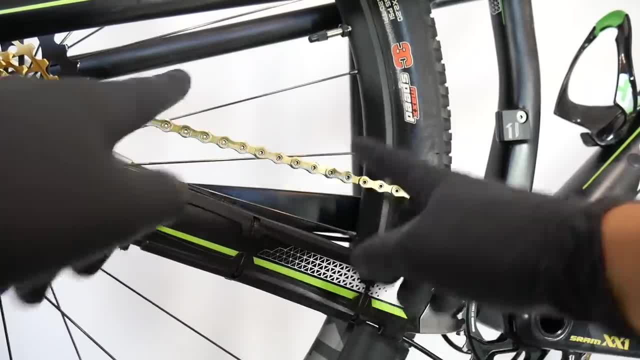 and for that we use a super cheap tool, which is the chain wear indicator. before I show you how to do it, I need to address one common question in this topic, and it is: do we replace the chain on the bike with aำ on the bike when it starts slipping through some of the sprockets on the 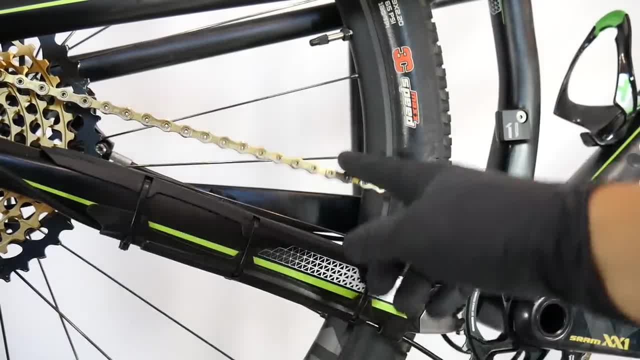 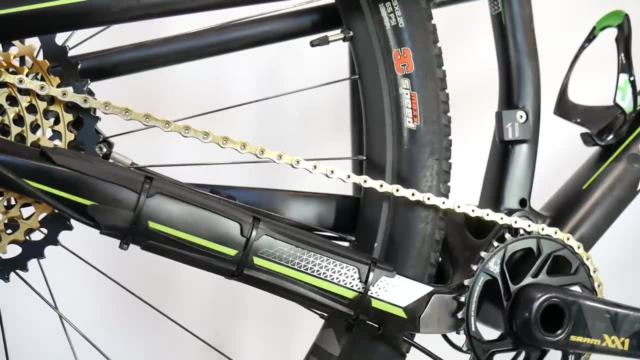 cassette. I'm gonna answer with the question: do we replace the time belt in the car after it snaps? Of course not, because then it's way too late. so it's same with the chain on the bike, when it's already slipping through some of the sprockets. on the cassette, it means it's really, really in bad condition, and 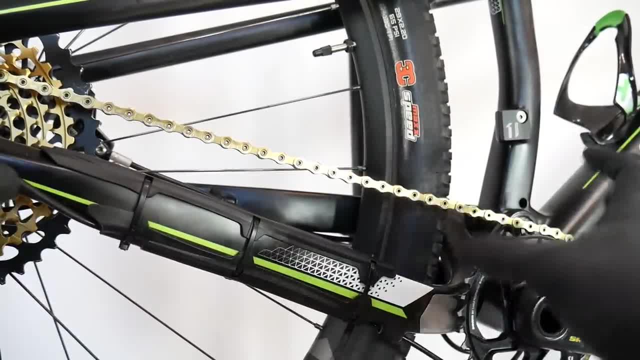 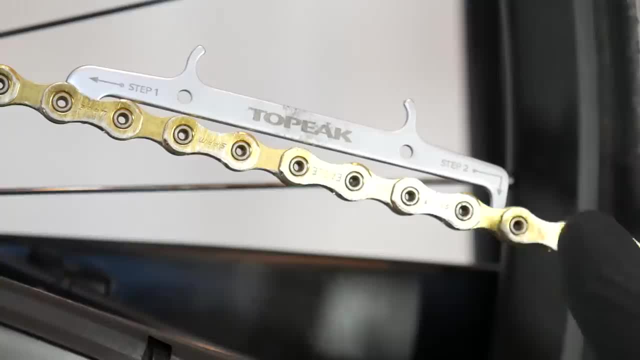 you're gonna have to replace most of the parts on your drivetrain Now check out this trick. I am done inspecting my drivetrain. It is that easy, that quick and pretty accurate. This little tool is the chain wear indicator. We are just 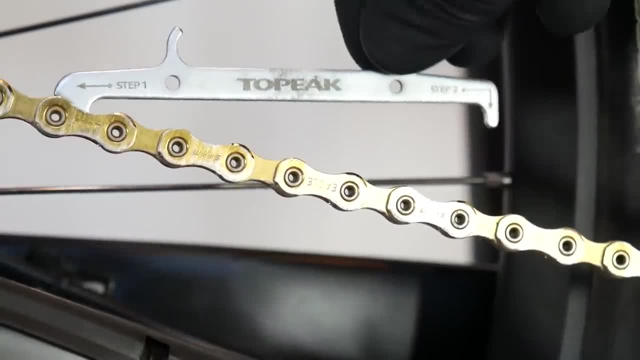 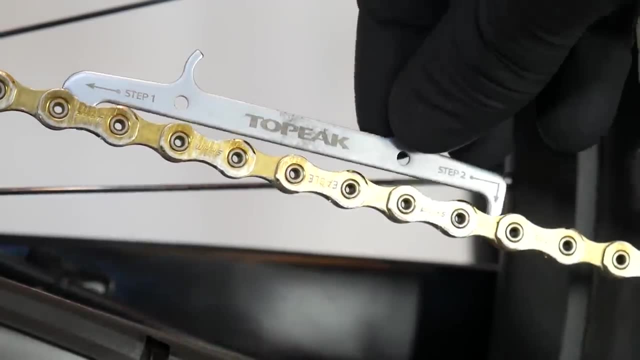 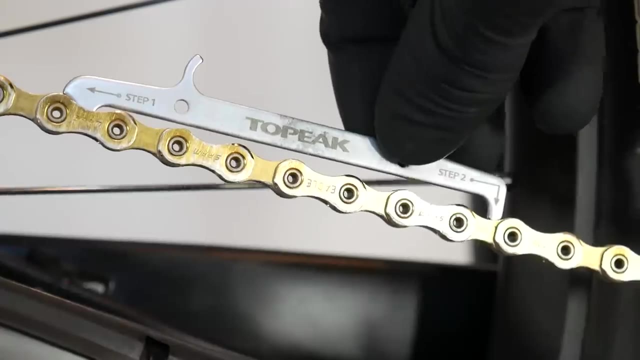 putting it on the roller of the chain with the one arm and the other arm will just lie down, like this, If the other arm will not go in between the rollers or the links, so like that, if it doesn't fall down, that means this: 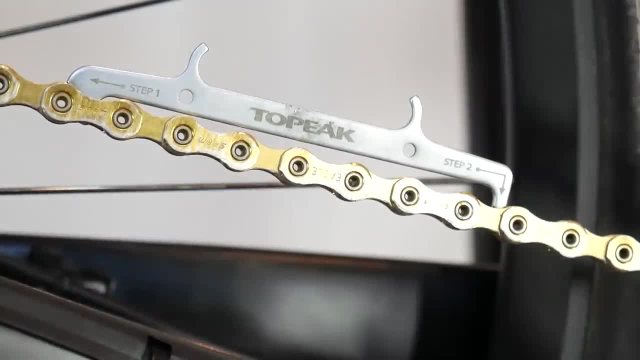 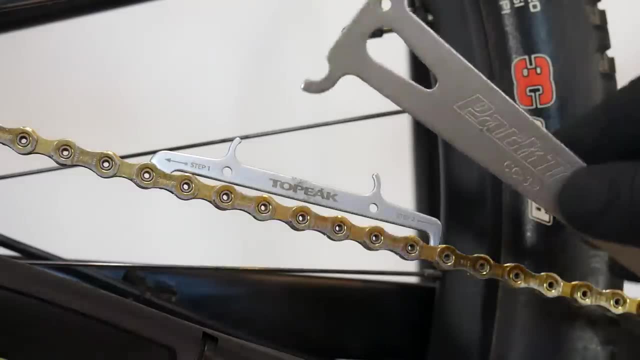 trick is done. The chain is still in very good condition. I don't have to replace it and I'm not wearing down my cassette and the crankset too much. If you get to like this game, we can be even more precise in measuring this. So let's just remove this one, This chain. 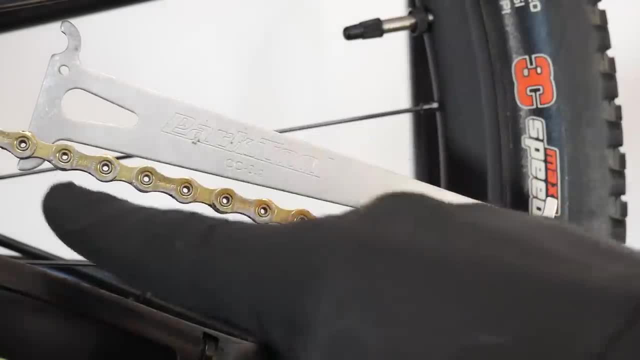 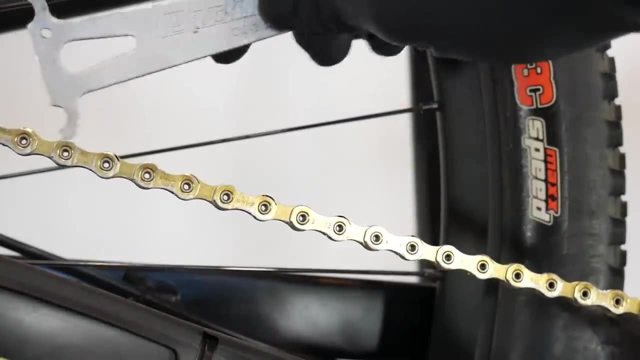 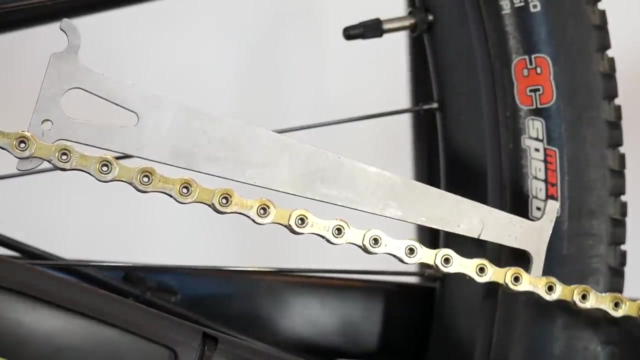 indicator is longer and has two sides. One side will indicate the 0.75% of the extension, and the other side- we're gonna use it like this- We'll indicate 0.5% of the extension. What it means for us is that when the 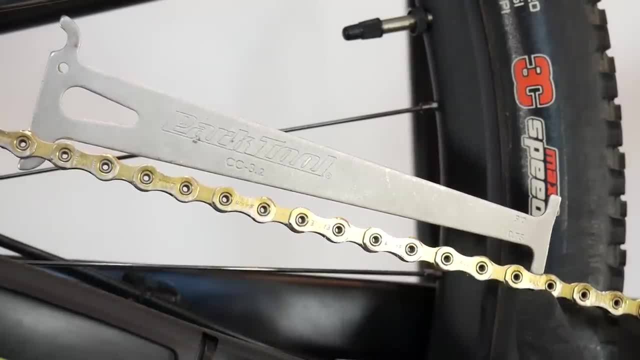 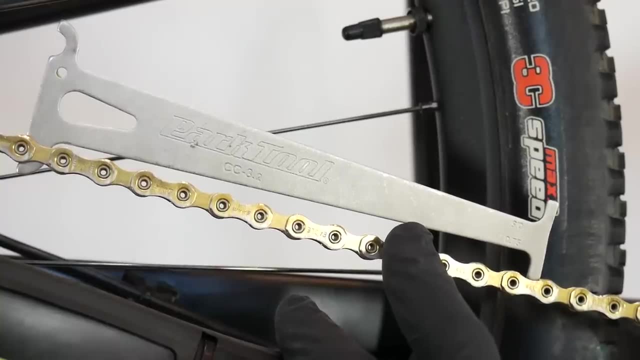 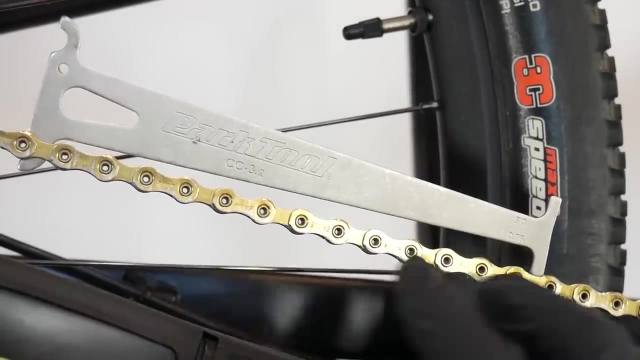 extension of the chain is already 0.5%. that would mean it's good to replace it if we have titanium or alloy sprockets on the bike, because they just wear down more quickly, And if it reaches 0.75% we should replace it, whatever drivetrain we. 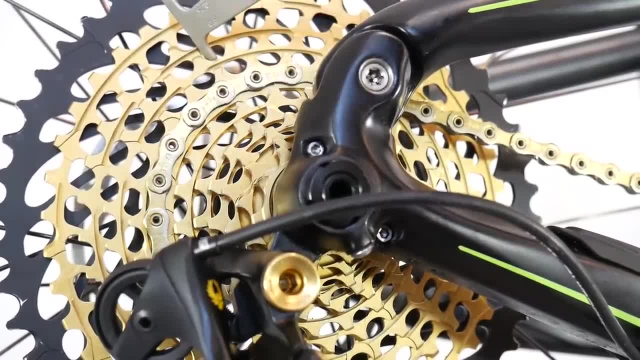 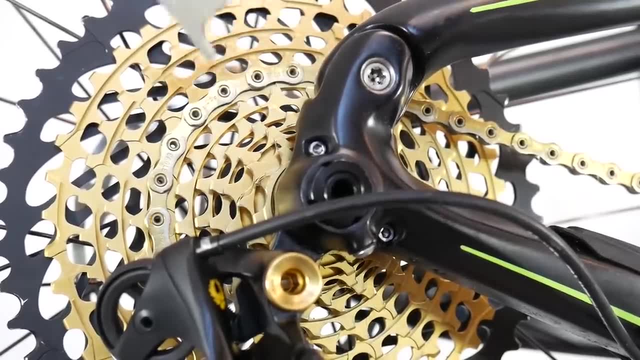 have, Of course, the sprockets on the cassette or freewheel, and the crankset will eventually wear down. So let's take a look, We're down. but if we do replace the chains regularly, the cassette should have a lifetime. of many chains That means many thousands of kilometers In some. 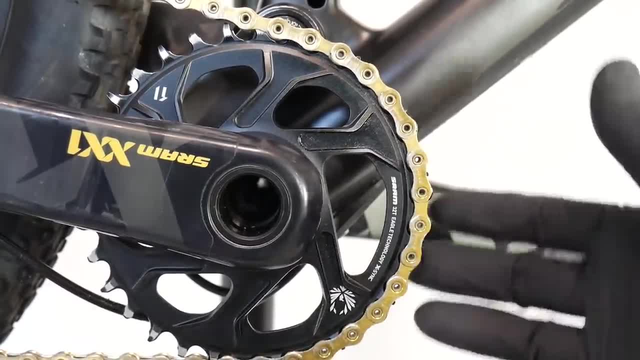 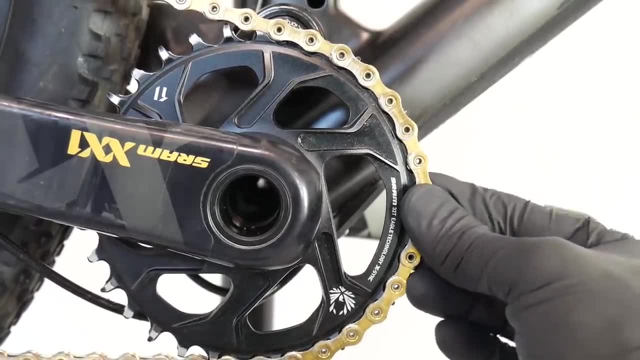 emergency cases. let's say we are visiting our friend or the relatives and we are inspecting their bike. We don't have the chain wear indicator with us. We can try to pull the chain away from the chainrings on the crankset and see how. 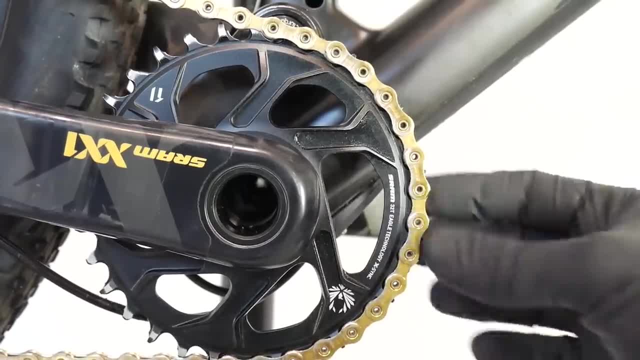 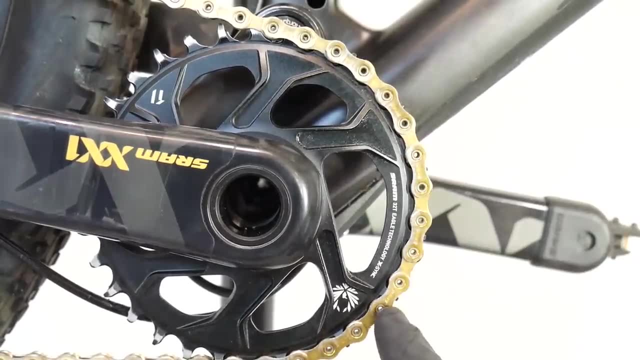 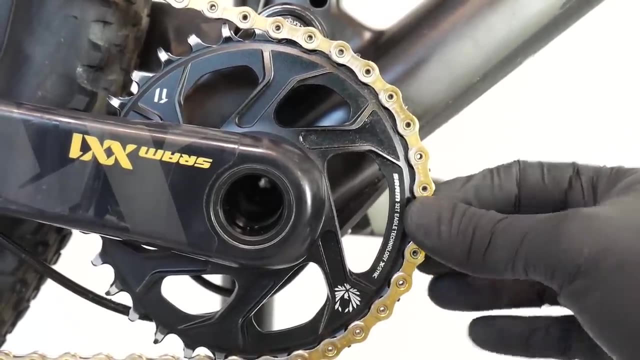 much it moves. As you can see, this chain is almost new It is and it's very difficult to pull it away of the chainrings. If the extension would be, let's say, around 0.7%, you would be able to pull maybe three. 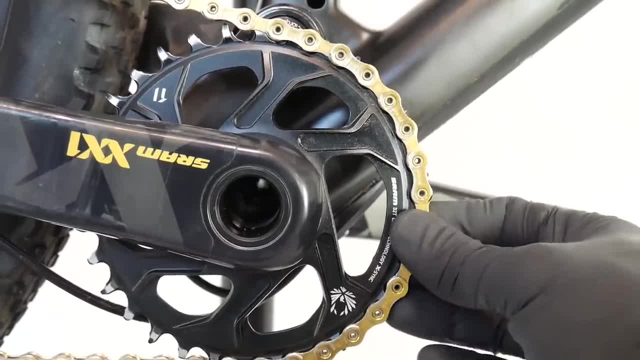 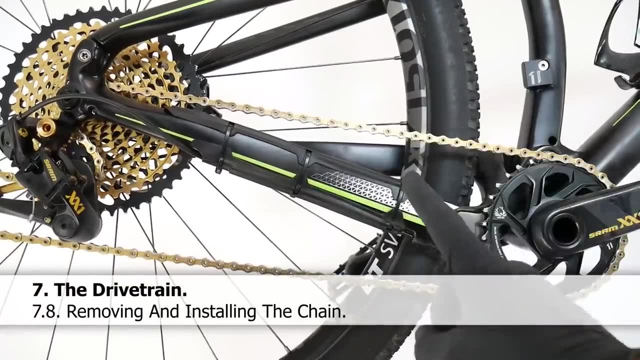 links away, a little bit away from the chainrings, But it's always the best thing to have the chain wear indicator. How to remove from our bike the chain and then properly put it back on, We need to consider two situations. Number one: 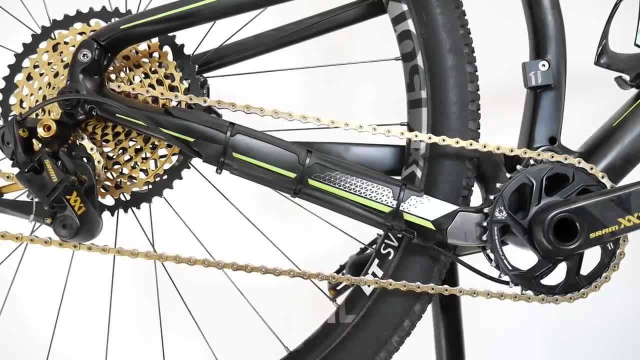 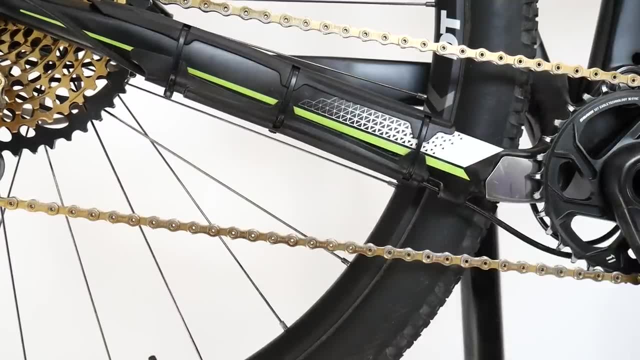 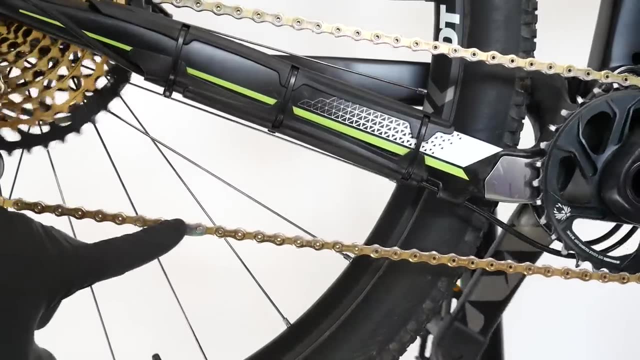 chain with a quick link. and number two, we need to use the tool called chain tool or chain breaker. First off, we need to find out whether there is a quick link on our chain. We can just spin the pedals searching for the link, which will look differently, and that's it. we've got a quick link on our chain. Before removal: 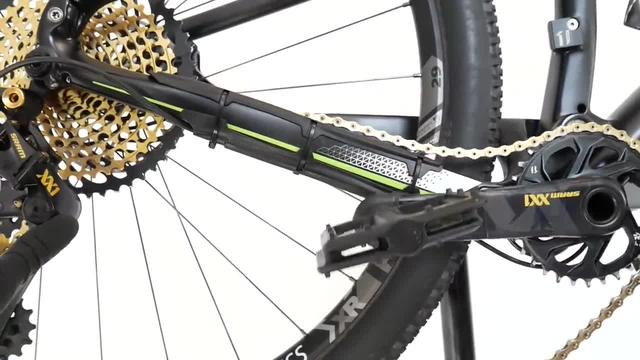 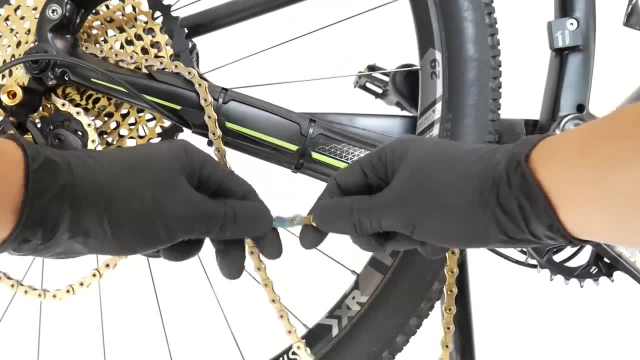 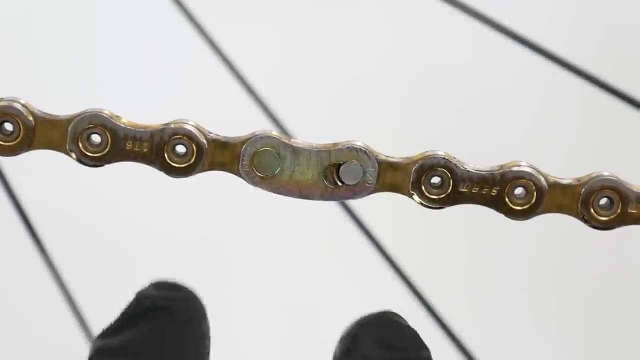 or installation. some will prefer removing it first from the chainring on the crankset so that it will be completely loose. no resistance on the chain. In order to break the chain with the quick link or power link, I'm going to squeeze against each other these links which are 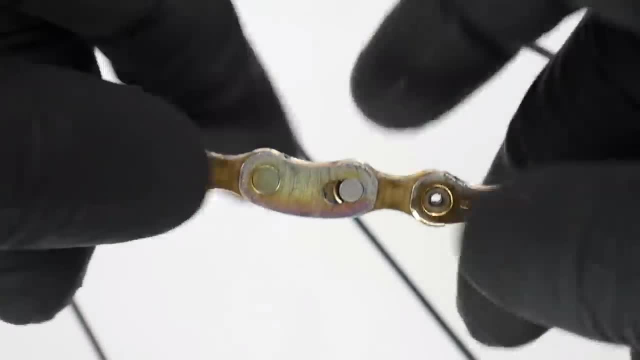 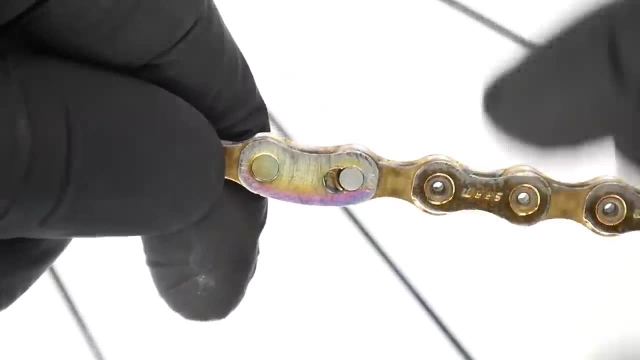 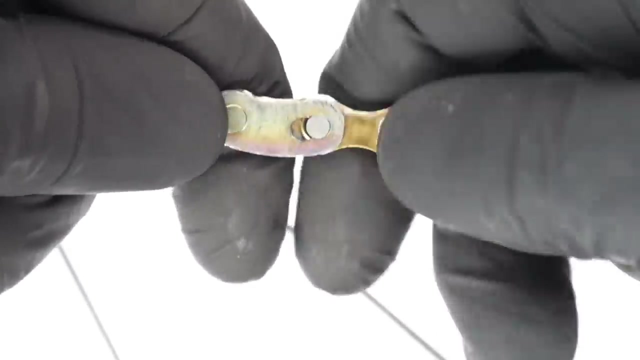 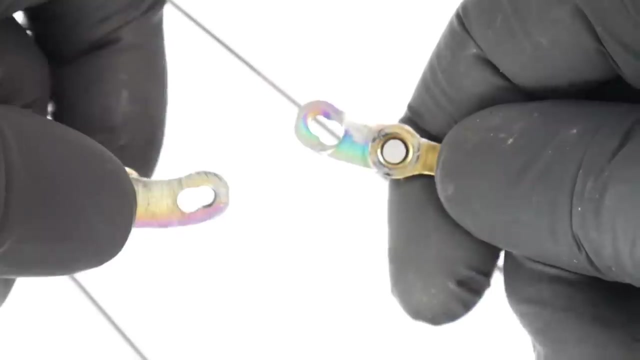 just next to my quick link. Some quick links can be pretty stiff, so doing such a motion inwards and outwards, but just a little bit can help. So now I'm squeezing those and moving the chain. you can see the pin moving here and in the second it will be opened. Now the chain is broken, but still okay Now. 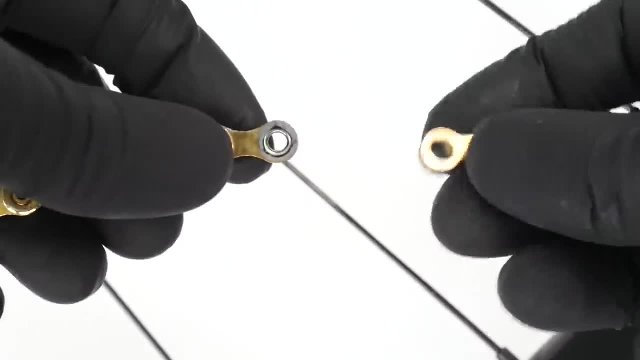 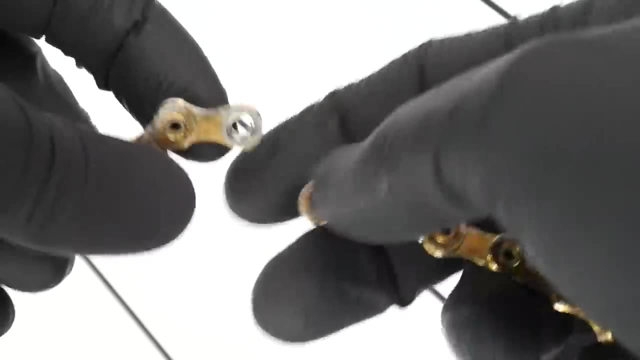 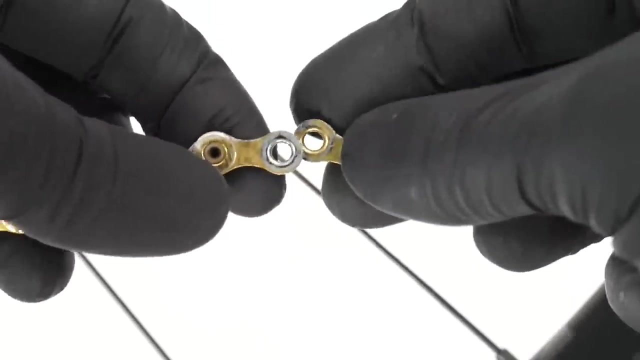 we're going to install the chain back of the bicycle using the quick link. In order to do that, we need both internal links on the left and right side. So this is the internal link, this is the external link. We need two internal corresponding links. Now I'm 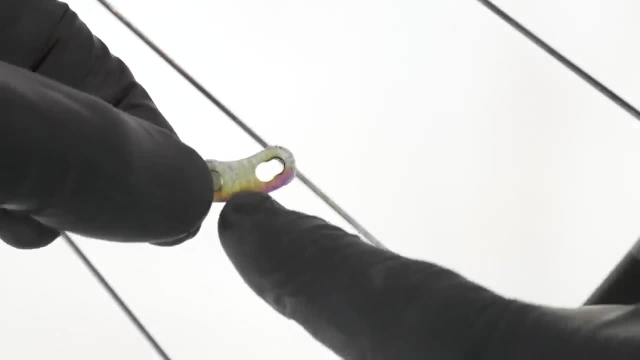 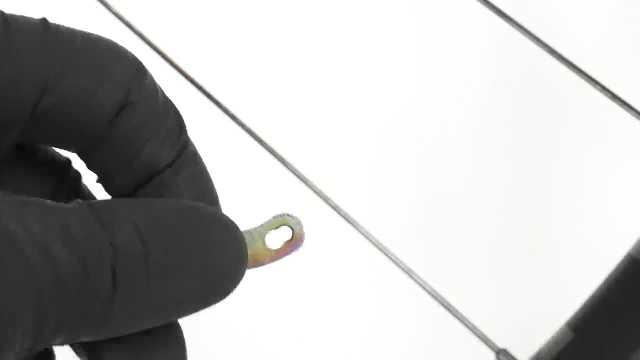 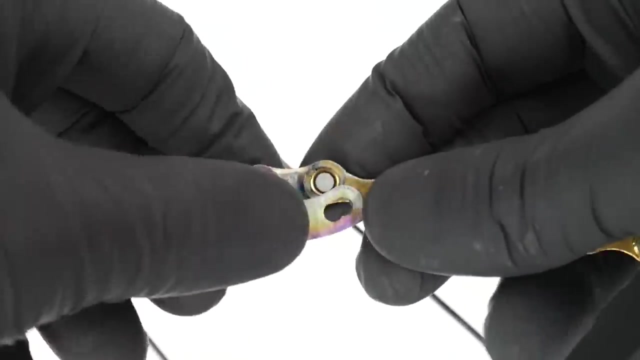 going to show you the internal link. It is very important how we use it and on what side we put it. I'm going to show you that just in a second. So one part on one side and then the other part on the other side. All right, now those pins have. 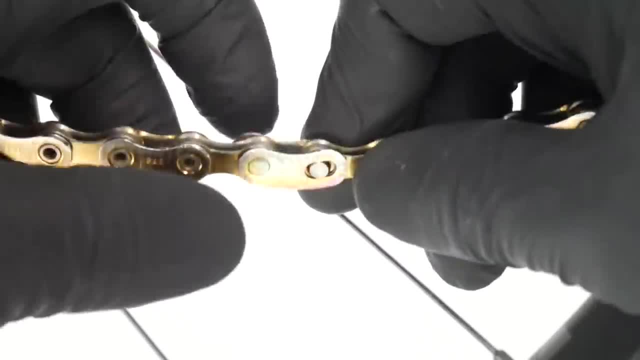 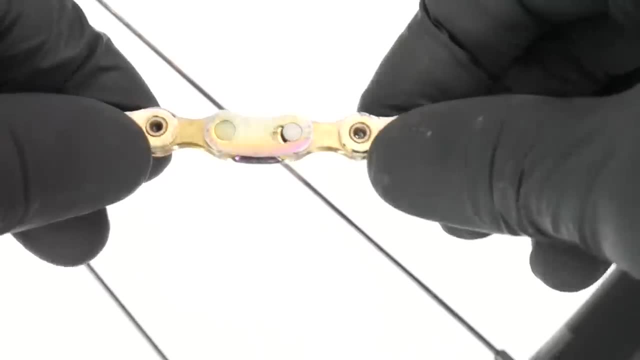 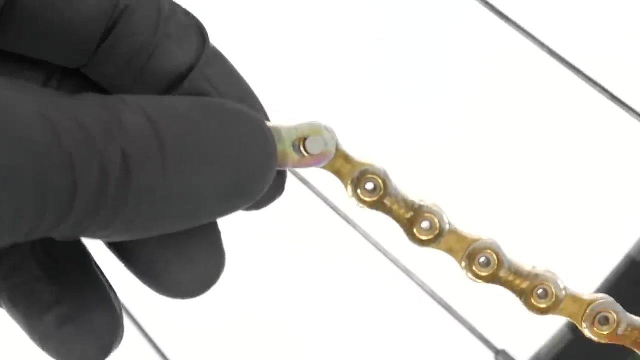 to go into those little holes and now I will just pull those links away from there, just like that. It's a very simple method, but it's very easy to do and it works very well, so I'll show you how I'm using it. So we need two of those. 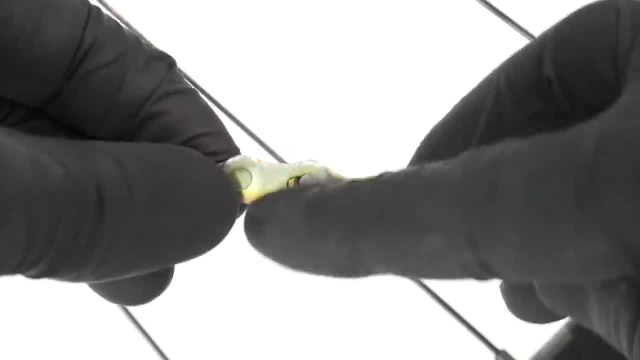 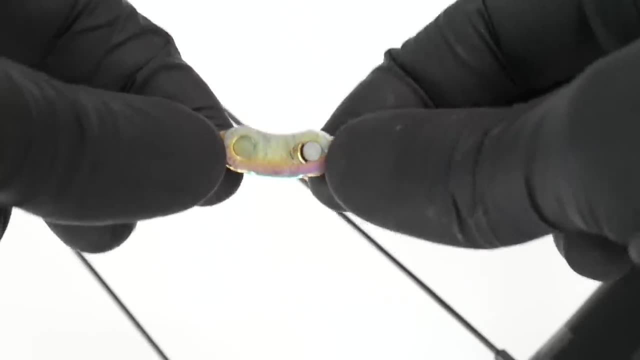 and we have three of those. so we need to pull those links from these two points and we get another one here. just to see how perfect it looks, We stick the chain back onto the crankset and then push the pedals, press on this button, and then we pull the end of the chain and just go like this: Click and it's. 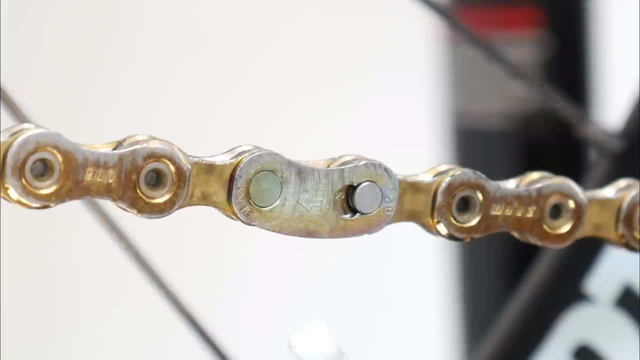 working. Sometimes you need quite a force in order to do that, So you can then put the chain back on the crankset and then push the pedals, Making sure that this quick link is well set and it will just click into its place correctly. When assembling the quick link, we need to pay attention to this little arrow. I hope you can see it well. The question is: why is it pointing now to the back of the bike and not to the rear of the bike? 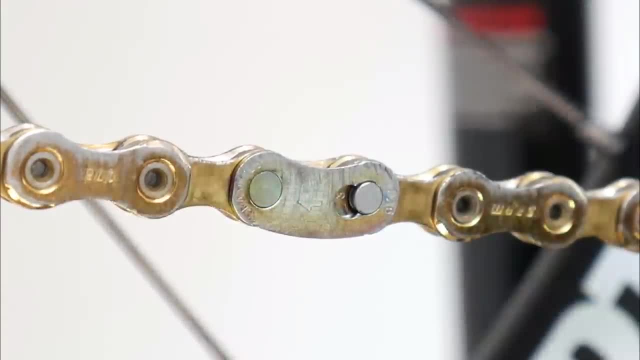 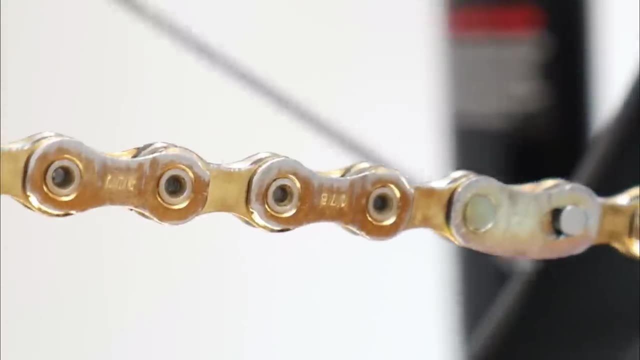 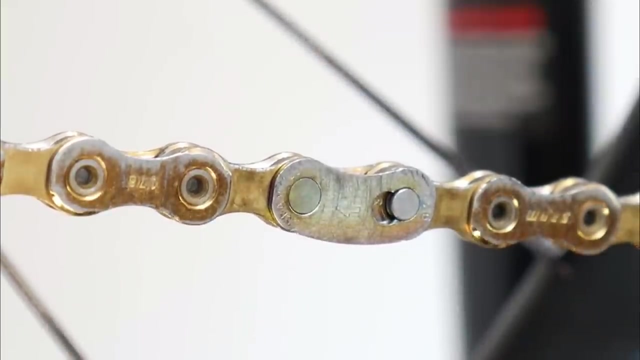 front. Well, it's not indicating the back or the front of the bike. it indicates the direction in which the chain will move while we are pedaling. So if it's below the chainstays, then it will point to the back and above the chainstays it. 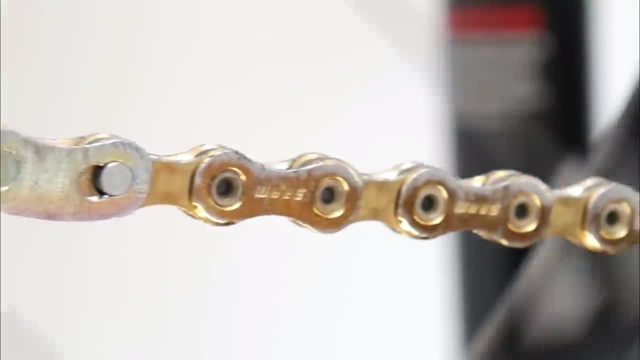 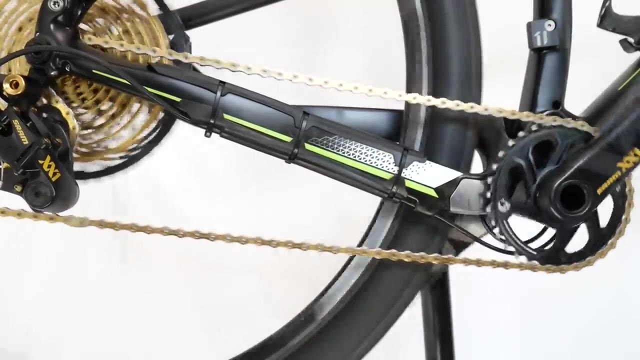 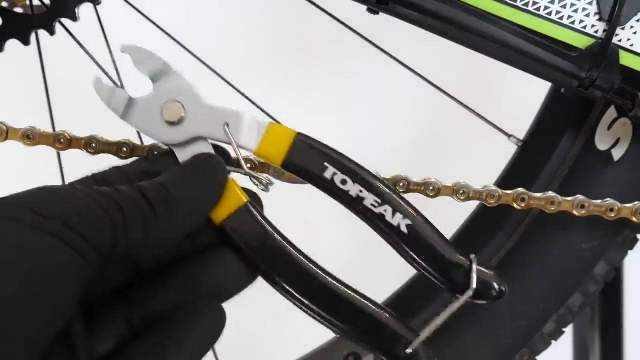 will point to the front, but always the direction of the chain while we are pedaling. So the arrow to the front and now to the back of the bike, Always direction of the movement of the whole chain. We can also use special pliers if 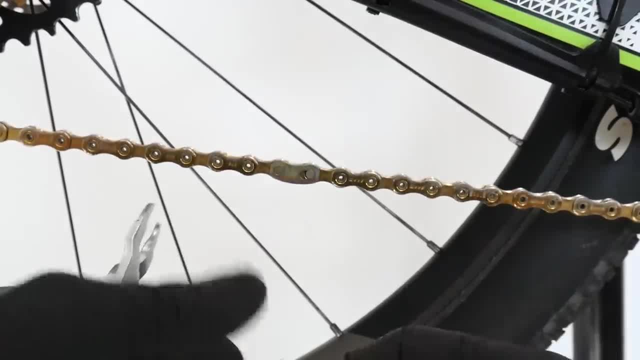 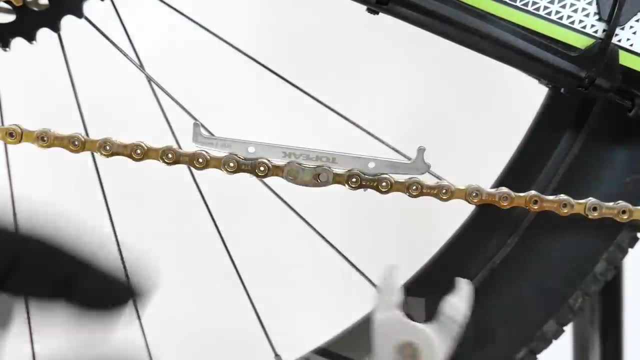 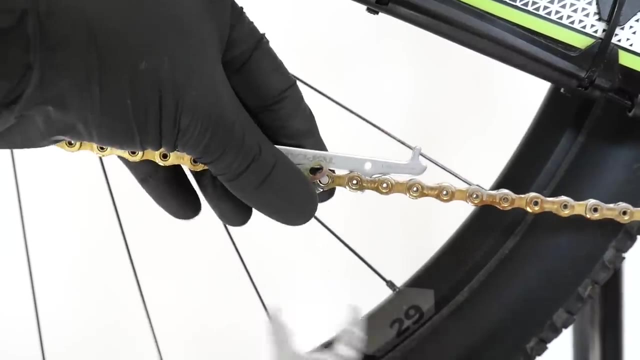 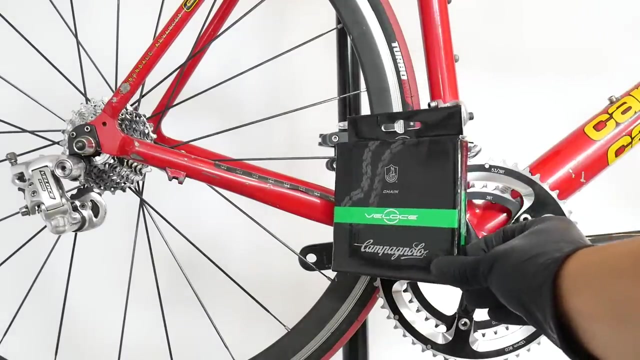 you will to break the chain with the quick link. I have also some smart device that will hold on to the chain, And now we are going to install a new chain on the bike. This will be a Campagnolo chain. We're going to break the chain with a special tool and then 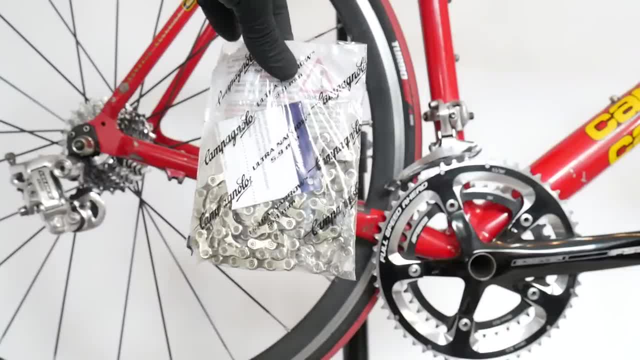 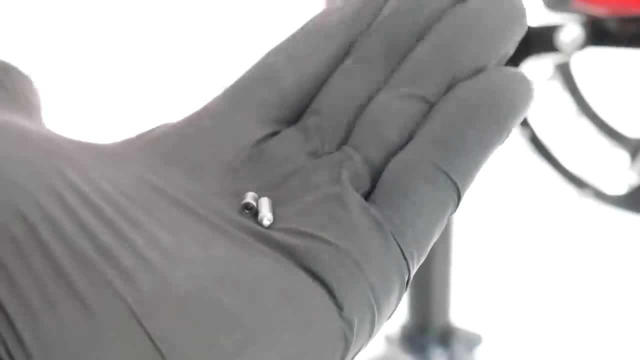 connect it with a special pin. This is our new chain and these are our pins. This one is the guide pin and this one here will connect our chain. The first question we need to ask ourselves is: is this the directional chain? meaning, are these eggs on the outside or on the inside? 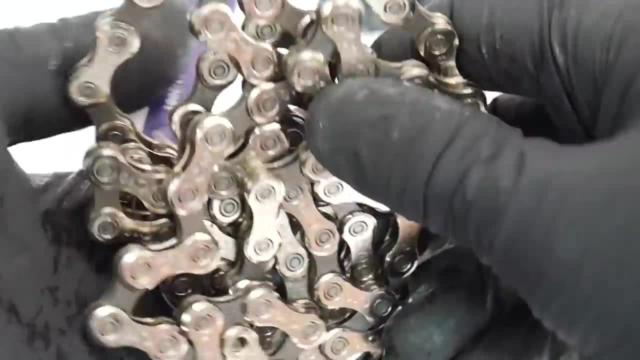 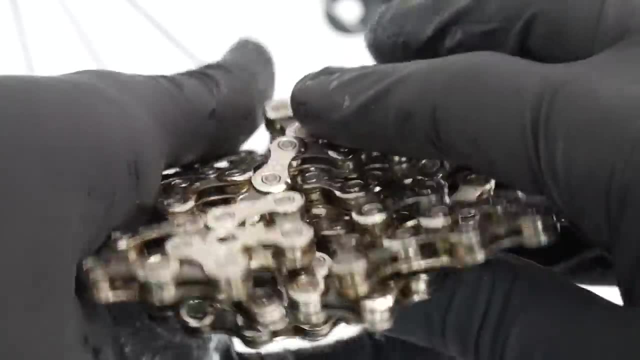 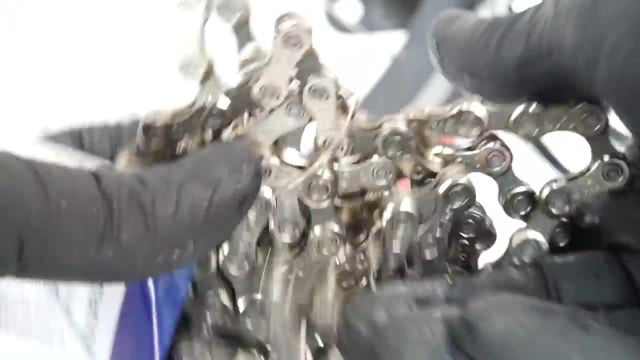 links looking differently on both sides. As you can see, this one has the same symbols- C10- on this side and on this side. That means it is not a directional chain so that we can just assemble it either on this side or on this side on. 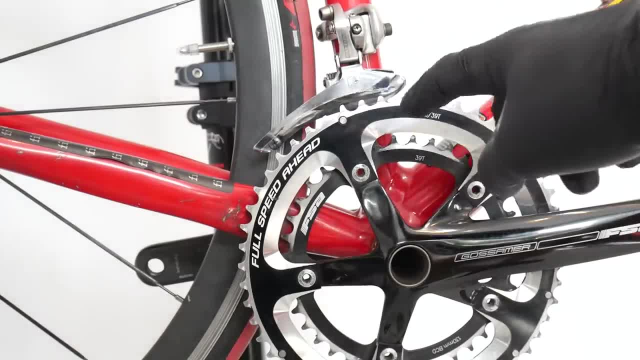 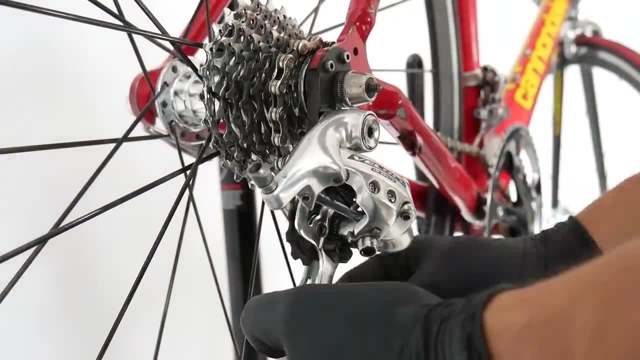 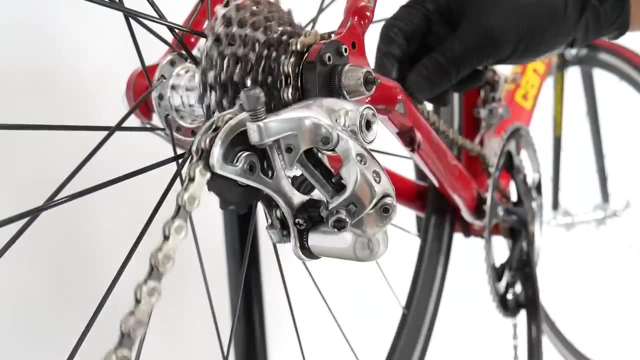 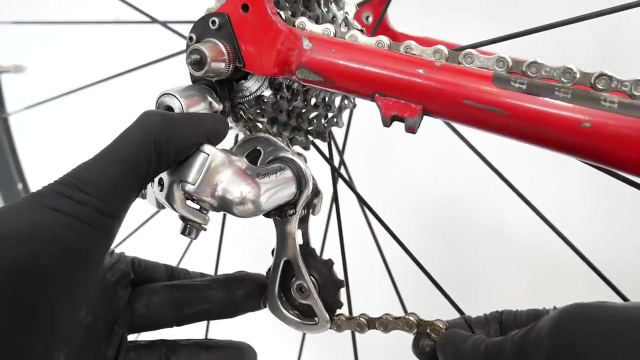 the bike. Now we need to guide the chain properly through both of the derailleurs. Please pay closer attention to the rear derailleur so that the chain will be guided correctly. This is a new chain, so it should be too long, and this one. 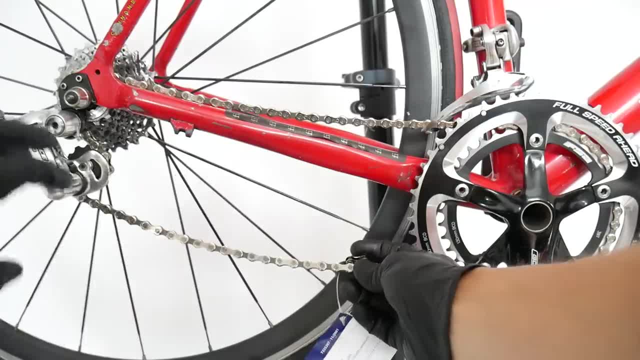 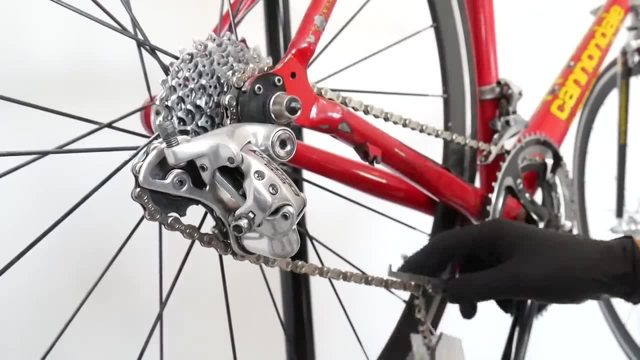 really is. We already know the method of determining the right length of the chain. Now we're going to use it. What if we remove from the chain two links? What if we remove from the chain two links? What if we remove from the chain two links? Well, the chain is still too long. Let's say we are. 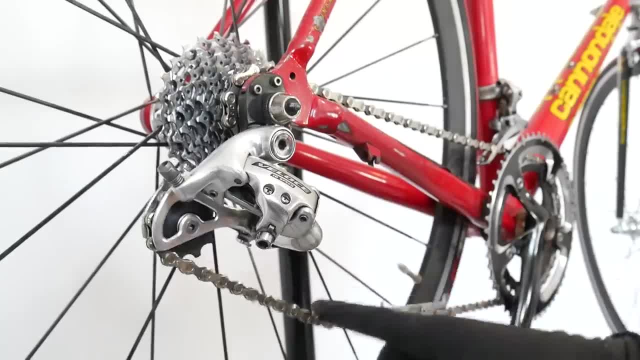 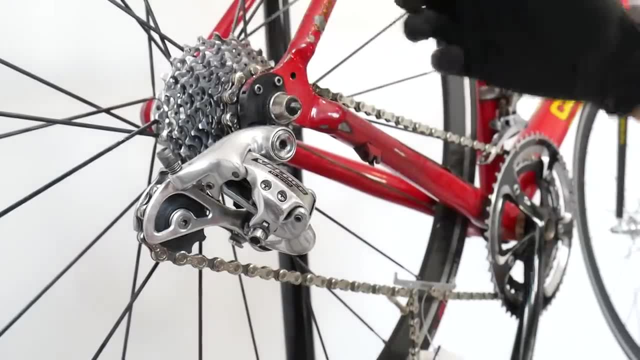 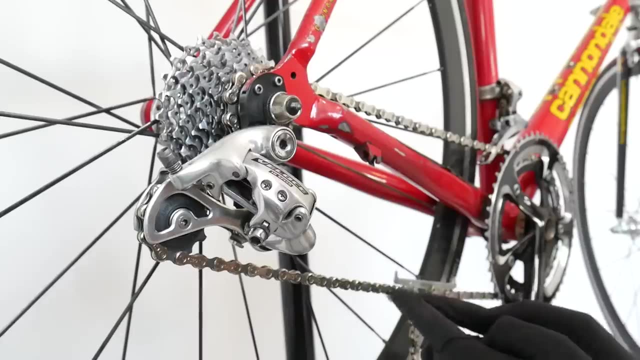 removing three links. Now the chain has the proper length At this moment. it's also good to think about the range of your gears. For example, if you've got the cassette 12 by 25 teeth, I would even remove at least one link more The bike. 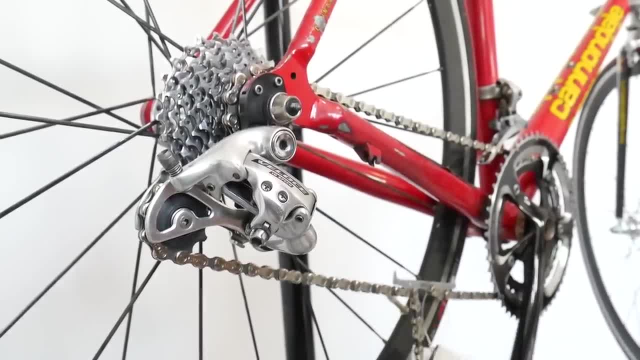 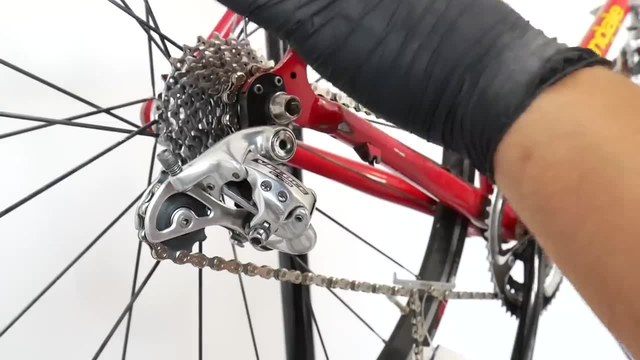 will be lighter, We will have a bit more tension on the chain and still the derailleur won't have any problems, have any problems going through the whole range of our gears. If we had here 11 by 28, for example, I would leave the length of the chain just as it is. 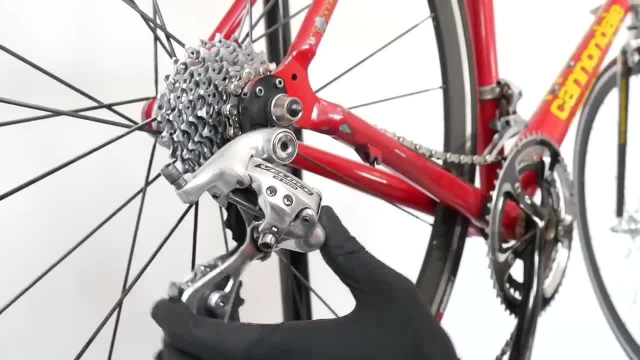 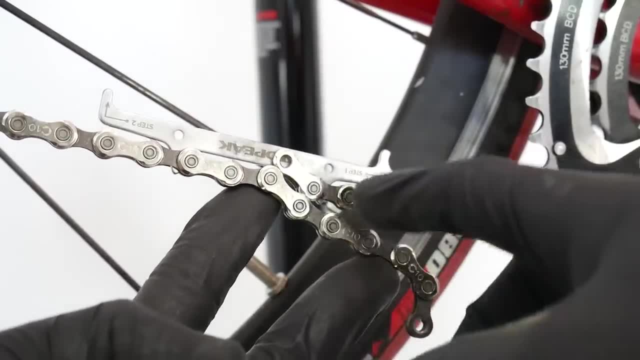 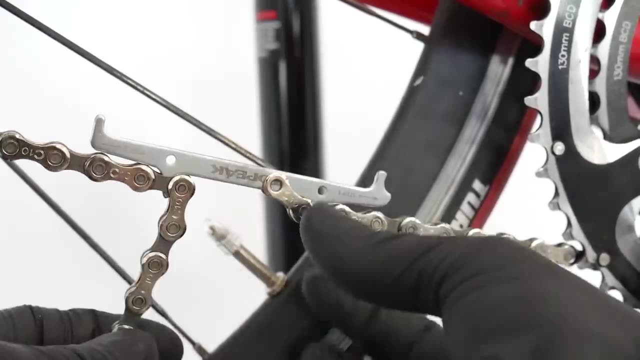 because the derailleur will work much more to go to the lowest gear. Great, we know now how many links we need to remove. This is the one, two, three external links, So all together this will be six links. Unlike with the quick link, now we need to have on one side the external links and on the other side the 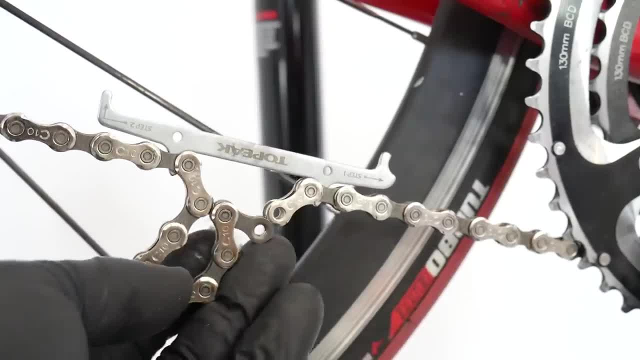 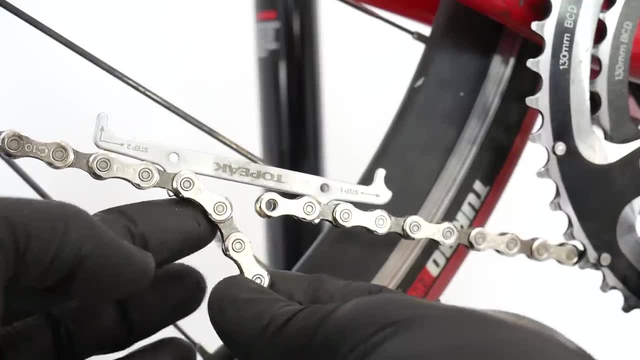 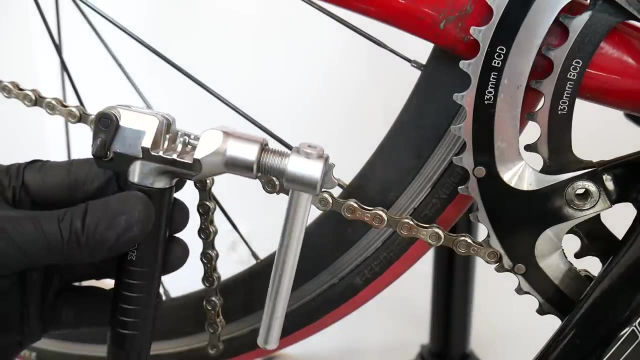 internal link and on the other side, the internal link. So remember about that, because with the quick link we needed both internal links. So we know that the chain should end right here with the internal link. It is time now to use our lovely chain tool. First of, we need to make sure which pin did we want to. 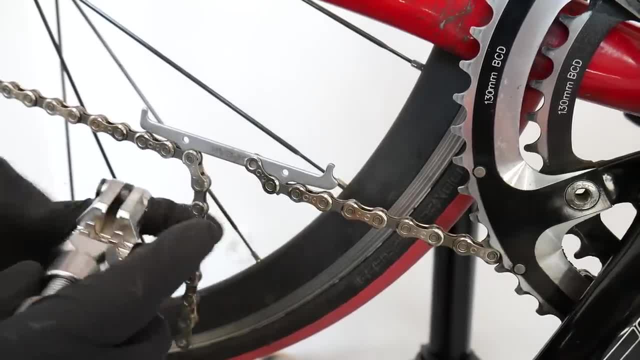 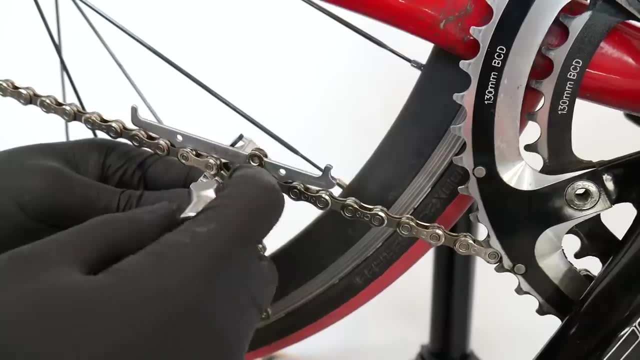 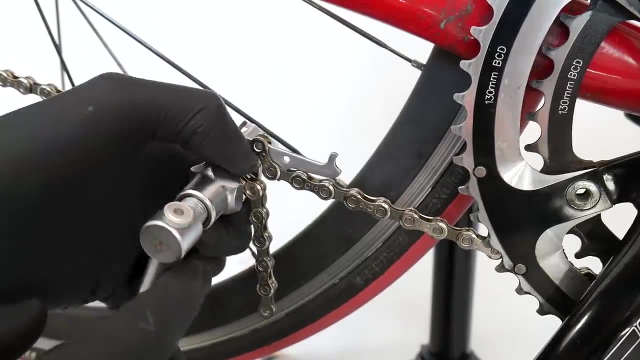 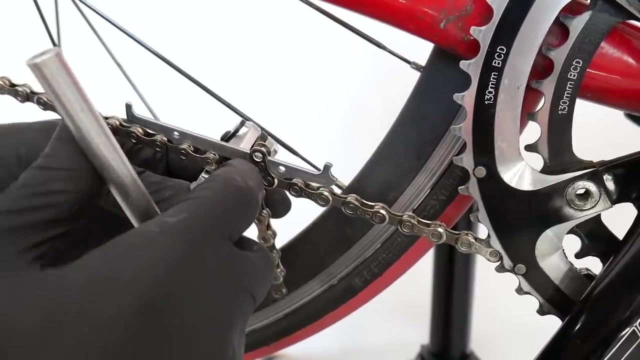 extract. That's this one here. and then, secondly, we have to be absolutely sure the chain lies exactly and correctly in the chain breaker Before I start extracting it. I will just help myself with the finger, with the thumb, here, and push the chain exactly to its place. I'm trying to show you how I'm doing it here. 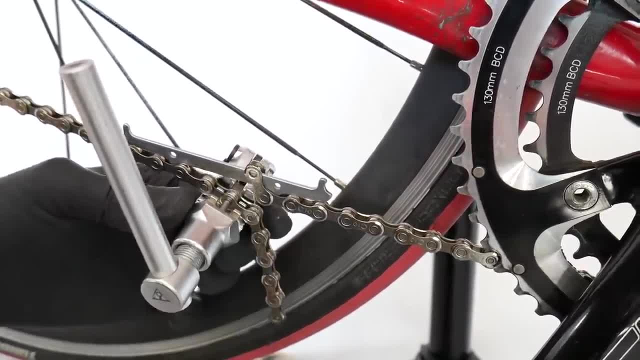 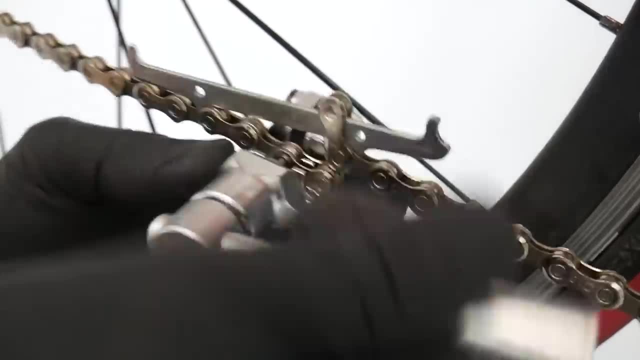 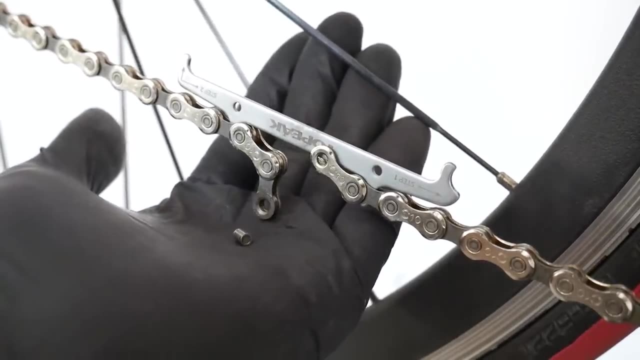 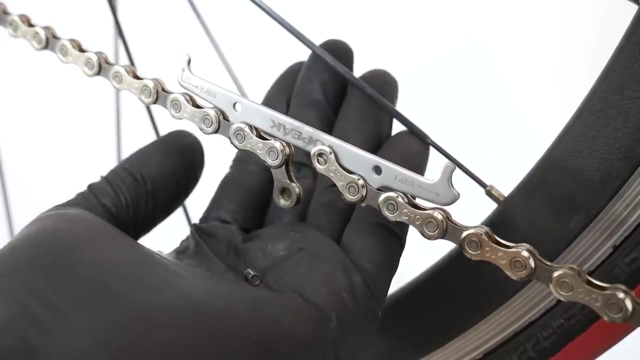 Now we are ready to extract it. This is our extracted pin. Do not reuse it. Reusing this one can cause a chain snap in a very easy way. So, in order to reconnect the chain, we are going to use either the quick link or a special connecting pin, which I'm going to show. 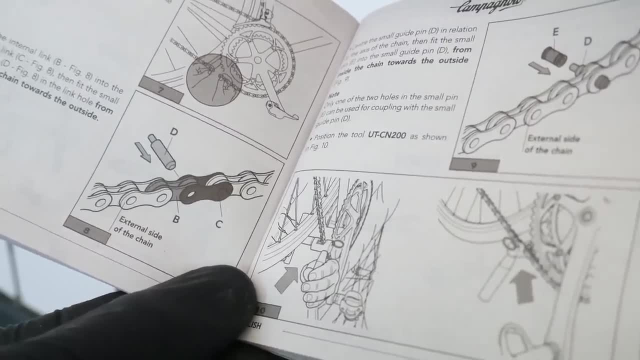 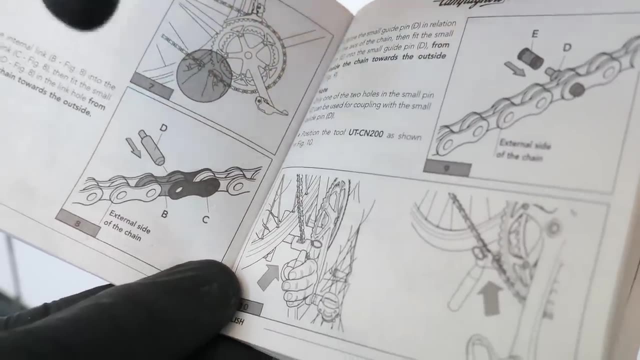 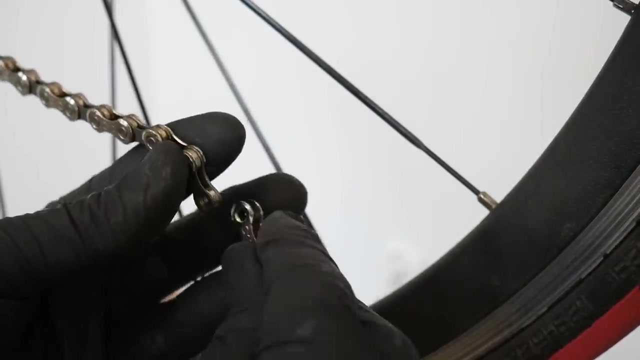 you right now. Even if you consider yourself an advanced bike mechanic, do read the manuals. In this case, Campanella want us to push the pin from the inside of the chain to the outside, So we're gonna go this way. First off, I've removed the chain from the crankset so that there is no tension. 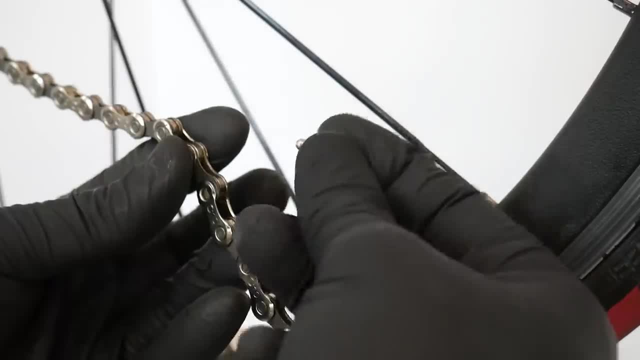 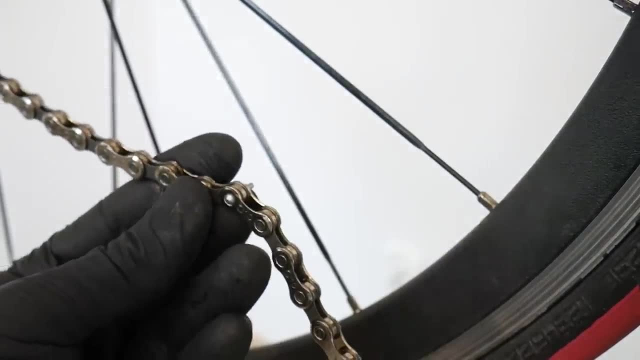 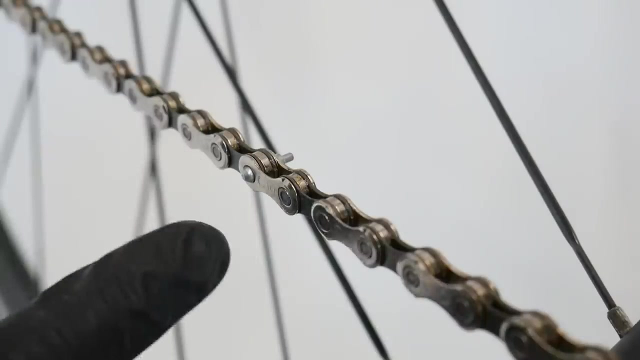 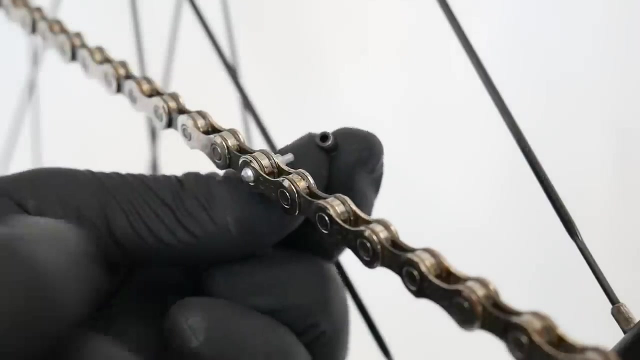 on it, and now I can connect those links with the guide pin from the internal side of the chain, just like this. The guide pin is on its place. Now we're going to fit the connecting pin into it. There's only one hole of this pin: that. 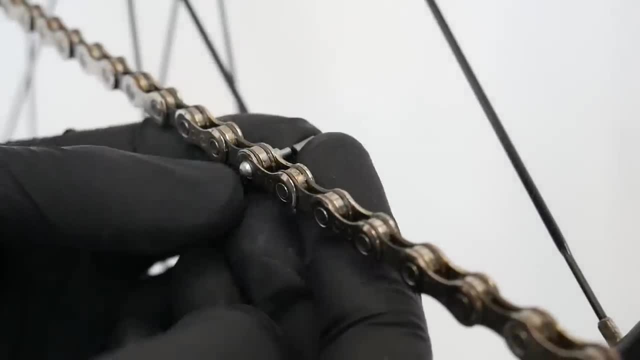 will fit the guide pin. Now we're going to fit the connecting pin into it. There's only one hole of this pin that will fit the guide pin, so it cannot be put just like that. It can be fit only one way, like this Now. 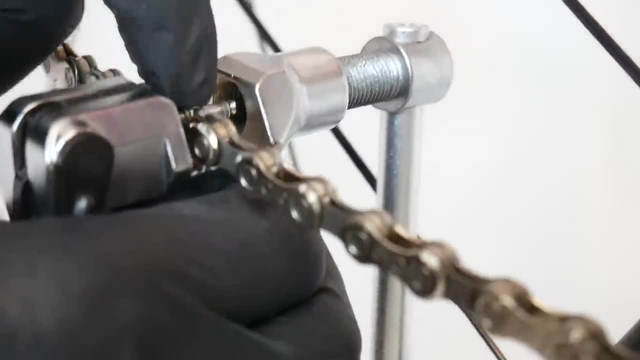 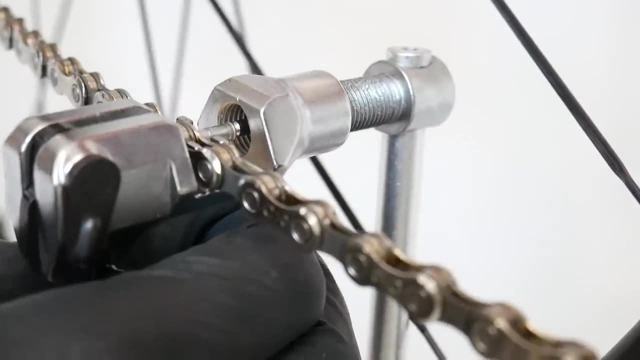 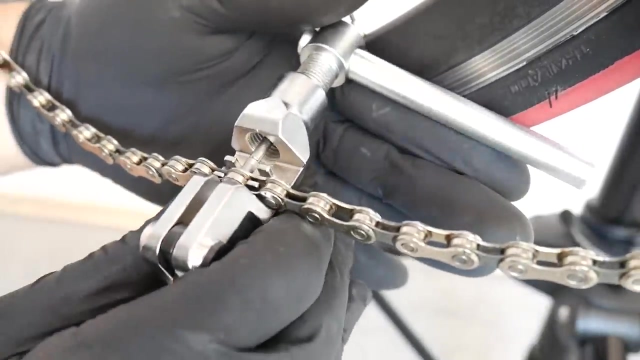 we are going to use the same chain tool, but for installation, not for removal. We are going to push this pin until into. it will be centrally located in the link. After pushing our connecting pin into the guide pin, we are going to push the connecting pin into the guide pin. 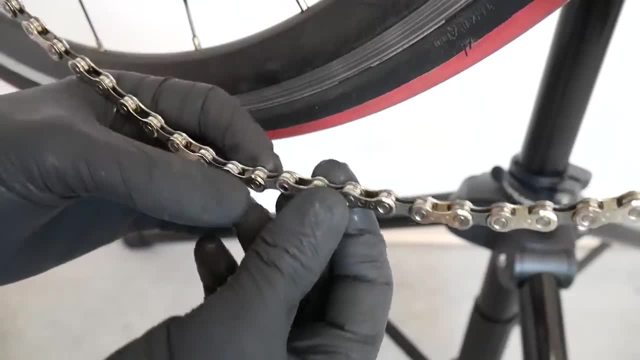 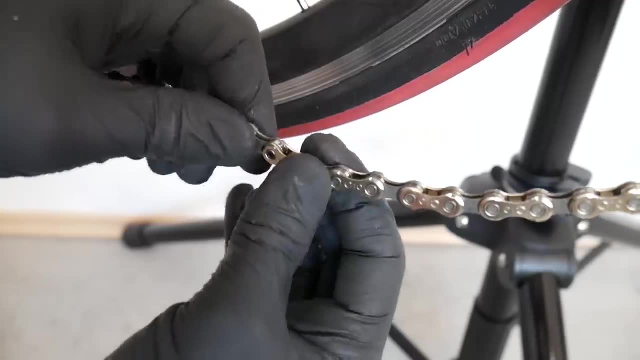 After pushing our connecting pin into the guide pin. we are going to push the connecting pin into the guide pin. We are just making sure whether it is working properly. So it has to be loose, not stiff. Sometimes just moving it around a little bit may help This one. 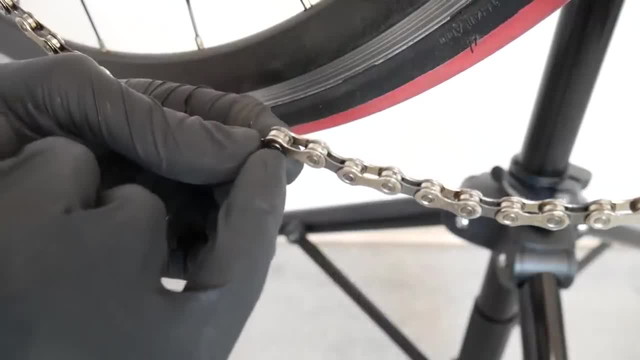 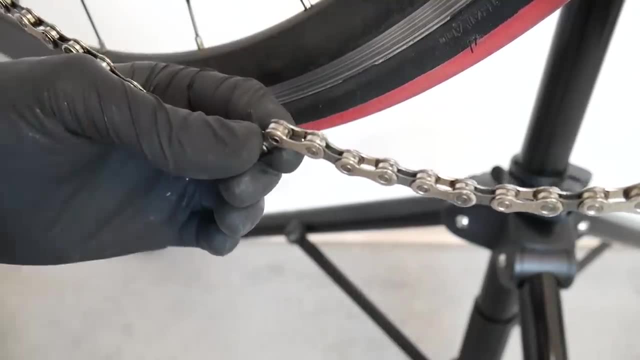 works fine. and also this pin stands out just about 0.1 millimeters on both sides, so evenly. that's very good, the job is done. Here is the simple method for determining whether your chain is. Here is the simple method for determining whether your chain is. 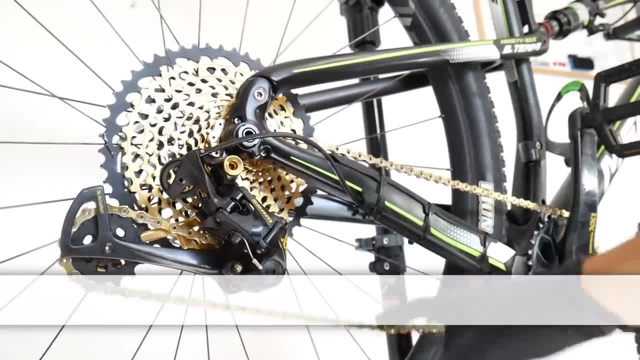 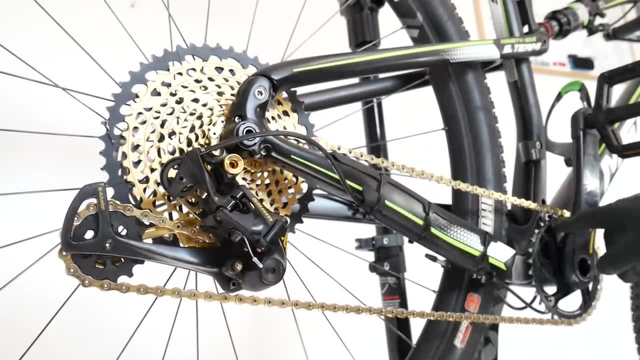 of the right length. First question: isn't the chain too long? Shift the chain down to the smallest sprocket in the rear and in the front. if you've got more than one here and your rear derailleur should still be able to put some nice. 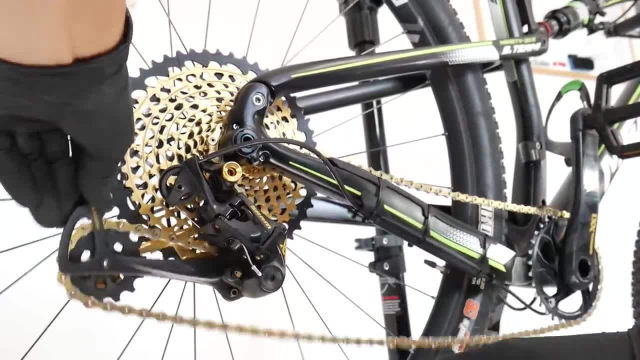 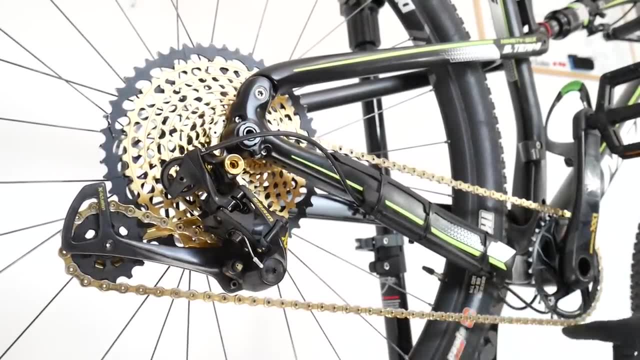 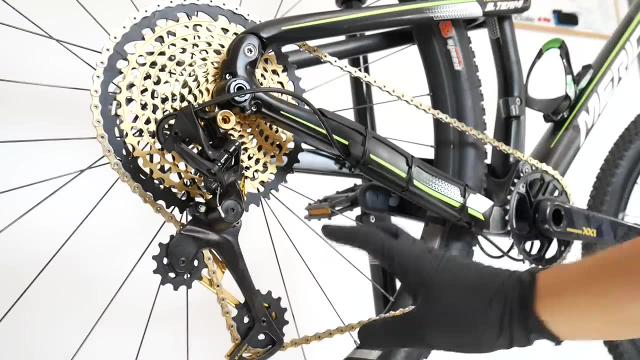 tension on it. So the chain cannot be loose like this. and also it should go straight from the bottom pulley to your chainring, not touching any other parts of your derailleur. So here it is pretty good. Now isn't the chain too short? In this case, we are shifting the chain to the 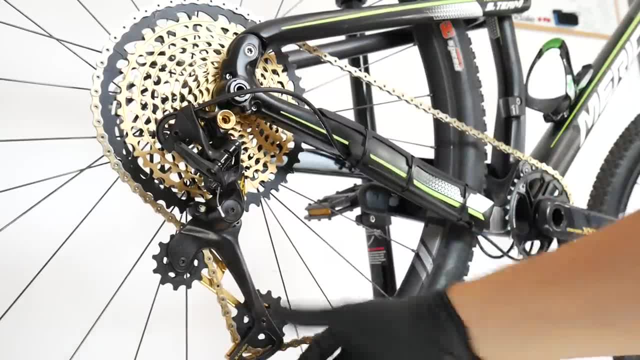 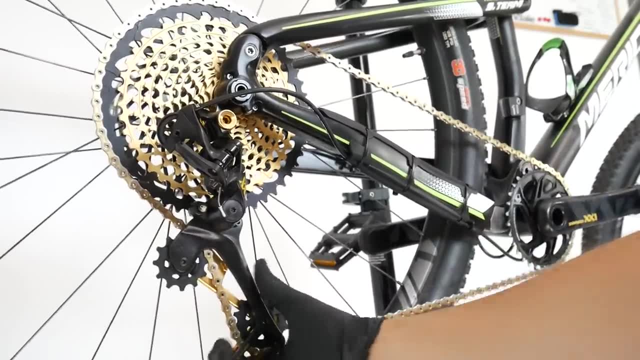 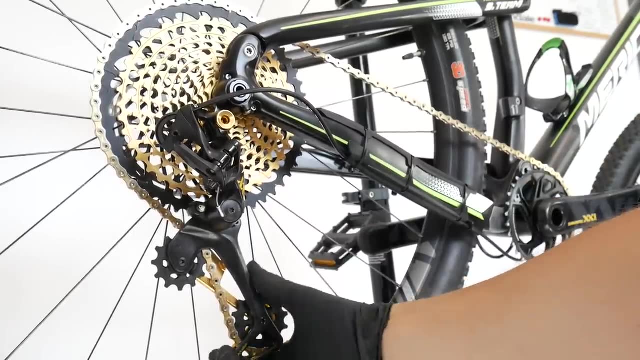 largest sprocket and also we are looking at the cage of the rear derailleur. As you can see, this one can still move much more and we can have. we can see some nice bend on the top pulley of the derailleur. This is really good If the 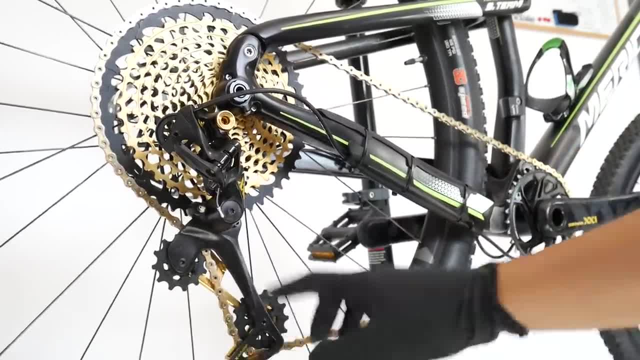 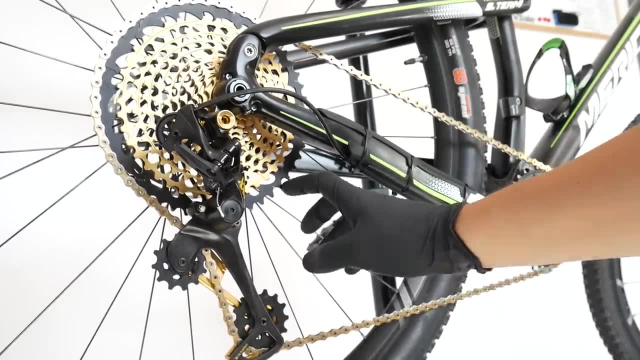 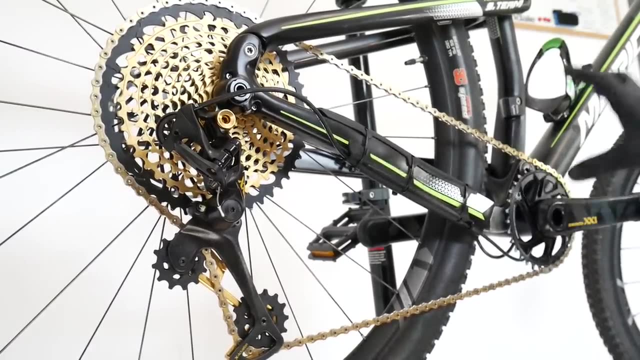 chain was too short. changing the gears in the lowest range on the cassette would be very stiff, not really good, sometimes impossible. So here it is just okay. But what if we have a double or triple crankset in the front? Well, if there is a double, there will be still some. 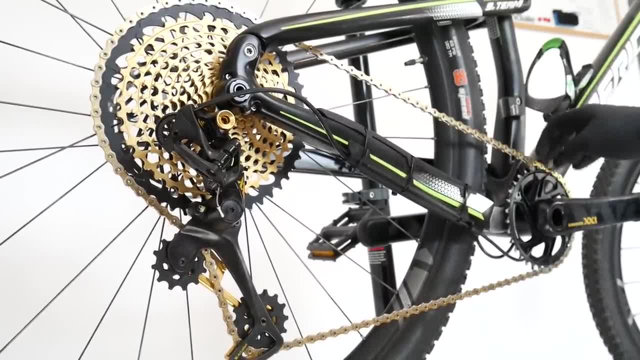 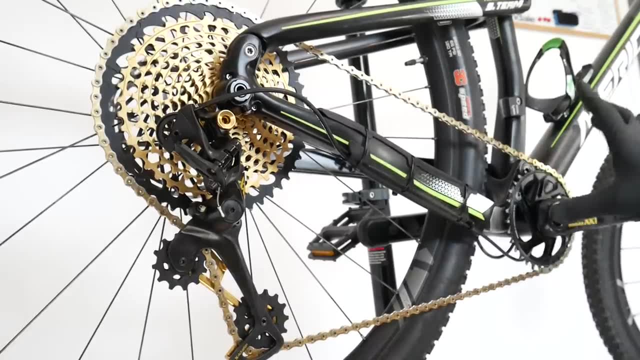 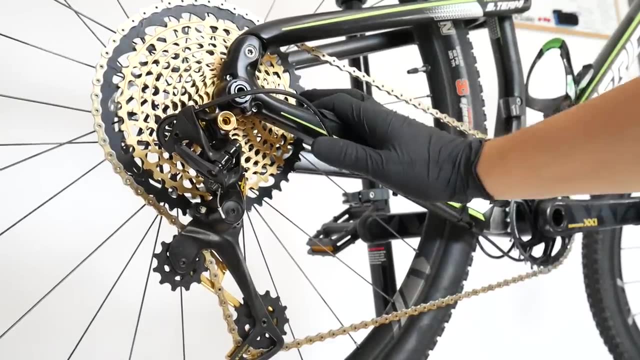 possibility to shift into the largest sprocket in the front and largest in the rear and check it like with it with the one by drivetrain. If you've got three chainrings in the front I would not really use the largest one with in the front and largest one in the rear, Maybe the largest one in the front and 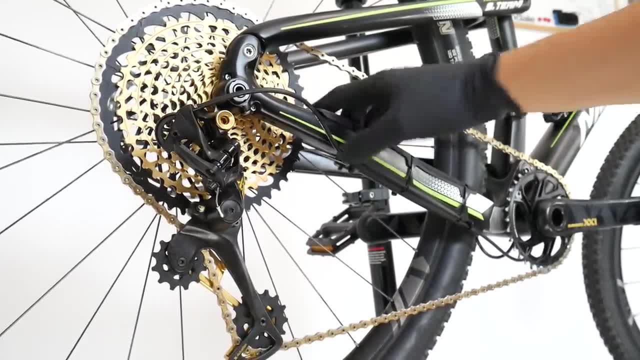 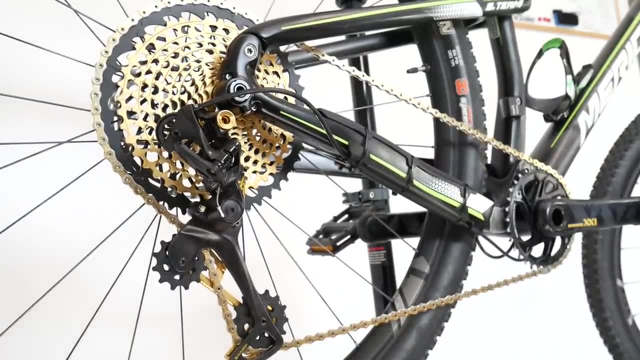 the third gear in the rear would be good, because we are never going to use such a combination of gears, So don't worry about that so much. if you have a triple crankset- How to remove and assemble the pedals on our bike- This is pretty easy. 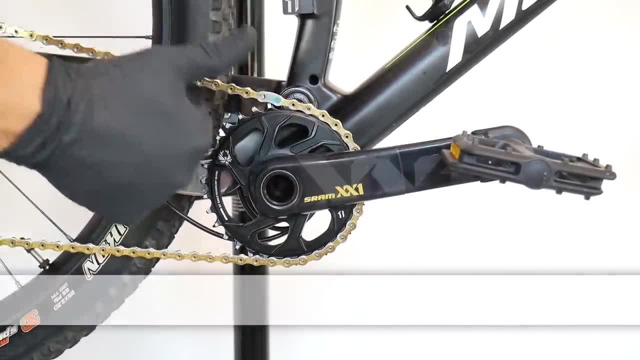 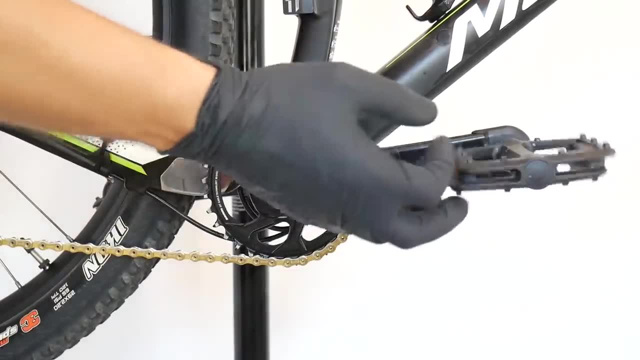 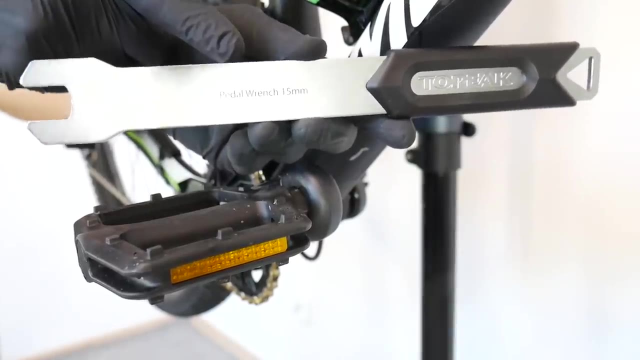 job. but the most common questions here are what tools to use, what kind of thread there is on each side on our bike and third, what torque should we use when assembling those to the bike, So threading those in? Let's begin The first question and first answer. The best tool to use here is the 15 millimeter wrench. 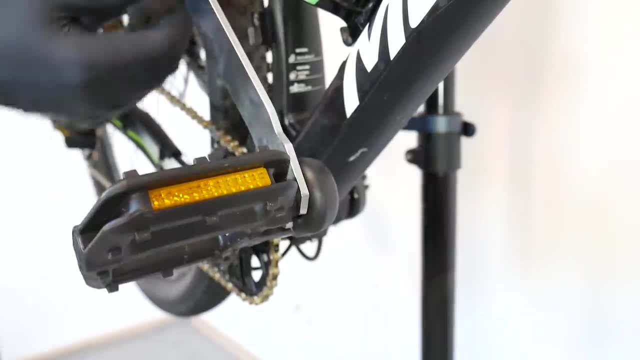 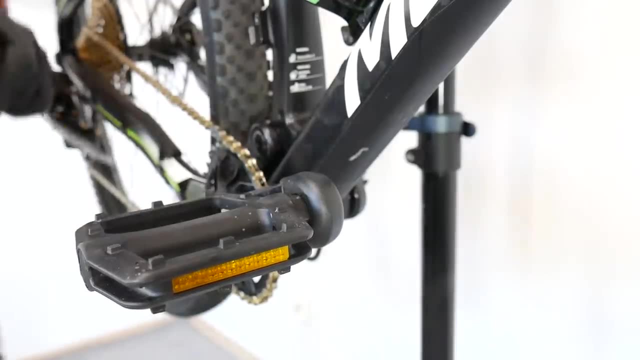 This one will give us a lot of control over the pedal when both unthreading and threading those in Some pedals- not this, for example, but this- this is the clipless pedal- will give us also the option of using the allen key, but still. 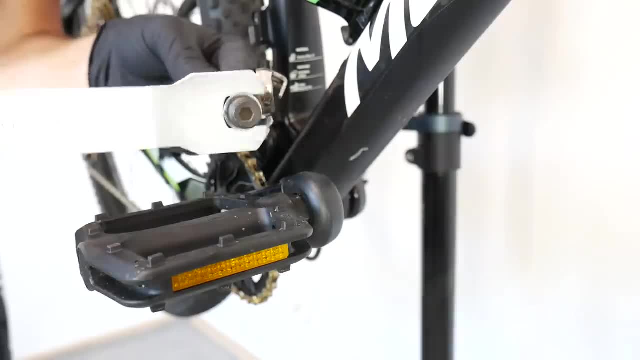 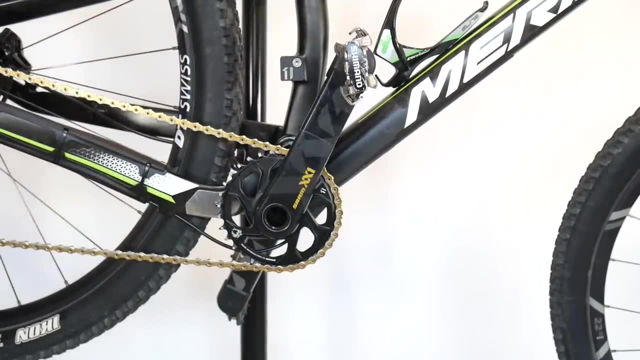 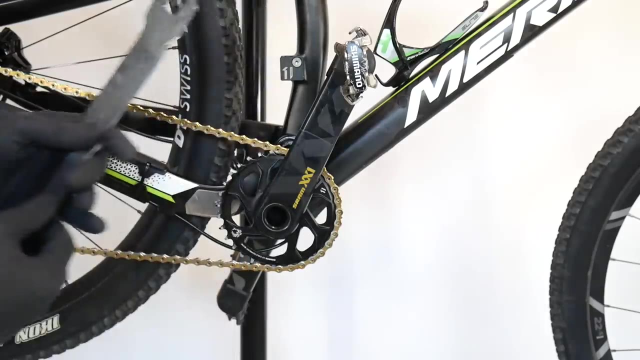 this is compatible with the 15 millimeters wrench, and that's the one I recommend here. How to unthread the pedals and then thread those in. First off, it is good to have a specifically designed tool for that- the wrench- because it will move our hand a little. 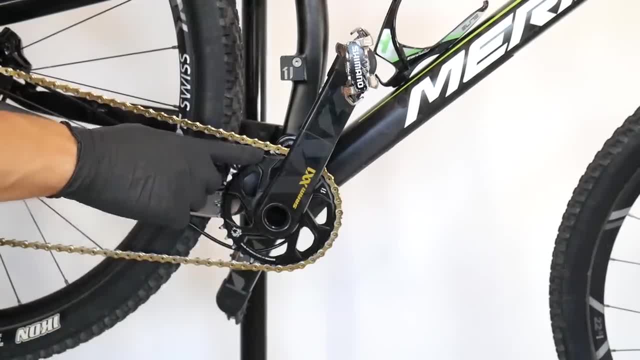 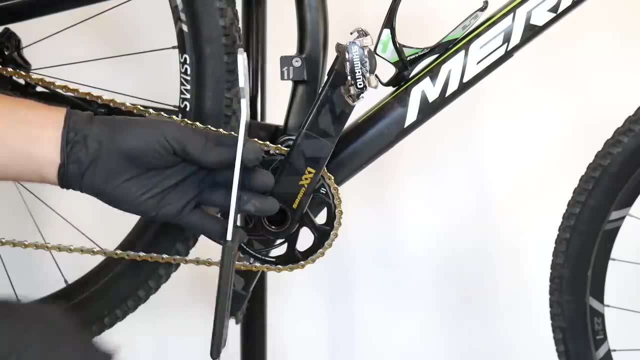 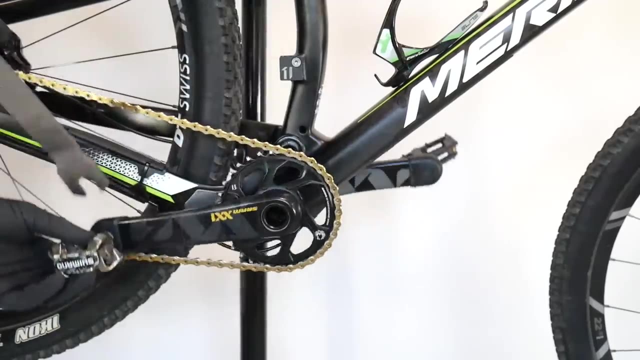 bit outward so that we will not hurt it against the chainrings, which is not that risky. but sometimes it happens that our hand slips and it could be dangerous. So having such a tool is really good, but you don't have to have it. The second thing is to find the right place to start the unthreading For. 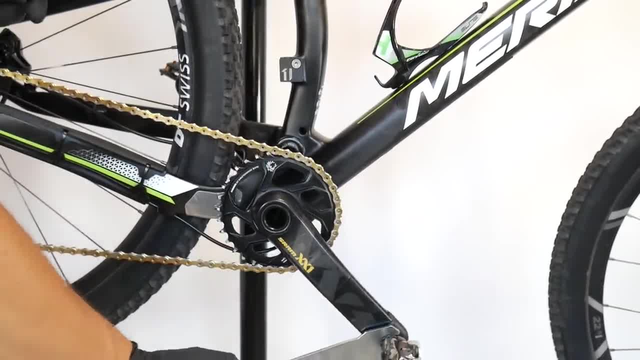 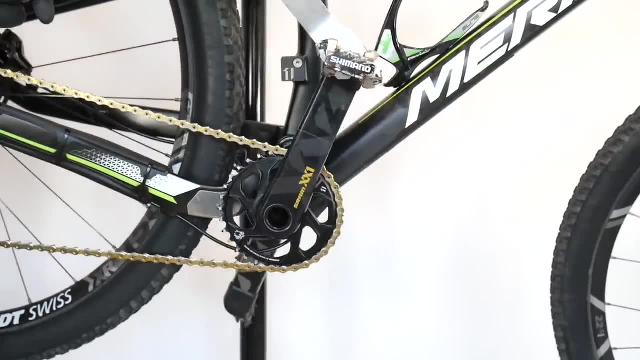 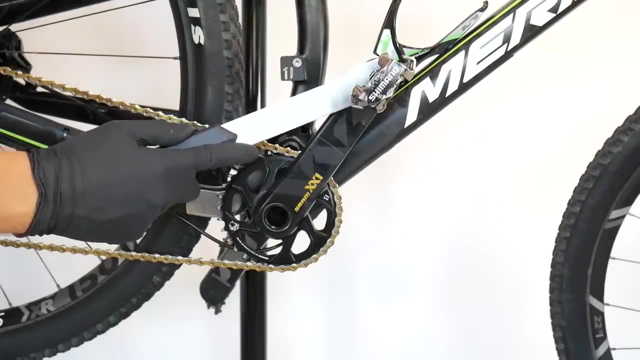 example, this one here is not the best, because when I'm pushing, the pedal goes up, so the other way around should be better. So now I will be just pushing down. that's what I'm doing and it will be the most easy way for us. 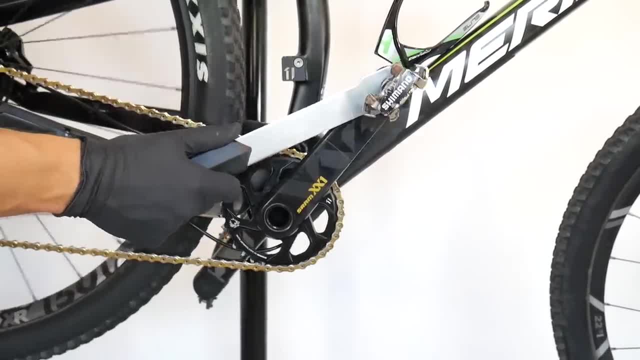 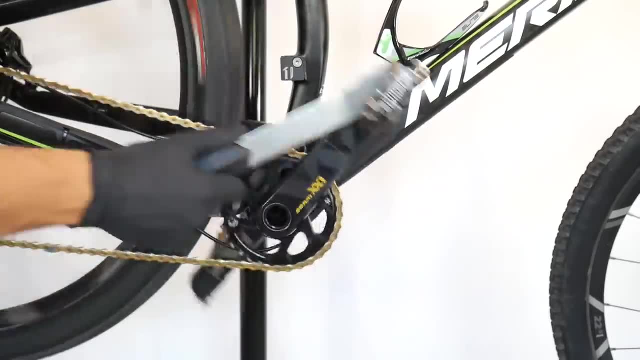 to memorize how to do it will be when threading those in. But when we unthread the pedals, just remember- the wheel turns to the front. So we are not spinning backward but just forward, and we do it on both sides. so you don't have to. 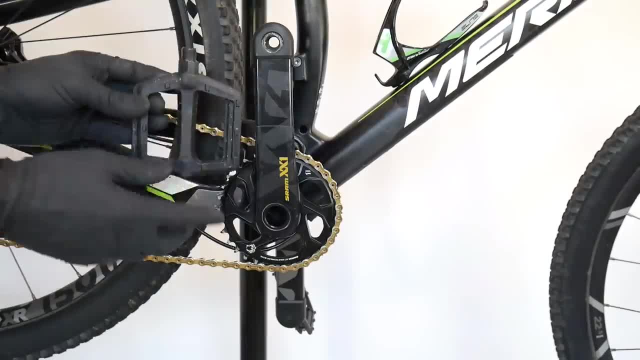 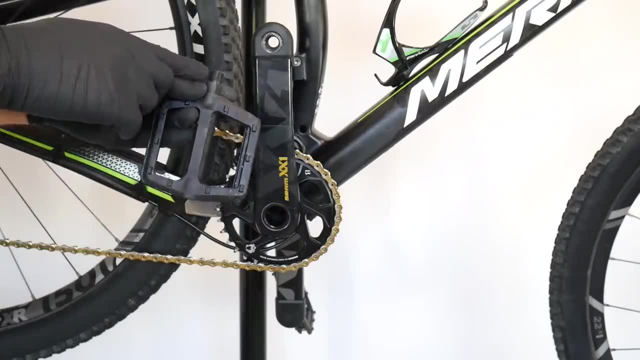 memorize the drive side, the non drive side. Now we need to thread this one– platform pedal back to the bike. How to do it? First off, it's good to use some grease, because maybe something anti-seize would be good. I am replacing the pedals. 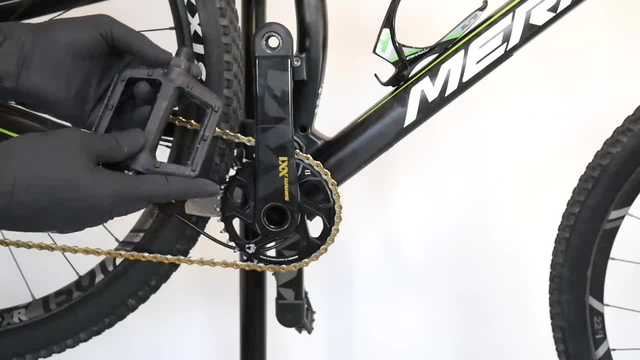 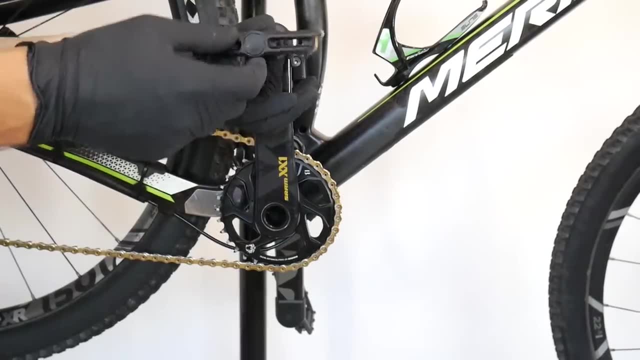 on my bikes 20 times a season, humanely, So I always started it like that. So going to the meet up подписchannel to us, so I don't even use it that often, maybe once a season. and now we need to find the right place in the thread. okay, this is the right one, and I'm turning here. 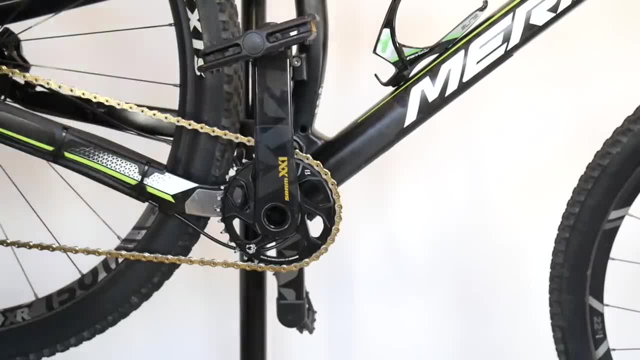 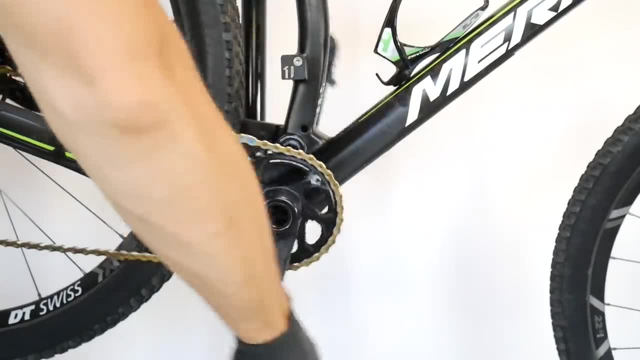 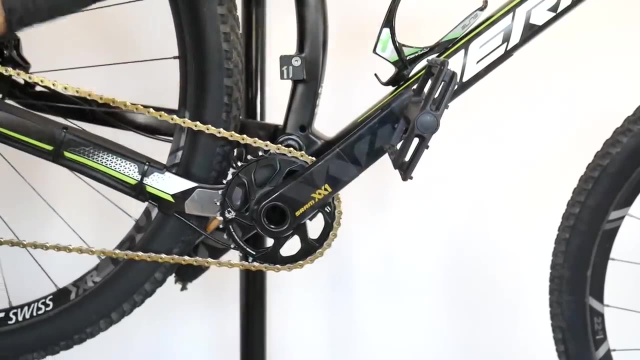 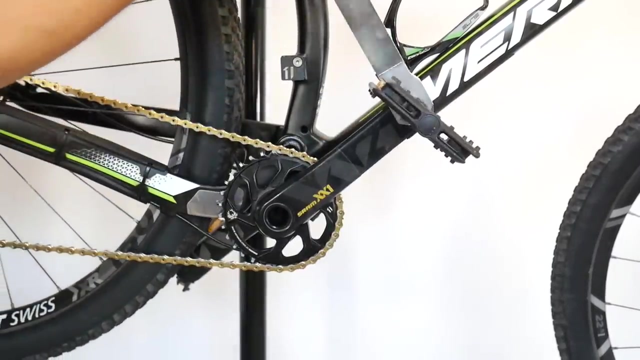 clockwise, but it doesn't matter. what matter is that I'm just holding to the pedal now and spinning backwards. right, I'm holding to the axle of the pedal, spinning backwards, threading this in. it will be the same, exactly the same on the other side. now, how much torque should we use? not too much, definitely less than. 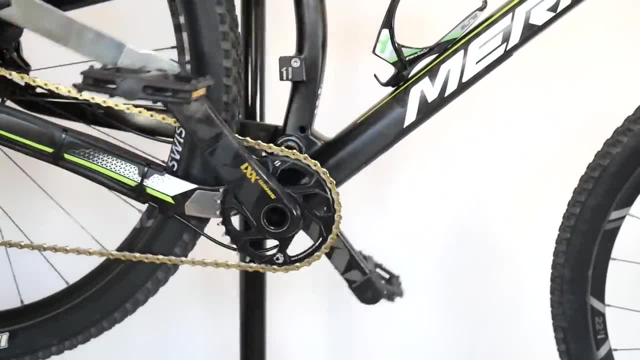 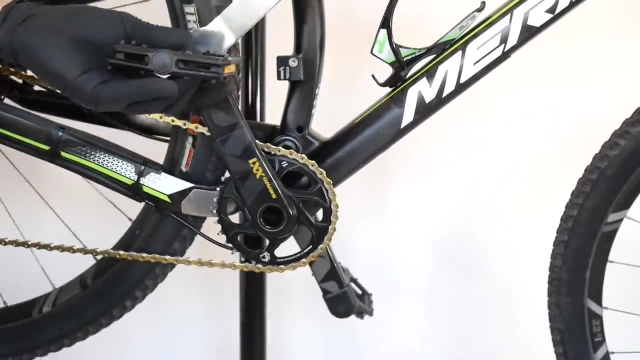 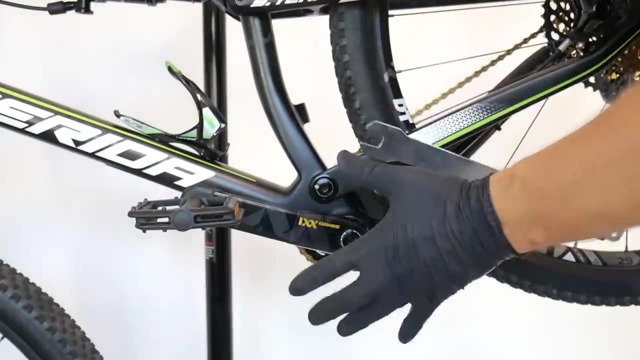 many beginner cyclists would think, okay, okay, now it's, it's starting to to resist, so I will just give it a little push now, like this: that's enough, let's go to the other side of the bike. now we understand the principles of unthreading and threading those in, let's just 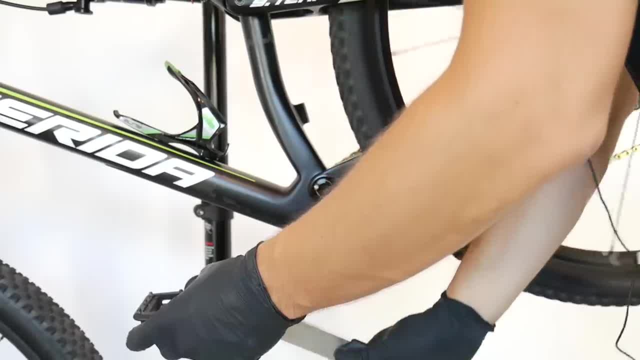 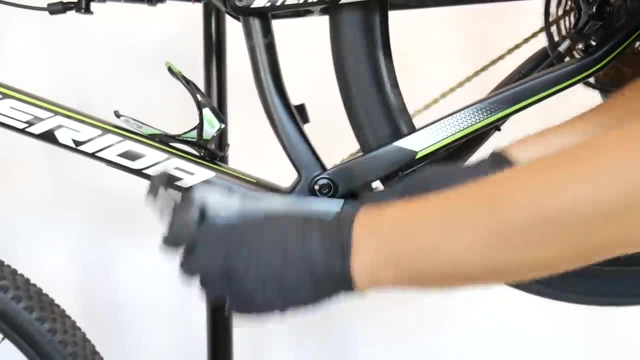 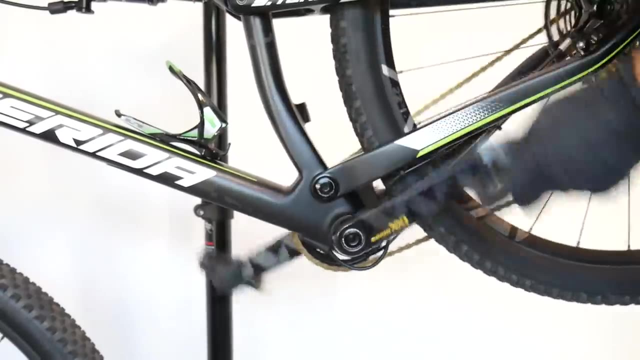 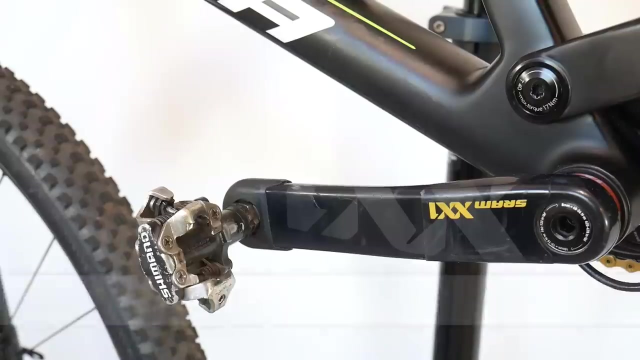 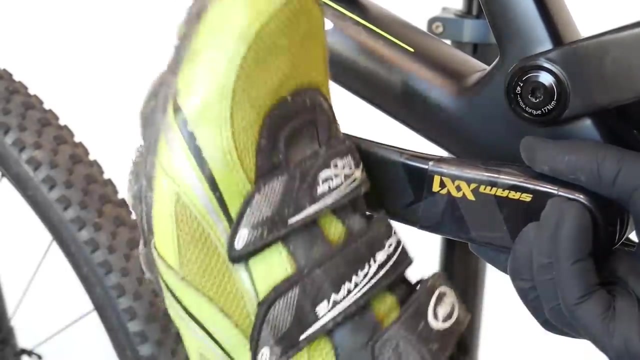 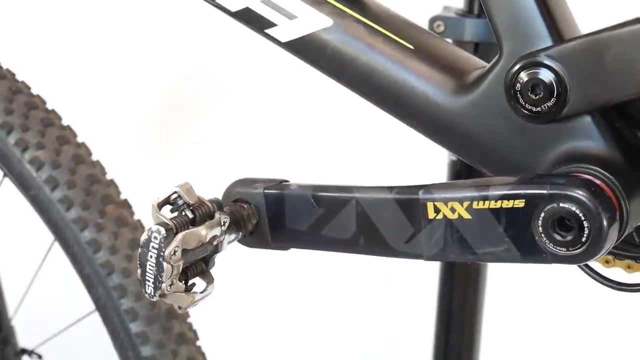 memorize the process. if you've got one of the clipped pedal systems on your bike, it is good to know that majority of different systems will have some kinds of the adjustment of the spring tension. that means, for example, on these Shimano pedals I'm using 3 millimeters Allen key, and when I 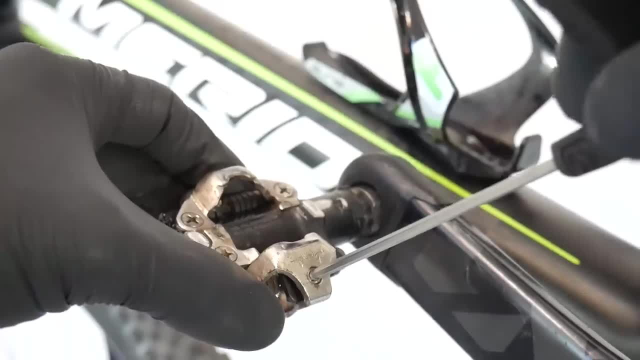 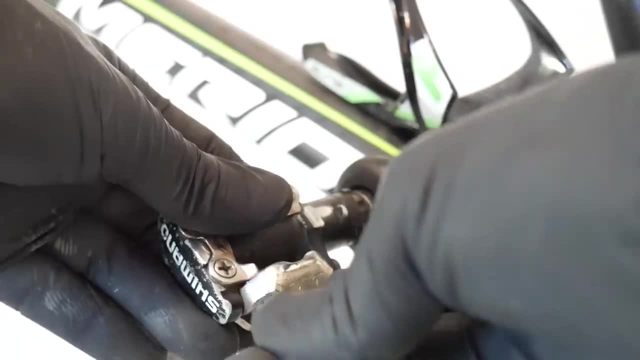 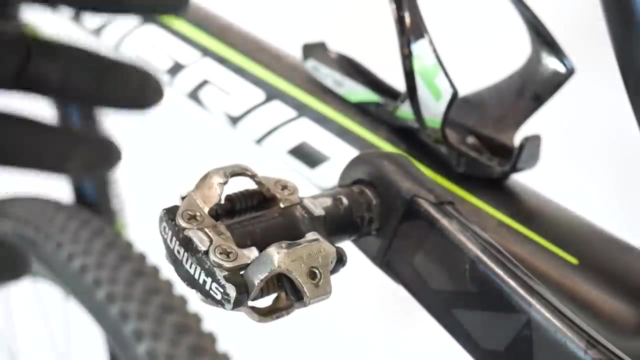 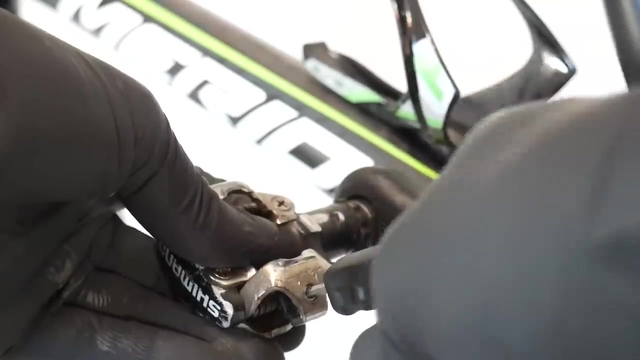 turn this little bolt clockwise, I will increase the tension. that's that's it. and when turning it counter clockwise, I will decrease the tension. that means less tension means easier clipping in and clipping out. more tension, like now, means more difficult, more resistance while clipping in and clipping out. if 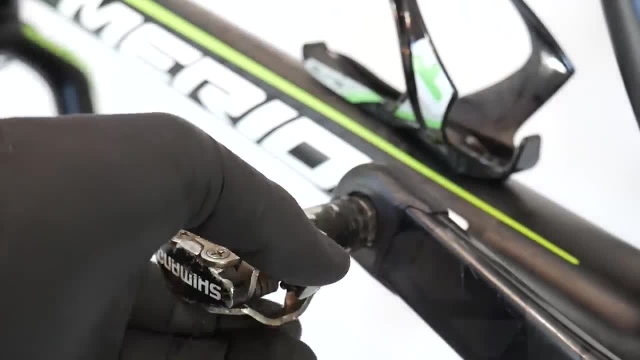 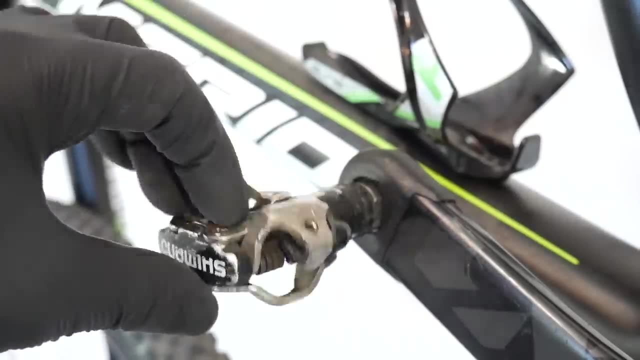 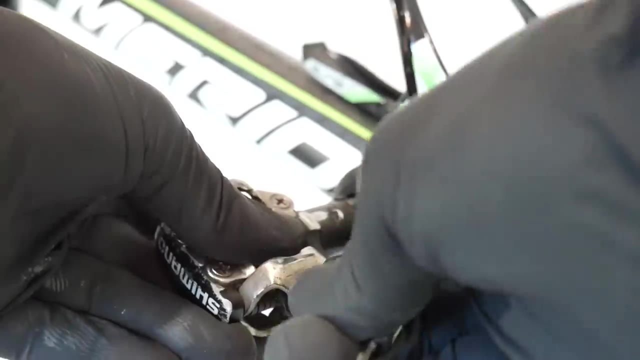 you are learning how to use this. it is good to set those on almost minimum, or even minimum tension, and also it's good to set the same exact tension on both sides, so you can, for example, unbolt these completely, let's say to the left, and then start. 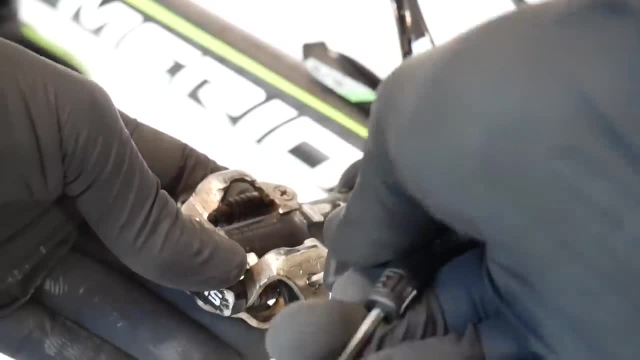 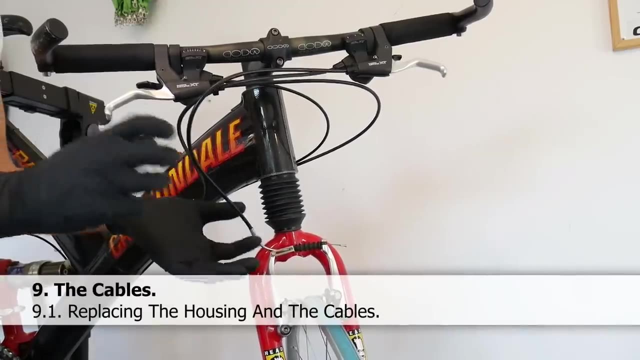 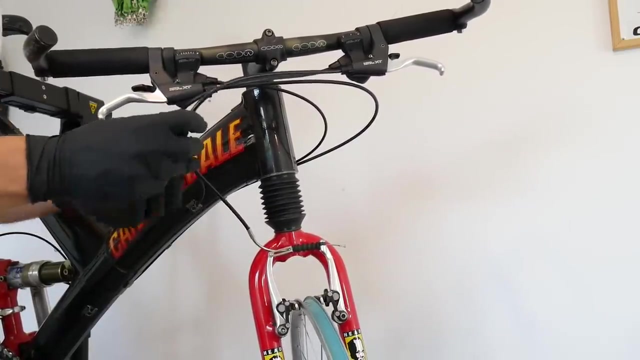 from the zero position, counting your turns and doing- do it in the same manner on both sides- how to replace or shorten the housings for the mechanical brakes or our shifters, in case of simply replacing the housing because the old one is rusty or just isn't smooth anymore. it's pretty. 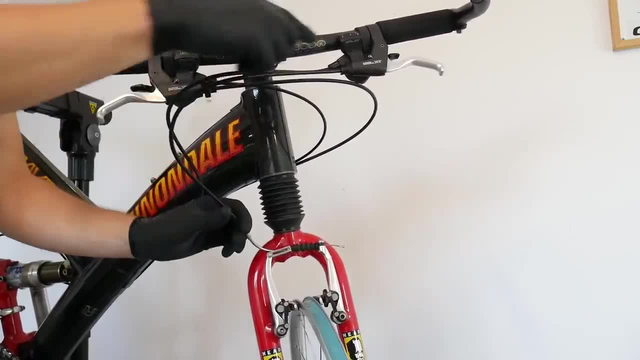 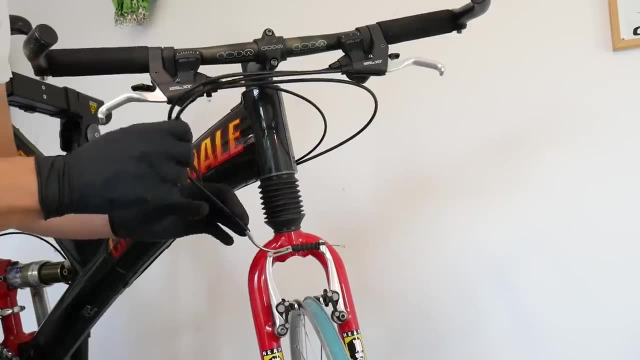 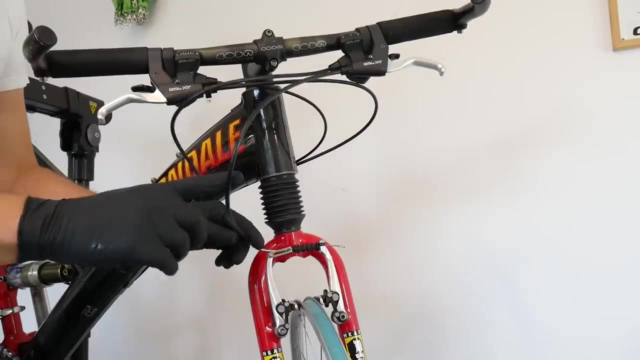 easy job. we want to cut the new one at the same length as the old one, but I would always check out whether the old one was really the right length and, as you can see, my expect. the inspection on this bike shows that at least this housing for the front front brake is too long and you can just 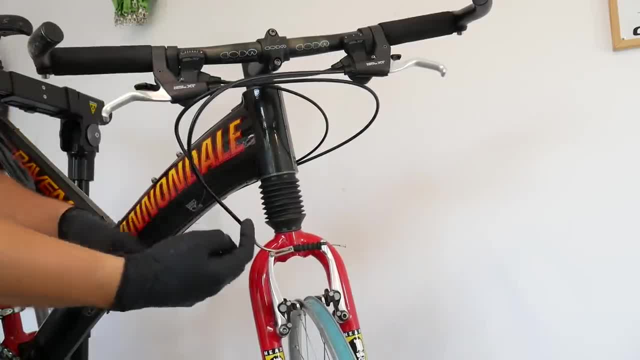 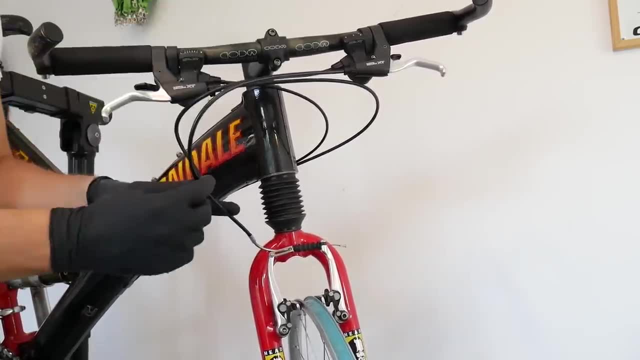 see how it looks on the front brake and you can see how it looks on the front brake and you can see that it that the cable makes really long way to the brakes. we don't want to have the shortest way possible. it should be just ideal for the cable. but at least here we can see that there is no. 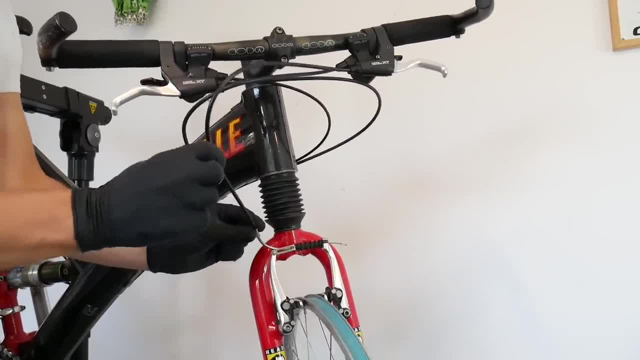 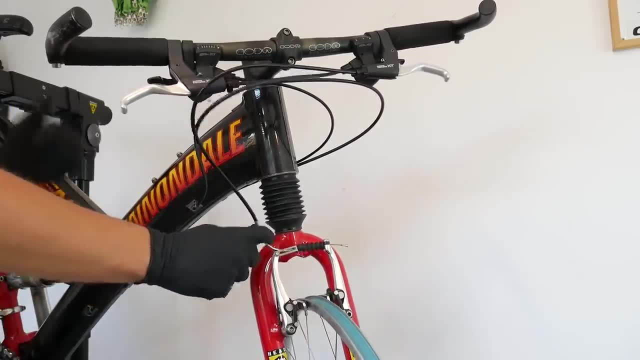 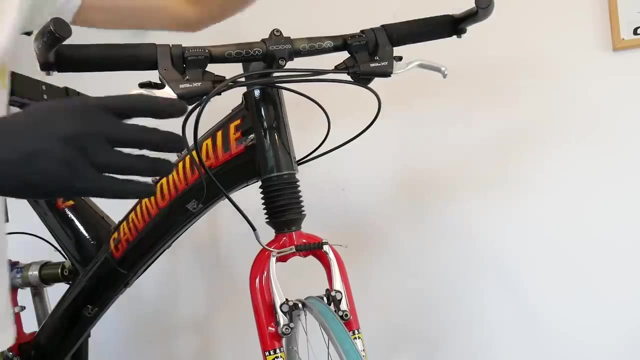 straight line between these two arms, because the housing is pushing this little part here. we would like to have it just like that. so when we are breaking right now, the brake can be a little bit spongy. that's why this one has to be shortened. now. how do we know how short or how long the housing? 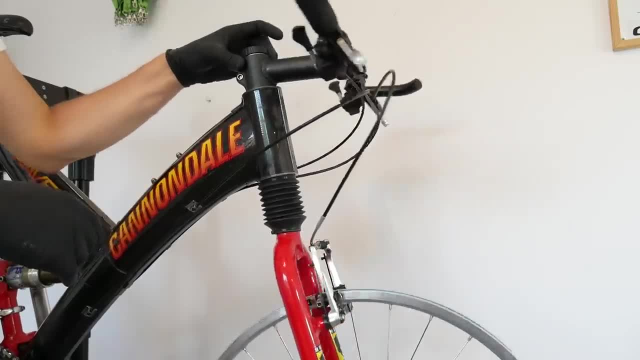 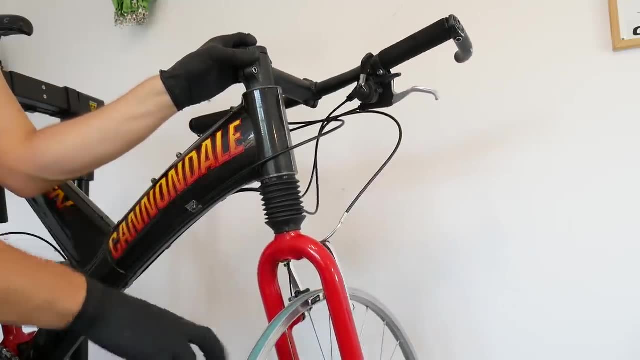 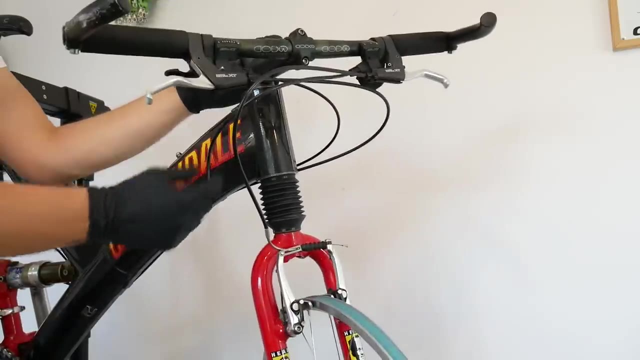 should be. we should always check what happens with the housings while we turn, so if the housing was too short, there was not enough of it for for those tight turns. I can see that this one is pretty long as well, so this one could be shortened also, but we're gonna focus on the front. 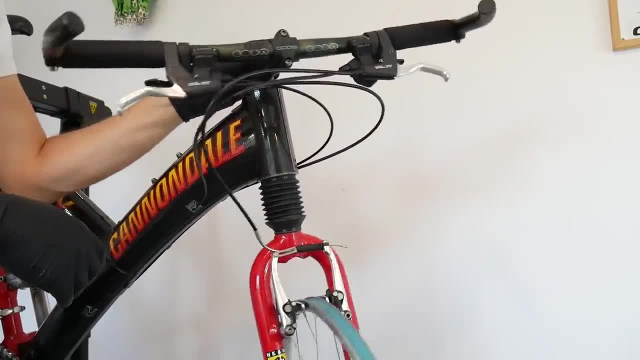 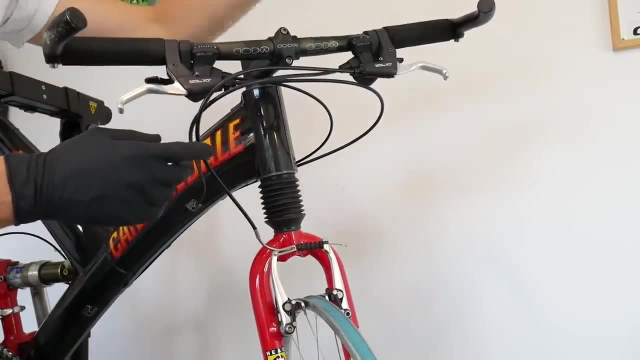 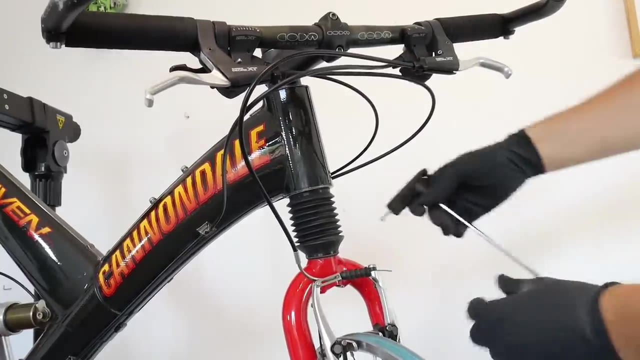 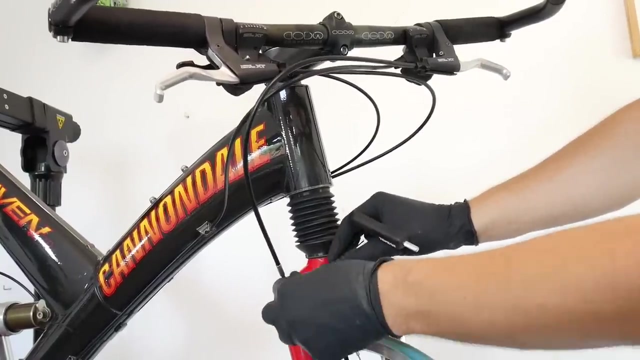 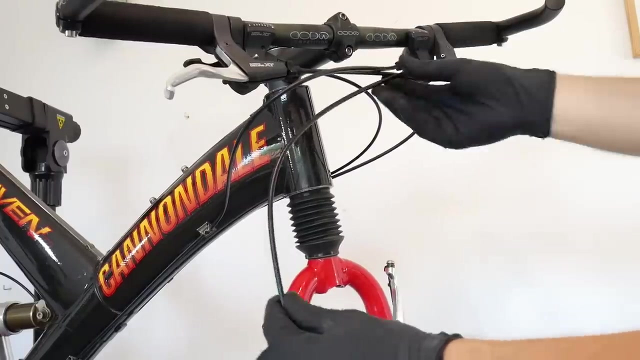 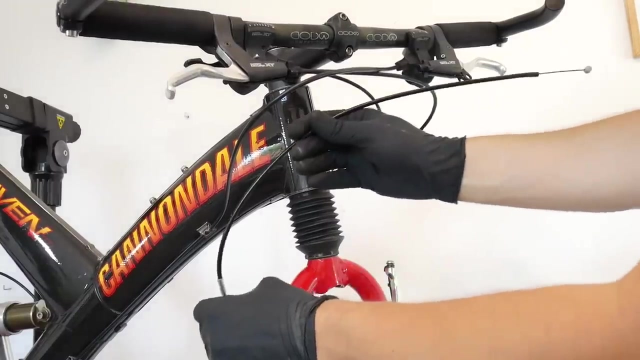 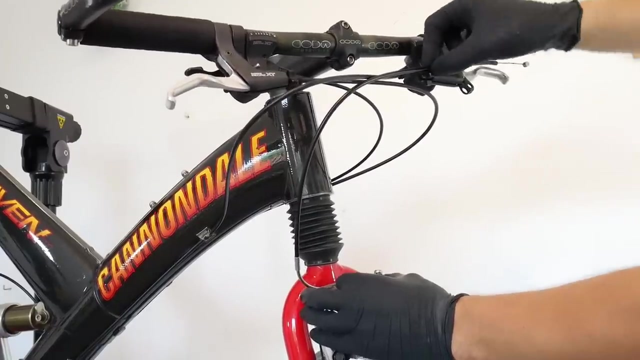 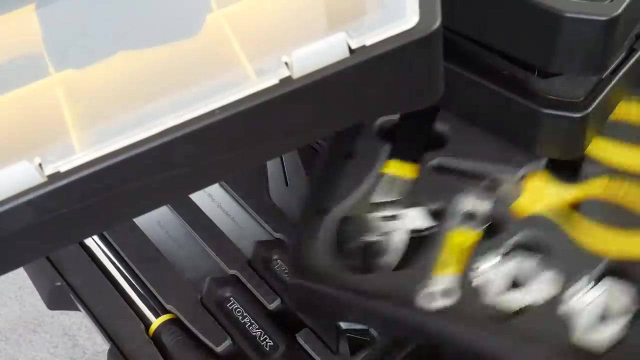 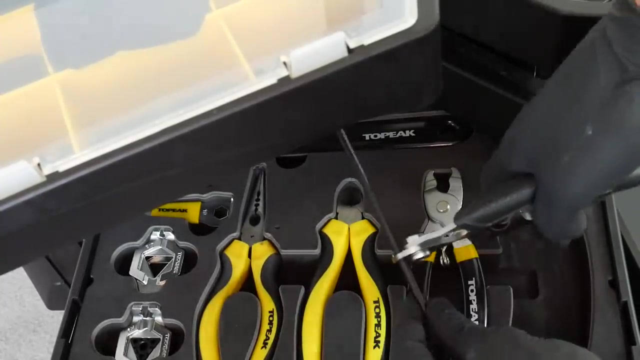 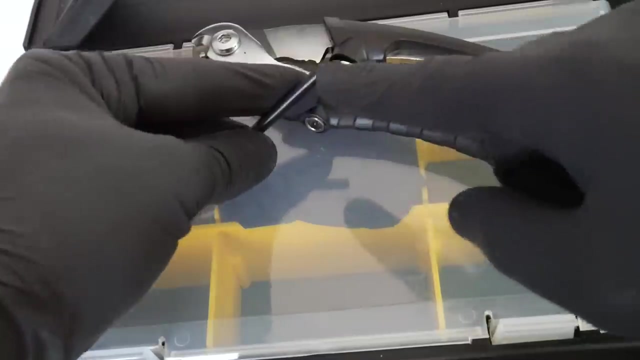 brake. so what happens when we turn? and does the cable have the ideal way from the shifter or braking lever to the derailleur or the brakes to the shifter or braking lever, to the derailleur or braking lever, to the derailleur or the brakes? always, after cutting any housings, we want to make sure that the cut is really nice and there 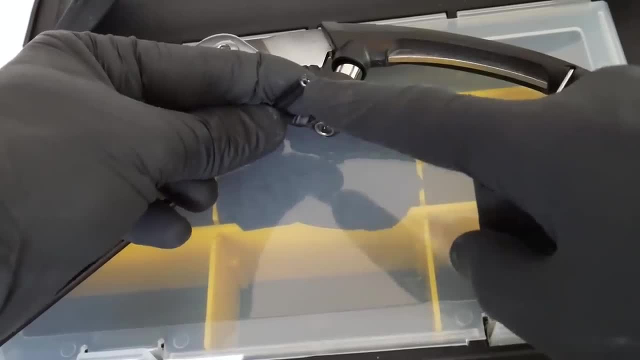 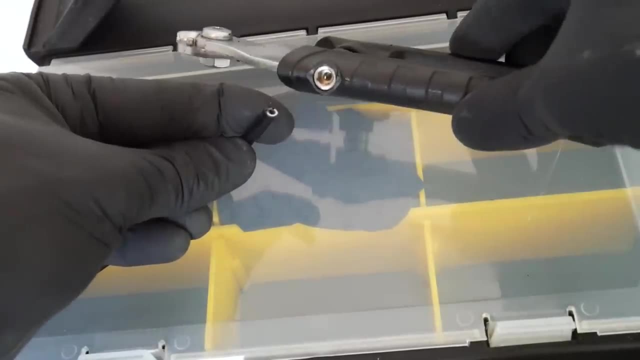 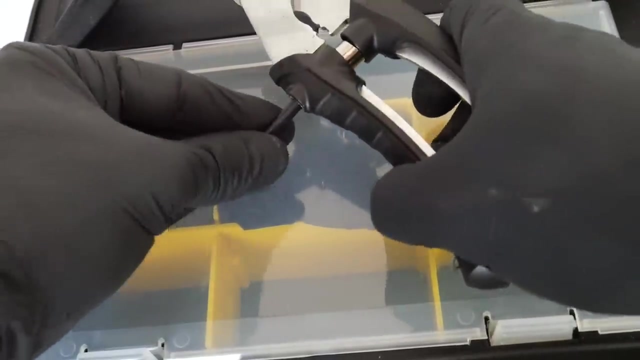 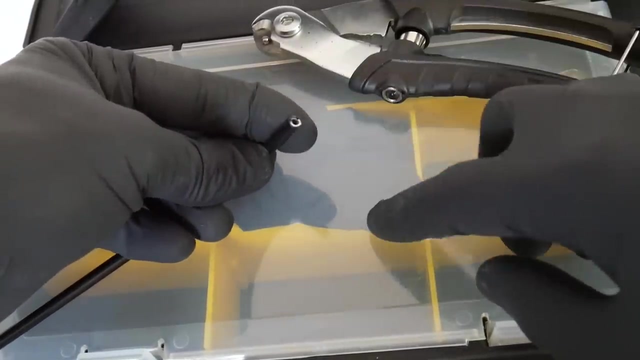 is nothing. sharp edges here, no sharp edges and nothing will will create friction between the housing and the cable. on some pro cutters you have some special pin something, something sharp, that will just help us to open up the housing so that it will be just nice and smooth for our cable. 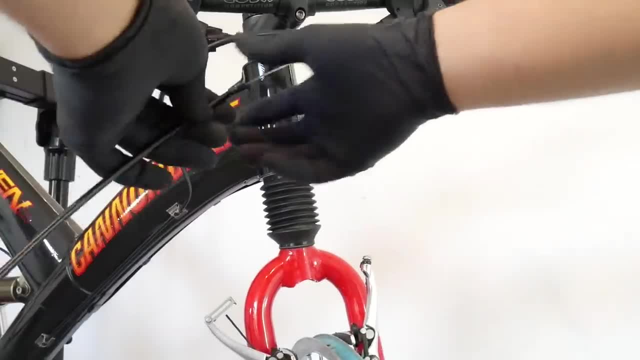 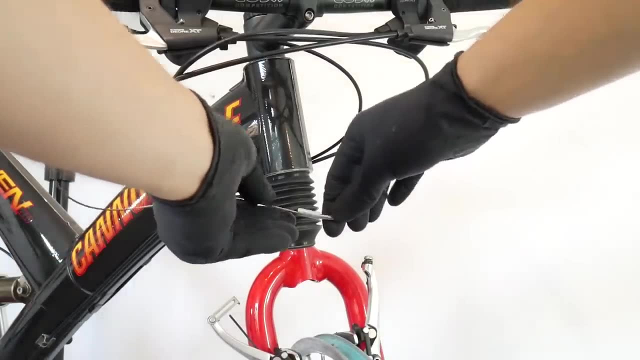 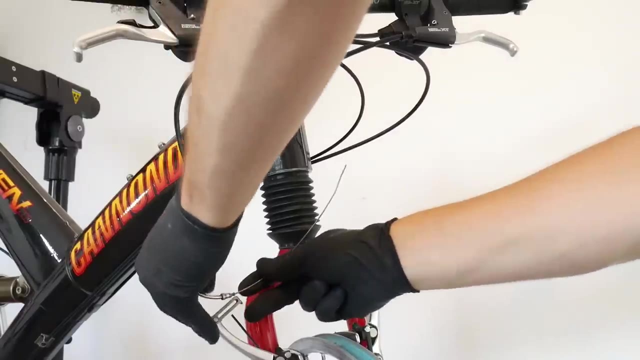 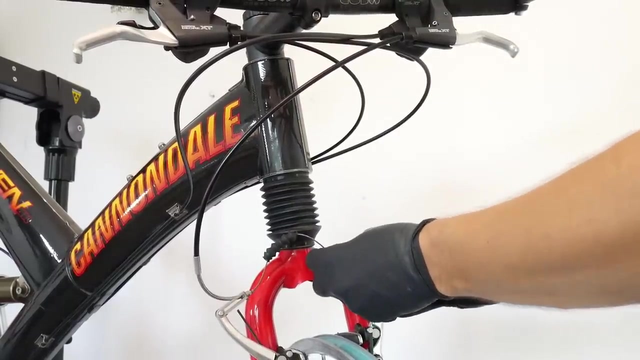 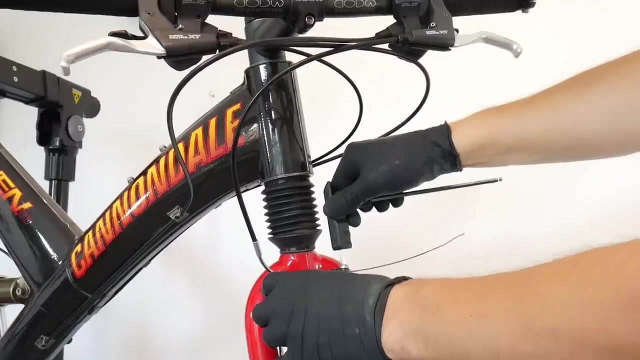 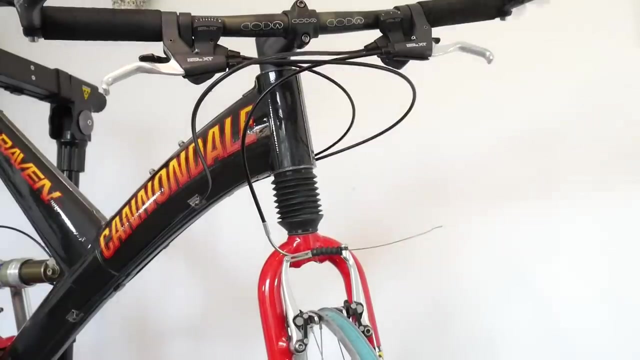 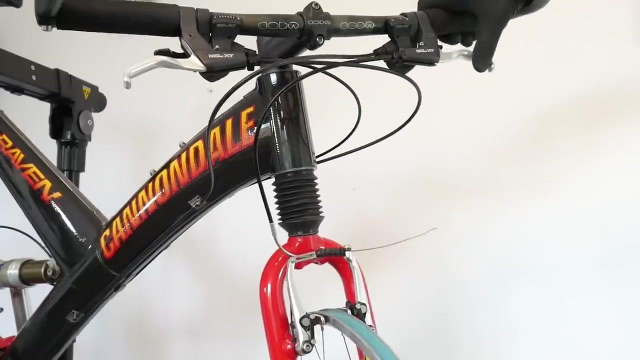 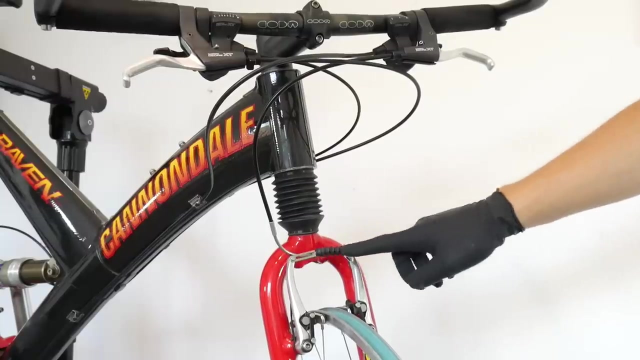 so shortening the front brake housing made so much difference. i can see that the turning is okay and while braking there is no sponginess because the housing is not flexing, and we have also almost perfectly straight line here between the two arms of the brakes. so this was really good. 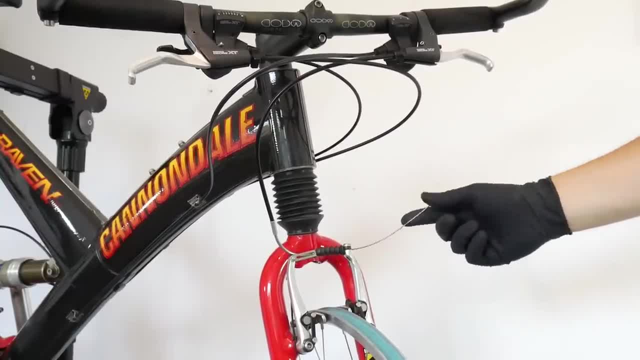 job. i have cut around 12 thousand second piece of fabric and i am going to show you how to do it and how to do it in this video. and i am going to show you how to do it in this video and a half centimeters of this housing. Also weight savings.